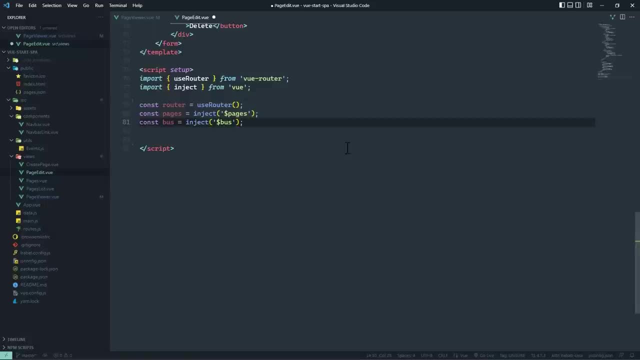 We'll start at the very beginning. And I'll teach you the fundamentals using just the Vue library. No build tools or tool chains required. 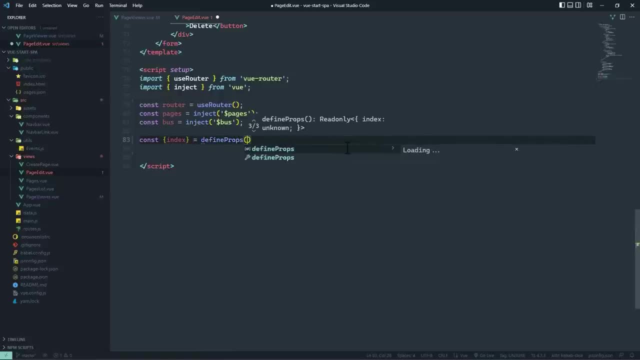 You'll learn how to create applications, define and use options, and organize your applications into smaller, more maintainable pieces called components. 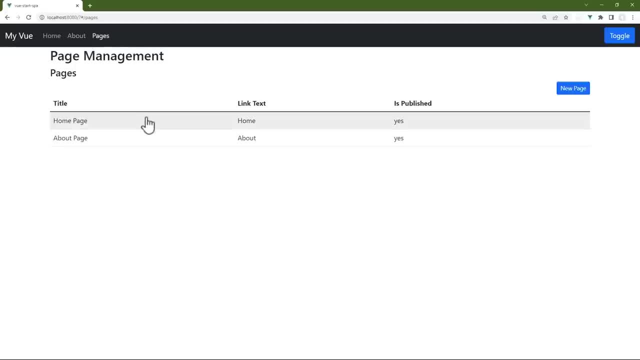 But then we will jump into the tool chain because it makes working on larger projects easier. You'll learn how to load and work with reactive data, how to handle user input, and create custom events that you can use in your applications. 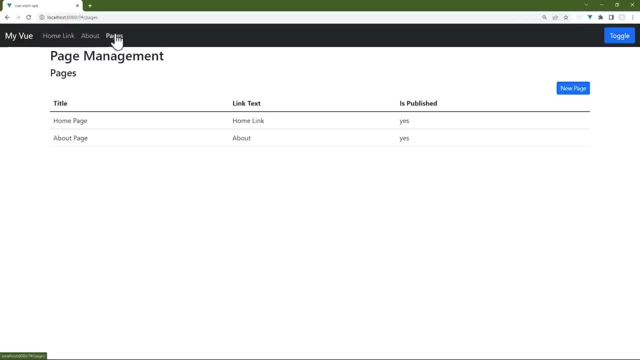 I'll also teach you how to manipulate style, create computed properties, and define objects that watch your data for changes so that you can react to those changes. 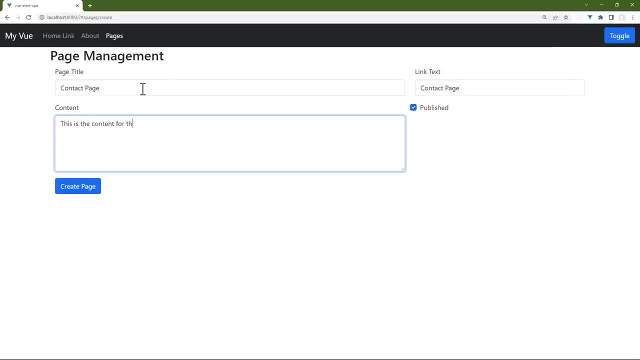 You'll learn how to create single page applications using the view router and how to use the composition API to improve maintainability. 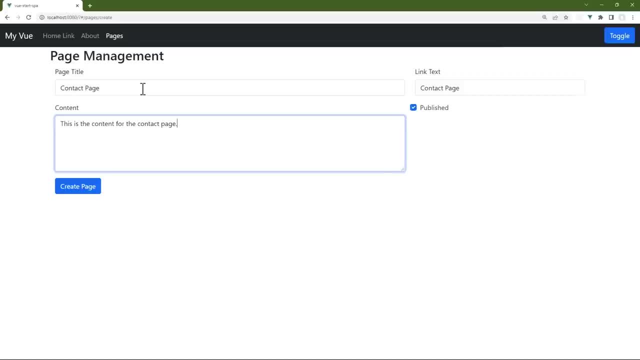 We have a lot of ground to cover, so when you're ready, queue up the first video and we will get started. 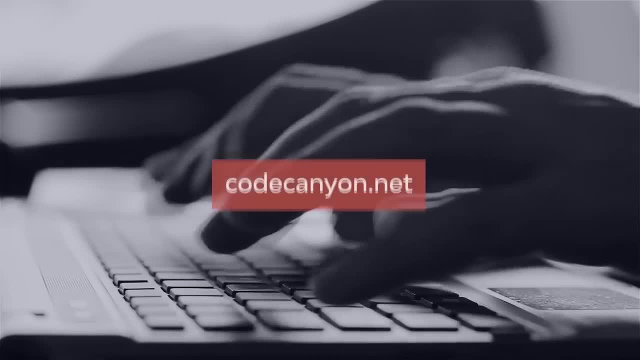 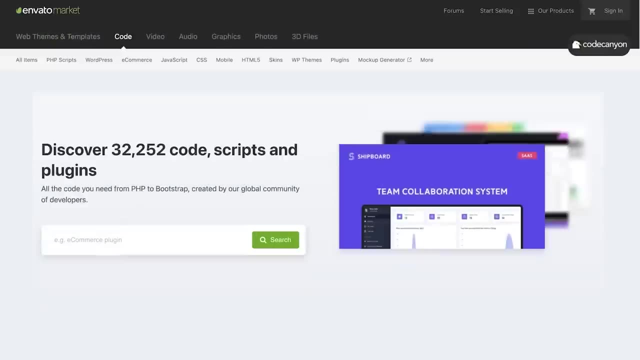 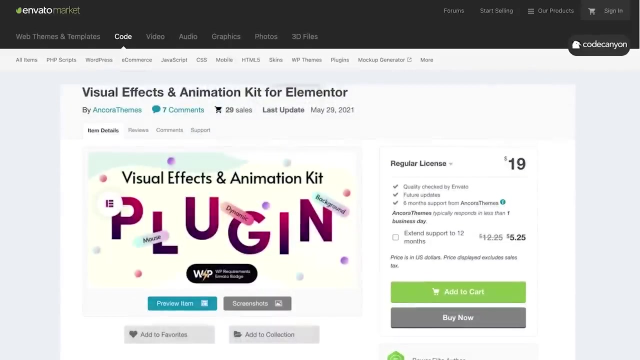 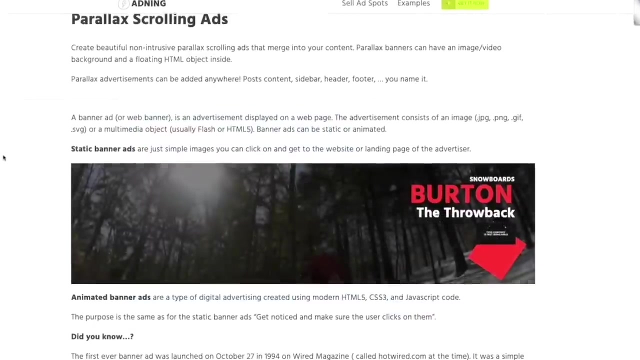 But first, if you're looking to create a professional website or you want to add features to make your website stand out, then head over to Code Canyon, the marketplace for high quality JavaScript and PHP components, HTML5 and mobile templates, and so much more. The items at Code Canyon can help you easily add the functionality and eye-popping visuals that you need to meet your business's goals. 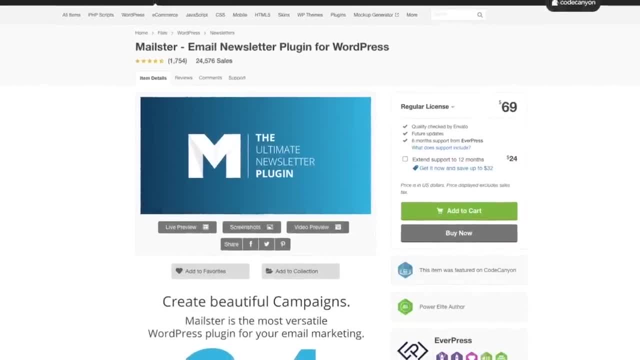 You'll find a massive library that contains thousands of JavaScript and PHP components. 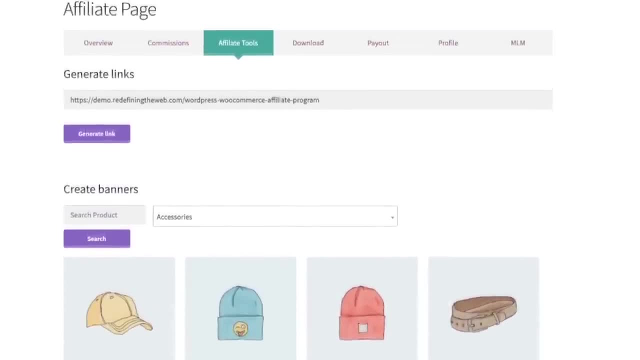 And almost 20,000 HTML and mobile templates. Needless to say, you'll find what you're looking for to take your site to the next level. 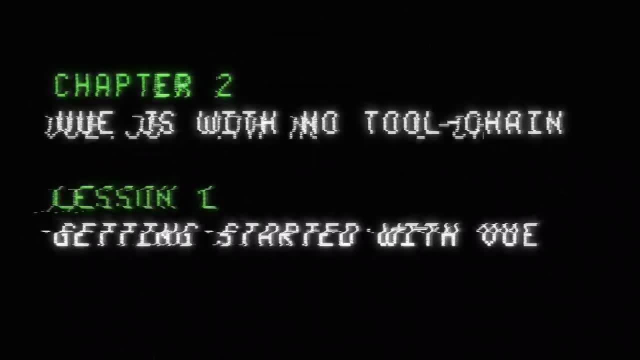 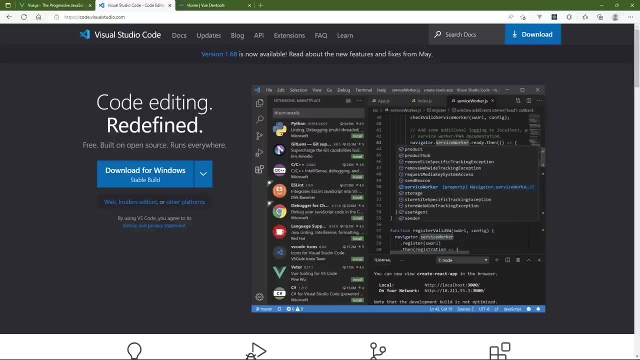 There are two things that I want to touch upon. First is your code editor. Now, technically, we are working with text. And we can use any text editor to do the work that we need to do. 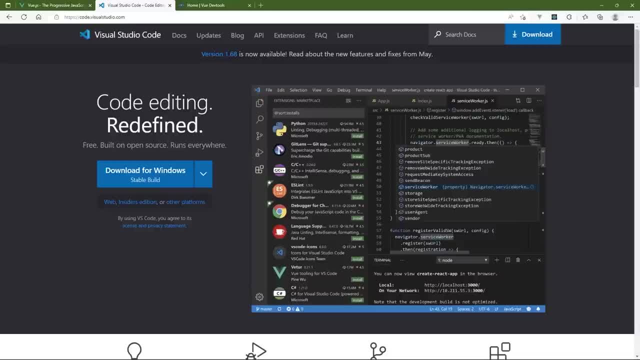 However, the text that we are working with is code. And code editors have features that make it easier to work with code. So I recommend using a code editor. There are many free and many that are not free. So feel free to use whichever one that you are comfortable with. I personally use Visual Studio Code because it's free. It's also cross-platform, and it is also the best code editor for JavaScript. But again, feel free to use whichever code editor that you are comfortable with. The second thing is the view dev tools. 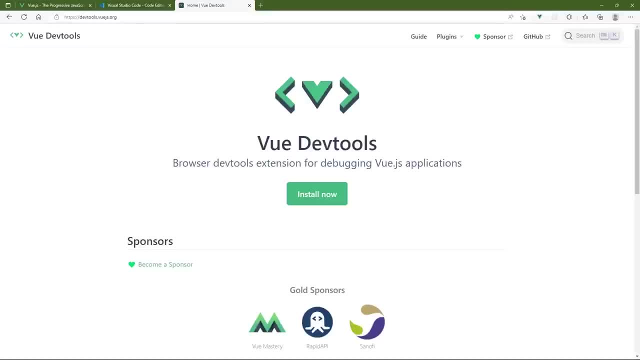 Now, these are tools that you install within the browser. They are used for 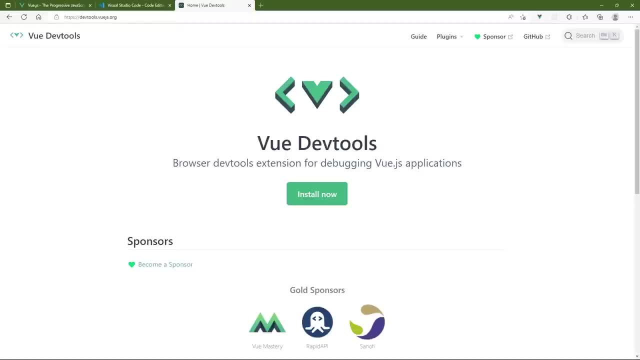 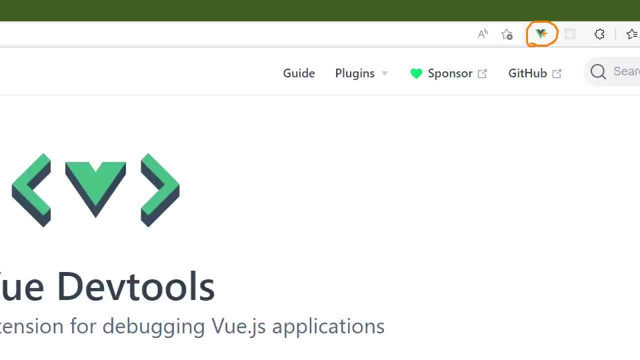 debugging, and you will see me use them throughout this course. In fact, if you look in the upper right-hand corner of the browser, you can see that I already have them installed. It's this view icon up here, and I recommend that you install this as well. 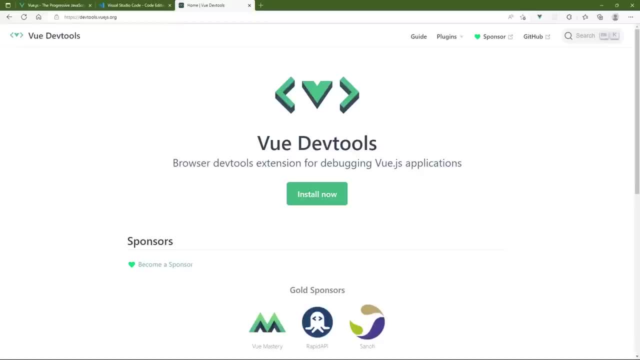 Of course, Firefox, Chrome, and well, everything else is based upon Chrome. So all of the browsers are supported by the dev tools. So once again, I recommend that you install them because they are very useful. 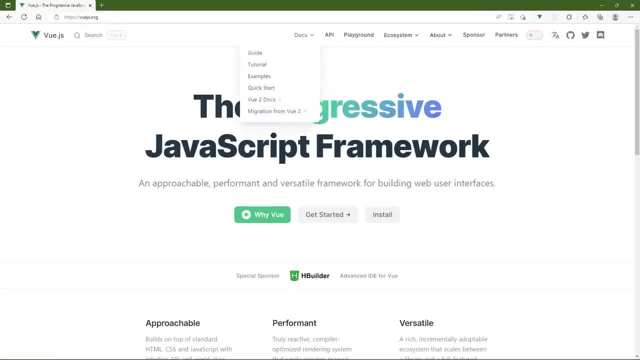 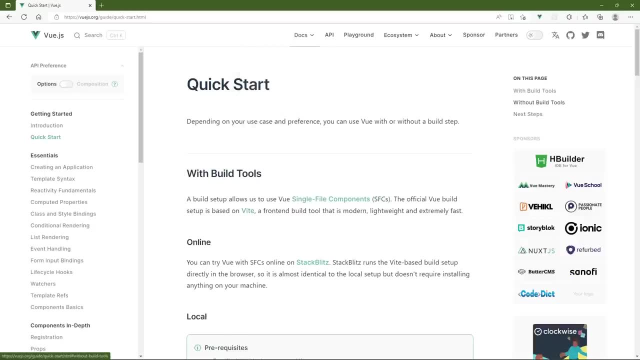 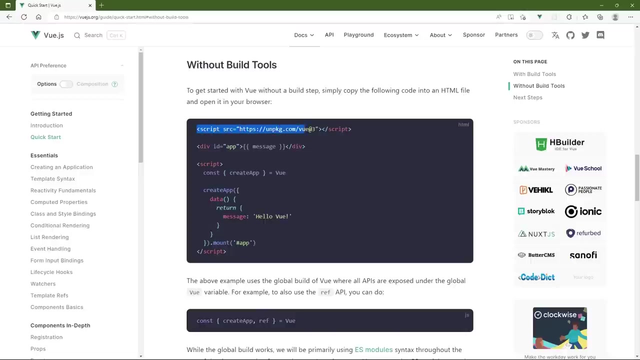 So as I mentioned, it's very easy to get up and running with Vue. So if we go to vuejs.org, let's go to the Quick Start, and there's going to be a section called Without Build Tools. Now, yes, eventually we will get into the build tools because, well, it just makes our lives a little bit easier. But for right now, let's go to the section Without Build Tools, and let's copy this first line. This is using the CDN, which is what we are going to do. So let's hop in. 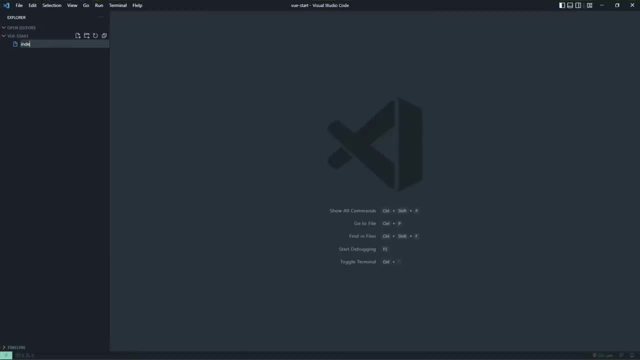 Let's hop on over to our code editor. Let's create a new file, which I'm gonna call index.html. And as far as the title is concerned, let's just call this Vue Basics. And then let's paste in that script element. Let's also go ahead and paste in the CDN for bootstrap, just so that we have things that don't use the default style sheet. And let's start with just some content that we are going to hard code into this page. 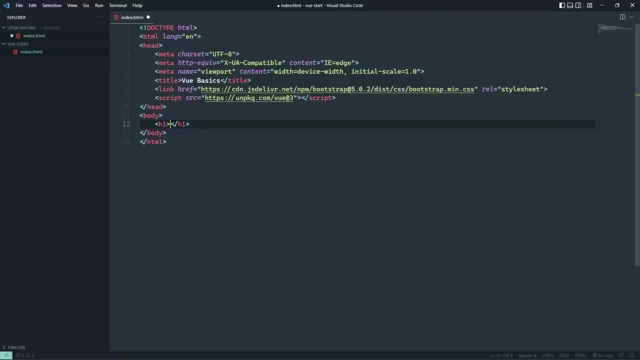 And eventually, we are going to use Vue to generate this content for us. 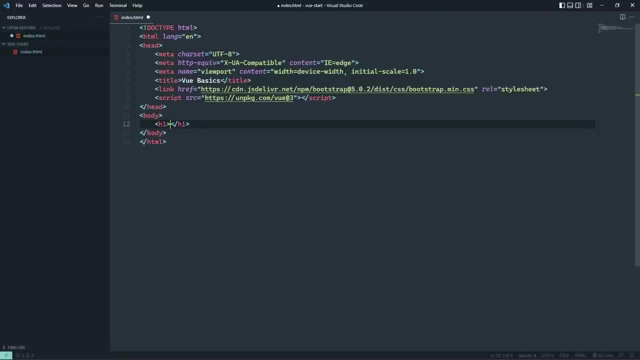 So we'll start with an H1, this is the title of our page. So let's just say hello Vue, and then we will have some content, 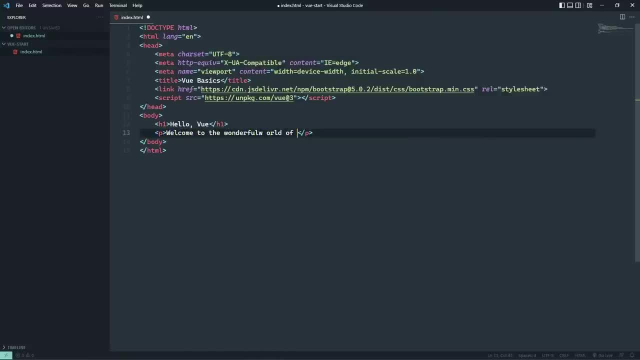 such as welcome to the wonderful world of Vue. 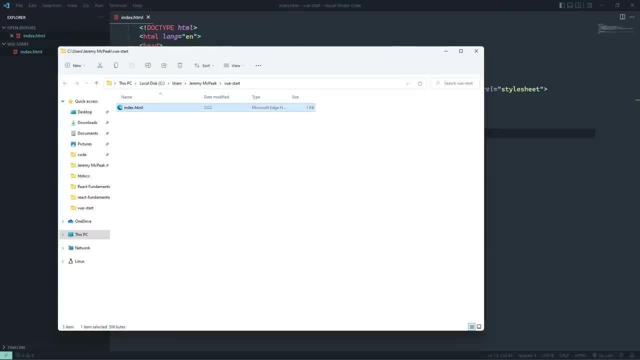 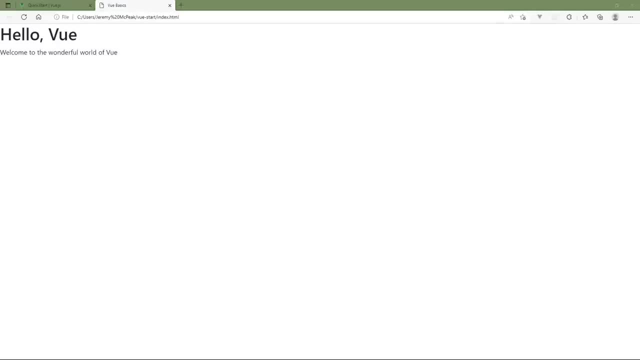 And then let's open this up in the browser, we can just double click on the icon. We aren't making any HTTP requests or anything like that, so this is going to be fine, and there we go, that's great. 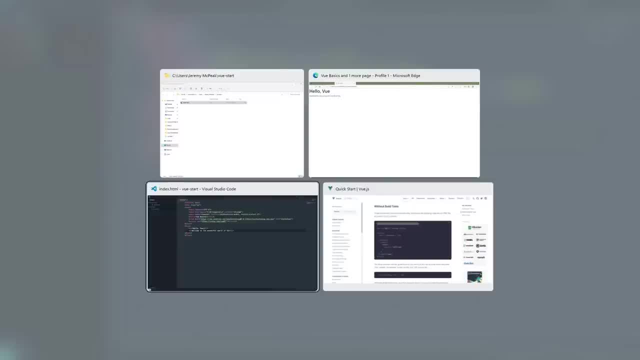 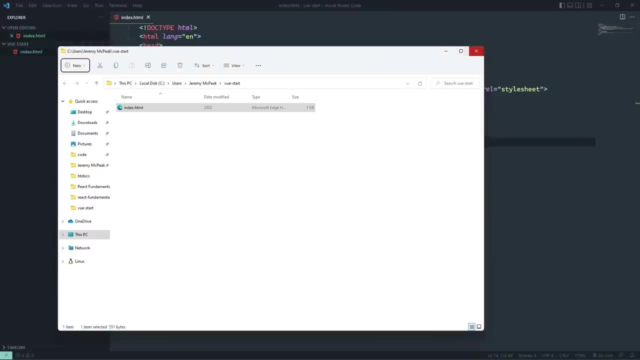 However, I want to add some styling here. So let's actually wrap this in a div with a container class, so that we can use bootstrap there. 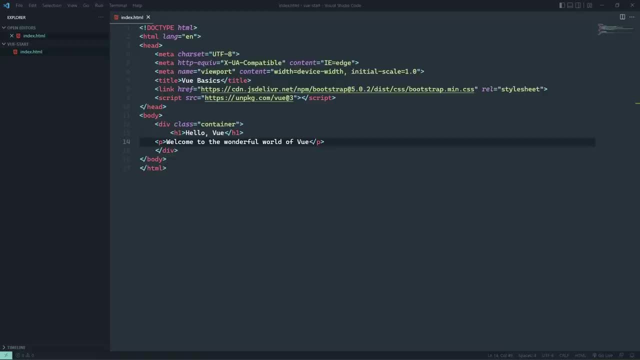 And as we refresh, okay, that got moved over, but that's okay. 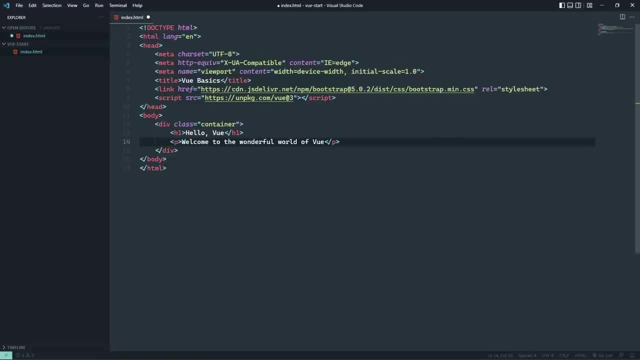 So we want to use Vue in order to essentially provide this same content. And we can do that by adding a script element to the bottom of our body, because we want this to execute after everything else has been loaded. And we are going to create a Vue application by using the Vue object. This is given to us by the Vue library, and we have a method called create app. Now I said that this is creating an application, which, hello, it's called create app. But this also creates what we typically call a Vue instance. 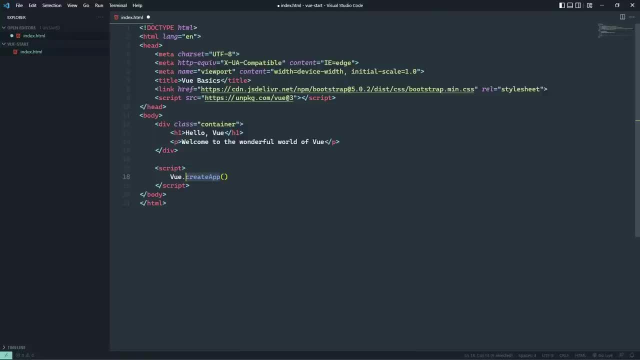 And one of the really cool things about Vue is that we can have multiple Vue instances within a single web page, 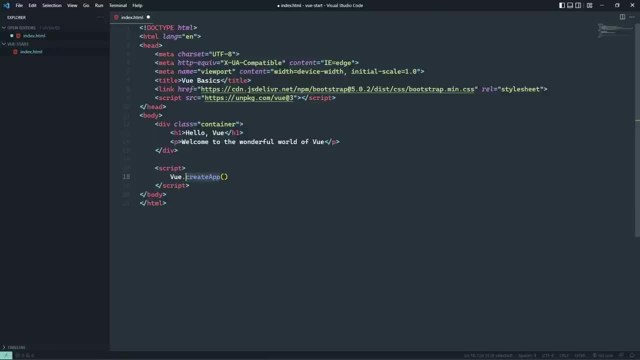 which is something that we will look at in the next lesson. But for right now, we're just going to work with one little application. 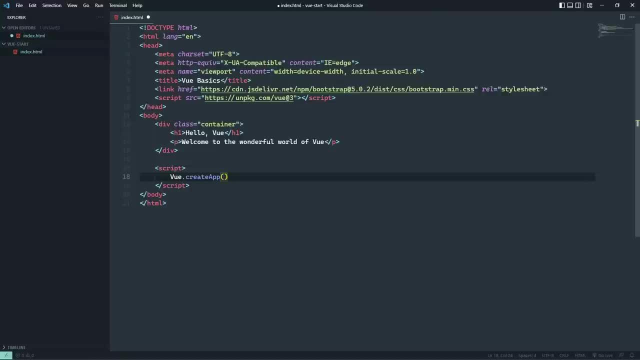 And we want to mount this somewhere within our web page. And we do so with the mount method. And then we specify the HTML element where we want to mount this. And, well, we want to mount this inside of our div element. 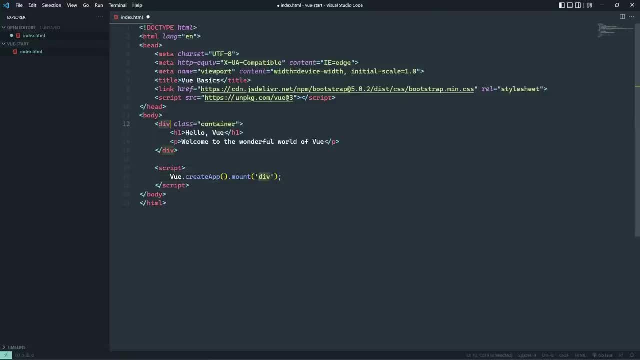 Now, this is a CSS selector, and right now we only have one div element. So this is going to be fine. 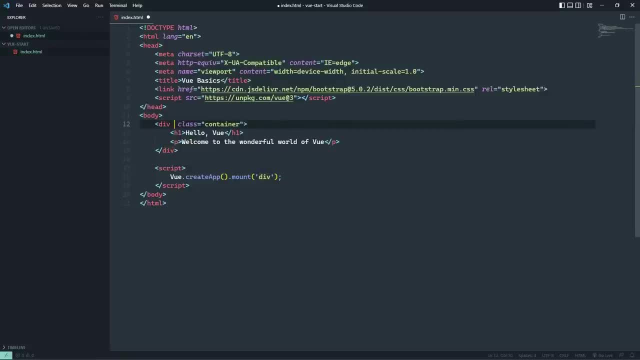 However, I think that we would be better served if we have some kind of unique identification. 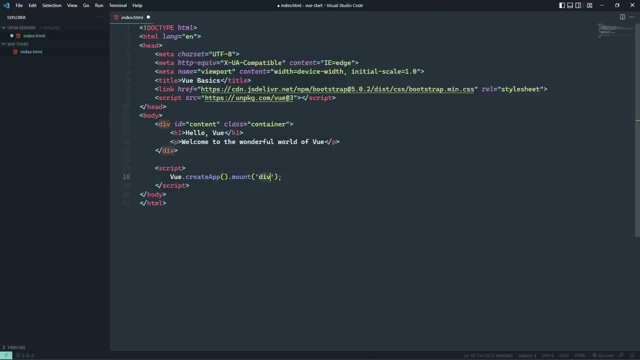 So let's just call this content. And so we will change our CSS selector to the ID of content. 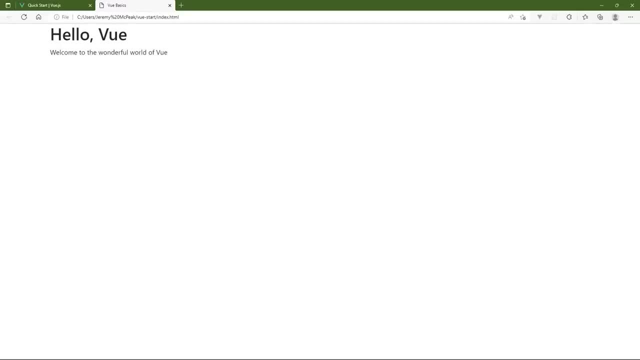 Now, if we view this in the browser, it's going to look exactly the same. There's nothing that's going to be different. 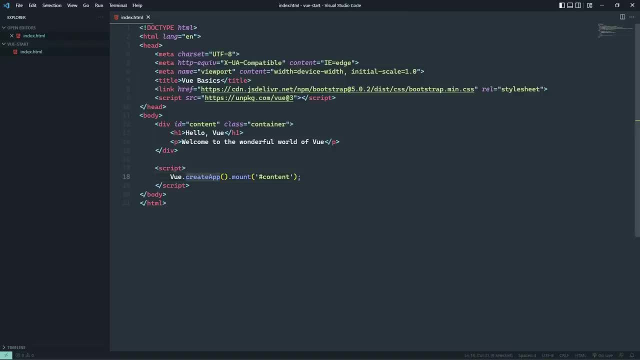 And that's primarily because, yes, we created a Vue instance, but it's not really doing anything. 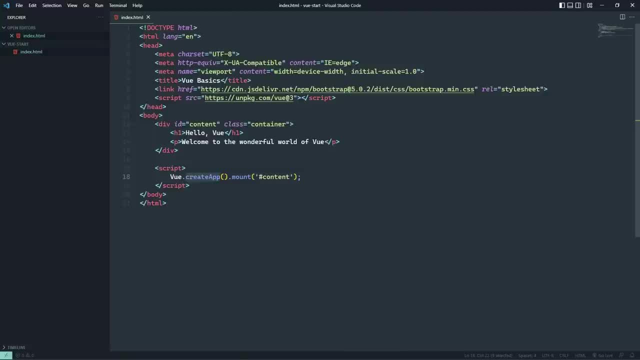 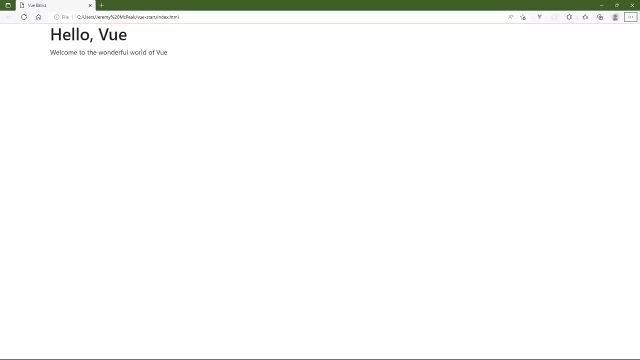 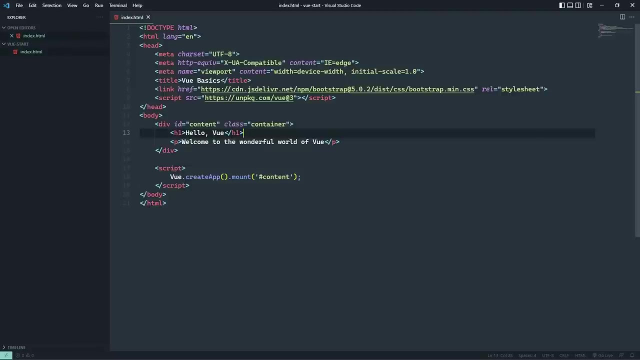 However, there's one very important thing that has happened behind the scenes. And that is, since we have mounted our application with this app, and, well, with this element with an ID of content. What we have inside of here is actually a template. And Vue is going to use this template in order to generate what we see inside of the browser. Now, of course, right now, our template is hard-coded HTML. But we want to soft-code this. We want to provide the data to our applications so that we can view them through our template. So we do this by passing what we call a view. So we do this by passing what we call a view. So we do this by passing what we call a view. 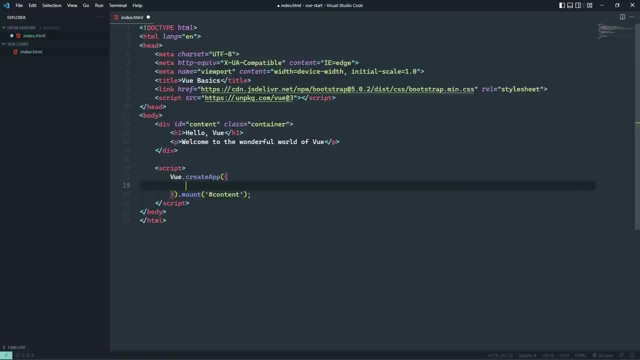 We call options to this create app method. The options is nothing more than an object. And the properties are, well, they're different options. The first one that we are going to look at is the data option. This provides data to our application. It is a function that returns an object. Now, if you're familiar with React, or other frameworks, this would be referred to as state. This is the state of our object. 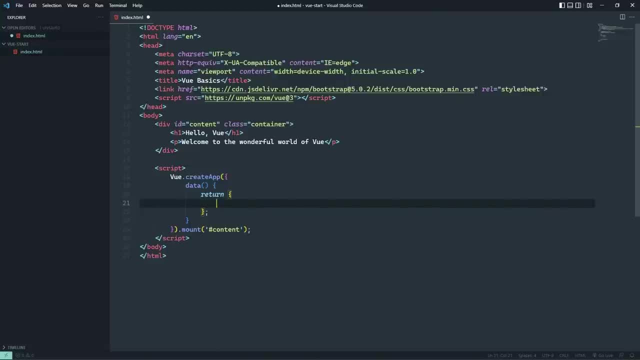 So we essentially have two things that we want our application to work with. The first is the title of the page, that string of hello view. So we are going to call this page title. And let's just go ahead and take that text. We'll cut it out of our template, and we will paste it as the string for our page title. 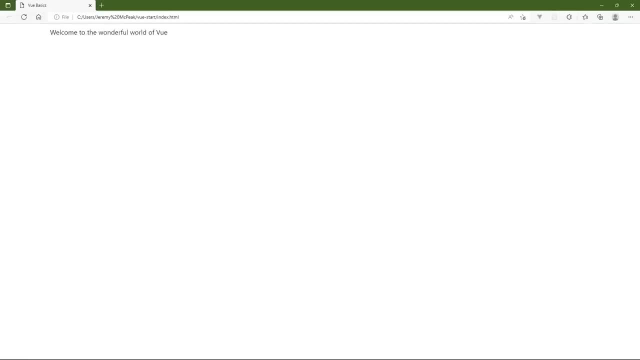 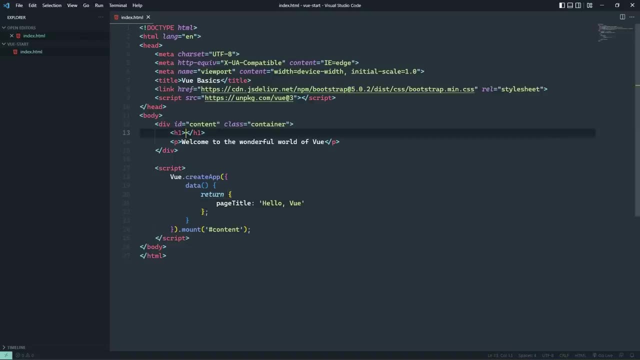 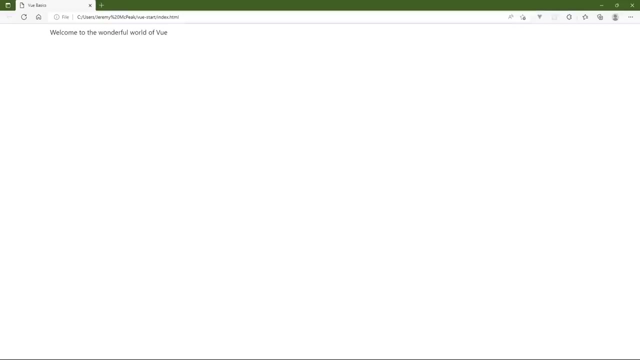 So let's hop on over to the browser, let's refresh, and of course we see that change. But of course, we want to display that page title. So we need to tell view where to display our page title within our template. We do that with a pair of curly braces. And then inside is our data property, page title. So if we go back to the browser and refresh, we see hello view. 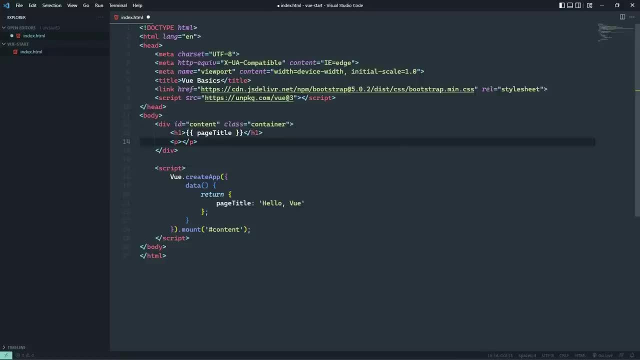 Let's do the same thing for our content. And let's just call this content. So we are going to use the templating. Syntax to output content. 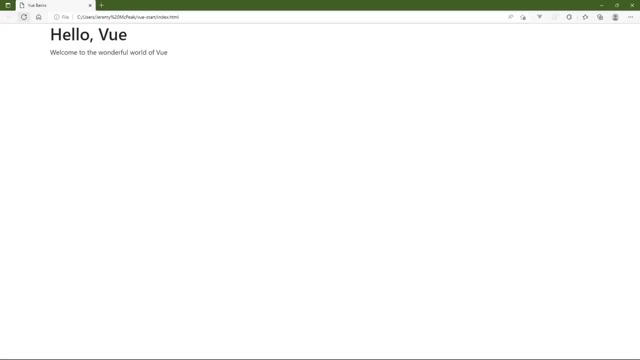 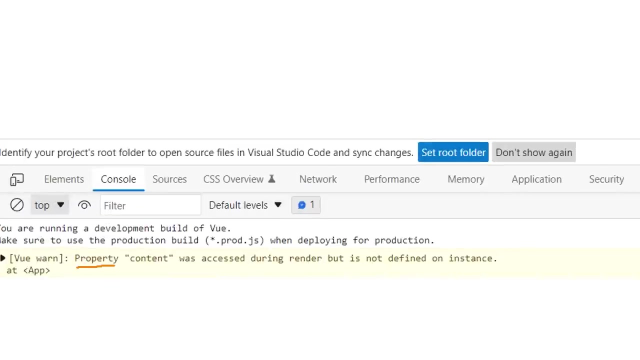 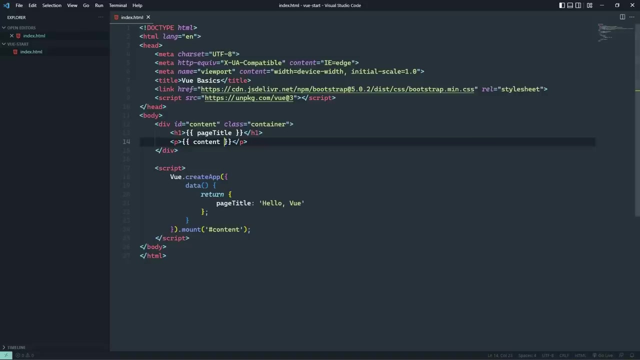 Now if we don't specify a content data property and we refresh the page, well, of course, we don't see anything because we did not supply anything for the content for our application. If we pull up the browser's developer tools, we will see a warning that the property content was accessed during render, but it is not defined on the instance. So essentially what that means is we've used content, but we've used content inside of our template, but we didn't define it within our application. So that's easy enough to do, we just need to add a content property to our data. 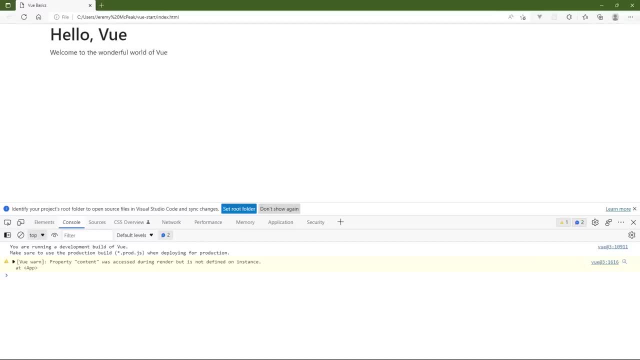 And now, whenever we go back to the browser, let's refresh, we of course see the content that we would expect to see, and the console does not have that warning anymore. 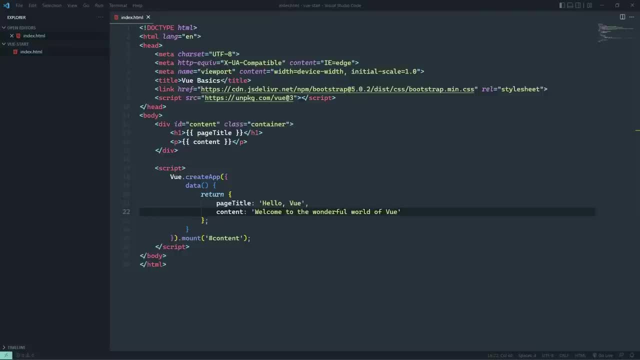 So we have now created our first view application. We did so by using the view object and calling create app. This created a view. In this view instance, we supplied an options object that defines the data that our application is going to use. We have two pieces of data, we have the page title and the content. We are mounting this application to an element that has an idea of content. 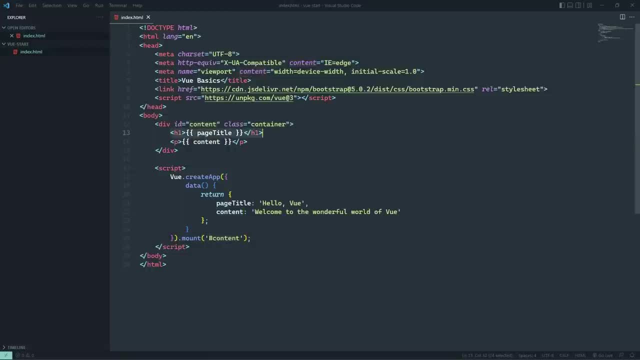 And in our template, we are defining where we want to display our application's data. 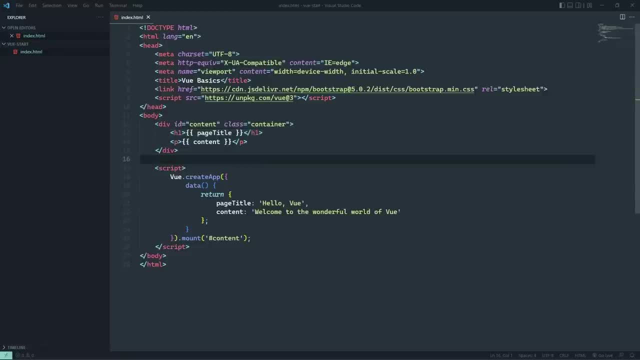 Well, in the next lesson, we are going to add another view application. This will be one that will control our application, and this will be one that will control our application. And this will be one that will control the navigation for our web page. 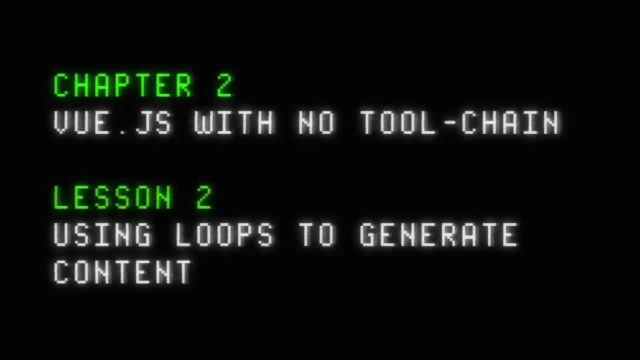 In the previous lesson, we created a very simple application to display some content within the web page. 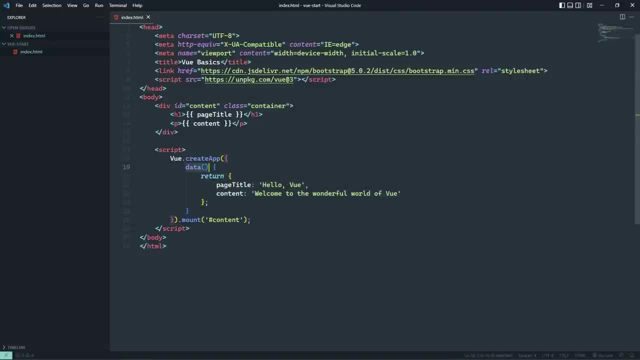 This application has two pieces of information or two pieces of data, the page title and the content. 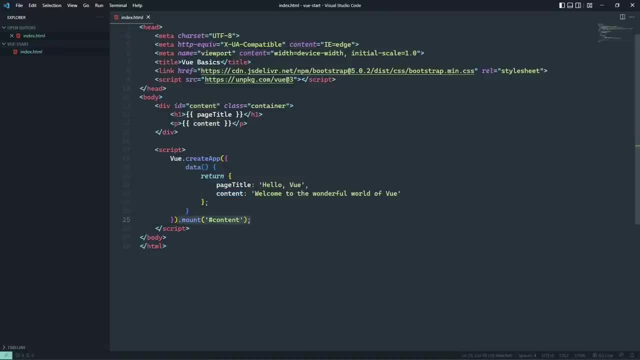 And we mounted this application in an element that has an ID of content, which is this div element. 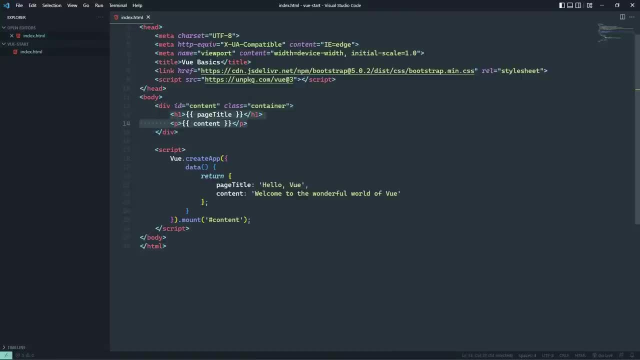 Inside of this div element, we have our templates where we specify where we want to display the page title and the content. 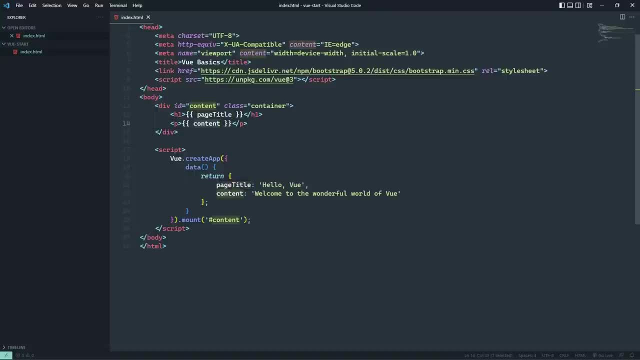 So in this lesson, I want to expand upon this. I want to create a new view application. Now, this doesn't mean that we have to create another web page. We can have as many view applications inside of the same page that we want. And sometimes we want multiple applications, sometimes we don't. 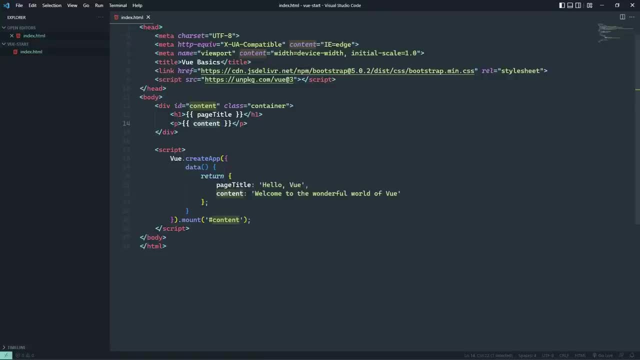 In this lesson, we are going to create an application that is going to control the nav of our web page. 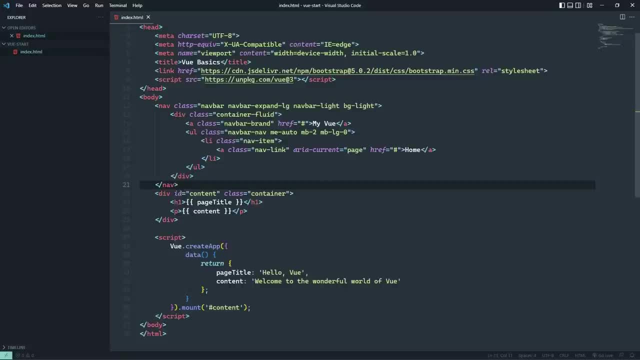 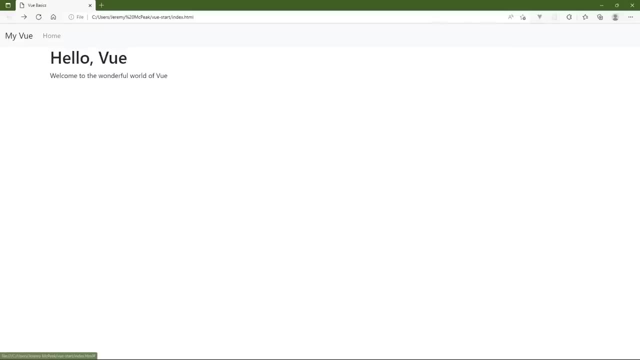 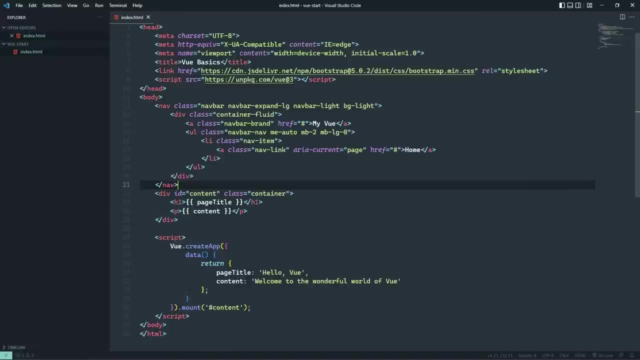 So I'm going to paste in the markup. For our navbar, this is just a typical Bootstrap navbar. If we go and look in the browser, there we go. We have the navbar brand, which is just my view. And then we have a single link of home. If you're not familiar with Bootstrap, if you wanted to add more links to a navbar, there is this unordered list. 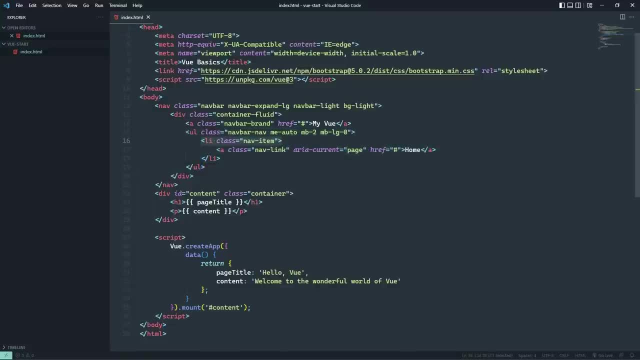 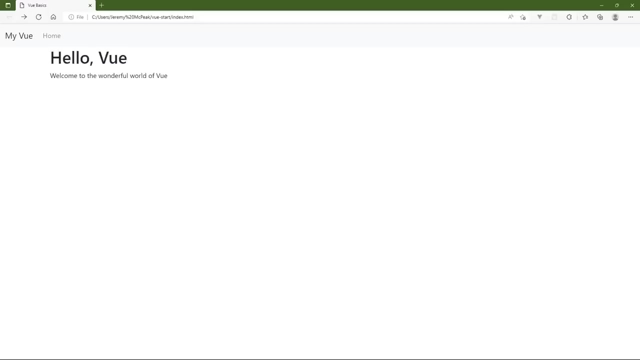 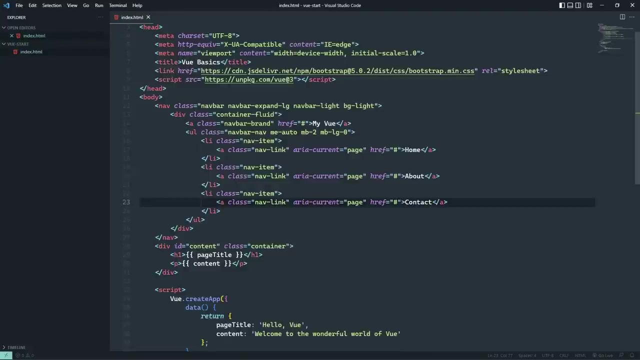 And each list item is going to be an item in that navbar. So here you can see that that is the home link. And if we wanted to add links for, let's say, about and contact, we would need to replicate that same markup. Change the text, and of course, we would also want to point to a different href. We'll get to the href later on. For now, I'm more concerned about generating the content of home, about, and contact. So we've done that with some hard-coded HTML. 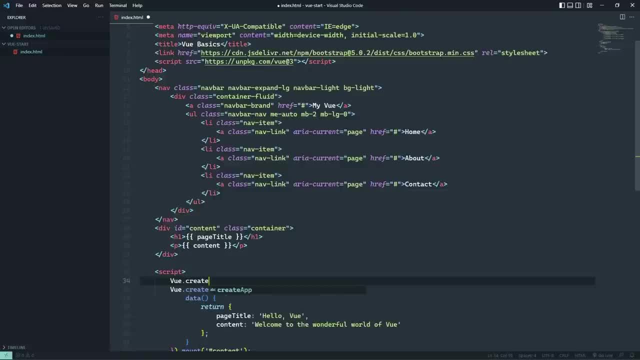 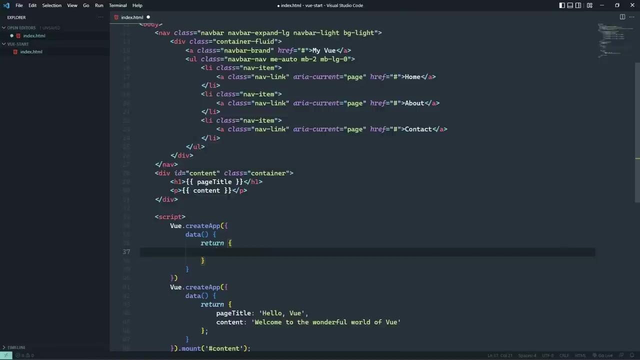 Let's use view to do that. So let's start by creating a new application. We're gonna go ahead and pass in our options object, where we are going to define our data. Because our data is going to define the links that this particular view application is going to generate. So let's have a property called links, which is going to be an array. And for right now, we're just going to work with simple strings, so that we will have home, about, and contact. 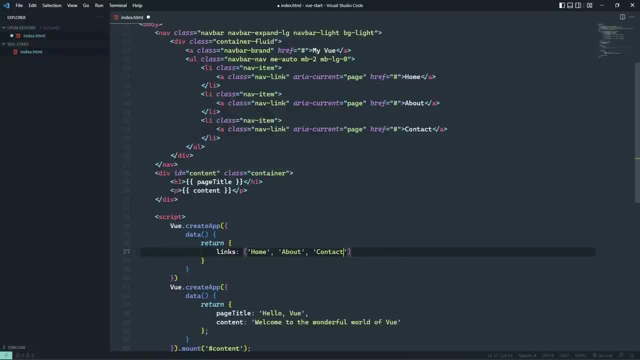 Of course, we need more information if these were going to be actual links, which we will get to that at a later time. 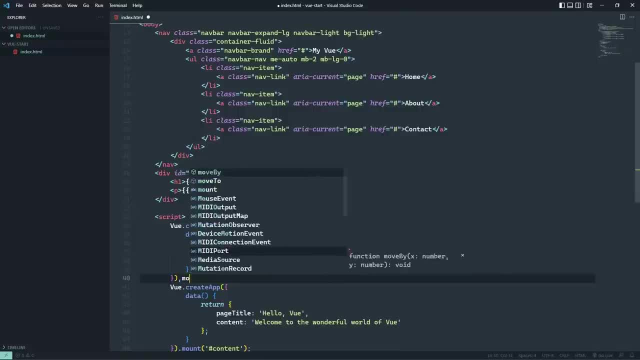 For right now though, this is going to be fine, and we want to mount this application to our nav. 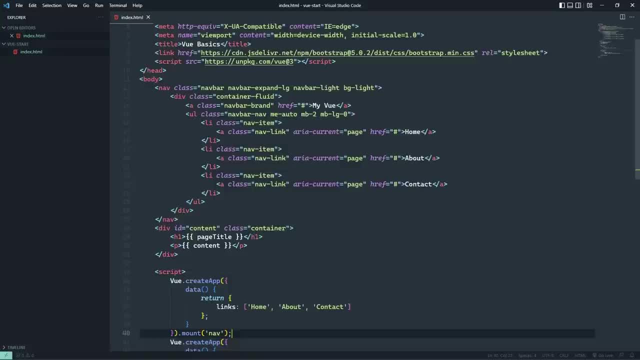 Now, for right now, this is okay, because I don't intend to have any other nav elements inside of the page. 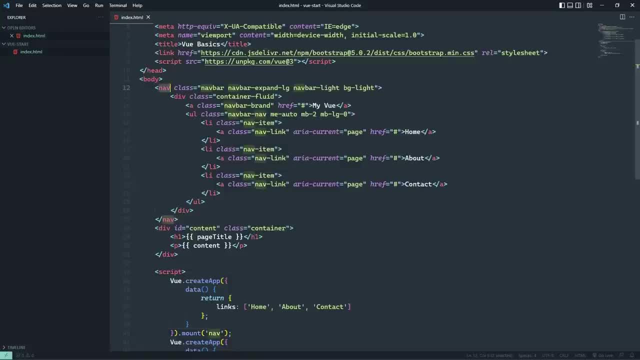 However, if it does turn out that we have multiple nav elements, then we would need to use something a bit more unique, but this is going to be fine. 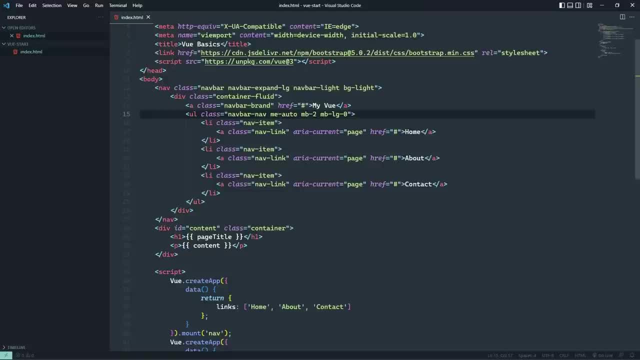 And so now that we have mounted this application to our nav element, that means that inside of the nav element, we have our template, and we can define where we want to essentially display 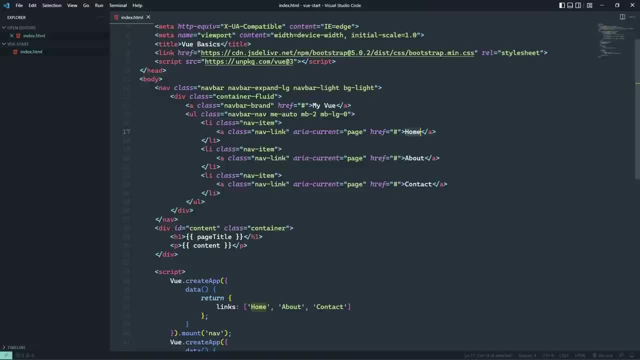 the text for our links, which are, of course, home, about, and contact. 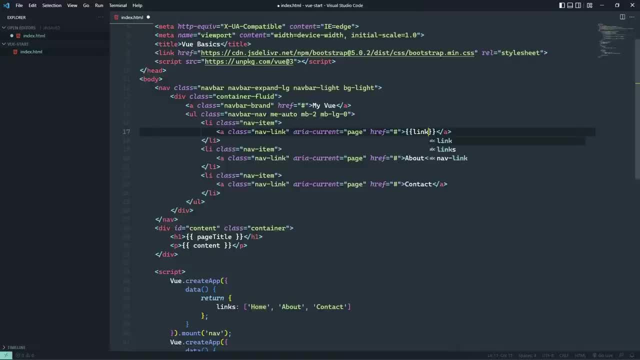 So one of the ways that we can do that is, well, like this. We can use the links array, and then specify the index of the value that we want to display. 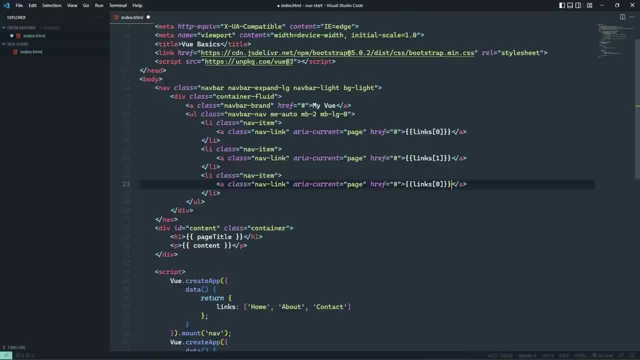 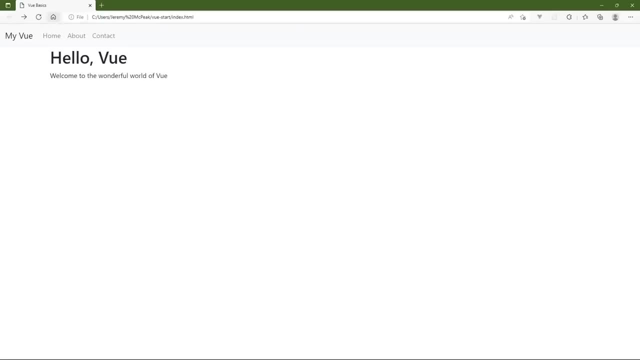 So home is index 0, about is index 1, contact is index 2. And of course, if we view this in the browser, we aren't going to be able to see, we aren't going to notice any differences in the nav bar. 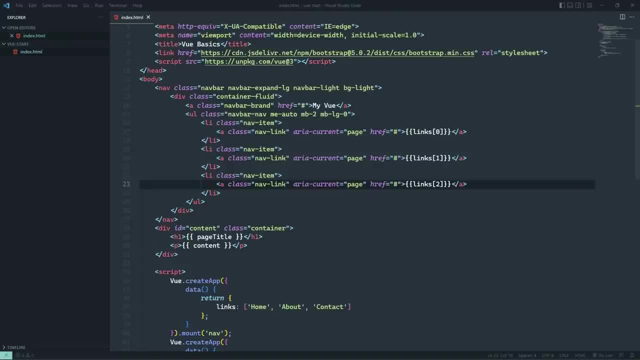 But that is a horrible way of going about this, because our links are in an array. And anytime that we work with an array, we typically want to use a loop. Now, if this were just normal JavaScript, we could do this in a couple of different ways. 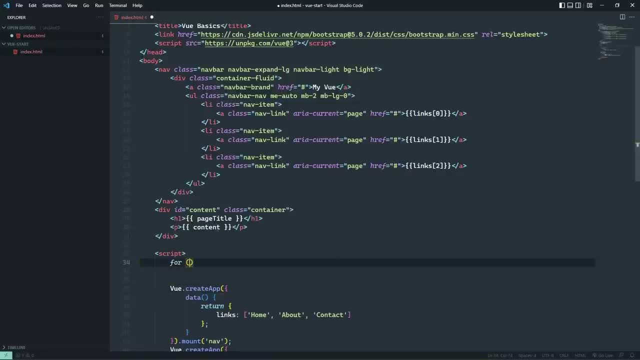 One of them would be to use a for in loop, so that we could say for link in links. 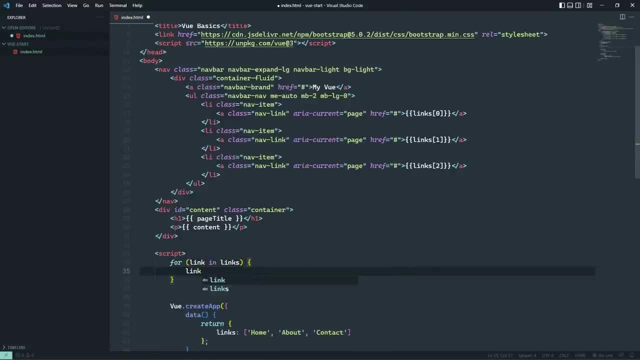 And then inside of that for loop, we could use the link in order to reference the value of home, about, or contact. 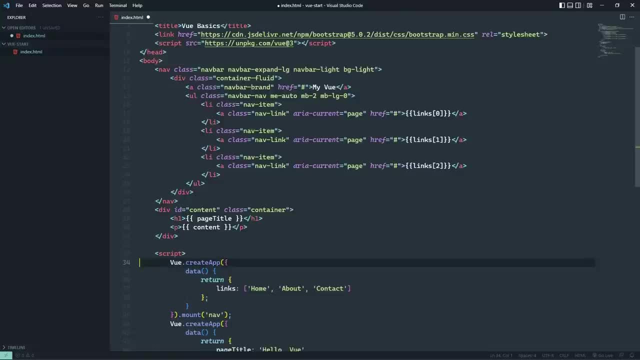 Well, we can essentially do the same thing with view, except that we don't do it inside of our JavaScript. Instead, we do it inside of our template. We use what's called a view directive. A view directive starts with v dash, and then there are many different directives. In our case, we want to use a loop. 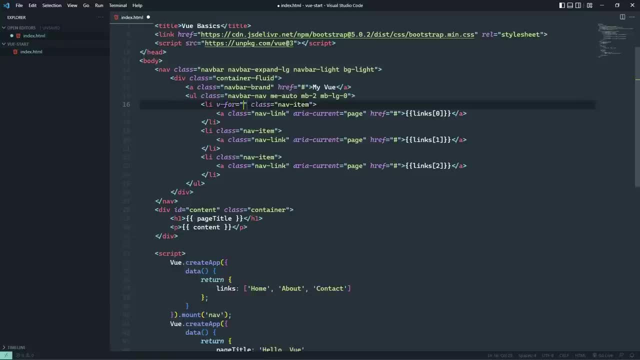 More specifically, we want to use a for loop, and it's going to look a lot like a for loop. 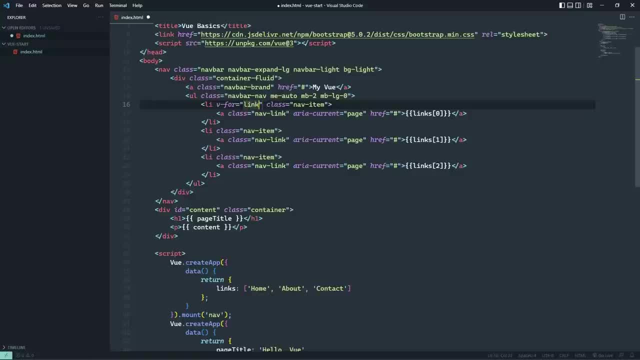 We want to use a for in loop, so that we can say for link in links, do this code. 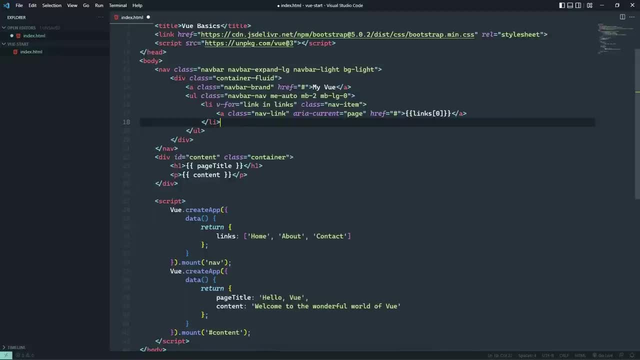 So I want to be very clear here, in that we are using the v for direct. This is a for loop, but we are using it on the li element. So we want to use this on whatever element that we want to repeatedly generate. If we used v for, on the ul element, then that would generate multiple unordered lists. 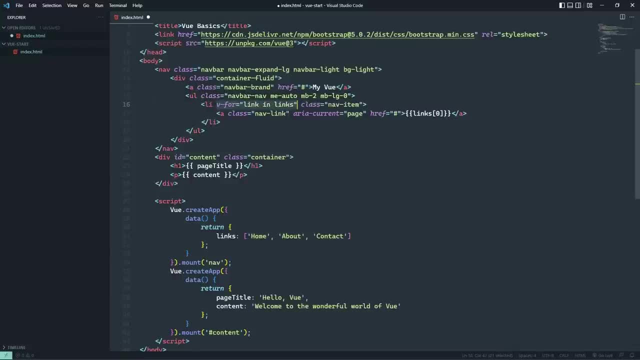 And we don't want that, we want multiple li elements. So for each link in links, we want to work with the individual link. 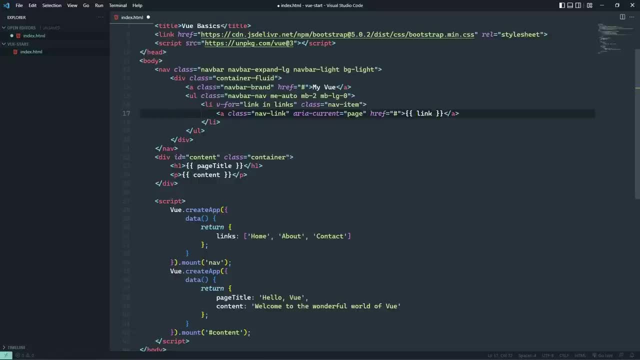 So when it comes to outputting the value, we just use link, which is defined inside of our for loop. 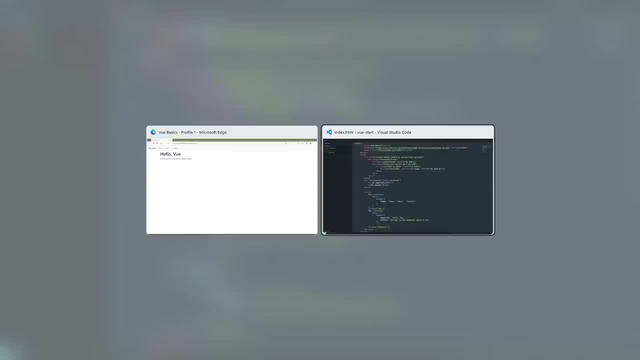 Whenever we go back to the browser and refresh, we see the same results. Now to prove that this is indeed generating data, we're going to go back to bring the links from our links data. 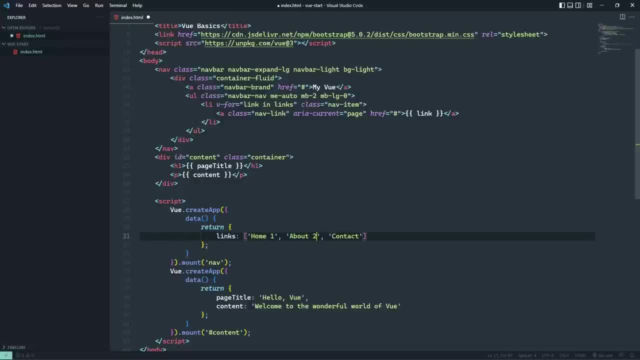 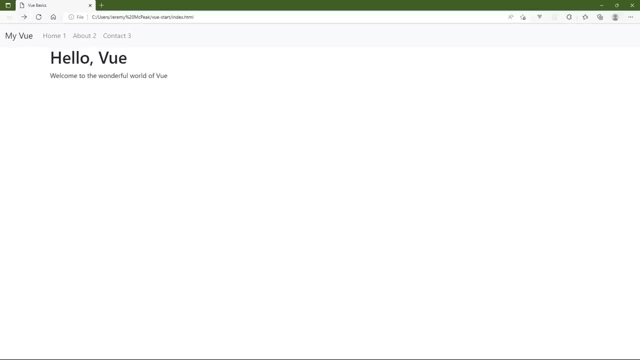 Let's change the text here, so that we have home one, about two, and contact three. If we go back to the browser and refresh, home one, about two, and contact three. 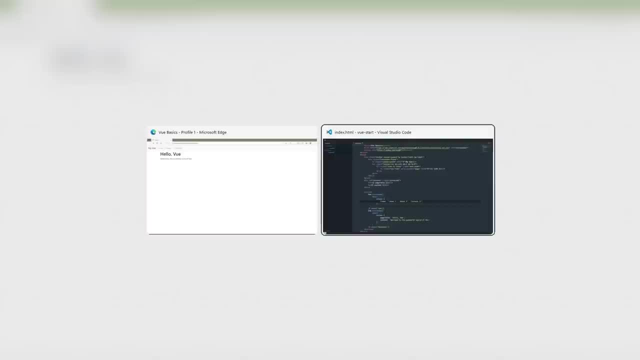 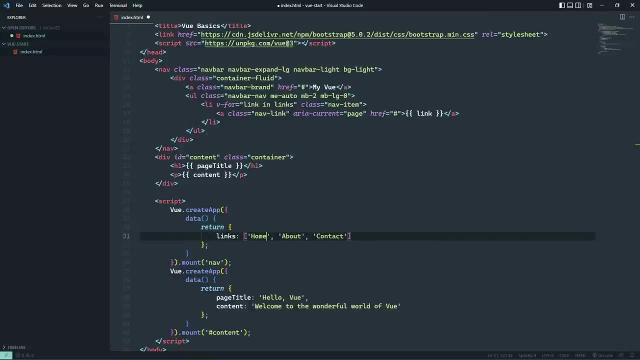 Now, this is very, very different from something like React, where you would generate your elements with JavaScript, and then output the results in the template. 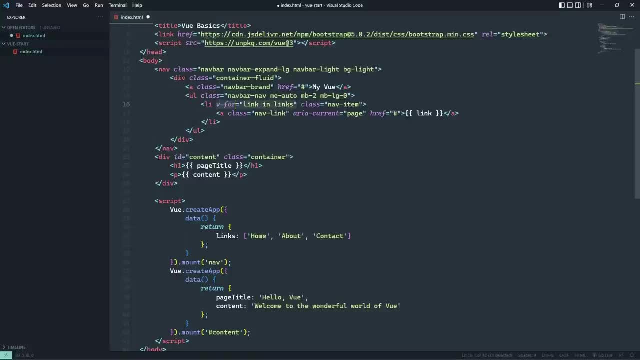 Vue uses a very declarative syntax, so that the goal is to generate a list of links so that you can read your template and understand exactly what is being output. 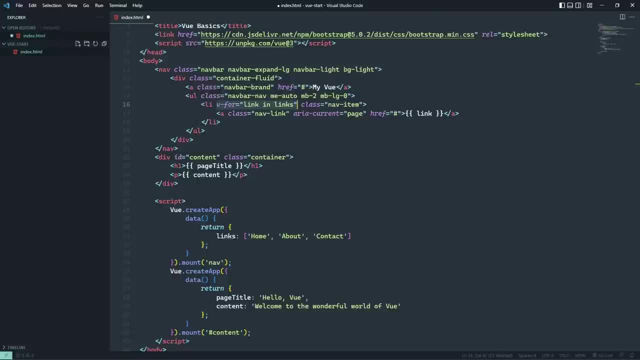 Now, in the next lesson, we are going to take this a step further and generate some actual links, so that we can navigate to different pages within our website. 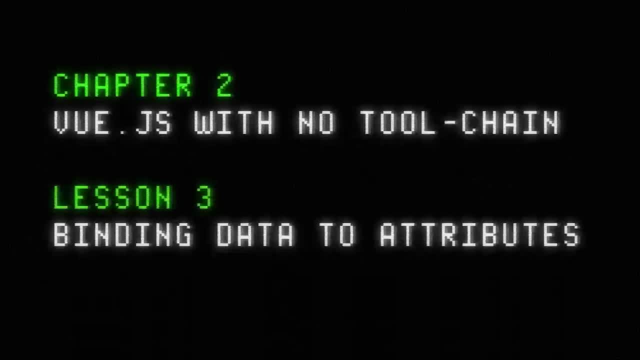 In this lesson, we are going to build upon the links that we created in the previous lesson, because as it is right now, well, they're just basically text. 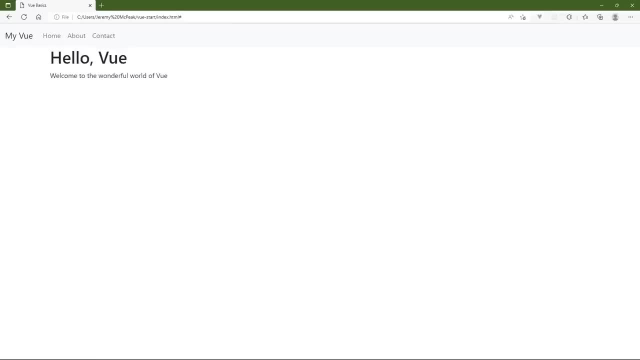 Of course, they are actual links, because they have href values, but it's set to. 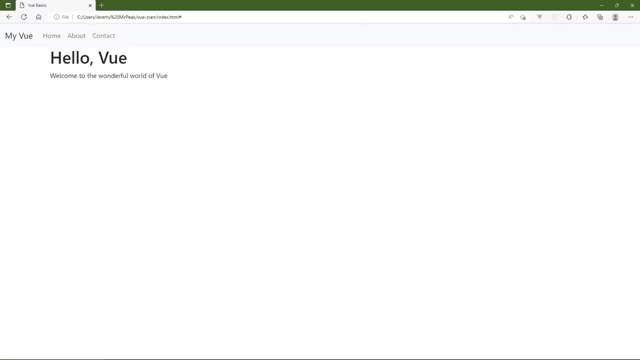 A pound sign or a hash. So we don't really go anywhere whenever we click on these links. 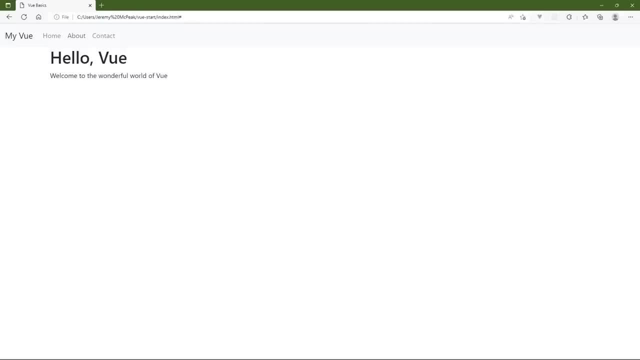 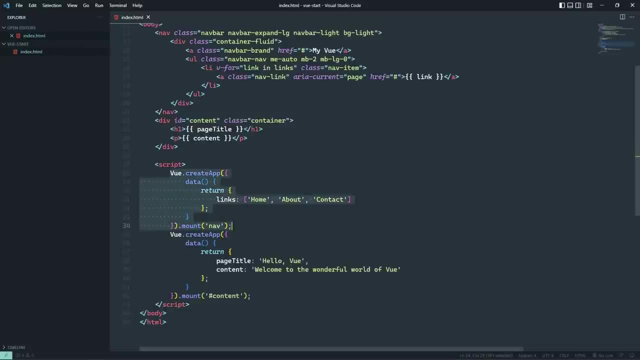 We want the user to be able to go to the home, about, or contact pages. Now, remember that our navbar is controlled by a Vue application. And the links are generated based upon that application's data. The data is an array called links, which has just simple string values. So if we want to generate actual links that go to an actual page, we need something more than just strings. 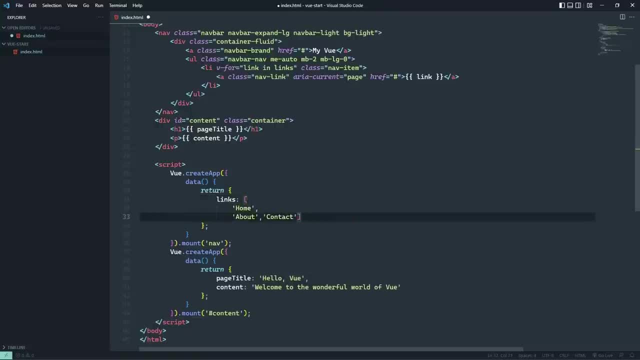 We need, really, an object, because an object can aptly describe a link. It can give us the text, as well as the URL that we want to navigate to. So I'm going to change the links array, so that it is an array of objects. Each object has a text property, and it has a URL property. Now, because I've changed this array, we need to address our template. Because we were outputting just a simple string value with this link variable. But now this is an object, so we want to say link.text. Because inside of the double curly braces, we can use any JavaScript expression that we want. 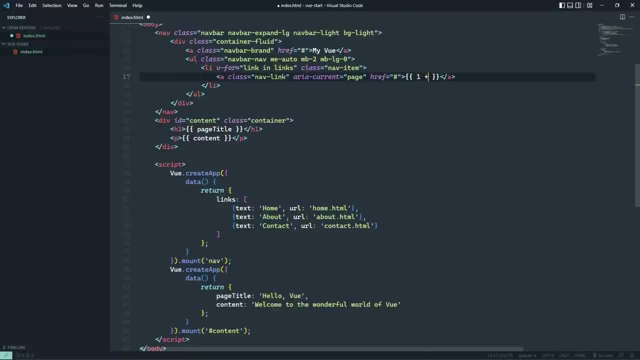 If, for whatever reason, we wanted to output 1 plus 1, we can do that because that is a valid JavaScript expression. 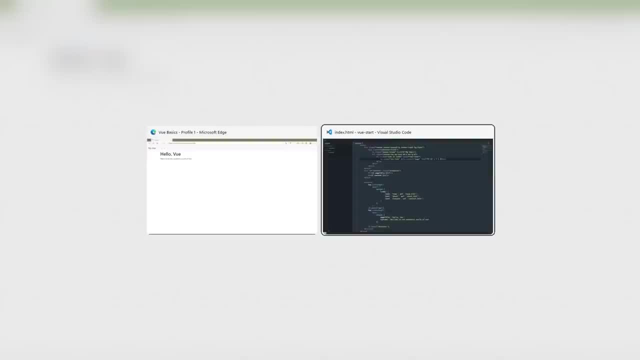 Of course, in the browser, we're going to see 222, that's not very useful, so let's change that back to link.text. 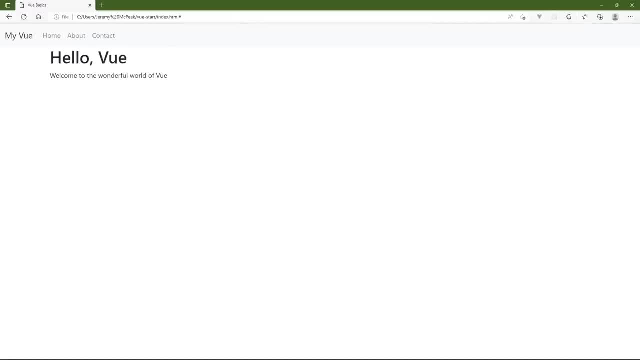 And if we take a look at this in the browser, we are going to see the results that we had before, home, about, and contact. 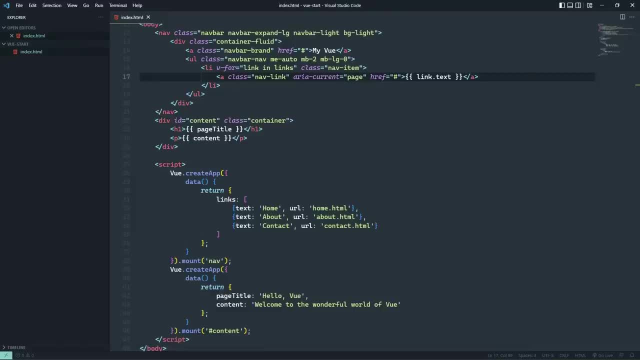 Now, Vue is a framework for building user interfaces. And as a web page, our interface is HTML, CSS, and JavaScript. And when it comes to outputting HTML, yes, we can output text, but there's more to it than just text. 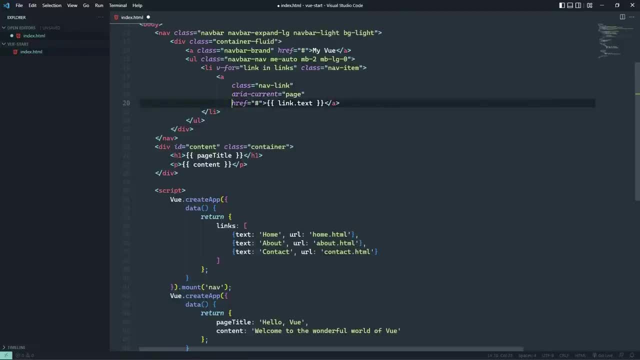 We also need to be able to set the values of HTML and Vue. 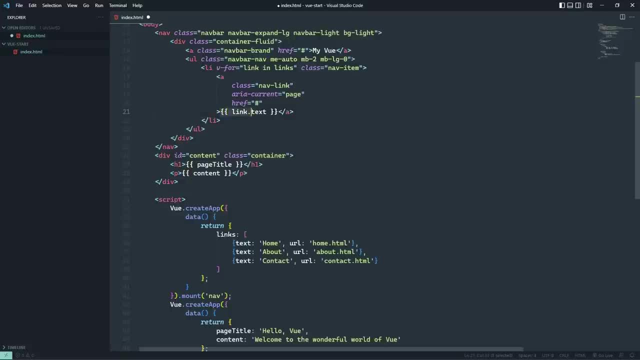 Attributes. So because we used the double curly braces to output text, 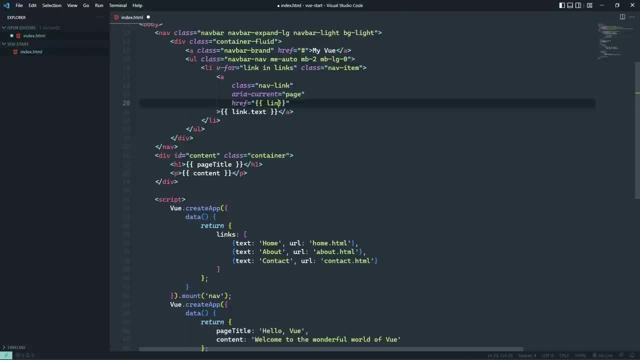 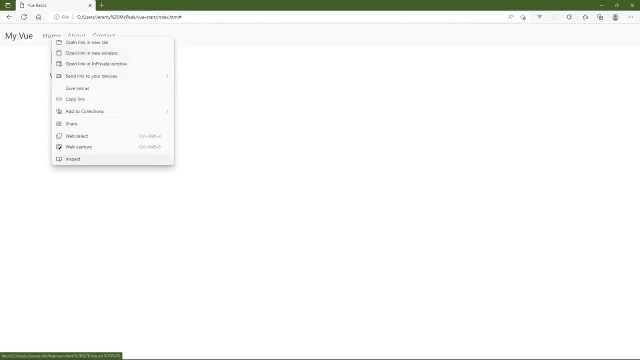 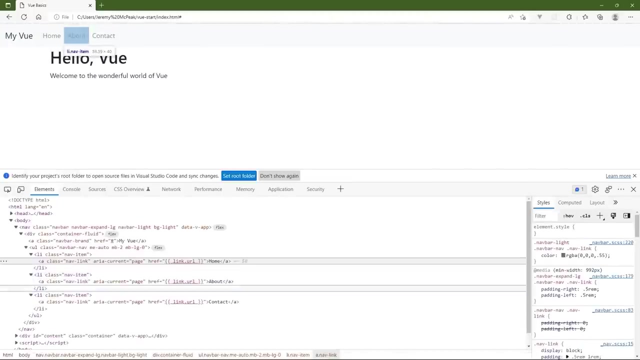 you might think that we would need to use that to do the same thing for the URL. So let's give that a try. Let's make that change. Let's go to the browser. Let's refresh, and let's pull up the HTML inspector so that we can see exactly what is being loaded in the browser. 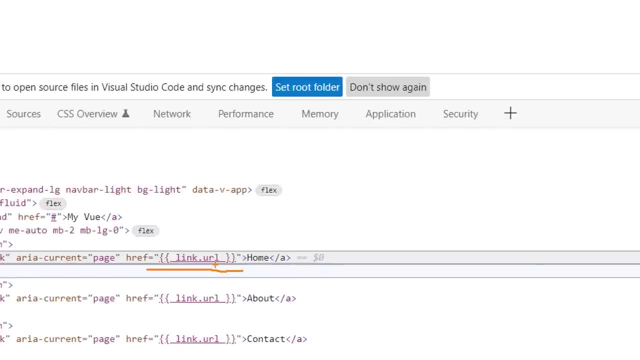 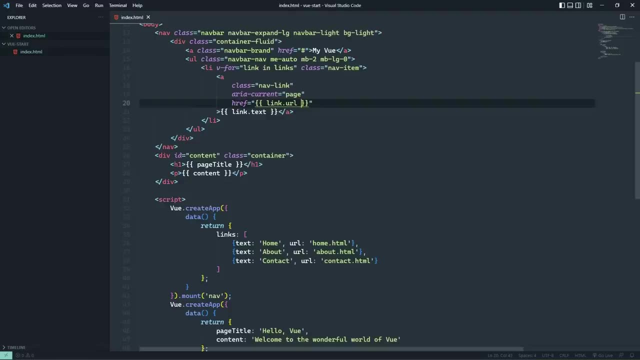 And we can see, well, link URL inside of a pair of curly braces. We see the exact string that we set for that attribute, which makes perfect sense because this is an href attribute. We need to tell our Vue application that we need to handle this a little bit differently, this needs to be special. So what we want to do is use a directive called vbind. Then we follow that up with a colon, followed by the HTML attribute that we want to bind a value to, in this case, it's going to be href. and then, then, and then the value that we assign to this attribute is a JavaScript expression. 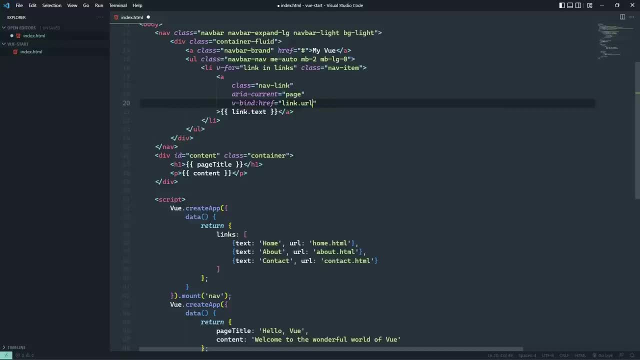 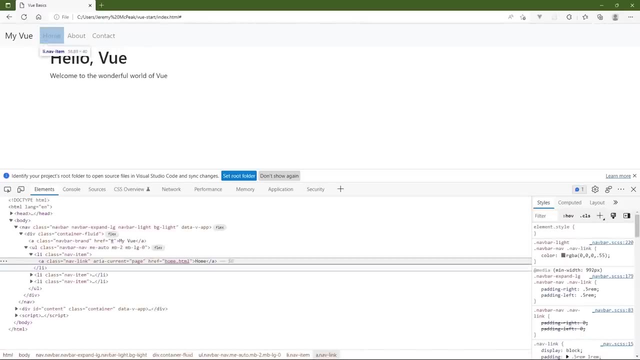 So we don't need the double curly braces, instead, we just need link URL. So that whenever we go back to the browser, we are going to see the results 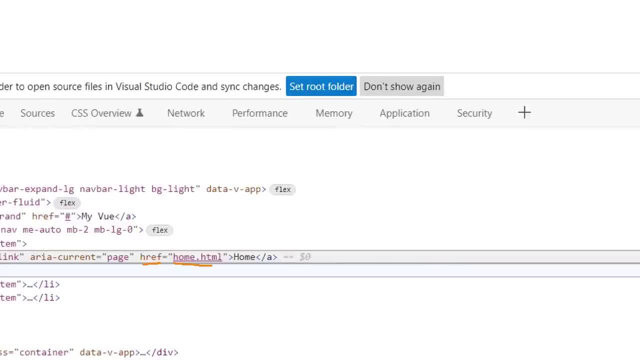 that we would expect to where the href is set to the URL property on our link object. 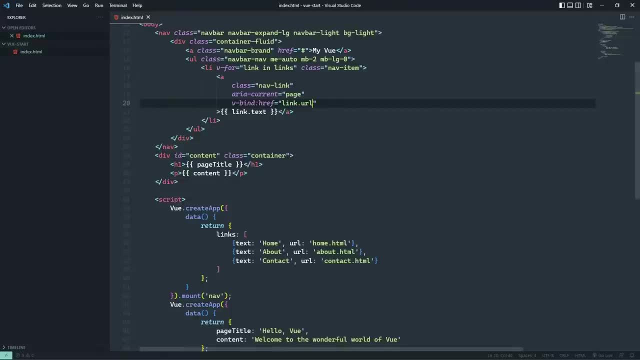 Now, binding data to an attribute is very, very common. So one thing that you're going to find is that if you have a link object, and you're going to find in the majority of projects that you look at is something like this, simply a colon, because we bind a lot of data. 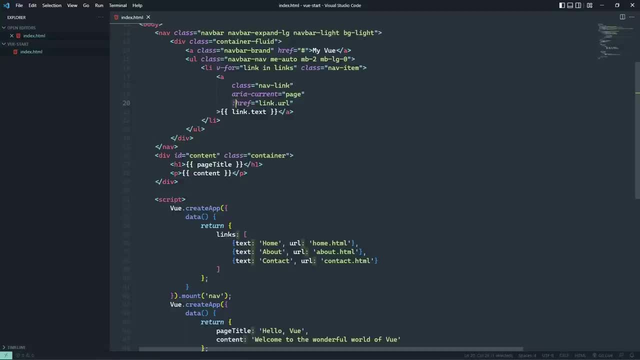 It makes sense to have a shorthand syntax to bind that data to an attribute. So instead of actually typing out vbind colon, we can just say colon followed by the attribute, and we will get the same result. 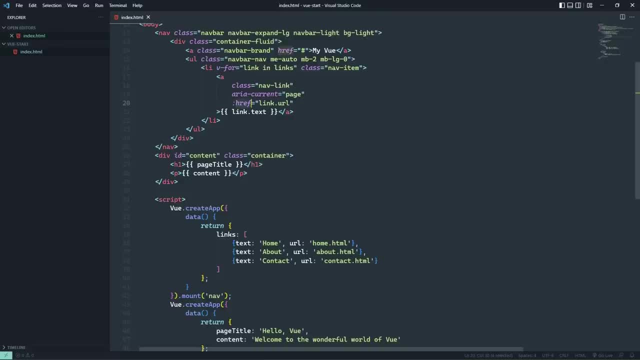 And we can do this for any HTML attribute, like for example, this is a link. And links should more or 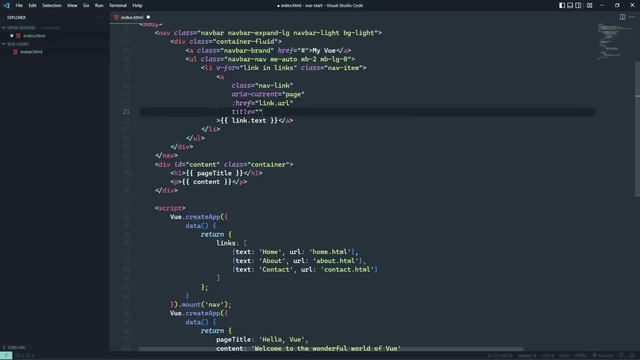 often than not have a title attribute, something that gives a description for the link, so that we can have a description of this link goes to. 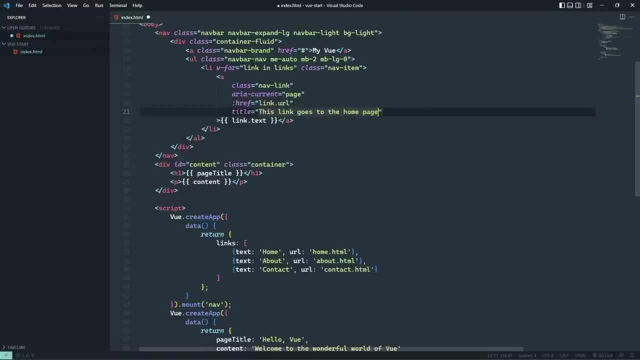 And then we can have the home page or the about page. But of course, we need this to be dynamic, because this is being generated dynamically. 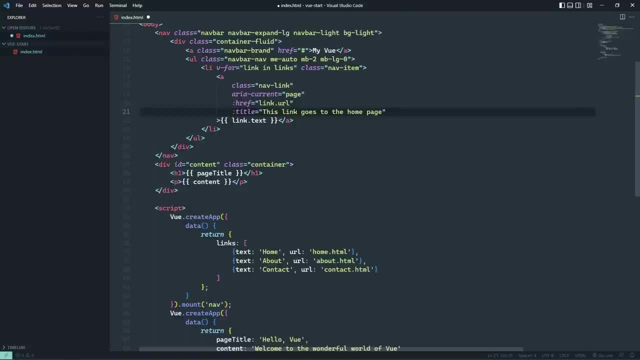 Well, we can simply use vbind on the title attribute. But remember that the value of this attribute is now a JavaScript expression. 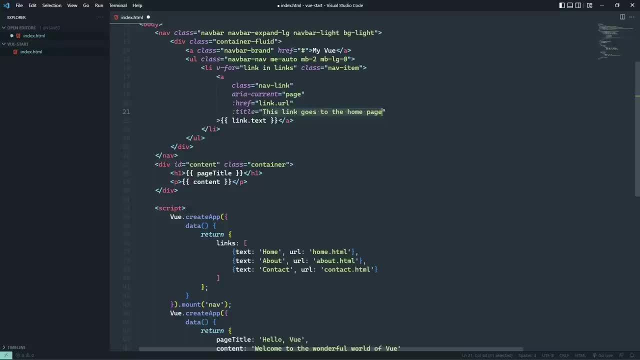 So having just normal text is not something that we want, because that's going to result in an error. It's a syntax error, because it's not a valid JavaScript expression. Instead, what we want is to output a string, a dynamic string based upon the text of the link. So I'm going to do this, so that we will use JavaScript's string interpolation feature to output a string that says this link goes to the, and then we can use the text. The text property on our link object. 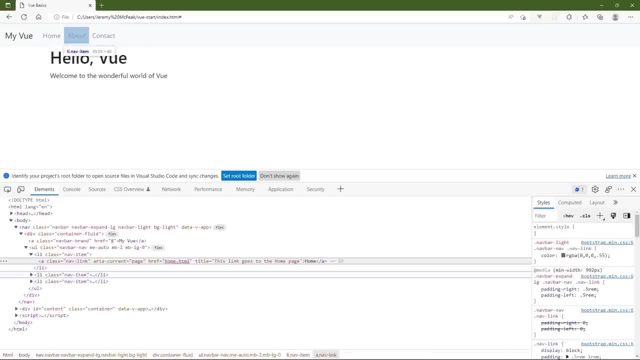 And whenever we view this in the browser, not only are we going to see the href attributes properly set, but we will see the same thing for title. This link goes to the home page. 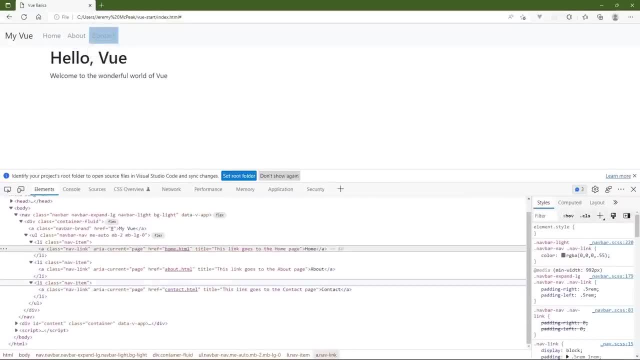 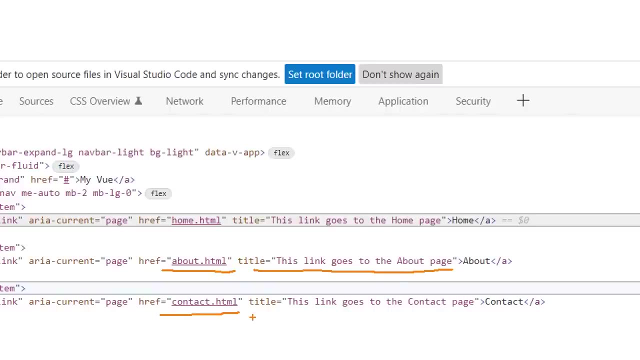 And if we take a look at the about and contact links, we will see something similar. The href is set to the appropriate value, as well as the title attribute for each one of those links. 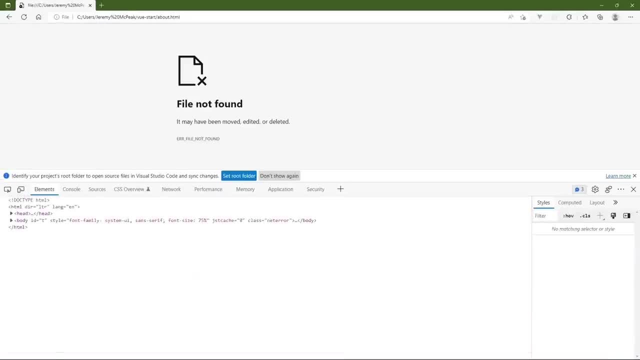 And so now whenever we click on these links, if we hit this, and If we had an about.html page, we would navigate to that page. 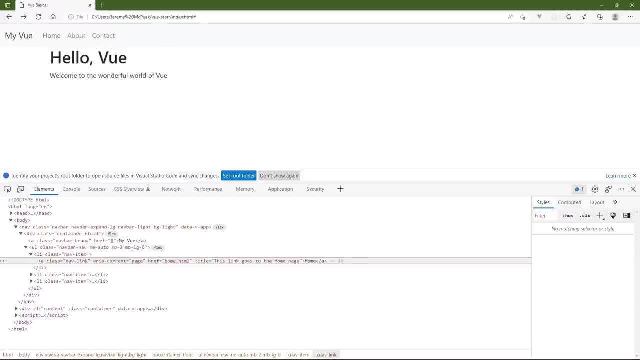 The same is true for contact as well as home. Although I guess home should probably be index, so let's make that change. 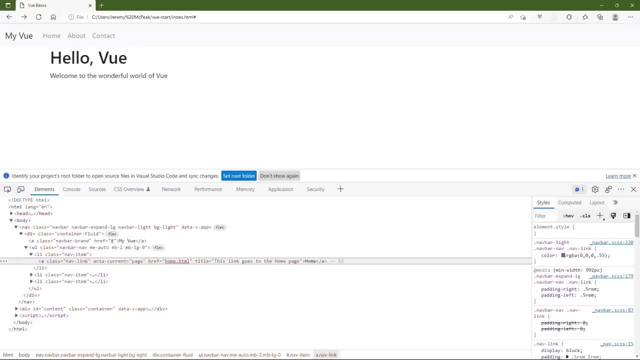 Home will be index.html, so let's refresh the page. Home goes to index, about goes to, well, 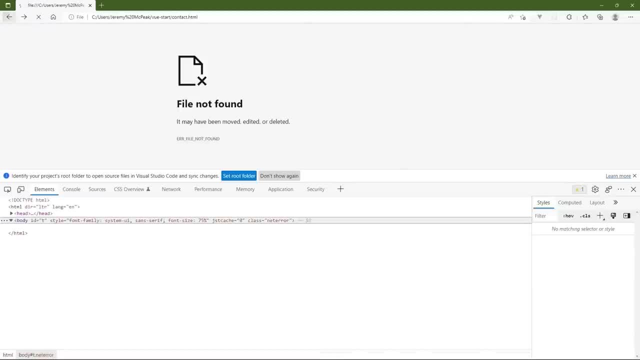 what would be the about page, contact goes to the contact page. 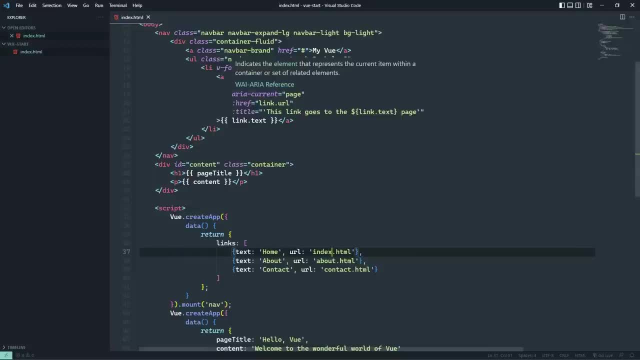 Now, there's one other thing, and it's not that important right now. Because the data that we are providing our navbar is static. We're not changing that data. 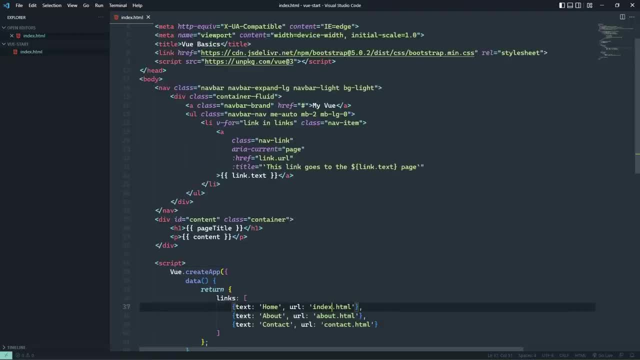 However, when we do change that data, Vue is going to automatically change what is seen inside of the browser. 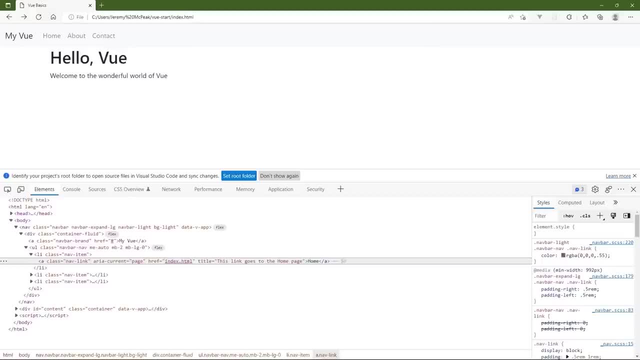 We don't have to do anything, Vue does it for us. But we do need to help Vue so 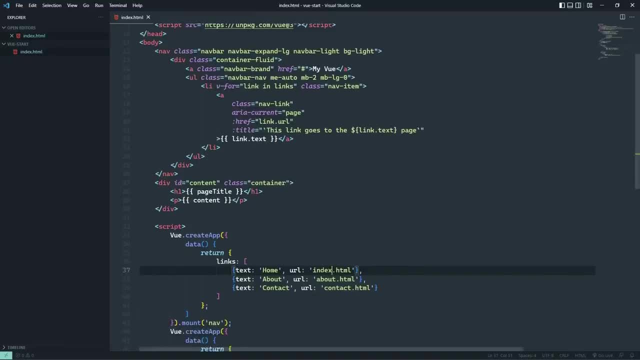 that it can identify which object that it needs to update. So we need to provide a key or a unique identifier for each one of the li elements that we are generating here with the v4 directive. So we do that by vbinding a key. And this has to be a unique value for each individual li element that is generated. Or a better way of thinking about it is a unique identifier for each item in the links array. 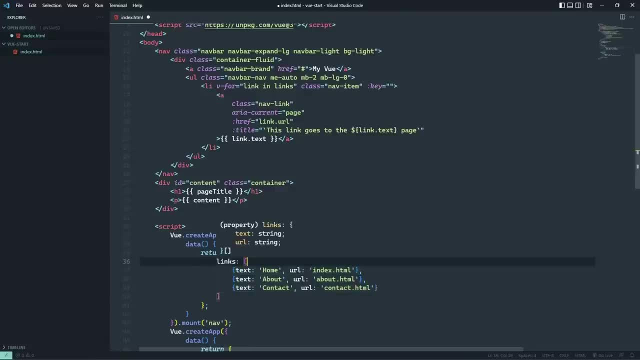 And one thing that is unique is the index of the elements in the array. Because the index of 0 is for home, the index of 1 is for about, the index of 2 is for contact. So we could use the index as the key. And we can do that very easily by modifying our for loop. So that not only are we going to be working with the link object, but we also get the index of that element in the array so that we can bind that to the key. And from a user's perspective, they aren't going to notice anything different. 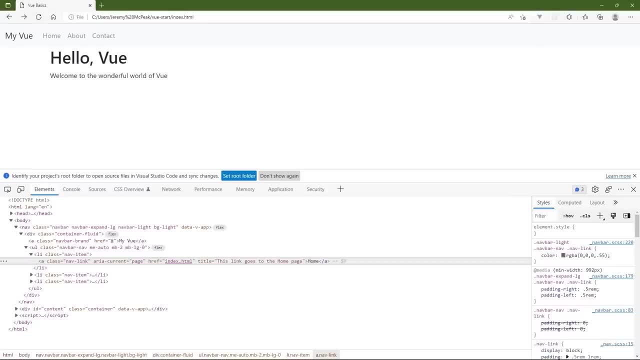 This is strictly for helping Vue do its thing behind the scenes. Now in the next lesson, we are going to transition this page into what's called 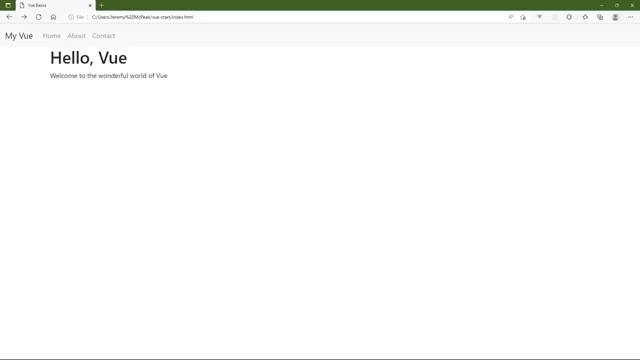 a single page application. Basically, it's a single page loaded in the browser, and the content changes based upon the user's interaction. So for example, clicking on one of the links is going to change the content. That is displayed in the browser. 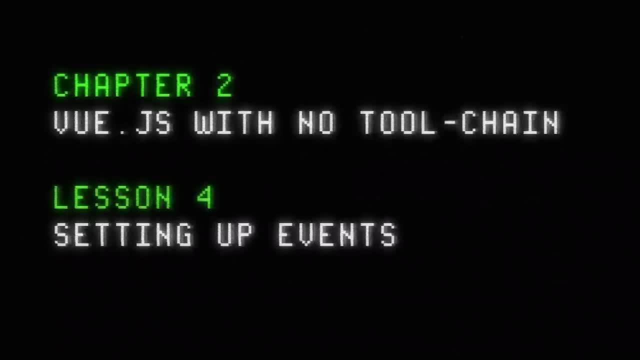 In this lesson, we are going to turn our web page into a single page application. 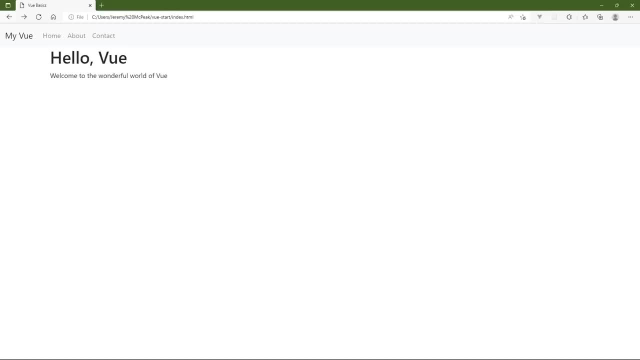 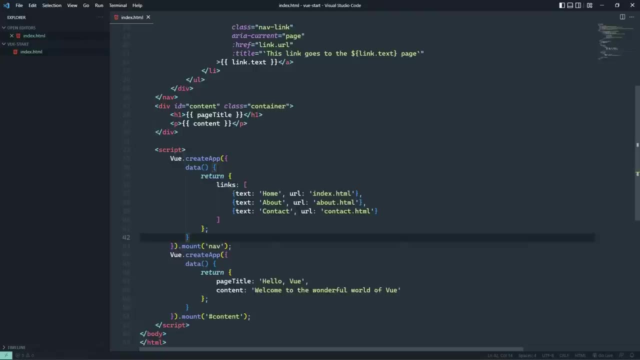 And we can accomplish this in a variety of different ways using Vue. However, with everything that we have talked about thus far, probably the most simple thing to do is to just combine our two Vue instances into one. So that we have just one data object that we are going to work with, which makes everything so much easier to do. So this transition is going to be relatively simple. All we need to do is take the data from one instance and put it inside of another. So let's take the links from our nav instance. Let's paste that inside of the data for our content. 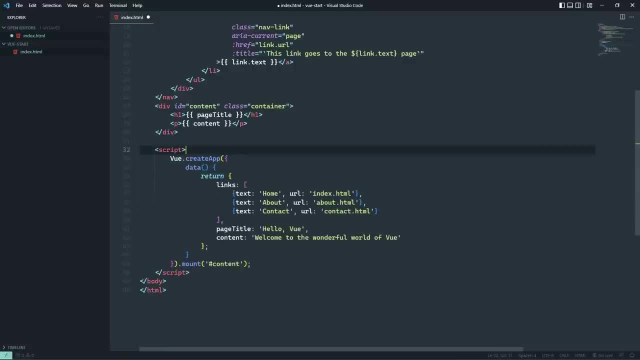 Let's delete the nav instance. And then we just need to change the CSS selector that we pass to the mount method. We can just pass in body. So that's it. 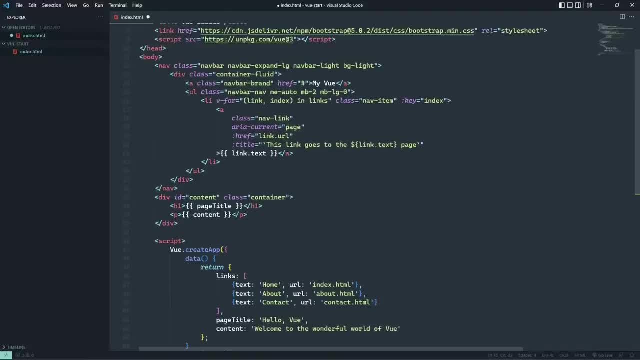 That we essentially mount our Vue instance in the body of this application. So this will cover both the nav and our content. 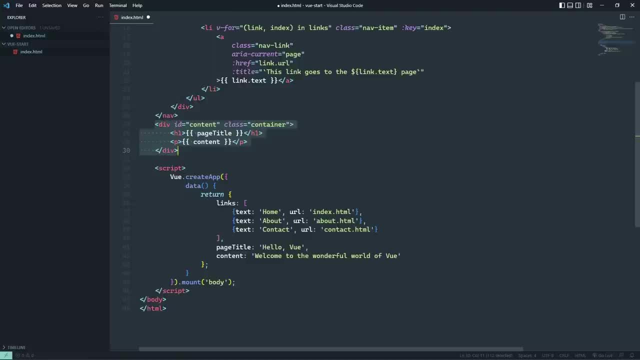 And so then the question becomes, how do we need to structure our data? Because we need more than just a set of links and a single page title and content. We need the link, the page title, and the content for each individual page that we want to display. 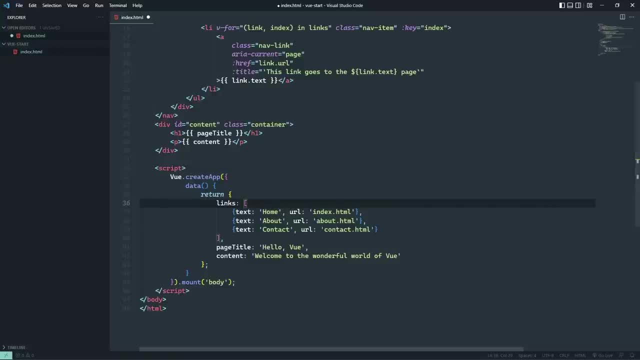 And we have three pages. Home, about, and contact. 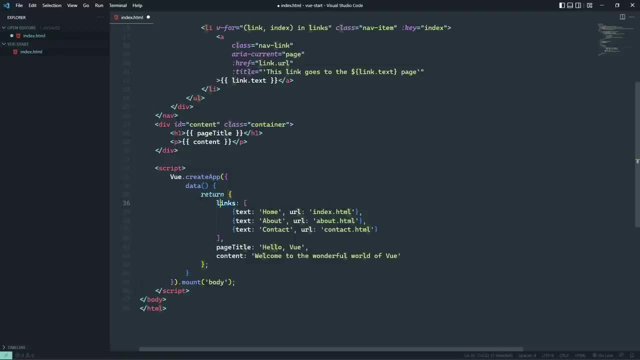 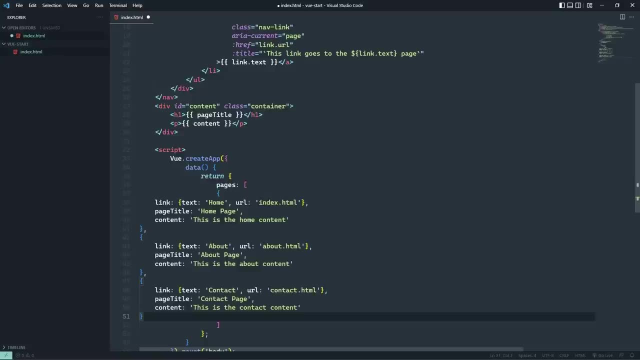 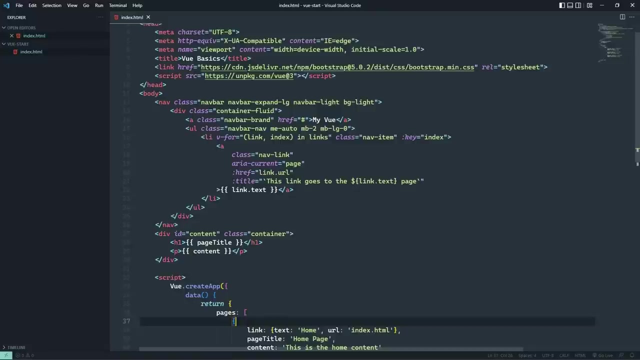 So I think what makes the most sense is to essentially change our data into an array of pages. And each one of these pages is going to be an object that has a link, that has the text and the URL. They have a page title and the content for that page. Now, because we're making this change, we do need to address our template, especially when it comes to generating the links. 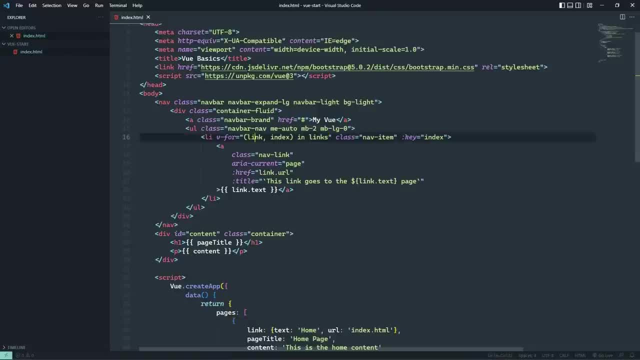 In our nav bar. So we are no longer working with links. Instead, we are working with an individual page inside of pages. We can leave the index alone because we need to bind that to the key for our list of li elements. But everywhere else we used that link. All we need to do is prepend that with page dot. And everything should work the same, at least as far as the nav is concerned. So let's do a sanity check. Let's go to the browser. Let's refresh. 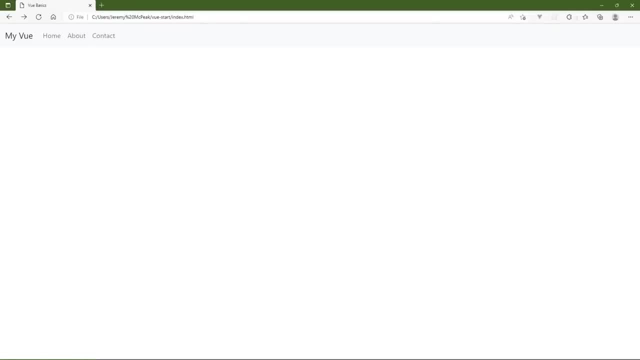 And yes, we have our links. So now we just need to change the content that is going to be displayed whenever we click on these links. 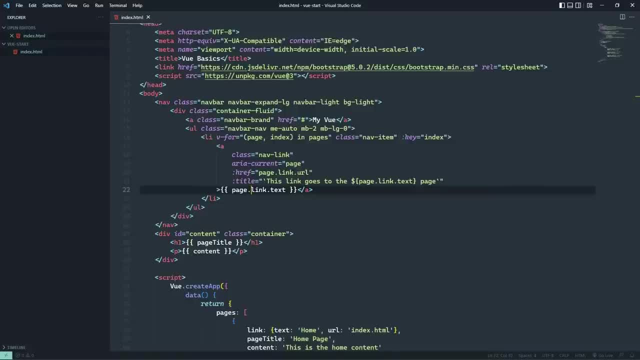 So this means that we need to set up a click event for these links. And this is very easy to do inside of view. It might look a little wrong because it is somewhat reminiscent to DOM level 0 events. 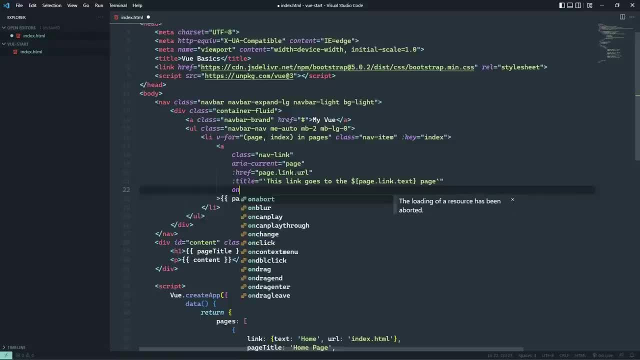 Now, if you're not familiar with that terminology, before there was any DOM specification. 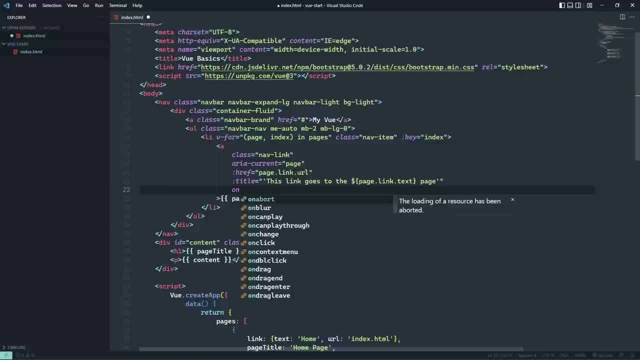 The way that we set up event handlers was through HTML. Every HTML element had attributes like on click, or on mouse over, or things like that that would let us set up an event on that element. So for a click event, we would have on click. And then the value of this attribute would be some JavaScript expression that would execute whenever the user clicked on that element. 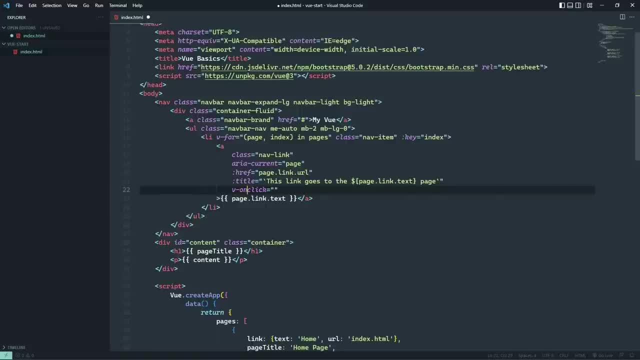 So we use a view directive called v on. 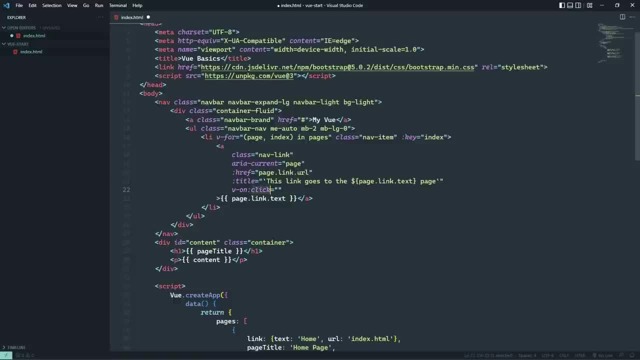 We follow that with a colon. And then we have the name of the event that we want to handle. In this case, it's going to be click. 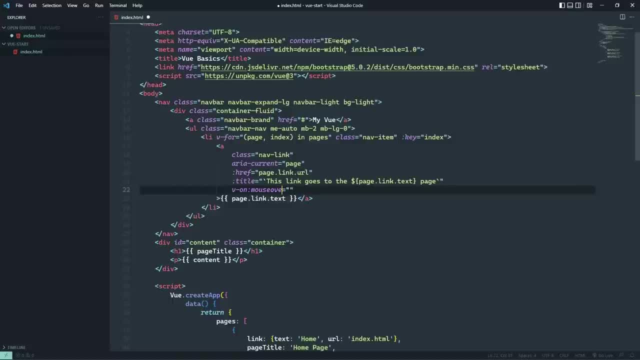 If it was some other event like mouse over, or mouse out, or mouse enter, anything like that, we would use just the name of that event. But we would prepend it with the v on directive. Now, there is a shorthand syntax. Instead of saying v on, we can just use an at sign before the event name. 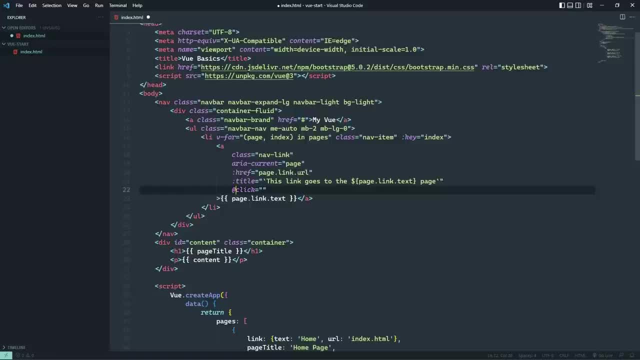 So at click is setting up the click event handler for this element. I like to think of it as action and then click. And then we just need to specify the code that it's going to execute whenever we click on this link. 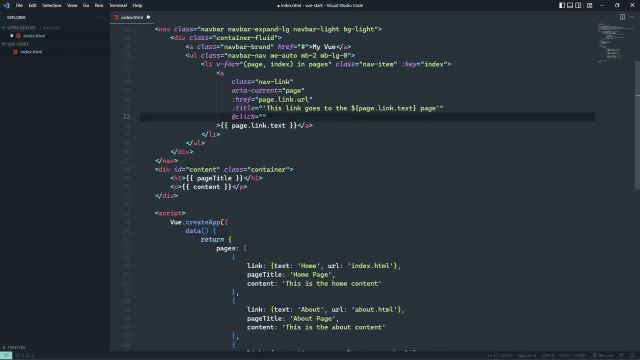 Whenever we click on the link, we need to be able to track the link of the page that we clicked on. So we need some other data property that we can use to track the active page. And let's just call this property activePage. And it makes sense to initialize this as our home page. 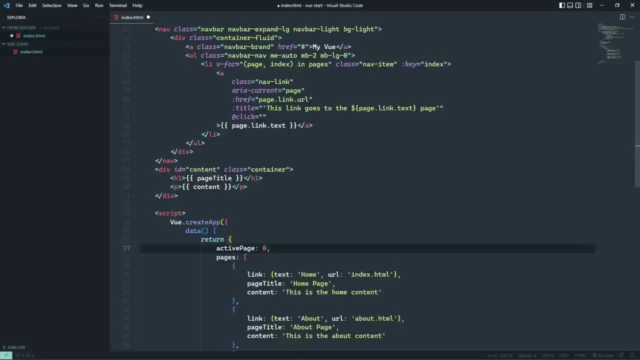 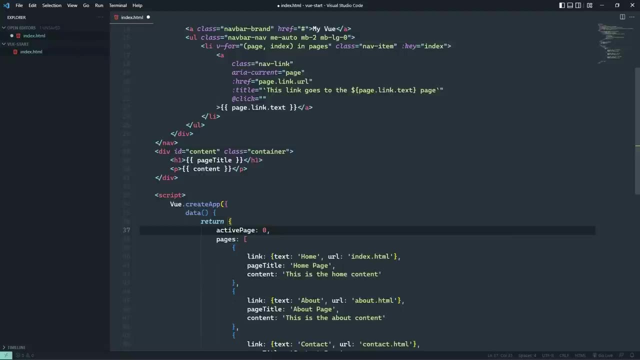 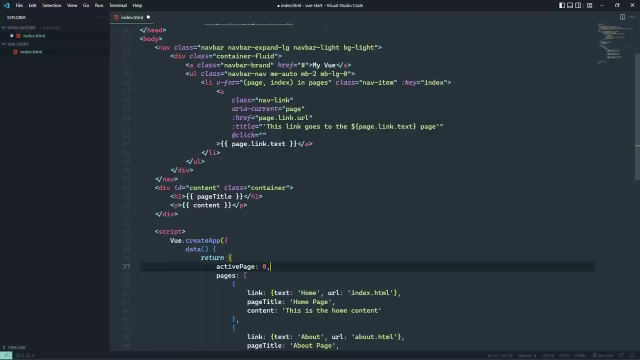 So let's say that we're going to track this based upon the index. So our home page is at an index of 0, as far as the pages array is concerned. So about will be index 1, and then contact will be index 2. So that whenever we click on these links, we want to change activePage to the index, or the index of the page. 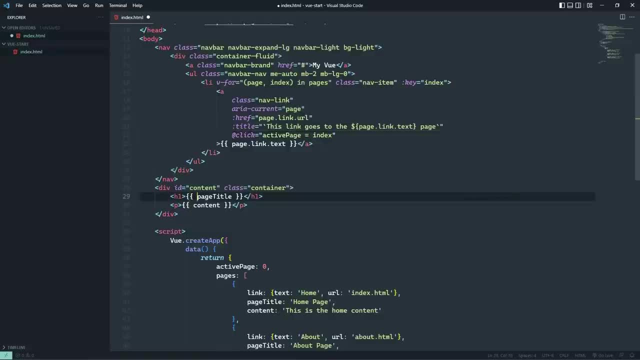 And that's for the given page. And so when it comes to displaying our contents, we'll use pages. We will use the index syntax so that we can use activePage. And then that will give us access to that page's title as well as the content. 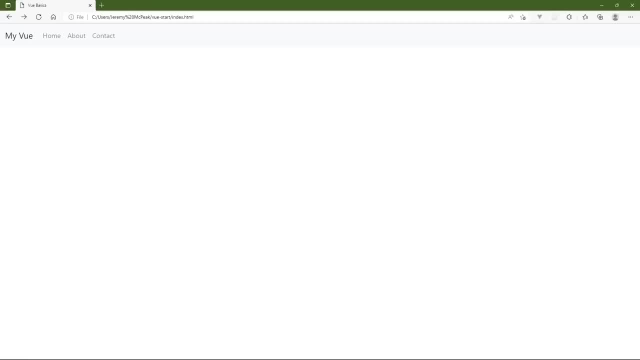 So another sanity check, let's go to the browser, let's give this a shot. So let's refresh the page. 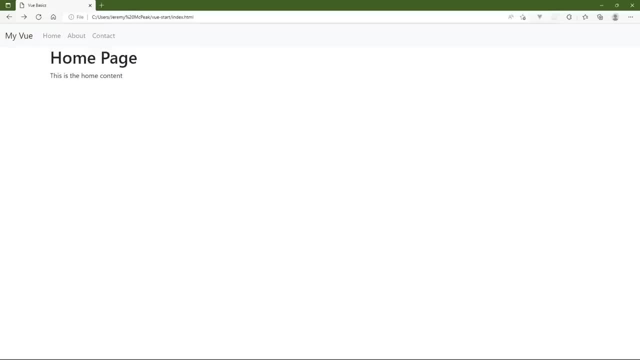 Since homepage is our default page, we can see that that content is automatically displayed. So 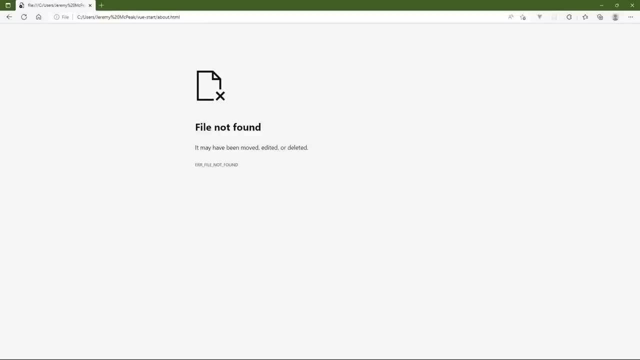 let's click on the About link. Well, we could see very briefly that the content changed, but notice that we navigated to about.html. That is the URL that was specified for that link. 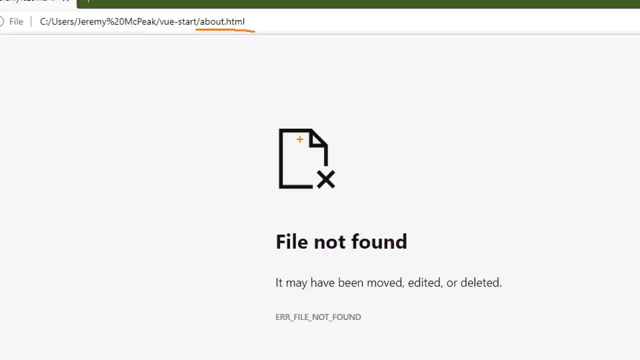 And we don't want that because all of our content is now being loaded through JavaScript. 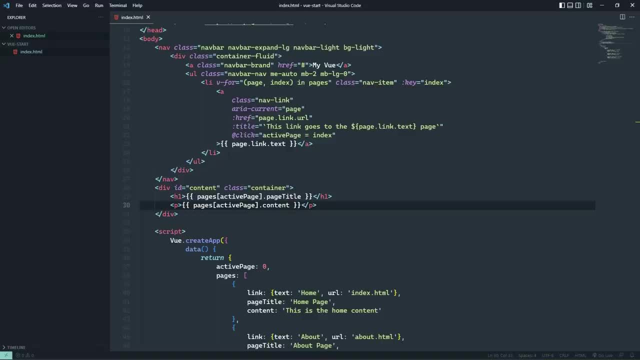 So we want to prevent the web browser from navigating to whatever URL is specified in the href. 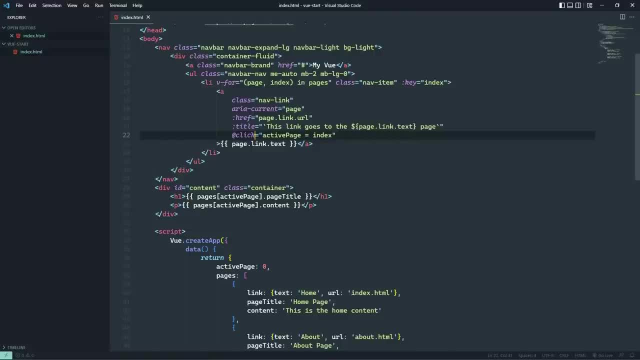 And if this was just a normal DOM event listener, we could do that using the event objects prevent default method. 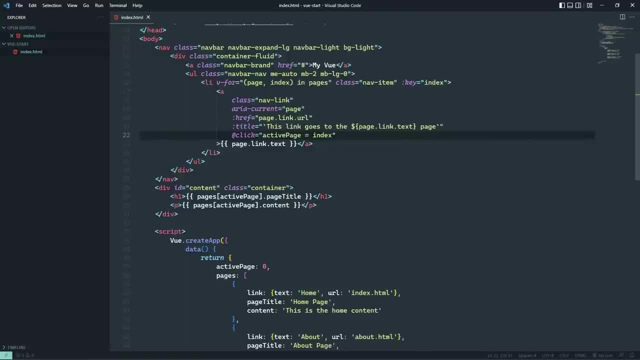 But since this is view, we have a more declarative way of doing that. Whenever we specify the atClick directive, we can follow that up with a dot, and then we can use this prevent modifier. 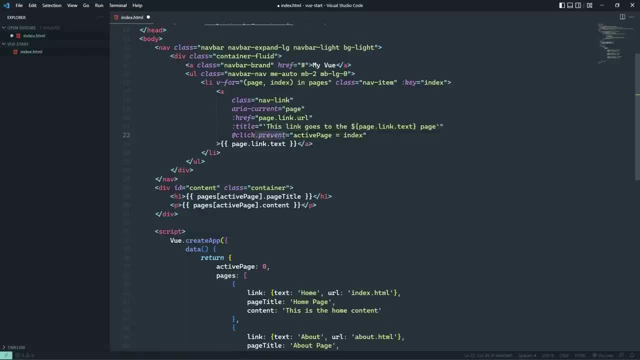 This essentially says that we want to prevent the browser from navigating 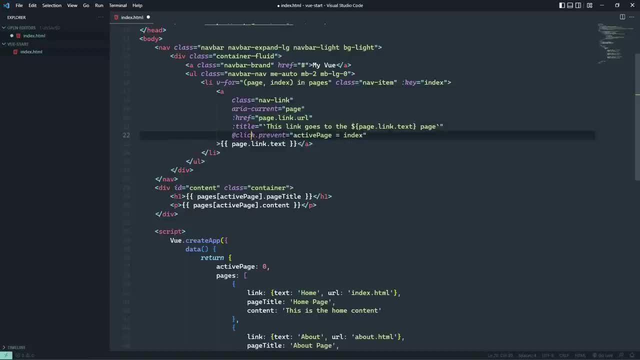 to the href whenever the user clicks on this link. 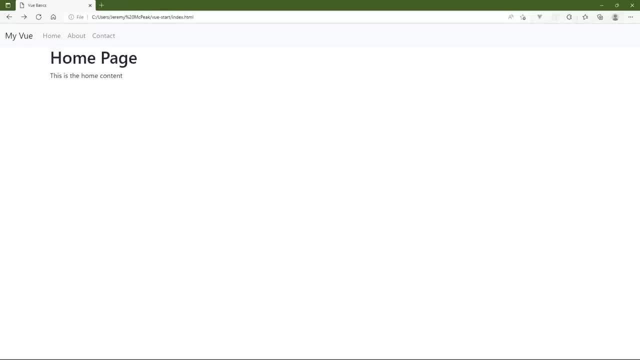 So with that in place, we can go back to the browser, let's refresh the page. Now whenever we click on About, we can see that the browser did not navigate 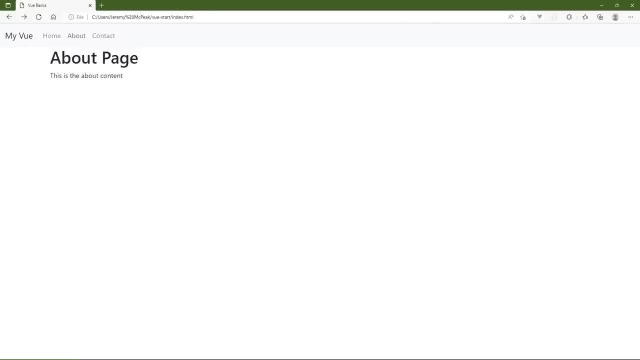 to about.html, but it did load the content that we specified. 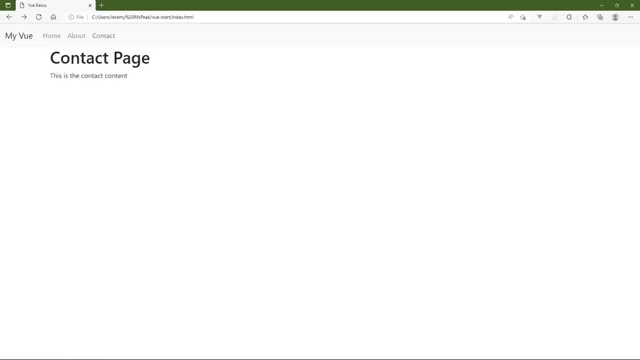 And then whenever we click on Contact, well, we see the same thing. Let's click on Home, Homepage, Contact, About. 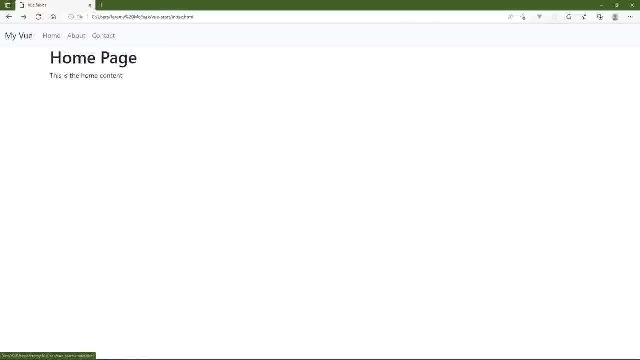 And we can keep doing this, and it's going to work just like we would expect it to. And this is one of the great things about view. 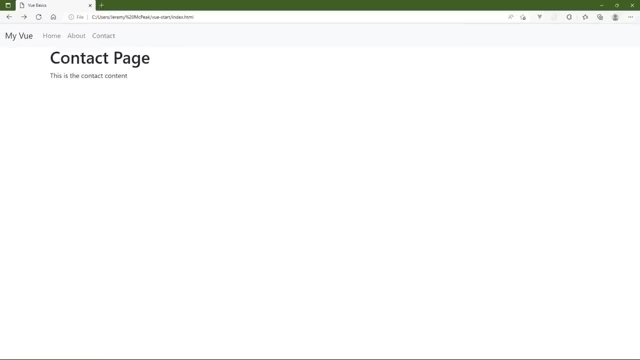 And really, it's not just view, but any UI framework like React, Angular, Svelte, Alpine, I mean, there's quite a few these days. 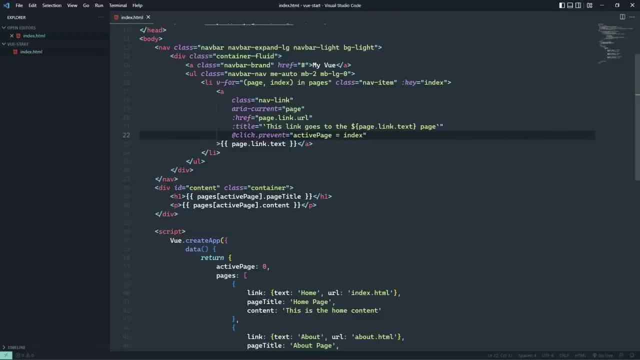 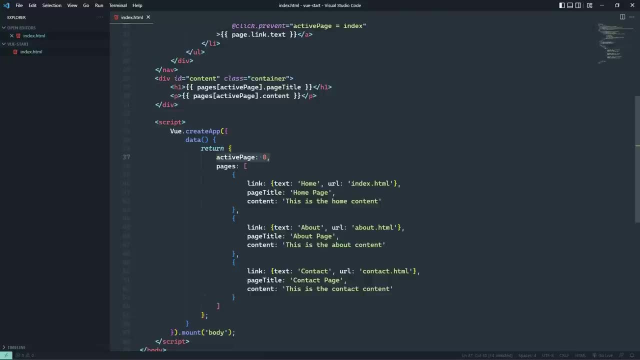 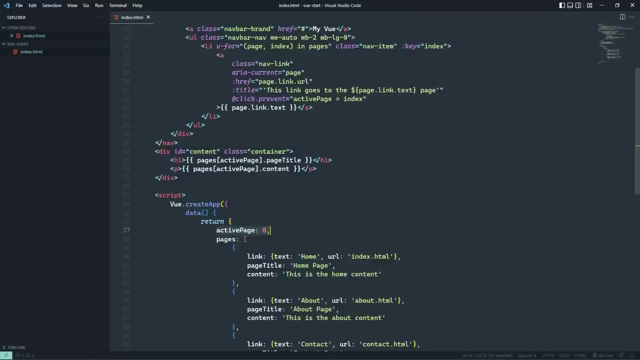 But we no longer have to write the code that actually changes the content. Instead, all we have to do is change data, and then our application will react to that change in data. For example, the only piece of data that we changed was the value of active page. Whenever we clicked on the link, we changed that value. And because of that very simple change, view automatically updated the content that was loaded in the DOM. 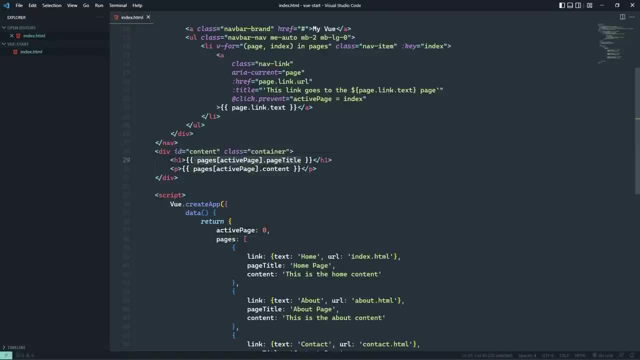 Because our code said to load the page title of the active page, and to load the content of the active page. 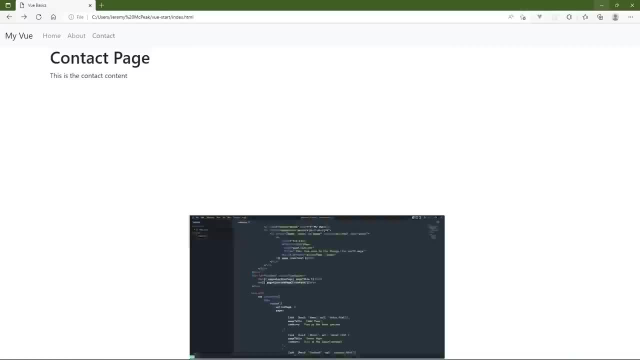 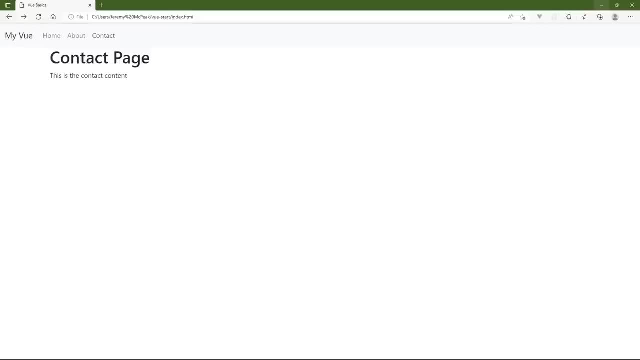 And so this is where the power and the popularity of these frameworks come from. Because we are no longer concerned with actually updating the DOM. The framework does that automatically for us. All we have to do is set up the UI to display the content that we've wanted, and then simply change the data or change the state of the application. 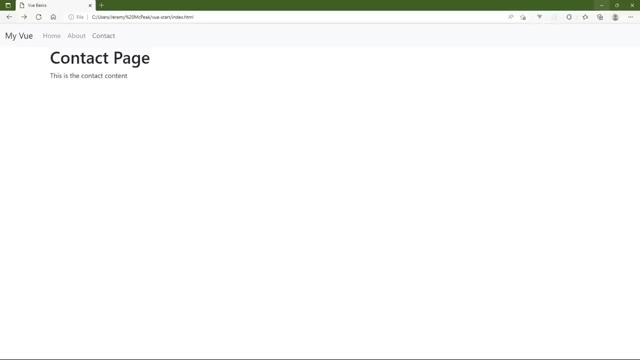 And view will automatically update the DOM for us. When it comes to building dynamic user interfaces, 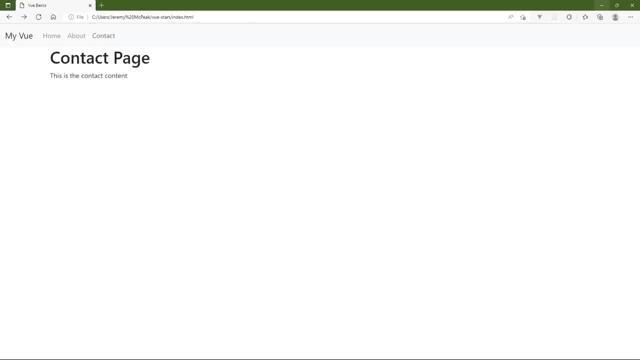 there's so much more than just changing the content or updating content. 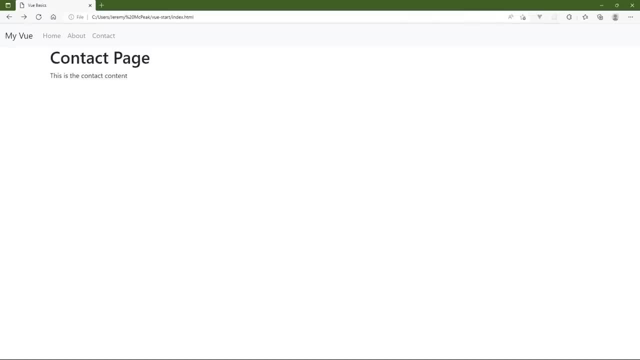 A lot of times we want to change or update the style that is applied to HTML elements. Like for example, Bootstrap gives us a class called active for our nav link. 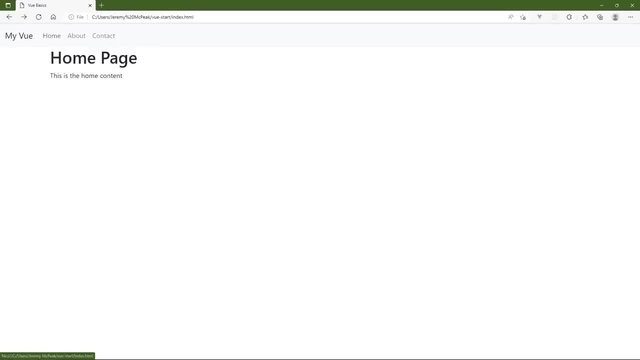 So that we can signify to the user that the home link, or the about link, or the contact link is active. It's just a visual cue that we can provide the user. 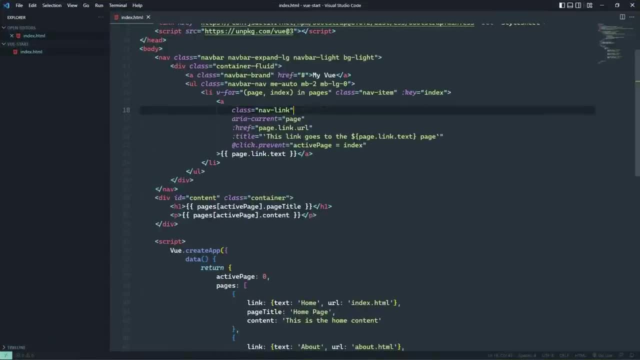 And as it is right now, we aren't using that class. Because when we look at our markup, all we have specified is the nav link class for these links. 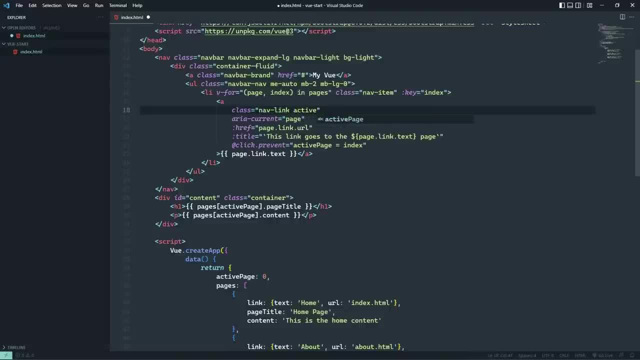 What we want to do is include active, but only when the active page is equal to the active link. 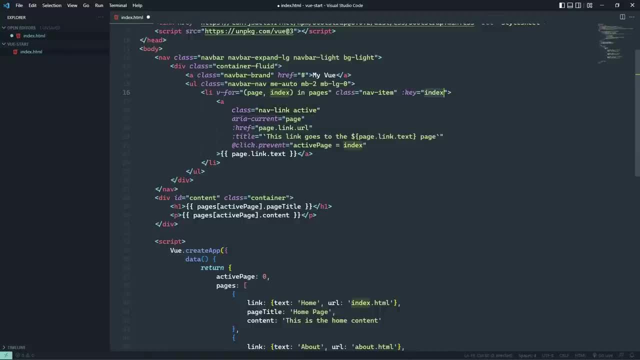 Or equal to the index of a given page. So we need to be able to add some kind of conditional statement. 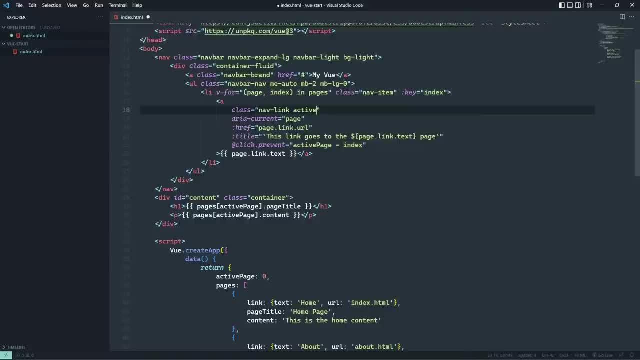 So that if the active page is equal to the index, then we would use the active class. 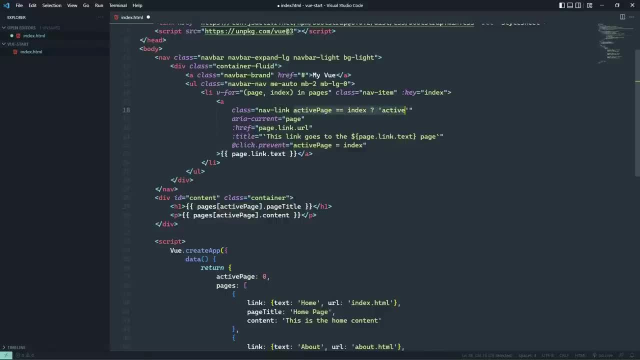 If we were going to use the ternary expression, it would look something like that. 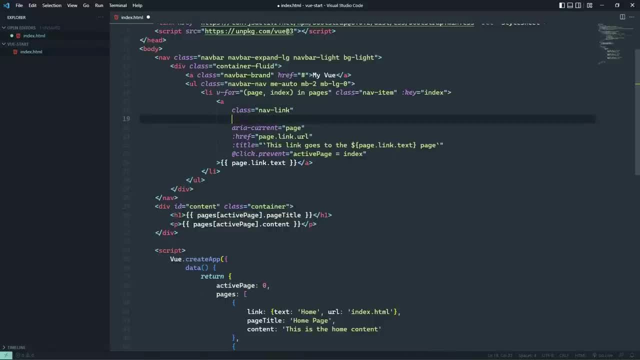 Well, we can do this very simply by using vbind, but I'm gonna use the shorthand on the class. 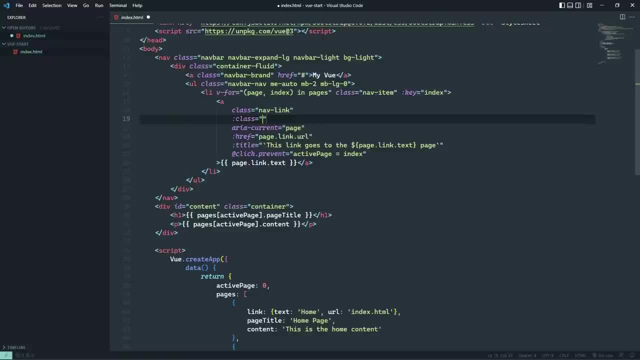 Now, this is going to look a little weird, because not only do we use the class attribute, this is the HTML class attribute. 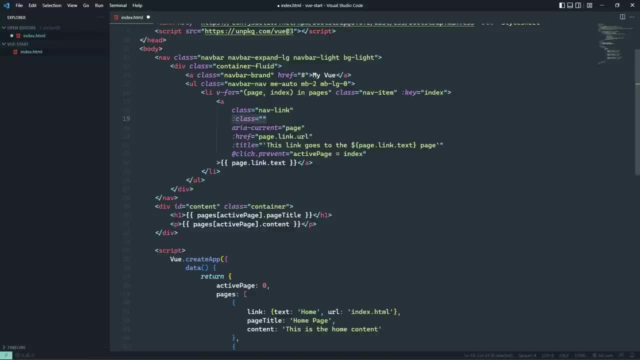 But we are also going to use the vbind directive on class. So you can think of this as, I want to apply these CSS classes always to the element by using the HTML class attribute. 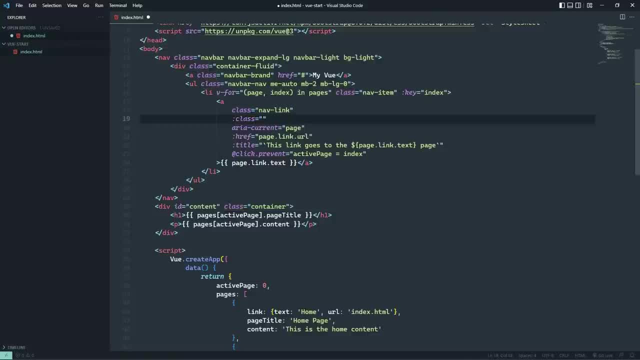 And then for classes that you want to apply conditionally, you'll use the vbind. 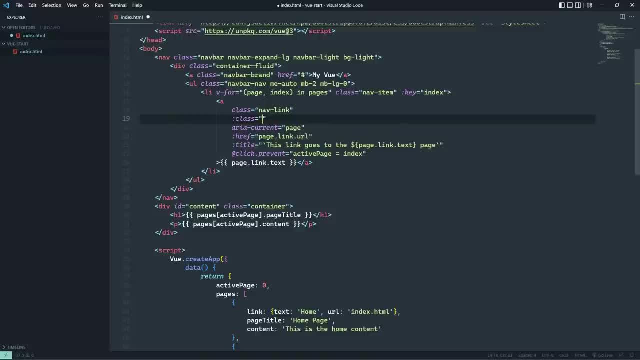 So the syntax for this is going to look a little weird, because we don't use ternary expressions or anything like that. 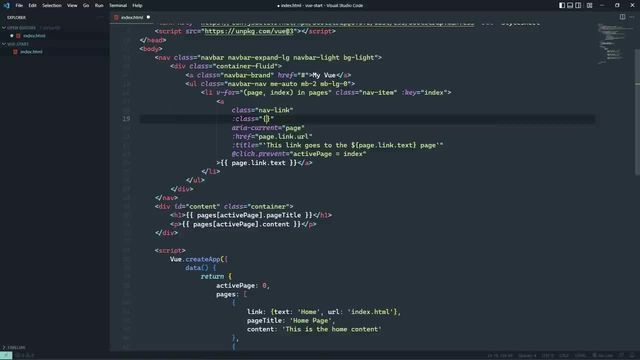 Instead, what we have is an object. And the properties of these objects are the CSS classes that we want to apply to this element. 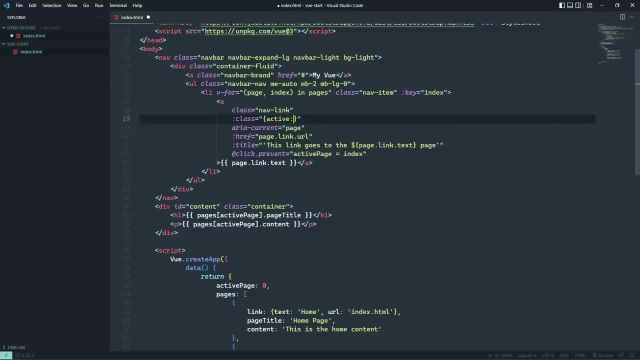 So in this case, we want to apply the active class. And the value is going to be our condition statement. So we want to apply the active class when the active class is equal to the active element. 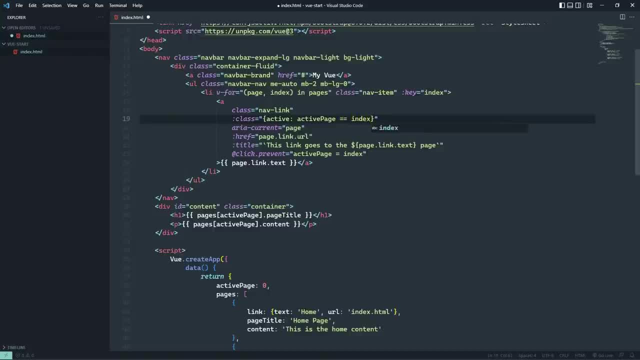 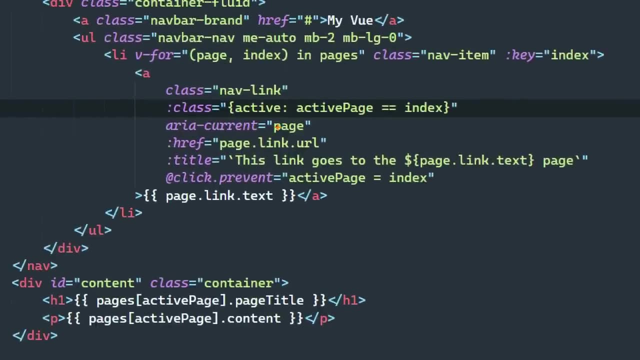 And the value of the active page is equal to the index of this given page. So let's just take a look at the syntax again, because as I said, this looks a little weird, especially when you are expecting to use an if statement or ternary or something like that. 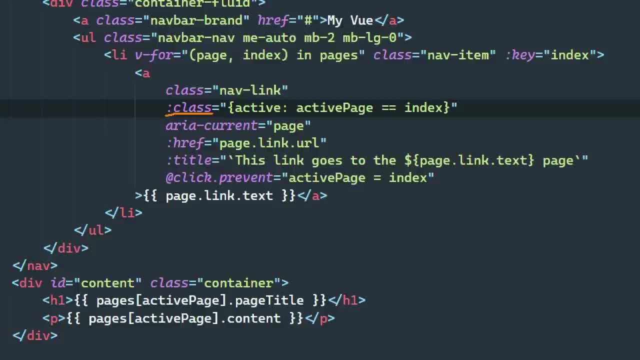 So we are using the vbind directive on the class. And we are providing an object where the property is the CSS class that we want to apply to the element, and then the value of that property is the value. 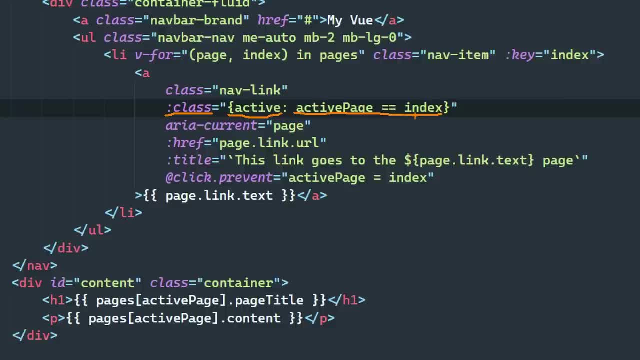 So we're going to use the conditional statement that will determine if that CSS class is applied. 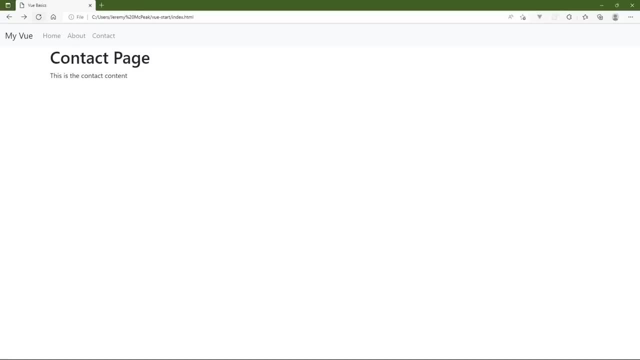 So with that done, we can go to the browser. We can refresh our page, and you can automatically see, it's a little difficult to tell due to the styling here. 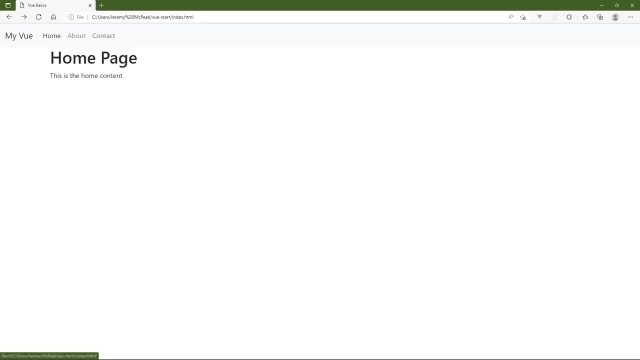 But you can see that home is a little bit darker than about and contact. 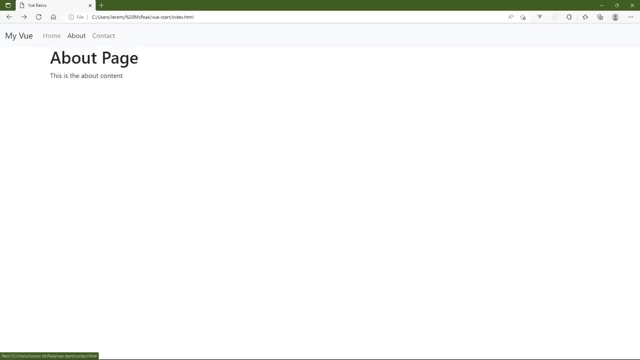 Whenever we click on about, again, it's a little bit darker. When we click on contact, it's a little bit darker. Now, we can make this much more apparent. 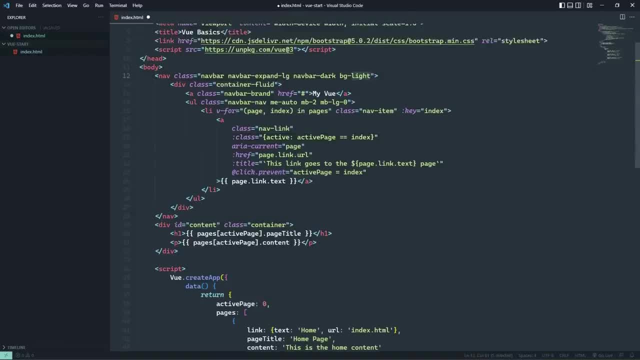 At least in my opinion, if we change it to a dark navbar. So I'm going to change the CSS classes from navbar-light and bg-light to navbar-dark and bg-dark. 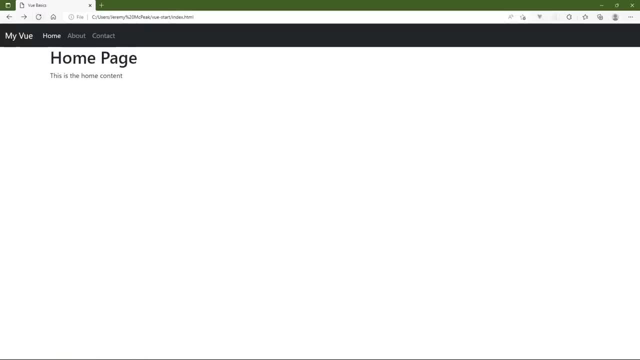 If we refresh the page, now we can definitely see that home is active. If we click on about, if we click on contact, we can see that those are active. And we can inspect these elements, and we can actually see the HTML automatically update. So here is the HTML. And 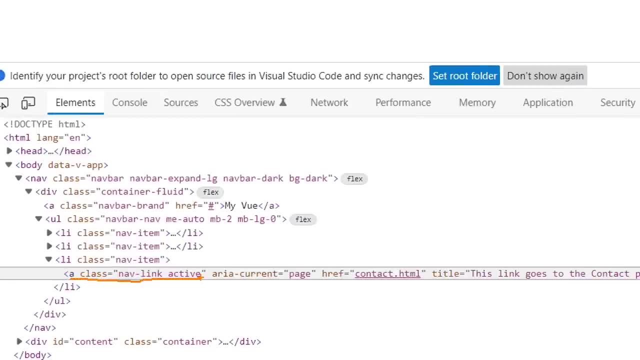 here are the A elements. We have the class of nav, link, and active. 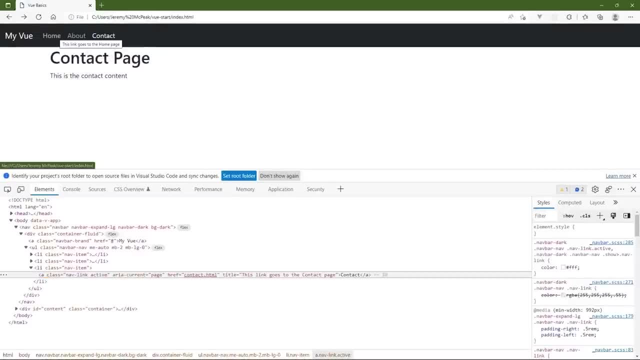 So keep your eye on that. Whenever I click on home, it's going to automatically update the CSS classes. 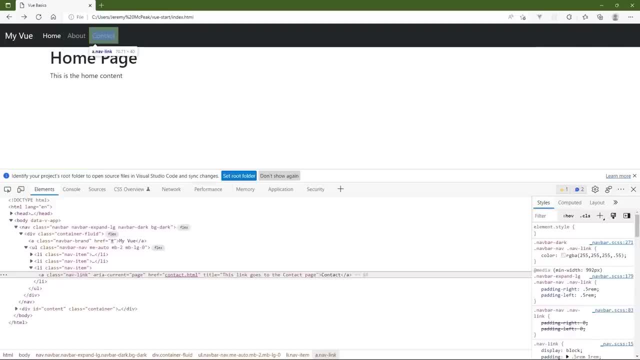 So that active is no longer applied to the link for contact. But if we take a look at the link for home, well, there it is right there. So this gives me an idea. 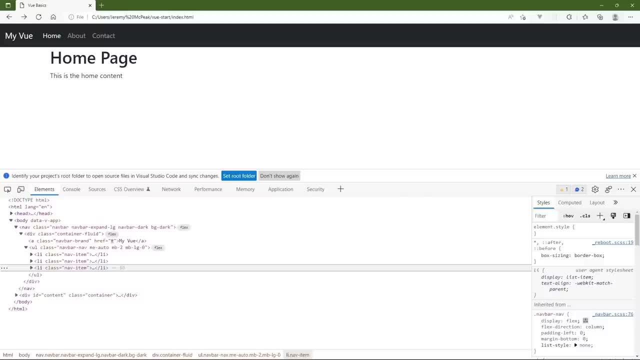 I want to be able to toggle the navbar from light to dark. So let's do that. 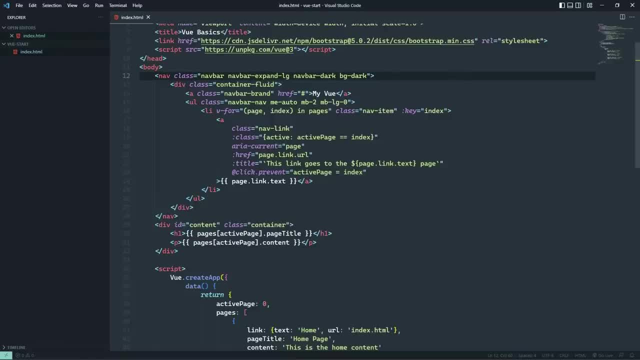 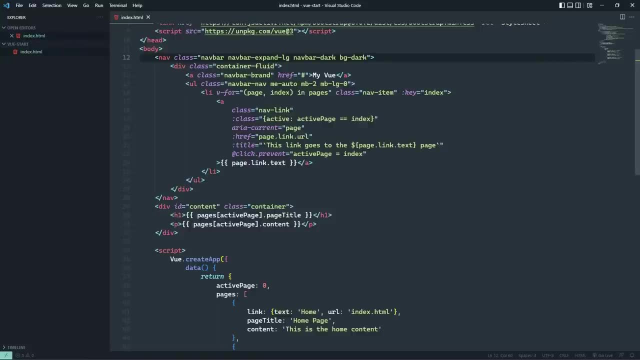 We know how to do that now that we can bind CSS classes. But we do need to be able to track if we are displaying a light background or a dark background. 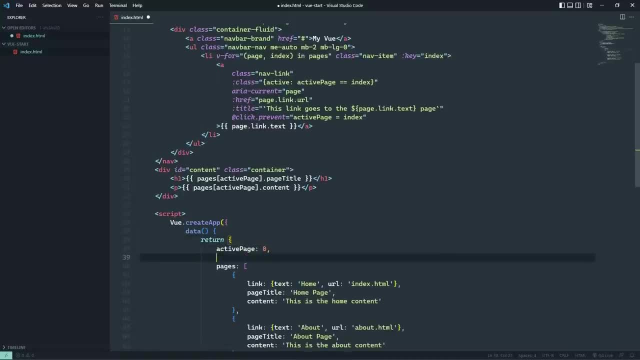 So let's add another data property. And let's just call this useDarkNavbar. So of course, if this is true, then the navbar will be dark. If it's false, then it will be light. 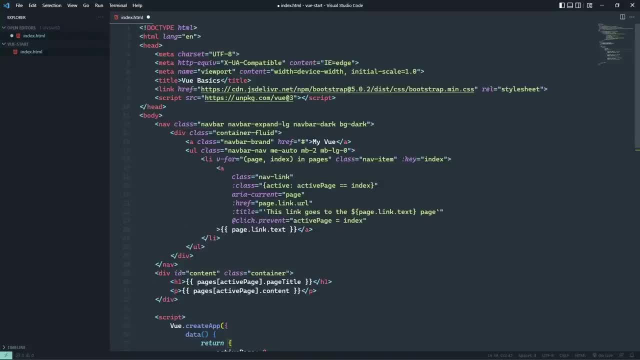 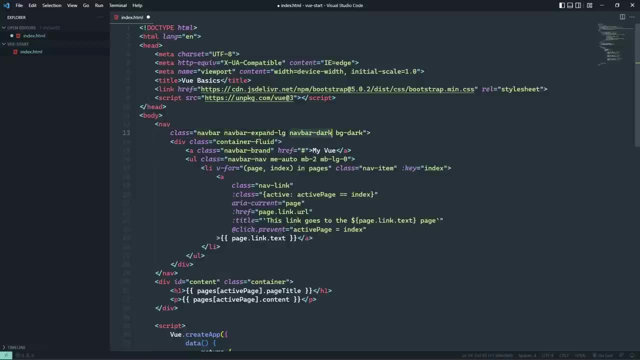 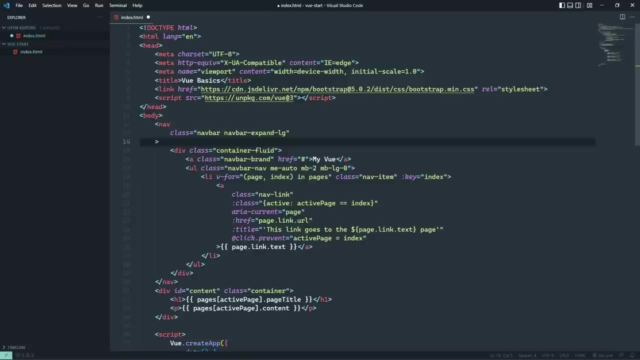 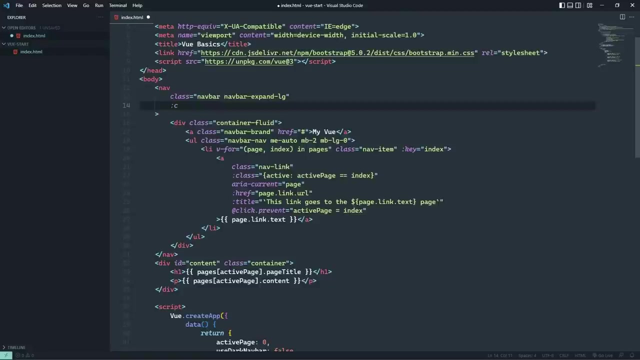 Let's initialize it as false. And this means that we are going to modify our HTML, and then we're going to modify it. Our HTML class attributes so that we aren't applying the navbar light and bg light. Instead, we want to dynamically apply the appropriate classes based upon the value of this useDarkNavbar. So once again, we are going to vbind the class. We're going to pass in an object. Things are going to get a little bit tricky here because the CSS classes that we want to apply use hyphens. 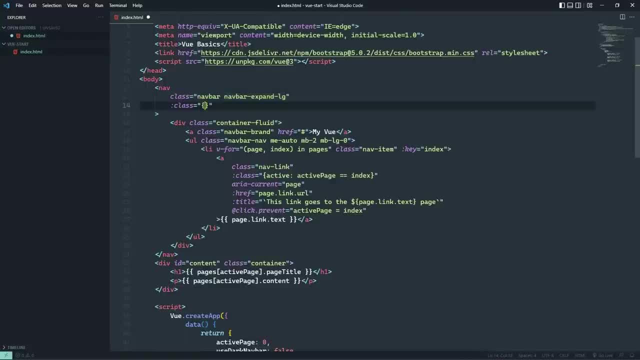 They're not valid in JavaScript identifiers. However, we can use a string as a property name. 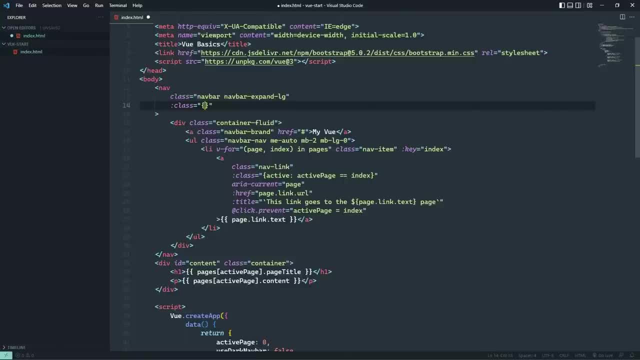 We can also apply multiple classes at the same time so that it looks like this. 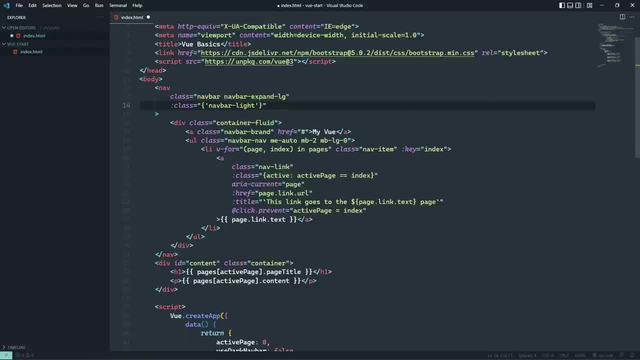 So that we want to apply navbar light and bg light when useDarkNavbar is false. And then we essentially want to do the same thing for the dark version, but 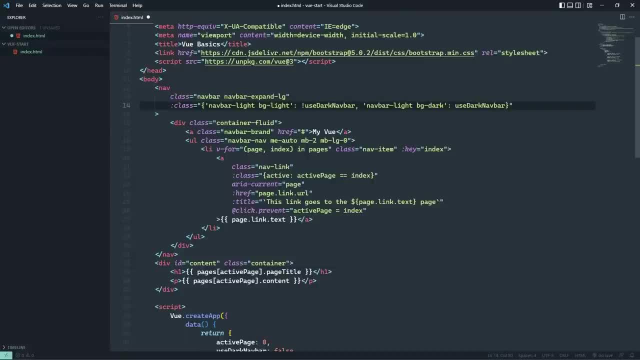 when useNavbar is true. So once again, we will change these values to navbar dark and bg dark. 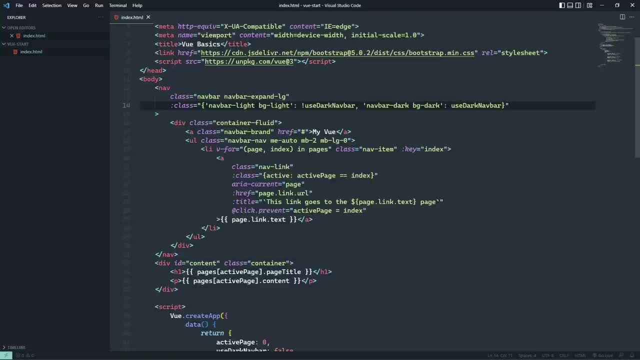 So this looks even weirder than before. So let's just take a brief moment to talk about this syntax. 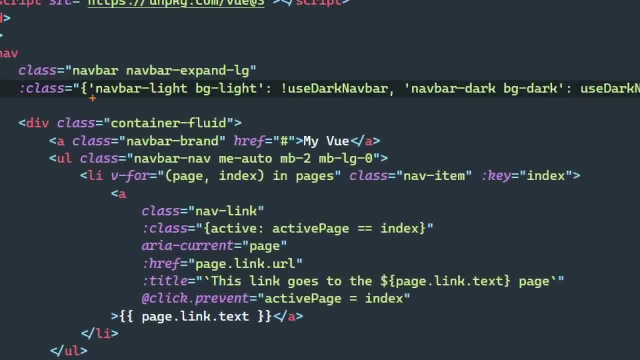 So once again, we are binding our classes. But since these classes use hyphens in their name, we can't use these as normal JavaScript identifiers. So our property name is denoted with a string. We're using two CSS classes. We're using two CSS classes. Separated by a space as the property name inside of the string. 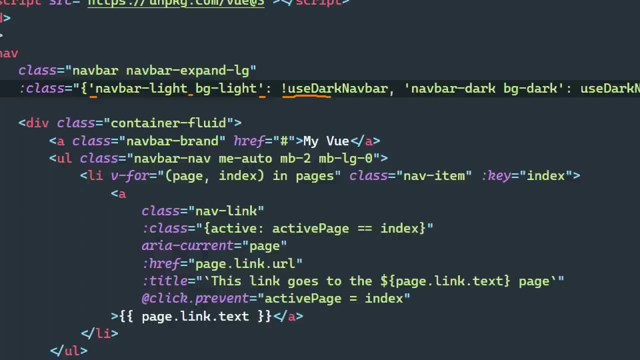 And then the conditional value is not to use dark navbar. So when that's false, we use the light classes. 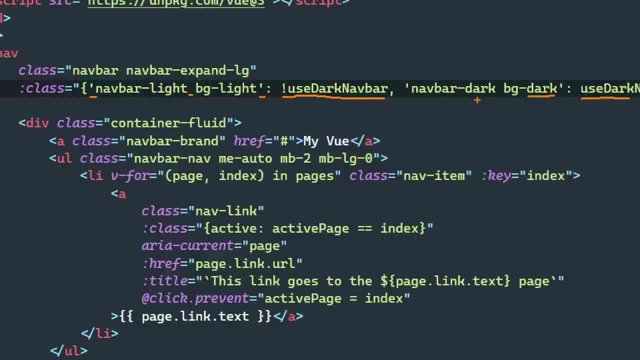 When it's true, we use the dark classes. 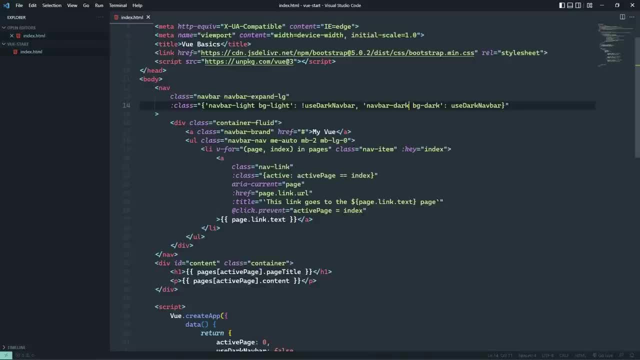 So with that in place, all we need is a button to click on so that we can toggle those classes. 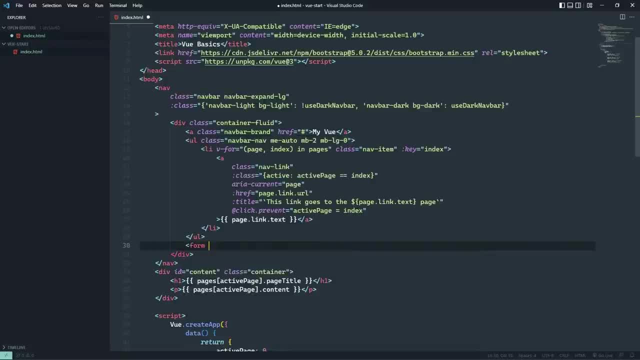 So I'm going to add a form after the unordered class. Let's add a class of Deflex. 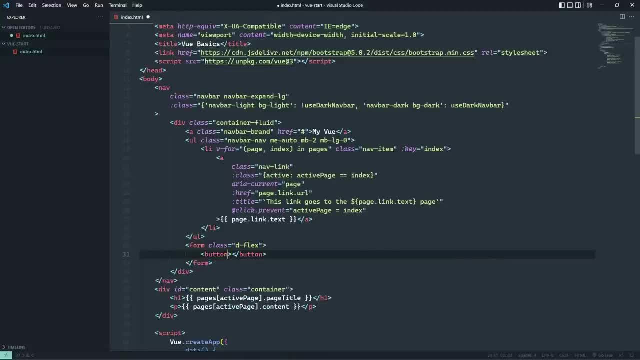 And inside of this form, we will have just a simple button. Let's go ahead and set up the CSS classes so that we make this blend in with Bootstrap. 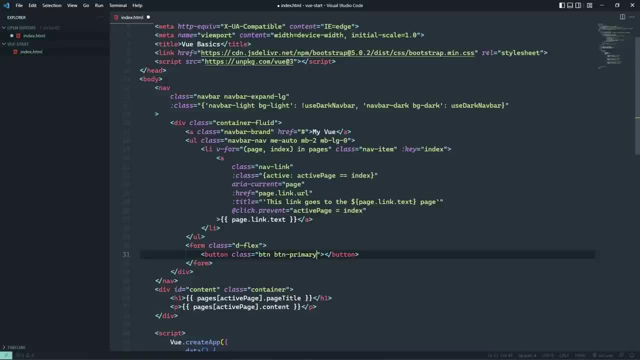 So we will use the button class. Let's also use button primary. We don't really need to specify the type, but we do need to handle the click event. So let's do that with at click. Let's go ahead and prevent the default. Since this is inside of a file, we're gonna have to do that. The form, off the top of my head, I don't know what the default action would be. So it doesn't hurt to add the prevent modifier to this event. And what we want to do is change the value of use dark navbar so that it is equal to its opposite. 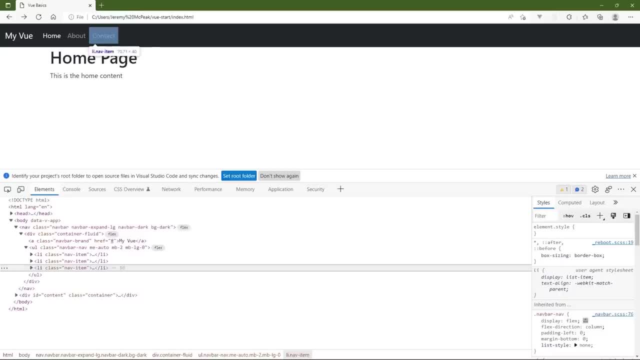 And with that simple change, we can go back to the browser, we can refresh the page. The default is to show the light bar. 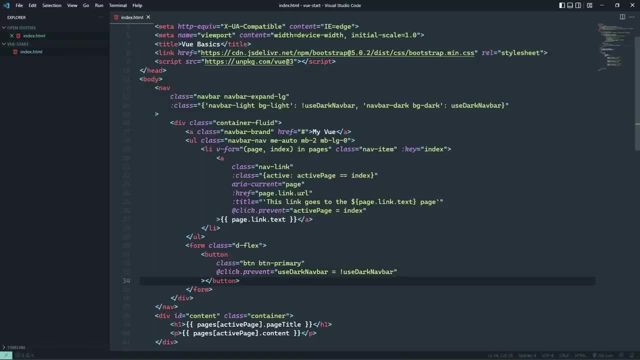 It would be useful to have some text, wouldn't it? Let's say, 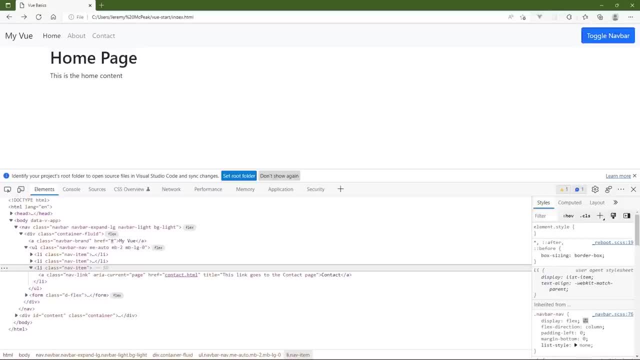 toggle navbar, so now let's refresh, the default is the light background. If we click on the toggle navbar, that should change it to the dark, and it does. The active class is being properly applied. Let's toggle back to the light navbar. Once again, the active class is properly applied, and everything works as it should. 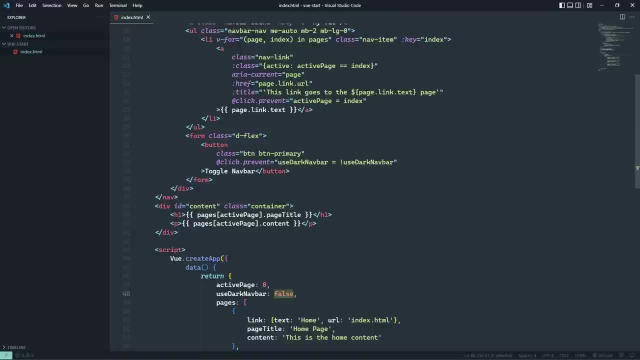 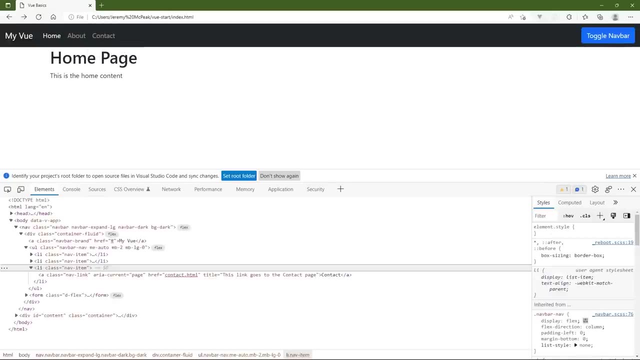 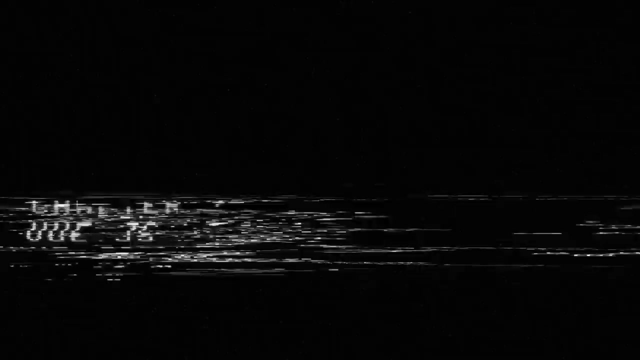 Now, let's do this, let's make sure that it's going to work if we set the default value for use dark navbar as true. And of course it will, we wrote this, so there it is. By setting that to default to true, our navbar is now dark. Everything else still works the same. We can toggle this to the light, but I think personally, I like the dark. So I'm going to leave it like that. 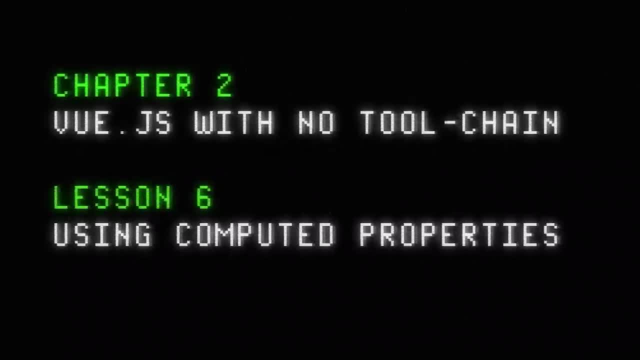 In the previous lesson, you learned about one of the ways that you can bind CSS classes to an element. 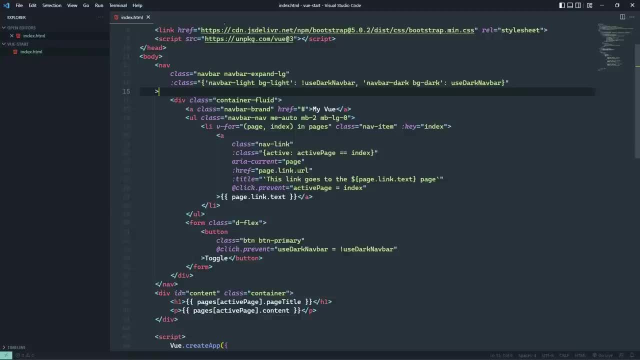 And yes, I said one of the ways, because when it comes to working with style in view, you can apply style in a variety of ways. 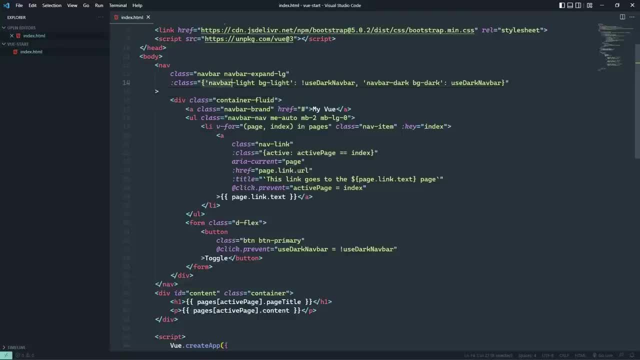 In the previous lesson, we used an object where the properties were the CSS classes that we wanted to apply, and then their values were a conditional expression that determines whether or not those classes are actually applied to the element. In the next lesson, we will look at how to use arrays. Now, in this lesson, I want to focus on this expression, because while it works, I'd make the argument that it's not the easiest to quickly read and understand what's going on. 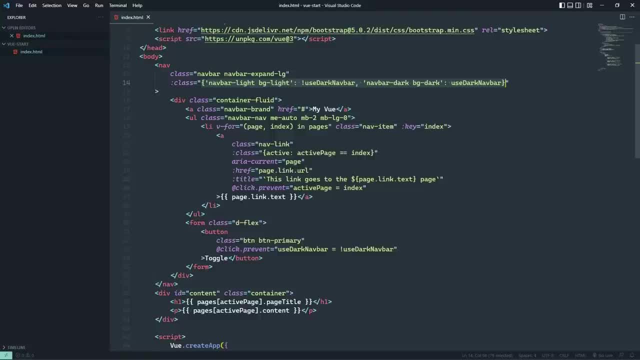 Instead, what I want to do is extract this out into an object that we would then just reference here, so we could call it navbar classes, and that makes it a lot easier. 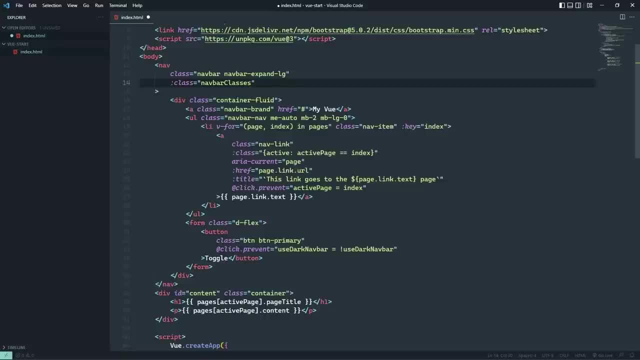 As we are skimming through this, we could see, okay, navbar classes are being applied. And then later on, we can look at the actual detail inside of our code. 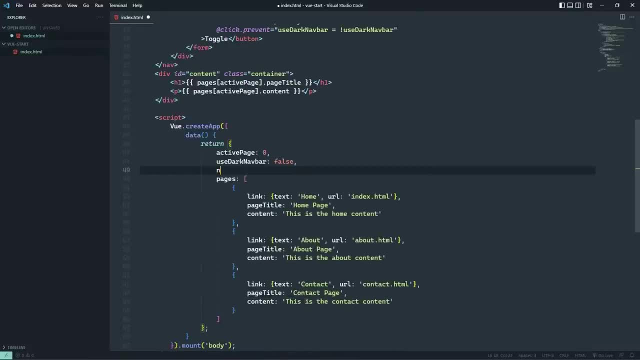 So you might think that we would need to define this navbar classes object in our data. 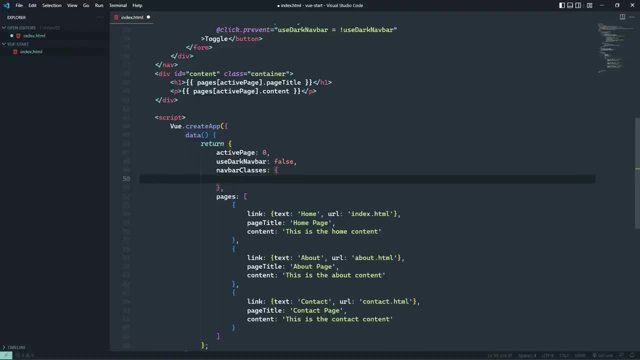 Yes, we can technically do that, but it's not going to behave the way that we expect it to. In fact, it's not going to work at all. 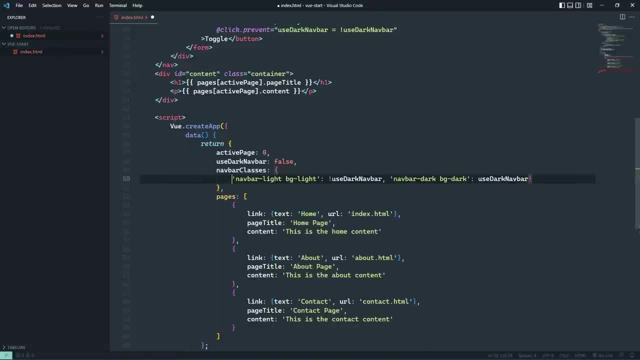 But let's look at it not working and talk about why it doesn't work, and then we will look at how we can make it work. 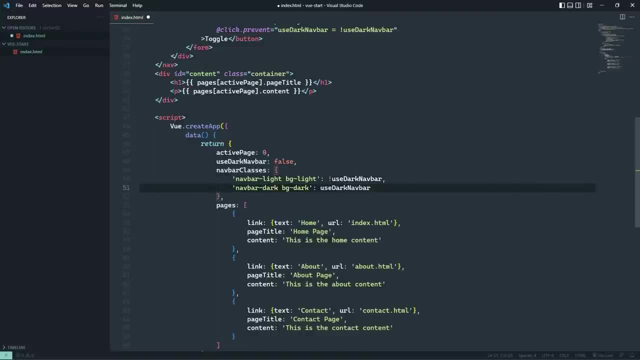 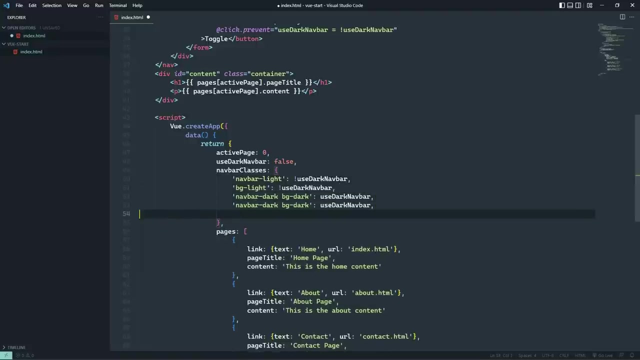 So the first thing I want to do is essentially turn this from two lines of code into four lines, because I personally think it's a lot easier to read and understand if we do something like this. So that each individual property is its own each individual CSS class. It's just my preference, but I don't mind writing extra lines of code if it means that I don't have to come back to it in three months and think, what am I doing here? Oh, yeah, so this is our object. 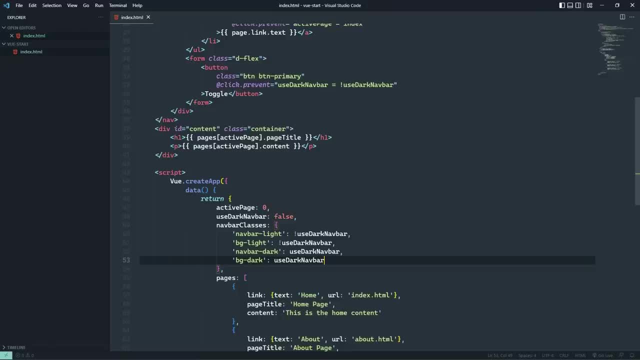 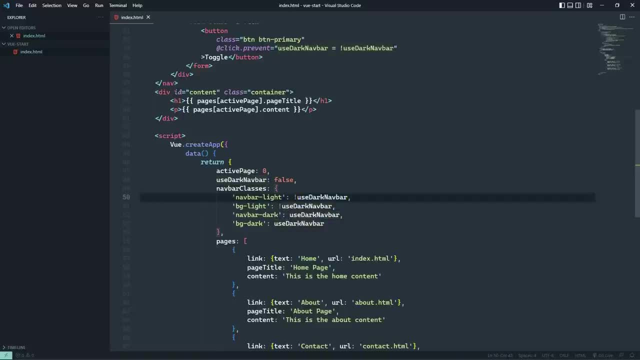 And the use dark nav bar isn't just a variable. It's a property inside of our application because, well, here it is. 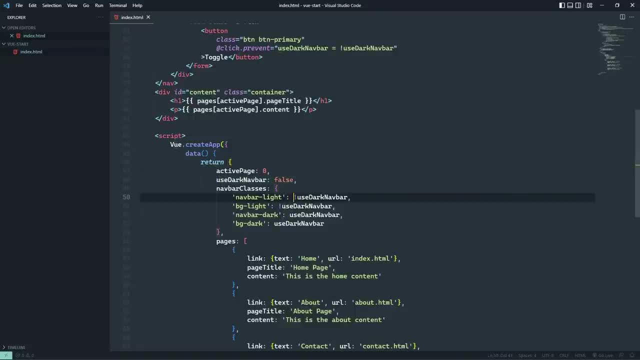 It's defined right here inside of this object. So we need to say this.use dark nav bar, and so that is going to be fine. 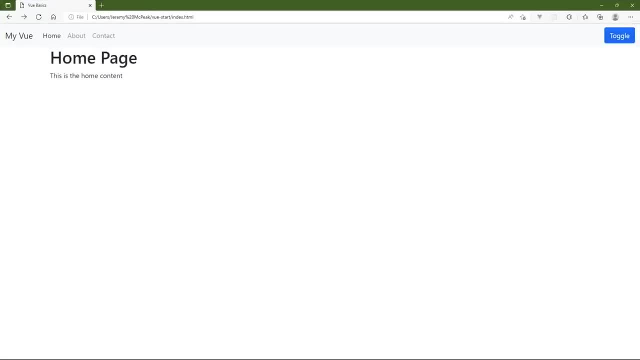 We can save this, we can go to the browser, we can refresh, and whenever we click on toggle, nothing happens. 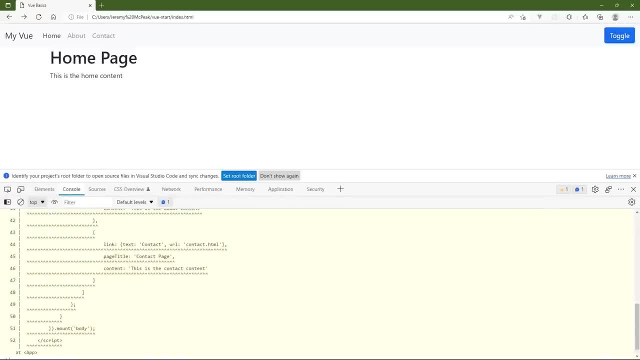 Now, it's not because that there's an error. We can pull up the console and And we aren't going to see any errors at all. We will see this warning, and the only reason why we are getting this is because this script is inside of the body tag, and we've created a view app that's mounted to the body. 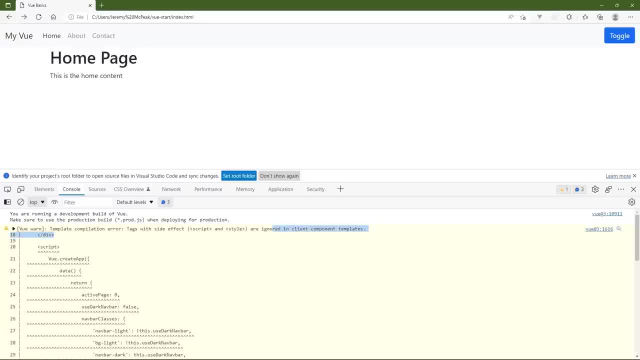 So we can see that this is being ignored, so that's fine, we don't care about that. 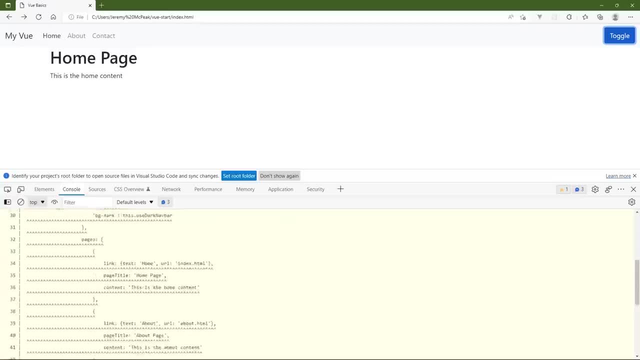 But as I click on the toggle button, there are no errors appearing in the console. So it's not working because there's an error, 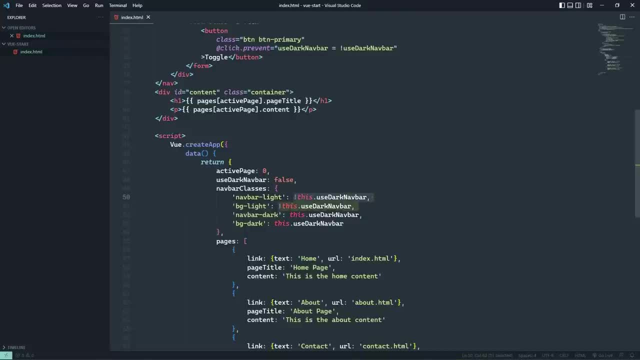 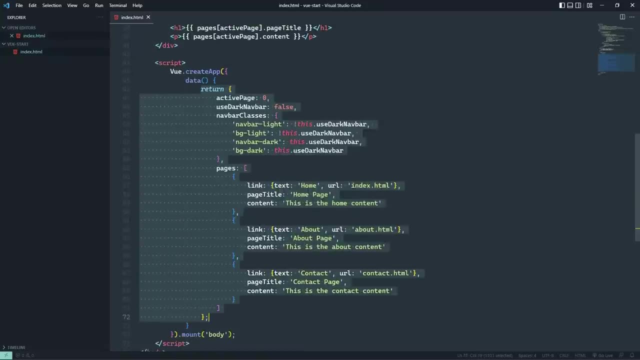 it's not working because we used our useDarkNavBar property. Because this code is initializing our application's data. It's not setting it up to be reactive or anything like that, it is simply initializing all of the values for these properties. So that means whenever the code executes to create this NavBar classes object, it is using the actual value of useDarkNavBar. 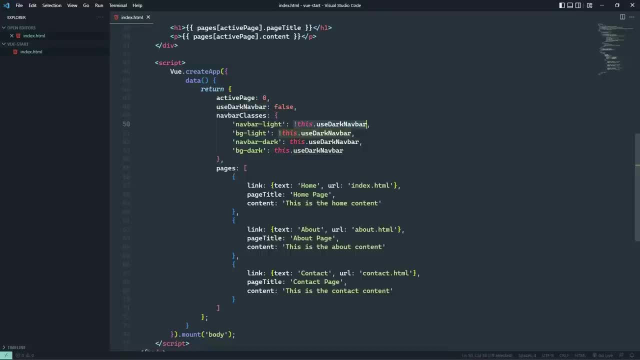 But it would essentially be translated into this, so that it will be not false. And the next line will be not false, which of course is true. 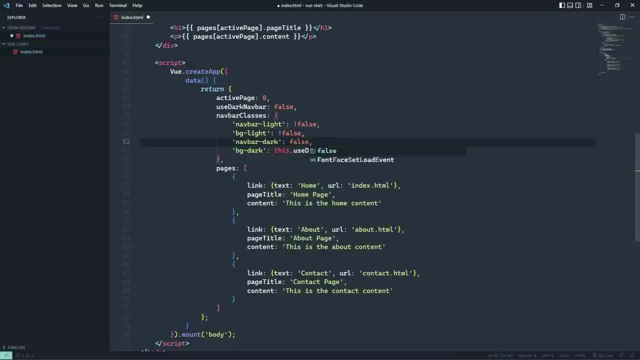 And then for NavBarDark, that would be false, and so on and so forth. So these are the actual Boolean values that are being applied to these properties. 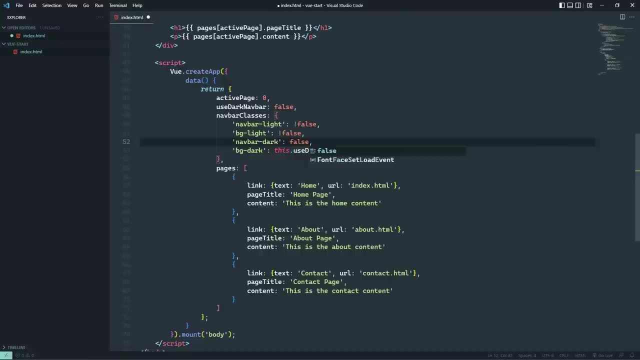 And so there's nothing that Vue thinks that it needs to react to. Inside of the browser, whenever we click on the toggle button, the useDarkNavBar property is changing, but that's not the problem. 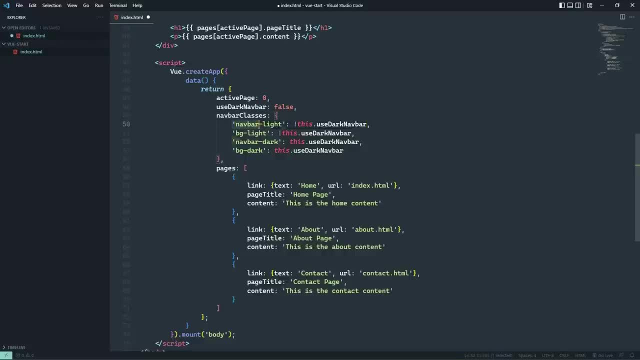 The problem is that the actual Boolean value is being applied to these properties. So the way that we can get around this is by using what's called a computed property. 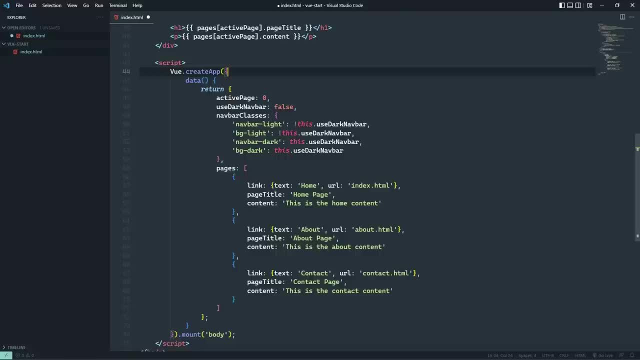 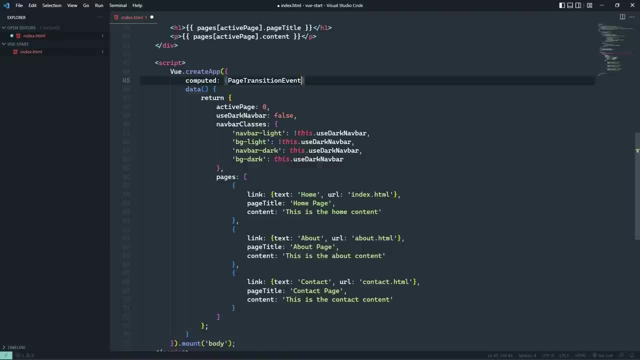 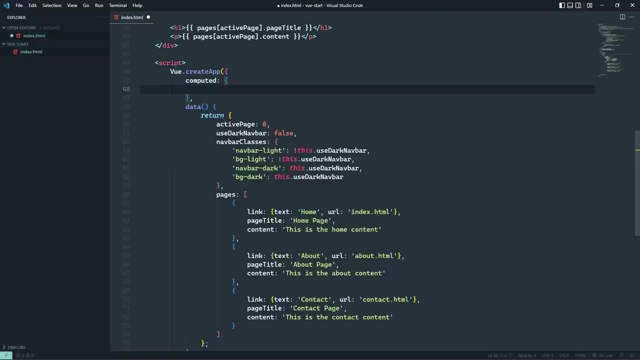 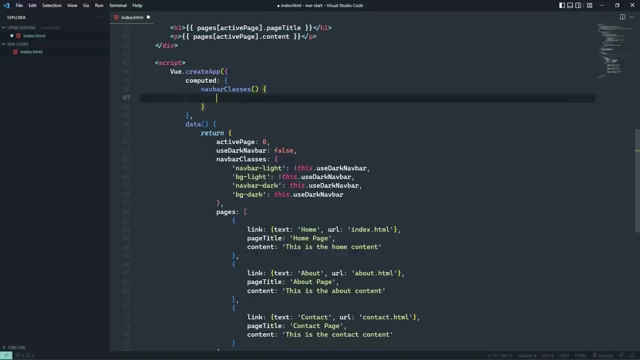 It is simply a property that is evaluated on the fly. And we create computed properties by using the computed option. So we have an option called data, which is what we've been using thus far. Now we are going to use the computed option. This is another object where the properties are functions that will execute. So this is where we will define our navbar classes. But this is going to be a function because this is a computed property. It has to execute in order to generate its value. And all we need to do then is essentially lift this code from our data. 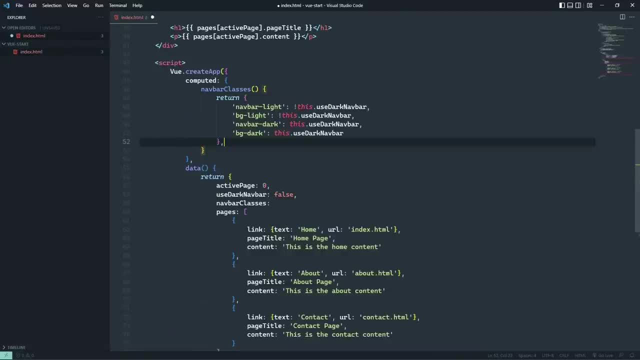 And we want to return that in order to generate its value. And we want to return that in order to generate its value. 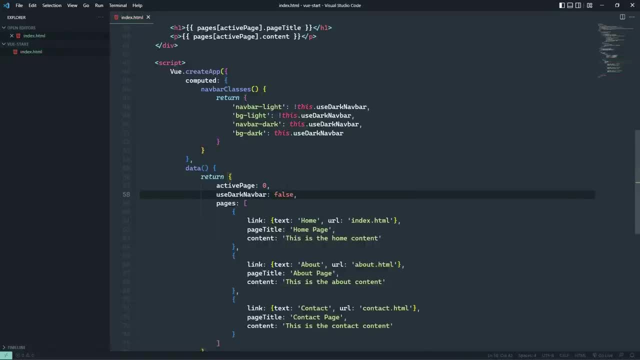 So the way that this works now is behind the scenes, Vue knows that useDarkNavBar is something that it has to react to. And because we are using it inside of this computed property, it will then automatically compute this value whenever useDarkNavBar changes. 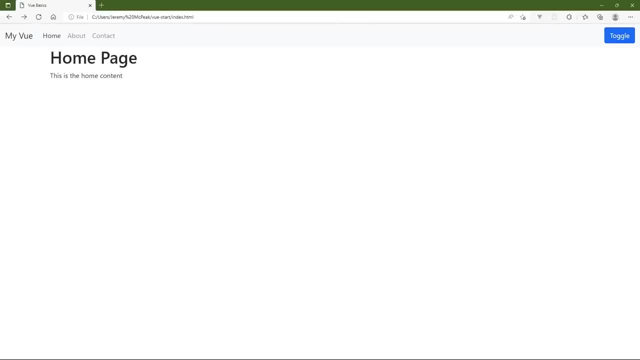 So we can go back to the browser now, let's refresh the page. And whenever we click on toggle, we see that that functionality is back. So because we click on this button, it changes the value of useDarkNavBar. 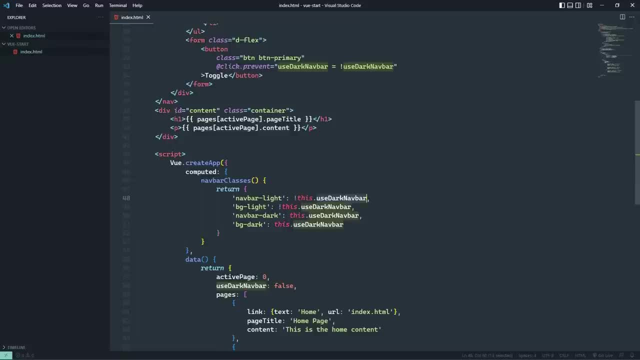 And because we used useDarkNavBar inside of this computed property called navbarClasses, it will automatically recompute this property. It essentially calls that function to compute it. 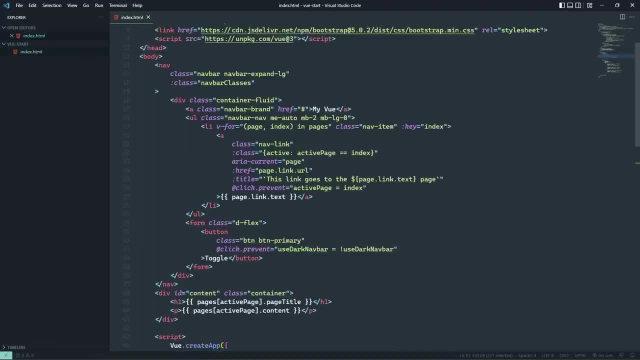 It returns the object that is then used to bind to the class on our nav. Now in the next lesson, we are going to look at how we can bind CSS classes using an array. 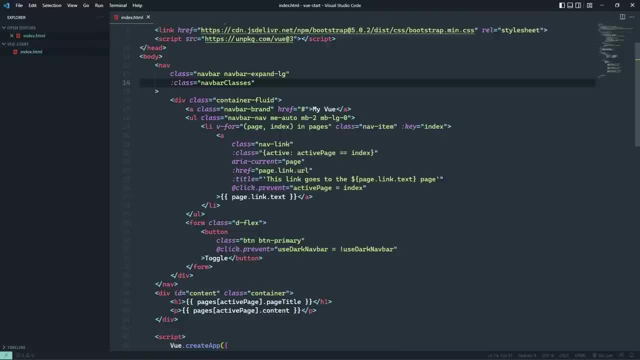 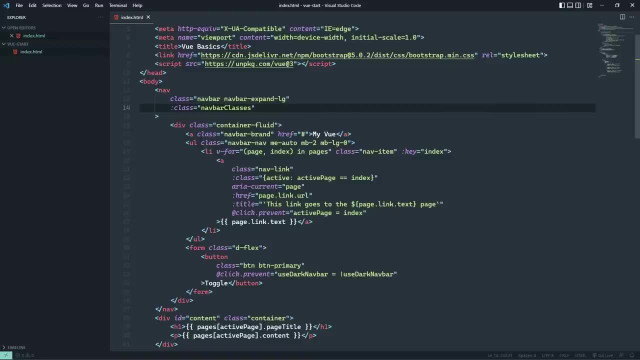 And how we can get the same functionality without using a computed property. In the previous lesson, I introduced you to computed properties, which are, 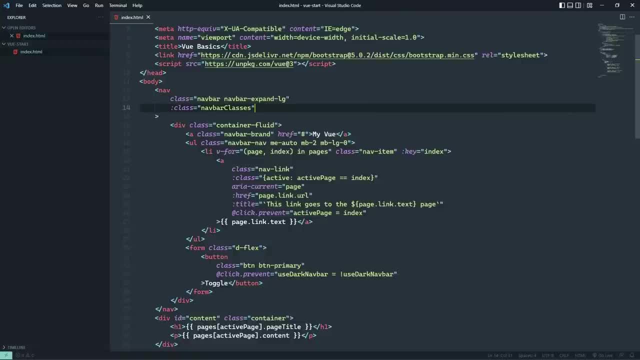 well, they're properties that are processed or computed on the fly. 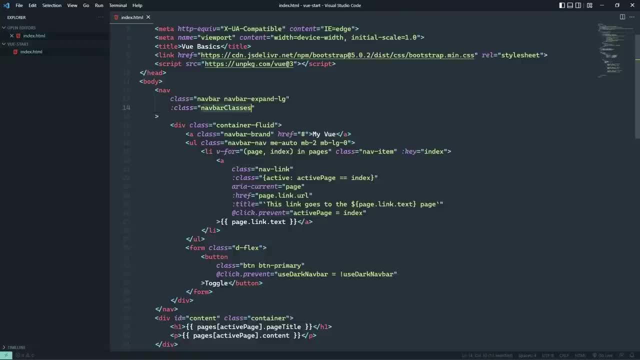 And we used a computed property to simplify our template, so that all we had to do was bind this navbarClasses property. And that just happens to be a computer. 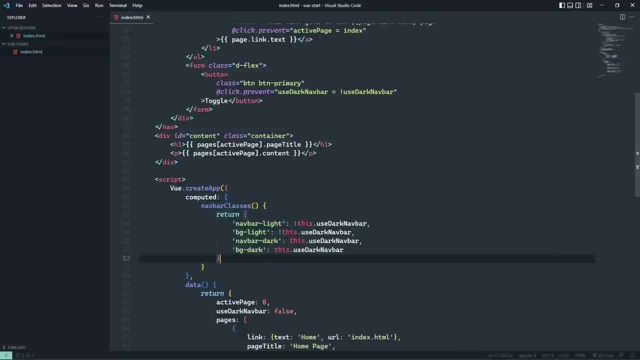 We have a computed property whose return value changes based upon the value of useDarkNavBar, and that's all well and good. 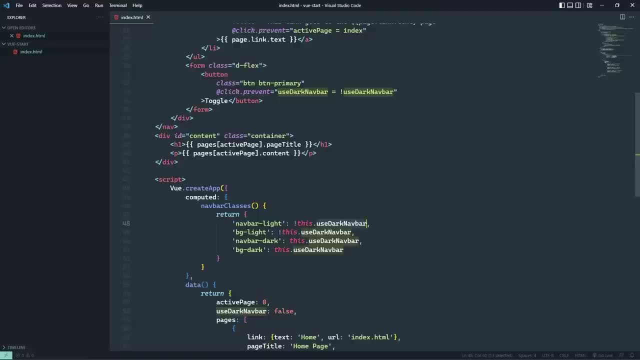 Computed properties are a wonderful feature. But we can also do the same thing without using computed properties. 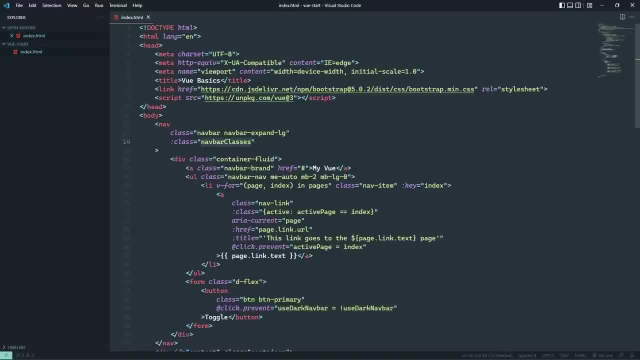 Because instead of using an object, we can use an array to bind classes. 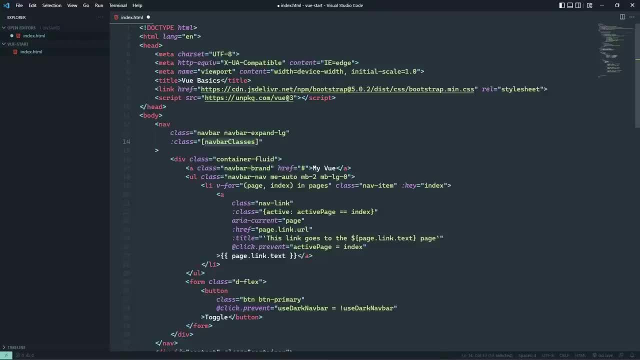 So the first thing we need to do is just define an array. And then the individual elements inside of that array will be the CSS classes, that are applied to the element. 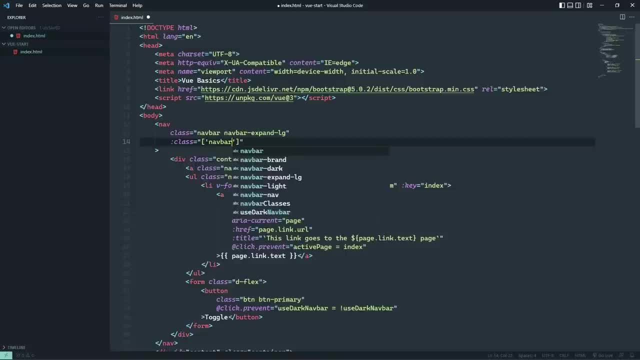 So for example, if we wanted the dark navbar, we would have navbarDark as one element in the array, and then bgDark would be the other one. 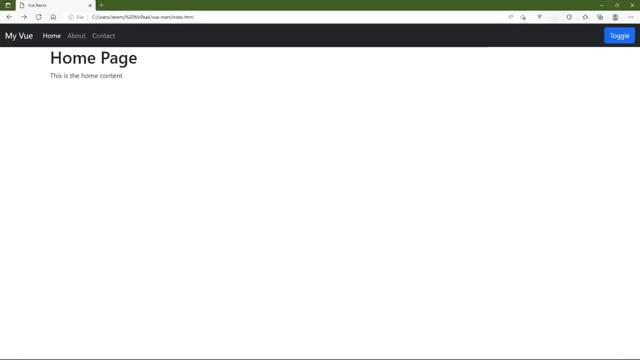 So we can hop on over to the browser, refresh and voila, we have that functionality. But of course, if we click on the toggle button, that no longer works, because we have hard-coded the dark CSS classes to our navbar. 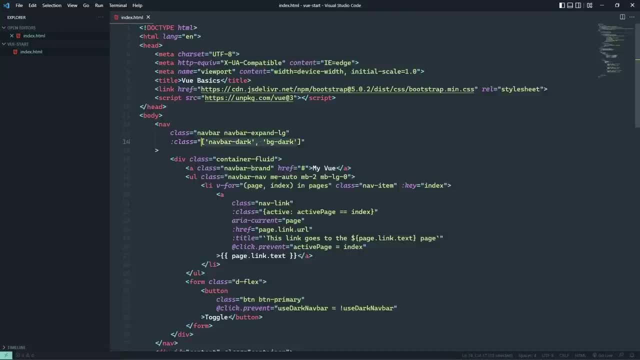 Now, without writing really any expression, any extra code, we can get away with doing something like this. 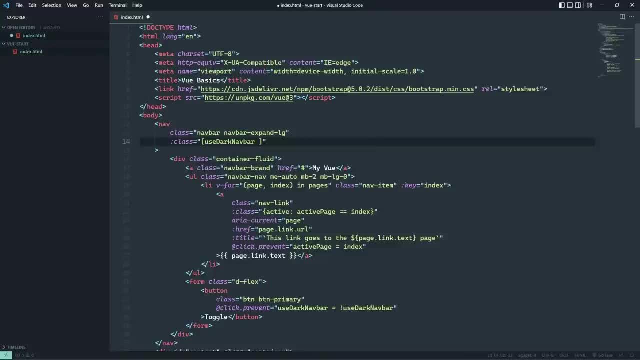 So that we would check the value of useDarkNavBar, and then we would have a ternary expression. 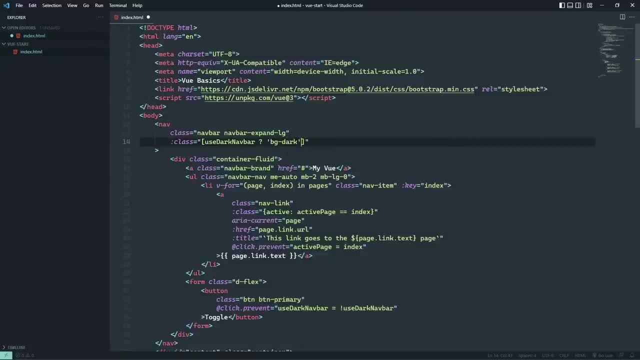 So that if this is true, then yes, we would use those dark classes. Otherwise, we would use the light classes. 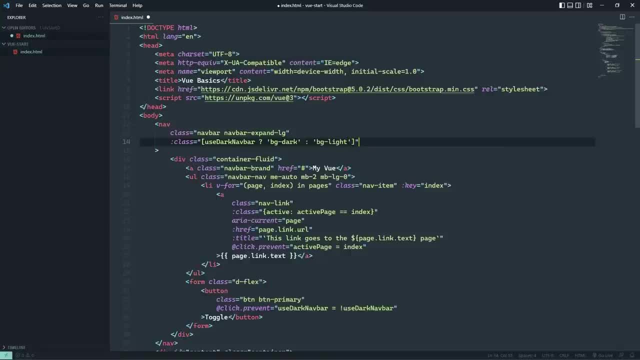 And I know that there's other CSS classes that we need to apply. I'm gonna be lazy and not apply them. 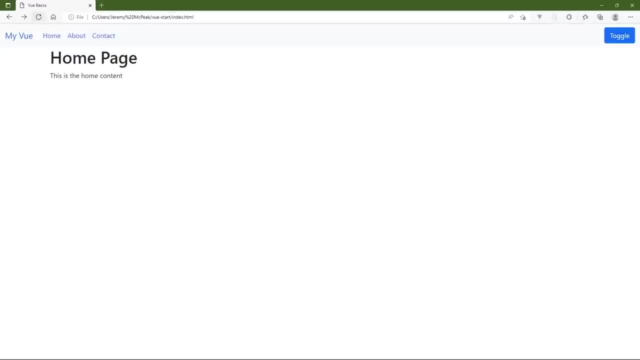 All we need to see is that the background color will change. So let's refresh. Let's toggle, and we have that functionality again. 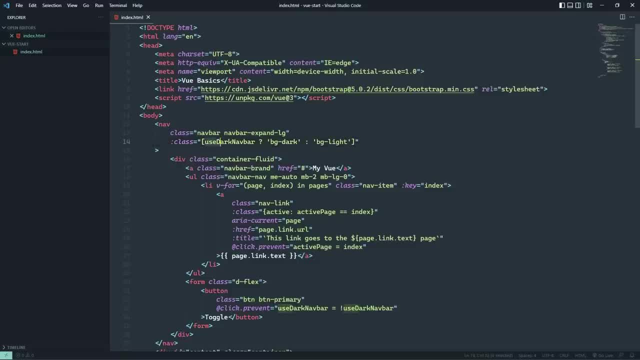 However, one can make the argument that our templates could be a little bit cleaner. I mean, yes, this is fairly clean, but the more CSS classes we add, the more of a headache it's going to be to try to decipher all of this. 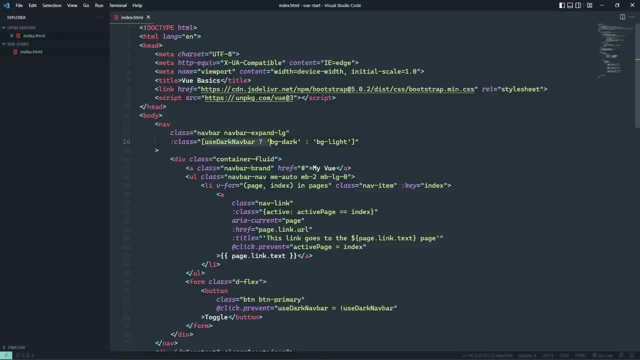 Now, before we want to move on, I want to note that this expression is for just one element in the array. 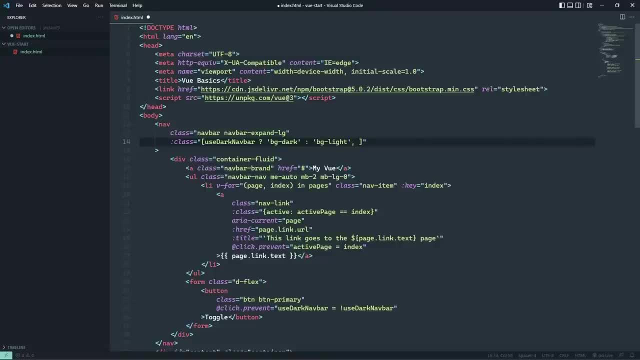 If we wanted to apply any other CSS classes and always apply them, like for example, navbar and navbar-expand-lg, we could do that just fine. 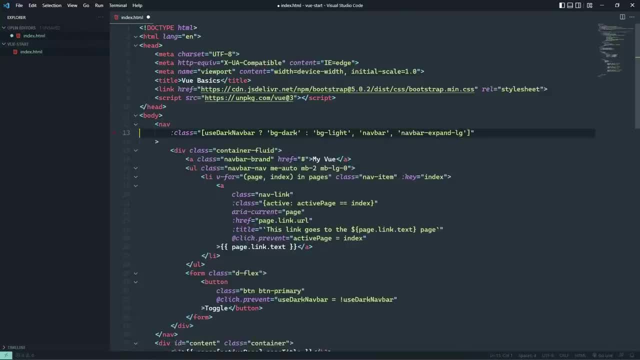 In fact, let's go ahead and do that, why not? So just as a sanity check, let's go back to the browser. 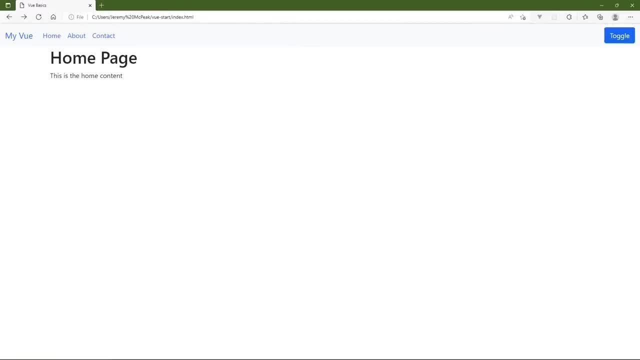 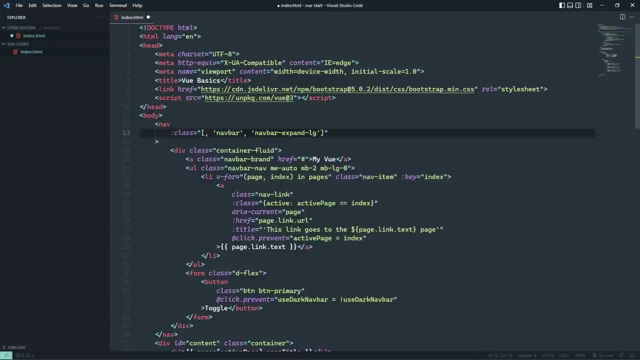 We will see the same functionality that we got before. All of the static CSS classes are still being applied because this would look very different, but we can still toggle between the light and the dark. But I want to do something not necessarily fancy, but it would be cool to do something like this, to where we would have our individual elements. But then we would have like a theme property, and then we would change the value of that theme. So that the navbar and the background colors would change based upon that theme. 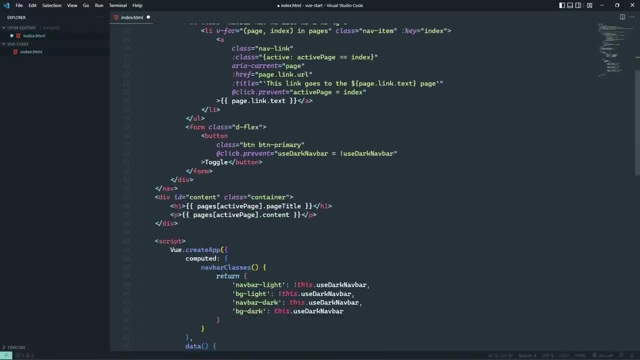 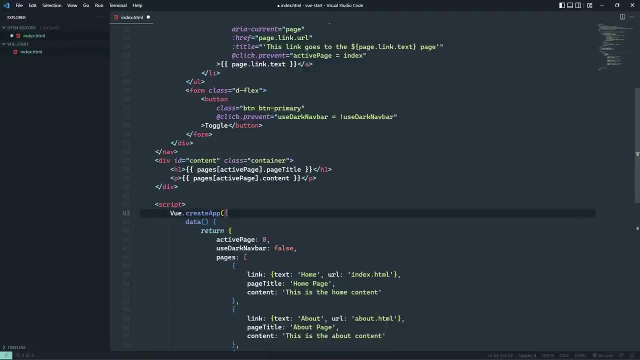 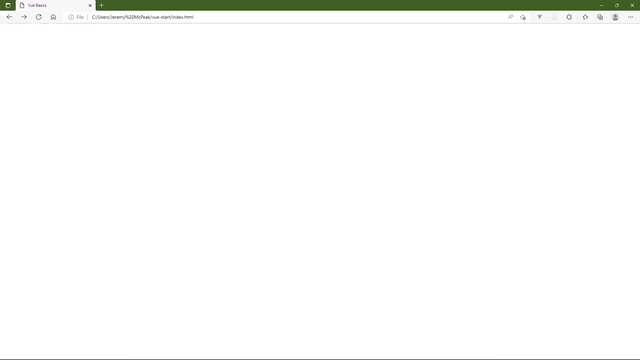 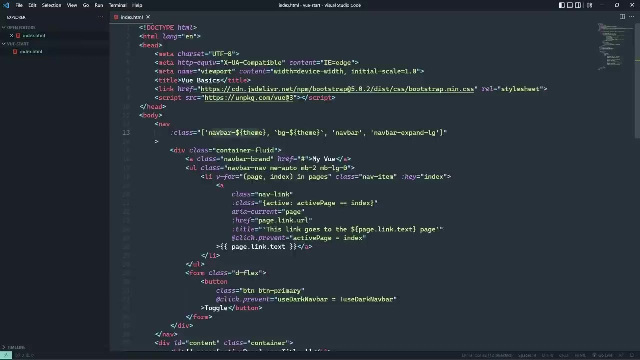 But of course, everything else would be fine. Now, this gets us away from using this computed property. So let's go ahead and delete that. This also gets us away from using this useDarkNavbar. Instead, we would have a property called theme to where we could initialize it as light or dark, really doesn't matter. Let's go ahead and let's start with light. Let's refresh, ooh, there's an error somewhere. It's probably a syntax error, and there it is right here inside of my template. I need to have that closing back tick. 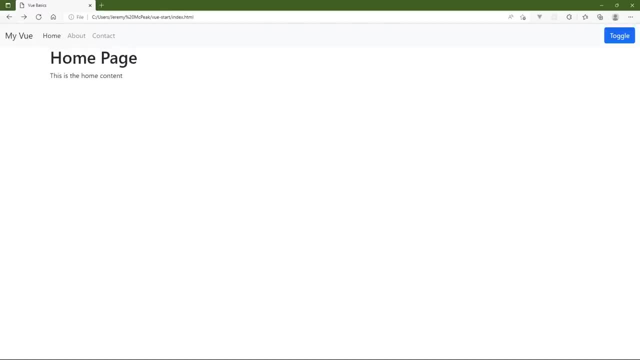 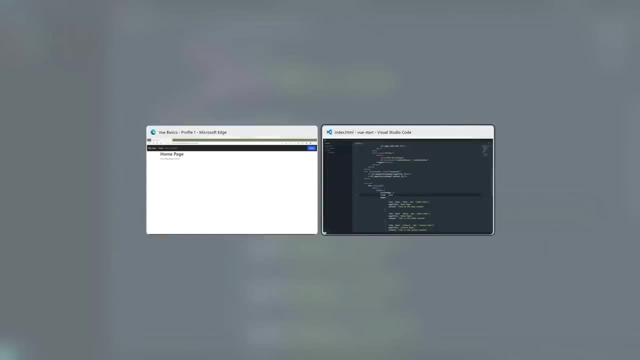 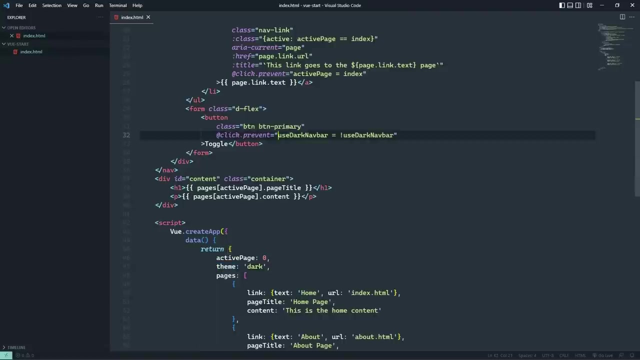 So let's go back, let's refresh, looks like a light navbar. If we change theme to dark, you will see the dark navbar, there we go. So now we just need to write the code that's going to change the value of theme. Now, we can do that like we've done for the useDarkNavbar property. In that, whenever we click on the toggle button, we could do something like this. To where we will assign a new value of theme based upon what its current value is. So that if theme is light, then we want to change the value of theme, and we want to change its value to dark, otherwise it's going to be light. 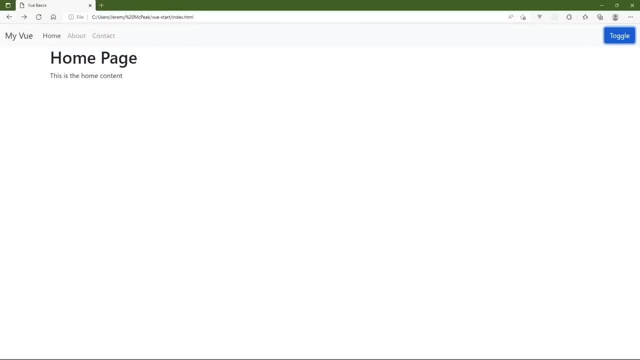 And that is going to give us the functionality that we are after. However, once again, I would make the argument that this complicates our templates. Now we have to decipher that. 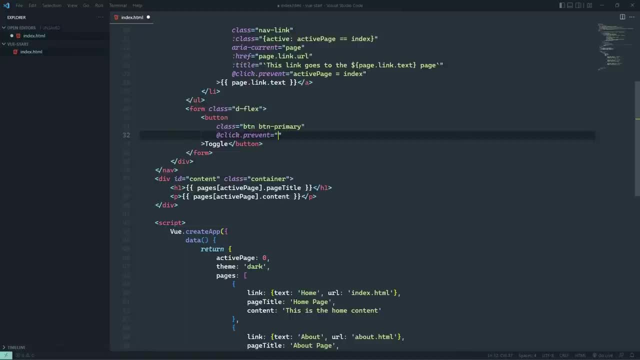 Wouldn't it be cool then if we could just have like a function that would execute? Because in a real world application, that's typically what we would do to begin with. 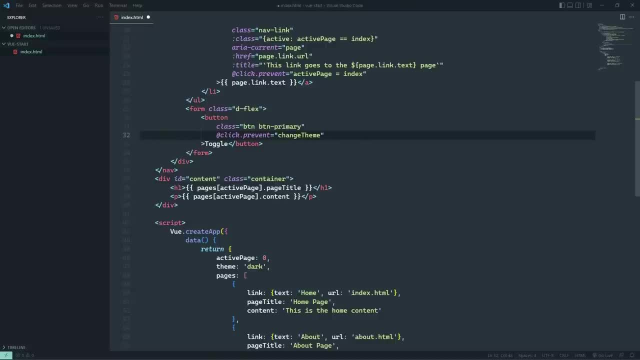 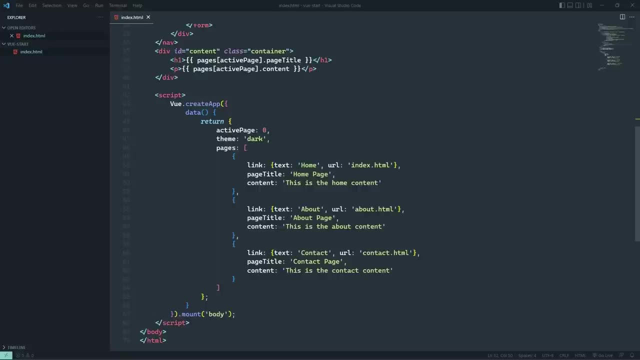 So we could have a function called change theme. That we would call whenever the button is clicked. So let's do that. We just need to add a method to our application, and we do so by using another option. 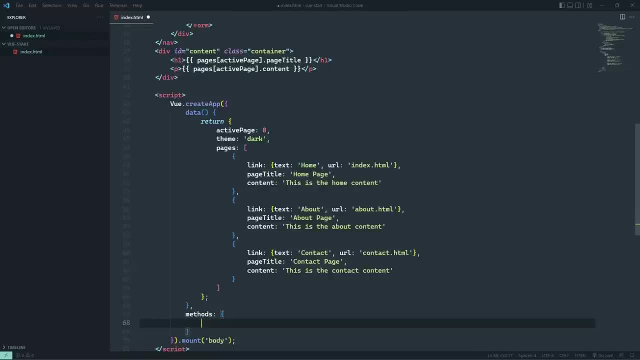 It's called methods. And inside of the methods objects are all of the methods that we want to define. 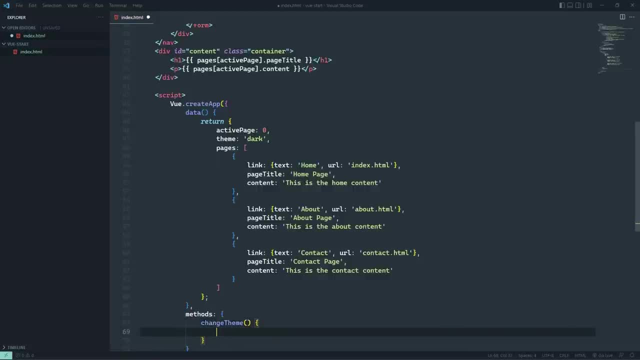 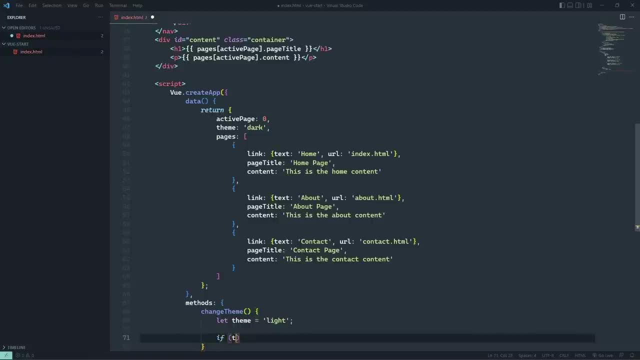 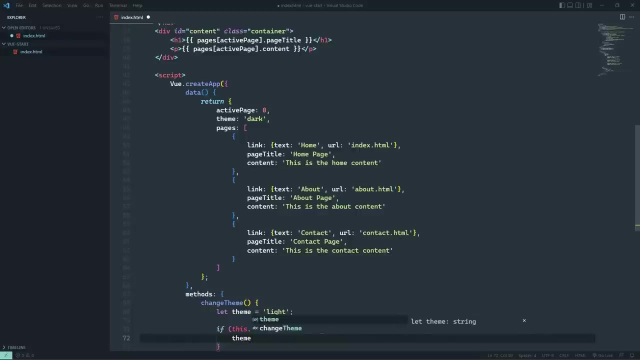 So in this case, we will have the change theme method. Let's start by creating a local variable. We will initialize it as light. And then we will check the current value. Of our theme property. If it's light, then we are going to set that theme variable to dark. 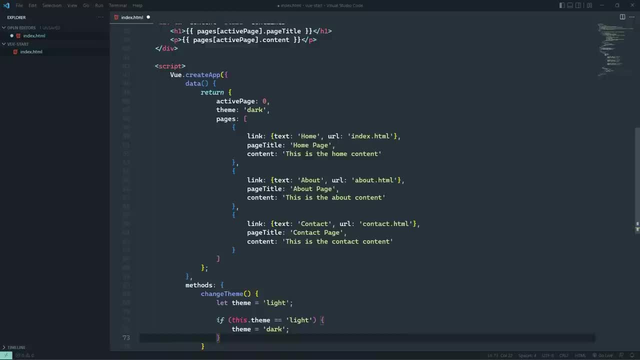 Otherwise, the current value of theme is dark. 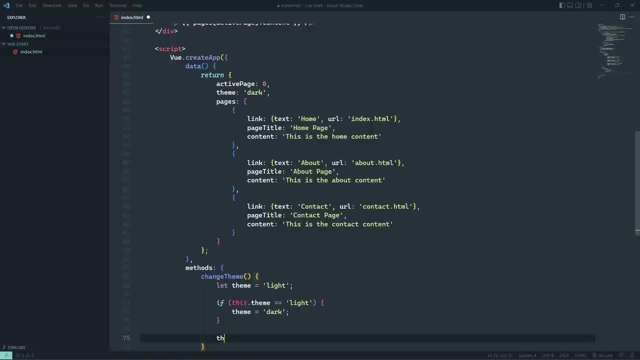 And we already have light assigned to themes. So that the final line of this method is simply going to define our theme property, the value of the theme variable. 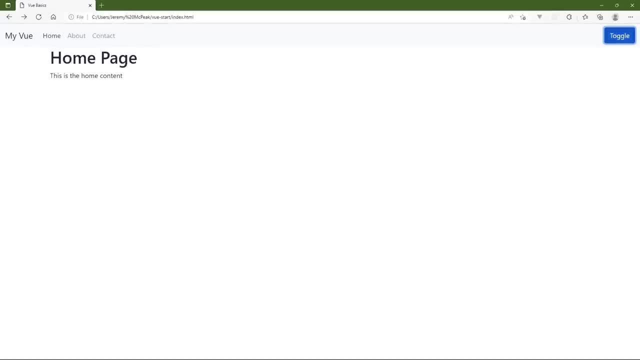 So let's go to the browser. Let's refresh the page. Let's click on toggle, and we see that we have the same functionality. 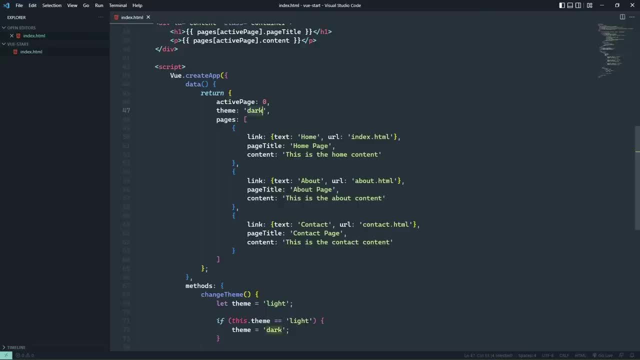 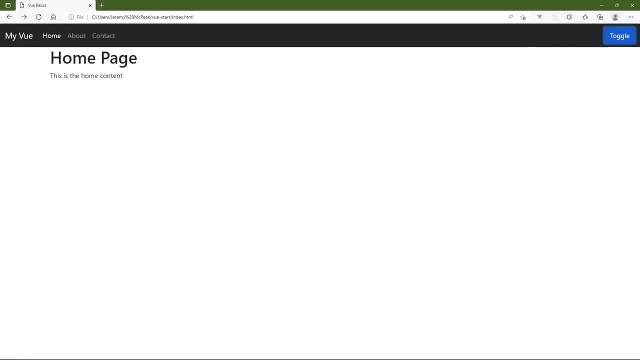 And of course, we can change the value of theme from dark to light, so that the nav bar will start off as light. And then whenever we click on toggle, it toggles it to dark. 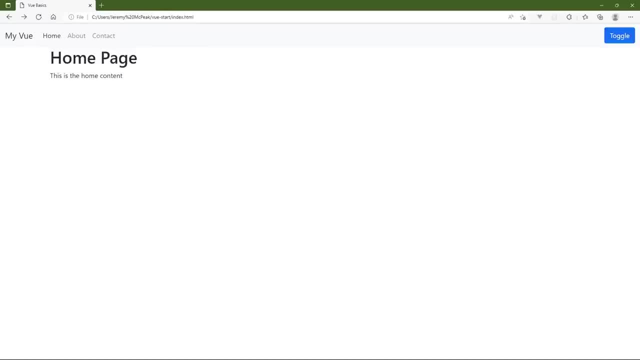 So one thing you're going to find, not necessarily with Vue, but just any framework at all, because all of these frameworks are based upon JavaScript. 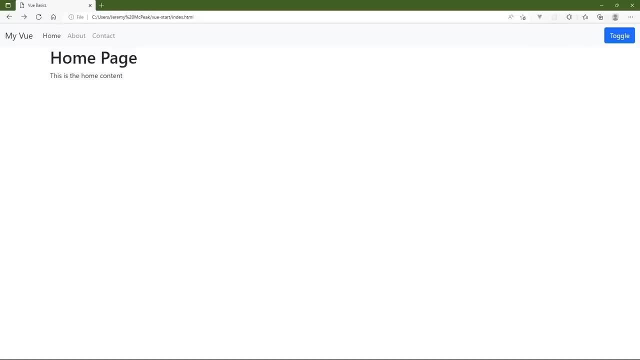 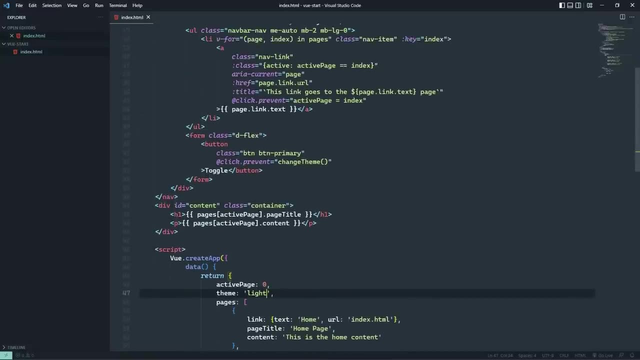 And when it comes to JavaScript, you can accomplish the same thing in a variety of different ways. Just like here, we have accomplished the ability to toggle and toggle our nav bar's theme in three different ways. 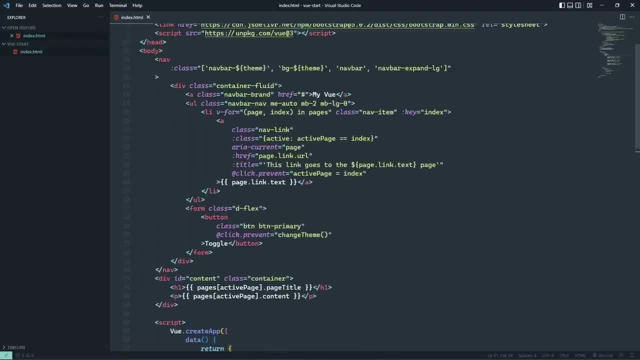 We've used computed properties, we are now using arrays and methods. And then we had an approach that didn't have anything. We just had a somewhat complex expression inside of our template. 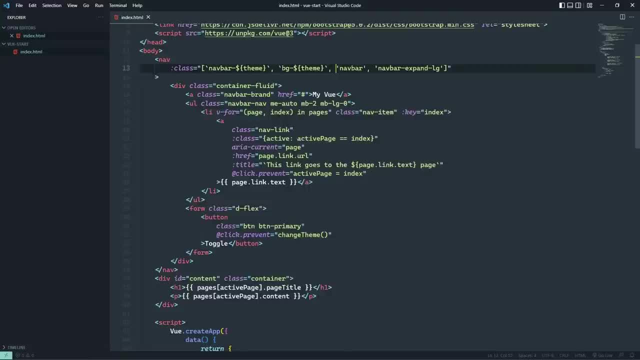 And so just like JavaScript, where we have several different ways that we can do the same thing, just because we have different ways doesn't necessarily mean that one way is better than another. 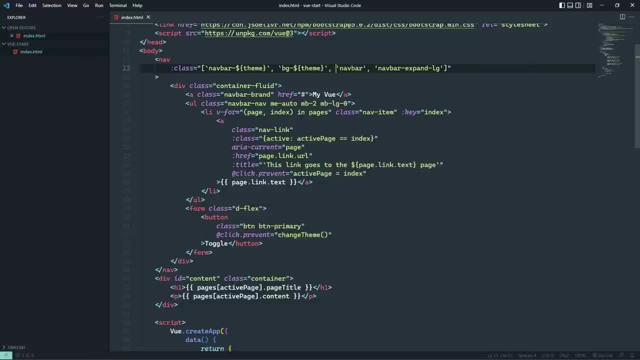 It's all going to boil down to the situation and what makes most sense to you. 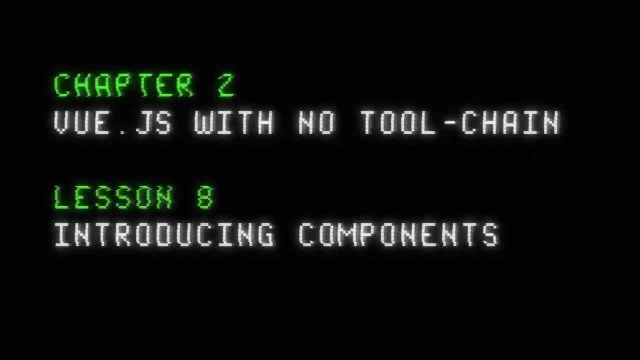 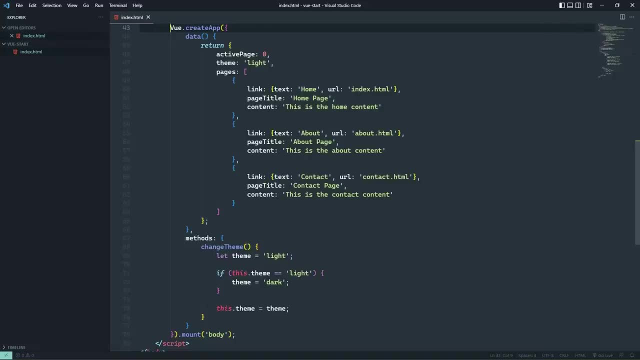 Our application is very simple, but it's also becoming a little unruly because we have all of this code just kind of thrown together. And if we took the time to study this application, we would essentially find two distinct pieces. 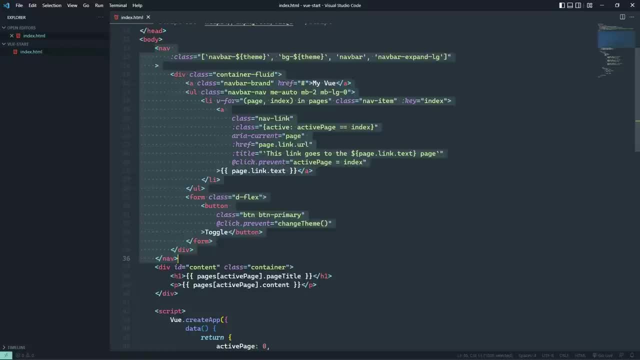 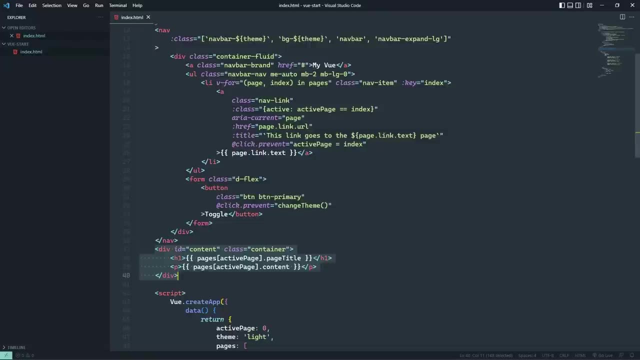 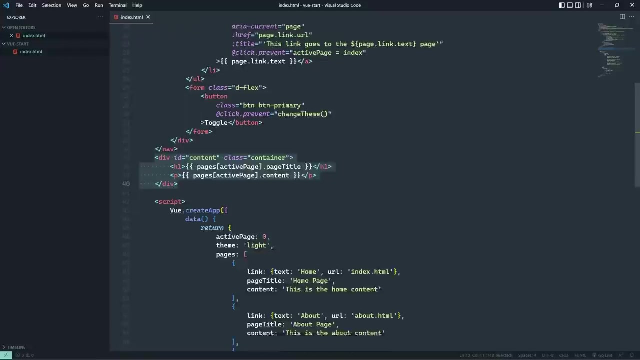 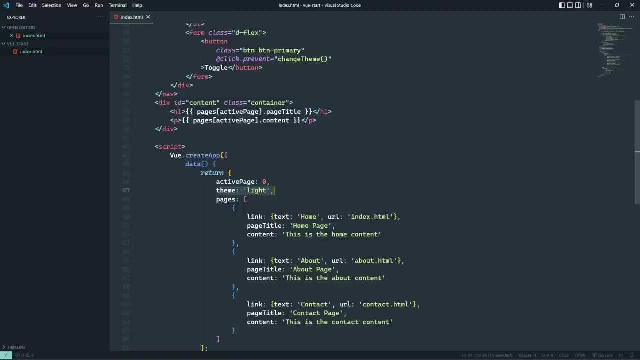 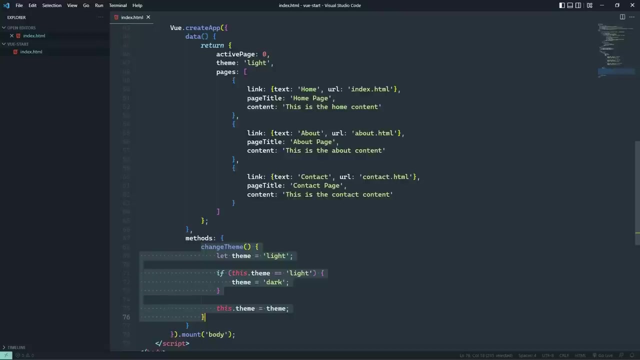 We would have the nav bar, and then we would have the content. And if you'll remember, whenever we started this journey in Vue, we essentially separated those two things. We had to view applications, one for the nav bar, and one for the content. In reality, it really doesn't make sense to have two separate applications, because they are related in some way, they are using the same data. At least as far as the active page and the pages. Now, however, theme and the change theme items are specific to the nav bar, so it still does make sense to separate the, and these two pieces, but we don't want to create different applications. 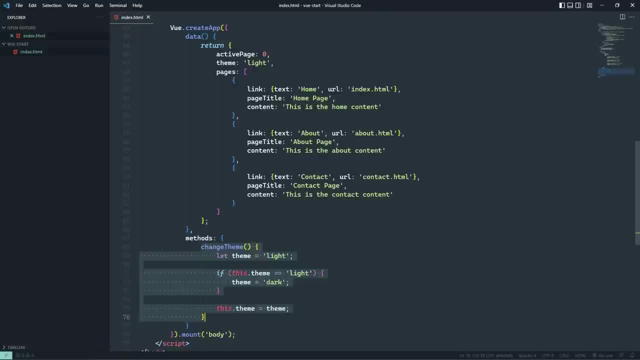 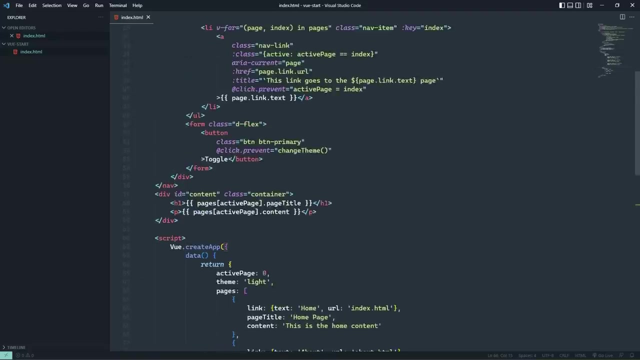 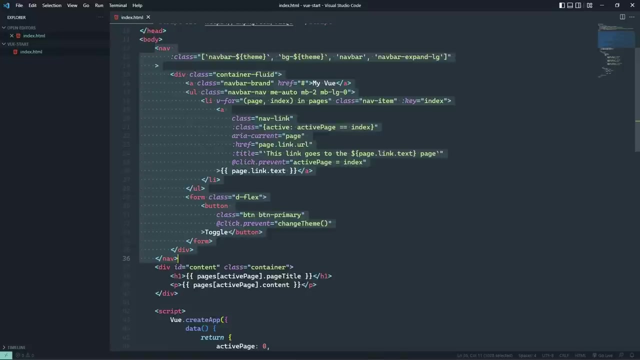 Instead, we will use what are called components. And you can think of a component kind of like a little mini application inside of a larger application. It's so that we can make our applications easier to write and maintain. But it's also so that we can extract functionality into a smaller piece that is specific for that functionality. Like for example, the navbar can be its own component. And it would be responsible for doing whatever the navbar does and only what the navbar does. 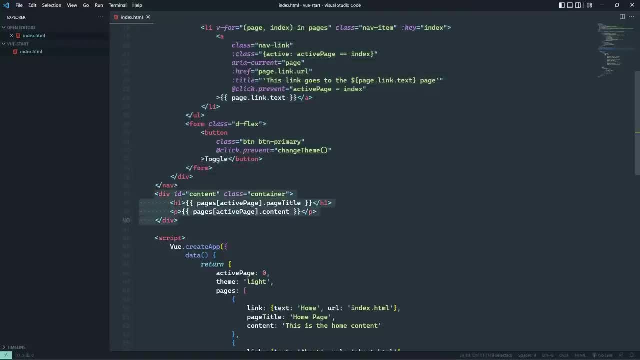 So in this lesson, we are going to create a component for displaying the page information. 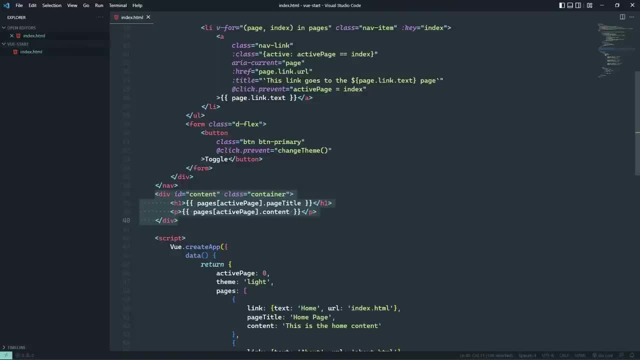 Because this will give us the opportunity to talk about a lot of the fundamentals. So that in the next lesson, whenever we create a component for the navbar, 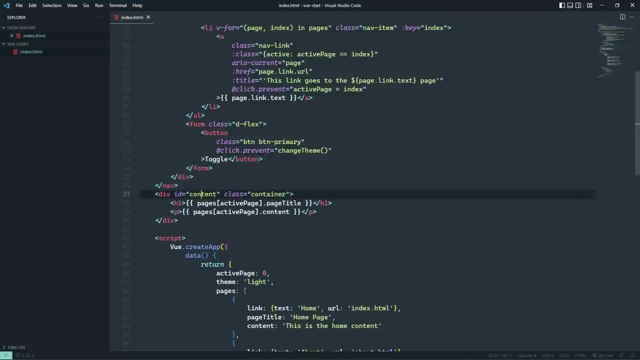 we can go into some more complex. 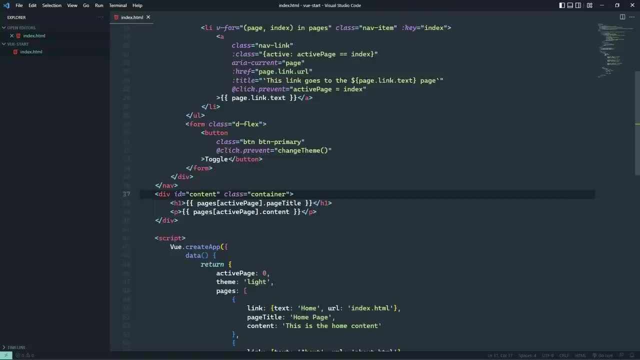 So we want to create a component for our content. The first thing we need to do is create a variable for our application. 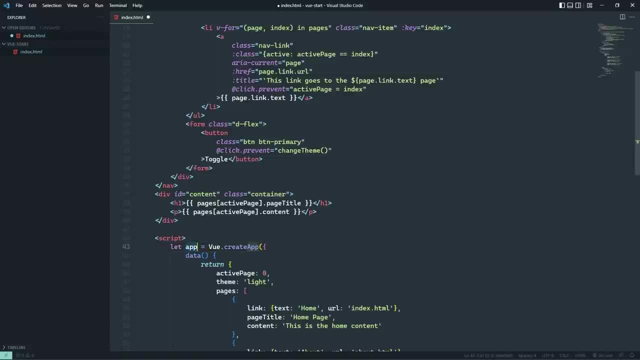 Because we need to reference our application in order to create a component. 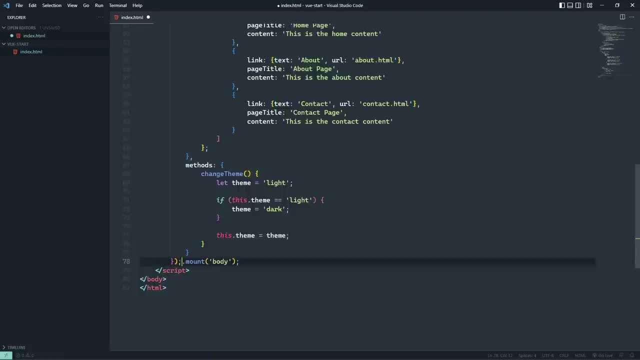 And we need to do that before we mount this. So we're going to separate these into two statements so that we create our app and then we will mount our app. 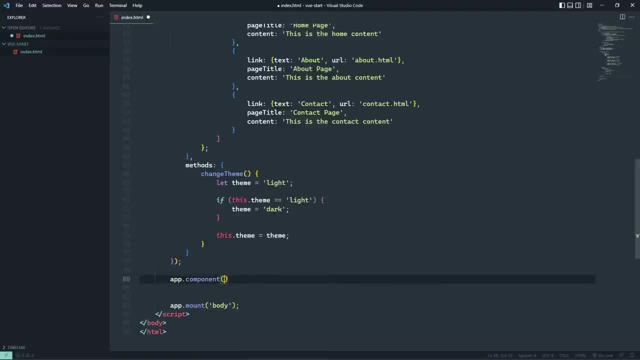 And before we mount the app, we want to create our component and we do so with a method called component. 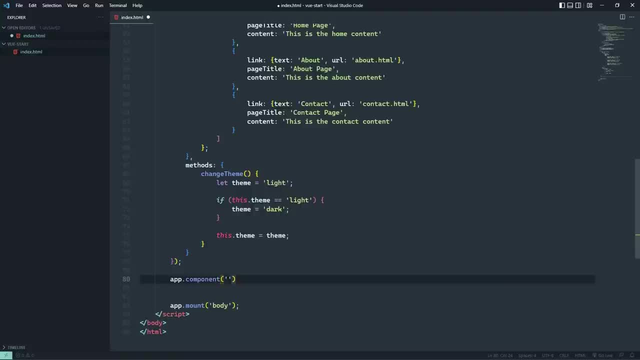 The element that we pass is a string name for our component. Now, there are some conventions that we need to follow here. It needs to be lowercase. And if it's just a simple word like page, then we just call it page. 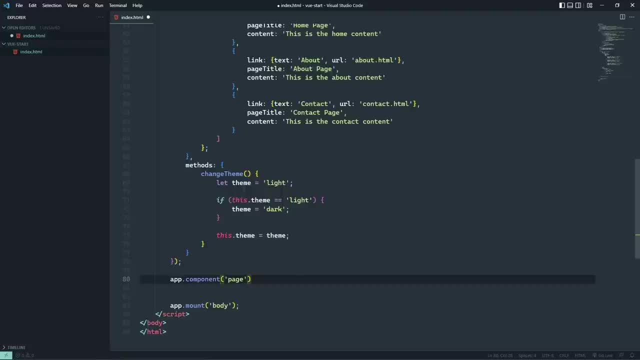 It also helps to not be an actual HTML element as well. But this is something I would call page content or page viewer. 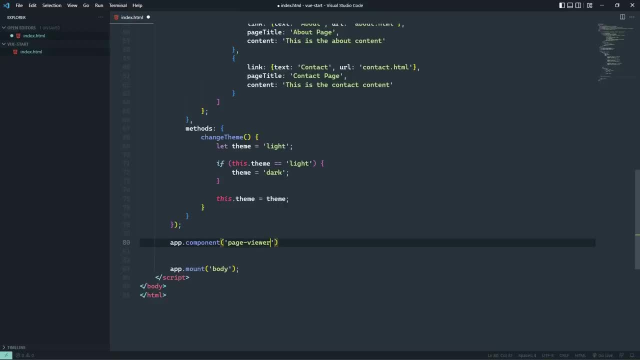 So if you have multiple words, then you will want to separate them with a hyphen or a dash. 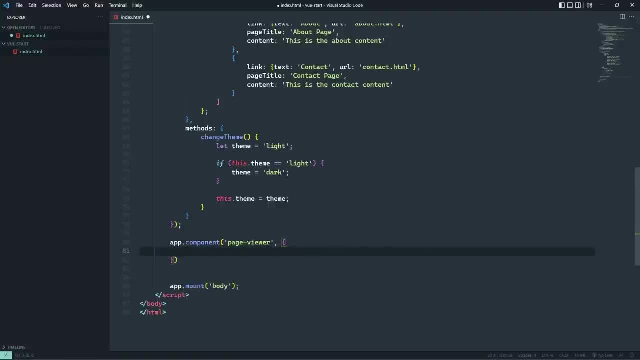 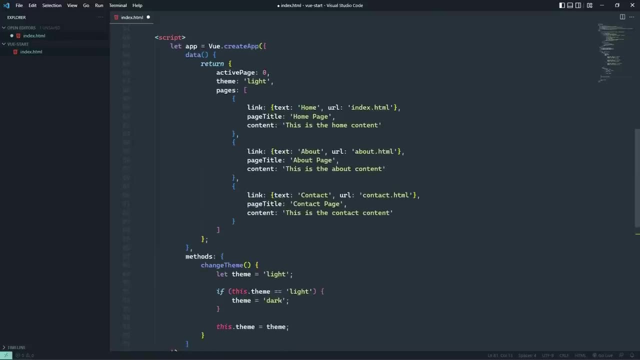 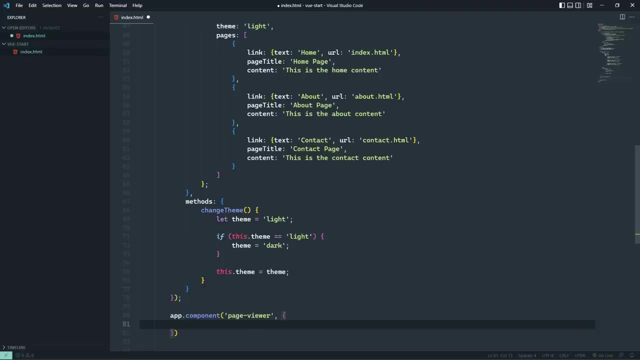 Now, the second argument that we pass to component is an options object. So all of the ideas and concepts we've talked about thus far, such as data, computed properties, methods, all of those are options. All of those can be used inside of a component. And the option that we are going to start off with is called template. 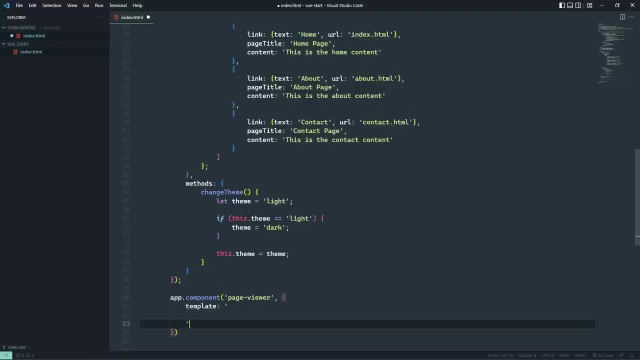 Because remember, an application needs a template and as I mentioned, a component is kind of a little mini. 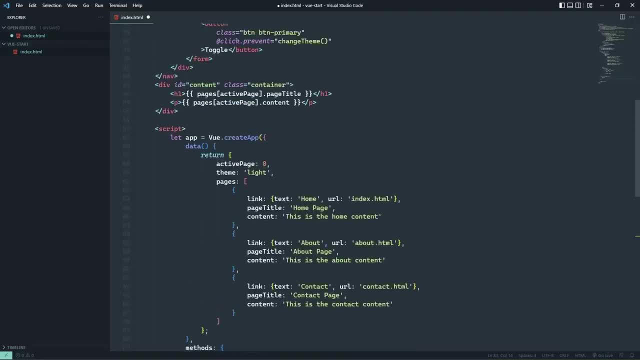 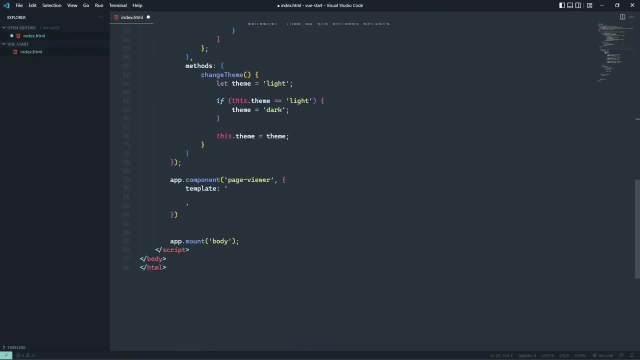 Application inside of our larger application. So we're going to take the markup that we have for displaying our content. Let's take that out of the body and we're going to use that as the template for this component. 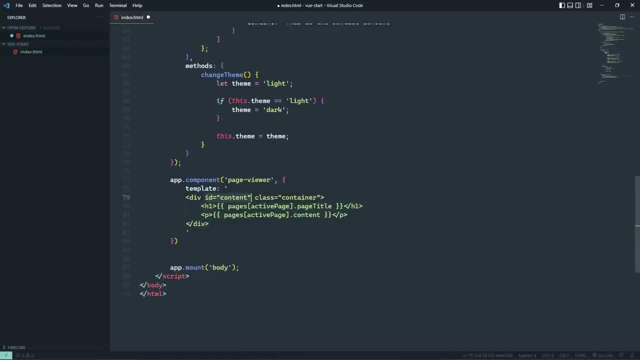 Now, we don't necessarily need this ID attribute, so let's get rid of that. We haven't needed that for a while. And as it is right now, if we tried to use this, we would run into an error. 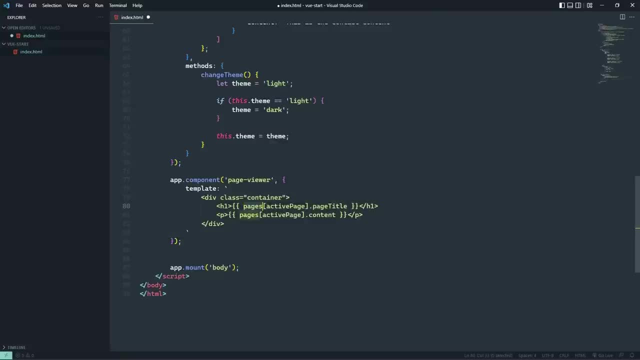 Because this component is trying to use the pages from our application. And by default, it doesn't have access to that information, because it is now inside of its own component. 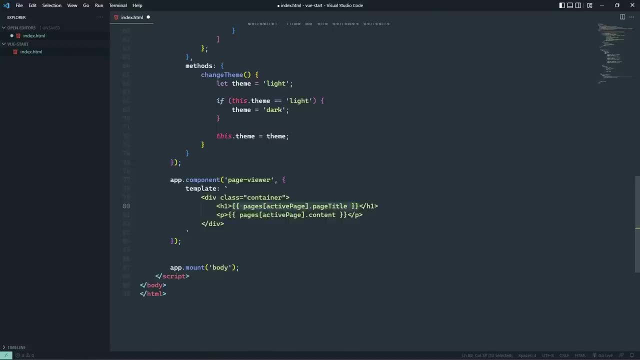 So for right now, let's get rid of where we are outputting this data. And let's just have some placeholder text, so that we have page title and then page content. 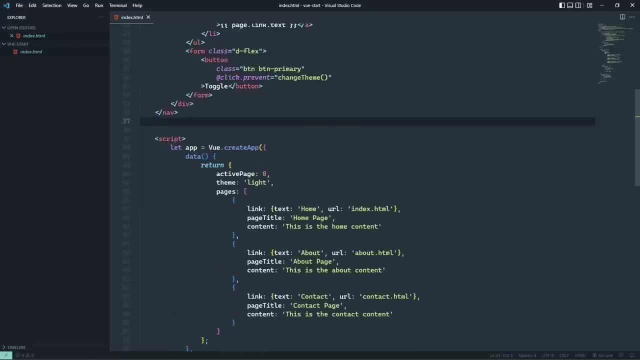 And then we will use this component inside of our application. And we do so as a normal HTML element, except that it's not HTML. This is a view component. 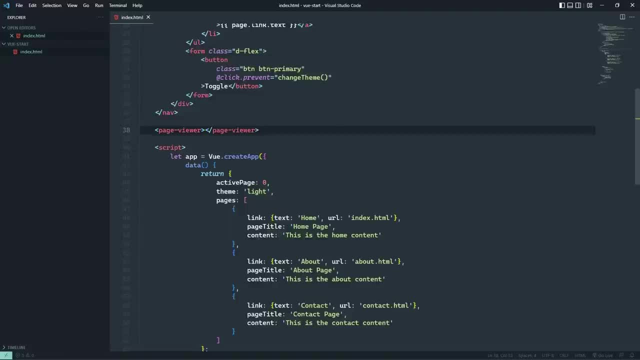 So we have an opening and closing tag. And whenever we go to the browser, let's refresh the page, and we will see page title and page content. So that's working just fine. 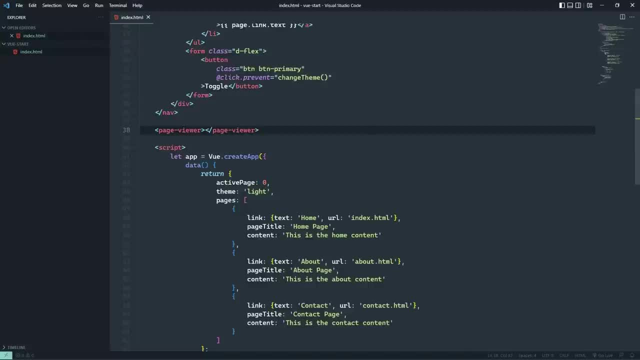 So now, we need to supply information for the page viewer to do its thing. It is responsible for displaying the page title and content. So we need to pass data, kind of like we would pass data to a function. Except that in view, we use the term props. So a component has props that we pass data to. 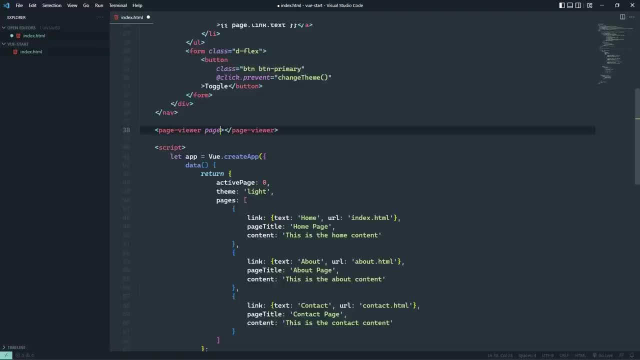 And we can pass data in two different ways. The first is going to look like just normal HTML attributes, except that they are going to be specific for these components. So we can say that we would have a prop called page title, which is just going to be a simple string. So we could have page title like that. And then we could also have page content. And once again, notice how I'm typing the text. I'm typing these out. 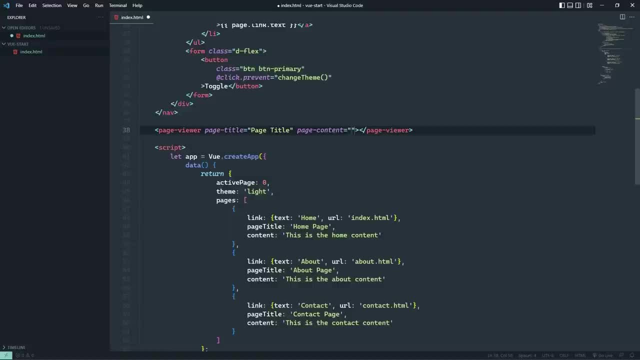 They look like normal HTML attributes, so that they are all lowercase. If they are multiple words, they are separated by hyphens. 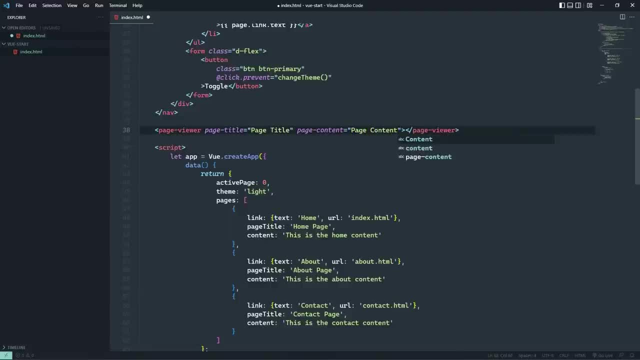 And we'll have page content here. And let's have something different, so that whenever we view this in the browser, we will see the difference there. 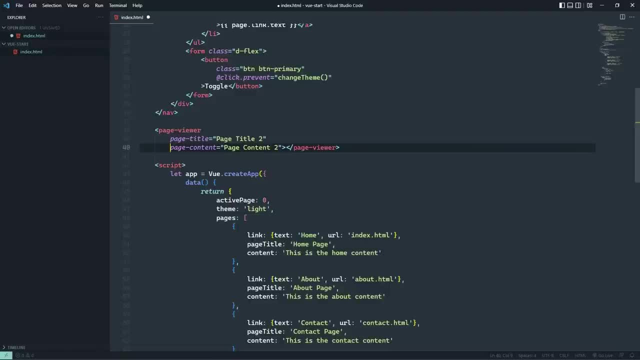 So we have these two props, and that's great, but it's not enough to just supply values to them. We have to define them inside of our component. So this is another option that we will specify. 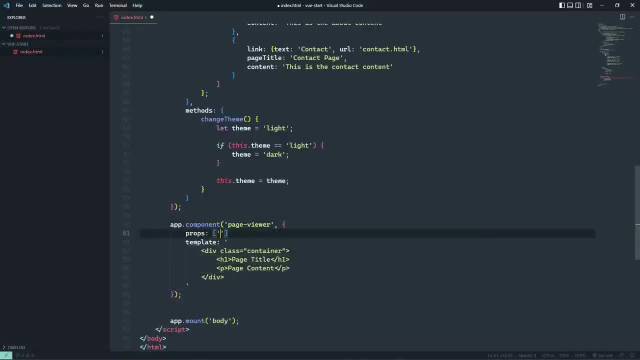 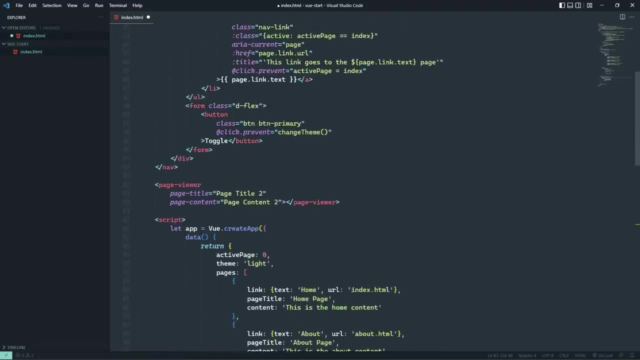 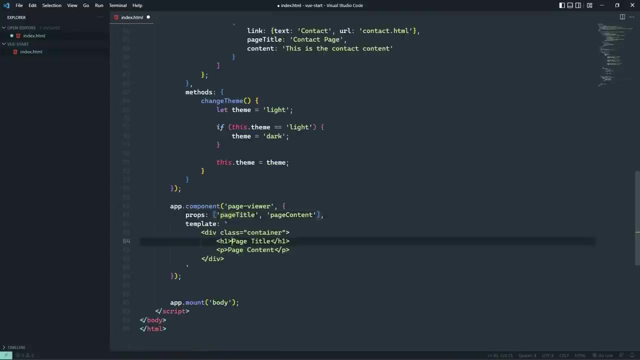 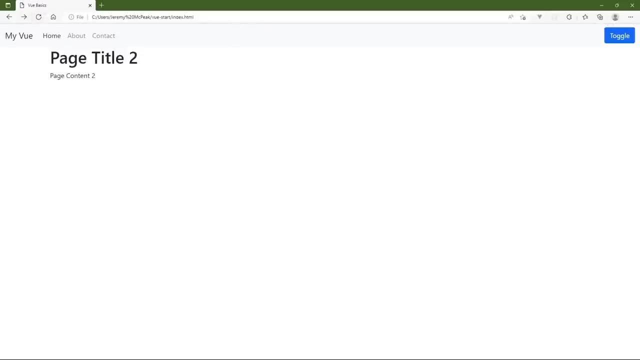 And it's simply called props. And it is an array that contains the name of the props. Except that here, we are going to use camel case. So we have page title and page content. So when it comes to our markup, we use what would be typical markup attributes. But when it comes to JavaScript, we use camel case. So now we can use page title and page content inside of our components template. We will have page title, and then page content. And whenever we refresh the page, we are going to see our title and content change based upon the data that we passed to those props. 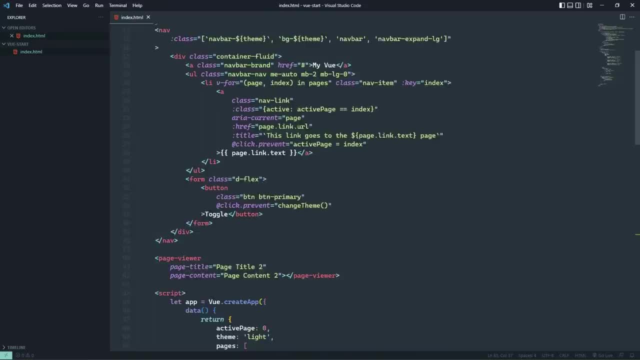 So this is the first way. We are passing just simple string values. And it's important to remember that distinction. 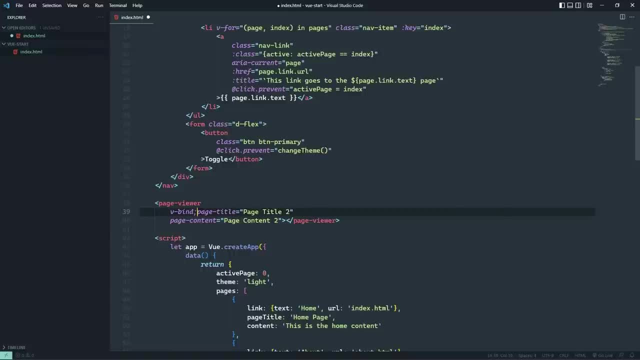 Because we can also use the vbind directive with our props. In which case, we are binding some JavaScript, and we're going to have to do that. So we're going to have to do that. And we're going to have to do that with our script expression too. But as you know, we don't have to say vbind. 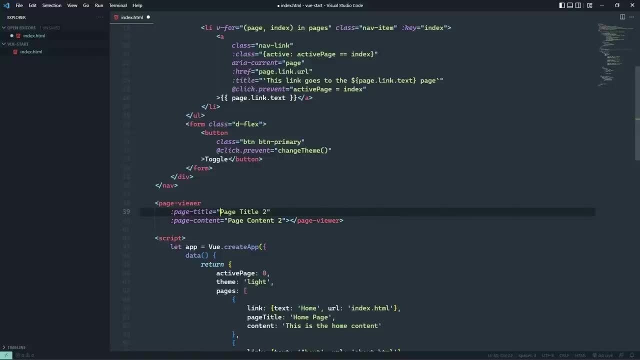 We can just use the shorthand, which is a colon. So in this case, if we wanted to use a string value, we would have to surround these with string delimiters. 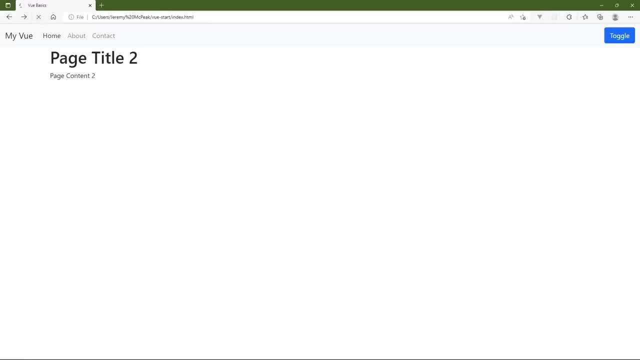 Which in this case are just simple single quotes. We refresh the page, we see the same result. 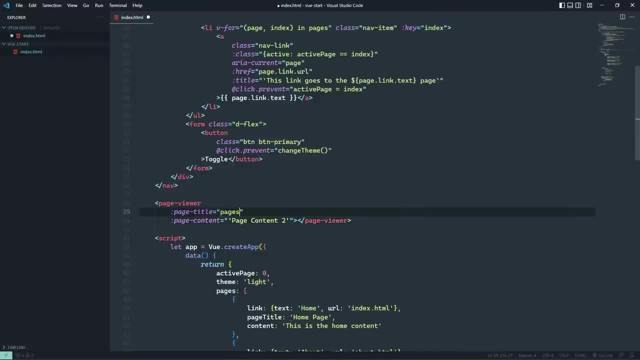 But we want to be dynamic here. So that we display the title and the content for the active page. So this is going to look somewhat similar to what we had before. Except that now we are passing this information as props. 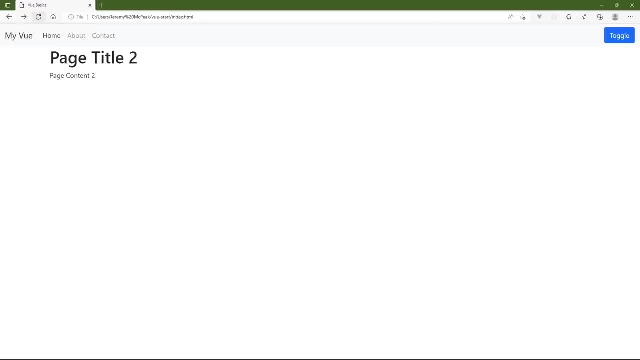 So whenever we go to the browser, we are going to see the same functionality that we had before. 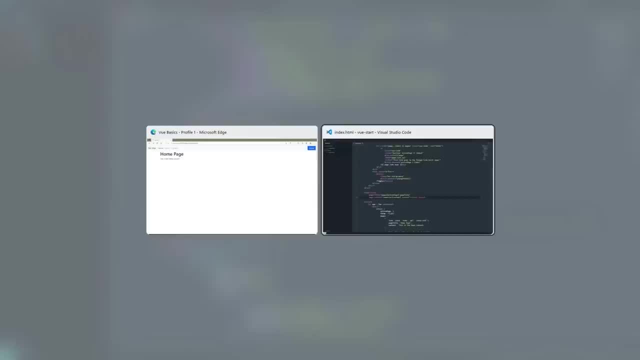 Homepage, about, and contact, that's great. However, I think that we can make this a little bit better. 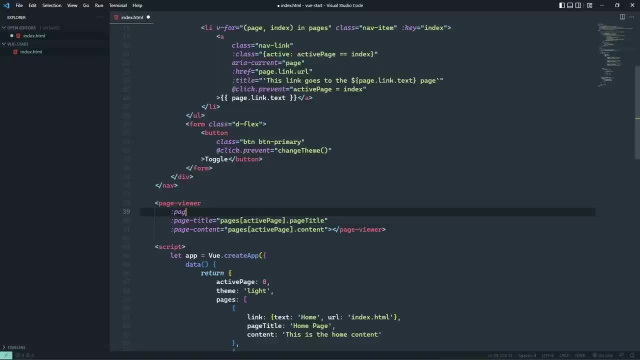 So that we have just a single prop that we can call page. And then we will pass in pages with the index of active page. So that inside of this, inside of our components, we would then use the page title and content properties. 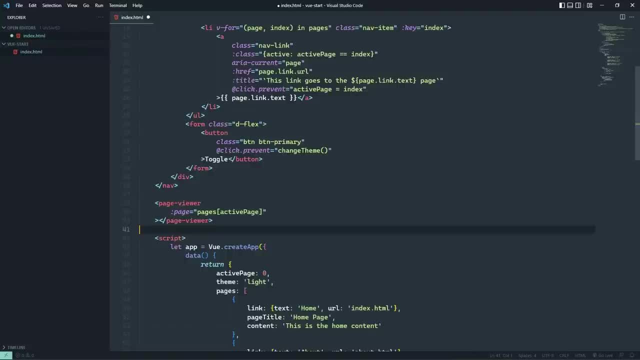 So whenever we use page viewer, this is all that we have to supply. 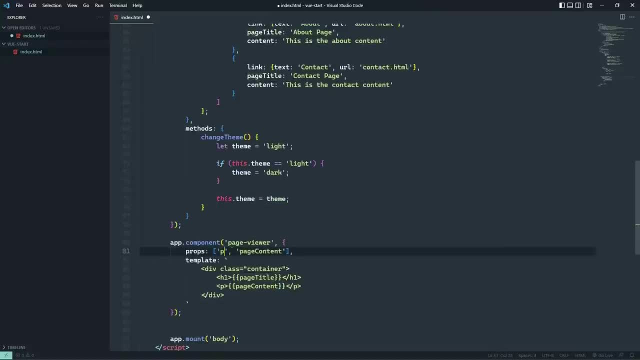 And then we just need to update our page viewer component so that it has a page prop and it is going to display the page title and then the page content. 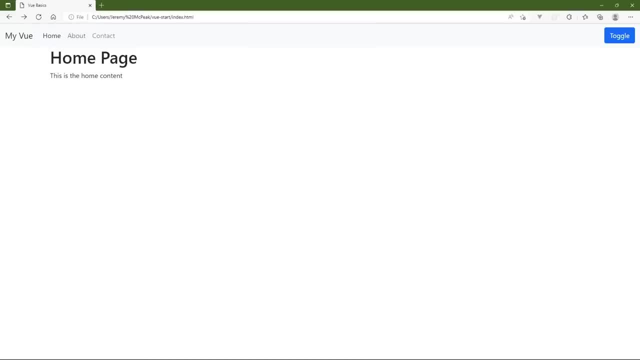 So just for a sanity check, let's go to the browser, refresh. Everything works exactly as it did before. And so, before we move on to the page, we're going to have to do a couple of things. 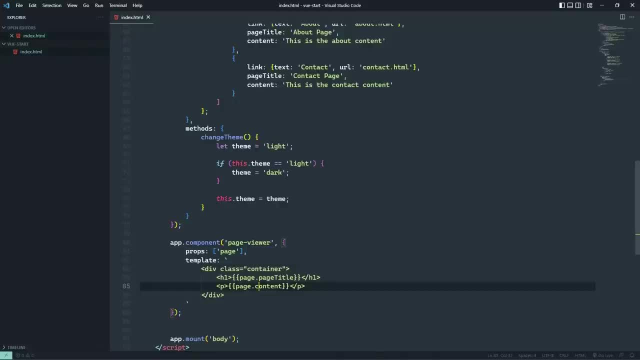 The next lesson, let's just go over the key things about creating components. Because this is important, our applications are going to be full of components. 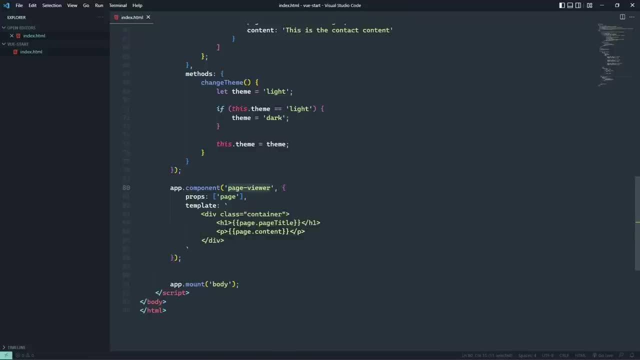 So we create a component, we give it a name, and that component can have options. One option is the template, another option is called props. 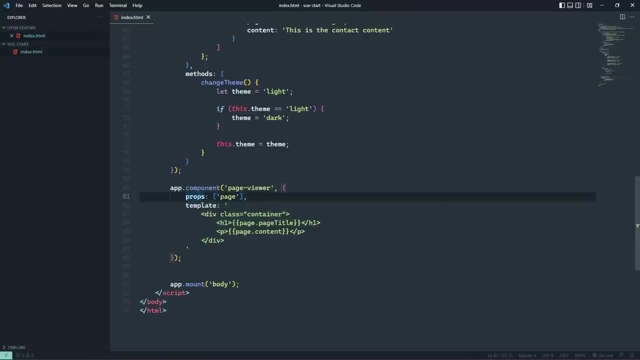 Props are essentially the arguments for this component so that we can pass data to our components. So that they can do whatever they need to do. 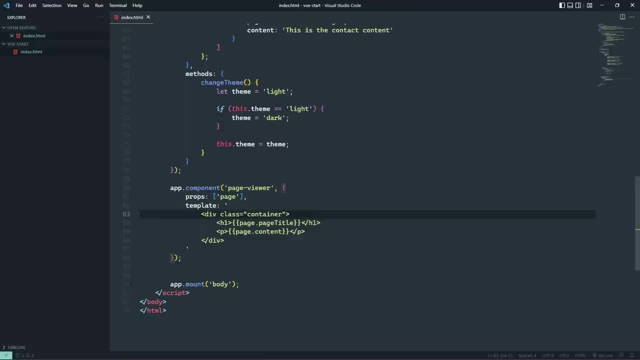 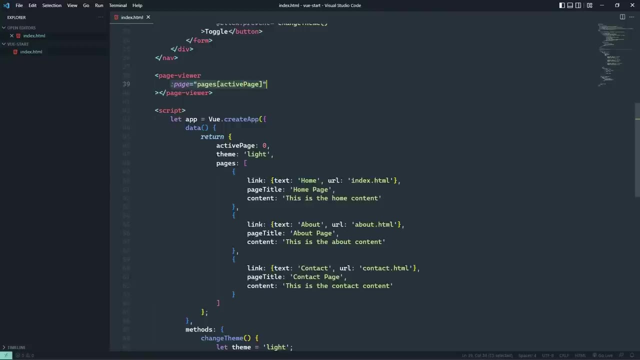 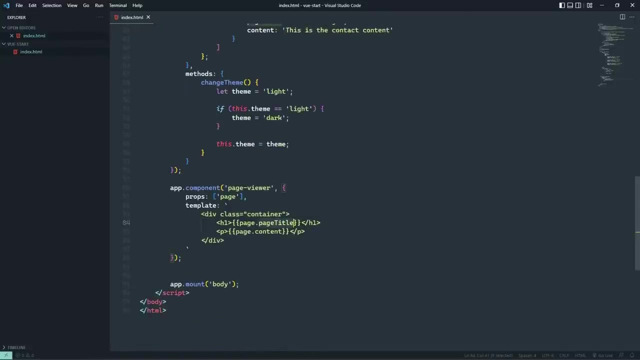 In the case of this page viewer, it is simply outputting data. So we have a prop called page. We pass the active page as the page prop by using vbind so that inside of the components, we can use that as an object to output the page title property and the content property. 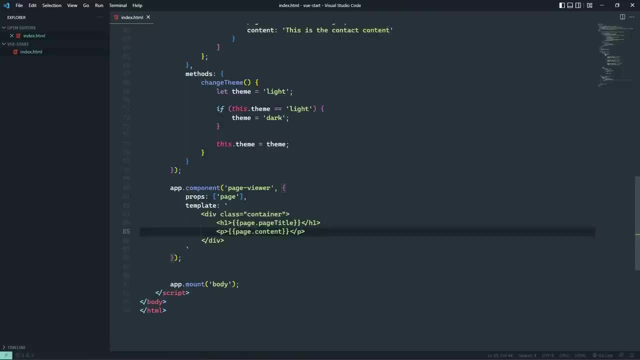 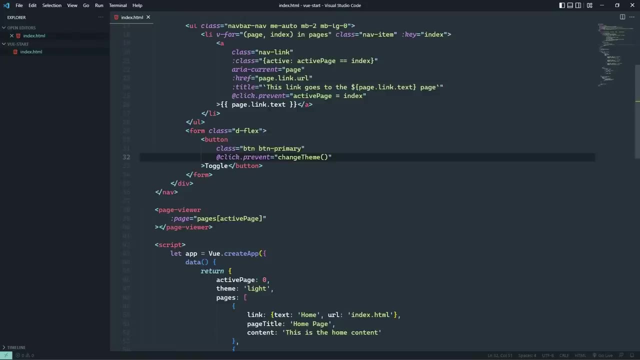 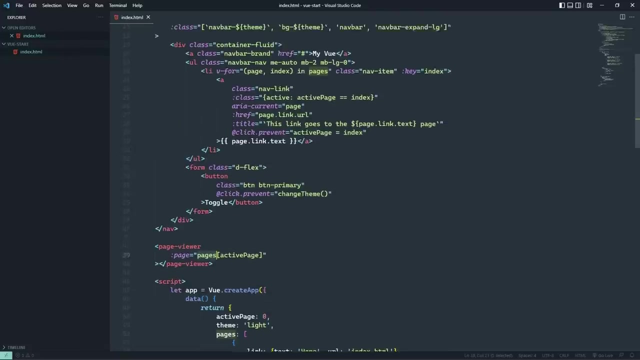 And so in the next lesson, we will create a component for our nav bar. And that component has the functionality for displaying the page information, that is the title and the content, into its own component called page viewer. It has a prop called page, which we pass in a page object so that it can use the appropriate properties to display that information. 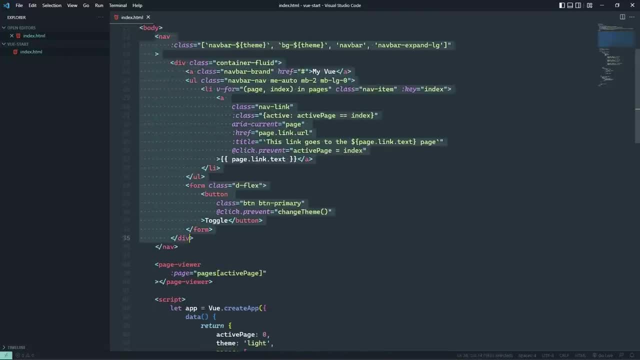 So now we essentially want to do the same thing for our nav. And so let's just get started with the concepts that we talked about in the previous lesson. I'm going to start by cutting out the markup for 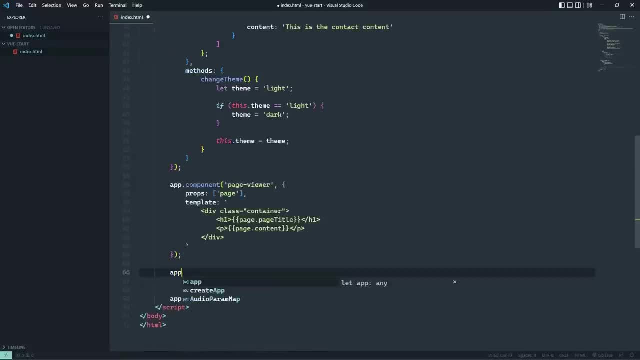 our nav bar so that we can go ahead and define that component and then use that markup as the template. 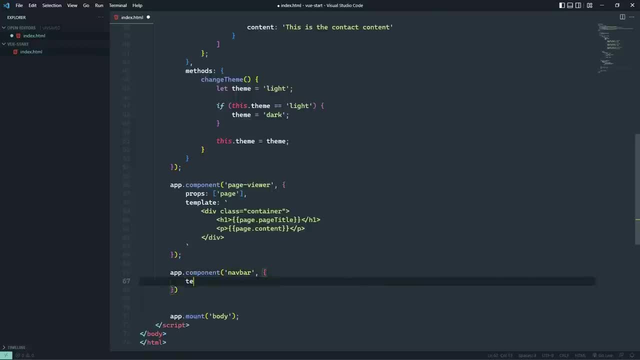 Let's call this simply nav bar. And then the template is going to use backticks in order to delimit the string. 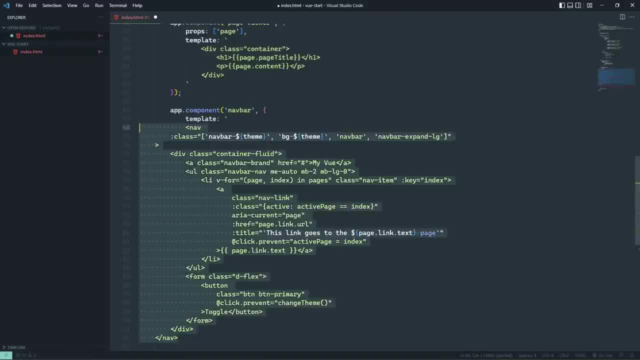 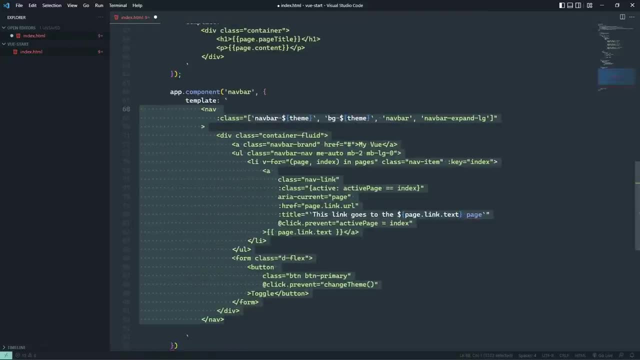 However, we already are using the JavaScript template strings inside of this template. So that means we will need to escape those, which is simple enough to do, but it is a pain. 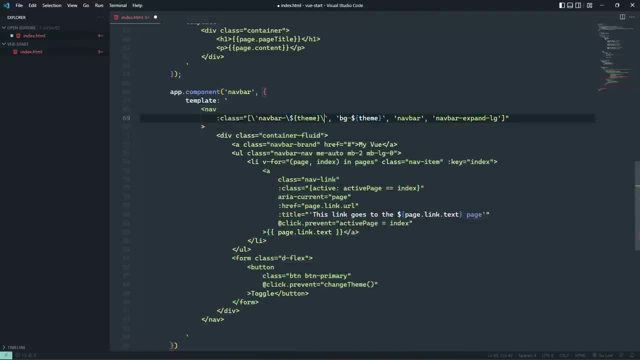 And this is one of the reasons why when you start getting into components, it makes a whole lot of sense to start using build tools and tool chains. Because when you start using JSX, you don't have to do anything like this. 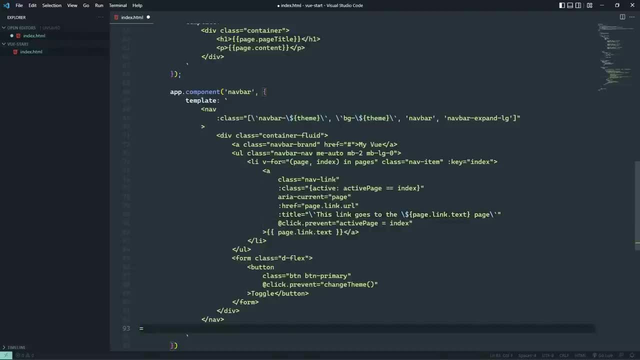 But thankfully, there's not a whole lot of escaping that we need to do here. So there's our template. 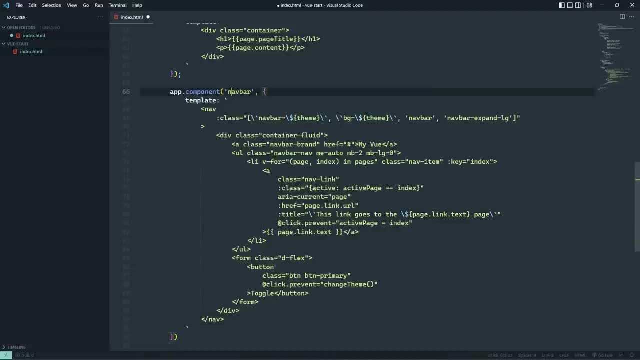 And since we're here, we can go ahead and define the props that this nav bar is going to need, because it needs the pages so that it can generate the, and the A elements for the links. 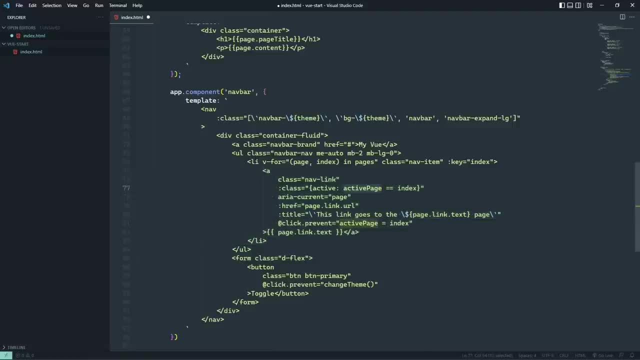 It also needs the active page, so that it can properly apply the active CSS class. So let's define those props. 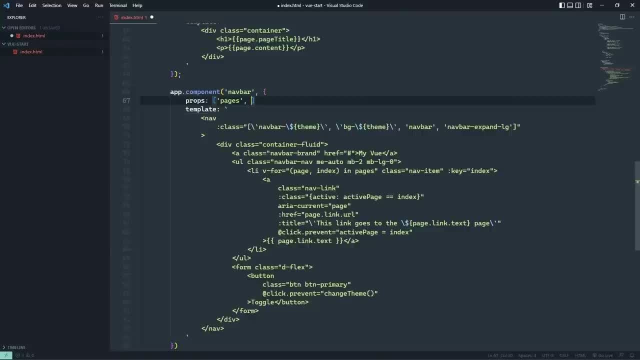 Now technically, we can call these anything that we want. Because remember that props are a lot like the parameters on a function. 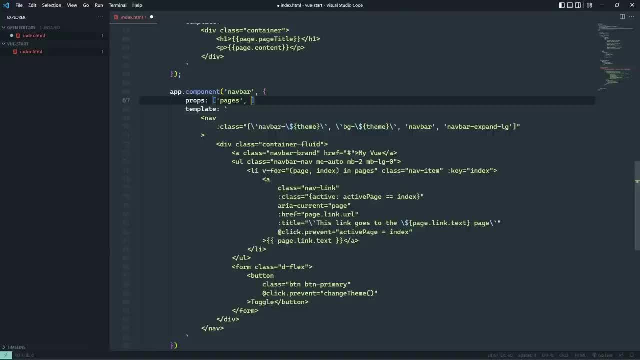 These are variables that we will use inside of our templates. However, if we call them something other than pages and active page, then we will need to make the necessary changes inside of our template, and I don't wanna do that. 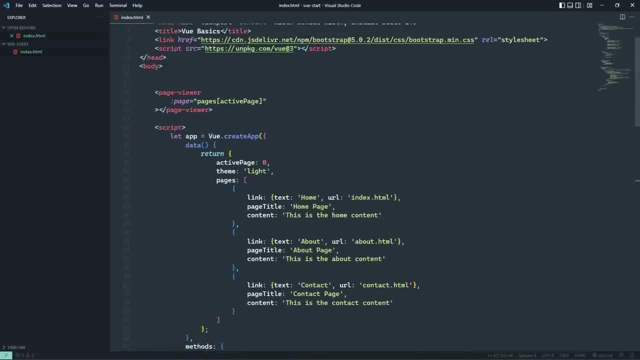 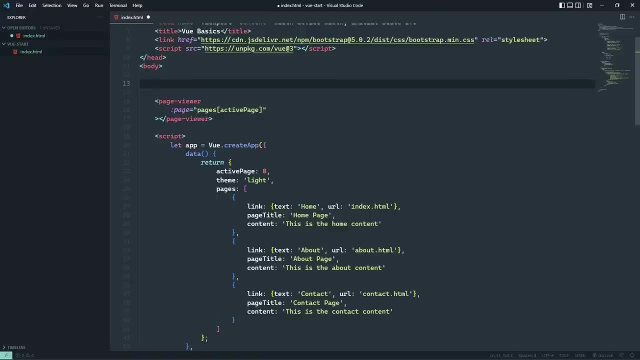 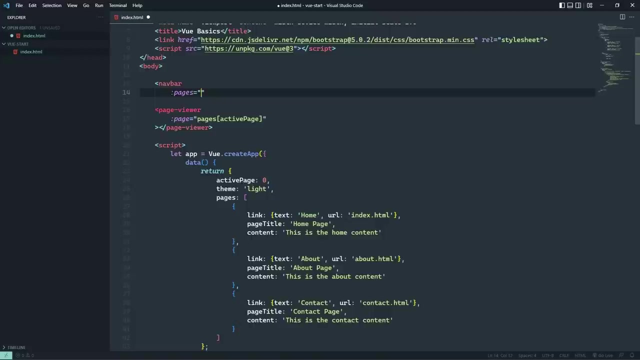 So there we go, we have our nav bar, or at least the beginning of our nav bar. So let's go to the body or to the markup of our application. And let's use our nav bar, and we will go ahead and bind the pages to the applications pages array, as well as the active page. 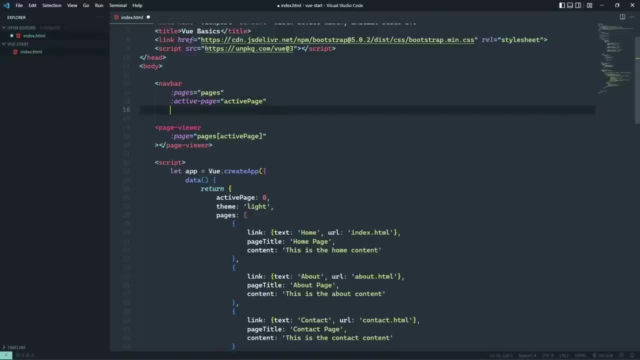 This is very important, because if we don't bind active page, then we're going to run into some issues. 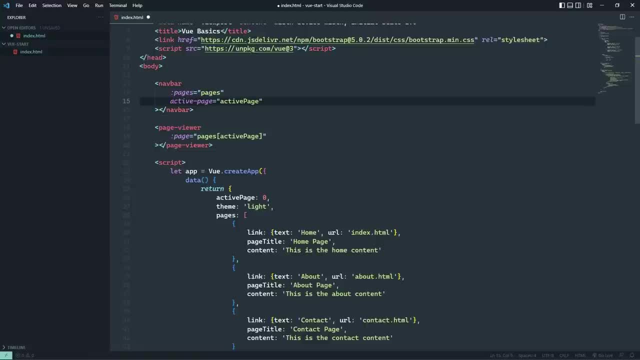 First of all, if we don't, then what we are passing is a string literal of active page, which of course is not going to work at all. 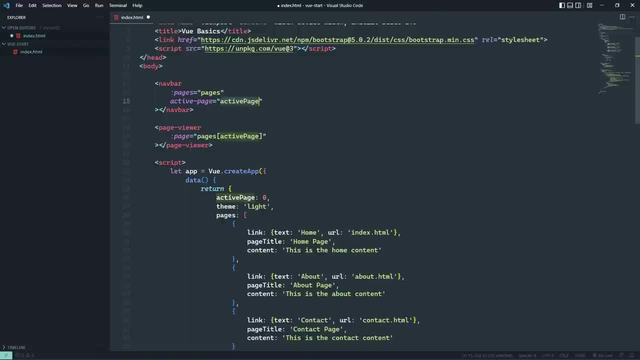 But let's just imagine that by not binding active page, we are still using that numeric value, which is initialized as 0. 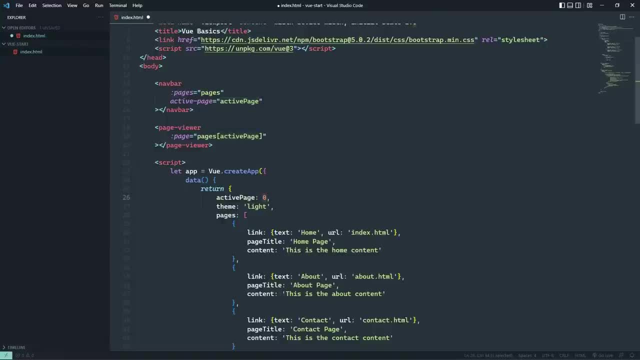 So, one thing to remember is, that data flows from parent to child. 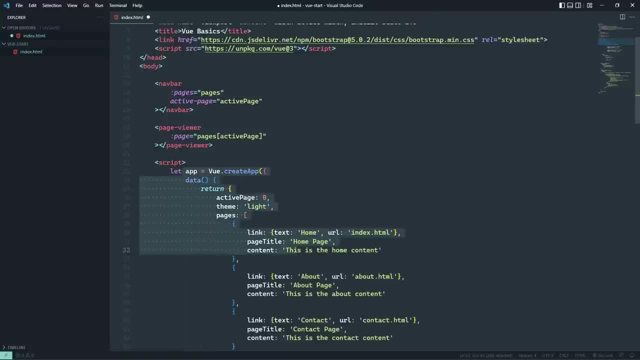 So in this particular case, the app is the parent, the child is the nav bar component. So the data active page, which initializes as 0, is passed down to nav bar. 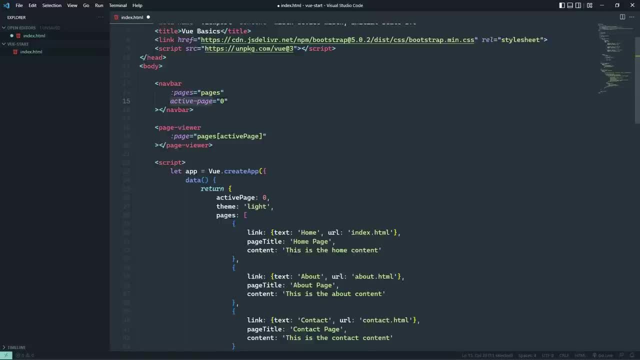 So the next time that active page is updated, that change is not going to be passed down to nav bar, because it is not bound. 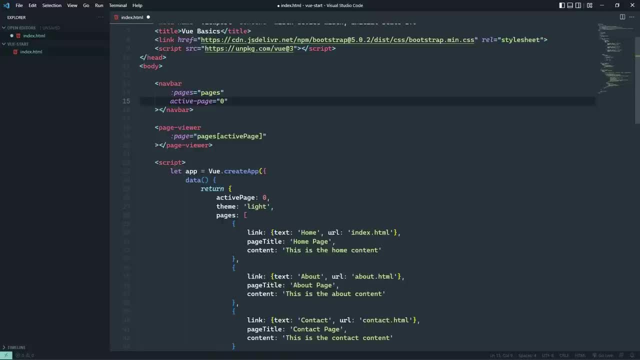 So if active page becomes 1, well, we essentially passed the value of 0 to it, and it will stay as 0. 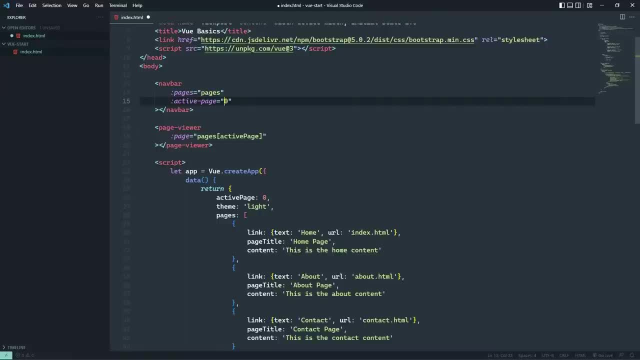 So if you want the child components to update based upon the data that it has been provided, then you need to bind the data to those props. So we want active page bound to the app's active page. 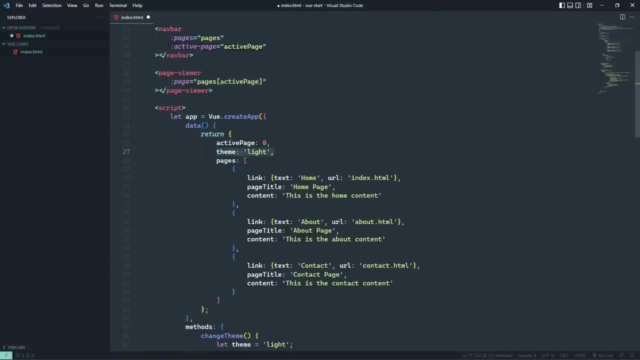 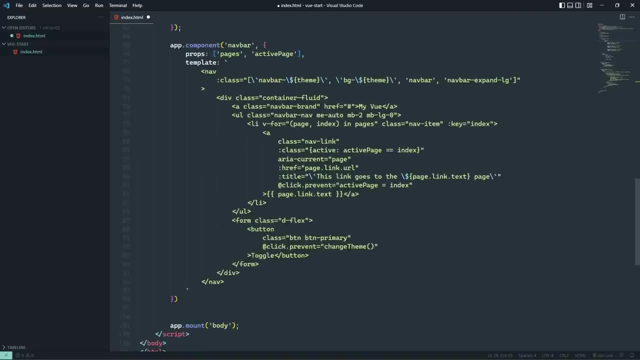 Now, there's a couple of other things that we need to do. The theme is specific for the nav bar. So we can take that out of the application. And we can define that as part of the data for the nav bar, which this is just like the data option in the app. 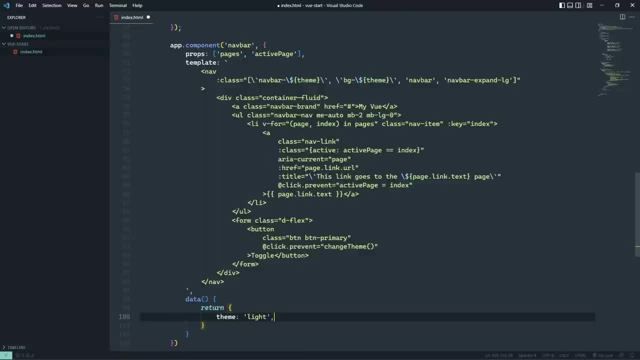 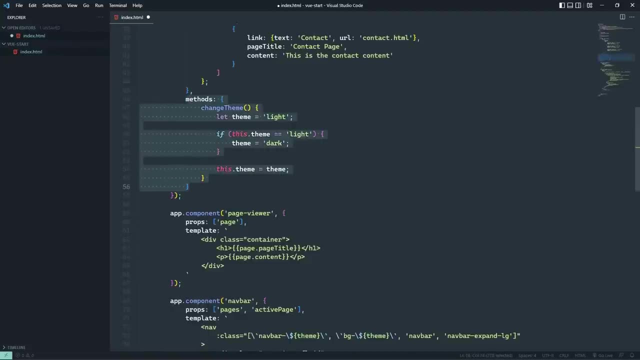 It's a function that returns an object, so there we will define theme. The same is true for our methods, because change theme is really only specific for the nav bar. 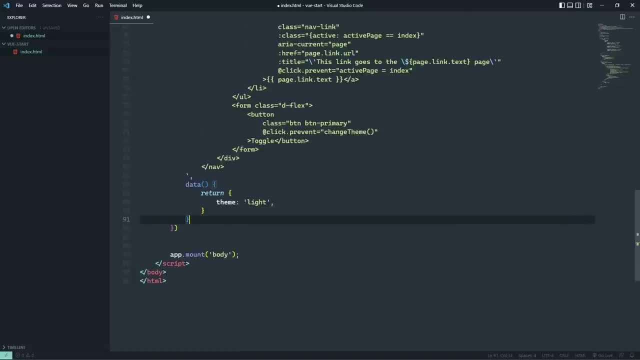 So let's cut that out completely, and let's add that methods option to the app. Okay. To the component. 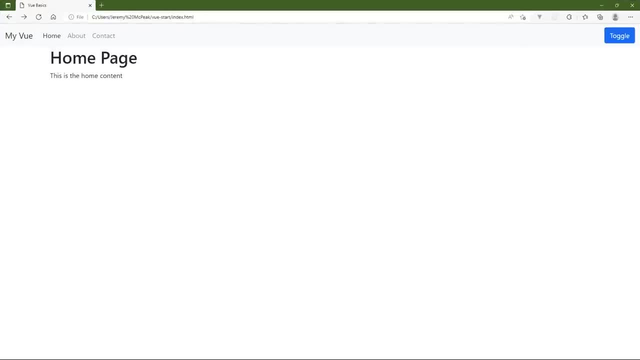 So with that done, let's go to the browser, let's refresh the page. Now, we're going to see that toggle works, that's perfectly fine. And I'm going to make it dark because it makes it easier to see what's going on here. 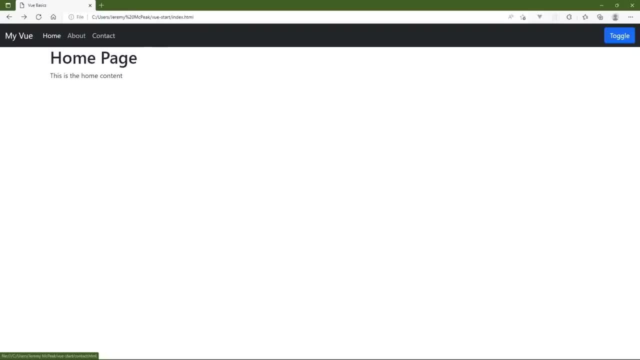 So I'm gonna click on About, nothing happens. Gonna click on Contact, nothing happens. Gonna click on Home, and of course, Home is already loaded, but nothing really happens. 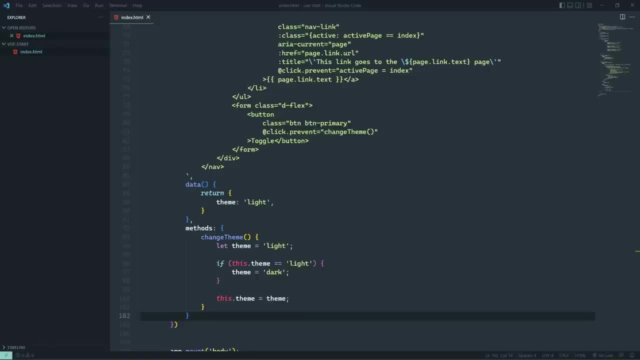 And the reason is very simple, and it's because we aren't updating active page. Now, 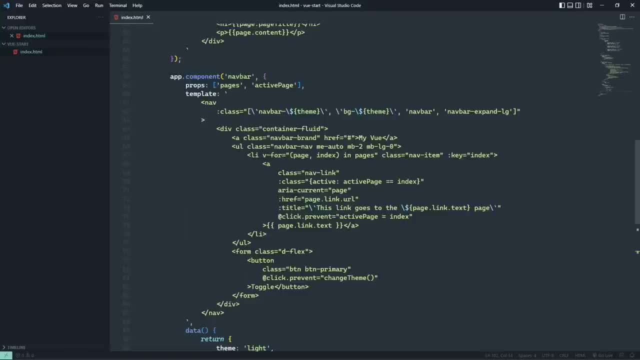 if we look at the template for navbar, whenever we click on one of these links, there it is, active page equals index, and active page is being supplied as a prop. But here's the thing, props are read only, so we can't change their value inside of a component. 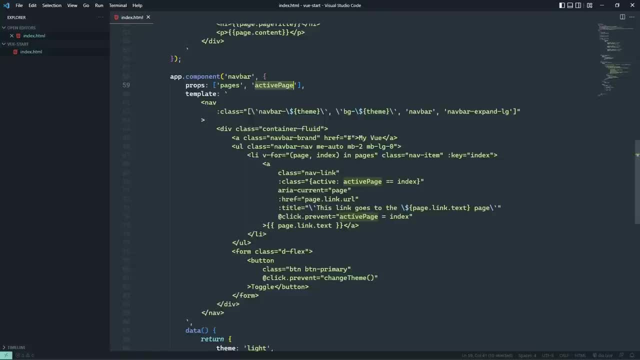 Now that makes perfect sense when you start thinking about how data flows. 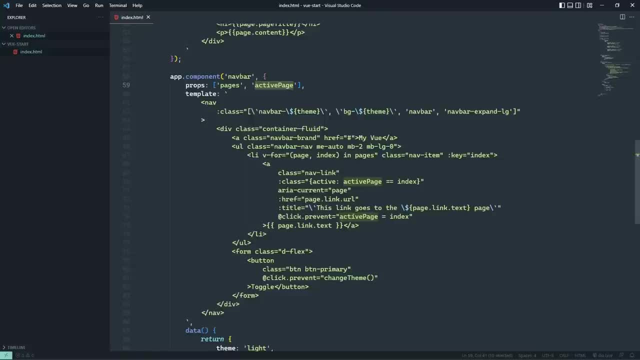 As I mentioned, it flows from parent to child, so if we were to change the value the value of a prop inside of a child, the parent would not know that the value changed because data flows from parent to child. 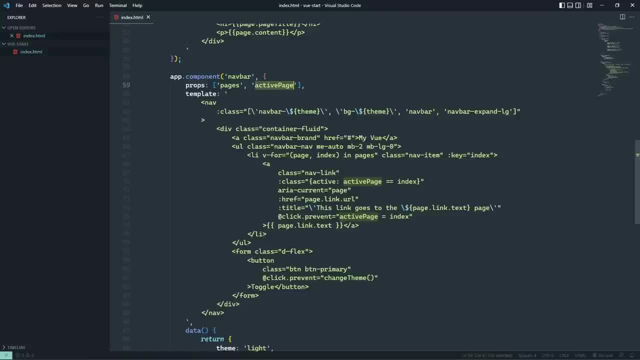 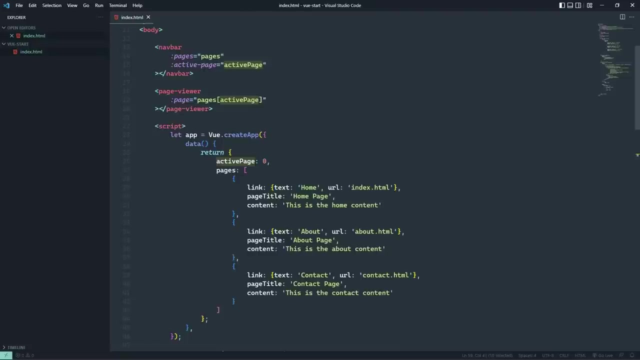 So then the question becomes, how do we do the reverse? How can a child notify a parent that something changes? Well, it's very simple, we use an event. Or rather we use what is essentially an event. Like for example, we've talked about the click event before to where we say at click, and then we have the code that's going to execute. 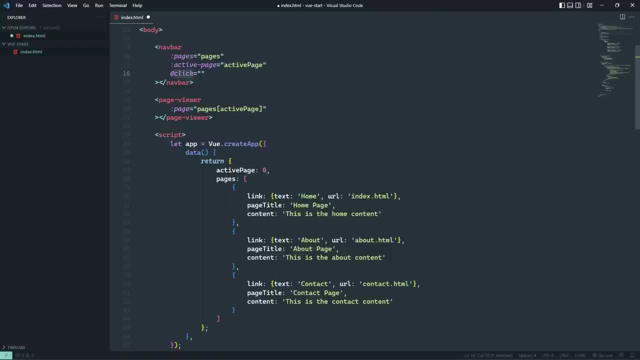 Well, in this particular case, click is essentially a prop. It's a special prop because it is an event. But we can essentially do the same thing so that we have a prop that will execute. And we can call this simply nav link click. So that we would have a function that would accept the index. So that we would change the active page. Now, remember that since this is the navbar component, we are now inside of the app. We aren't inside of the navbar. So this code here is specific for the application. 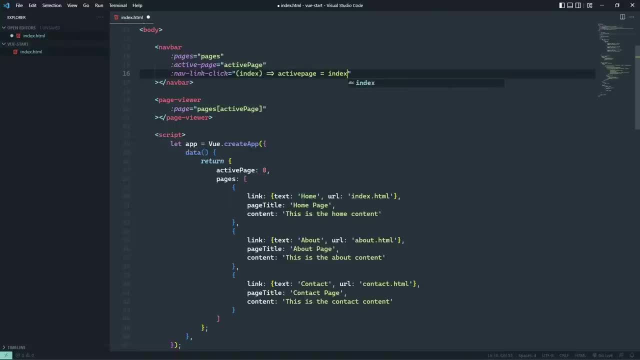 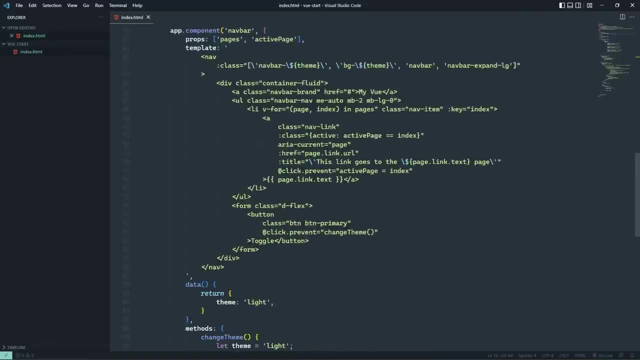 But all we need to do is set the active page equal to index. And we need to make that active uppercase P page. So that's inside of our component, all we need to do is change where we click on the index. 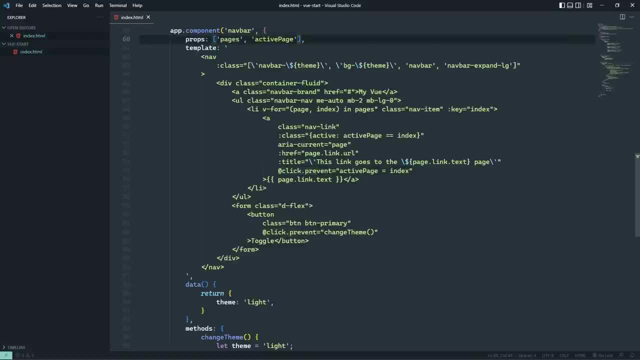 Well, we need to do two things. First of all, we need to say that we now have a prop called nav link click. And that this is a function that is going to execute and we will pass in the index. So it works a lot like an event. 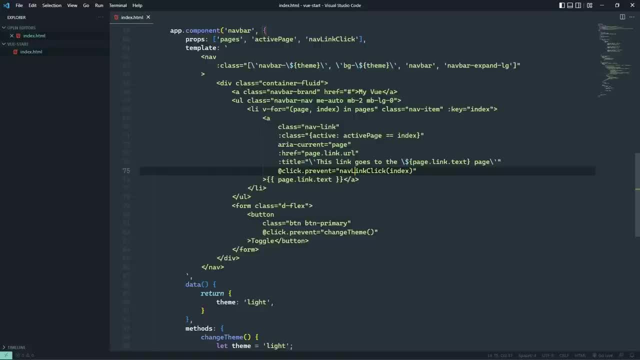 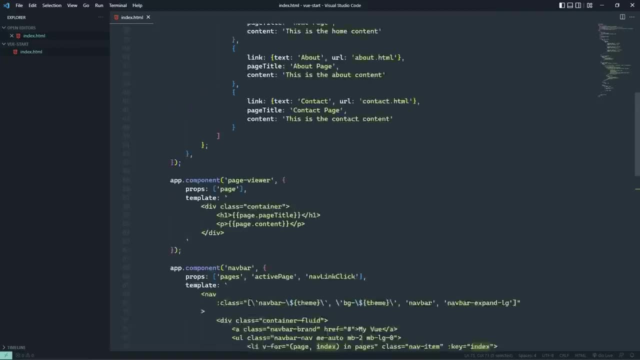 So the parent is supplying the function to nav link click that the child is going to execute, it's going to pass the index back so that inside of the application, we can update active page to that index value. 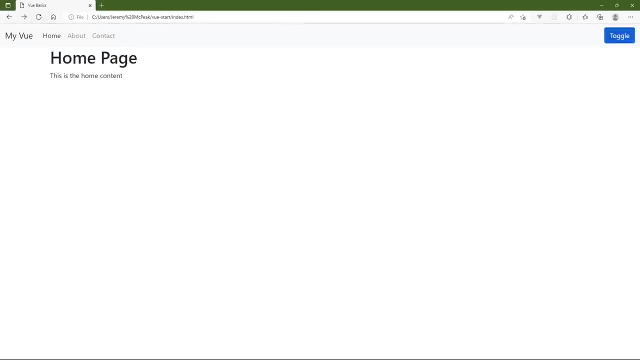 So with that done, we can go back to the browser, we can refresh. Let's toggle that to black so that we can see. 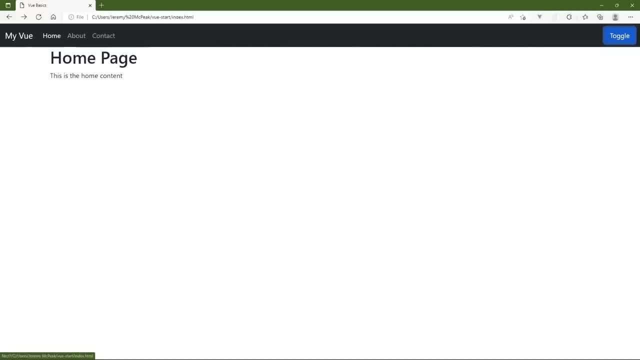 And we're going to see that this works exactly as it should. So home, of course, is the default, we see that. We also see that home is active, whenever we click on about, home is no longer active, about is active. 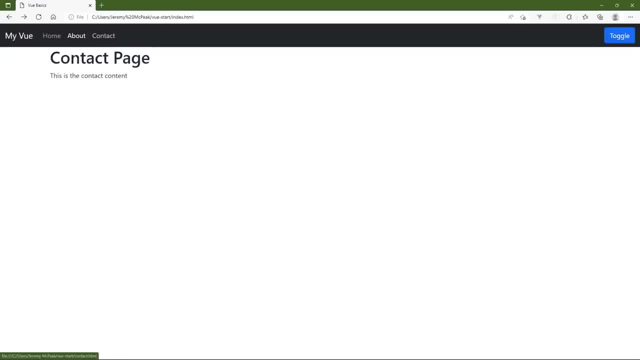 And of course, we see the content for about whenever we click on contact. I mean, I hate to do a play by play here, but 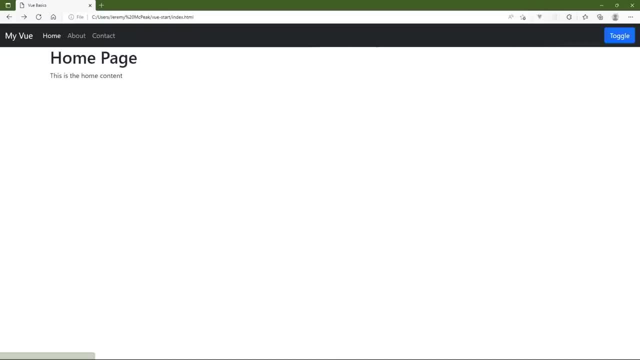 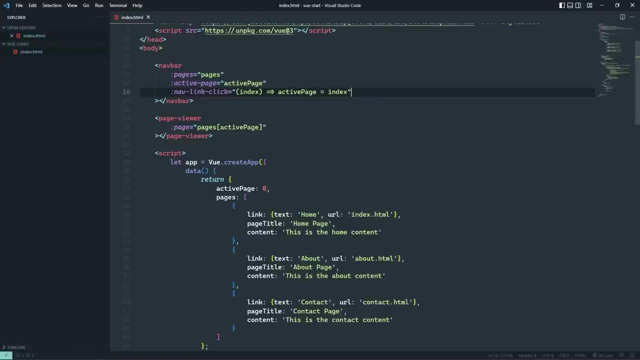 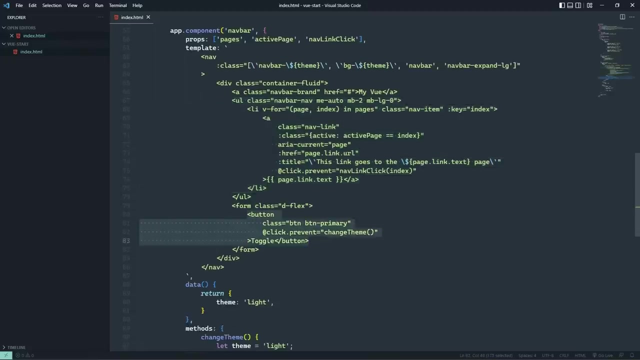 this is the exact functionality that we would expect. Except now, we have our application broken up into two different components that are responsible for their own functionality. The page viewer is responsible for displaying the page information. The navbar is responsible for generating the navbar, keeping track of the theme, as well as notifying the application when the user clicks on a link. 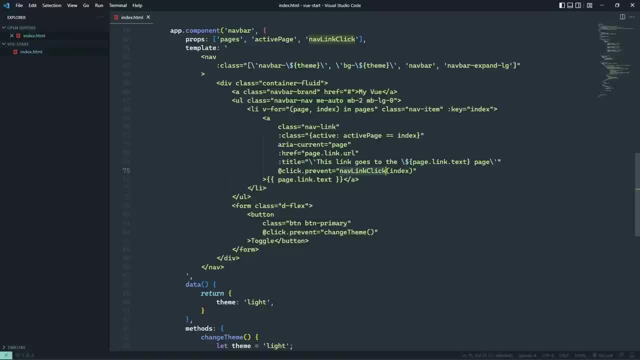 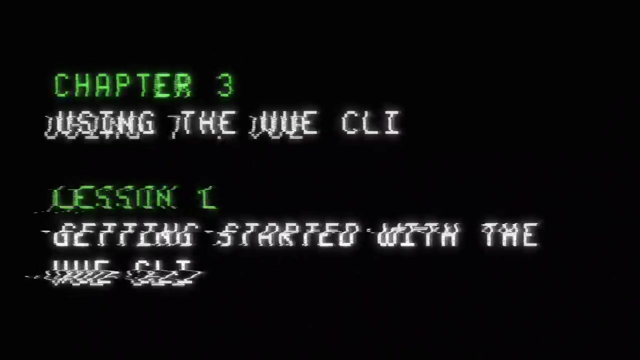 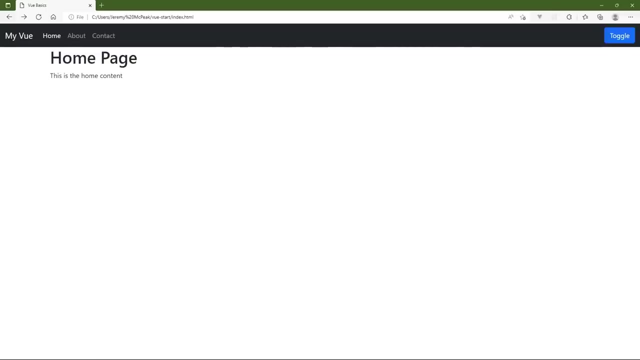 And so in the next lesson, we are going to get started looking at the Vue CLI, which is the tool chain that makes it easier to build Vue applications and Vue components. Since the beginning of this course, we've used nothing but the Vue library to go over the fundamentals. And I wanted to do that because I want you to know that you can build Vue applications using just the library. You don't need tool chains, you don't need build tools, you don't need anything except the Vue library, a text editor, and of course, a browser. However, we do have tool chains and build tools specifically because they make our lives as developers easier. And while they are extremely useful for building large applications, you can use these tool chains for building any size of application. 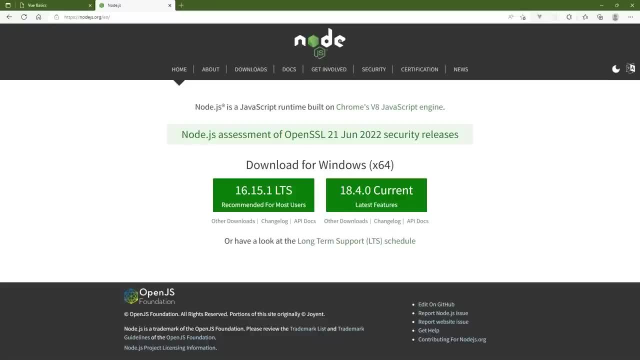 I always reach out to you for that. You can reach for the build tools just because it makes our lives easier. 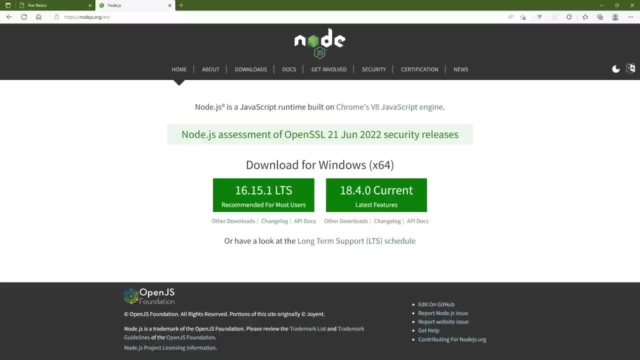 So what we are going to do is install what's called the Vue CLI. CLI stands for Command Line Interface, and it gives us all of the tools necessary for building our Vue applications. 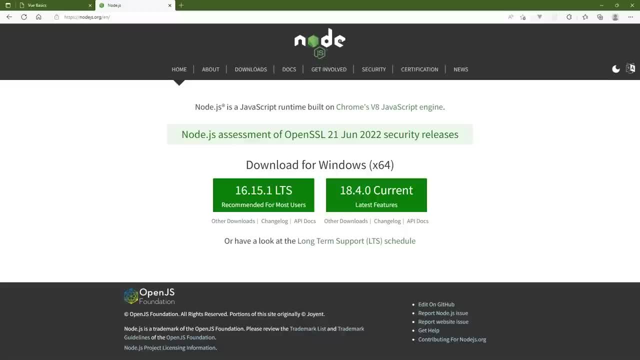 But we also get to use features like JSX, which is JavaScript and XML, as well as newer features to JavaScript. 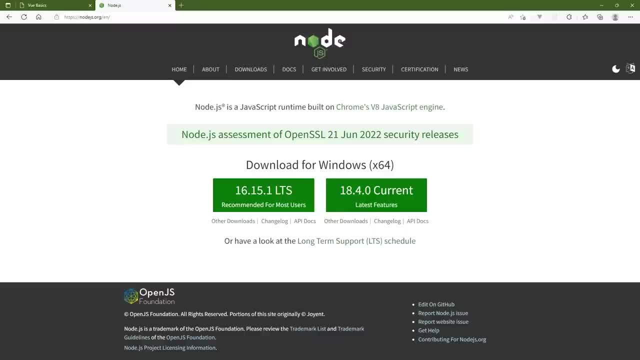 So things that aren't natively supported by the browser really doesn't matter because the build tools are going to be going to handle that for us and translate it into things that the browser understands. 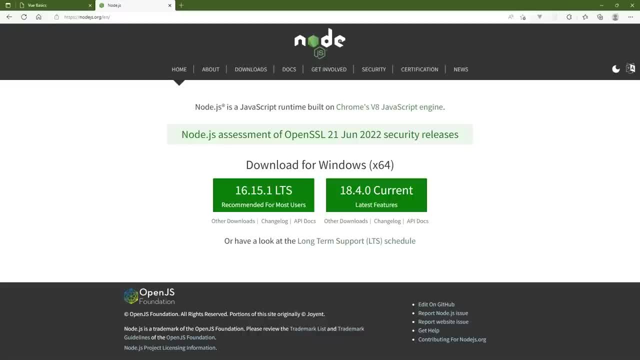 But in order to install the Vue CLI, you need Node.js. And if you don't have this, then now's the perfect time to do it because it's not used just for Vue. It's not used just for React or anything. This is how we manage our dependencies. Node, and more specifically, Node Package Manager is just part of modern web development. So if you don't have it, now's the time for you to go ahead and to get it. 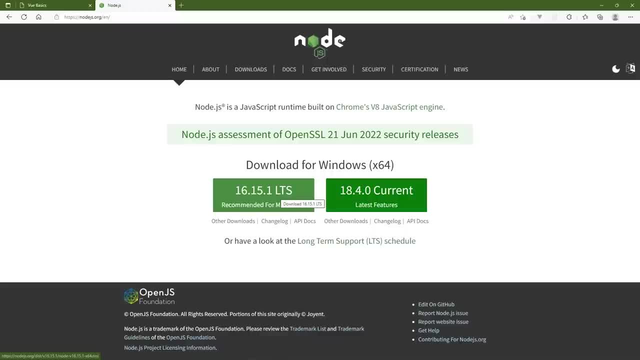 Just go to nodejs.org, and download the LTS version. The version number doesn't necessarily mean anything from our perspective. Now, if we were going to build Node applications, yeah, the version number matters, but that's not the case. 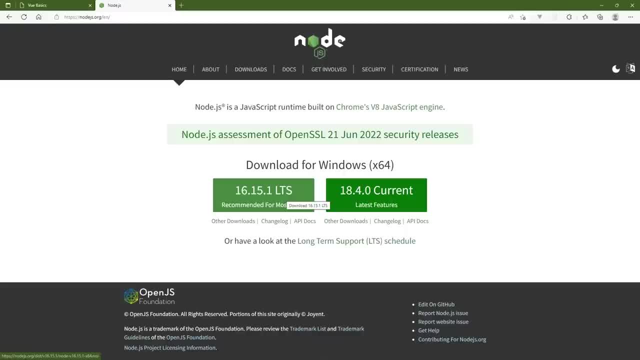 Just look for LTS, that's Long Term Support, and download and install it. It is a straightforward installation. Just take the defaults. 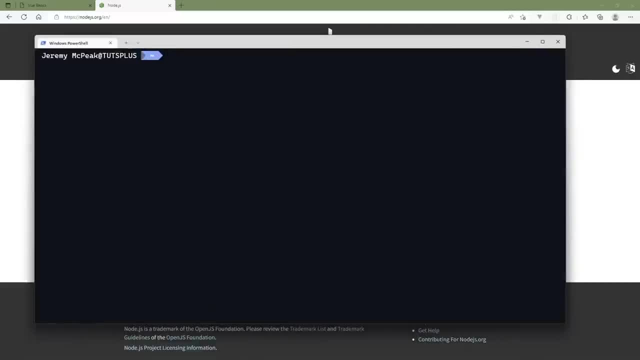 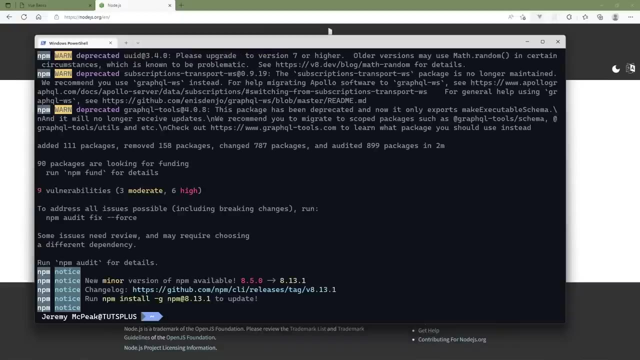 And once that's done, you will want to go to the command line, because NPM is a command command line tool, and we want to install the view CLI. So it's at view then slash CLI, and we want to install this globally. Now, the reason why we want to install this globally is so that we can use the view command regardless of what directory we are in. And we will use the view command to create our first project. 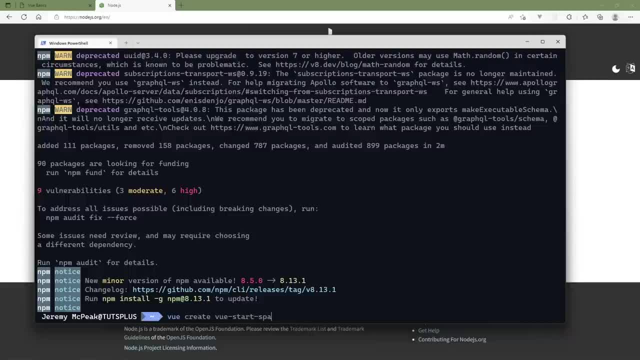 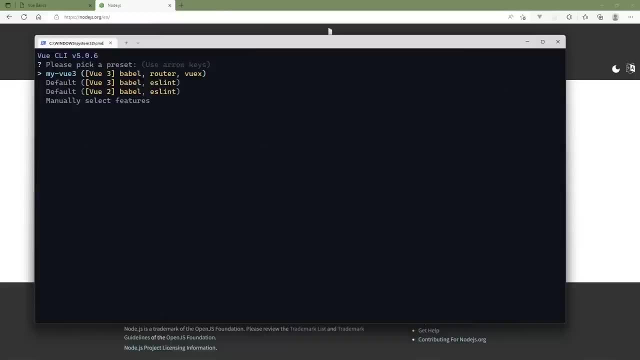 So let's call this view start SPA for single page application. We are essentially going to recreate the page that we've been building over the past few lessons, but we're going to use the view CLI. 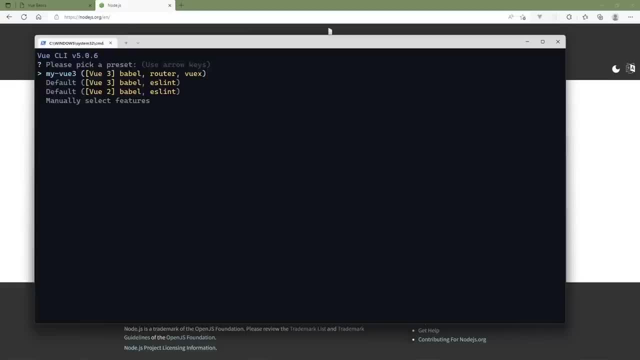 And this is going to give us several options that we will need to go through. Now, I have some presets already done because as I said, I use view. So let's go down to manually select features. And we want to select Babel because that is a compiler. That allows us to use new JavaScript features in browsers that don't support it. 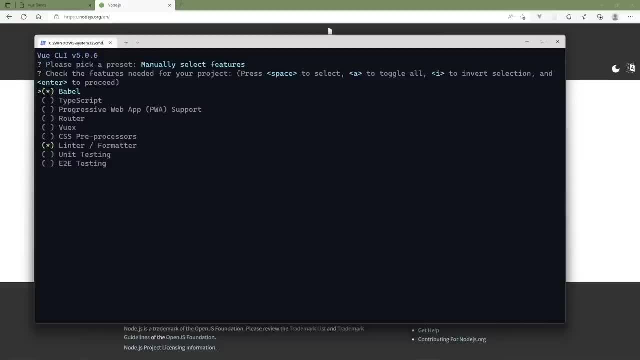 Babel will translate that into JavaScript that the browser does understand. So we do want Babel. 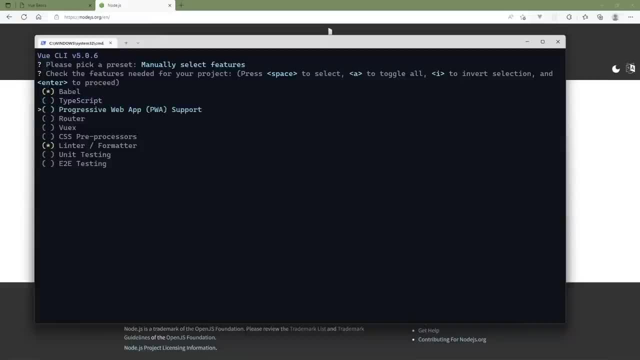 And if we wanted to use TypeScript, we could do that as well. We aren't, we're going to use just normal JavaScript. 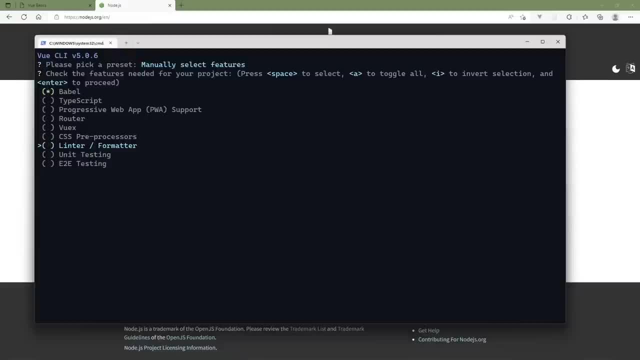 Now, I'm going to uncheck the linter slash format just because that adds a little bit of extra stuff and I want things to be nice, neat, and clean. 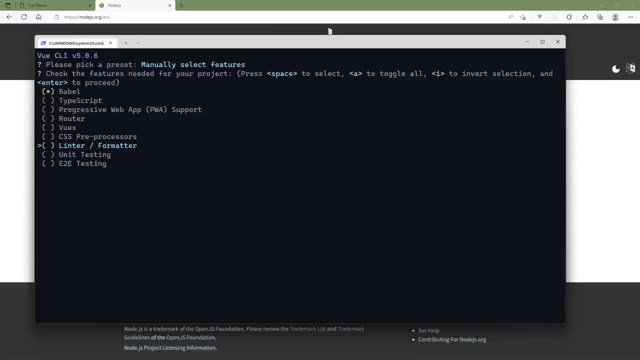 Now, of course, in a real project, I would probably check the linter just because that's a good tool to use. But it does also take some processing time. 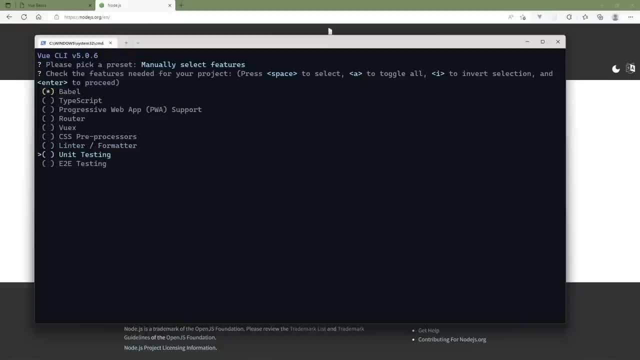 And since time is of the essence, we're going to leave that alone. So Babel is really the only thing that I want to use right now. 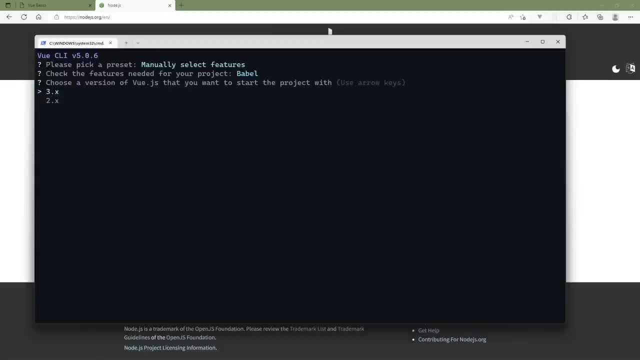 So let's hit Enter to go on. We get to choose the version of Vue.js. 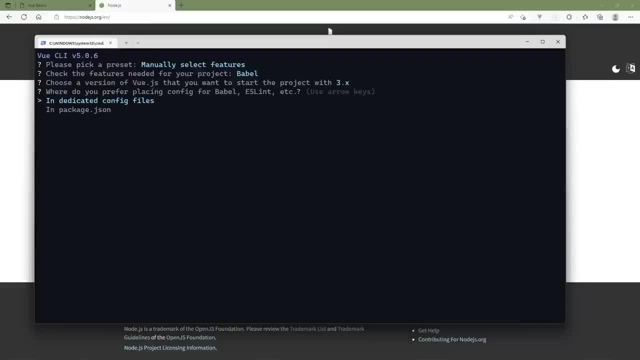 The latest is 3.x. And then we get to choose how we want our config to be laid out. Do we want them in dedicated config files or inside of the package.json? 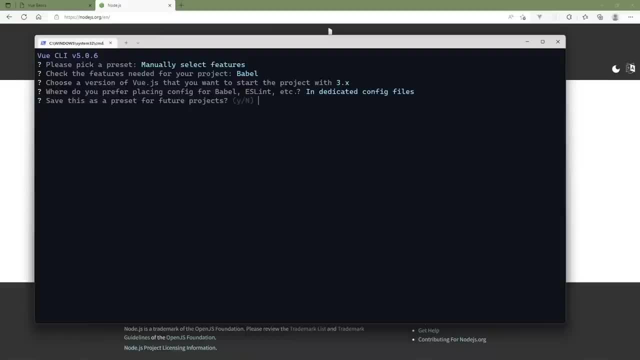 We want dedicated config, well, I want dedicated config files. And we can save this as a preset, I'm not. 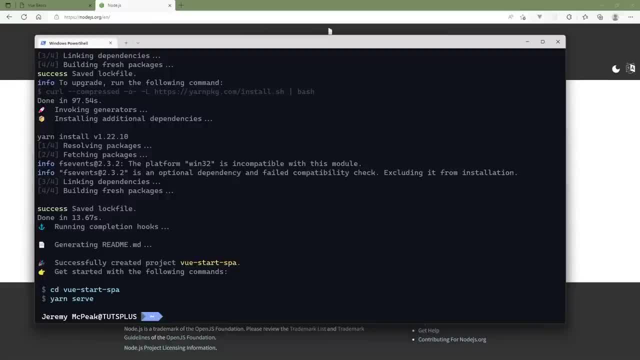 And so this is going to build our project. And when the project is ready, we want to cd into that new folder. 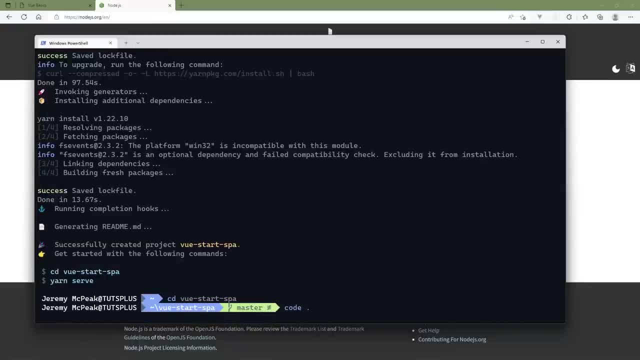 And then we'll fire up our code editor so that we can take a look at the project. Because this is going to be very different from the single HTML file that we've been working with thus far. 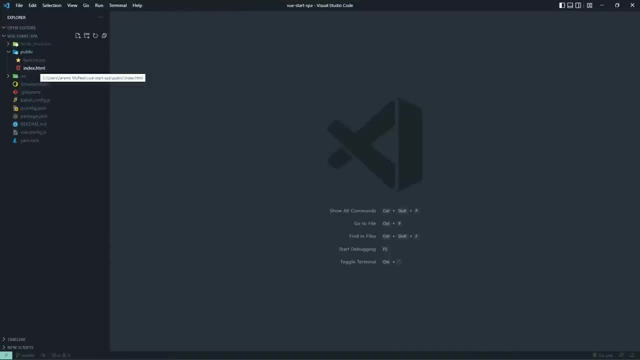 The first is going to be this public folder. Now this is, well, it's the public folder. This is what the end user would want. 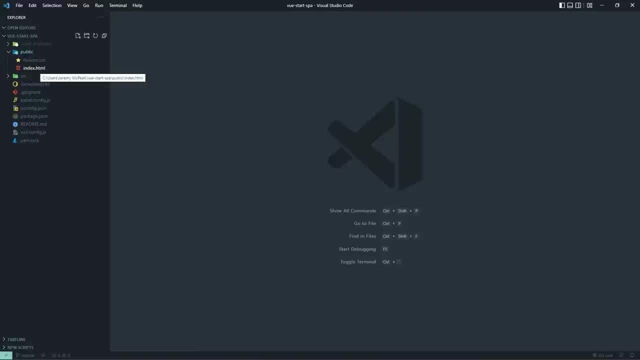 The end user would see if they go to our application. 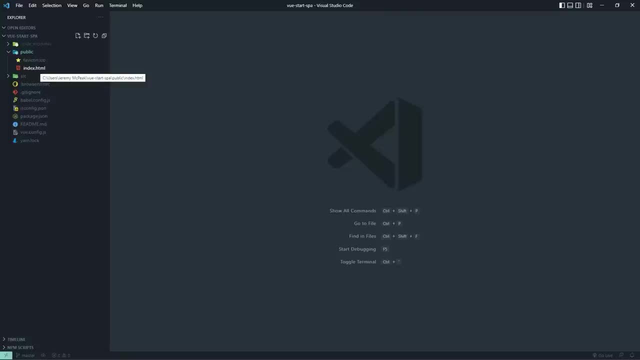 This is also a place where we can put our static files, like images and things like that. 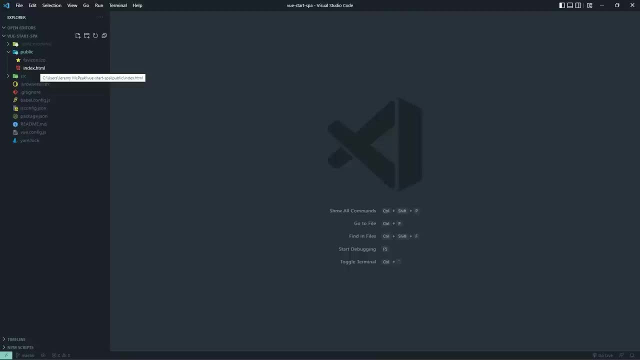 However, there are alternatives to that approach, which that is something we will talk about at a later time. 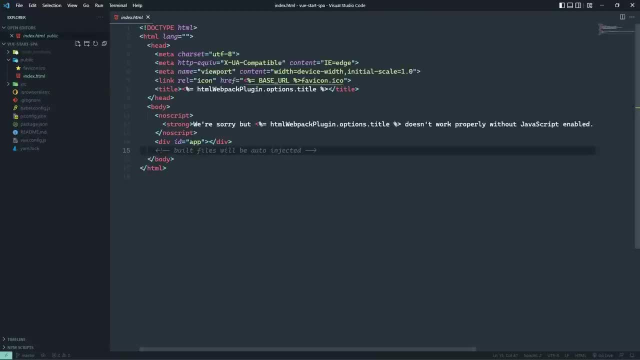 Now you'll see that there's two files. There's the favicon and there's also index.html. And there's not a whole lot here inside of the HTML file. But do notice that there is this div with an ID of app. This is where our application is. Okay. And this is where our application is going to be mounted. 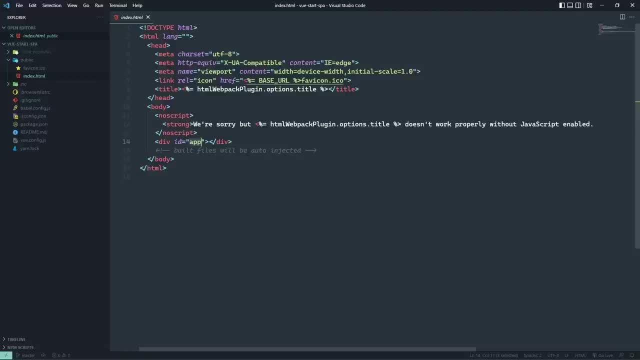 Now we can change that because we have complete and total control over our application. 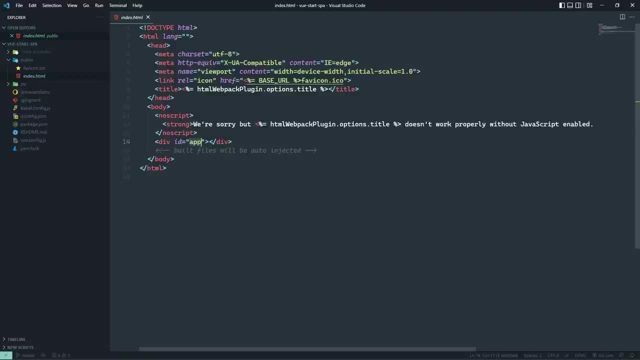 But this is convention, we'll just stick with this. And notice that there's also this comment that says that built files will be automatically injected. 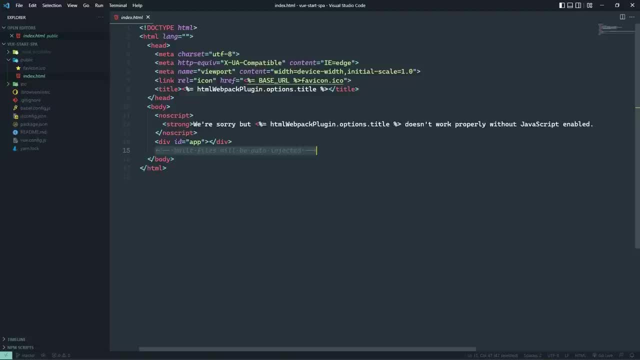 Now for the vast majority of time in this course, we are going to be using the development mode. 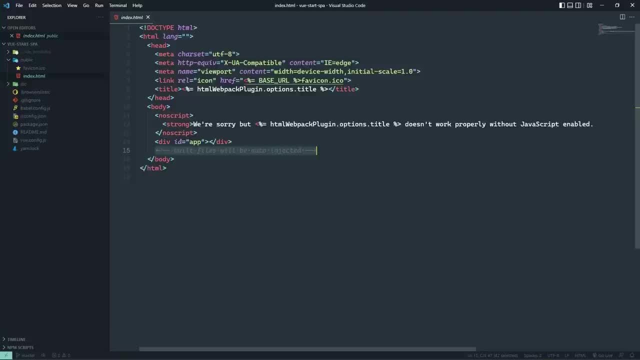 Which is essentially going to build our application as we develop it. And any change that we make is going to, or to automatically be reflected inside of the browser. 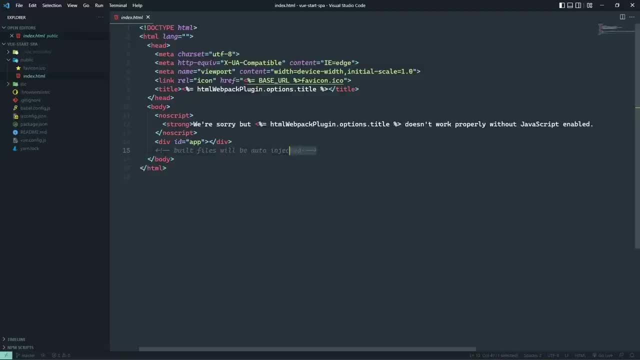 So those files that are being built behind the scenes are going to be injected here. So we don't have to worry about any of that, it's just done automatically for us. 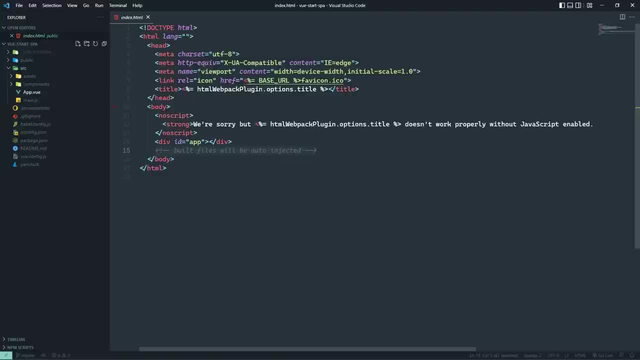 So that's the public folder. But then there's the source folder, and this is the folder that our source code lives. 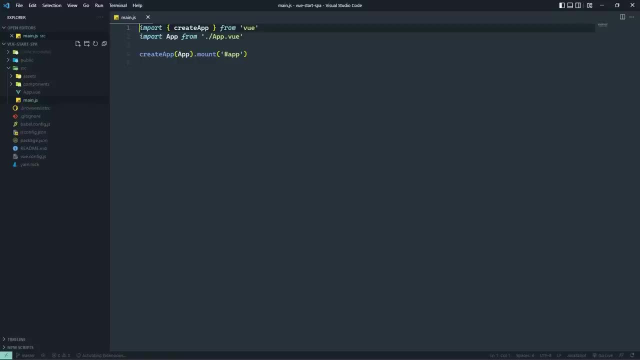 The entry point of our application is this main.js. You're going to see that the create app method is being imported. 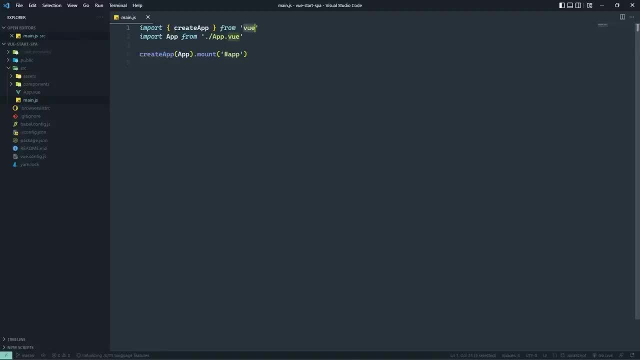 This is being imported into this file from the view library. It's also importing this thing from a file called app.view. This is a component, which we will look at here in a moment. But notice here that the application is being created. The app component is being used as the application. And it is being mounted in the element that has an ID of app. So let's take a look at this app.view. And this is going to look very different than what we are used to. However, after I explain these things, then you are going to recognize, okay, that's what it is. 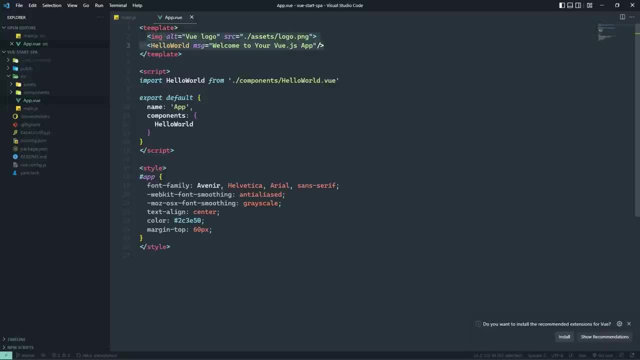 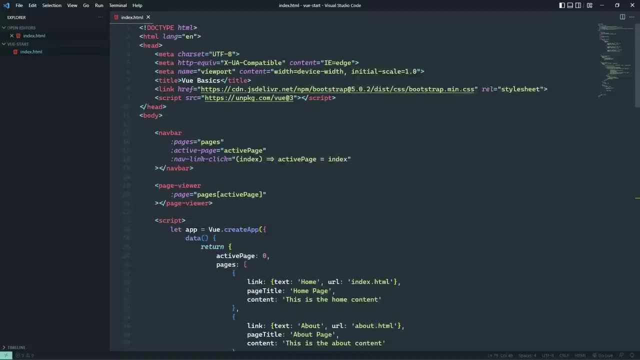 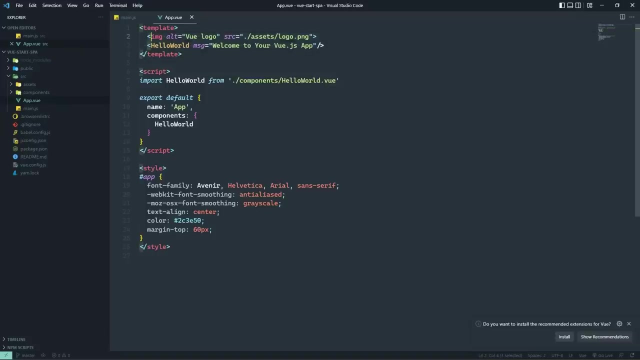 So here we have the template. If we take a look at the file that we've been working with, index.html, I've referred to the markup that was inside of our application as the template. That is exactly what we have here in this new application. So this template is the markup. You'll see that there is this image element that's being used. You'll also see that there is this hello world, which is not an HTML element. It is, however, being imported from another file that has a view extension. This is another component. 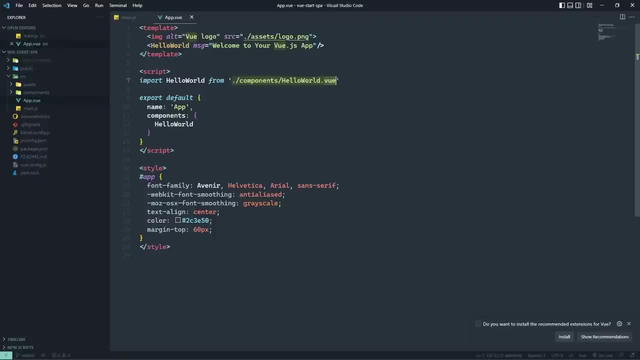 And then there's a few other things such as an object that is being exported and then there's some CSS here. 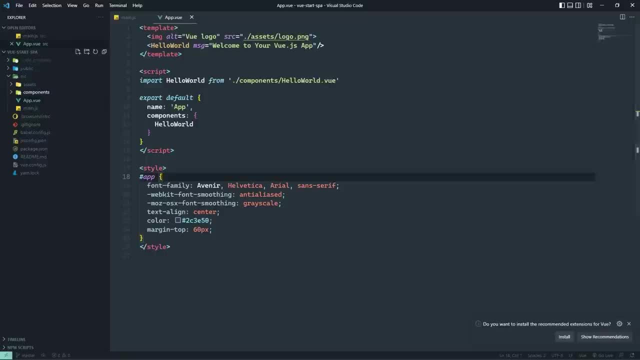 Don't worry about any of this, we're going to go over all of these things. But if we take a look at the hello world, we're going to see here that we mentioned, this associate tag has a lot of states here. But if we take a look at the hello world, we're going to see that we're going to see a lot of department and we're going to see an application that is being dzisiaj. Of course, there are some other components that have been implemented. we're going to see something that looks a lot more familiar. 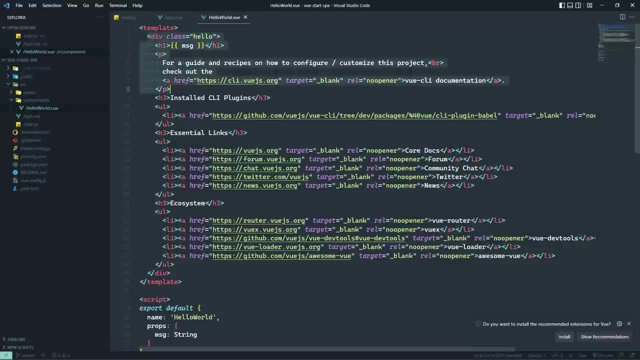 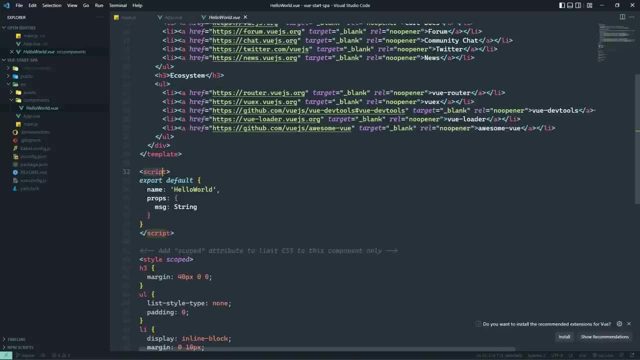 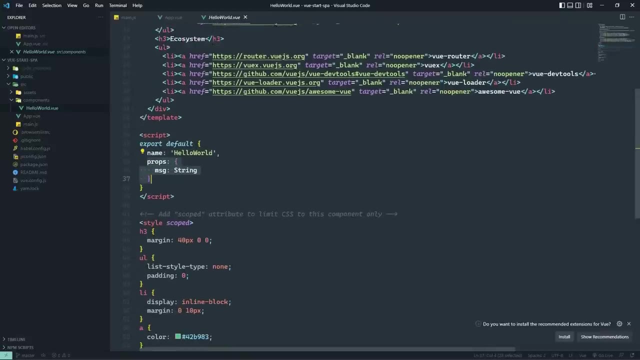 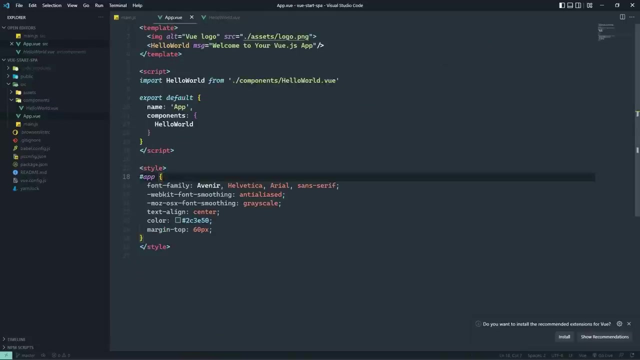 So if we look at the templates, we see more HTML elements than anything else. And if we scroll on down, we're going to see the JavaScript for this component. It has an object that has the props option. And then there's, of course, some more CSS. So this object here that we see that's being exported, that is the options object that we have been using. So everything that we have talked about, all of the fundamentals are still here. It's just in slightly different places. And because they are in different places, it makes it a whole lot easier to develop and maintain these applications. 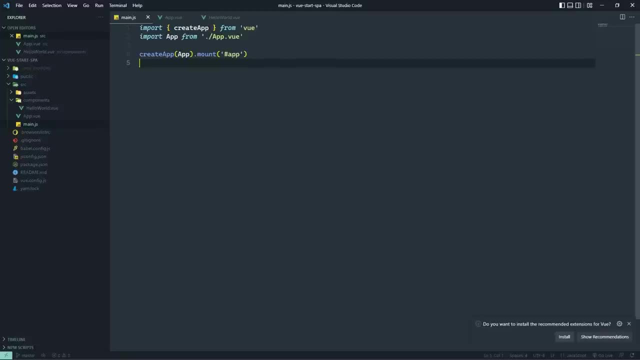 So in the next lesson, we are going to start translating our existing single page application, which uses just the view library, into another application that uses the tool chain and build tools. 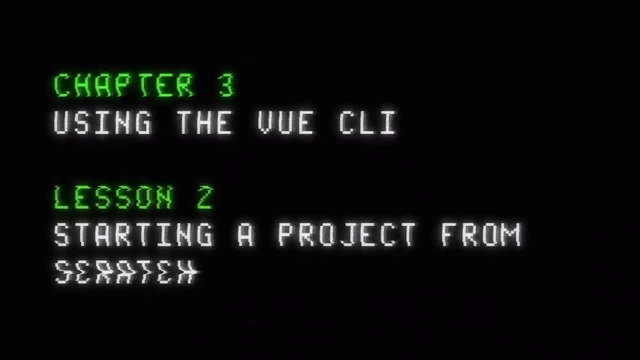 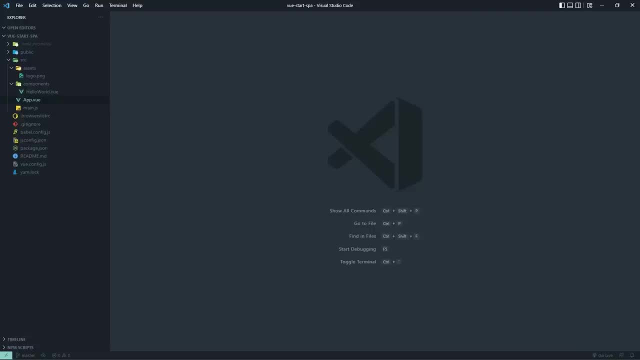 When I create a new project, the first thing I like to do is delete. Well, not necessarily delete the whole thing, but just about everything inside of the source folder. Because I like to start from scratch. That way, I know that my applications have only the things that they need. And plus, it's good practice because programming is a skill. And just like any skill, it's good to practice. 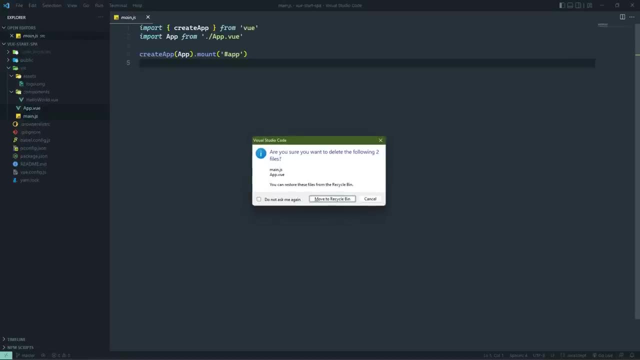 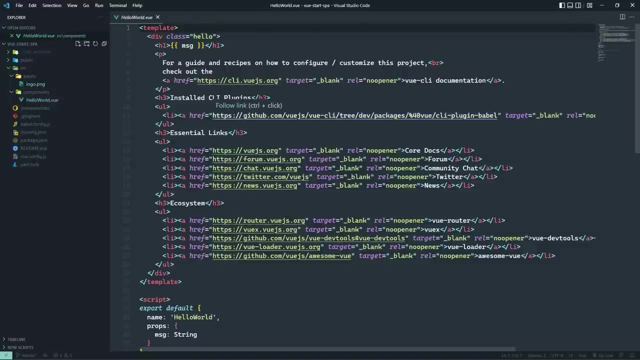 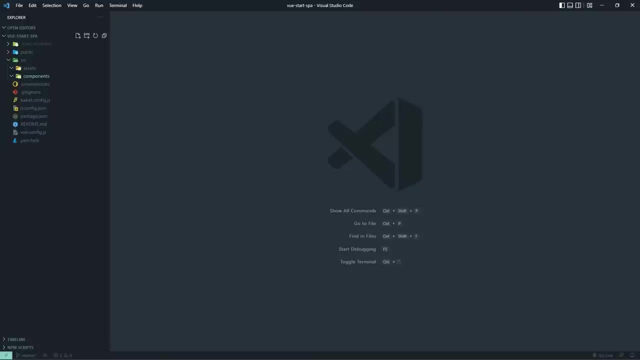 So I'm going to delete main.js app.view. I'm also going to delete hello world inside of the components folder, as well as the logo.js. And I'm going to delete the main.js.png inside of assets. Now, one thing about the source folder is that everything inside of it is essentially arbitrary. 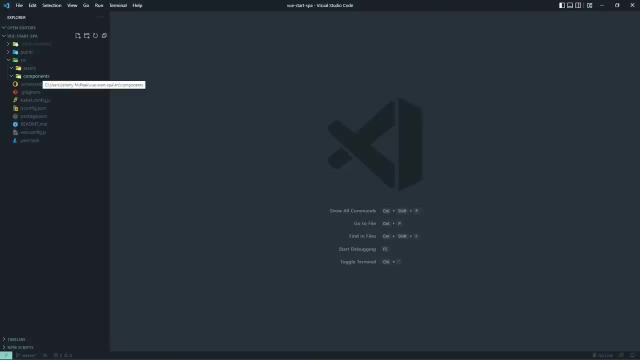 So this components folder, it really doesn't matter. We can call it whatever we want. 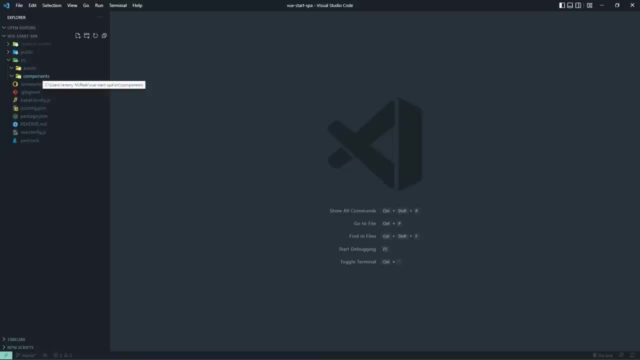 We don't even have to have it if we don't want to. So we can delete everything inside of the source folder. The only thing that we absolutely positively need is a file called main.js. Because this is the entry point of our application. Now, we can change the name of this, but we also have to change the configuration of our project. And there's really no reason to do that for most projects. So we're just going to leave it as main.js. And the first thing we are going to do is import create app from view. 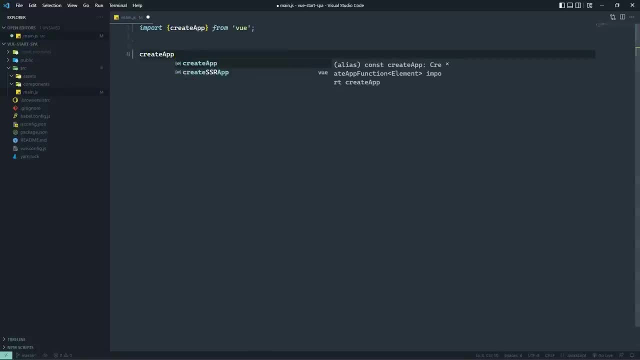 So this is going to give us direct access to the create app function. So we don't have to say view.create app or anything like that. 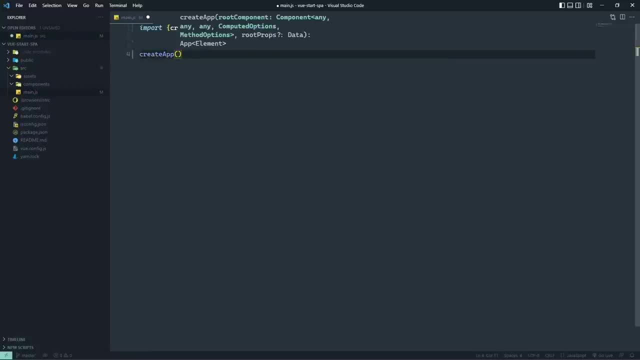 We just call create app. And this is just like the create app method that we used before. We paste it into our project. And then we're just going to leave it as main.js. And this is just like the create app method that we used before. We paste it into our project. And then we're just going to leave it as main.js. 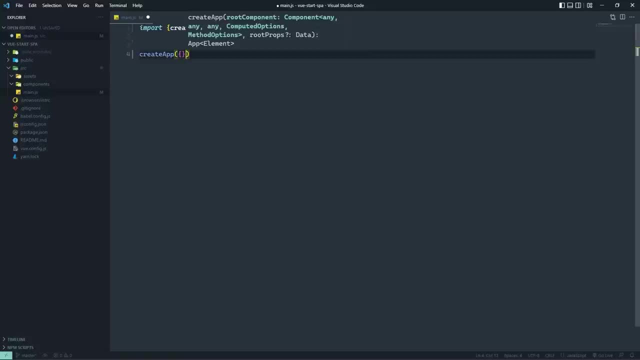 And then we're just going to leave it as main.js. 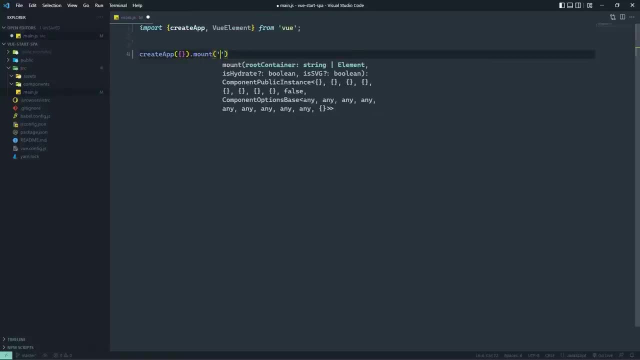 And then we want to mount it to whatever element I believe the one that we want has an ID of app. 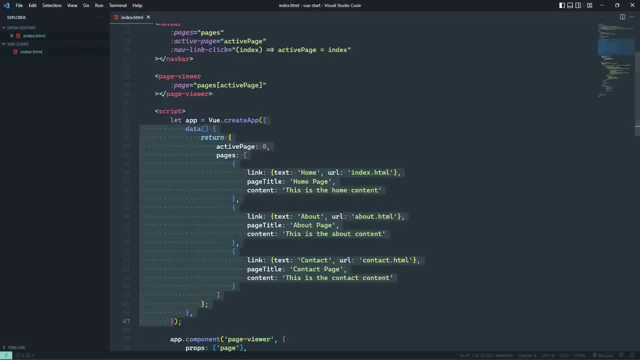 Now, one thing if you'll remember from the first version of this application is. We had to create an app object so 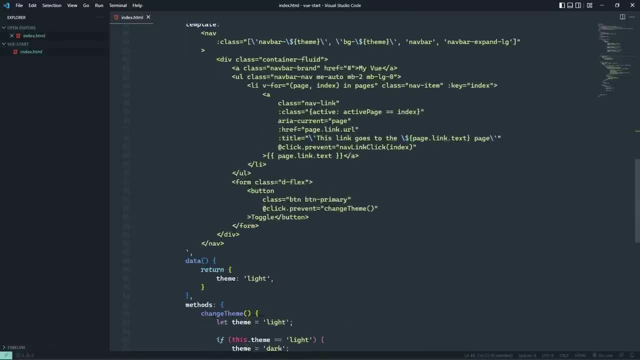 that we could create our components using the component method. And then we could mount the app to an element. We don't have to do that using the tool chain. 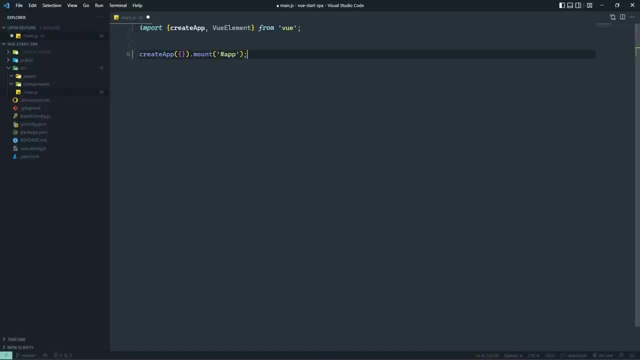 Because as we build our components, we are able to define the components that we are using there, which you will see whenever we create our app component. 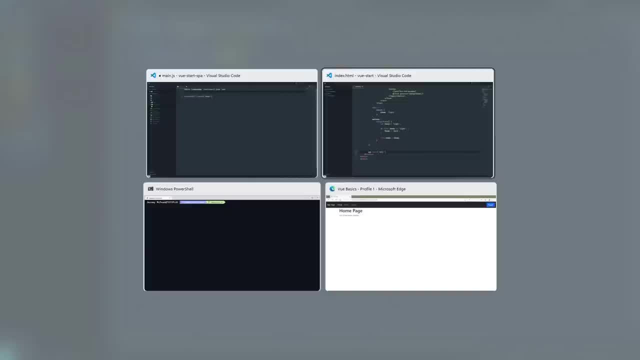 The app component for our application is essentially going to be the options object that we passed whenever we called create app. 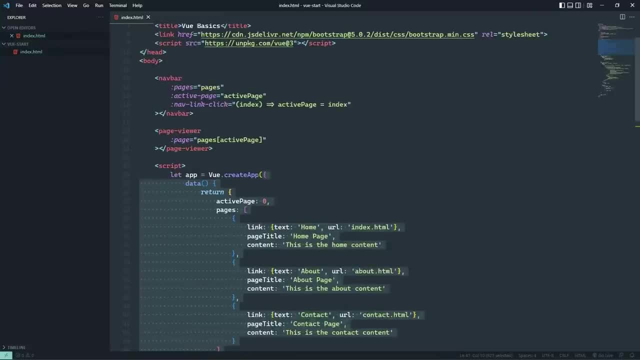 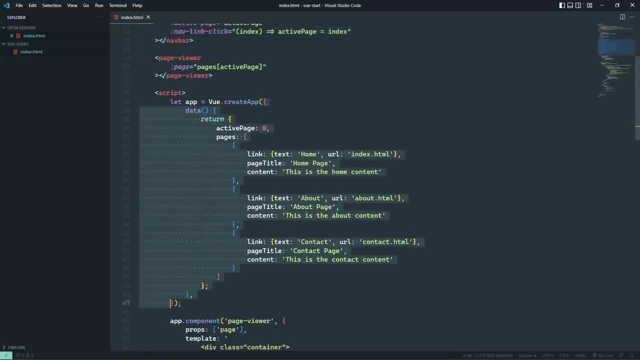 But it's more than that, because remember that we also have a template, and the template for our application has the navbar and the page viewer. So one thing I'm going to do is just go ahead and 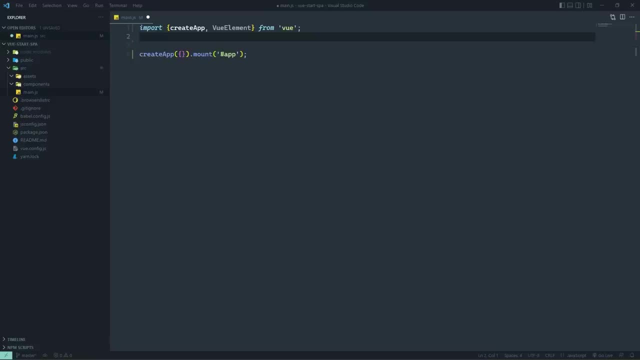 grab this object whenever we create this application, because we will need that. Let's create a new file, we'll call this app.view, this is the convention. We have a component that serves as the container for our application. We typically call that app.view. 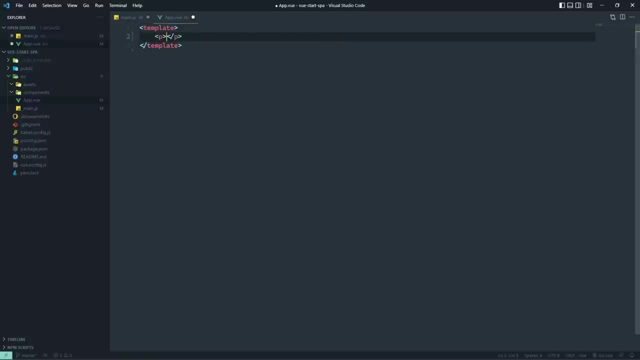 And we need a template, which for now, let's just have some simple text. And then we will have our JavaScript. Now, 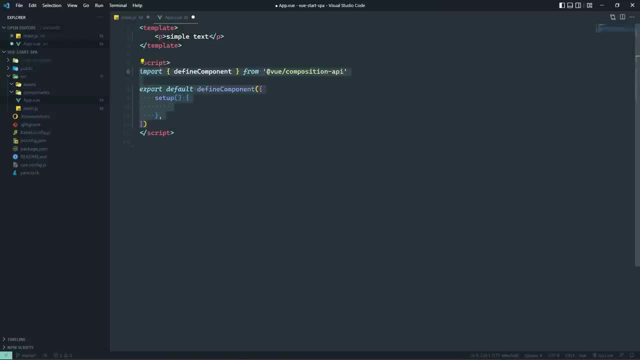 the audio code automatically injected this in this file, and I don't want that. Instead, we want to export a default object that contains the options that our application needs, which is the data, where we have an object that has the active page property as well as our pages. Now, we're going to add some more here, but let's first of all, import this app component inside of app.js, and we're going to run this, just to see if everything is going to work right now. 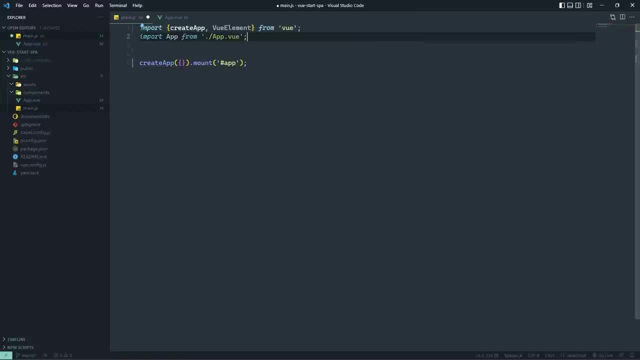 So we want to import app from app.view. And we're going to use this app, which is an object, because that is what we exported from this file. 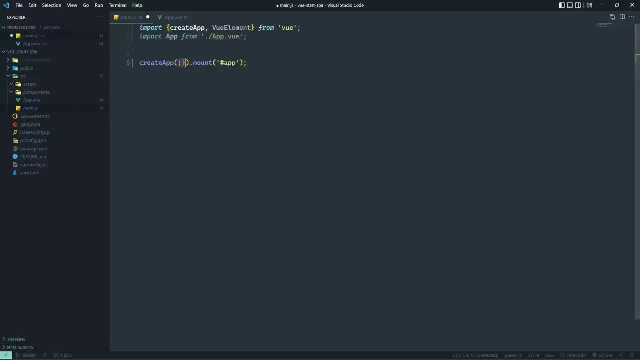 We're exporting this object here. And we're going to use that as the options object for our application. 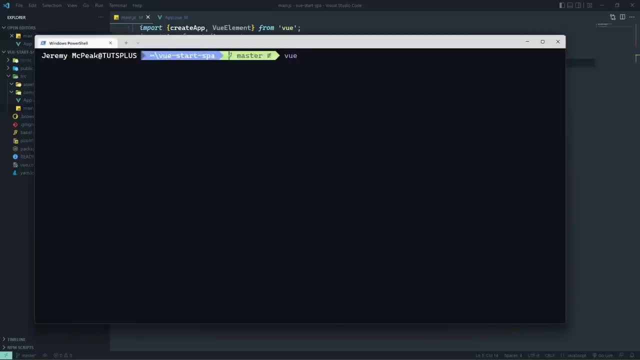 So now, let's go to the command line, and we want to use the view command. And we'll follow that up with just serve. This is going to serve our application for development purposes. 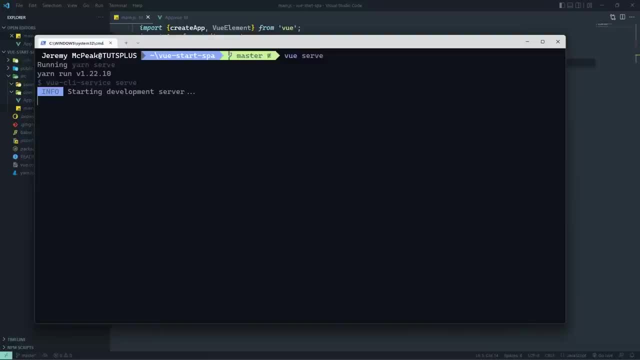 So this is going to take our code, it's going to build it into a running application that we will be able to view in the browser. 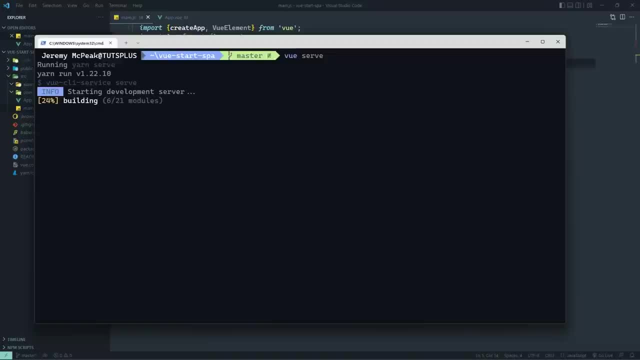 And it's going to watch for changes to our files. And every time that we make a change to our files, it's going to automatically update our application that's running in the browser. 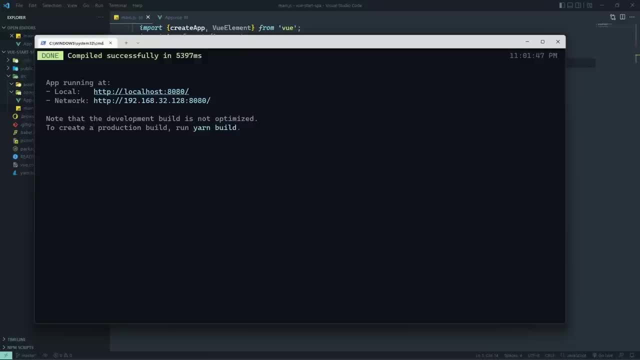 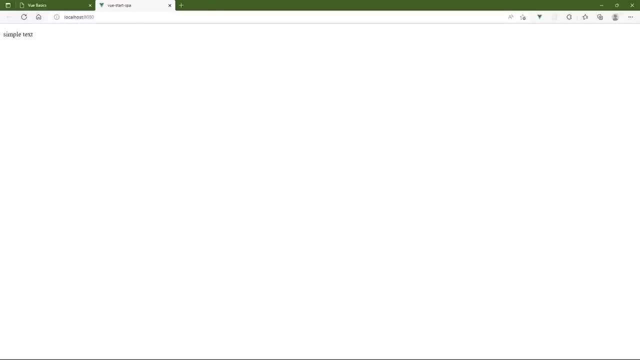 And it tells us where it's running, localhost 8080. So let's open that up in the browser, and we will see just some simple text, which is what we would expect to see, because that's all that we have right now. So let's go back to our application. 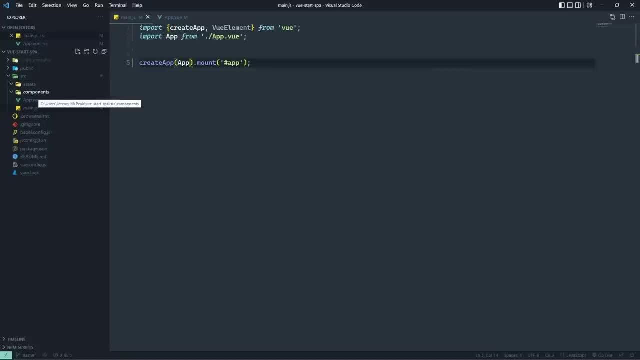 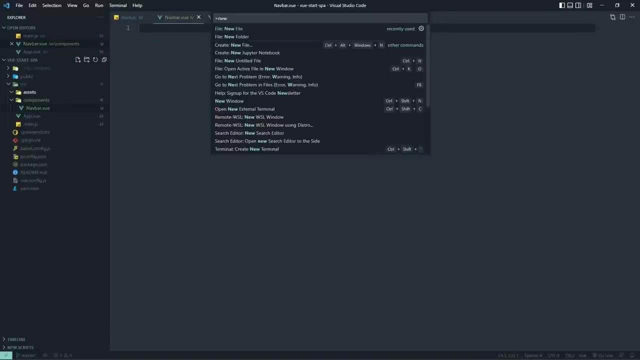 And we want to create our navbar and our page viewer components. And I'm going to create these inside of the components folder. Once again, the components folder is completely arbitrary. There's nothing special about it. We can rename it, we can delete it, and we can organize our project however we want. But it does help to have some kind of organization. And I'm going to call this first file navbar.view. Then we're going to create another file, which we will call page viewer. 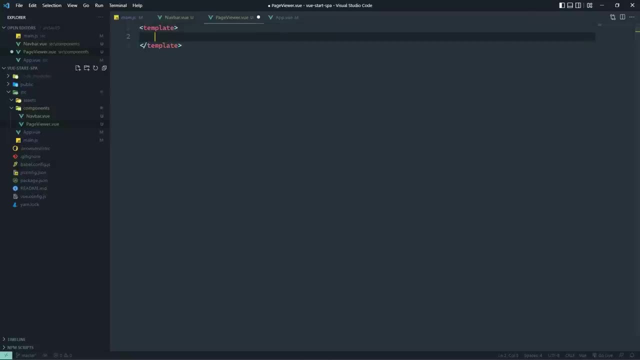 View and just like the app component, we need a template. We also need a script element. 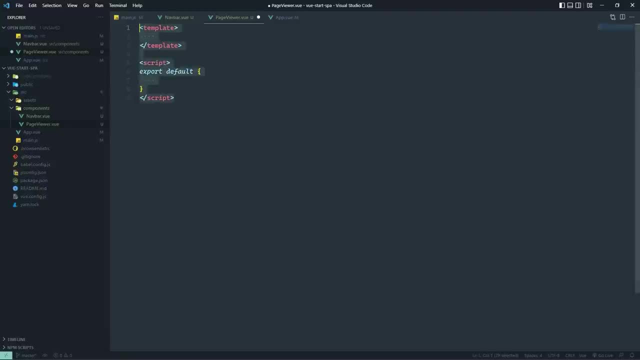 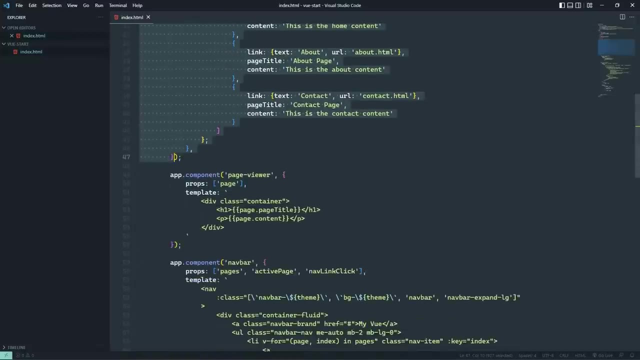 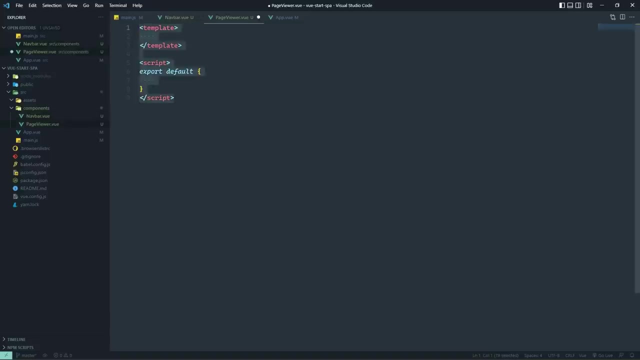 And let's start with our page viewer because this is the more simple one. And we're going to go to our older application. We're going to copy the options object that we have for it. And we're going to paste that inside of the script or the JavaScript. Now our template, we can leave here if we wanted. However, there's really no need to do that. However, there's really no need to do that. 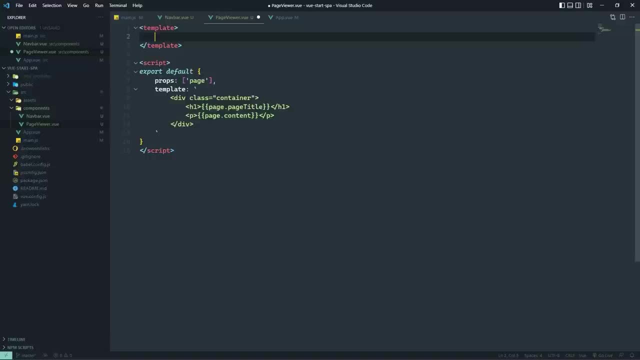 Because we can actually define our template inside of the template element. So let's just cut that out, paste that inside of template. And now this is so much easier to work with. 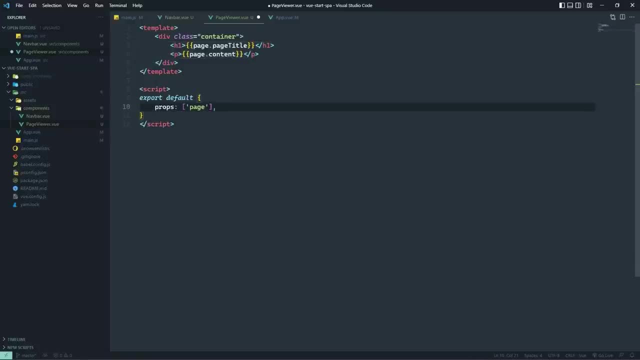 Although with this particular component, the template was simple to begin with. The navbar is the one where we had to do some escaping. 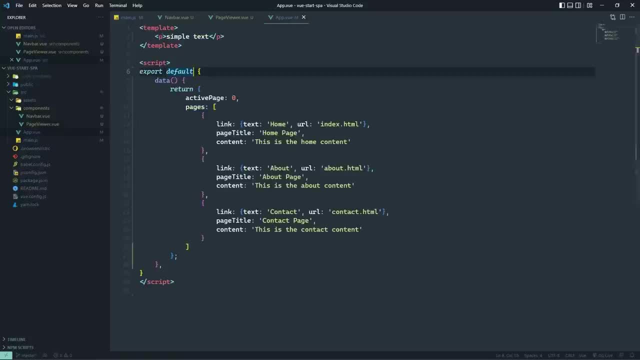 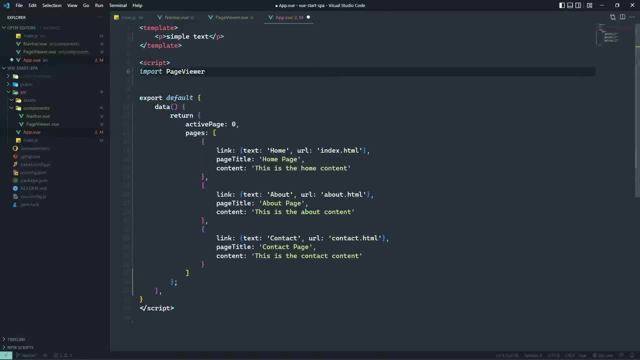 But before we get to the navbar, let's go to our app.view. Before we export our options object, we want to import that page viewer component. That is from our components folder. 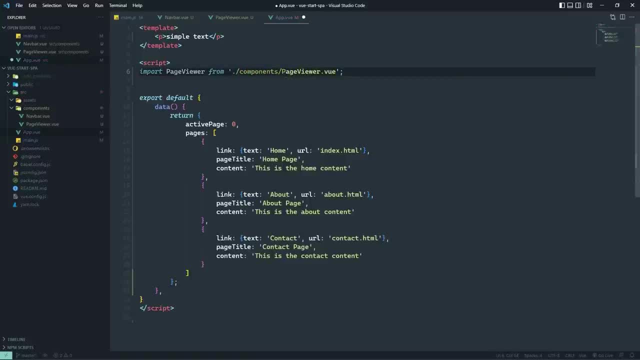 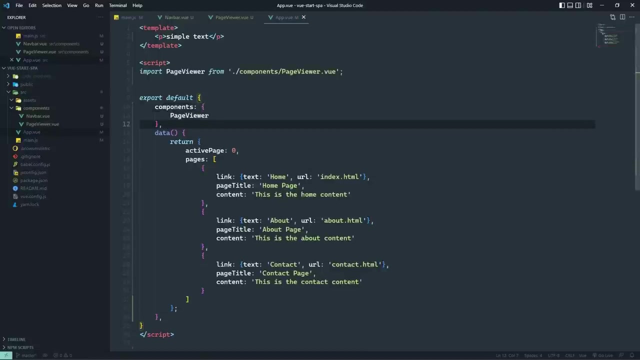 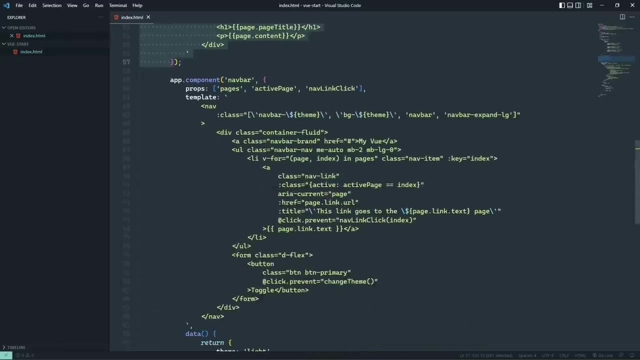 The file is called pageviewer.view. And we want to tell this app component that we want to use our page viewer. And we do that using a components option. This is an object that contains the components that we use inside of this component. So we have page viewer, we can use that in our template. But of course, by itself, the page viewer is kind of useless. We also need the navbar. So let's go ahead and go back to our index.html. Let's take the entire options object that we used for the navbar component. 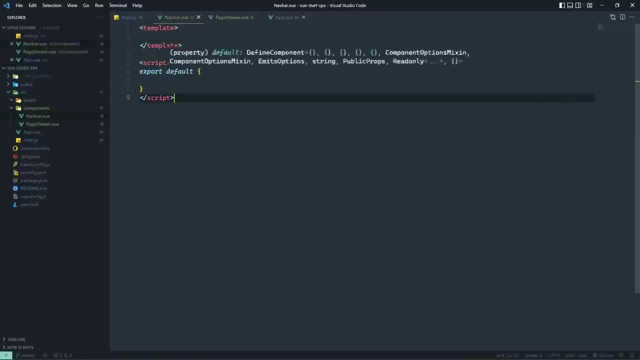 And we're going to paste that in the JavaScript so that we are exporting that object. 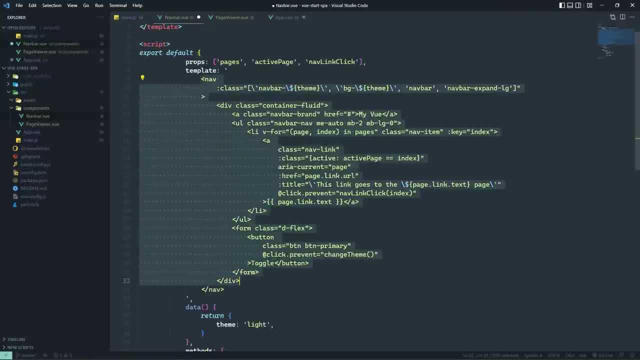 But once again, we have this template that we want to cut out of this options object. 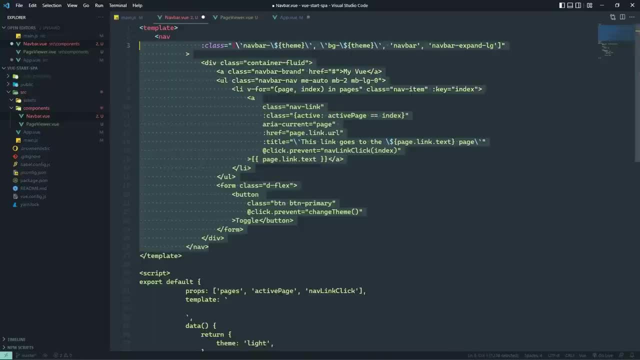 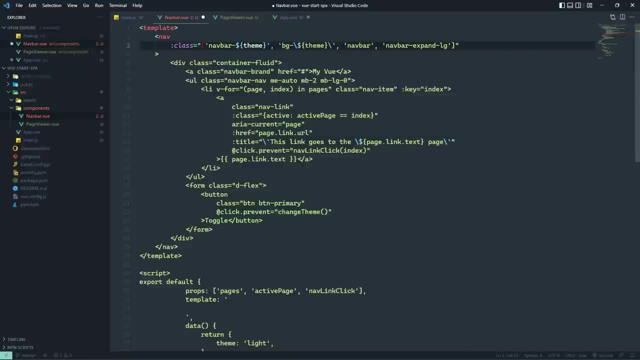 We will paste the template inside of the templates element. But we do need to make some changes. For one, we need to get rid of all of the options. For one, we need to get rid of all of the options. For one, we need to get rid of all of the options. For one, we need to get rid of all of the escaped characters which thankfully there weren't a whole lot but we do need to be sure to delete the correct ones. 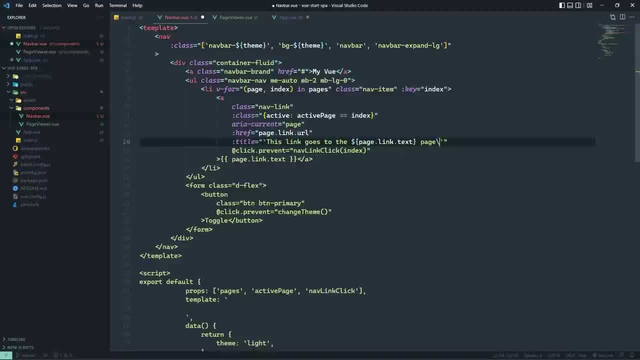 And then we also have it inside of the title here. So we will delete those everything else should work. 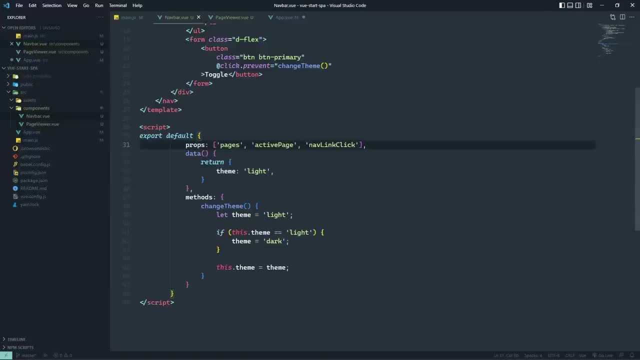 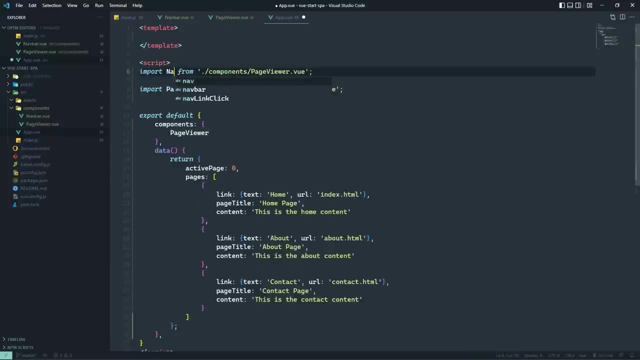 Let's delete the templates here. And so then we want to import the navbar inside of app.view. So let's just copy and paste that code to where we import navbar from components, navbar.view. 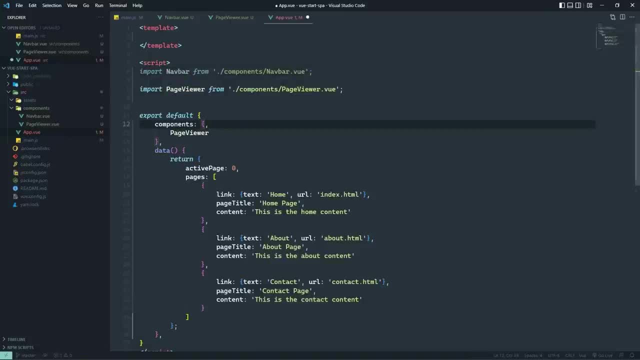 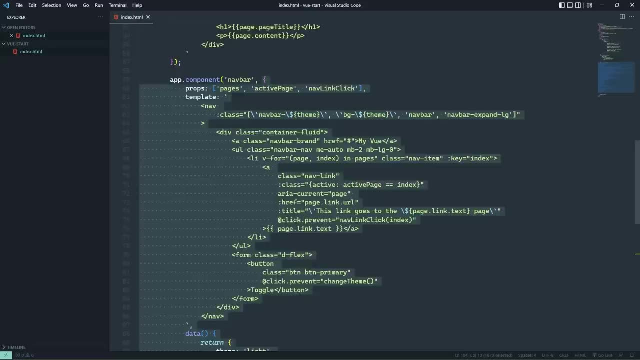 We are using navbar inside of app.view, so we need to add that to our components. And then we just need to use the template from index.html. So let's grab navbar and pageViewer. 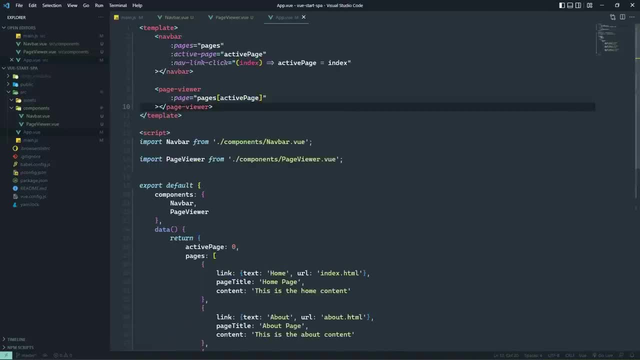 Let's paste them inside of the template for our app. And let's see if this works. 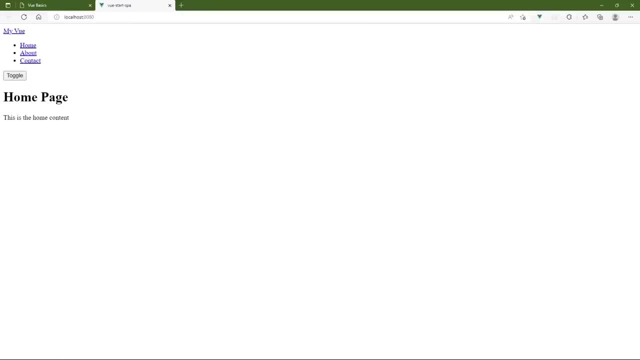 Let's go back to the browser. We'll see that our styling does not work very well. 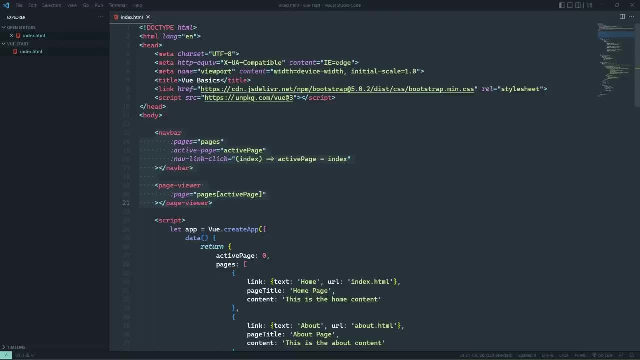 So that's one thing we need. Let's go to index.html. Let's grab this link element that references the Bootstrap CSS. 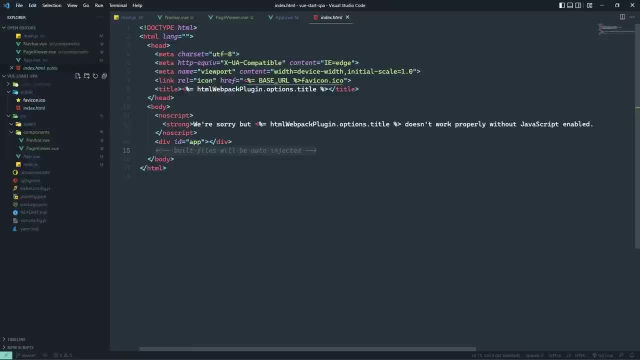 And we're going to put this inside of our index.html. Now since we are using NPM, we can actually install Bootstrap as a dependency for our project. 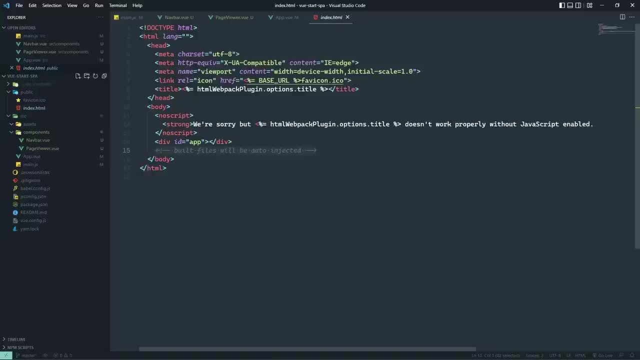 And then we can import that into our application, which is something that we will look at. 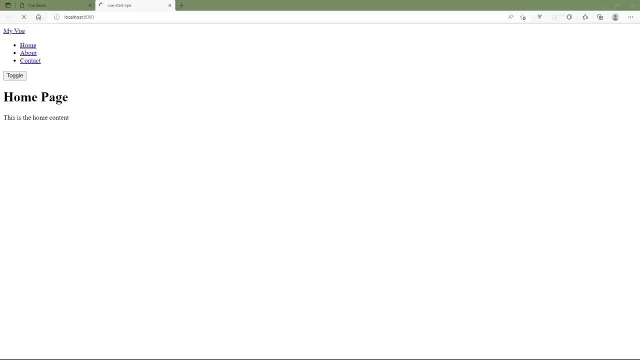 But for right now, we are just going to take this route. So whenever we get back to the browser, all of our styling is there. So now is the moment of truth. 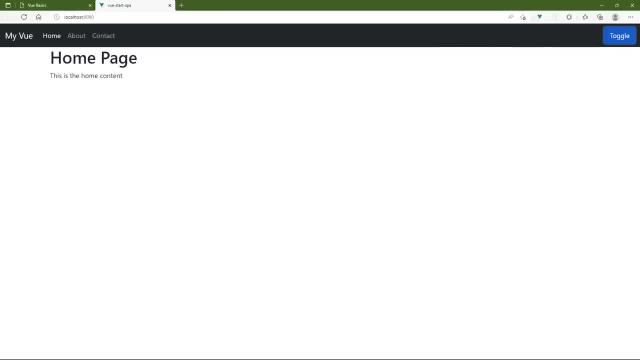 Whenever we can get back to the browser, if we click on the Toggle button, we can see that the style for the navbar toggles. 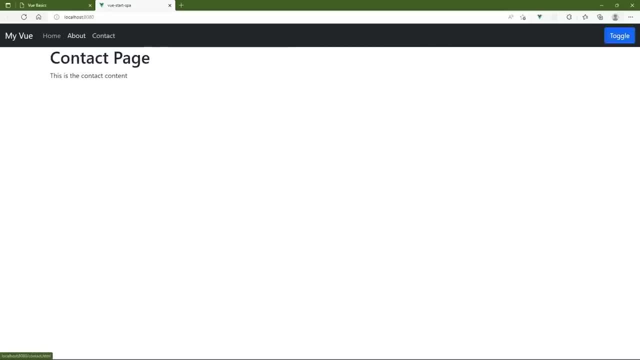 If we click on one of the links for about or contact, we can see that that is indeed working as it did before. 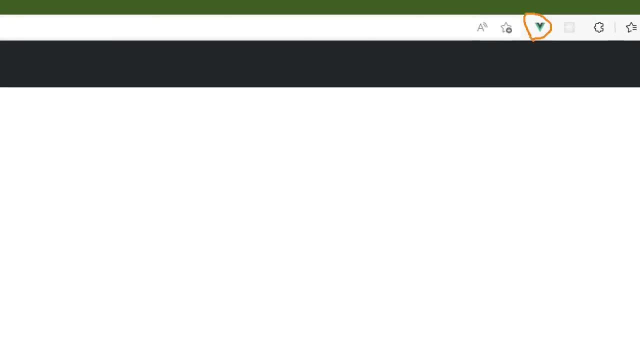 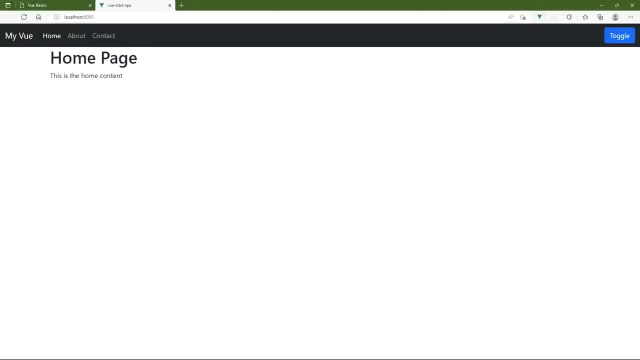 Now also notice that the view icon for the developer tools is lit up. That means that it recognizes that view is running in this application and we should have access to the developer tools. 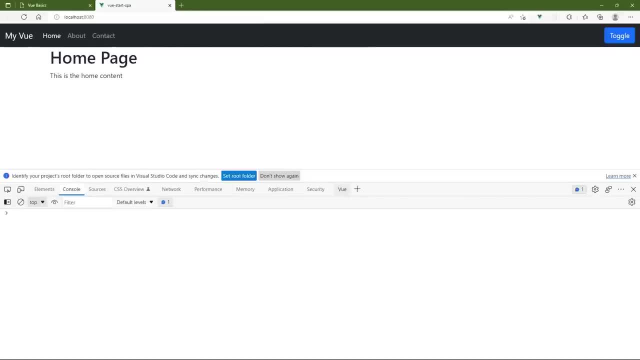 So I'm going to pull those up. It's not going to show by, well, it is going to show by default. 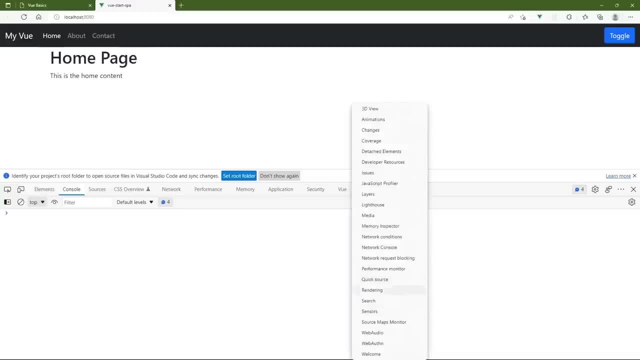 Sometimes you have to click on the plus sign for more tools and then choose view. But here it is. And we can take a look at our application in the developer tools. 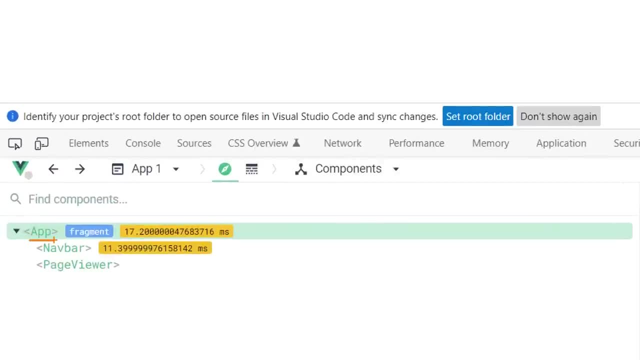 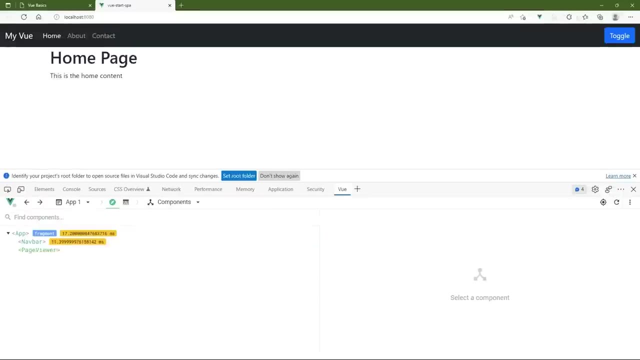 So you can see that we start with app, that is the container for our application. Then we see the navbar component that's being used as well as the page viewer. 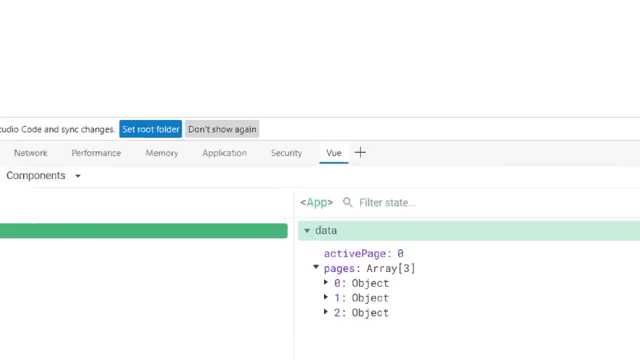 And whenever we select one of these, I'm going to select app. Over on the right hand side, you can see that we have our data options. 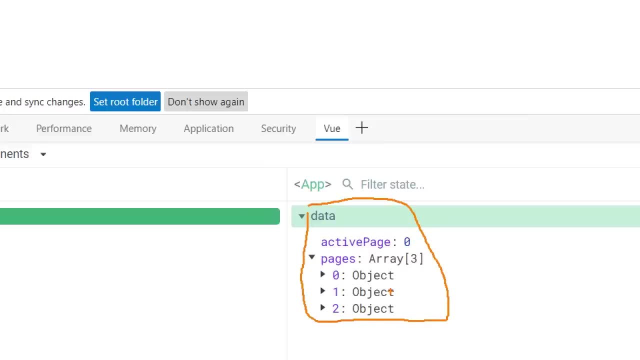 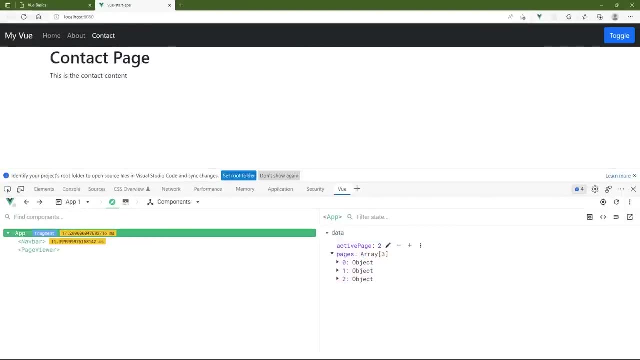 So we have the active page and then we see the pages array. Now, if we click on one of these links, let's just go to contact. You're going to see that active page automatically updates. So any change that we make through our application is going to automatically appear within the data and the state of our application. We can also edit this value. 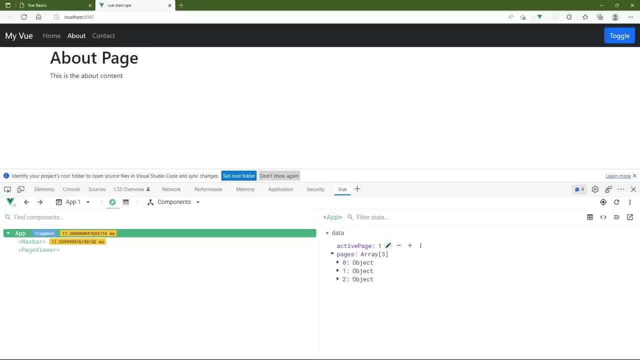 So right now the about page is active. If we change this to zero and then submit that change, we can see that our page is now active. So we can see that our application updates accordingly. 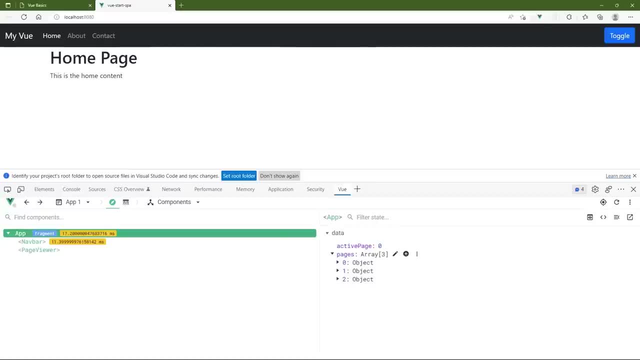 And the reason is very simple, because Vue is watching for changes to not just active page, but also to the pages array. So if there's any change to these values or objects, it's going to automatically update the DOM. 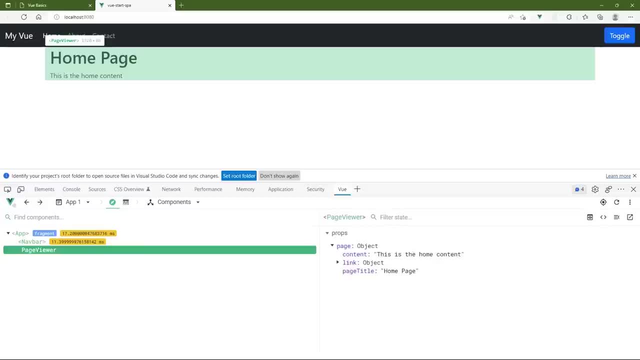 And this gives us the ability to easily debug. 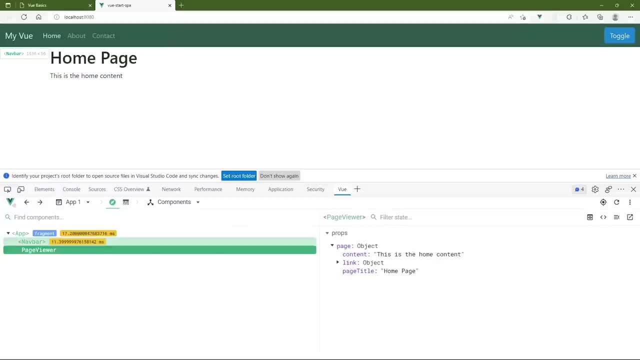 If we run into any issues, if a component isn't necessarily rendering correctly, for whatever reason data isn't properly flowing down, we can use the developer tools to debug those problems. Makes our lives a lot easier. So there we go. 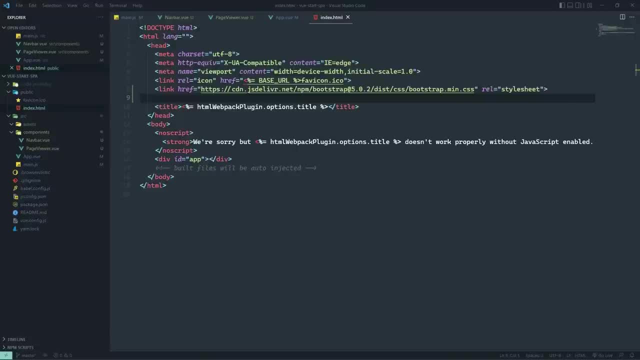 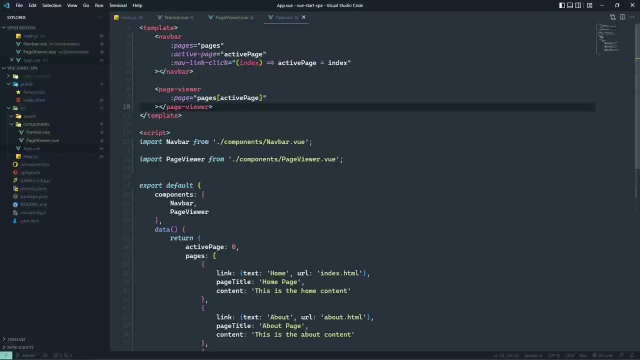 We have recreated the application that we've been working on using the Vue tool chain. It does require some extra code. However, now our application is so much easier to develop and 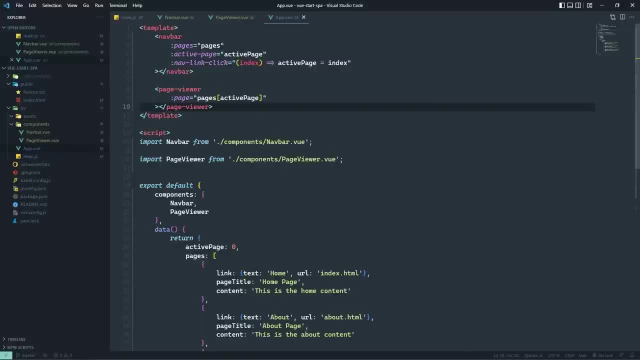 maintain because everything is compartmentalized into its own files. 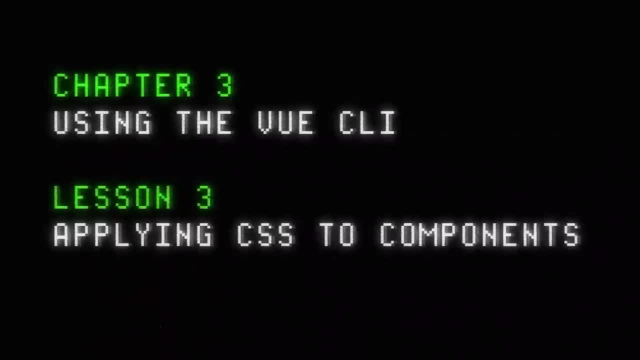 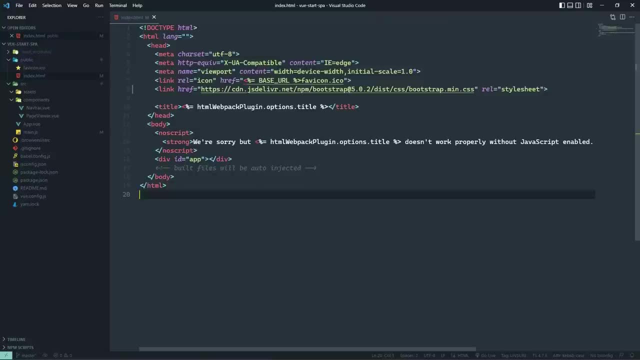 Now that we are using the tool chain to work with and build our application, we need to talk about style. Because the way that we work with an import style will change just a little bit, at least as far as what we are used to. Now, everything that we have talked about thus far about applying CSS classes to elements is still valid. It does not change. What I want to discuss first of all is how we bring in CSS from an external source. Like for example, in the previous lesson I added the CDN to bootstrap inside of the index HTML. And while we can do that, I'm going to show you how to do that. I'm going to show you how to do that. 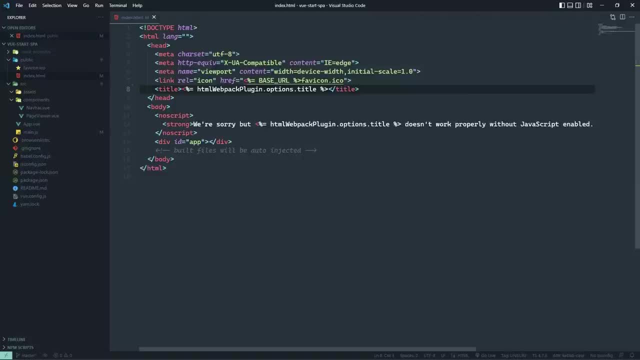 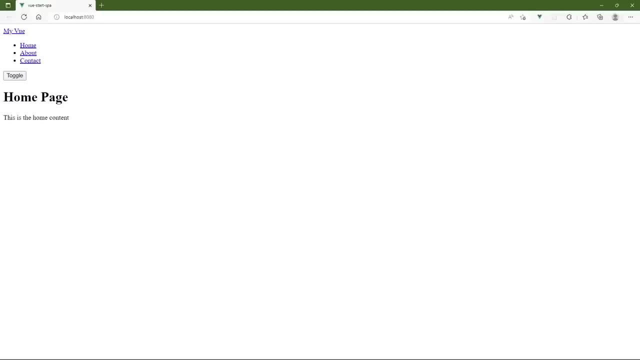 Really what I want to do is take that out, because I want to install bootstrap in this project and then import the CSS file into the application that way. 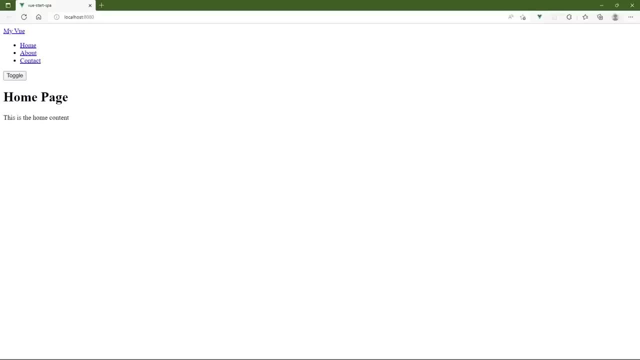 So this is what it looks like right now without the CSS from bootstrap, which of course that's what we would expect. 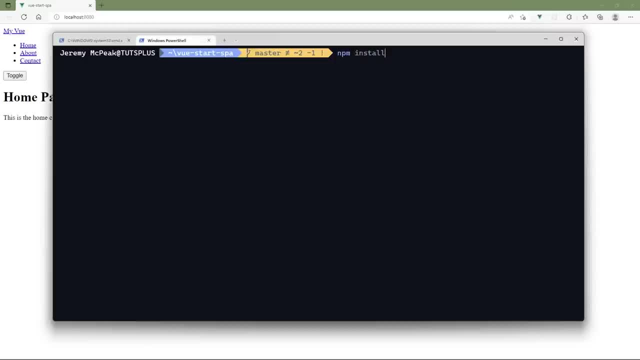 And then I want to go to the command line, and we will install bootstrap. And we are going to save this as a dependency. And the reason why we want to save this is so that whenever we need to do something, 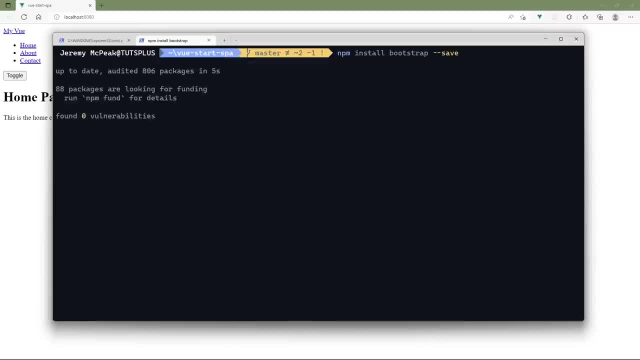 we need to install everything all over again. 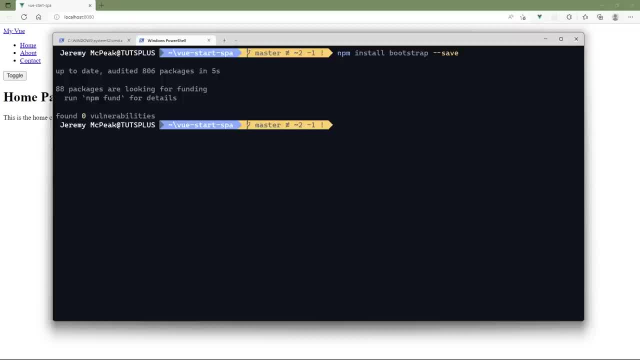 All we have to do is say npm install, and then everything including bootstrap is installed. 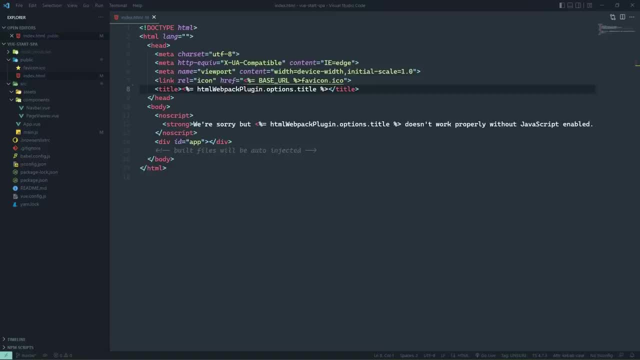 So we are good to go now. Let's go back to our code. 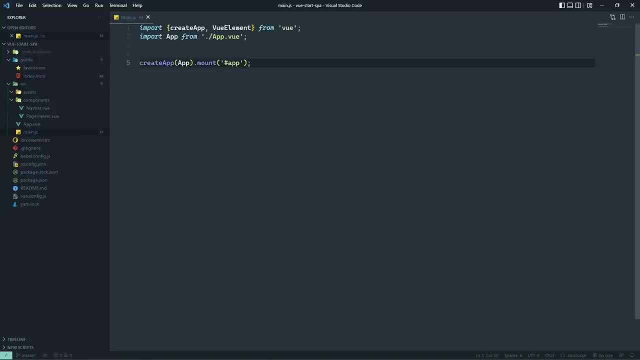 And I'm going to open up the main.js file. Because this is where we will import that bootstrap CSS. 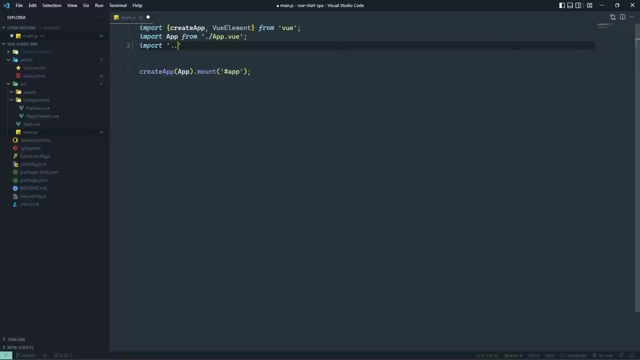 If you've never done this before, it's going to look pretty weird. But what we want to do is import from node underscore module. 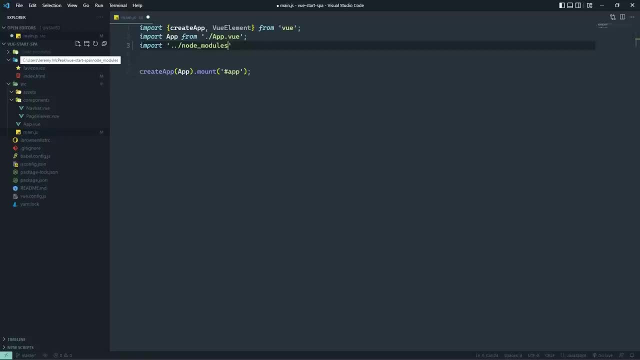 Now, if you're not familiar with node at all, and this is your first experience with it, everything about our project is installed inside of this node underscore modules. 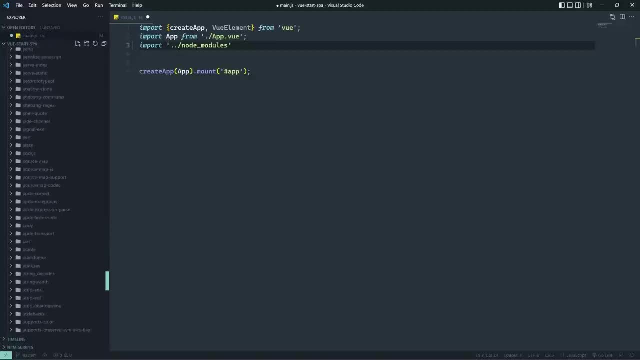 As you can see, there's a lot of stuff here. So everything that's here is because our project needs it, 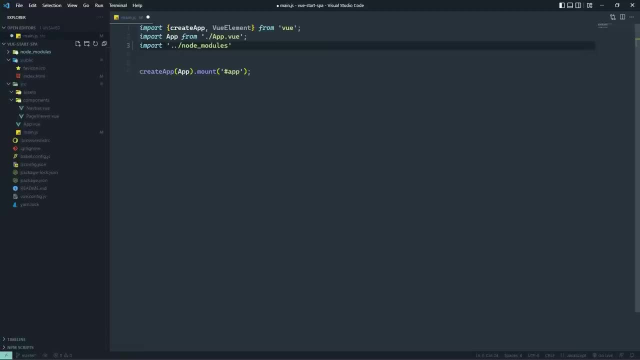 either because of the Vue CLI or because of bootstrap. 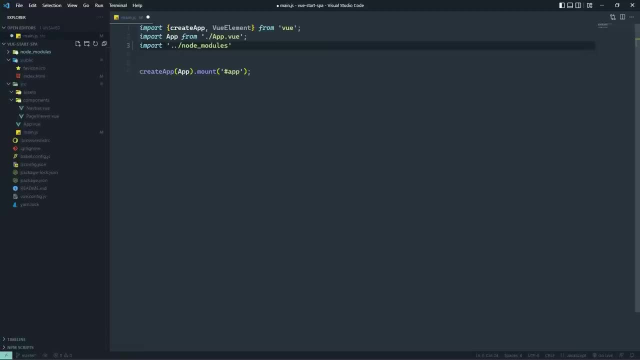 So we want to leave node underscore modules alone. In fact, we very rarely ever open a document, 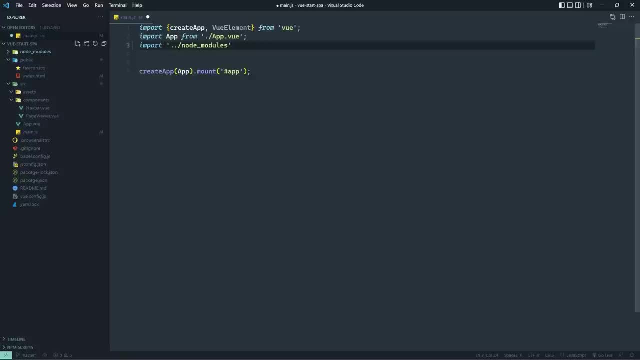 but we do want to do that. It can be useful because there is source code in there that you can read if you 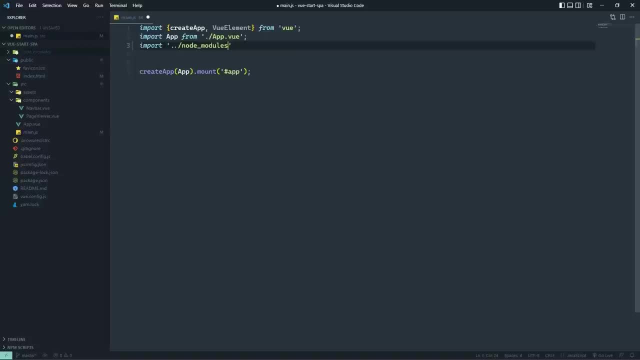 ever need to figure out how something is working. But for our purposes, we don't want to do any of that. 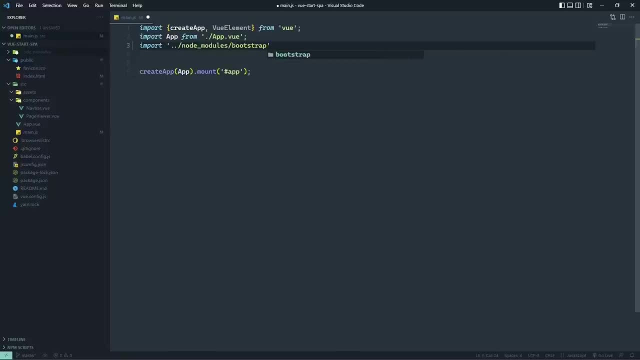 We want to import from node modules slash bootstrap slash dist for distribution CSS slash bootstrap.css. 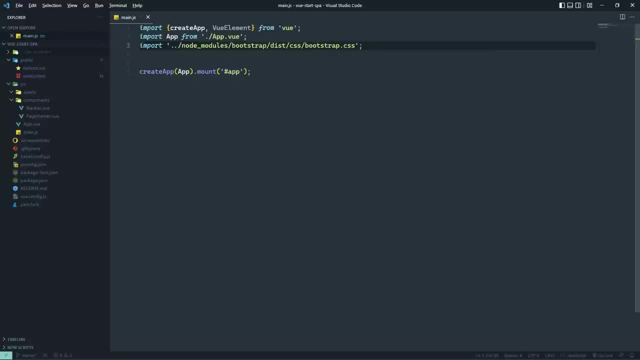 Whenever we save this, then the build tools are going to pull that into our application, and it's going to automatically inject that into the browser. 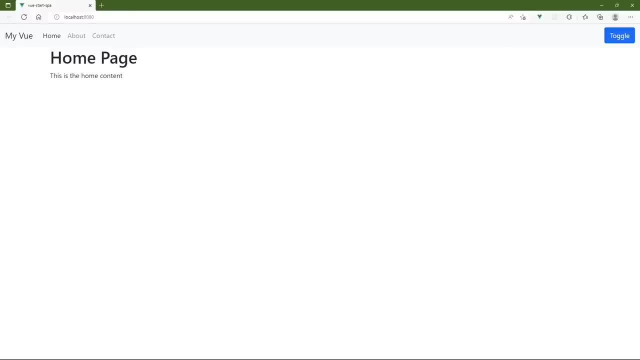 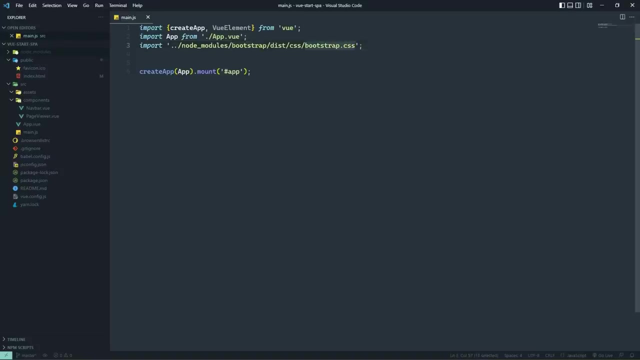 Now, there are several advantages to doing this. Because we have these build tools, part of their job is to optimize the files that are being built. So in this whole process, it is going to optimize the files from bootstrap.css as well as our source files. 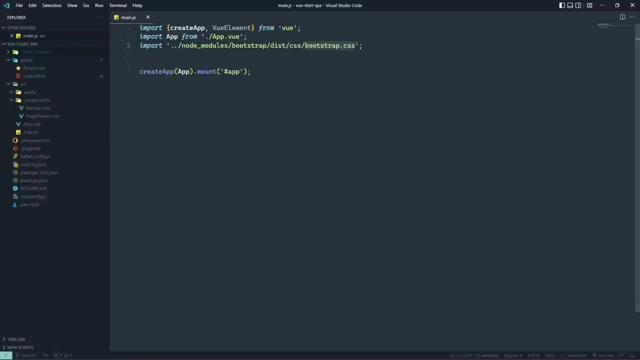 And anything else that we import that is ran through the build tools will be optimized as well. 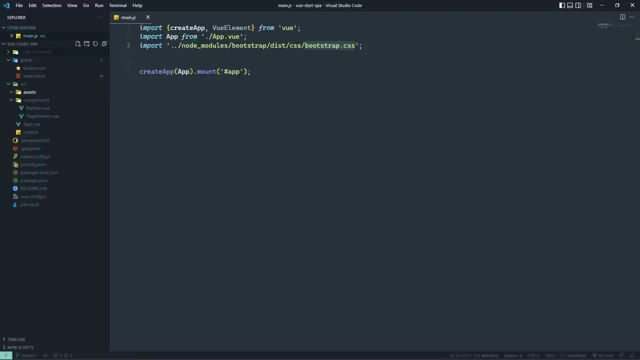 So we don't want to be running images. So sometimes we do want some images run through the build tools as opposed to putting them inside of the public folder. 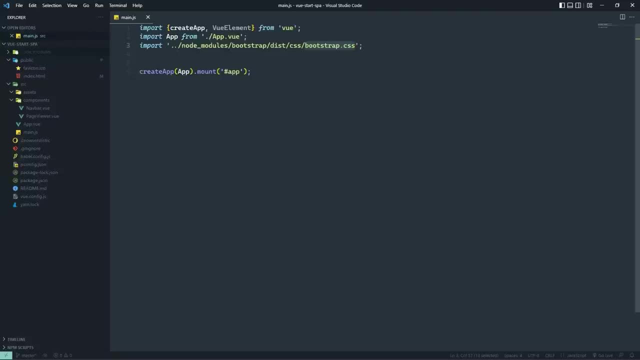 That's for later. Right now, we now have bootstrap. 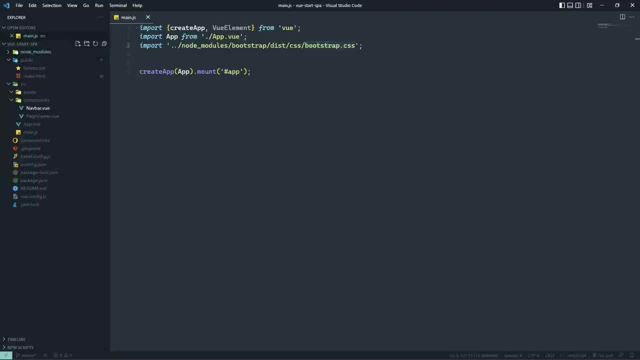 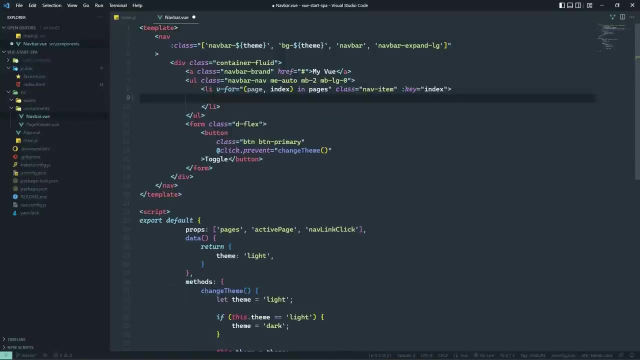 What I want to do now is break out some functionality inside of our navbar. Specifically, I want to take this A element, and I want to essentially turn it into something like this. 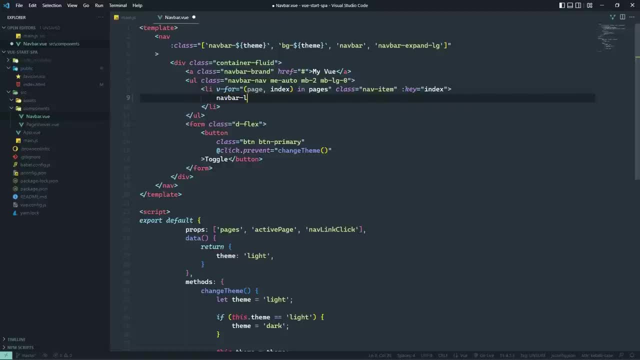 So that we have a navbar link, and we will supply it. Essentially two things. 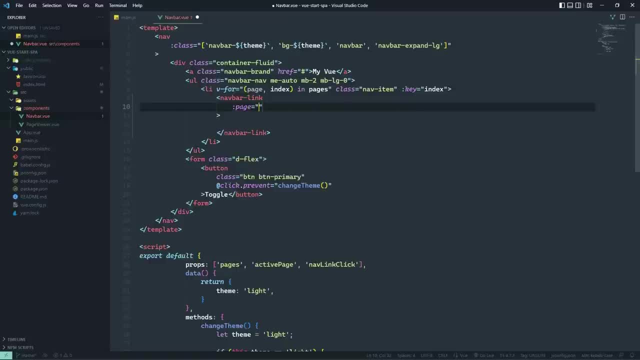 We will have the page that we want to display, or at least the link to. And then we will have something called is active. And the value of this is going to be based upon whether the current active page is equal to the current index. 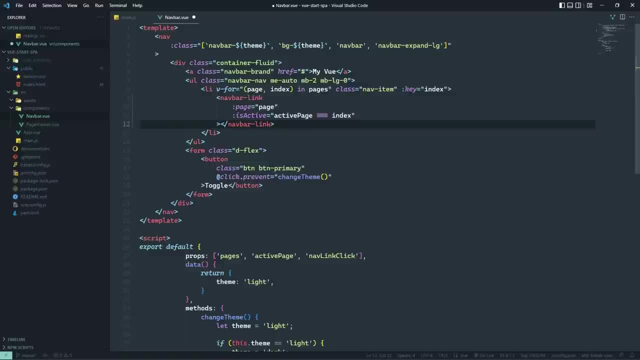 Now, you might think that this is a waste of time. Why would we want to do this when we can essentially do the same thing with just this A element that we've done before? 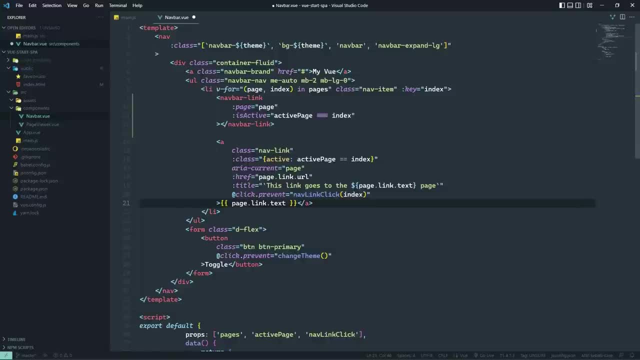 Well, there are many reasons, and probably the most important reason is that by breaking this functionality out, we now have a component that is going to be strictly for the purpose of displaying a single link. 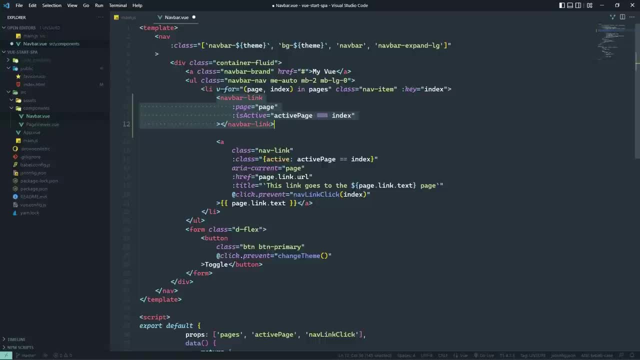 It's responsible for displaying the link as well as the different states of that link, if it's active or if it's not. 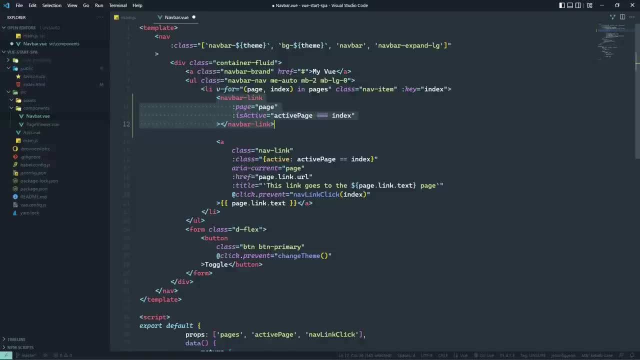 There's some benefits to having that functionality extracted inside of its own component. 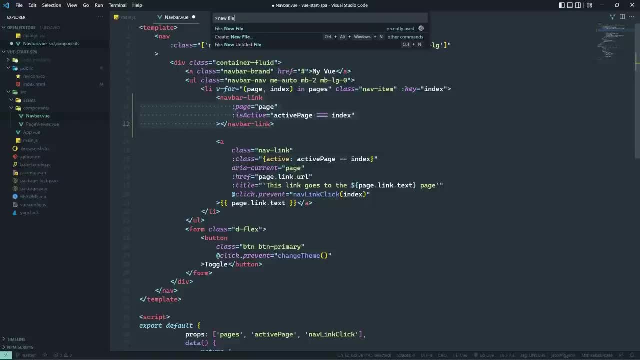 So as you are developing your applications, you might find, hey, I can extract this out, even if it's something as simple as this. There's no harm in doing it because ultimately, it makes your application easier to develop and maintain. 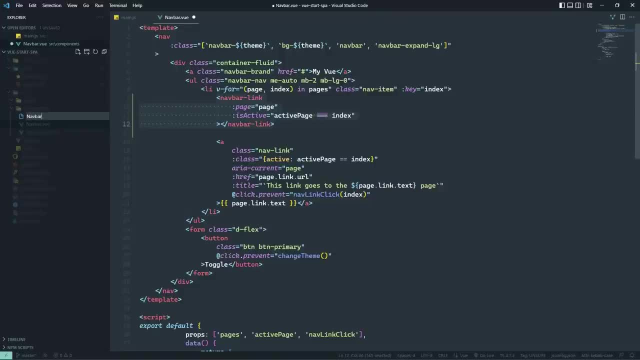 So we're going to create this navbar link component. 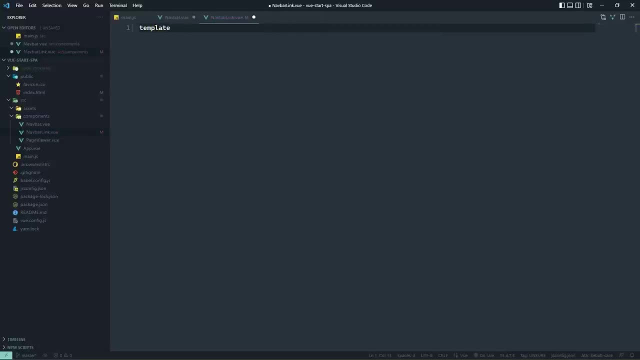 We'll have the template, which is essentially just going to be that A element. 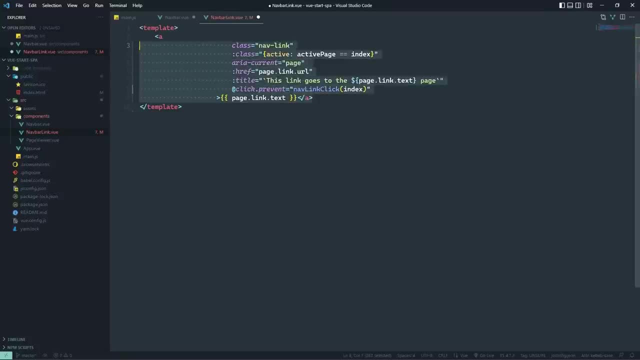 However, we get to clean it up a little bit because we no longer have this active page. But we'll get to that. Let's add a link. Let's add the script. 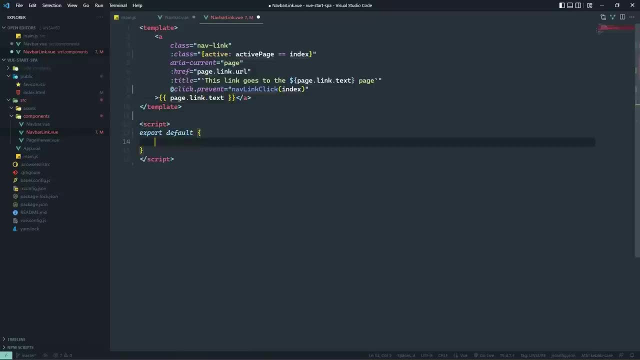 And we want to export a default object. Let's go ahead and define the props to where we have the page. And we have that isActive. And then we are also going to have the computed option. 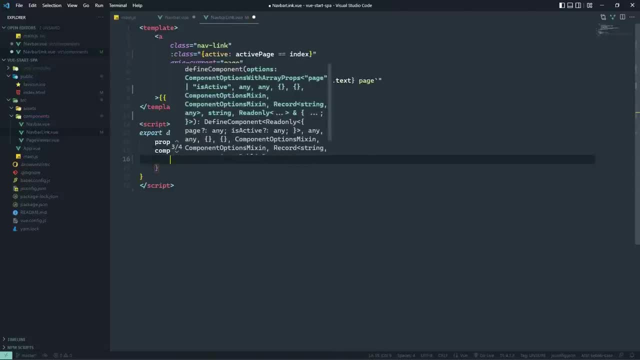 Because we're going to create a computed property called activeClasses. Because really what I want to do is apply multiple classes whenever a link is active. Of course, the first one is going to be active. It's going to be the active class. And we can now use the isActive prop to control that. The second one that I want is called emphasize. And this is also going to be based upon the isActive prop. So that we can use this active classes right here whenever we bind our CSS classes. Now, we don't need this click event listener. 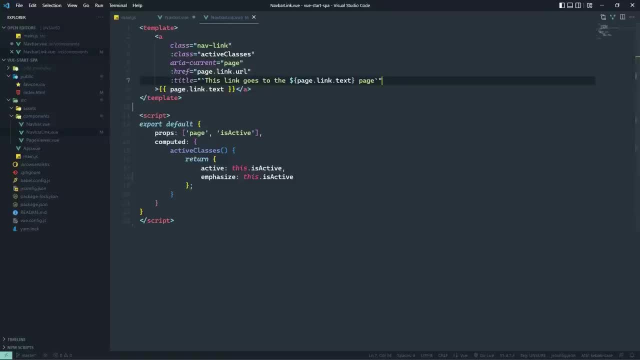 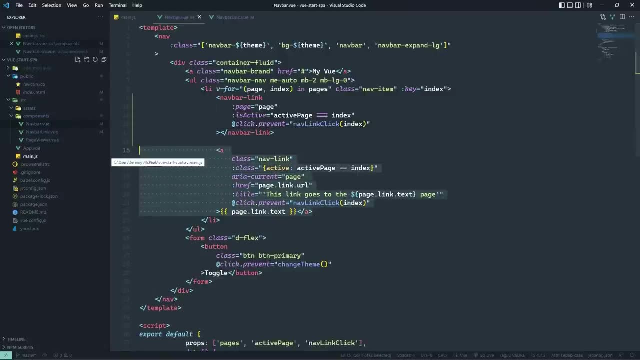 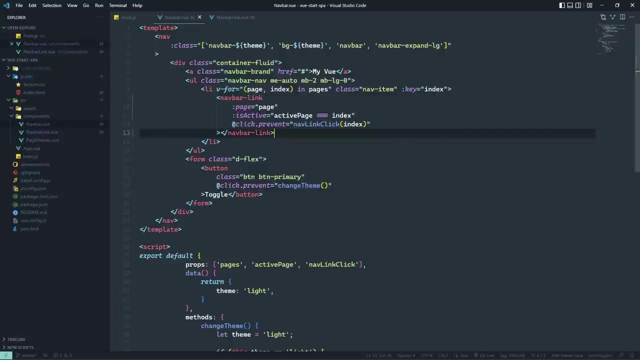 I mean, there is nothing that says that we can't do that here. However, if we add this to our navbar link component here, we are going to see that it's automatically going to be applied to the A element. So that whenever we click on this A element, we are still going to get the same functionality. This way, we don't have to define this nav link click both here and on the navbar link. And this is just one of the magical things about Vue. This click event is going to be placed upon this link. On this A element. 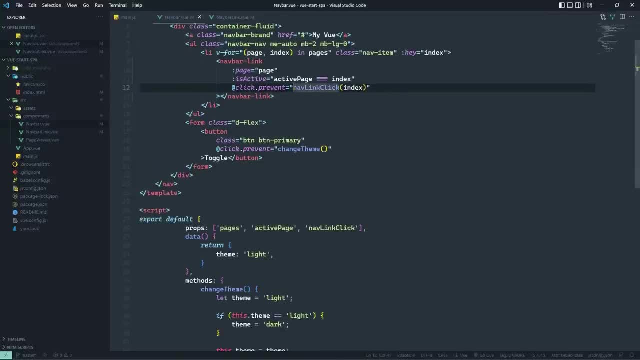 Now, it's not going to work as it is right now because inside of navbar, we do need to import this navbar link component. 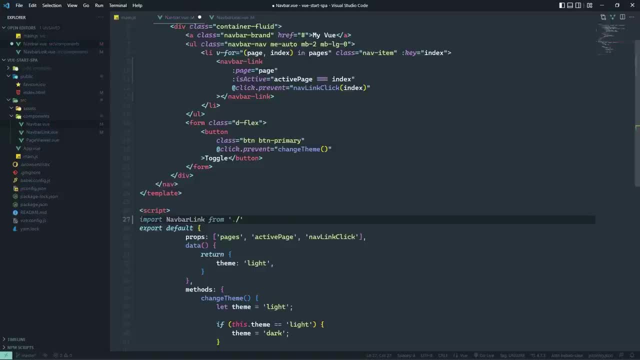 This is from a file inside of the same directory. So we just need to say ./.navbarlink.vue. And then we need to add the components option to our options object here. 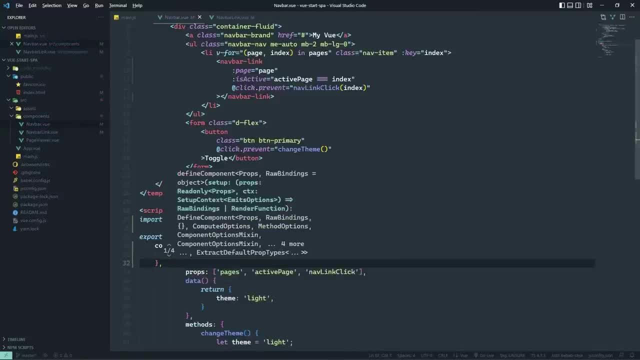 And we will, of course, reference navbar link. So with that done, let's just go back to the browser. Let's do a sanity check. Make sure everything is working as it did before. 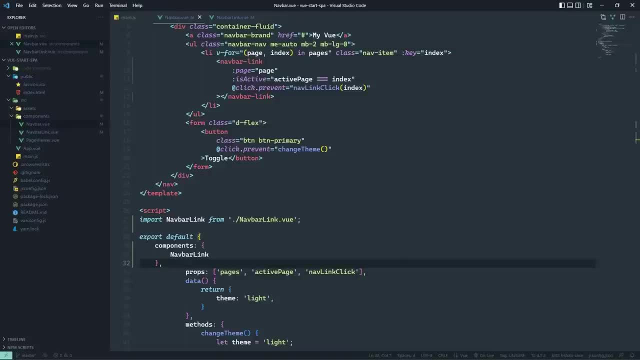 It does, so that's great. But now I want to add that emphasize CSS class. 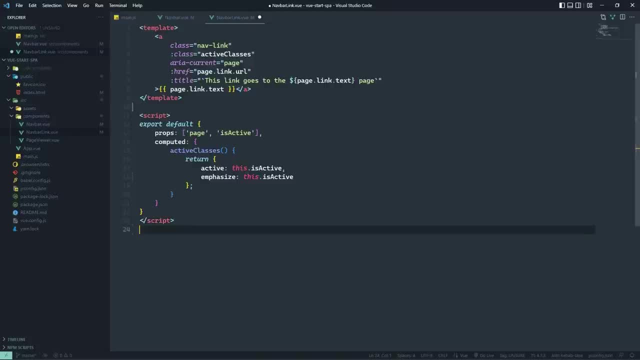 So back inside of navbar link, I'm gonna add a style element. And inside of this, we'll have that emphasize. 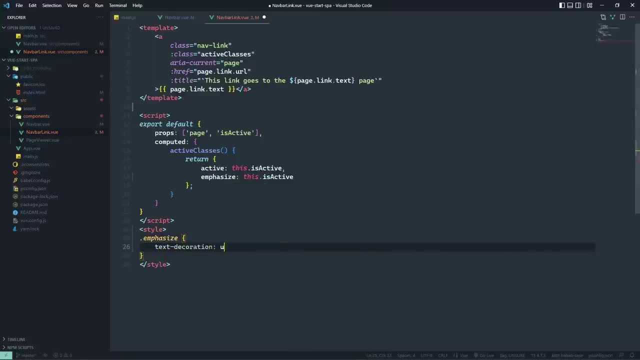 And we are going to set the text decoration to underline. But let's do important because I think Bootstrap is going to override that. 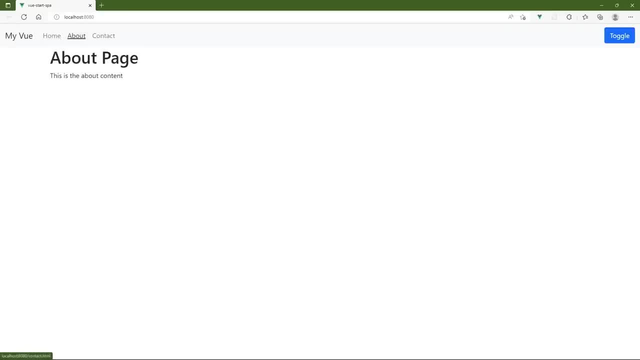 So let's go to the browser. There we go. There we can see the underline. 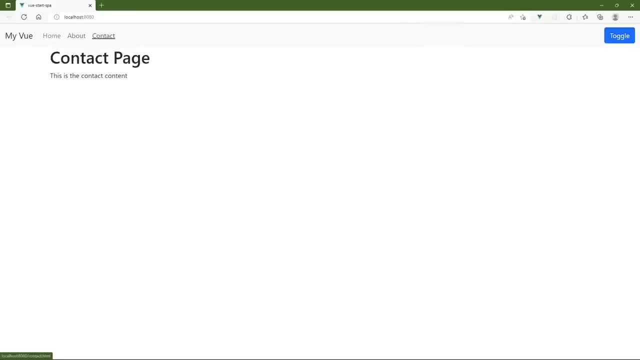 And whenever we click on the links, of course, we see the underline follow the active link. That is what we would expect to see. 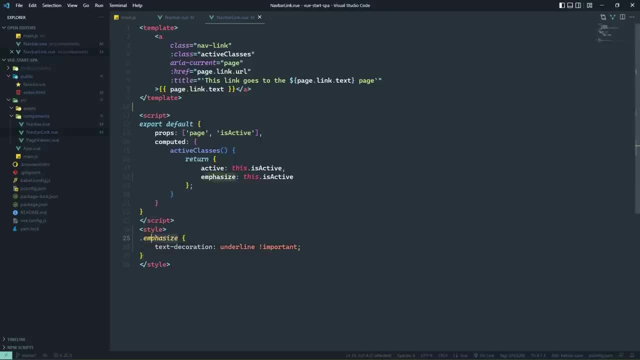 Now, we might think that because we defined this CSS class directly here inside of this component, that it is scoped to this component. That is not the case. If we go to page viewer, which is a completely separate component, there is no relationship between that and the navbar link, at least as far as components are concerned. 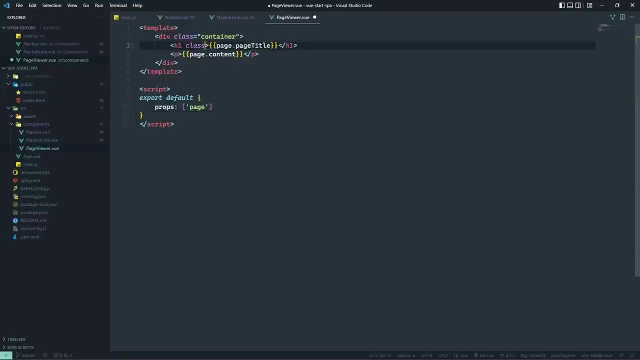 So we can go to this A element, and let's add the emphasize CSS class. And we are going to see it underlined as well. 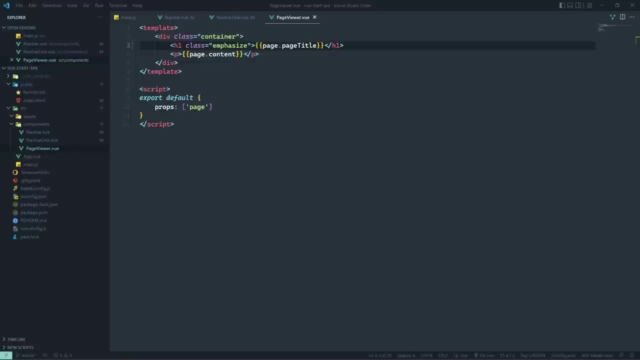 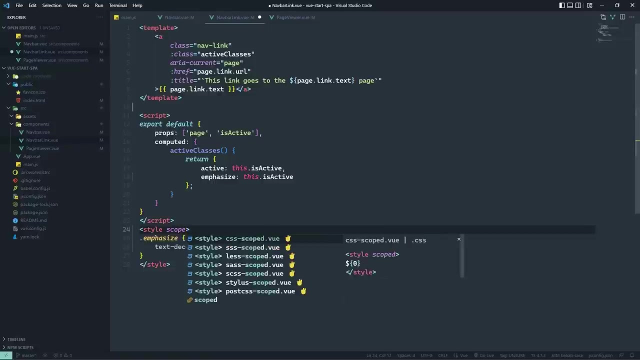 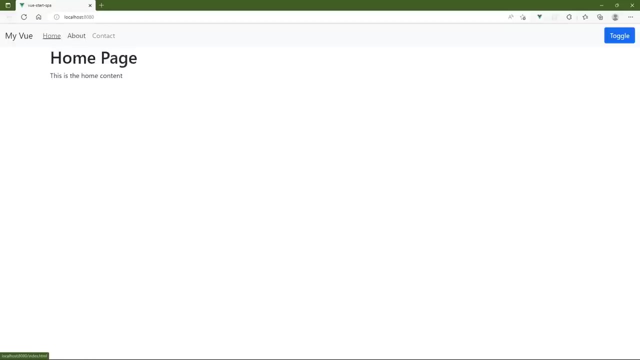 So we can define CSS inside of our components. But by default, they are not scoped, they are global. However, we can make them scoped to the component that they are defined in by adding a scoped attribute to the style element. All we have to say is style scoped. And now, whenever we go to the browser, we're going to see that the underline is still available for the navbar links. 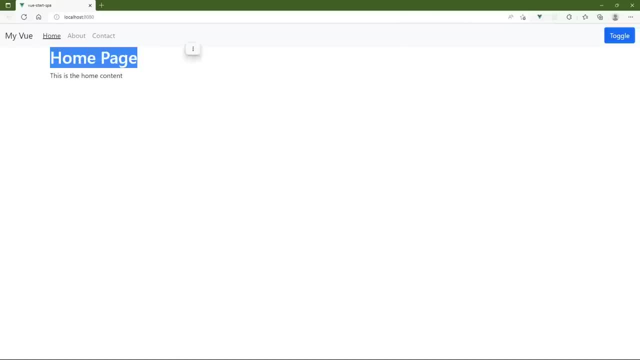 But notice that it is no longer available for our page viewer. And this means that we can go inside of page viewer if we wanna do. 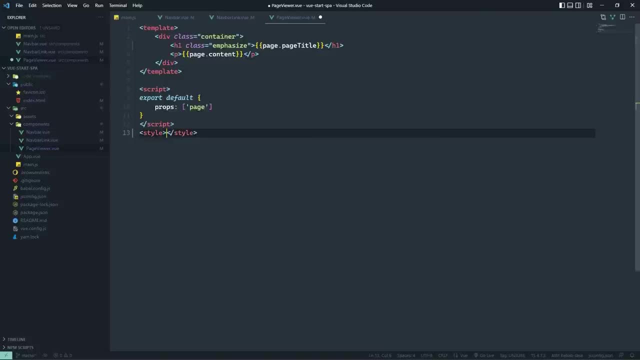 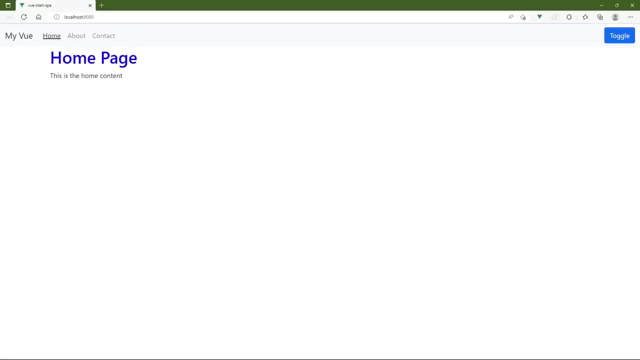 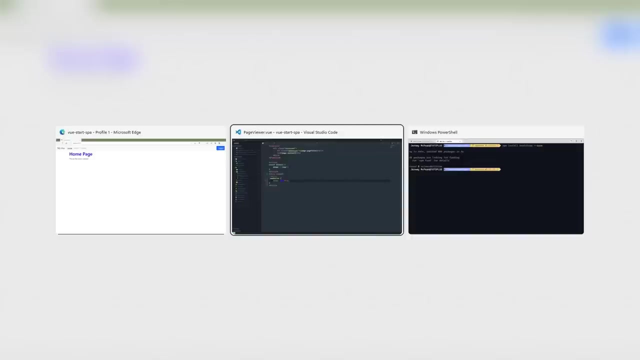 And we could define a completely separate emphasize class. But we would probably want to make this scoped as well. So let's add emphasize. And let's just make this color blue, something that's not an underline. And there we can see that our title is blue. Of course, whenever we go and look at the other pages, the title will be blue as well. So when it comes to adding CSS to our projects, we have several different options. 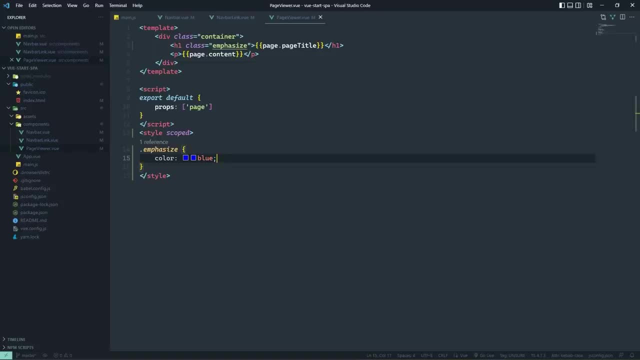 We can install them as a dependency for our project and import them just like we did with Bootstrap. 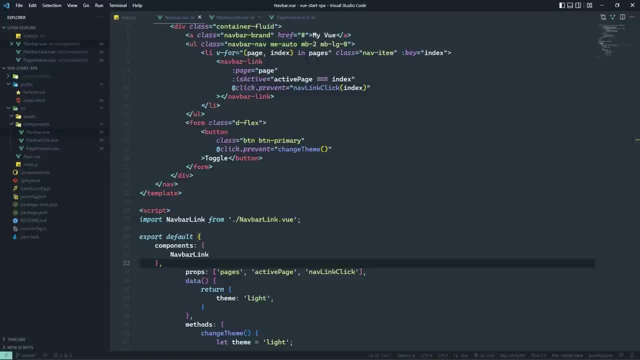 We can also define CSS for our components. We can make them global, or 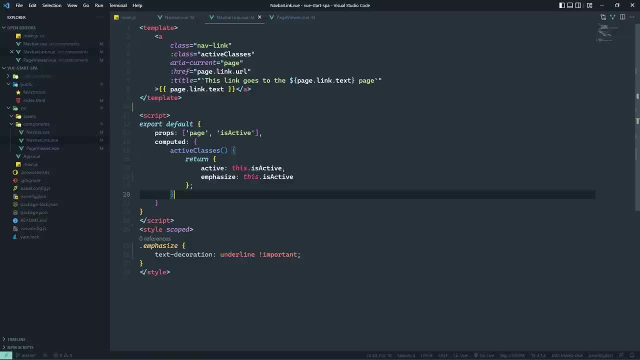 we can make them scoped to the component that they are defined in. 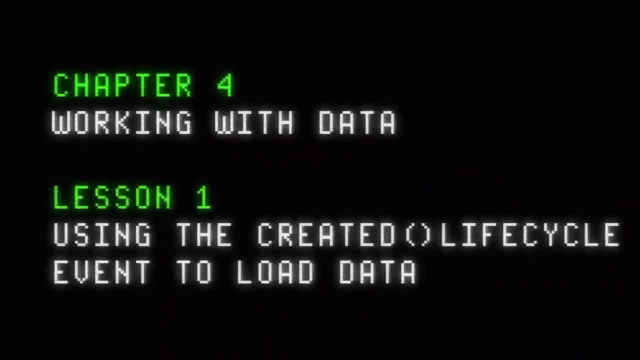 As software developers, our whole purpose is to build applications so that users can work with their data. And as web developers, our situation is a little unique, because we essentially have two applications. 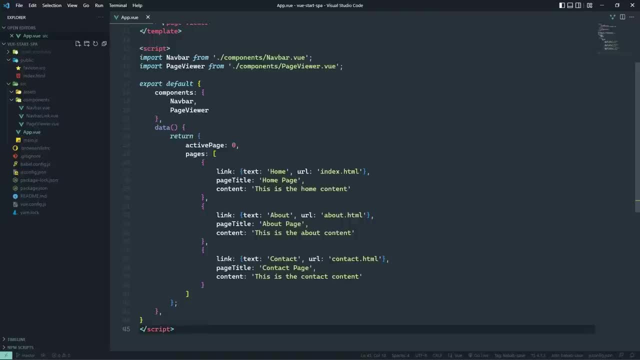 We have a server application that is responsible for processing all of the data and identity stuff. 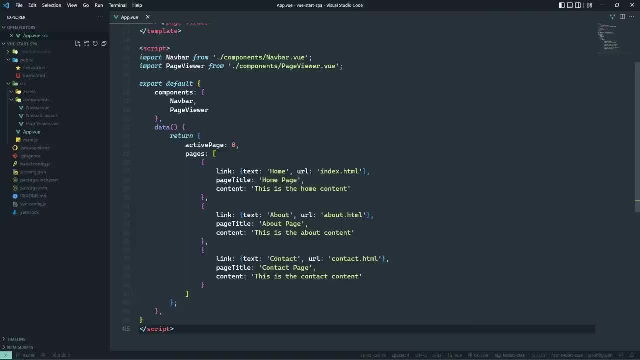 And then we have a client side application that is loaded into the browser. That's what the user interacts with in order to work with their data. 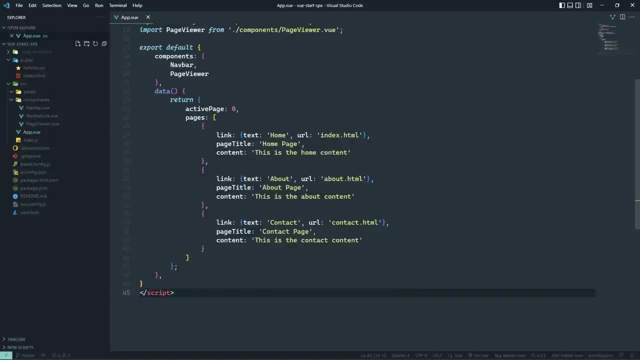 So you can make the argument that probably, the most important thing about our application is to load data so that the user can access it and work with that data. 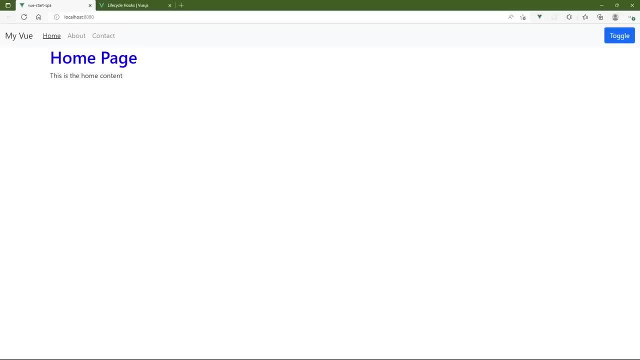 Now, the question becomes, how do we do that? Because it's not always just clear cut. 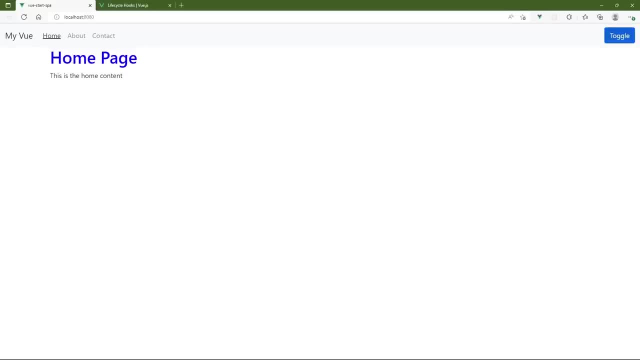 Like for example, if we had a button that the user could click on, and that would fetch data, that was the purpose of that button. 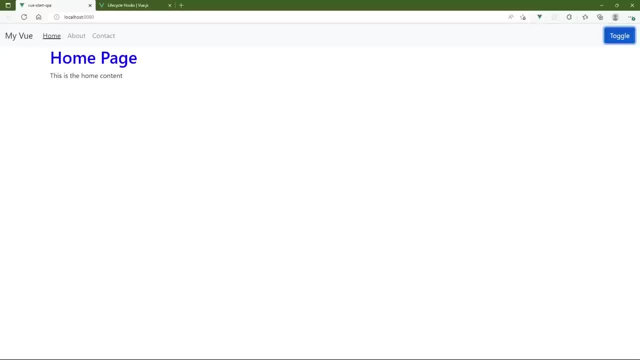 That's pretty clear as to when we would fetch that information from the server. However, what about the data that we need to access? 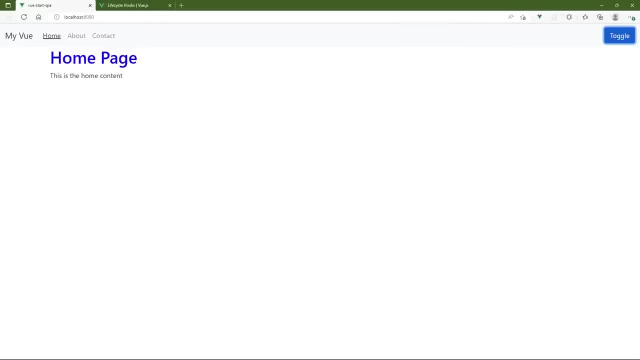 That's pretty clear as to when we would fetch that information from the server. However, what about the data that we need to access? That's pretty clear as to when we would fetch that information from the server. We need to initially load so that when the user first pulls up the application, 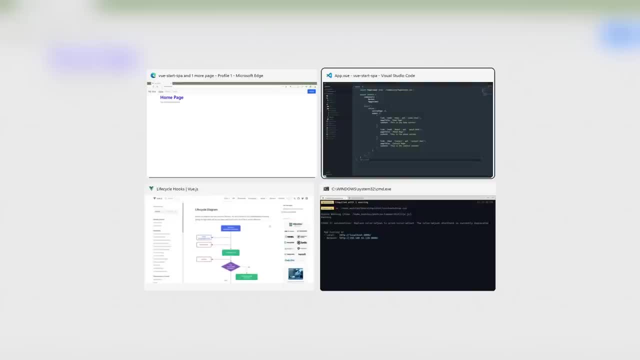 their data is right there ready for them. Because if we look at our application, we don't really have a clear-cut way as to load that information. 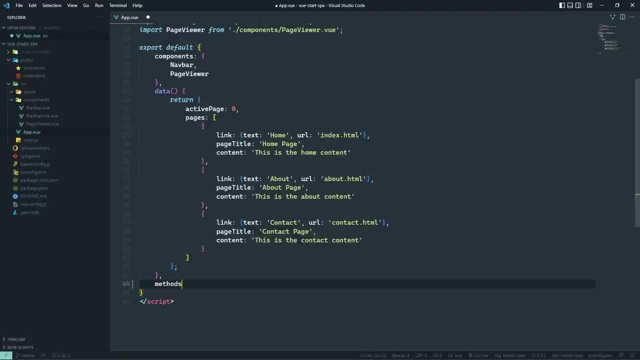 I mean, yes, one of the things we could do is add a method that we could call get pages. 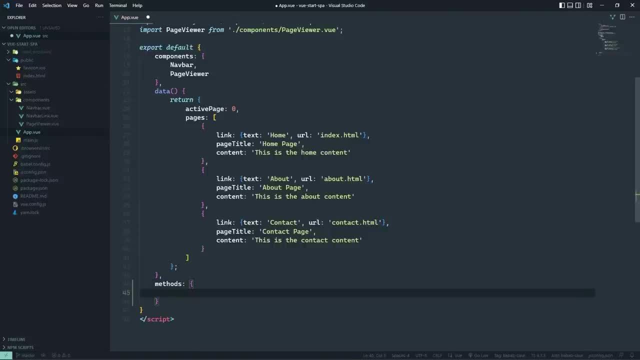 So for example, the pages are data that we would want to dynamically load. So we could have an asynchronous method that called get pages and this would be responsible for fetching that information from the server. 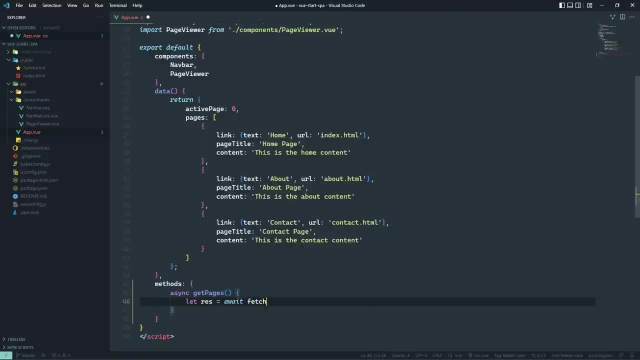 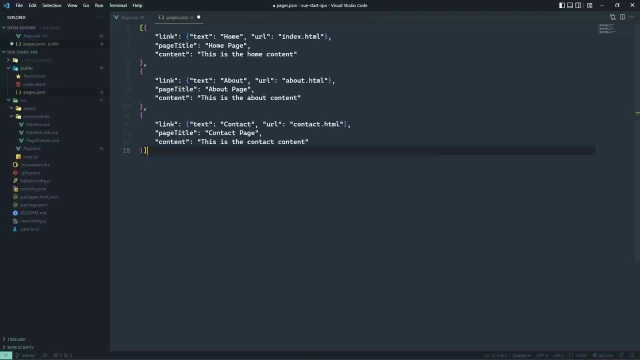 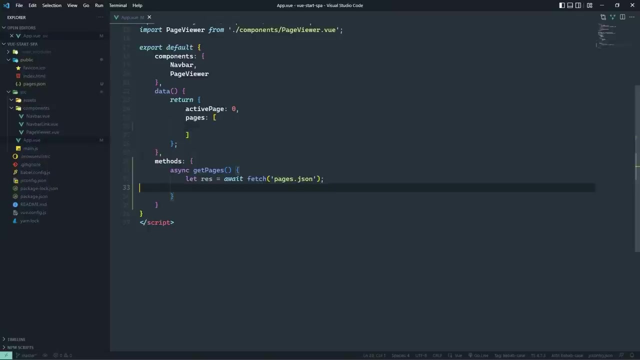 So we could go ahead and write that code to where we would fetch the pages.json and of course in a real application this would be hitting some end point on the server application. What I'm going to do is take out these page objects and inside of the public folder I'm going to create a new file called pages.json and I'm going to paste in the json structure that has the same information it's just formatted in json. So this is the file that we are going to fetch we of course need to parse that into a javascript object. So we can use the response objects json method and then we could return the data so that inside of data we would actually call the getpages.json. And then we could return the data so that inside of data we would actually call the getpages.json. 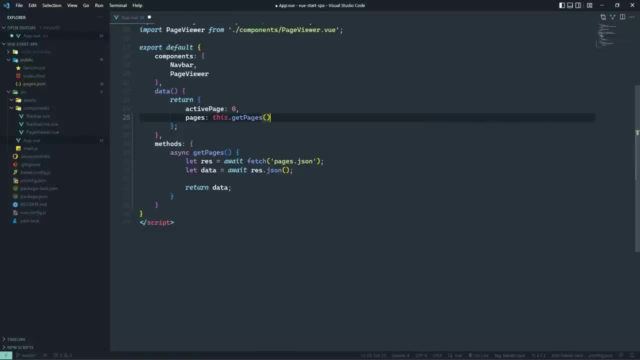 That's an option but that's a very poor option. So instead what we can do is take advantage of the 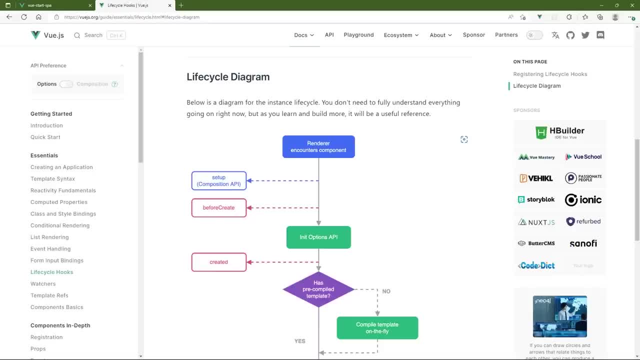 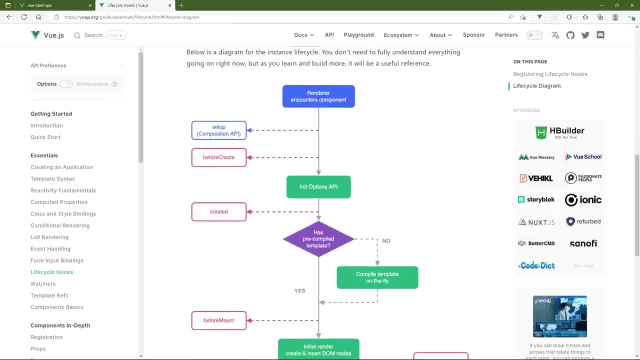 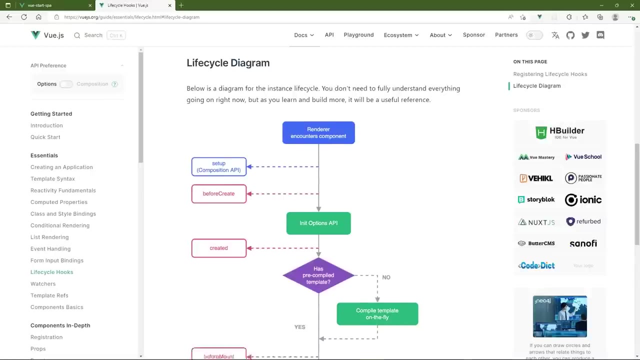 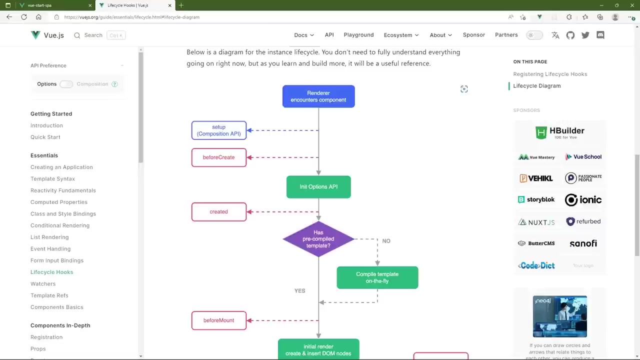 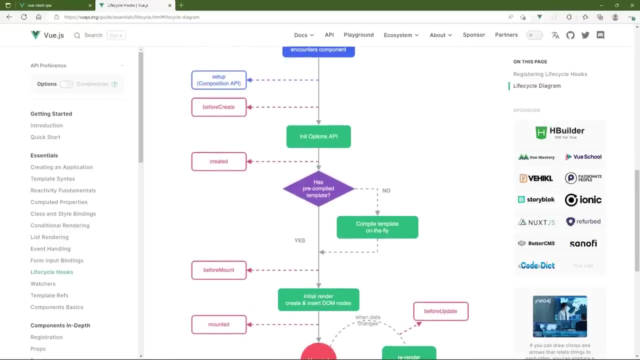 lifecycle events of a component. So in the view documentation there's this lifecycle diagram which may or may not be easy to read depending upon your understanding of the terminology and just your understanding of the lifecycle of a view component. But basically it starts at the top where the renderer encounters a component. So this is the view runtime, it encounters a component that it needs to load into the browser. So there's this beforeCreate event that's going to occur. And this is an event that we can hook into and execute code when the component instance is initialized. 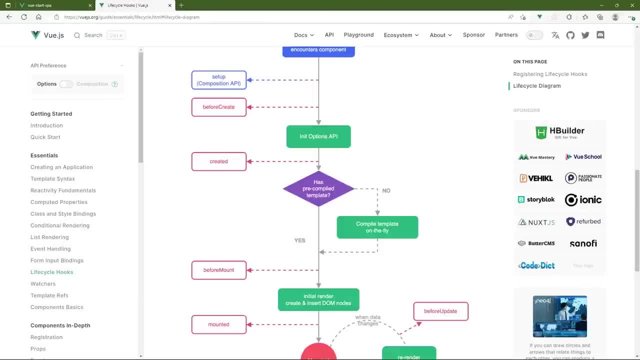 The props are resolved, but there's no processing as far as the component's data or computed properties. 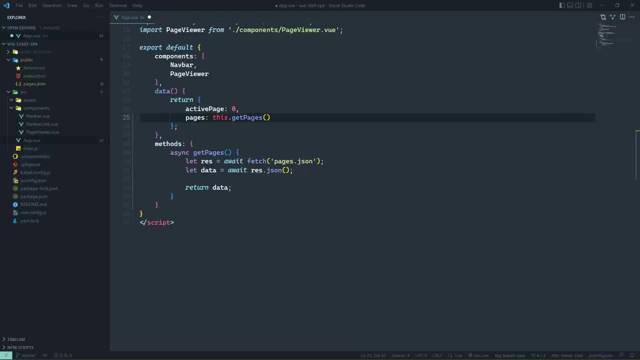 So in the terms of our needs, the beforeCreate isn't really something that we would want to use to load data. Primarily because we want the data to already be processed, as well as the computed values as well. So let's go back to the diagram. 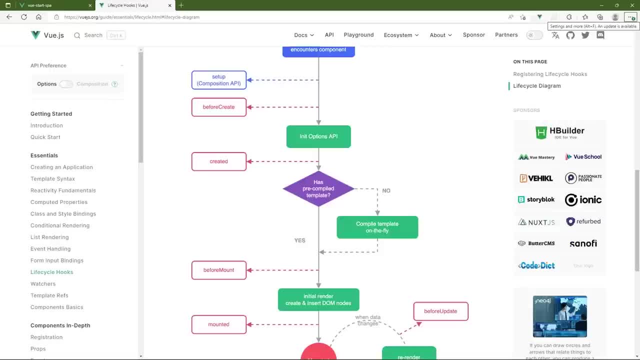 After beforeCreate, then there's the initialization of the options API. That is the API that we are using. 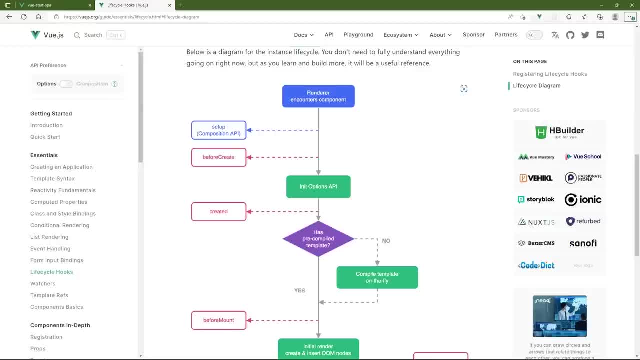 Up here at the top, you can see that there's this setup and then this composition API. 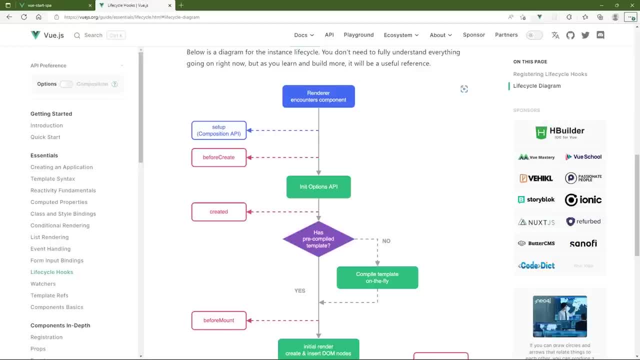 The composition API is the one that we're going to use to load the data. So the composition API is a different way of creating the same components that we 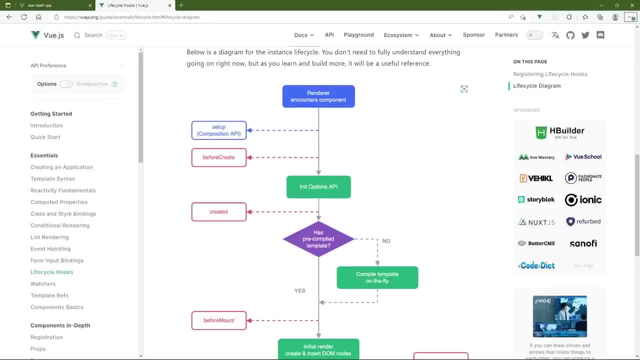 are working with, and we will look at the composition API. For now, we are working with the options API. 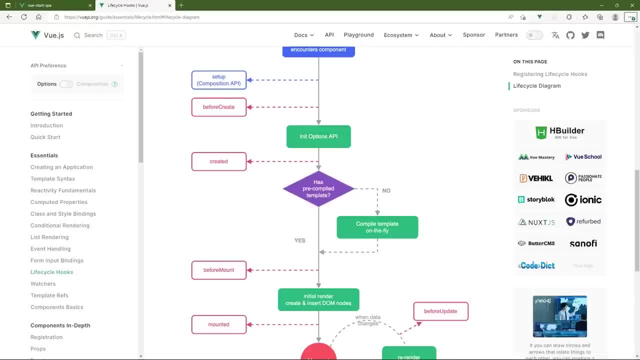 So after the options API is initialized, then there's this created event. This created event occurs after the data and the computed properties have been processed. 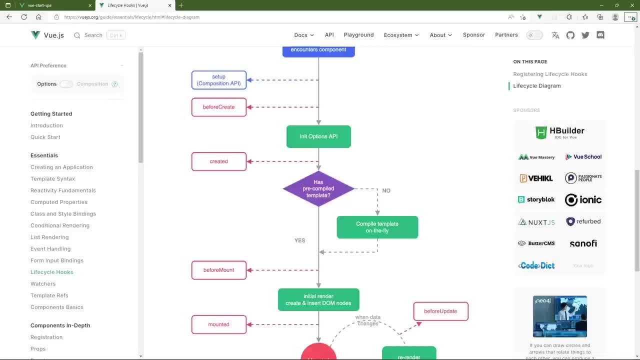 But before the component is loaded into the document in the browser. So this is ideally the place where we would want to load our content. Because this means that the data is processed, so that whenever we load our data, then Vue is going to be able to react to that change. 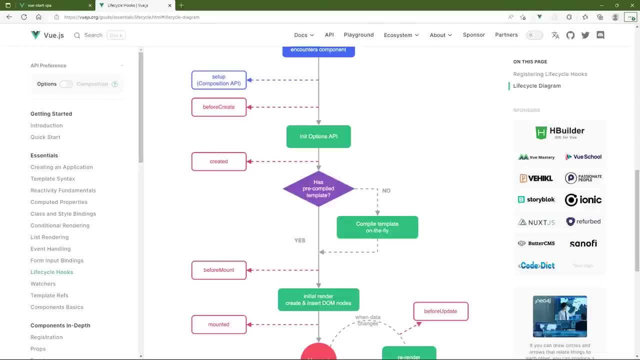 But it's before it is visible in the browser, which is very useful for the end user experience. 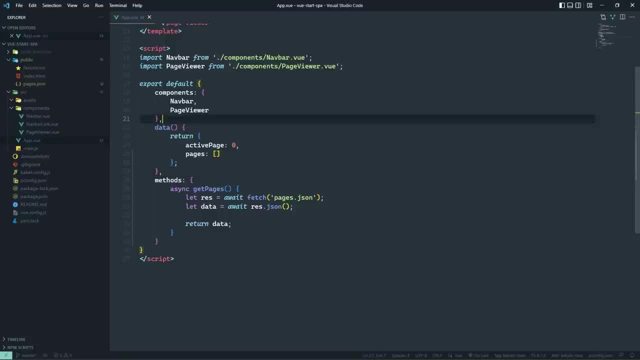 So we want to use this created event. And all we have to do is add created as a method to our options object. So this is just another option, just like if we wanted to use beforeCreate. 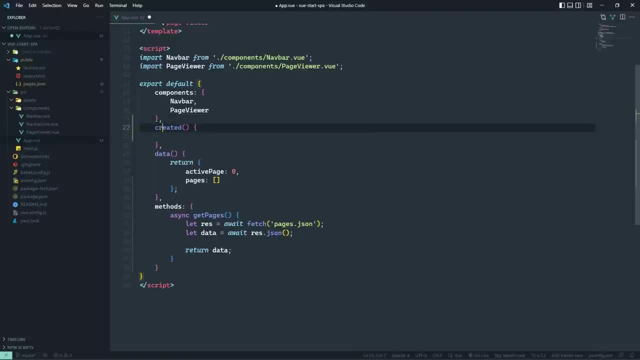 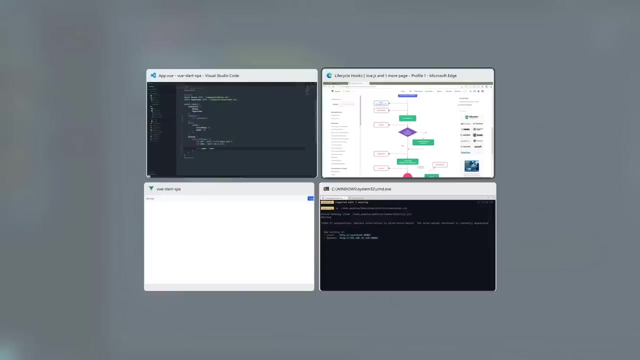 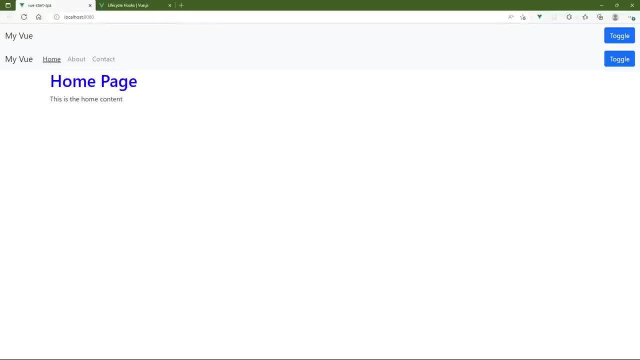 We would do the same thing. And then inside of this created method, we would call our getPages. Now, we could assign this to the pages in our data like that. Or what I would probably do is something like this. So that inside of getPages, we would go ahead and set pages equal to our data. So with that simple change, we can go to the browser. And we are going to see something that looks a little bit different. So weird, we have two nav bars. So let's look at the developer console, because we are going to run into an error here. 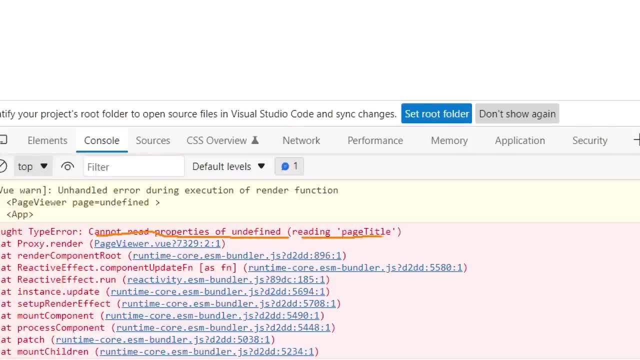 It says that it cannot read properties of undefined. It's trying to read page title, and it tells us where that is, pageViewer.vue. 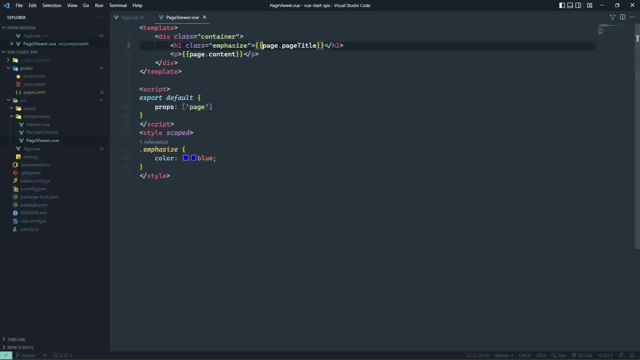 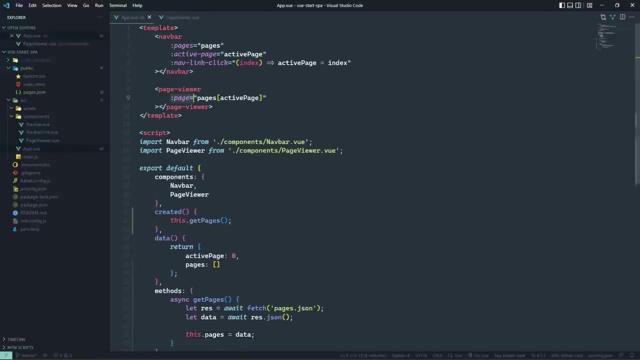 So let's open up page viewer, and let's see, it is right here on line three. It's trying to access this page title property, but it doesn't exist. And the only reason why that wouldn't exist is because this page object is null or undefined. And the only reason why that would be null or undefined is because the page that was passed as the page prop is null or undefined. So basically, it's this pages. 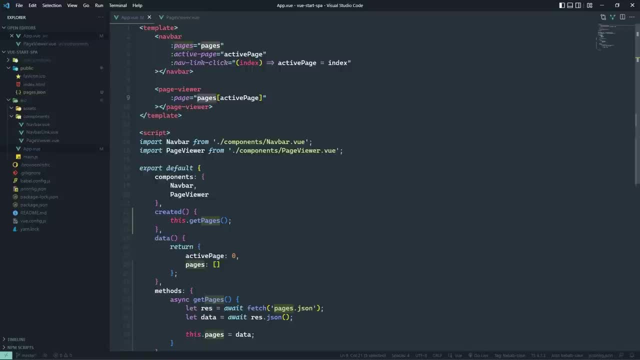 Before our data has been loaded, pages is an empty array. So undefined is being bound to the page prop for the page viewer, and we're running into that error. 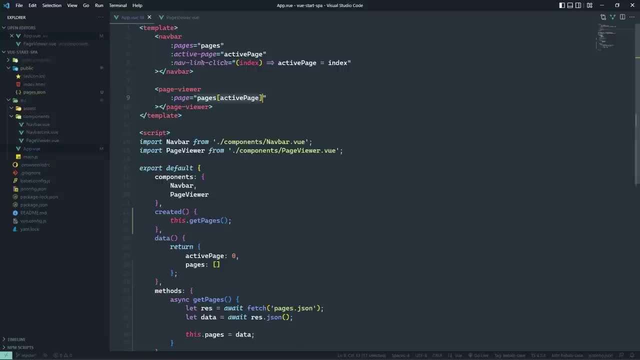 So then the question becomes, how do we address this? And there are a variety of different ways, which is what we are going to look at in the next lesson. 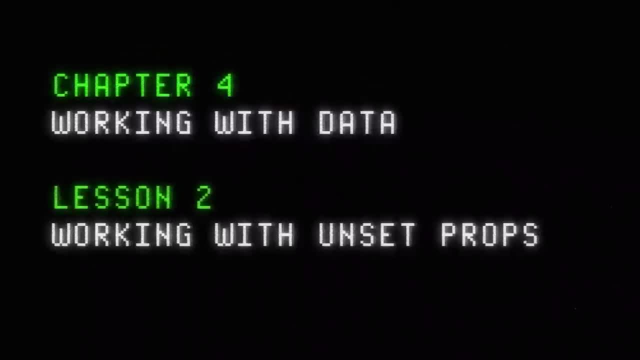 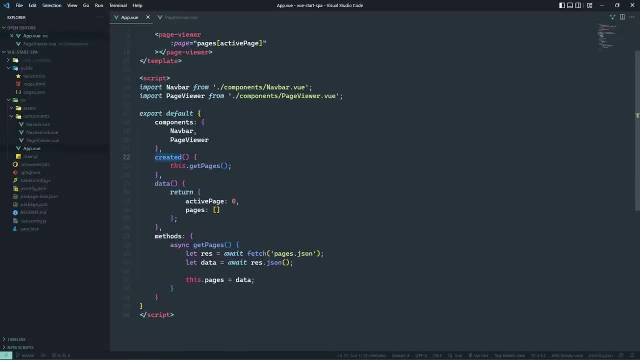 In the previous lesson, we loaded data into our application by making an HTTP request from inside of the created hook. So we retrieved that information, we parsed it into a JavaScript array, and then we stored that array in the pages data property. 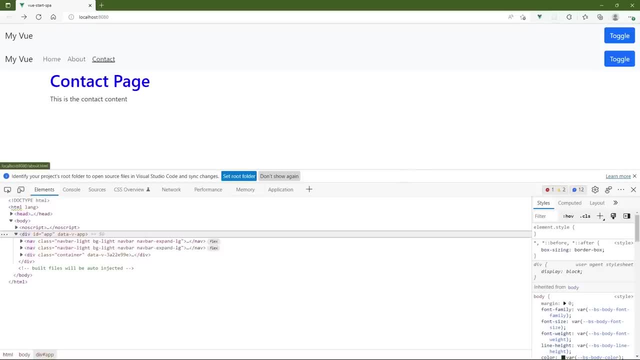 However, whenever we view this in the browser, it still kinda works, but it looks really weird. 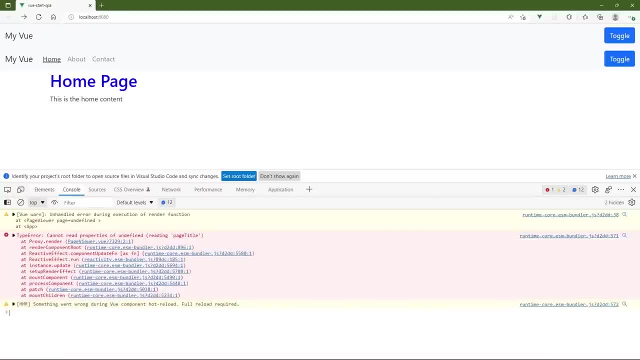 Because we have to do a lot of work. We have two nav bars, and if we look at the console, we have an error. 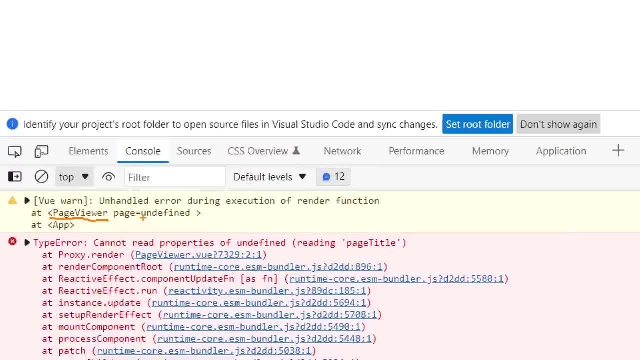 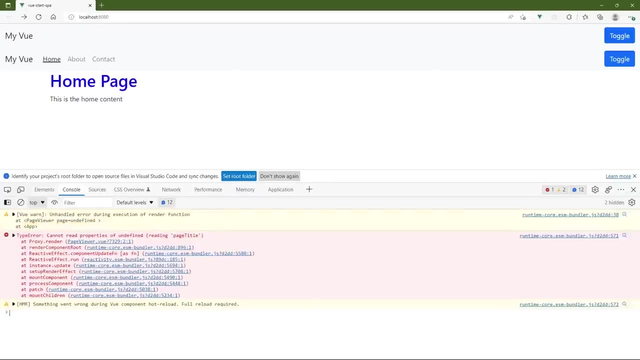 And it's because of this right here, the page viewer component is getting the value of undefined passed for the page prop. And the actual error is that it's trying to use the page title property on undefined. Well, of course, undefined doesn't have any property. So that is, of course, going to fail. 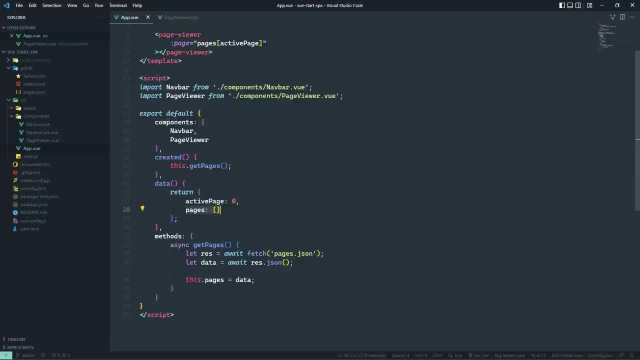 And the reason why we are seeing this is because pages is initialized as an empty array. 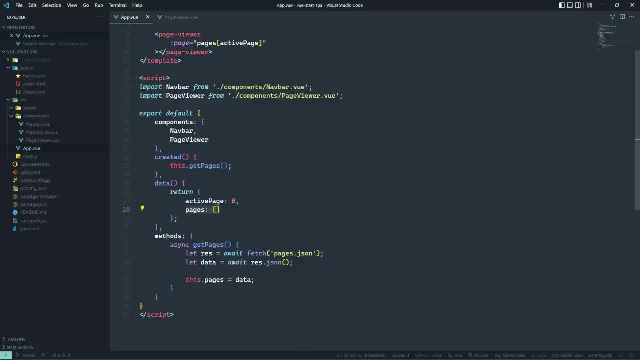 And it's not populated until the component is initialized, the data is processed, and then the created hook executes. So there's this tiny little brief moment where pages is empty. 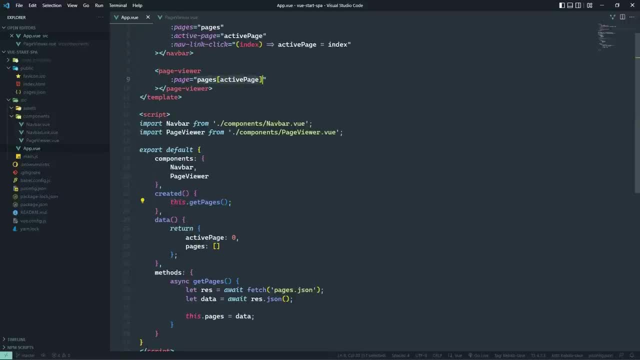 And the page viewer is trying to retrieve the element at index 0 from an empty array, which of course, that's impossible, so undefined is passed to the page viewer. 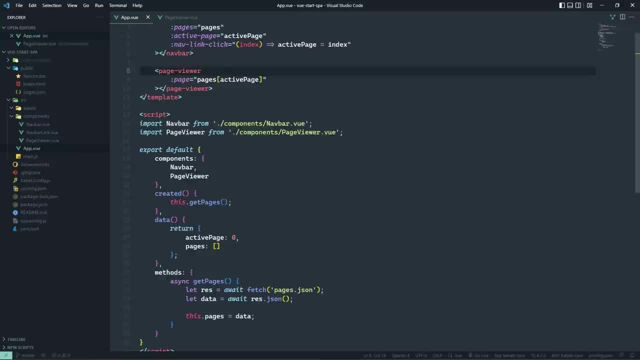 So there's a couple of different ways that we can get around this, this particular error. 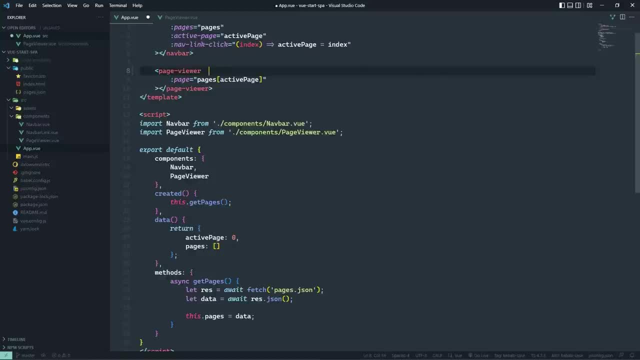 And probably the most straightforward is to do something like we would do in just normal JavaScript. And that is to check if we have any elements inside of the pages array. We can do that using a directive called the if. This is very much like the if statement in JavaScript, and we can use it on any element. It doesn't have to be an HTML element or a component. As long as we use it and we provide a truthy or falsy value, it's going to work just fine. 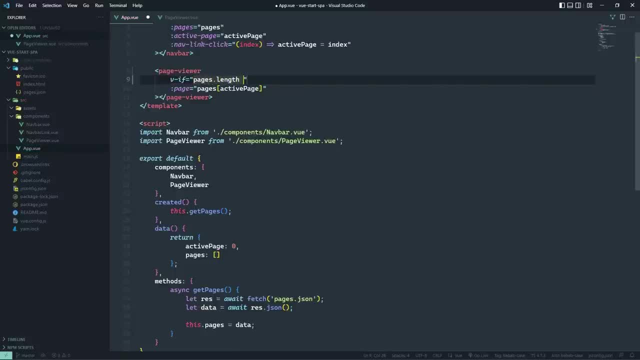 So here, we want to see if we can get the element to be true or false. We want to check if the length of pages is greater than 0. 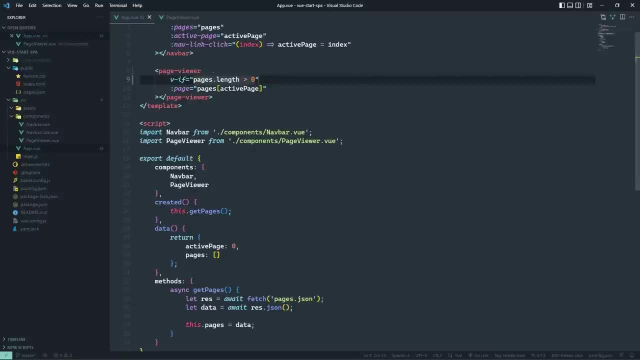 And this is going to do one of two things. If the value of the if directive is true, then page viewer is going to be output into the document. 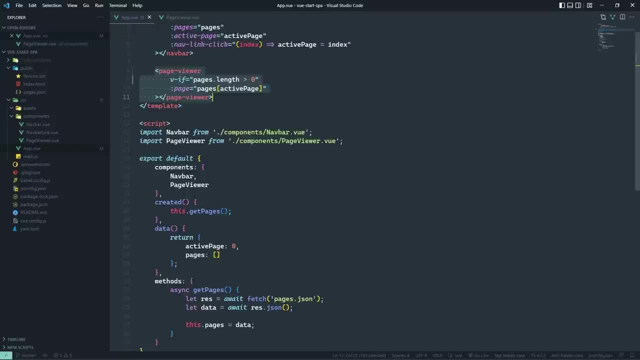 If it is false, then it is not going to be in the document at all. 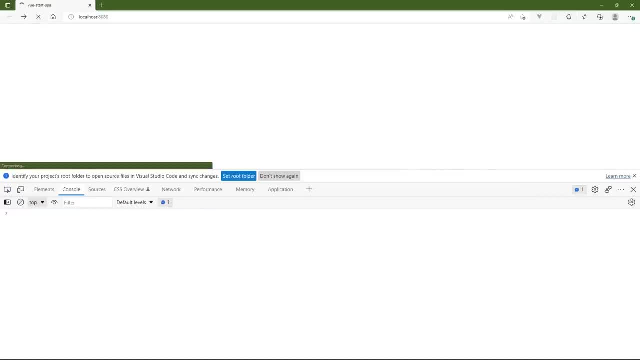 So let's take a look at this. Let's refresh just to load everything from scratch. Notice that we now don't have two nav bars, and we don't have any errors inside of the console. 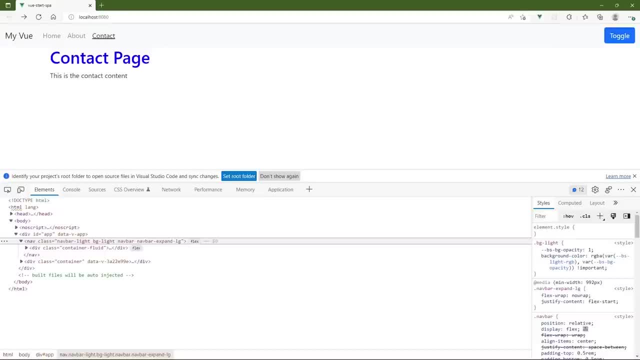 And everything works like it should. If we take a look at the elements, we can see, of course, we have our nav bar. 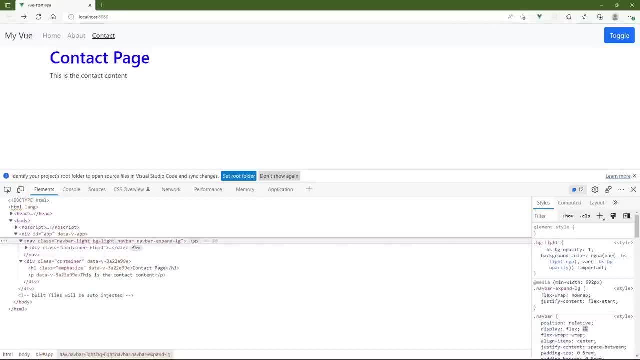 We also have the div element that contains the page information. But let's do this. 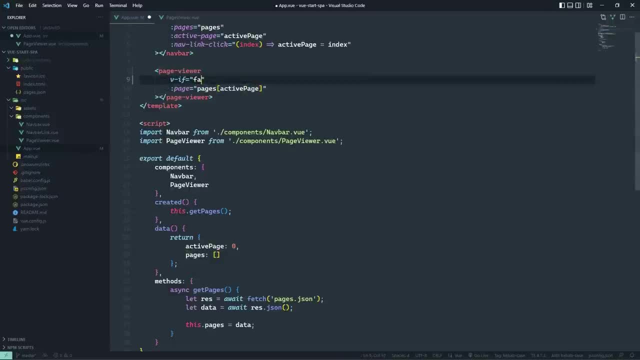 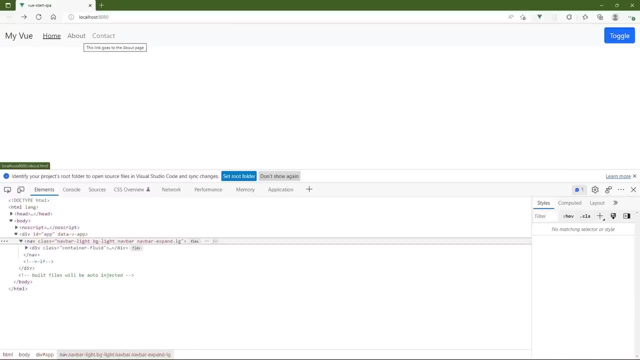 Let's set the value of false for the page viewer. Let's go back to the browser, and let's refresh the page. We are still going to see our nav bar, because what we just did does not affect the nav bar at all. 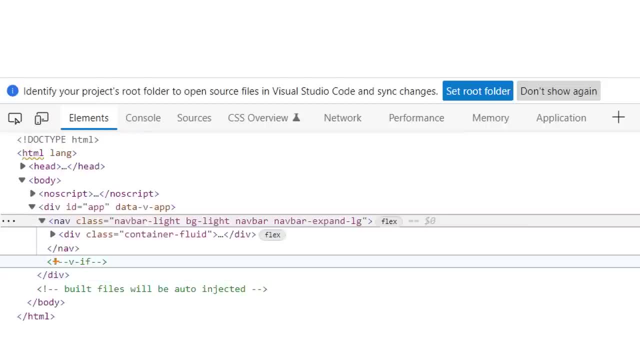 However, we don't see the page content, and if we look in the elements, we see that, we see that the page content is false. 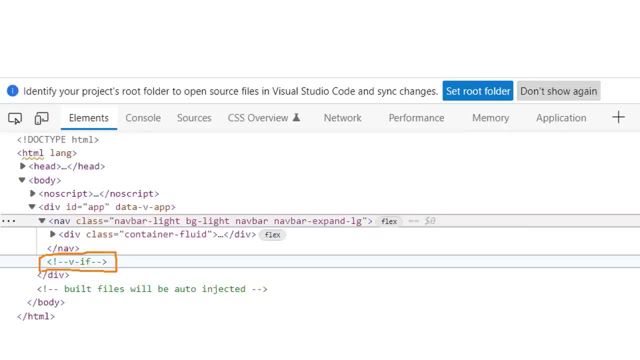 Notice this vif HTML comment where that div element would be. 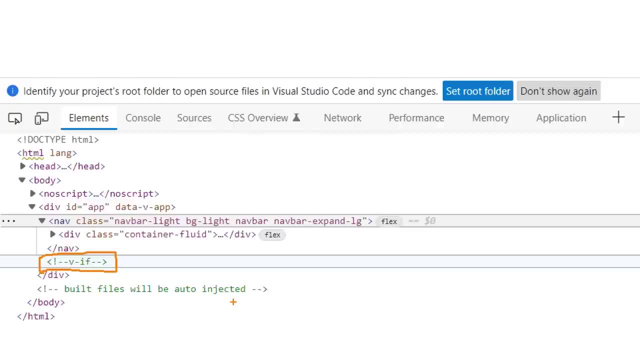 So that div element is not in the document at all. It is completely gone. 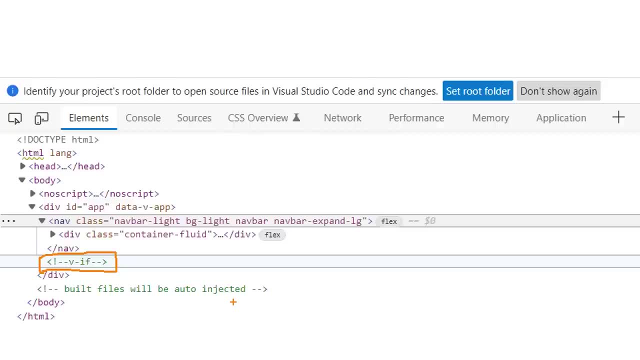 And it will stay gone until the value of that vif directive is true. 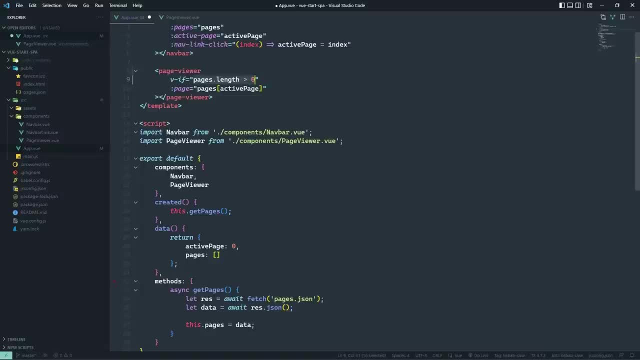 So this approach is very much like what we would do in just typical JavaScript. If the length of pages is greater than zero, then display the page. If it's not, then hide it. 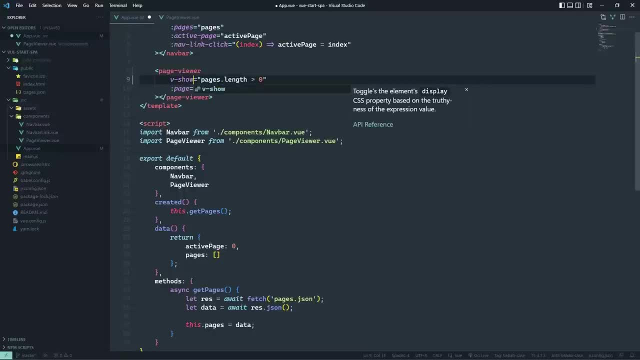 Now, there's a similar directive called vif. And it's purpose is to show or hide content, but it does so in a different way. 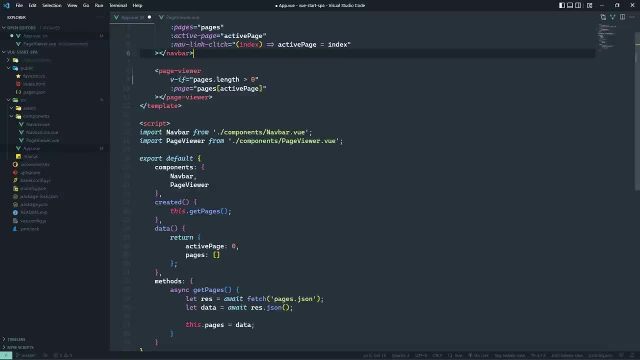 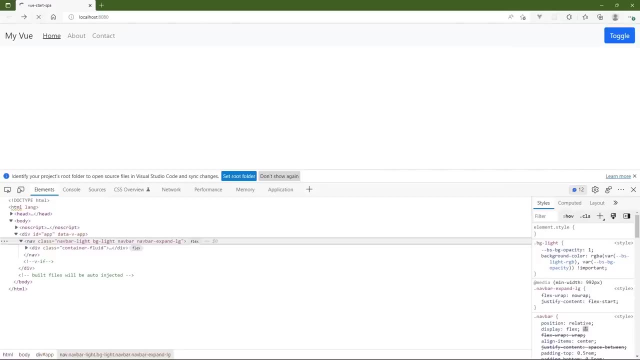 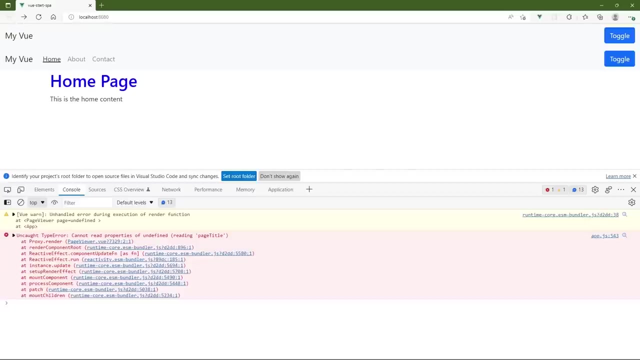 Instead, it uses CSS to show and hide the element. So if we use vshow here, we are still going to run into an issue. Because from the standpoint of the page viewer, it is still in the document, even though it would be hidden with CSS. Whereas with vif, it wouldn't be there at all to generate. An error. So let's take a look at what vshow would do. 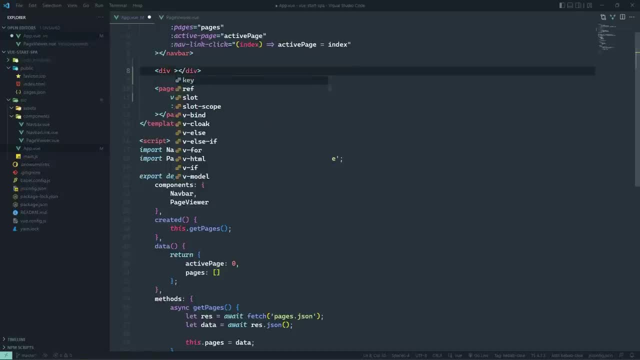 So let's create a div element. We don't need any classes or anything like that. 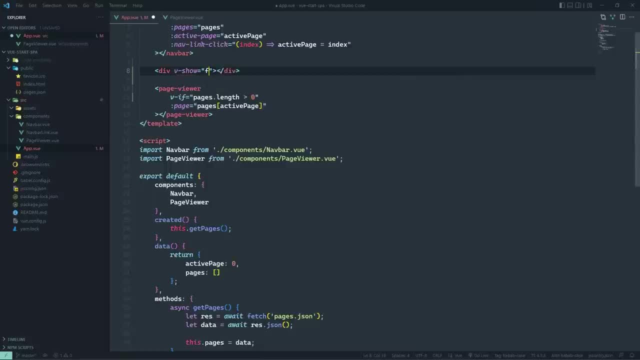 Let's just have vshow. And let's set this to false, so that we will hide this content. 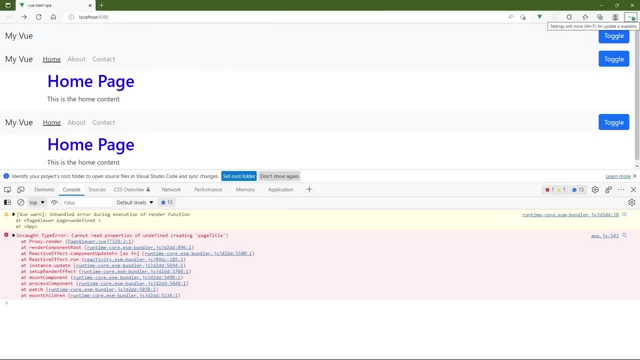 So of course, we're not going to see this rendered within the browser. However, whenever we look at the elements, we will still see that element is there. It's just that its display has been set to none. 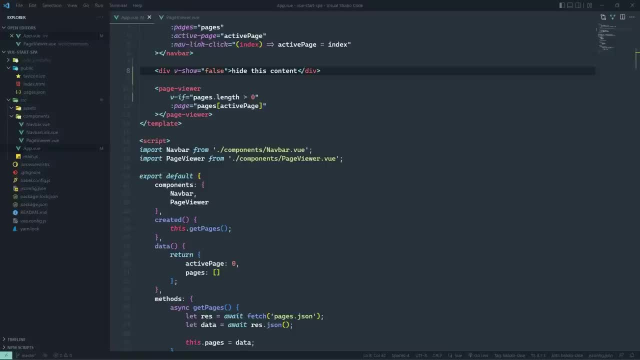 So you can show and hide content with two directives, vshow uses CSS to hide the content. 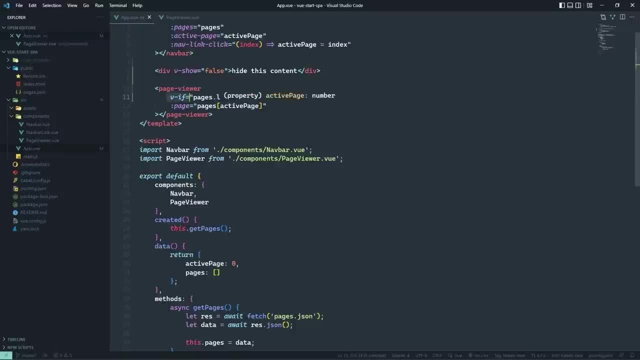 The vif directive does not output that element at all if it is false. So that is the first way that we can solve this particular problem. 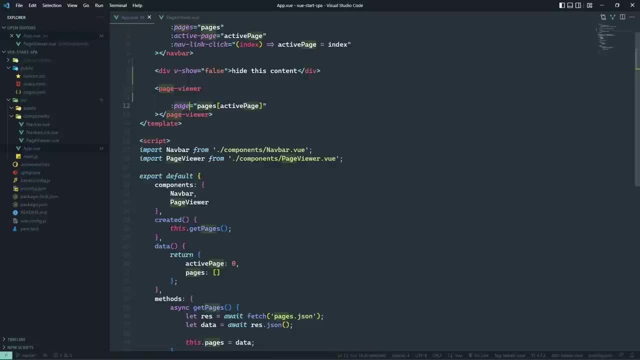 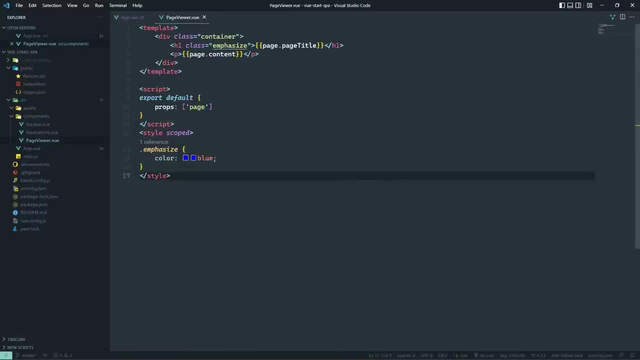 The second way would be to provide a default value for the page prop. And we would do that inside of the page viewer component. Now, this approach can be a little tedious because it changes the way that we define the props for our component. Instead of using an array of just simple string values, we would use an object where the property names are the names of our props. And then there would be a descriptor object that would be used to validate that prop as well as provide default values. So the first descriptor would be the type. So this is an object. 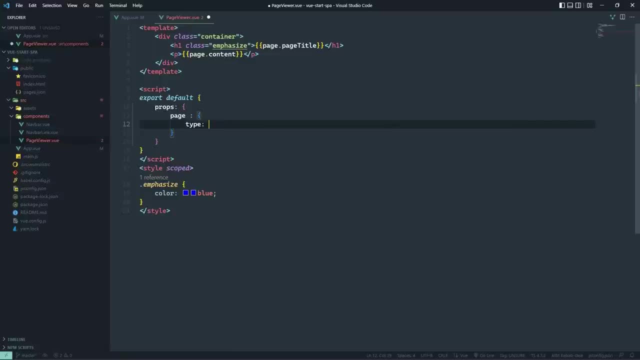 If it was just a simple string, we can use string or number or whatever. But this is an object. 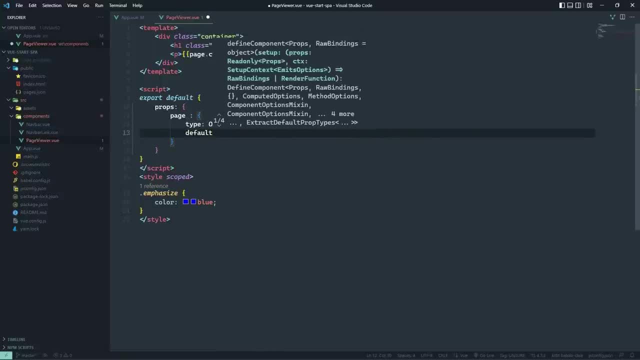 And since this is an object, we can provide a default value for it. We don't need a default value, but we have to write it as a factory function. If this was a simple value, like a string, then all we would need to do is provide the string value. But since this is an object, we have to write this as a function to where we receive the raw props. 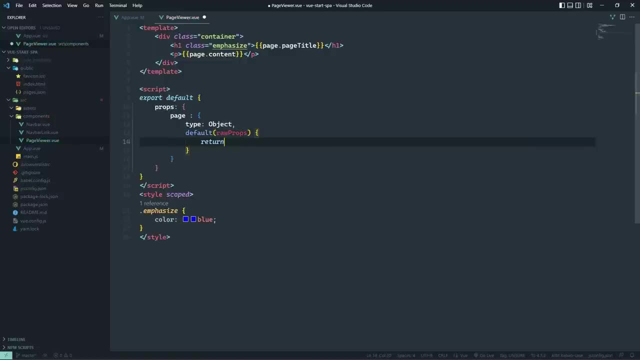 But in this particular case, we don't really need any of that information. We just need to return an object that has a page title property. 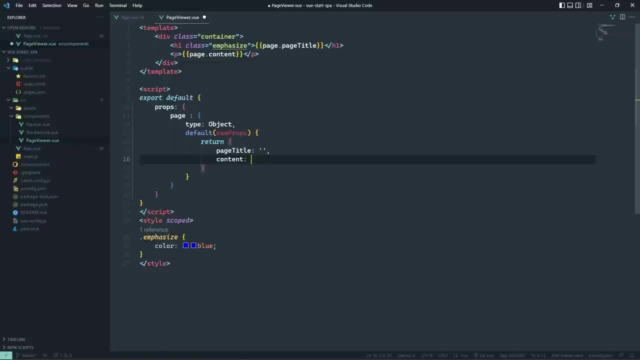 We can initialize that as an empty string. And then we can also provide an object that has a page title property. And then we can also provide the content, which would be an empty string as well. 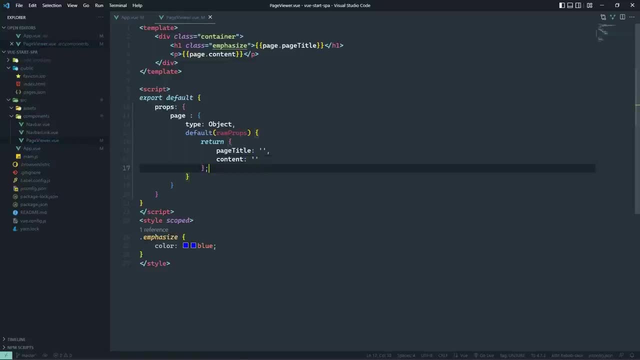 So you can imagine if you have a component that has a lot of different props. If you decide to use an object to define your props, you're going to have to essentially describe them. So at the very least, you would have to have an object for each prop and have the type for each of those props. 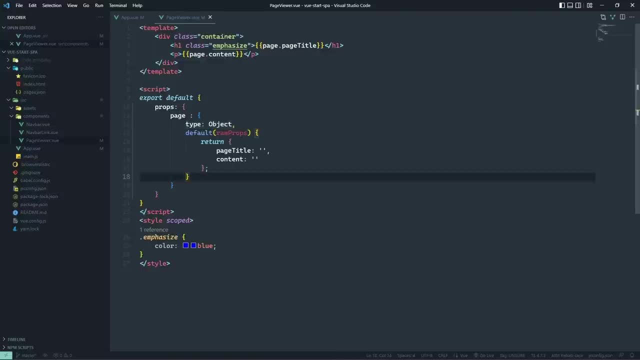 But this is going to fix our problem as well because we have now provided a default value for our page. 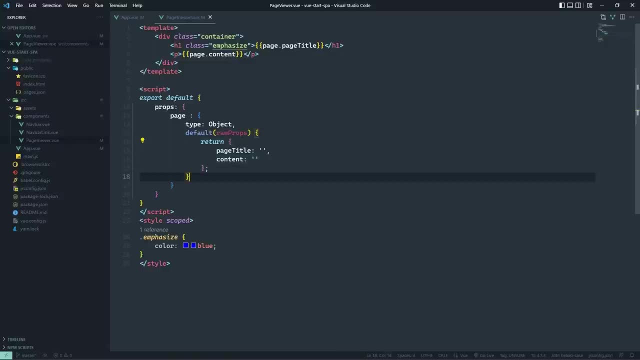 So if undefined is passed, this default value will be supplied to where page title will be an empty string. 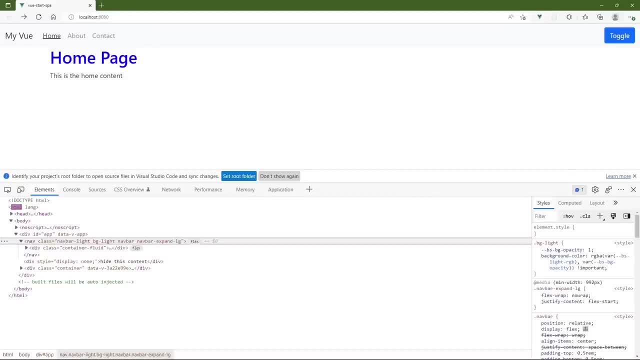 So let's refresh to start from scratch. And once again, we see the behavior that we would expect, and the application works just fine. 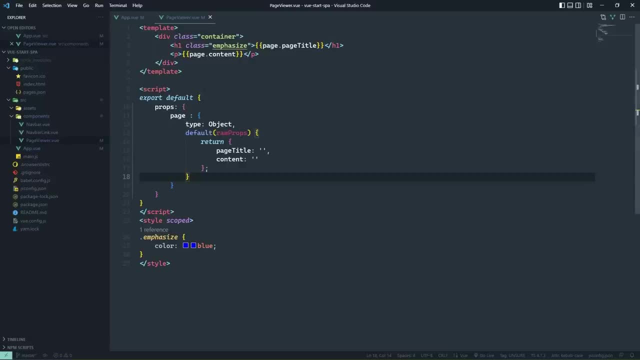 Now, there's no right or wrong approach to this, but they do serve different purposes. If you choose to define the descriptors for your props, this is primarily for prop validation, just so that you would get better error reporting as you're developing your application. 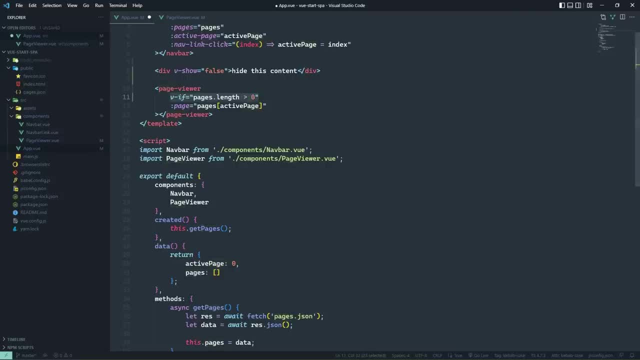 Whereas using the VIF directive would be the more straightforward and simple approach. 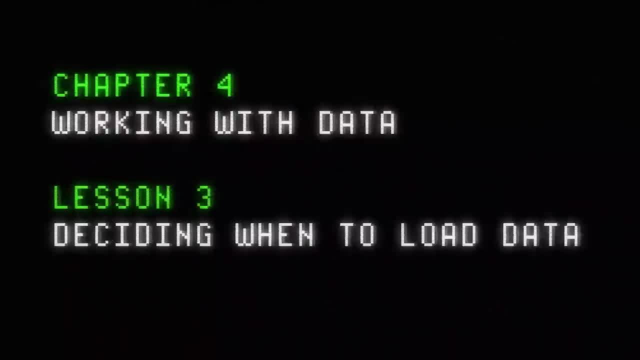 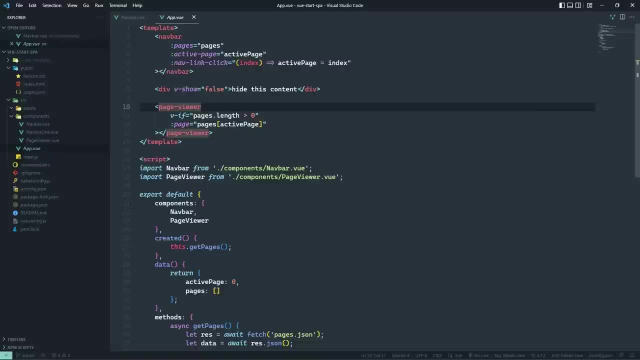 Either way, it gets the job done. When you start incorporating data in your applications, especially loading data, it can be confusing as to when you should load data. And unfortunately, there are no hard and 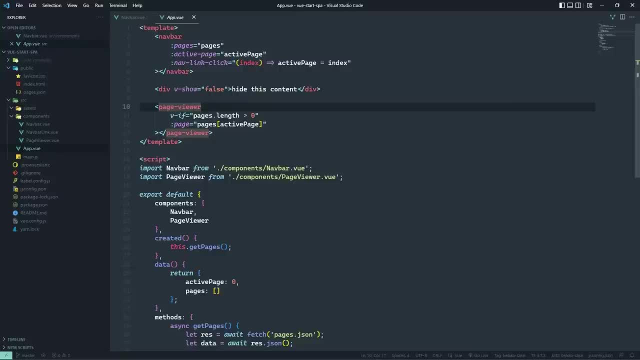 fast rules that say that you should load this data when. It is completely subjective. It depends upon your application. 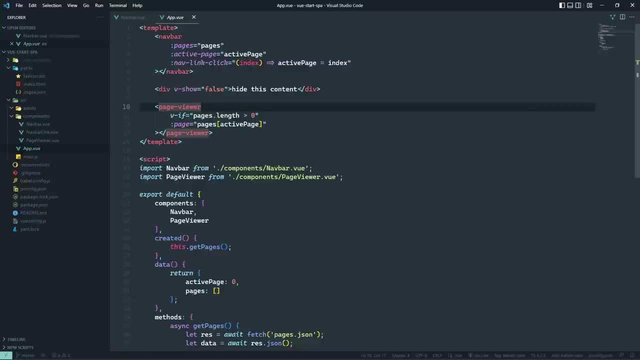 It also depends upon your opinion of when your application needs to load that data. 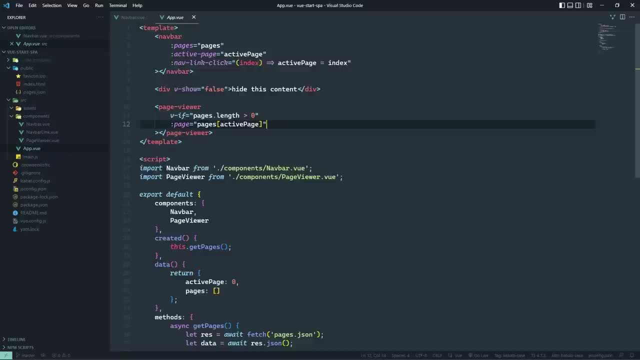 But what I typically do is boil it down to two criteria. Is the data used across multiple components, or is the data specific to a single component? 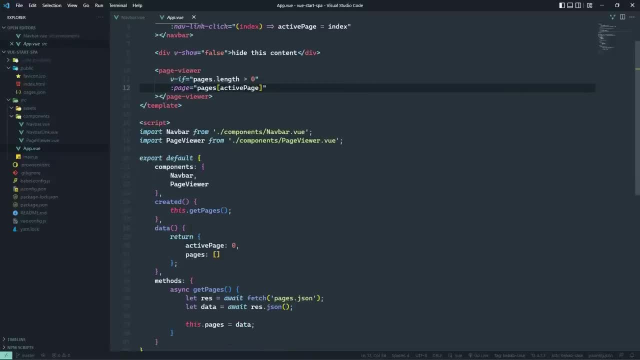 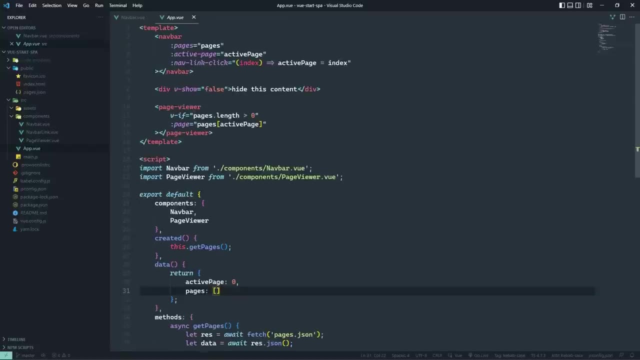 So let's look at an example of both of those. Now, we have the pages array inside of the app component. And of course, this is the pages that our application is using to generate and generate the links in the nav bar. The pages array is also used to display the content of the current page. 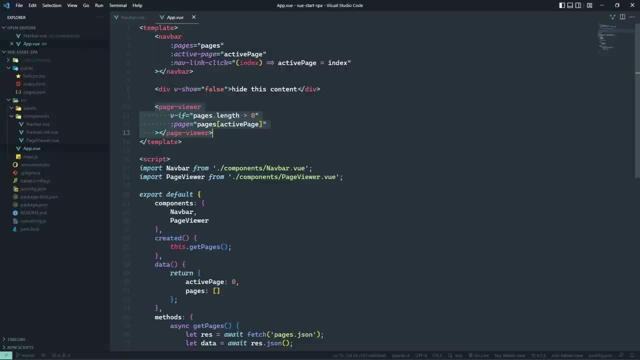 So while the page viewer doesn't necessarily use the pages array inside of the component, it is dependent upon the pages array. 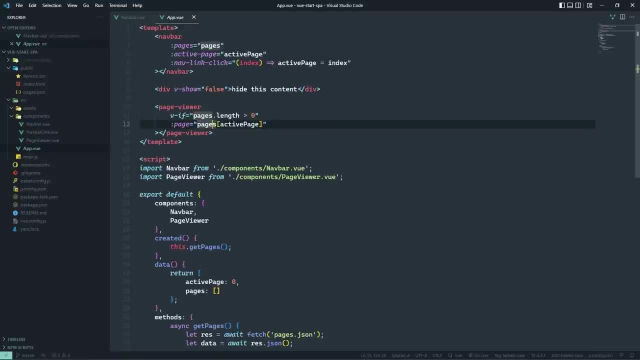 So since this data is used across multiple components, I want to load this as soon as possible, or at least before those components are created and loaded. 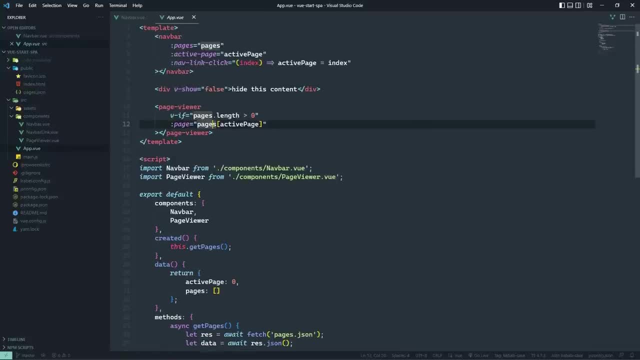 In our case, it made sense to load the pages inside of the app component using the created hook, so that's great. 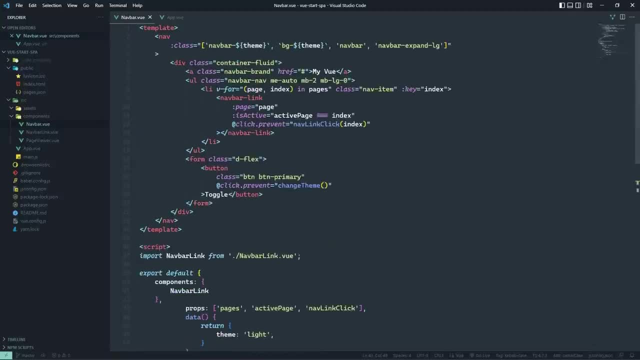 But let's take a look at the nav bar, because the nav bar has data. Now, of course, it has data being supplied through the props, such as pages. 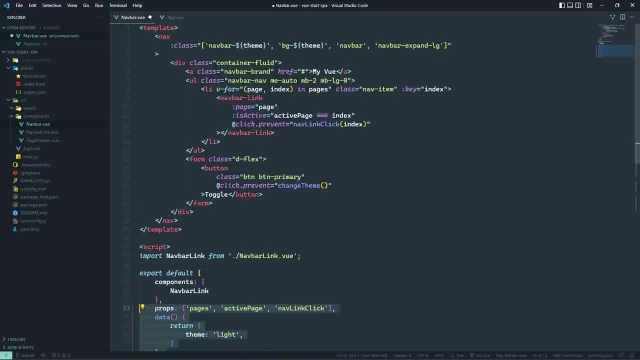 But there is data that is specific to this component and only this component. 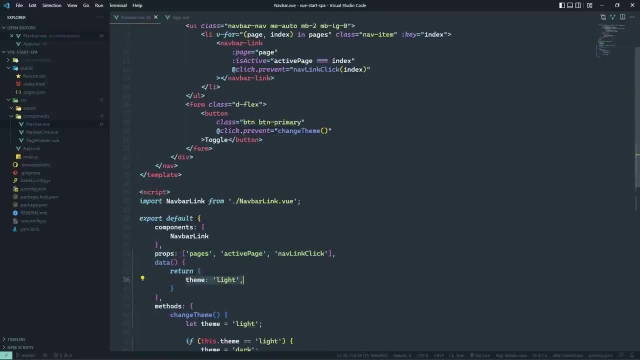 And it's this, the theme. Now, in the grand scheme of things, this data isn't as important as the pages. Because without the pages, the application doesn't work at all. 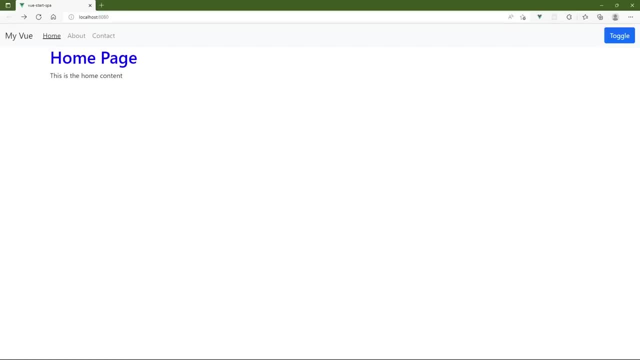 But this is part of providing the user's experience. We give them the ability to change the theme of the nav bar. So it kind of makes sense to go ahead and store that information, so that whenever they revisit our application, we can load the settings that they prefer. 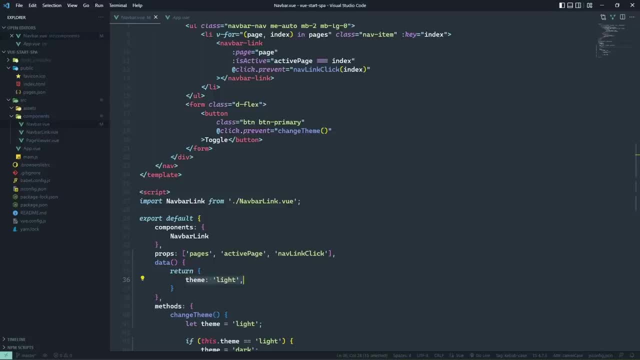 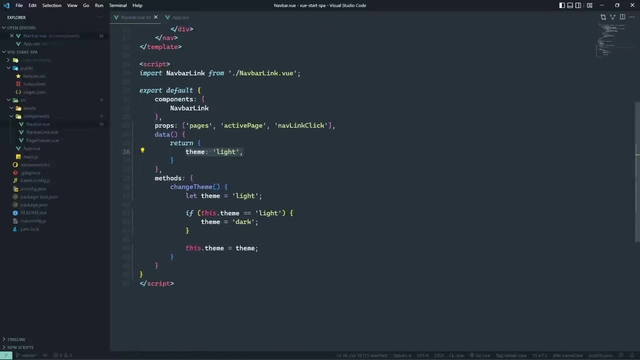 Now, you could make the argument that settings are also an application level component, because when you start talking about settings, there are components that would have different settings and it can make sense to load all of that information upfront. However, you can also make the argument that it should be loaded by whatever component is going to be using that setting. And that's what we are going to look at in this lesson. 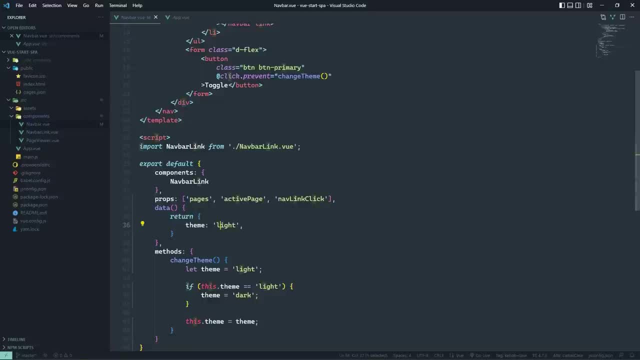 So, when it comes to storing and retrieving the theme information, we can approach this in a variety of different ways. 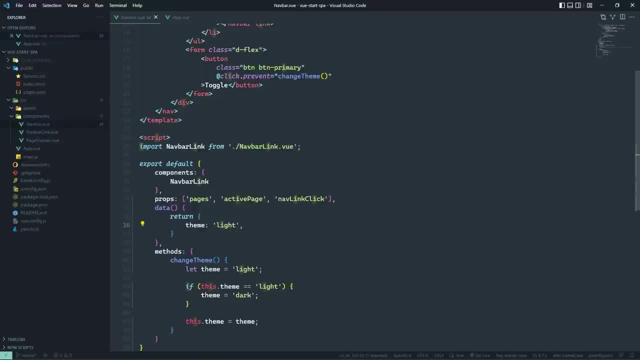 And there's no right or wrong way. I'm going to take the most straightforward way in this lesson, and later on, we will, 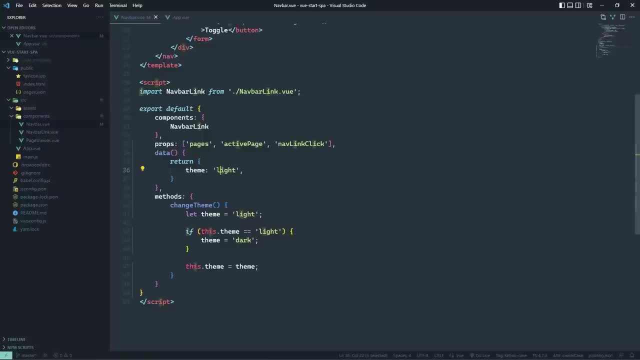 probably readjust it so that you can get an idea of another way that we can approach it. So for this lesson, we're just going to add two methods. One that is going to store the theme setting, in which case what we'll do is take whatever is inside of the theme data property and store it in local storage. Now we need to decide upon what key we are going to use, and I think theme is going to be just fine, so that we will set an item in local storage. 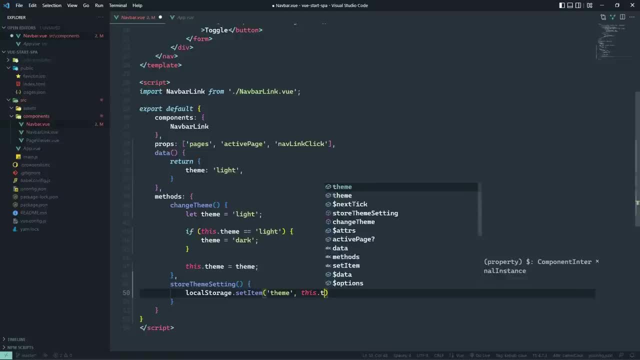 The key is theme, and the data will be whatever is inside of the theme data property. 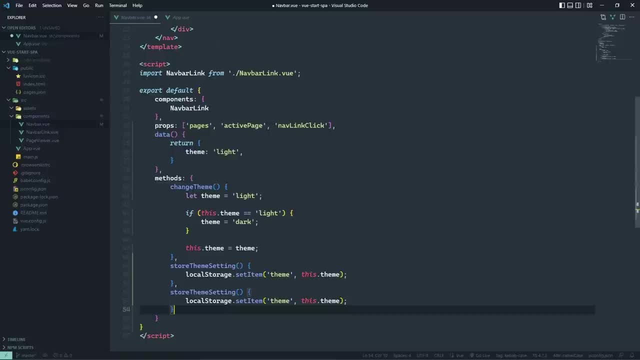 Let's copy this, because this is gonna be the basis for getThemeSetting. In which case, we want to retrieve the theme in local storage. So we will call the getItem method with the theme key. Now, it is possible, that this item doesn't exist in local storage. The first time the application is loaded into the browser, it definitely won't be there. So we do need to check if we have a value. If we do, then we can go ahead and we can set the theme equal to whatever is in the local storage. 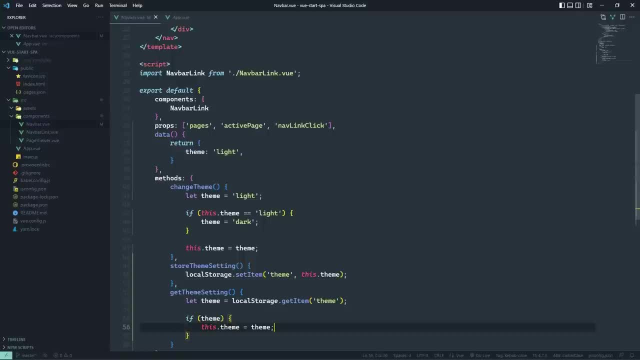 Otherwise, we'll just leave theme as the default, which is light. 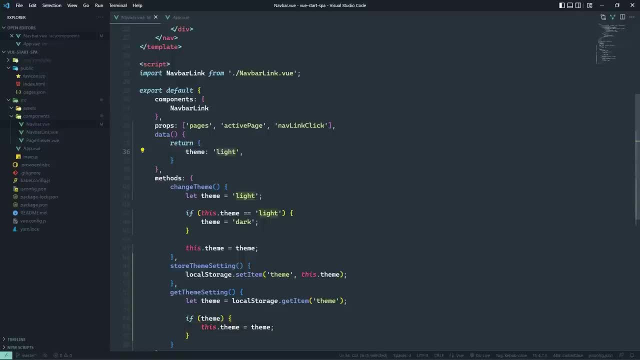 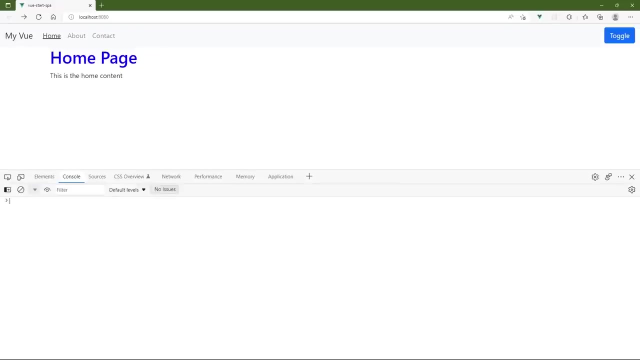 And so then we just need to decide when we use these methods. So we need to store the theme setting whenever we change the theme, so that makes sense to call it after we set the theme. And then we can call the getThemeSetting inside of the created hook. So let's go ahead and let's create that method. We will call the getThemeSetting, and that should be fine. So let's go to the browser. Let's pull up the developer tools, so that we can go to the application tab. 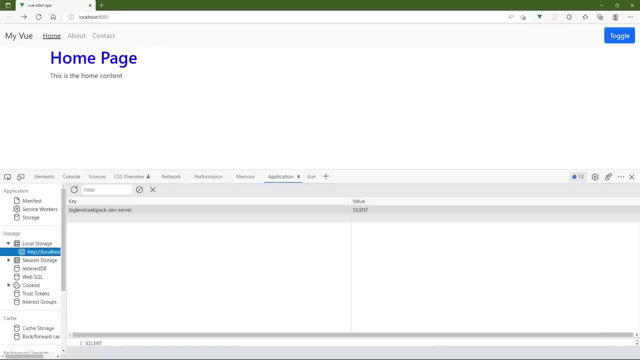 So if we go to local storage, and then the urls, and then the application, and then the url here, we can see that there is not a theme key. 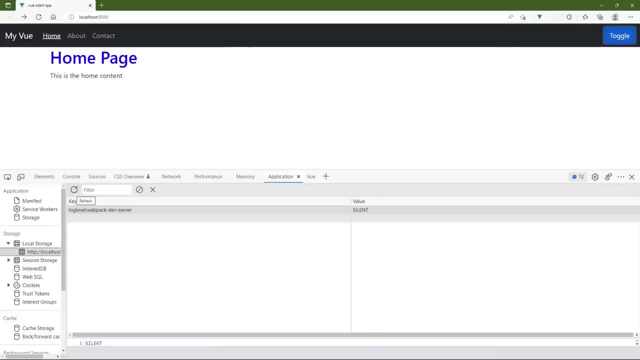 Whenever we click on toggle, and then we refresh local storage, we see that the theme is set to dark. 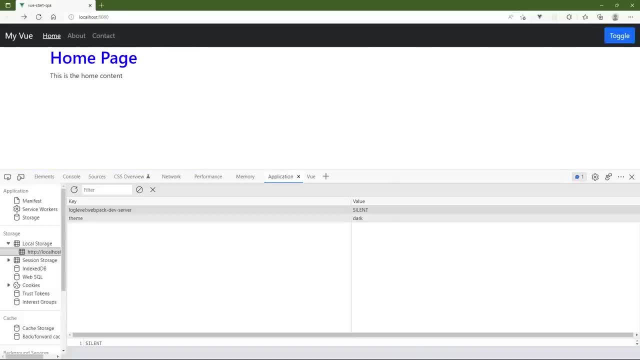 So if we refresh this page, then the theme should probably be set, it is. If we change it back to the light theme, let's refresh our local storage. 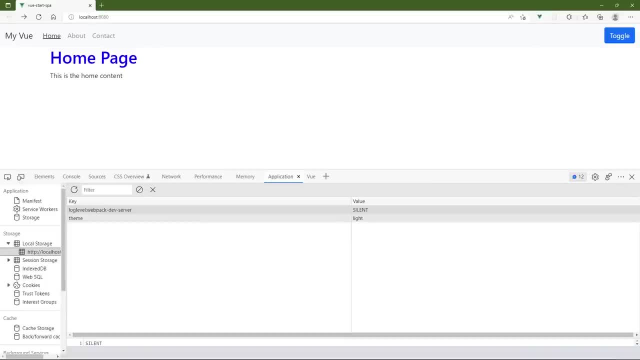 We see that it is now light. We refresh the page, and of course, that setting is loaded. Now, as I said, 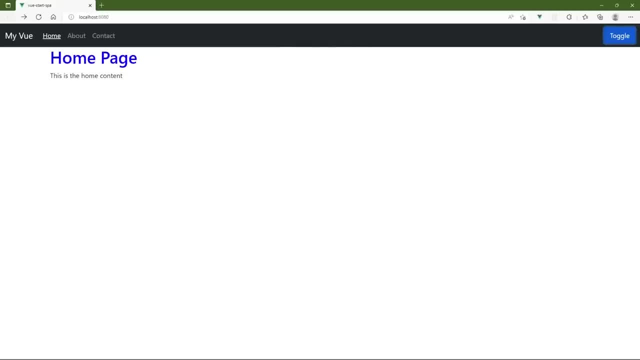 this is completely and totally dependent upon your application. 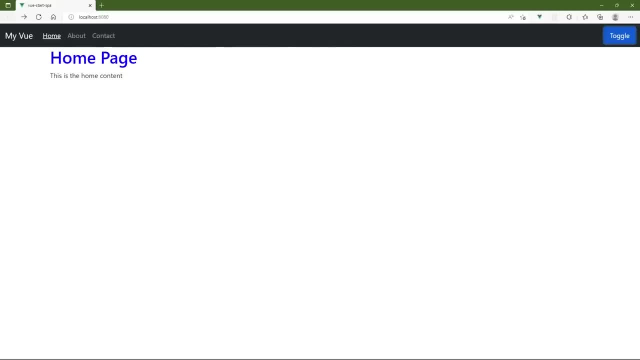 It's also dependent upon your opinion of when you should load the data within your application. 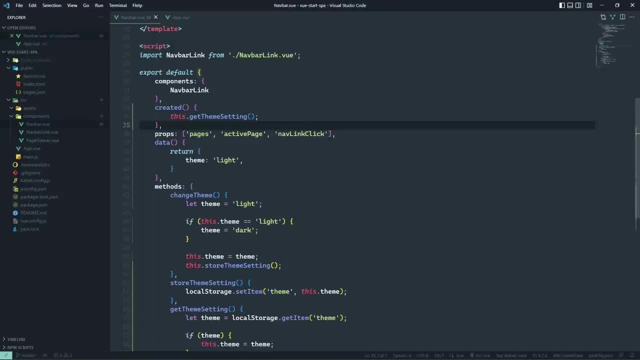 As we add more settings, it might make more sense to load everything up front, so that we aren't hitting local storage multiple times all at the same time. 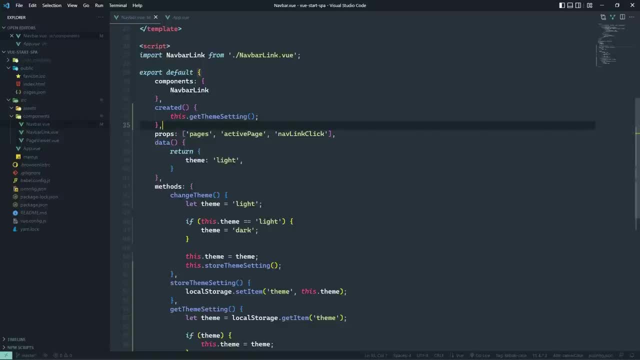 But then again, it is application dependent. 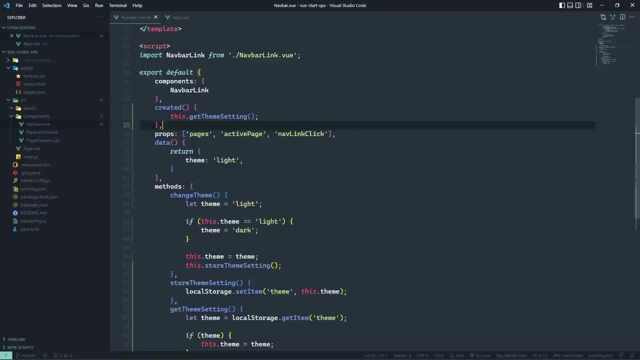 And also, don't be afraid to make changes to your application. Sometimes designs change. We very rarely never get it right the first time. So go with what makes sense. 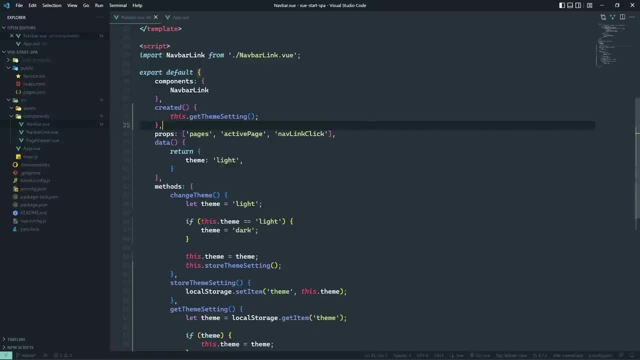 If that changes later on, well, that's why we are developers. 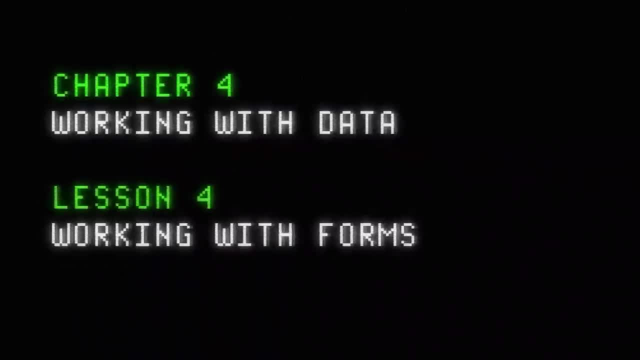 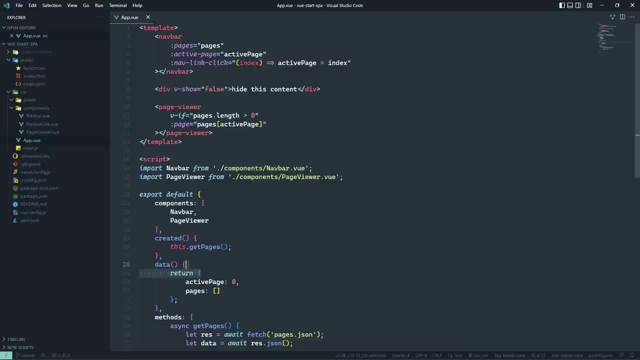 We can't talk about data without talking about getting data from the user. And the primary way that we do that is with forms. Now, traditionally, forms are the most tedious thing that we can work with in JavaScript. But thankfully, Vue makes it so much easier. In fact, it is dead simple. So, what I want to do, and 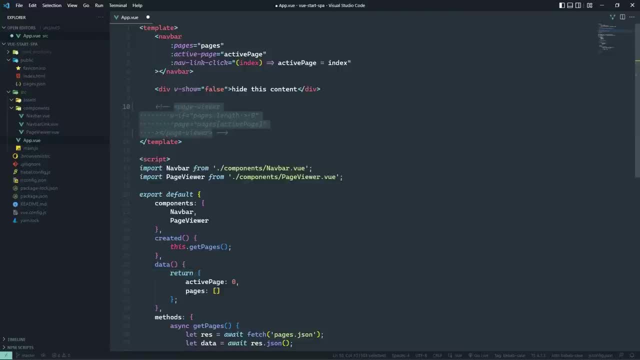 this lesson is essentially take out the page viewer, because we know that that works, and eventually we will add that back. 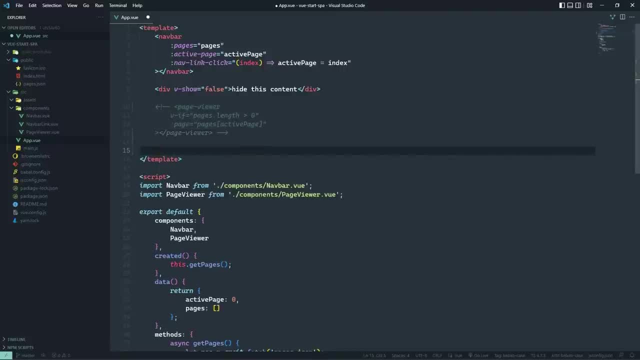 But for right now, I want to focus on forms. And I want to create a new page object that we will eventually add to our pages 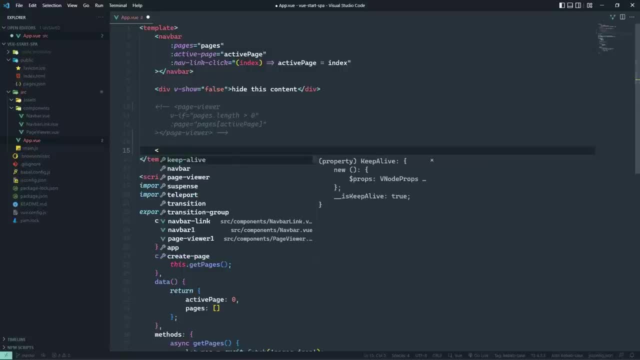 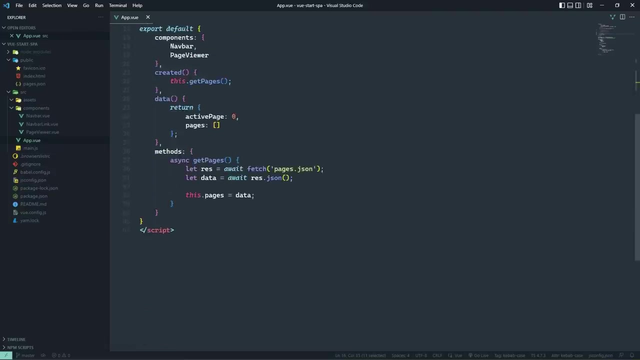 array, and we're going to do this inside of another component. So let's just call this create page. And this component needs to have a callback, so that the app will know when a page has been created. So let's just call that page created, and we'll handle it with a method called page created. Let's define that inside of our methods here inside of app. 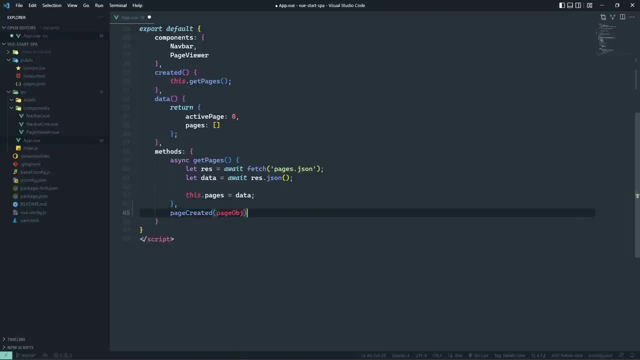 And for right now, let's just take the page object that this is going to receive and write it out to the console. 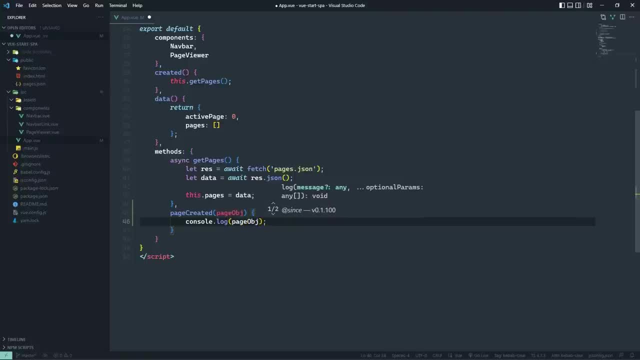 And eventually, we will then add this to the pages array. So that's the basic functionality here inside of the app component. 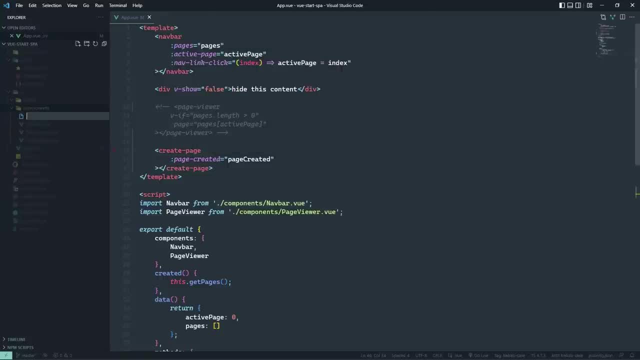 We can go to our components folder, and let's create a new file. We'll call it createPage.view. 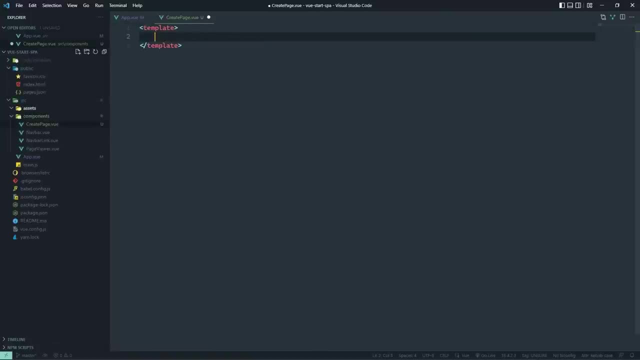 And as far as the template is concerned, I already have the markup. Just because it's a lot of typing, and there's really not a whole lot here. There's two form fields, one for the page title, one for the content, and 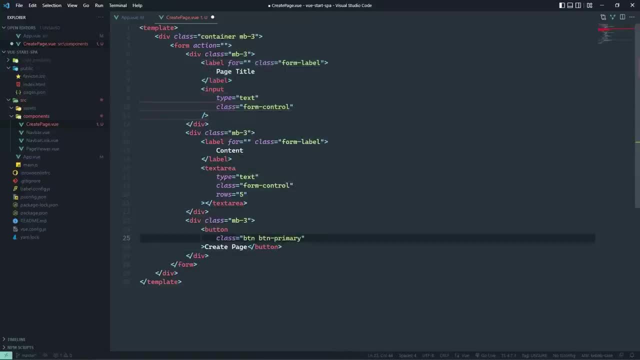 then there's a button, which is going to execute that page created. 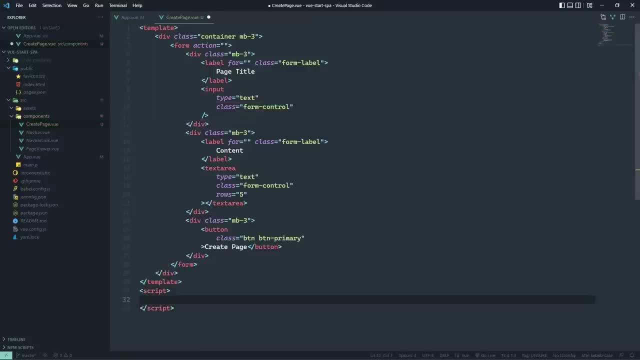 So we know that we have that prop, let's go ahead and define that. And we can use just the simple prop. 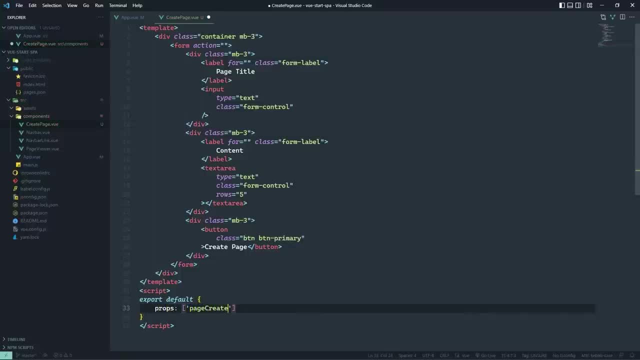 Definition, there's no need for us to use the descriptor object notation. And we know that this page created is going to execute whenever the user clicks on the button. 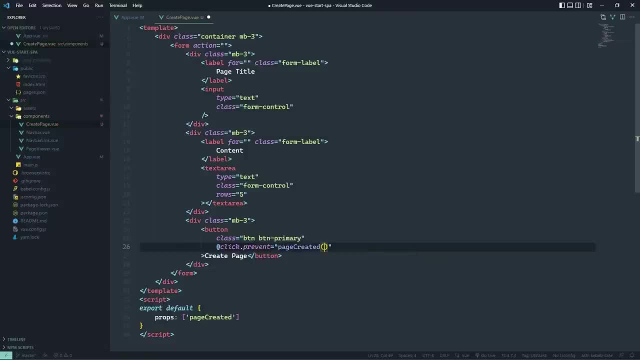 So let's go ahead and set up that click event. And we don't necessarily know what we are going to pass. Well, we know we're going to pass an object, we don't know what the values are going to be yet. 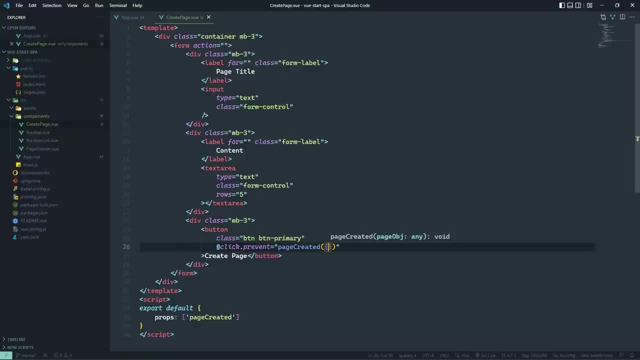 So we have all the preparatory stuff ready to go. Now we can focus on getting data from the form. 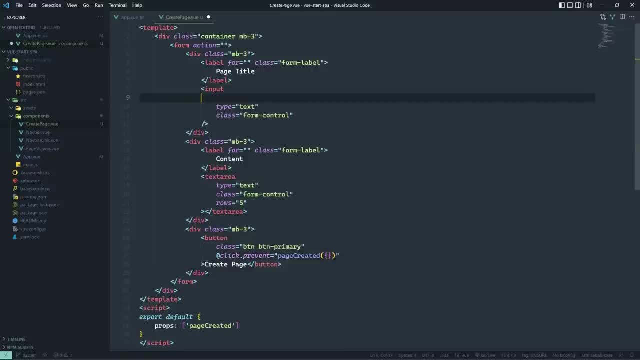 Now, with traditional JavaScript, we would typically apply an ID to the input and the text area elements, so that we can reference those elements, get their values, and then we're good to go. 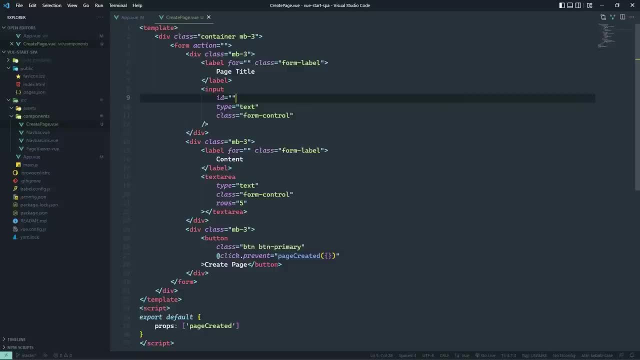 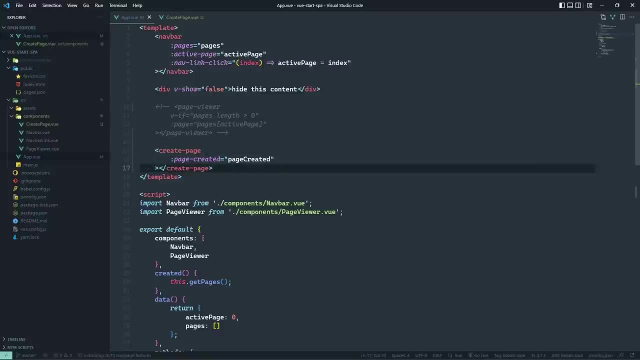 We can't necessarily do that with view, because remember that we are inside of a component, which means that if we wanted to, we could use multiple create page components within the same view component. 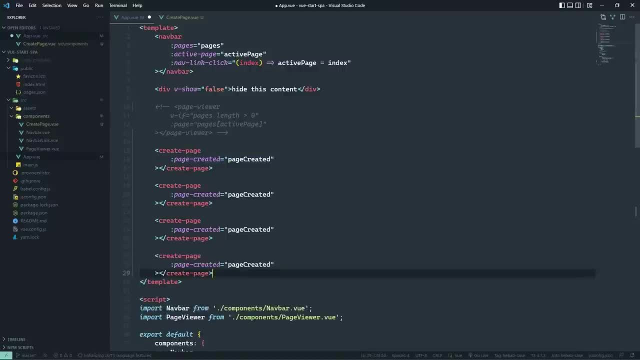 Which then we would have multiple text area, multiple input elements that have the same IDs, which that's not gonna help anyone. 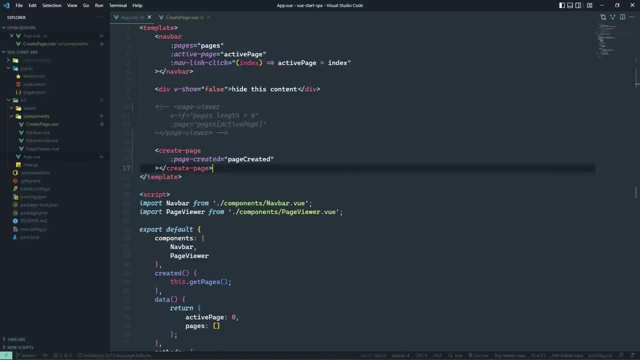 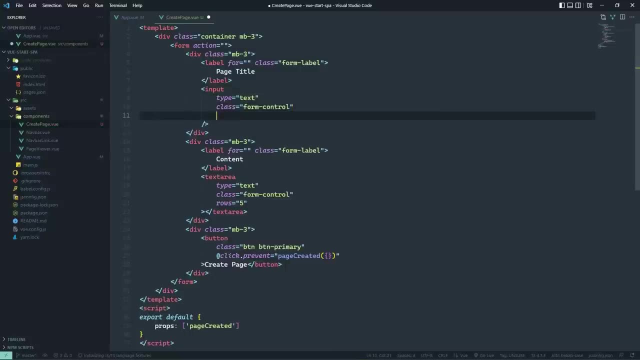 So instead, we need to think about using tools that we already know about, such as binding data. So for example, for our page title, we could do something like this, to where we bind to the value of the input element. And we could call this simply page title, which means that we would need to define this inside of our data. So let's go ahead and do that. 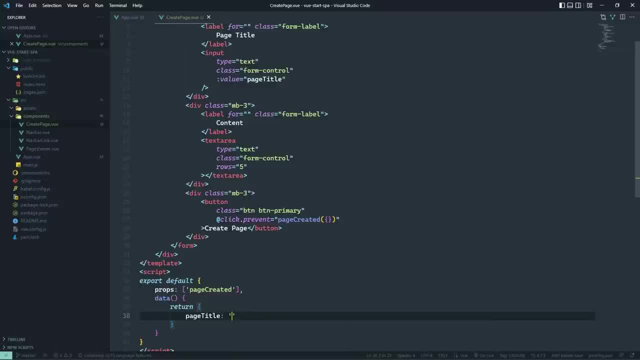 We can. initialize it with an empty string, and that's great. 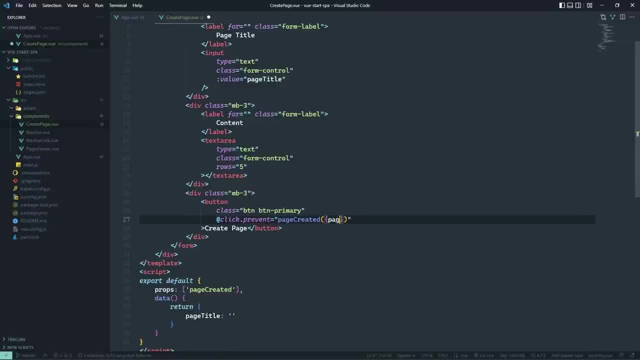 So whenever we click on Page Created, we could include the page title there. So let's go to the browser. And we don't see our form because I did not import that inside of the app component. So we want to import create page, and 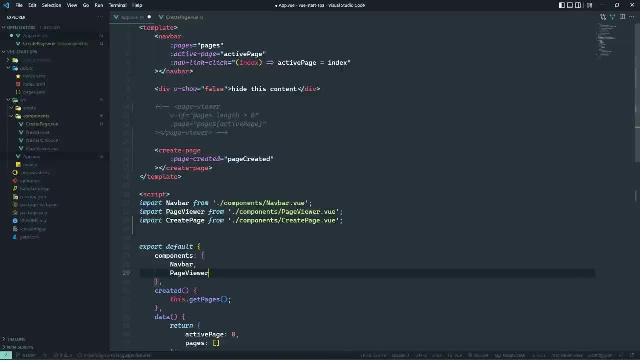 we want to include that within the components option. So there we go. Now we should see the form. 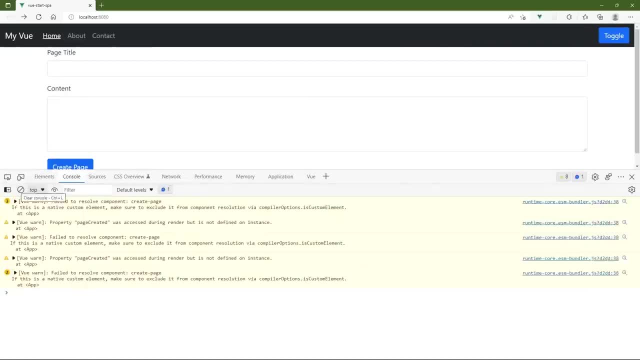 Let's pull up the console so that we can see what result we get whenever we click on Create Page. 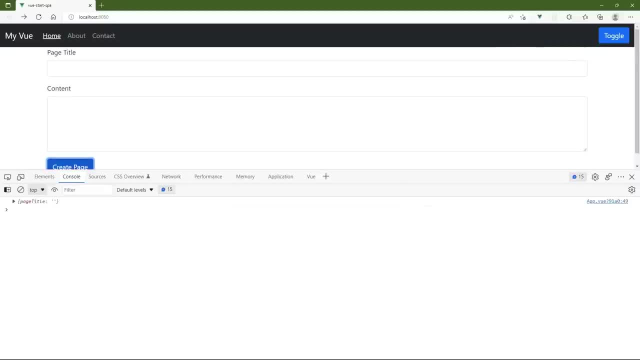 Let's just click on it. We see that we have an object with page title that is set to an empty string, which makes perfect sense. 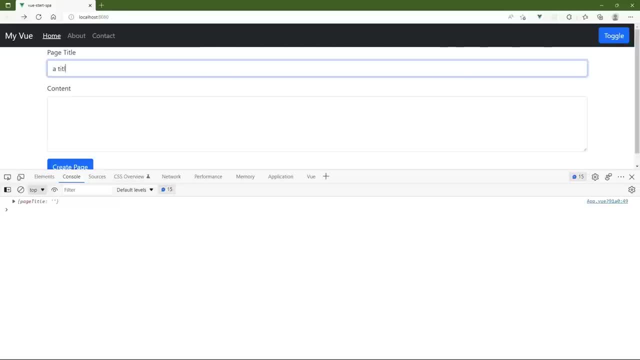 That's what we would expect because we haven't provided a title yet. But let's provide a title. 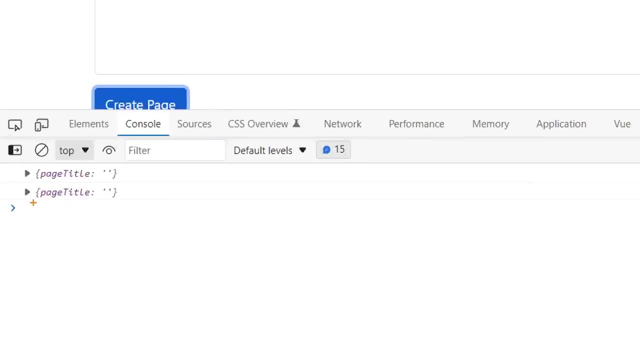 Let's click on Create Page and notice that the output is the same. Page title is still an empty string. 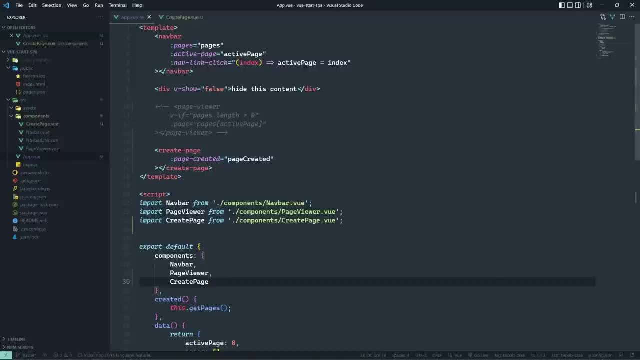 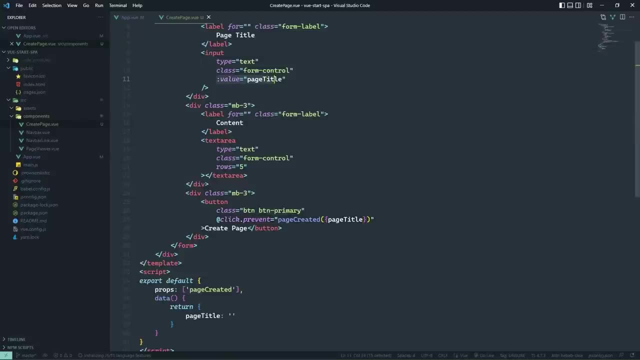 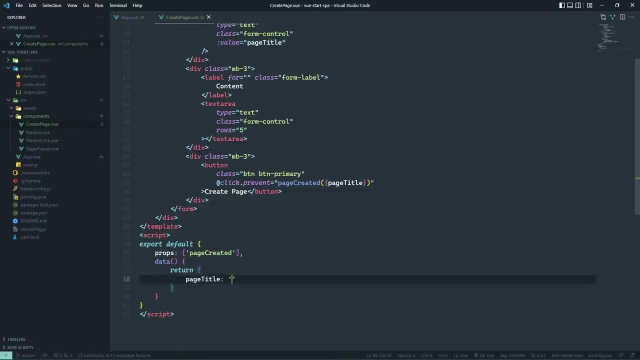 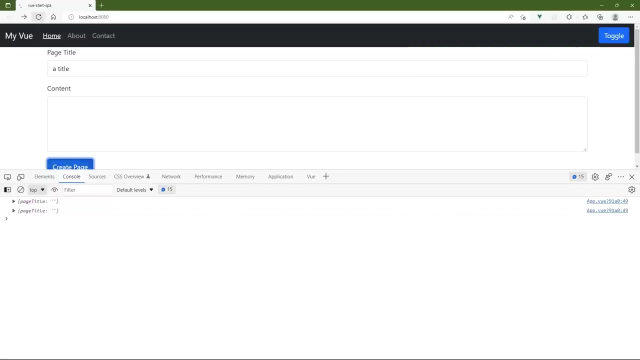 And the reason is very simple, because whenever you bind data using VBind, yes, you are binding data, but we are essentially saying that the value of this input element, whatever page title currently is, which right now it's currently an empty string. So if we provide any text as the initial value for page title, whenever we go back to the browser, let's refresh, we're going to see that value being displayed for page title. It's a one-way binding. 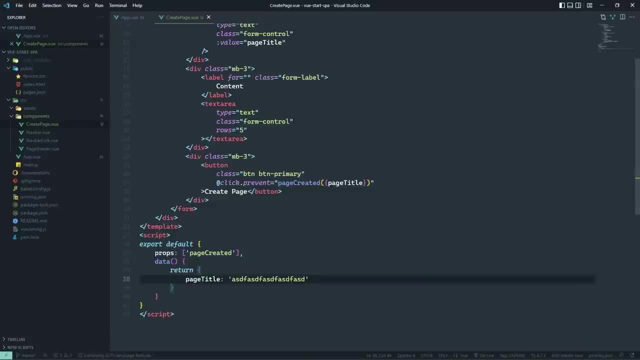 So instead, what we have to do is update page title. Whenever the value of the input element changes. 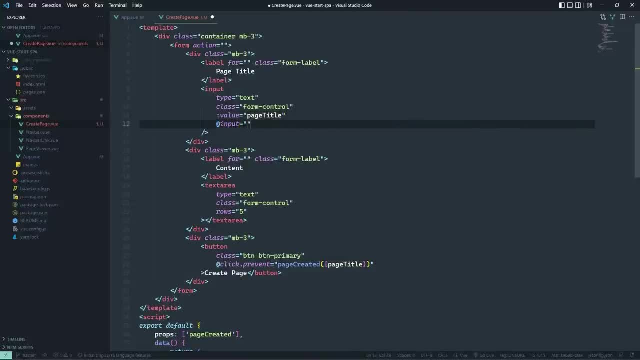 And we can do that with the input event. This is the normal DOM input event. So we can have a function that's going to handle the input event. We get the event object, and we will set page title equal to the target 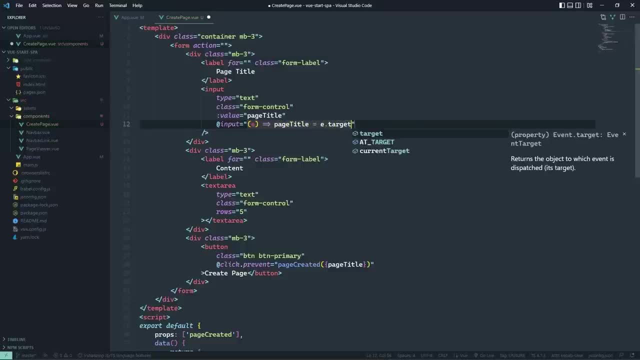 of the event, which is this input element, and we would get its value. So now we have this two-way binding. 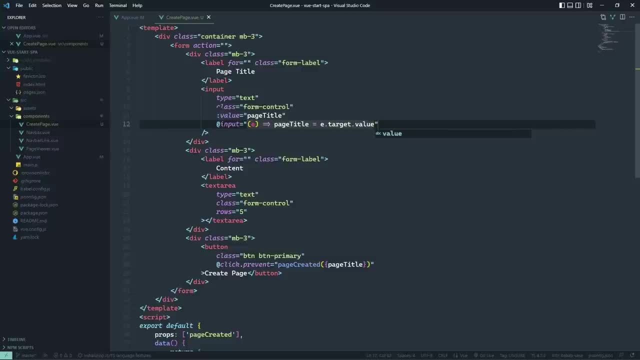 So now, even though we have a one-way binding, and one way binding with the value and the page title. 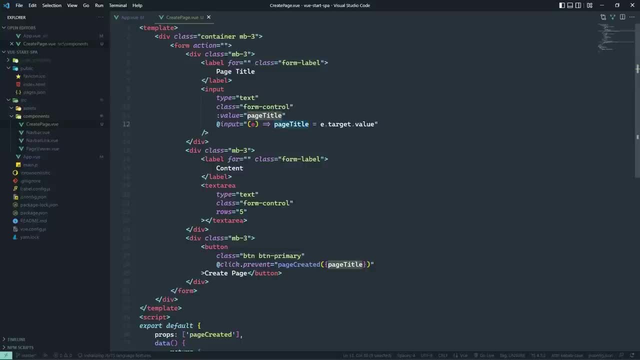 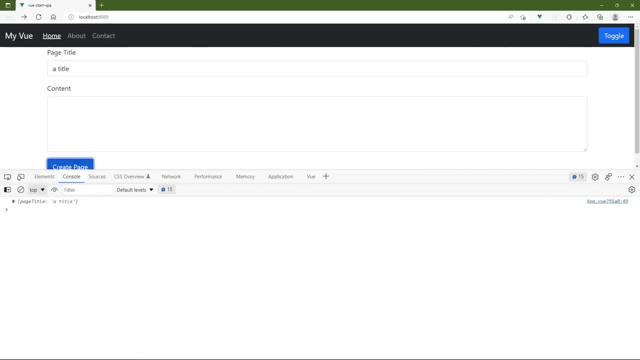 Now we are updating the page title whenever the value in the browser changes. So let's go back to the browser. Let's type in something. Let's click Create Page. And now we see that the value is what we would expect it to be. Page title is a title. 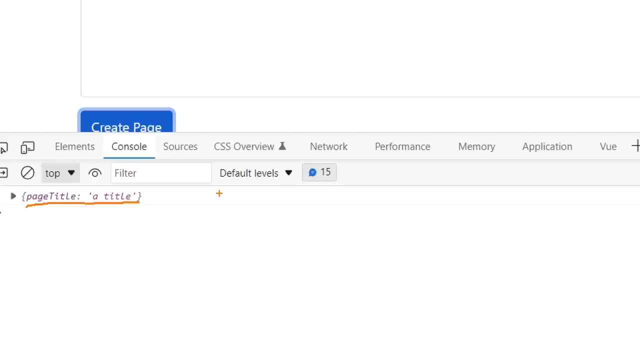 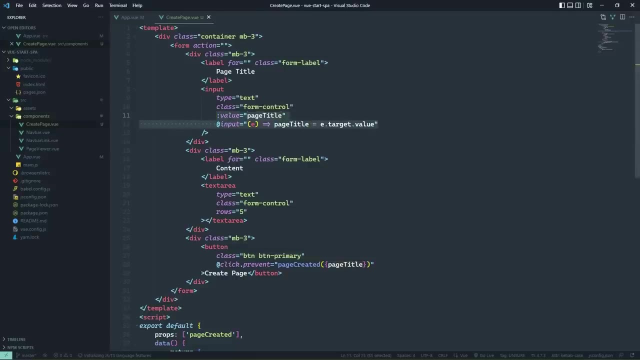 But also remember that I said that Vue has the easiest way of working with forms. This necessarily isn't very easy. However, there is a directive that we can do that essentially does this same thing. 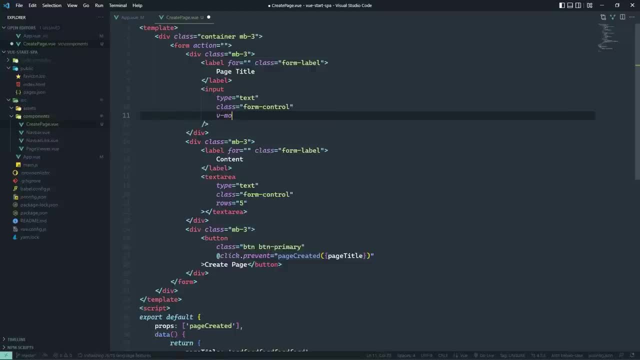 And it's called vModel. And this sets up a two-way binding between this input element and then whatever we specify as the vModel, which is going to be page title. 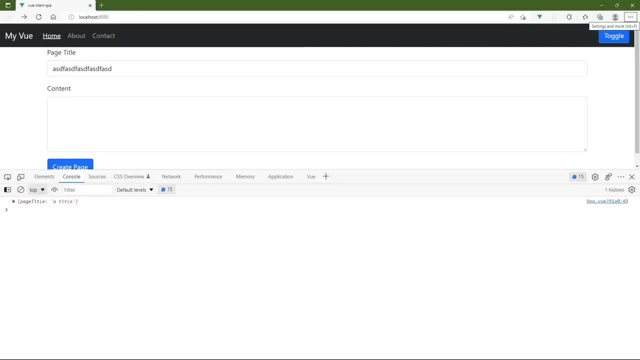 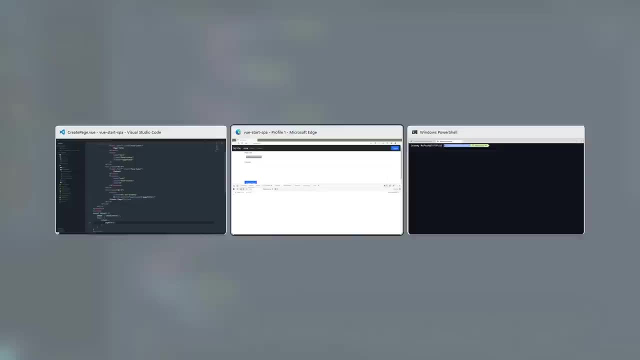 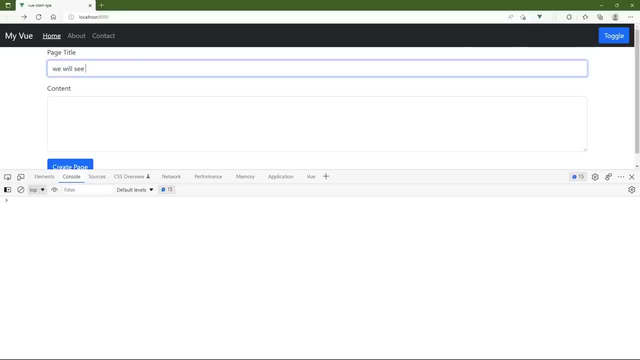 So now we're going to see that same functionality. We can see that the page title is initialized with that initial value. Let's change that because that's silly. So we'll initialize it with an empty string so that it is empty. But then, no matter what we type inside of this, we will see it as the page title. So let's click on Create Page, and there we go. 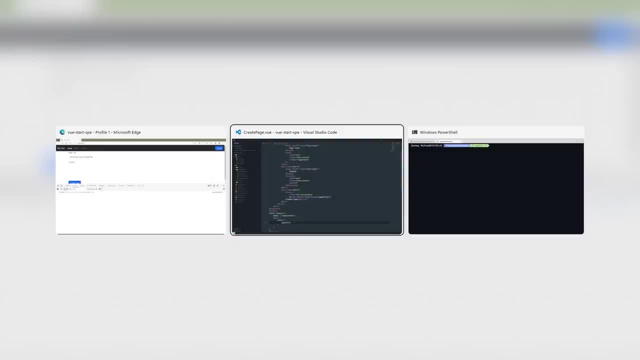 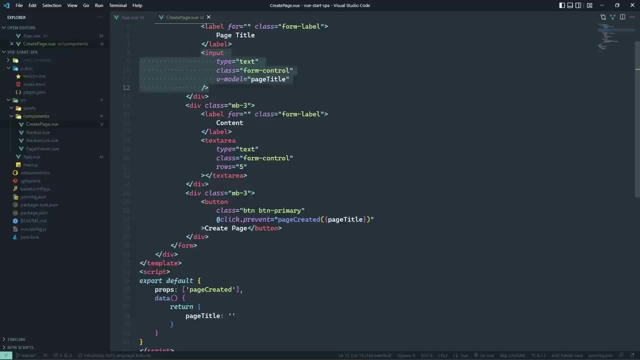 So in order to work with simple form elements, all we need to do is use this vModel to bind a data property to that form control, and that's it. 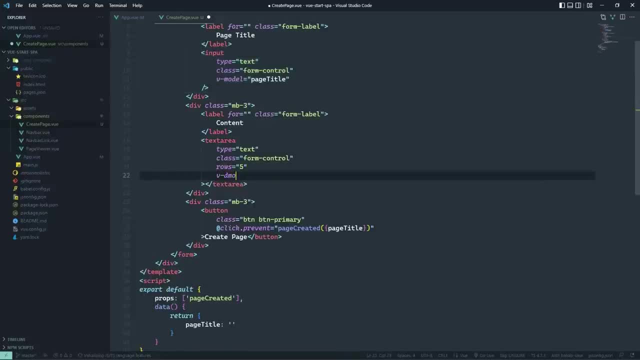 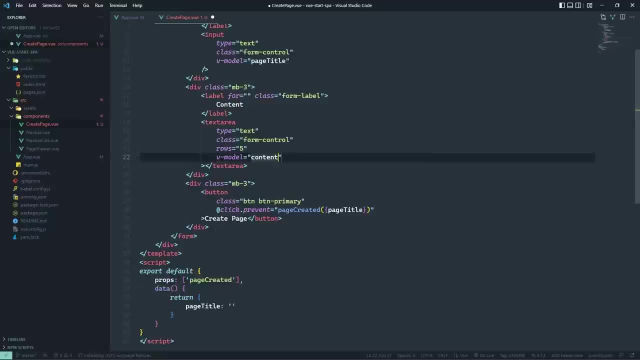 So we can essentially do the same thing for our text area. So we will have a data property. So we can essentially do the same thing for our text area. So we will have a data property. We will have a data property called Content. We will use vModel to bind that content to this text area so 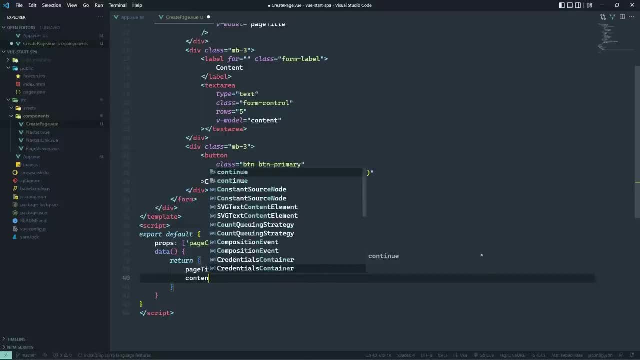 that then whenever we click on our Create Page button, we will provide both the page title and the content. So let's go back to the browser, 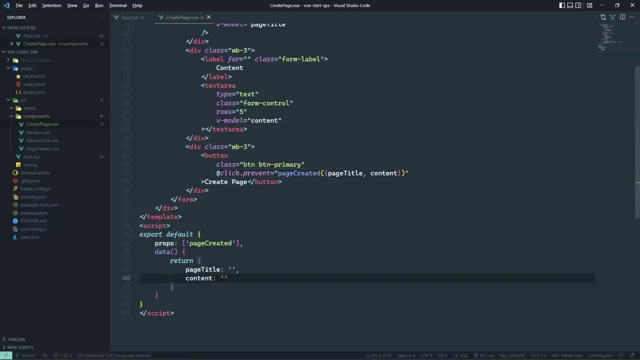 although we do need to initialize content with a value. 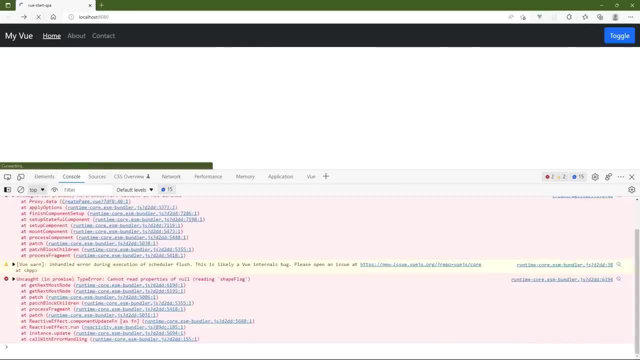 So let's go back to the browser and let's refresh the page, because we did have an error there. And now let's provide a title. 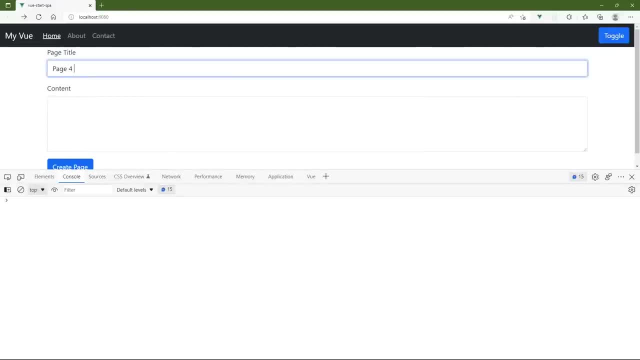 And now let's provide a title. Let's just call this Page4Title, and this is the content. 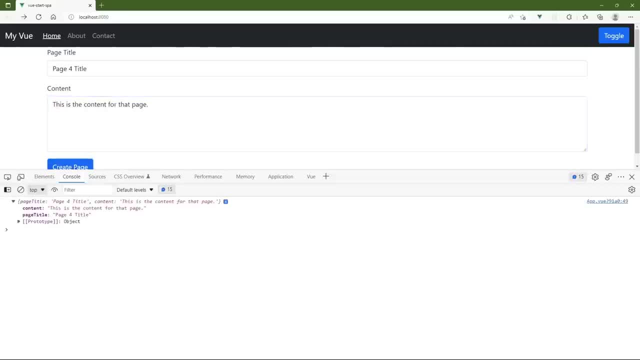 Whenever we click on Create Page, we will see in the console that we have an object that has the content that we typed, as well as the page title. 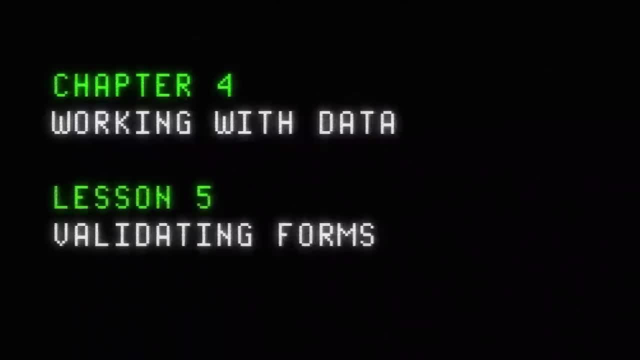 In the previous lesson, I introduced you to the vModel directive, so that you can set up a two way binding between a form control and a data property. 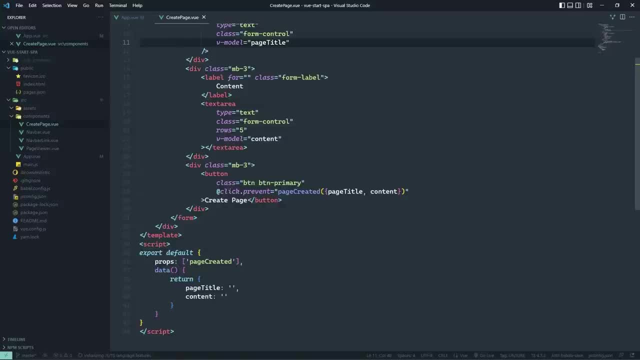 And that's all well and good, but there's more to working with forms than just getting information. 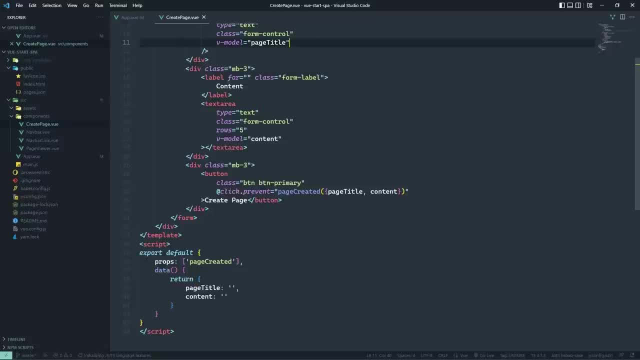 We also need to be able to validate the information, and it would also be useful to have some visual cues. 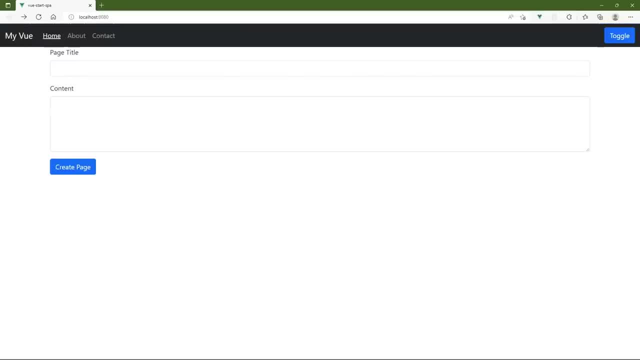 For example, if the form is not valid, then we could disable the Create Page button. And it could stay disabled until we have a valid form. 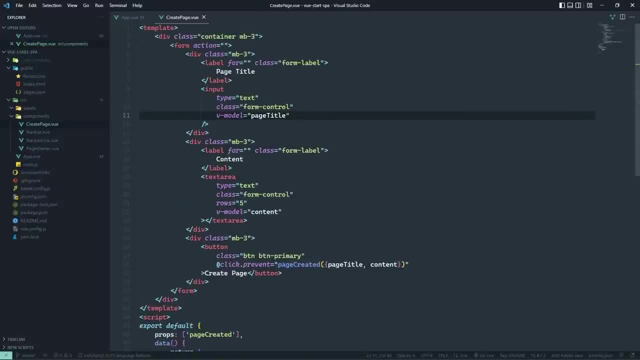 So let's start by changing up our form, because the object that we are creating is not complete, we also need a link. 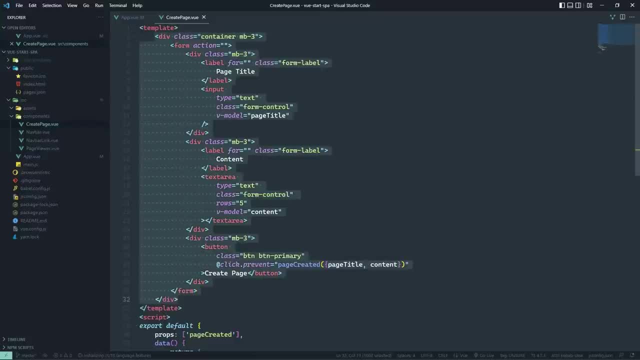 So we need at least two other pieces of information, such as the text and the URL for the link. 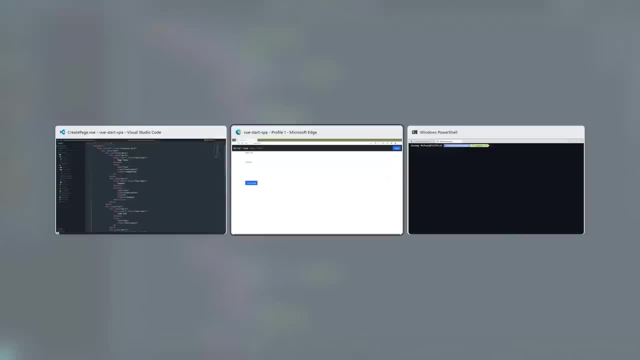 So I'm going to paste in some new markup. It's just changing our form so that now we include the link text and the link URL. 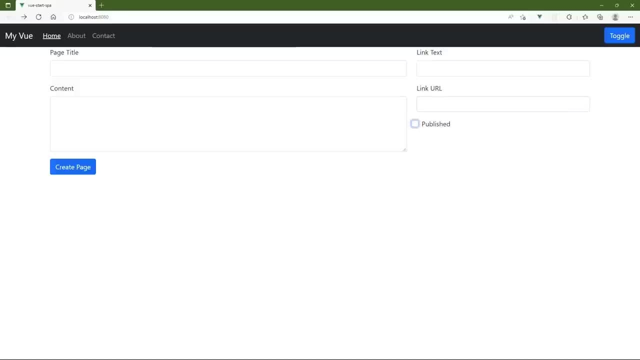 I also have this published checkbox, which we don't have to worry about just yet. But the idea is going to be that if it is published, then we see the link in the menu bar. 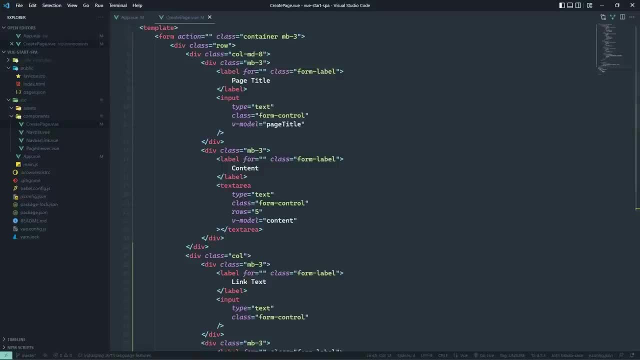 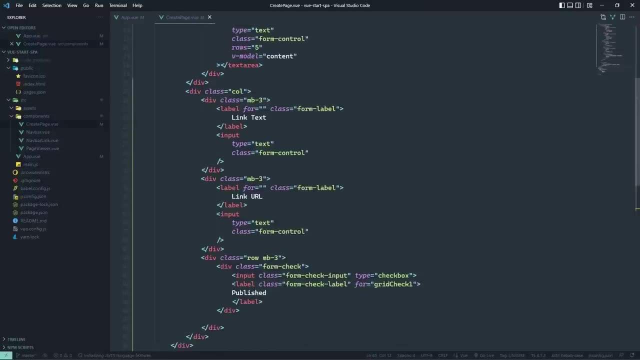 If it's not, then we don't. So the first thing we need to do is set up the two-way binding between the form control and our data properties for the link text and the link URL. 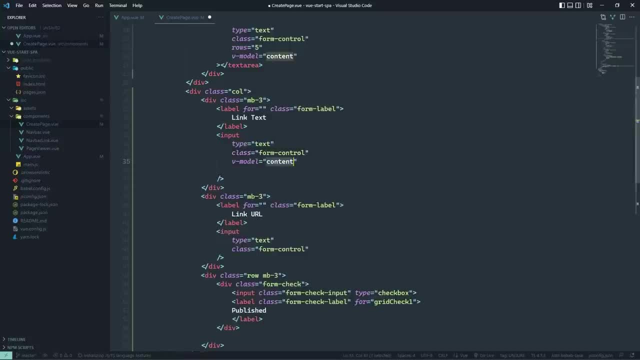 And of course, we don't have those values, but they're going to be simple enough to create. 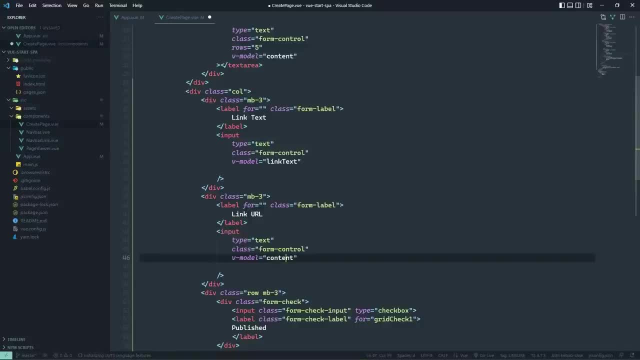 We'll call the link text, just link text, for the URL, we'll call it link URL. And we will initialize these values as empty strings as well. 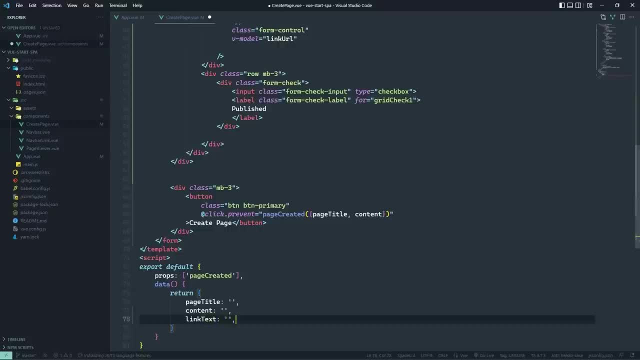 Now, because we are adding this extra information, it makes sense. 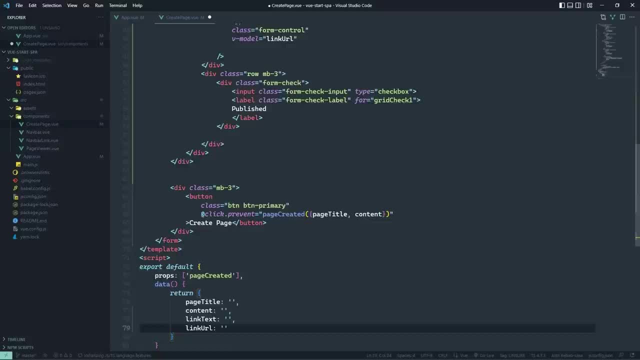 That we modify the code that is handling the click on our button. Because we just called page created, we passed in a simple object with the page title and content. 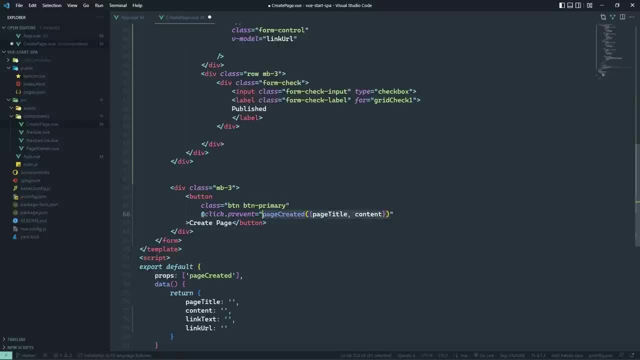 Now we need to do some validation, and we need to build a more complex object. So let's define a method, we'll call it submit form. 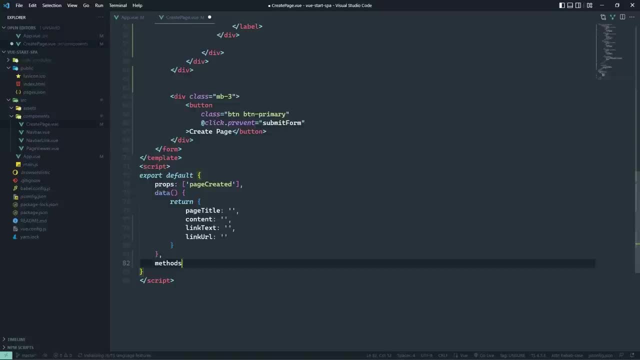 And we need to add that to the methods option. Now, as far as this submit form method is concerned, we don't need any extra data friendly release material for our exiting that can be there in a JS. We can use something called data await instance here that contains external data, such as the event object, which would be passed here. 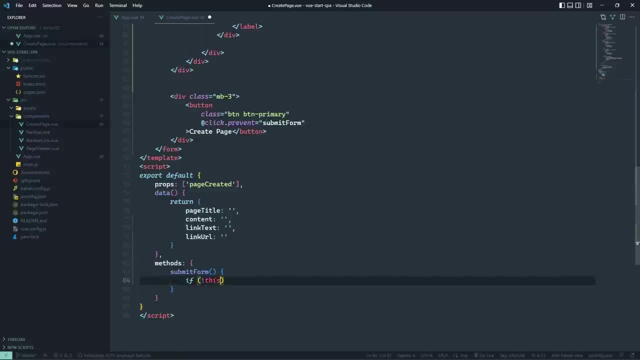 And the reason is because all of the data that we need is right here inside of our data, so the first thing we're going to do is going to be rather tedious. 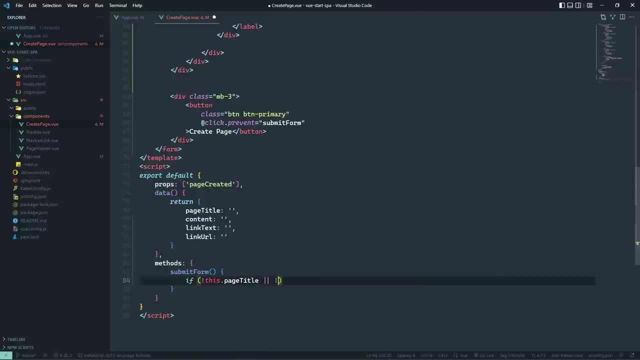 We need to make sure that we have some values. In fact, we need all of the values, because in order to create a page object we need a title. We need the content. And. of these values is missing, then we can't do our job and create that object. 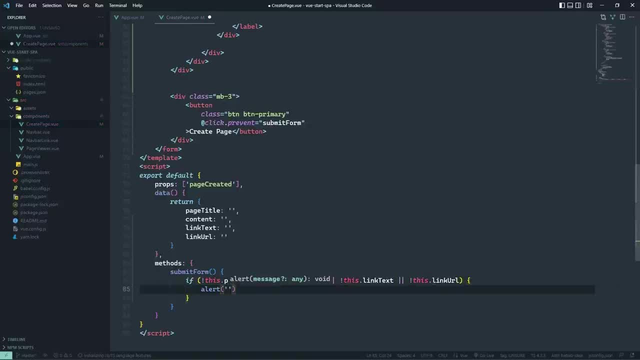 So we are going to alert to the user that they need to fill out the form. And then all we need to do is return because there's nothing else for us to do. 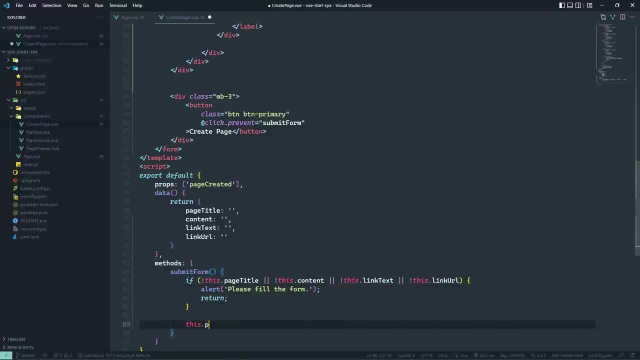 But if we do have all of the data, then we can call the page created function. 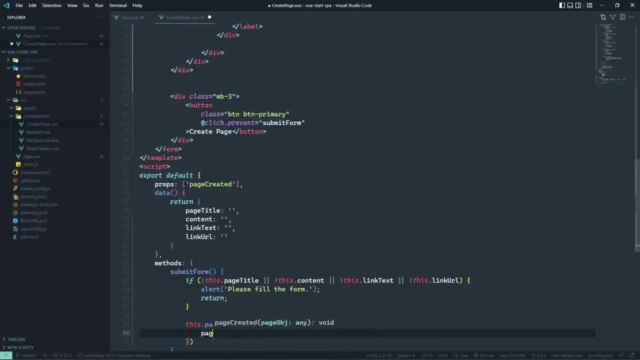 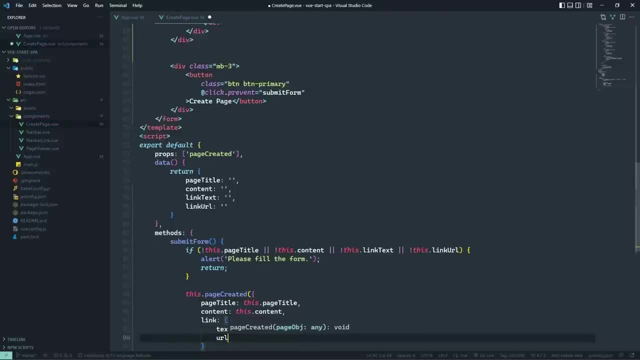 And then we will pass in an object that has the page title, the content. And then we will build the link object, which has text and URL properties. 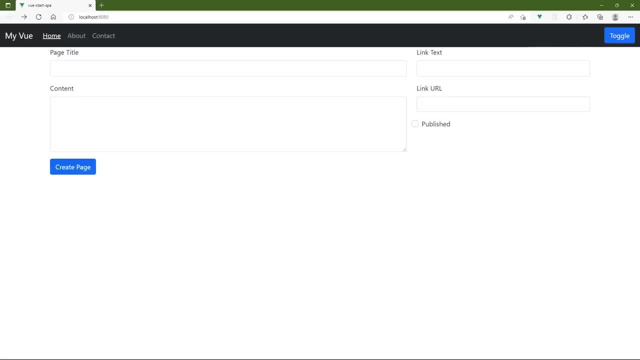 So with that done, let's do a sanity check. Let's see if everything is going to work. So let's first of all click on the Submit button. 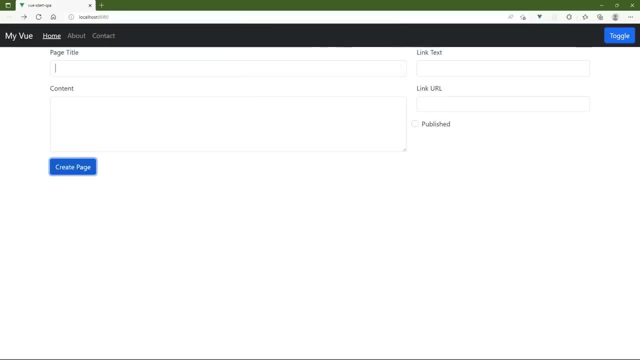 And we see that, of course, this is not going to work. Please fill out the form. So let's just add some content and make sure that we aren't going to be able to submit this object without providing all of the information. 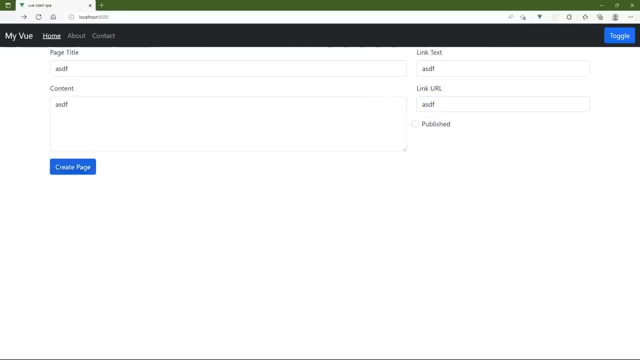 And we should still have everything set. So that we output that object to the console, and we do. 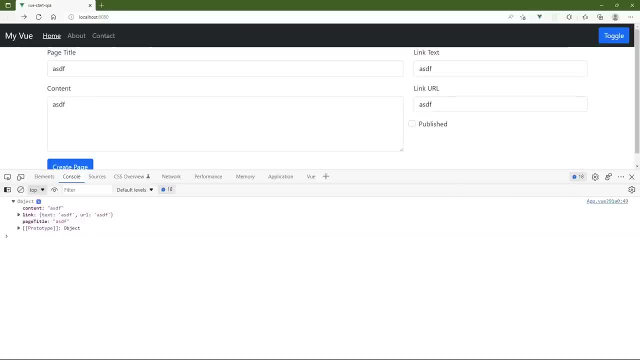 So there's the content, the link, and the page title. That's fantastic. 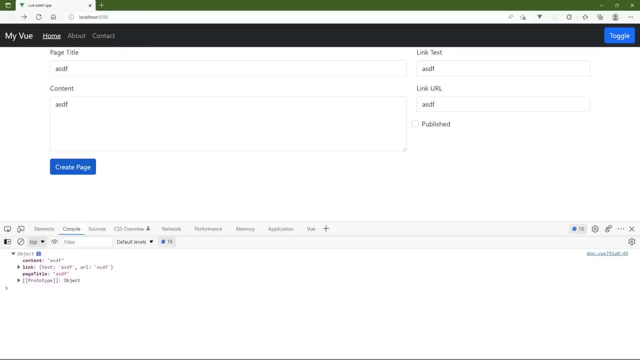 Now I want to set up a visual queue so that the button will be disabled until the form is valid. And that might seem kind of redundant, especially since we've already set up the submit form method to check these values. But it never hurts to have redundancy, especially when it comes to checking if something is valid or not. 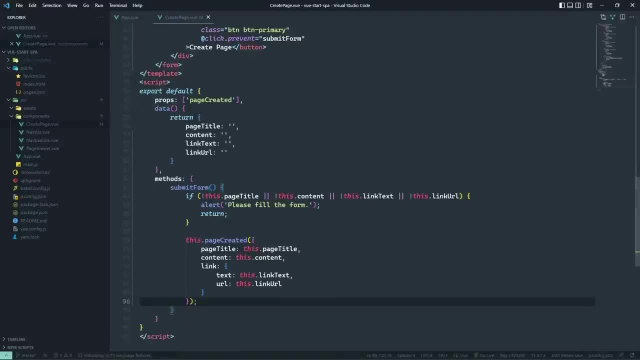 And besides, having a visual queue is always a good thing. So we can accomplish this in a couple of different ways. 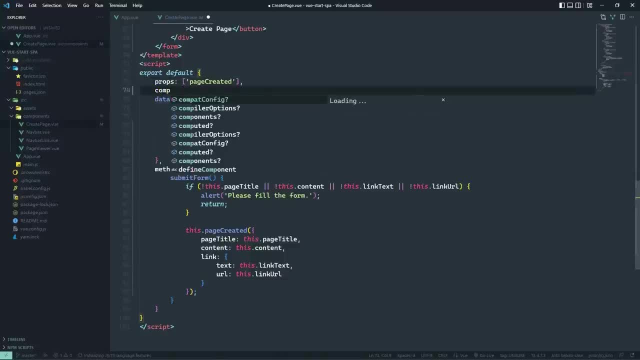 But probably the easiest and most straightforward will be to use a computed value. 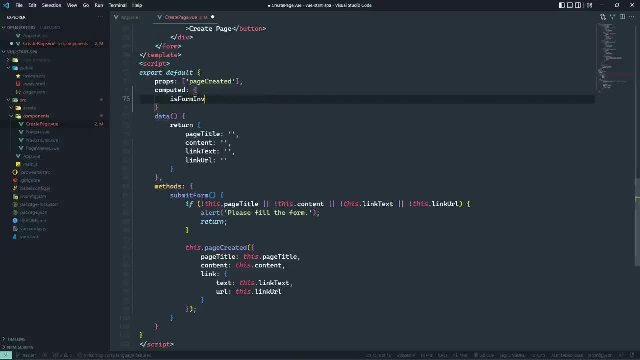 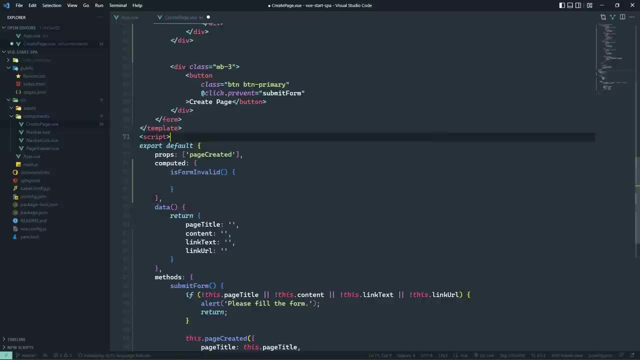 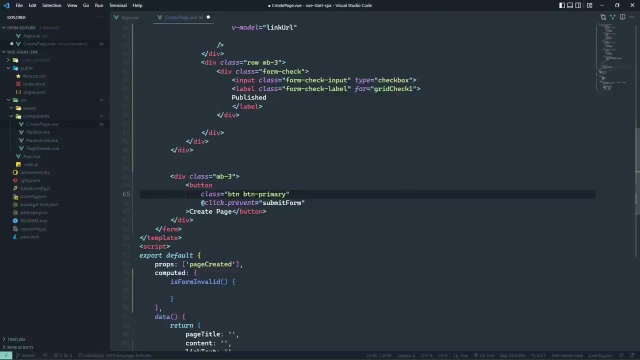 And let's call this isFormInvalid, which kind of sounds weird because I would typically want to say isFormValid. But we're going to be binding this to the disabled attribute on the button, which means that when disabled is true, then of course the button is disabled. 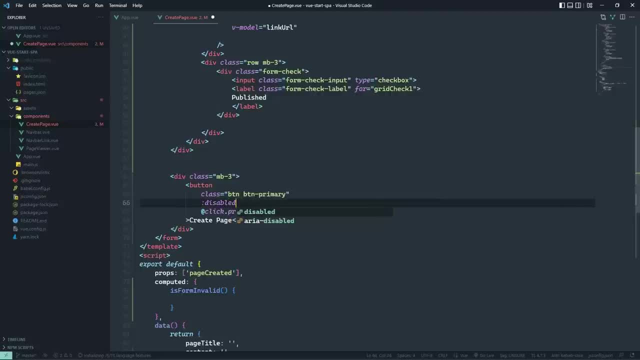 If it's false, then it's not. So the wording is to make it a little bit easier to understand what's going on so 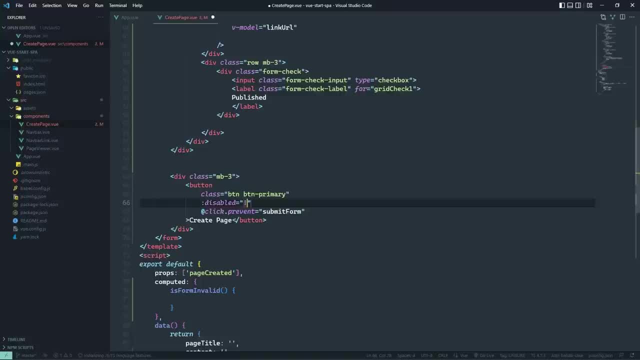 that we don't have to parse it out and do something like this, is not, isFormValid. So it's just to make things a little bit easier. 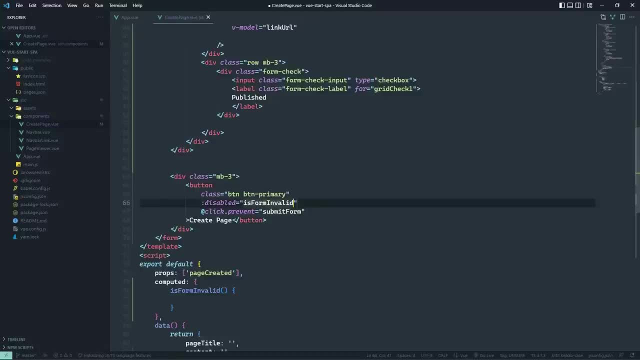 So if isFormInvalid is true, that will disable the button. So now we just need the code to check if the form is invalid. 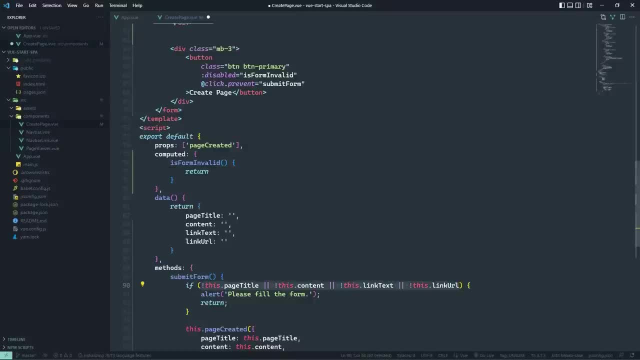 And we basically already have that. If any one of our values is empty, then that will return true. 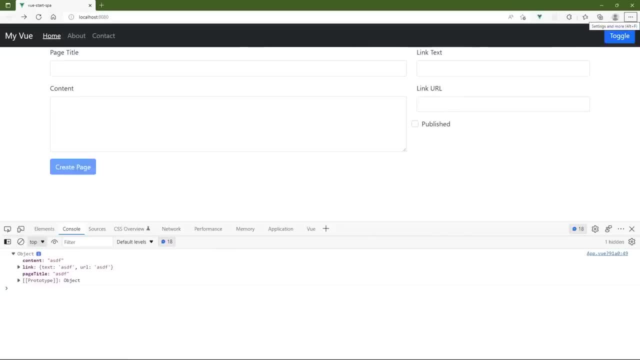 So we can go back to the browser, and we can see that the button is disabled. 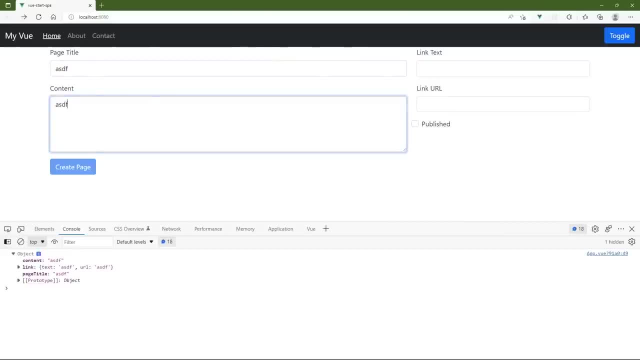 And as we start adding values, you see it is still disabled until the entire form is filled out. 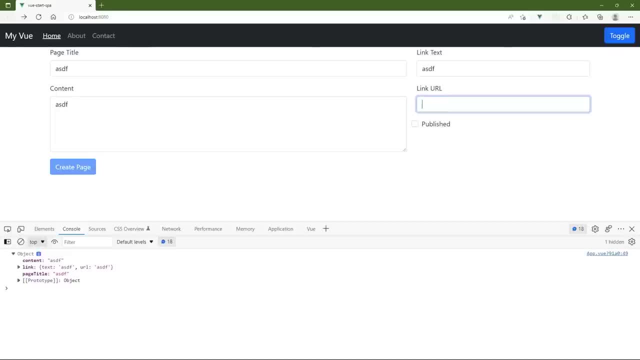 If we clear out any one of the form fields, it goes back to being disabled. And of course, whenever we submit the form, the object is sent back to the parent, that app component, 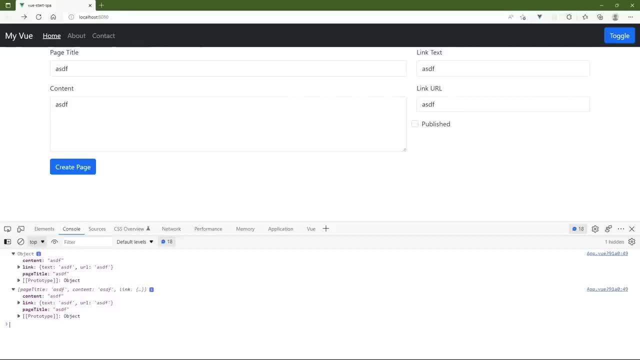 where we can add it. And we can output that information. In the next lesson, we are going to modify the pages array so 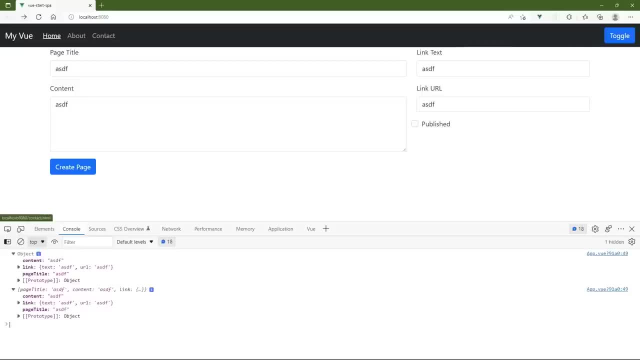 that whenever we create a page, it will update the menu. 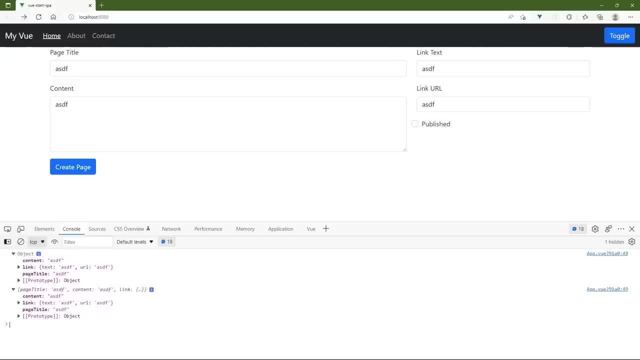 But we also want to only display the pages that are published, which means we will need to filter the pages that are in the nav bar. 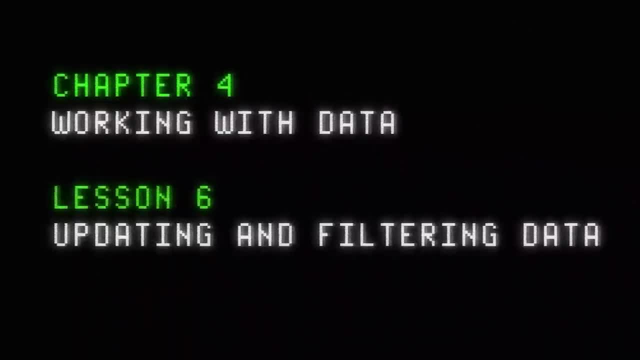 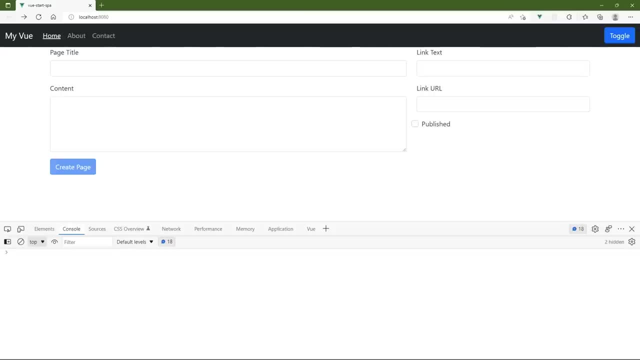 In this lesson, we are essentially going to do two things. We will first of all add the code to add page objects to the pages array, so that we will display those. In the nav bar, but we also want to take into account this new published value. So that if a page is marked as published, it is displayed in the nav bar. If not, then well, it's not. 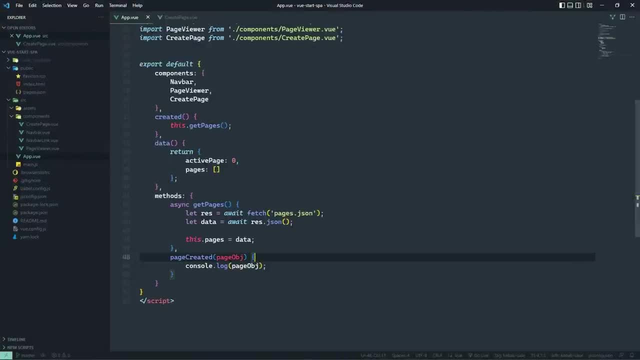 So let's start with the easiest thing, and that is to modify the pages array. 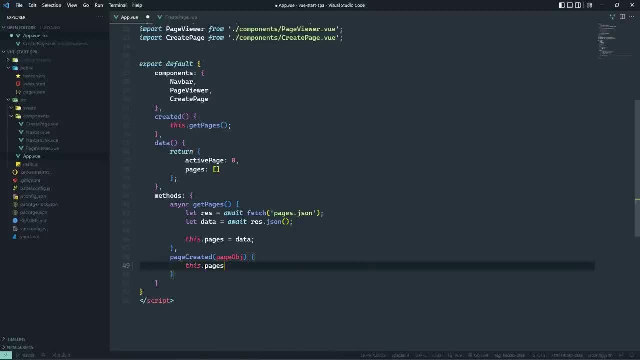 This really, literally cannot be simpler. All we need to do is push in the new page object, and we're done. 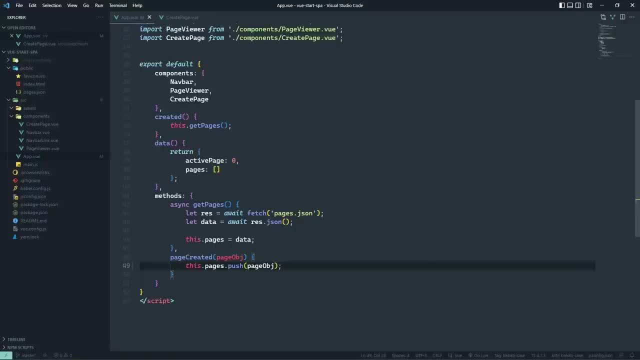 So the lesson here, is that anything that modifies or mutates our pages array, is going to automatically signify to view that this data changed, update all of the UI that uses the pages array. So any built-in array method that mutates the array, and there are several, push, pop, shift, unshift, splice, sort, even reverse, those are methods that mutate the array. 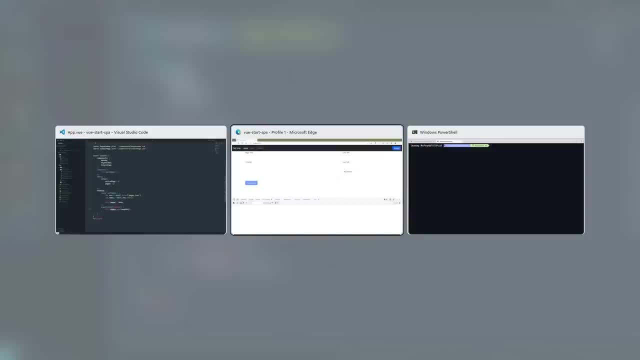 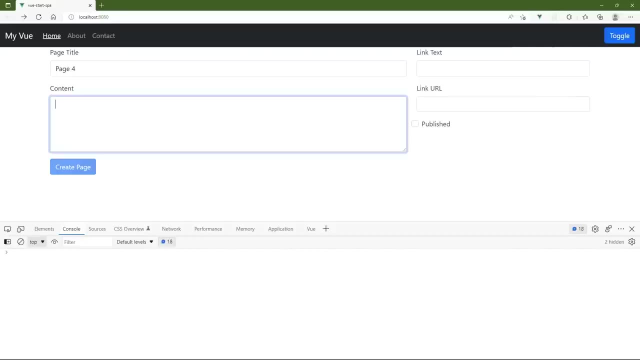 So therefore, those changes will be reflected in the UI. So with that simple change, we can add a new page. We can say that this is page four, and we'll just have some content. We're not really displaying this information right now. For the link text, let's use page four as well. And in fact, we might could do something to make this a little bit easier from a data entry standpoint. 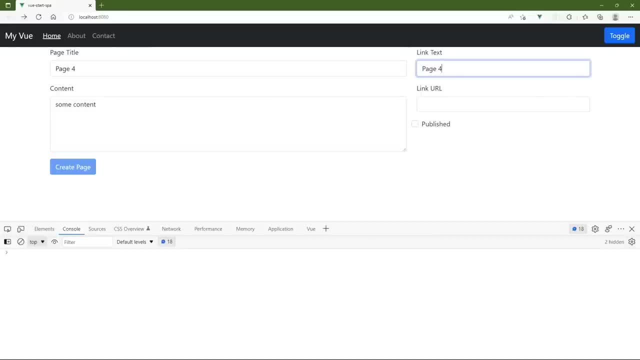 Because a lot of times the page title might be the same for the page link. Something that we might want to consider. 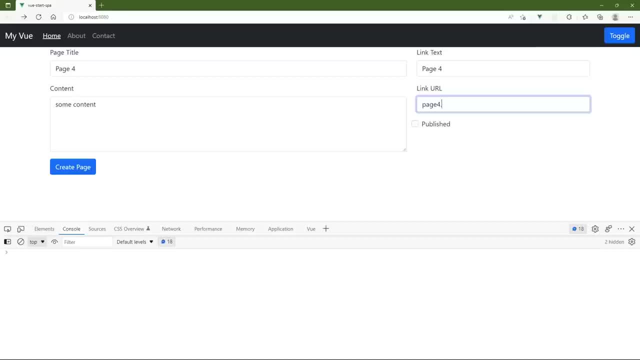 And then for the URL, let's just call this page4.html. And we will click on Create Page. 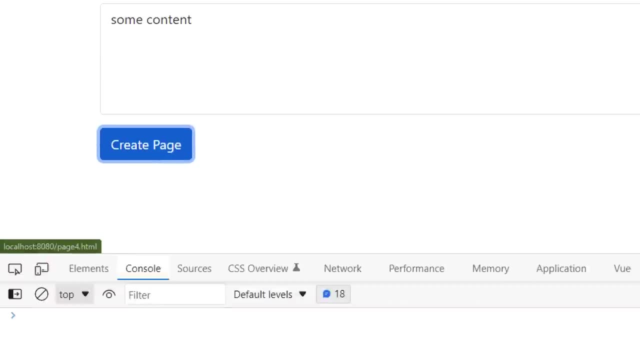 We see page four in the menu bar, and the URL is page4.html. 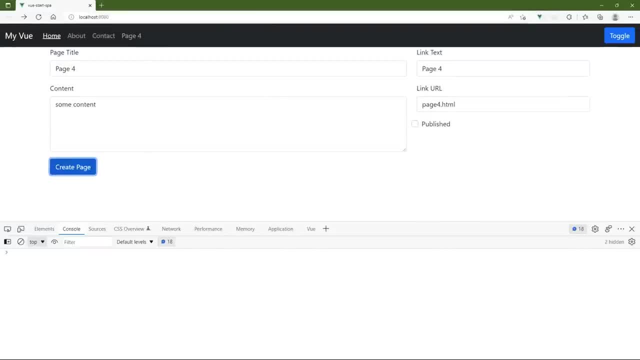 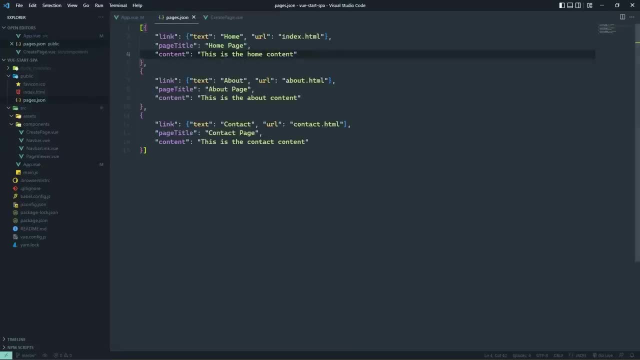 So as far as that code is concerned, we are golden. Now we just need to take into account this published value. Now this is going to require us to modify our pages.json file, because this is the original place our data is coming from. So let's do this, for the home page, we'll set published to true. We'll also do the same thing for about. 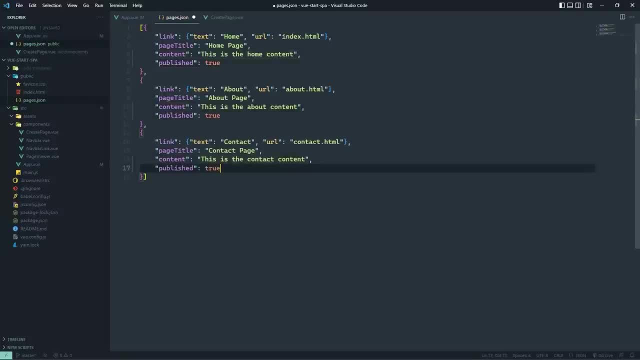 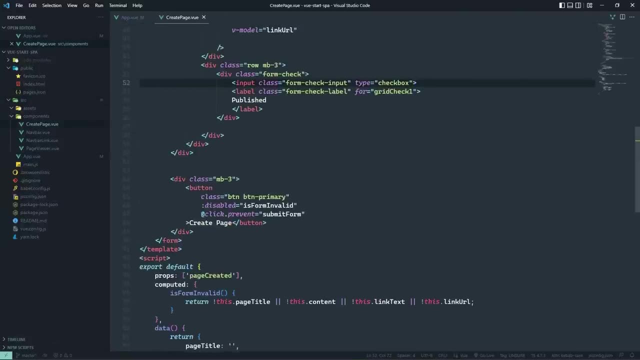 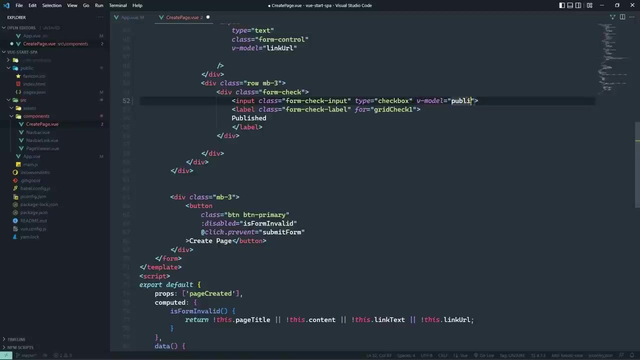 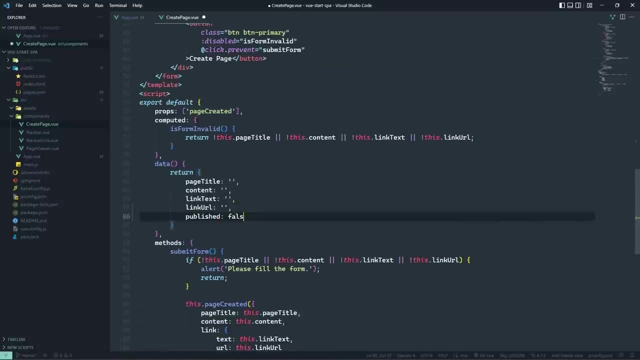 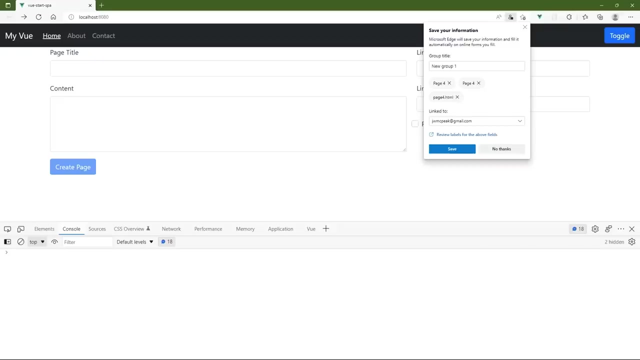 But for contact, let's set it to false, so that we will not see that in the navbar. So with that done, we need to go to our create page component, because we need to take that published value into account. So we need to set up a vmodel for that checkbox. Let's just call it published, and let's initialize this as false. So that if something is supposed to be published, we have to check it. Although it might be something that we want to default it as true. I guess we can default it as true, it really doesn't matter. And we can see inside of the browser that yes, it defaults to true, so we're good there. 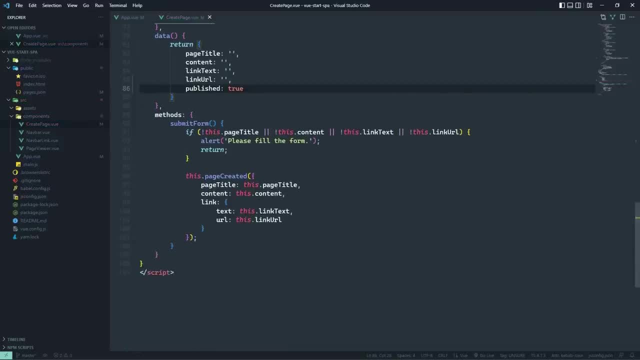 But we do need to take that into account whenever we call page created. 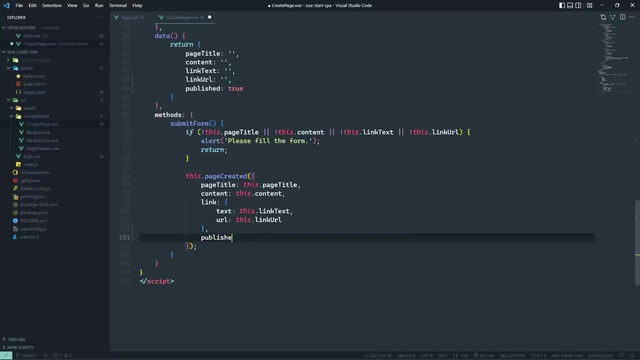 So we'll add the published property there, and we should be good to go. Except we need to filter what we have in the navbar. And the most straightforward way to do that is with a computed value. 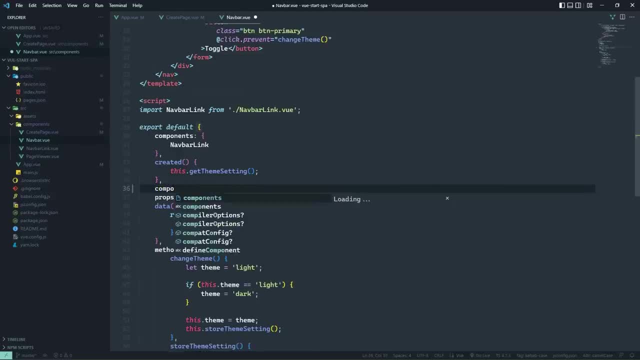 So let's go to navbar, we'll add the computed option. And let's just call this published pages. And we don't want to modify the pages array in any way. Instead, what we need is to return an array that only has the published pages. And we can do that with calling the filter method. 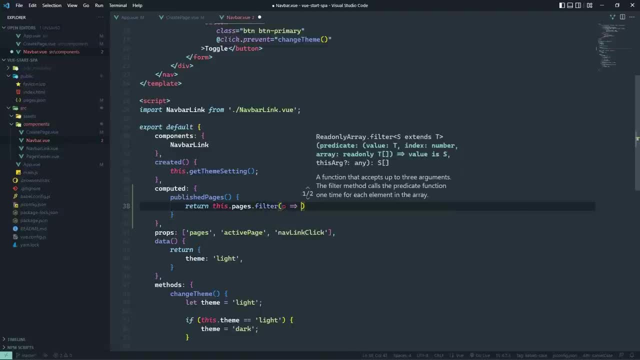 This accepts a callback function. That returns a Boolean value. If it's true, then that element in the array is going to be in the new array. 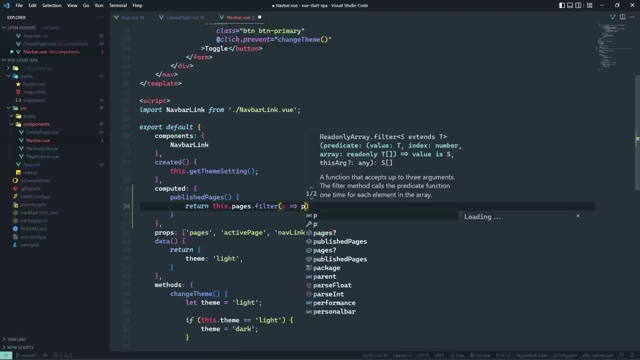 If it's false, then it's gonna be left out. So in our case, all we really need to do is check for published. And that will give us the filtered array. 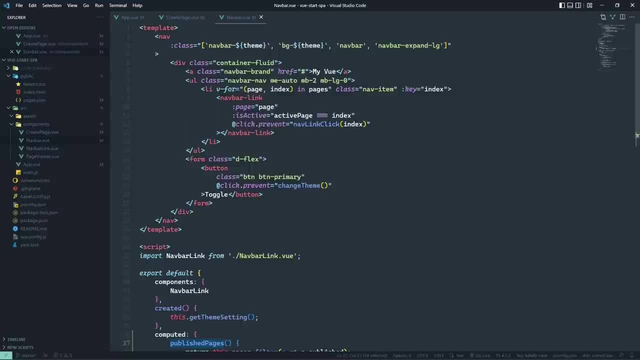 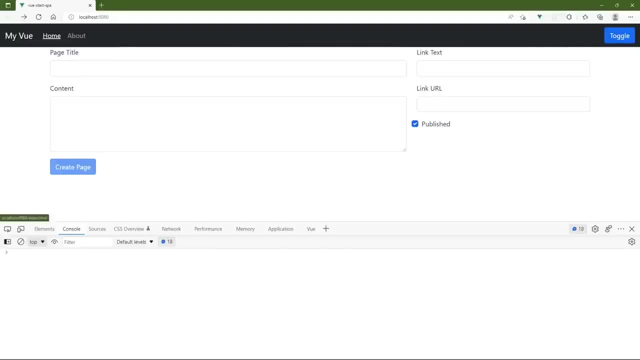 So now we can use published arrays in our for loop. So we will replace pages with published pages. Let's go back, and voila, we see home and about. 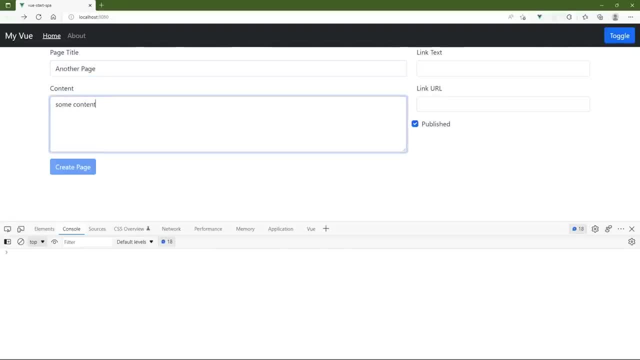 So let's add another page. With some content, the link text will mirror whatever the page title is. 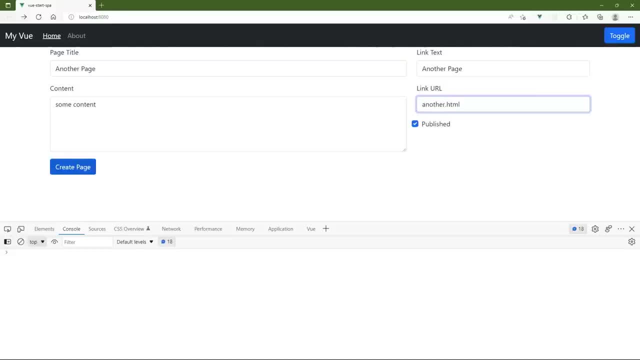 URL really doesn't matter because we don't have that to begin with. Whenever we click on Create Page, we will see it. 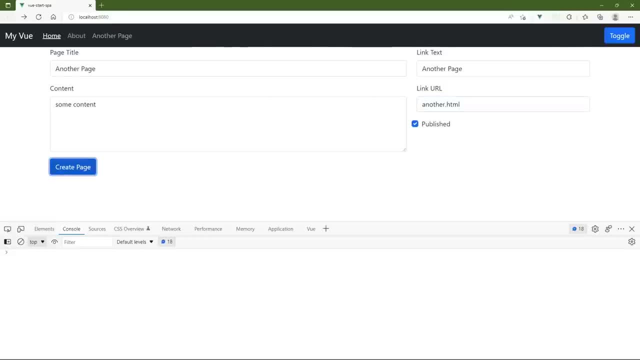 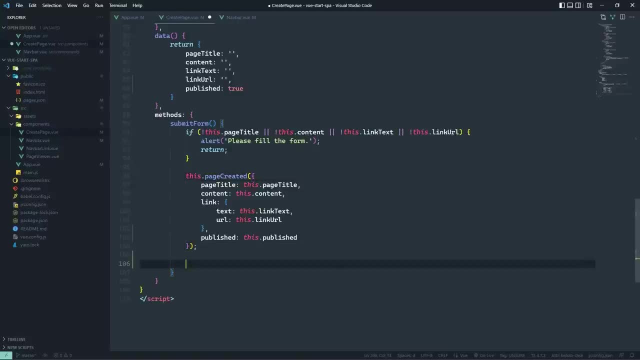 And whenever we create a page, it would be useful to clear that form. So let's add that code as well. So that after we call page created, we set all of our properties back to their original value. And this can be a little tedious process. 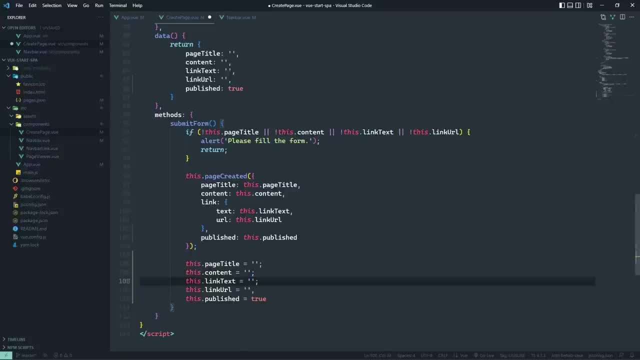 And if this is something that we need to do multiple times, then we can just write a method called clear form. And that would reset the form to their original value. 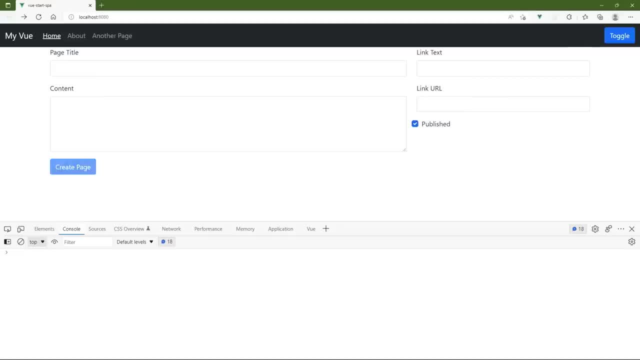 So just to make sure everything works as we expect it to, let's add yet another page that has some content. 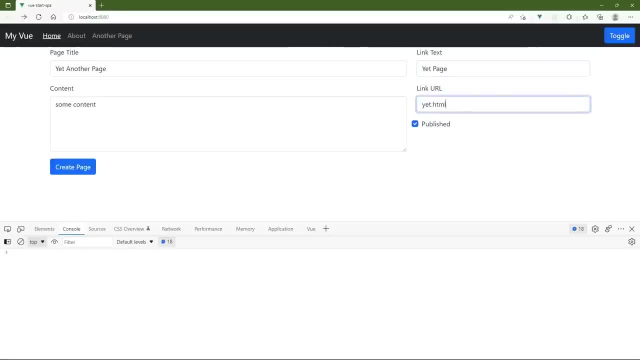 The link text will be yet page, URL will be yet.html, but this will not be published. So before we click on Create Page, what I want to do is go to the View Developer 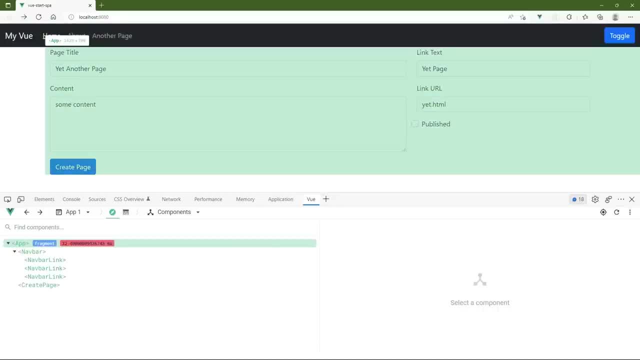 tools because I want to see what the app data is going to be. So here we have the pages array. 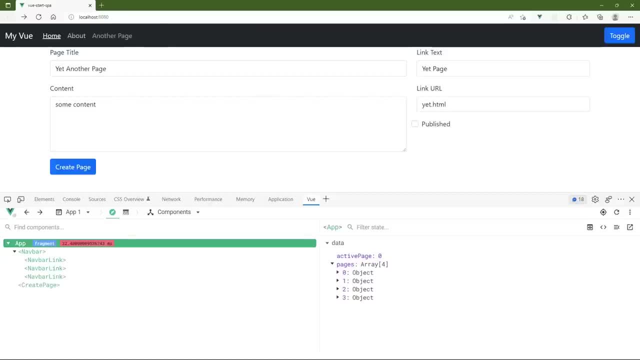 We can see that we have four pages, but we are, of course, only displaying three because the contact is currently set as not published. 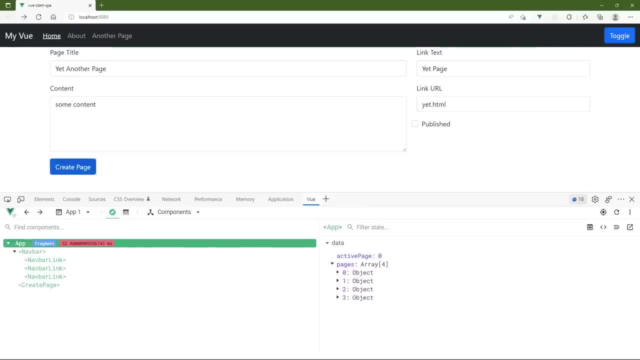 So we are going to add another object here that is not published. So we don't see that in the nav bar, but we didn't see the pages update, did we? Let's go back. Let's go to another component. Let's go back to app, and there we go. 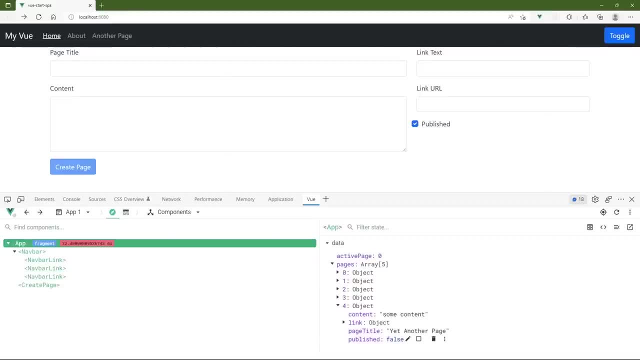 Now we have five elements in the array. And the really cool thing about this is if we change any one of these published values, we're going to see the results automatically in the browser. 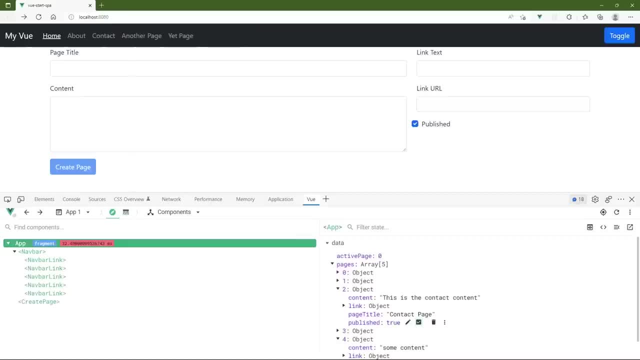 So let's change published to true for contact, and there we can see that. 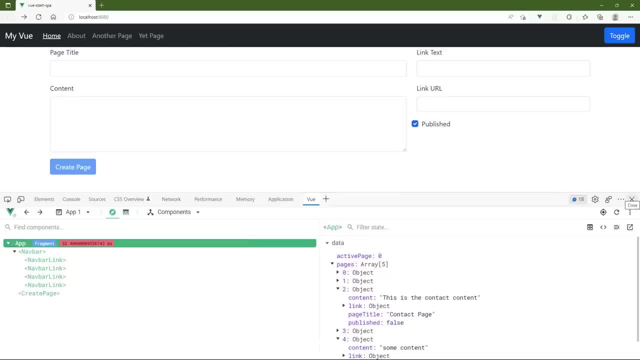 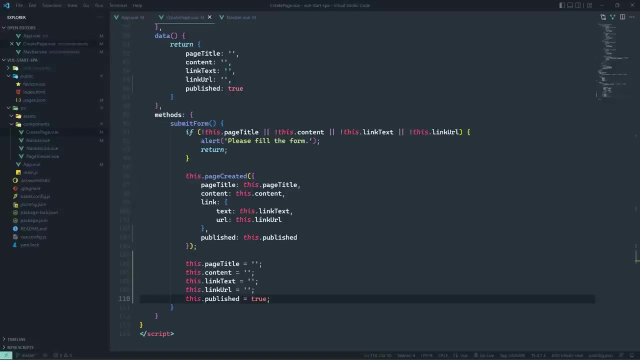 Well, in the next lesson, I think I want to make this a little bit easier for the end user because there is a relationship between the page title and the link text. A lot of times they are going to be the same. So it would be nice that as we type into the page title that we see the link text automatically update. But of course, it's not going to be as simple as that because nothing ever is, but it'll be a nice feature nonetheless. 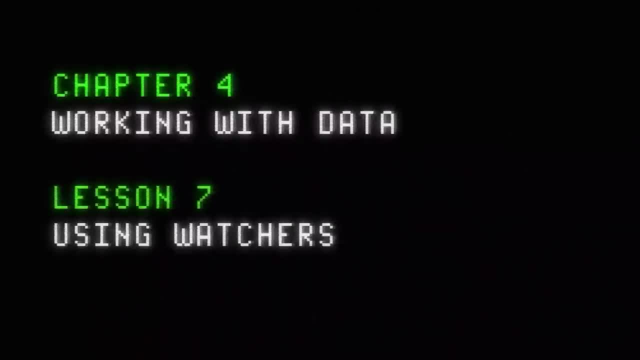 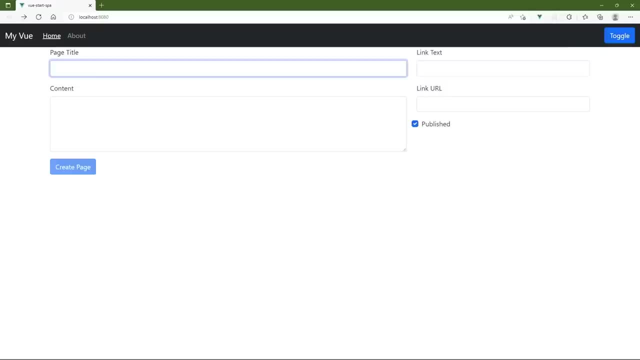 In this lesson, we are going to enhance the user's experience as they create a page. And the reason is because there's almost a one-to-one relationship between the page title and the link text. For the majority of pages, they are going to be the same. So I want to do this. As the user types into the page title, I want those characters to be automatically replicated in the link text field. So that for the vast majority of pages, the user doesn't have to type that value. That would be a huge production boost. 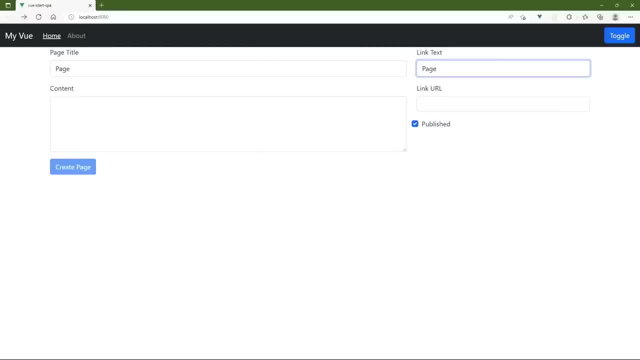 And as a software developer, it is my job to empower the user to get the work done that they need to get done. 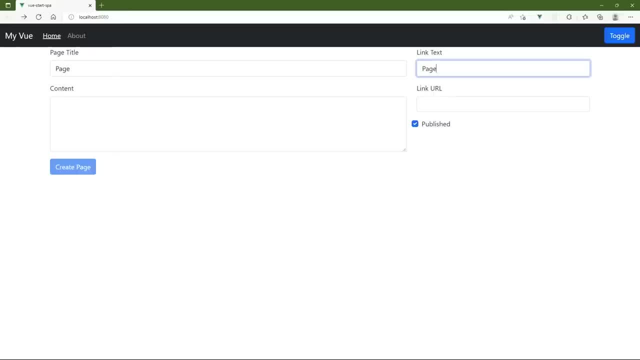 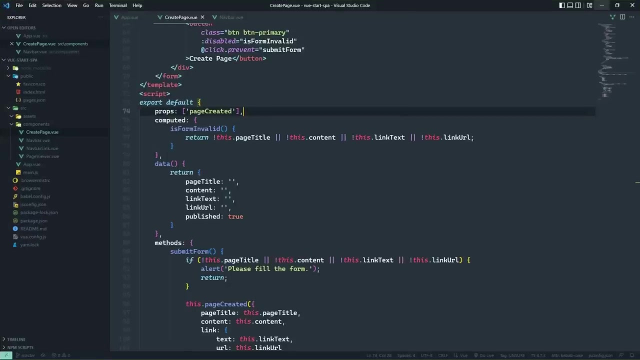 However, it can't. it can't be that simple because not every link text is going to be the same as its page title. So in the case of when the link text is different, we need to be able to preserve that value so that when the user updates the page title, that isn't reflected in the link text. So this sounds rather complicated, but in actuality, it's very simple to implement. 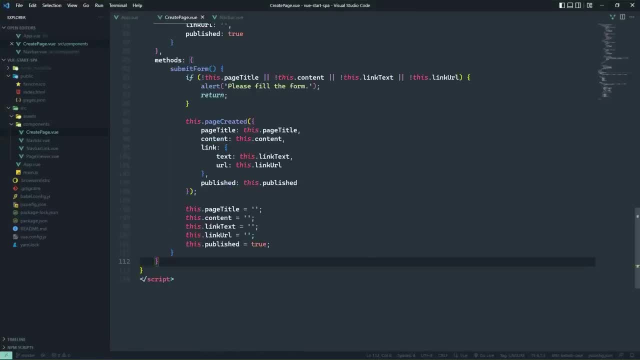 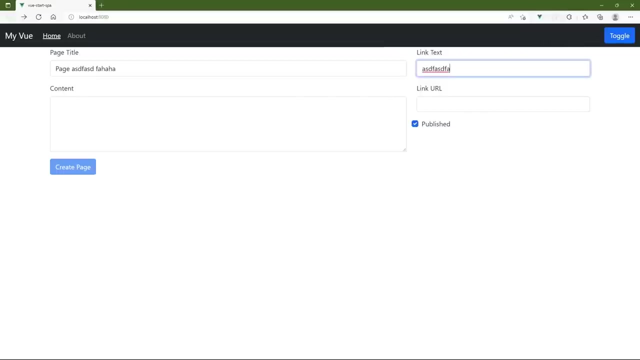 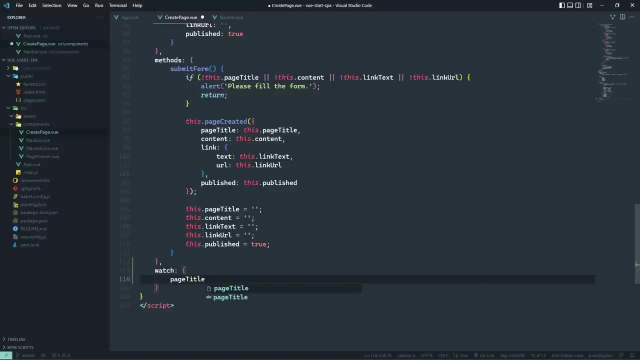 We are going to use what's called a watcher. To add a watcher, we need to add the watch option to our component. And then we create a method that has the name of the value that we want to watch. So in our case, we want to watch the page title because that is what the user is going to be typing. So when the value of page title changes, this watcher is going to execute. And it's going to give us access to the new title value as well as the old title. And this is really all that we need to do. 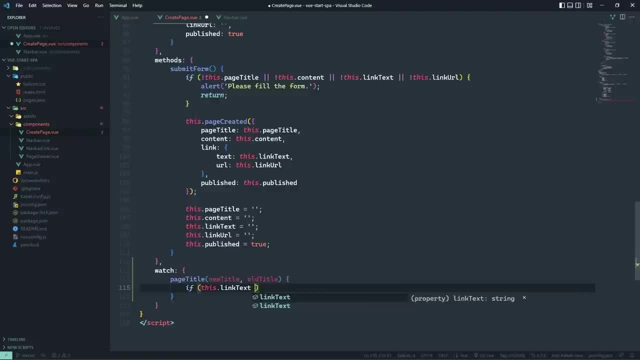 We need to check what the link text is. We need to see if it is equal to the old title. Because if it is, then we know that the user hasn't changed the link text. So in this case, we would then update the link text to the new title. However, if the user changed the link text, then of course it's going to be different from the old title, in which case we don't do anything at all. So we can go back to the old title. We can go back to the browser, and we can test this out. 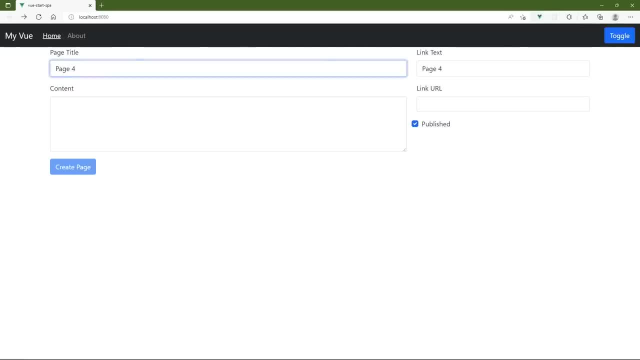 So as we start typing into page title, we can see that the link text is automatically updated. 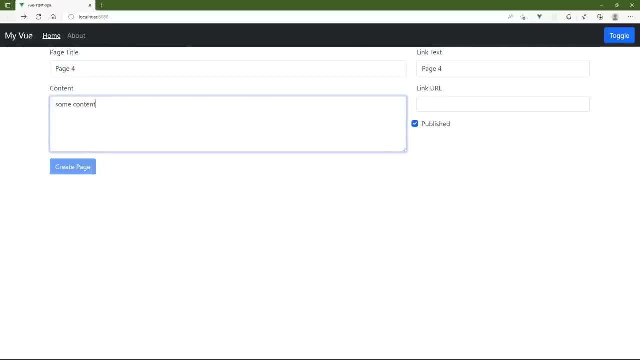 This is going to save us a whole lot of time so that we can add some content. Then we can add the URL, and then we will be done. 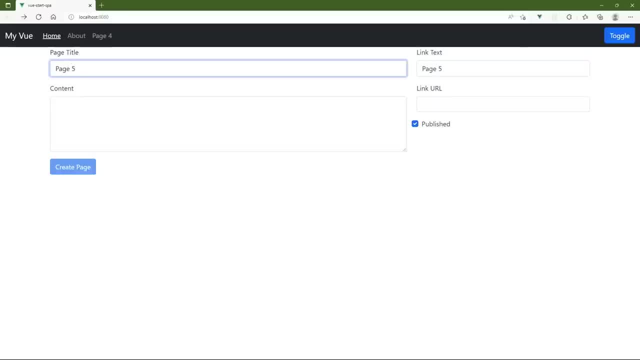 So then we can start adding the fifth page. 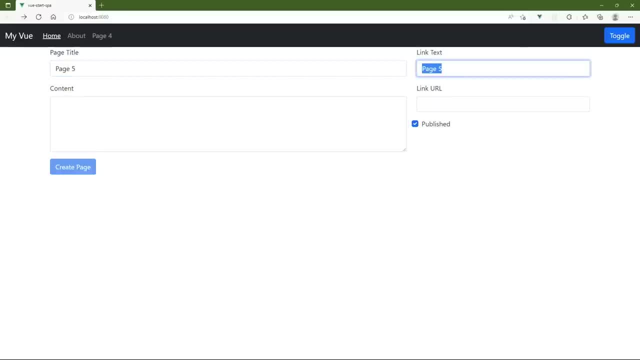 But the user might decide, okay, I want a different value for page five. Or at least this is for the link text. So this is going to be. Some page, but then, yeah, I don't want the page title to be page five. This will be something completely different. And notice that the link text is staying the same value. 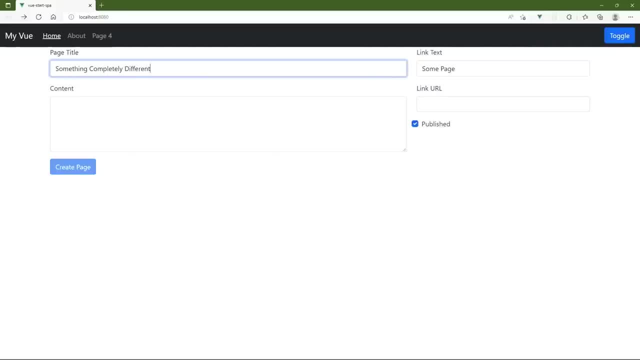 So we have the functionality that we want. And we could even take this a step further by doing something with the link URL. There are so many different ways that we could approach that. We could take the link text, we can make it all lowercase, replace the spaces with an underscore, and then automatically change it. 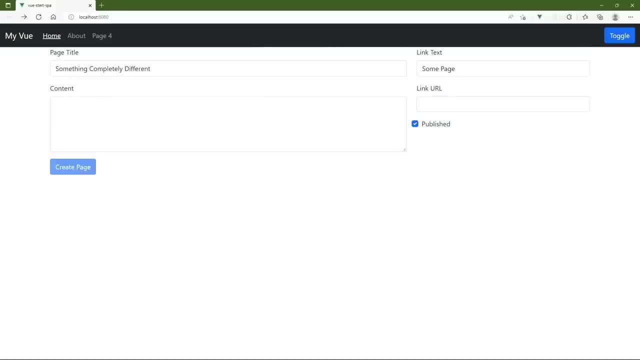 And we can automatically populate the URL. I mean, there's a lot of things that we could do to make the end user's lives a little bit easier. 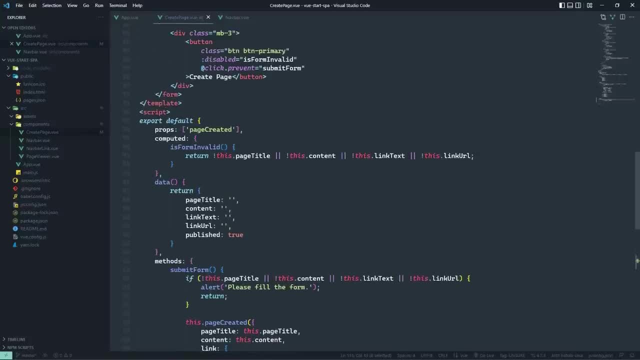 But instead of doing that, I want to talk about the differences between a computed property and a watcher, because there is a lot of confusion between the two. 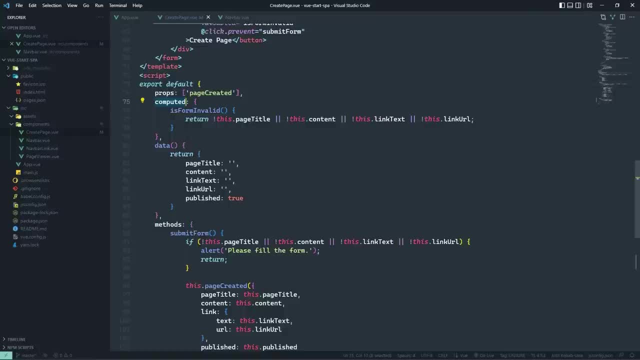 But basically, it runs down to this. Computed properties simply return a value. They use the existing data in order to compute a value that is then used in our template. 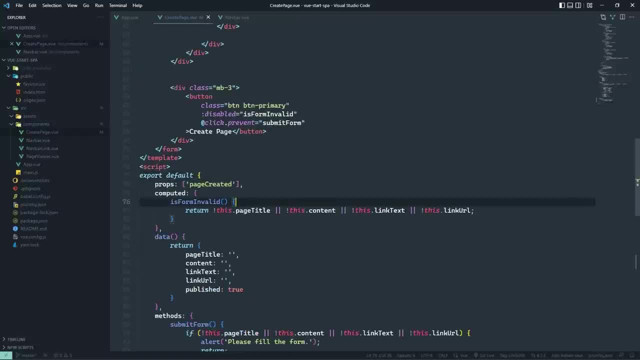 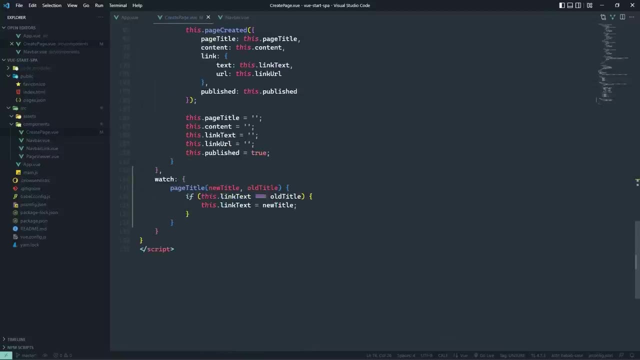 It does not change. It does not make any change to our state. It does not mutate anything at all. It simply computes a value based upon the current data. 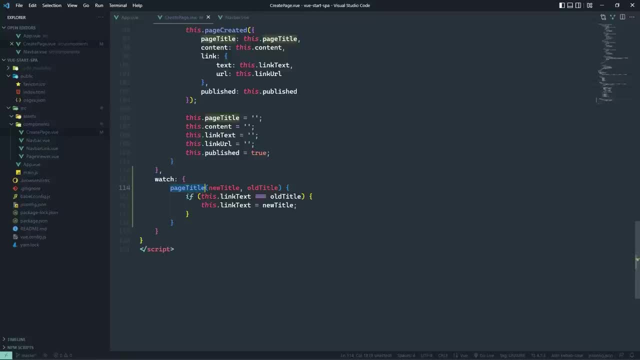 The watcher, on the other hand, watches for a property to change. 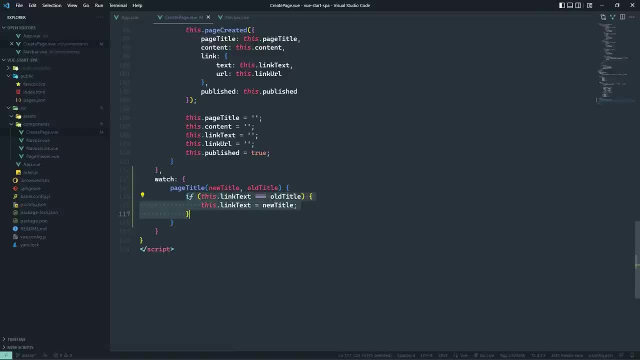 And it gives us the ability to make changes to our state. So computed values compute and return a value. Watchers watch for a value to change and allows us to mutate our state. Remember those two rules, and 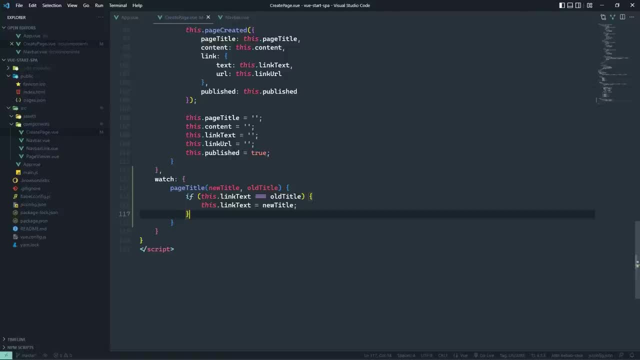 you will have no problem using computed properties and watchers correctly. 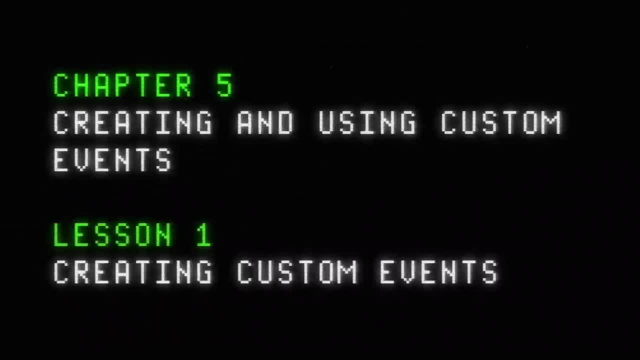 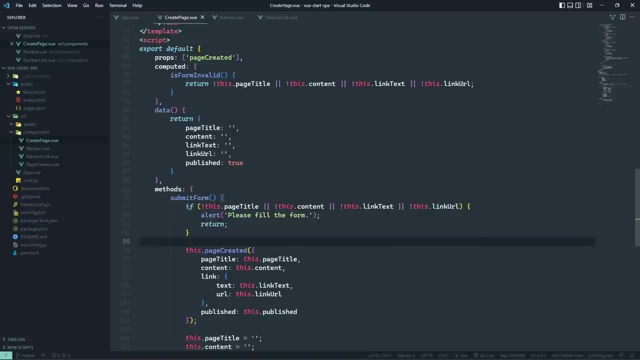 Events are the lifeblood of any application with a graphical interface. It's the primary way that we interact with users. But in the terms of our view application, it's also a way that components can communicate with one another. 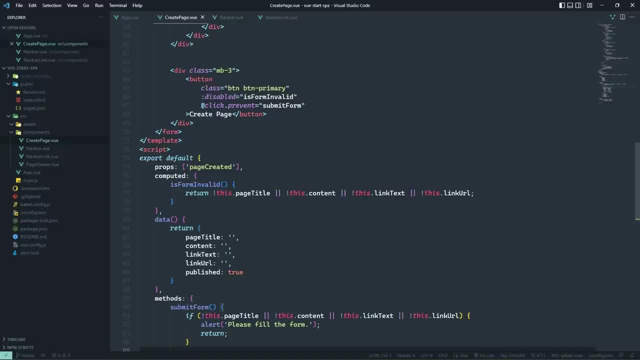 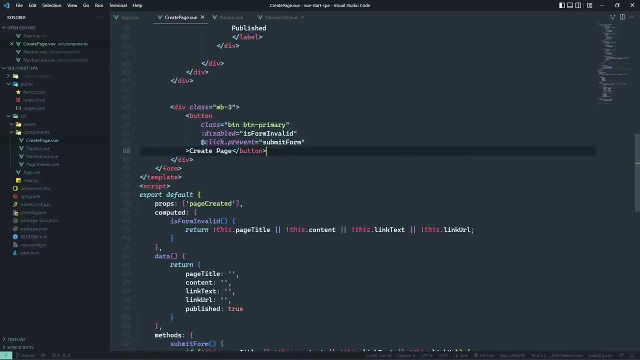 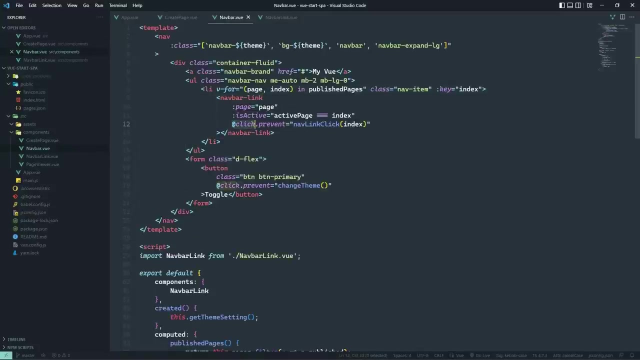 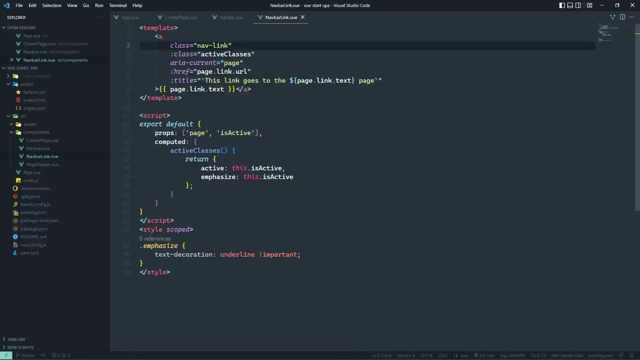 Now, technically, the only events that we have used thus far are DOM events. Anytime that we have set up the click event for a button, and even the click event that we set up inside of the navbar. We have this navbar link component where we set up the click event. Even though that's done on the navbar link, that's actually following through to the A element that is directly inside of that component. So everything so far has just been typical DOM events. 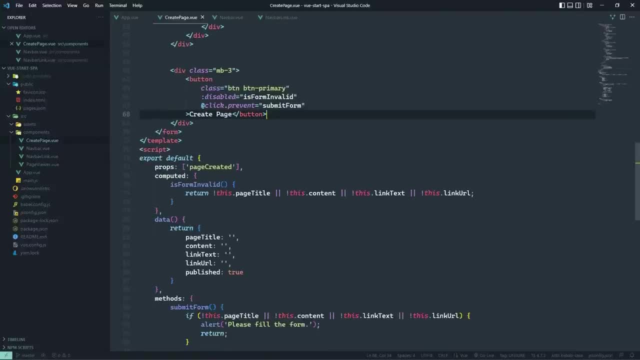 Now we have emulated events, like for example, inside of the create page components. 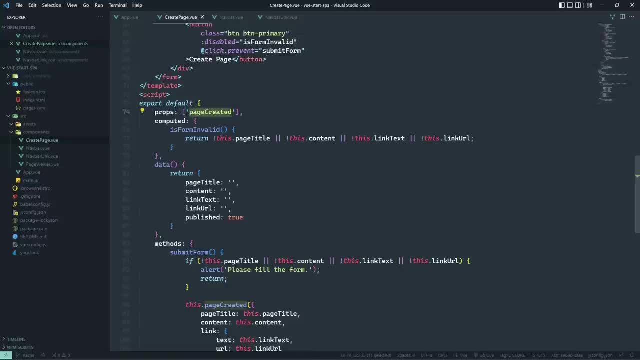 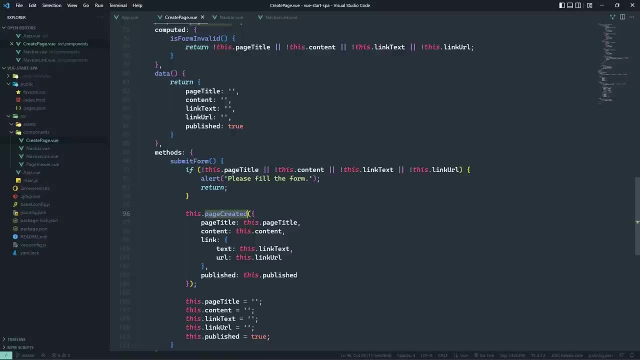 We have that prop called page created to where we bound a function to that prop. So that whenever the page object is created, we call that function and then we've emulated that event. 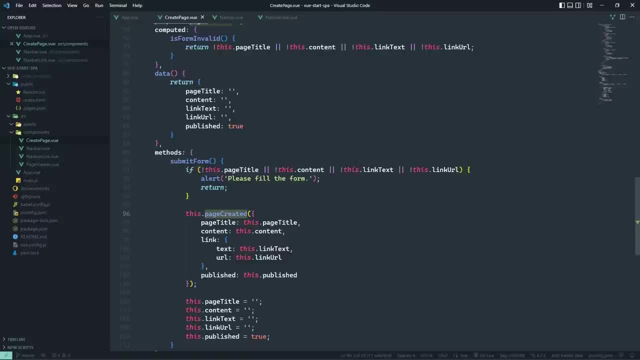 But that is technically not an event. We can, however, create our own custom events. And there are benefits to doing so as opposed to emulating them like we have done. 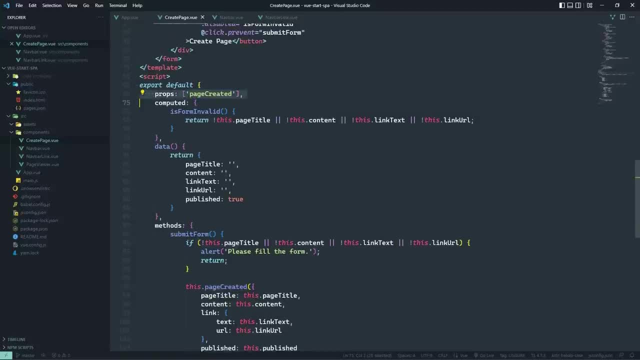 For example, we can actually simplify our component because we don't have to declare. Our events. 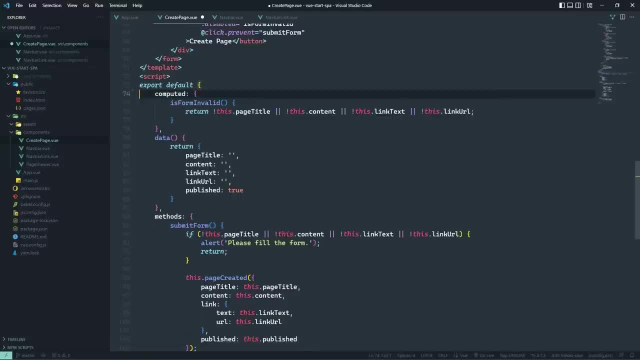 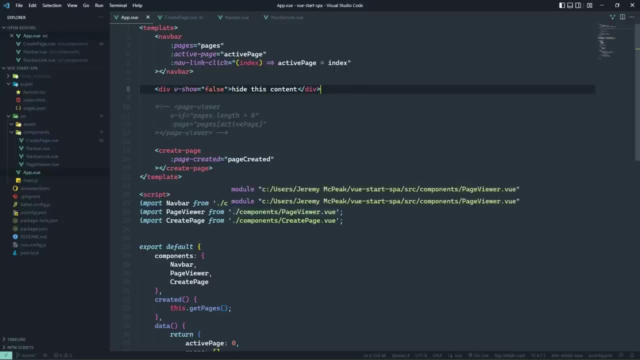 We can if we want to, and there might be some benefits to doing that. But we don't have to declare them, so that's one thing. The second thing is that it makes our code easier to read. Because let's look at our app component. So we have our navbar where we've bound a lot of data to different props. Then we look at the create page component. And we have bound something to page created. But we don't necessarily know what that is. Until we look down at the code and we see, this is a method. 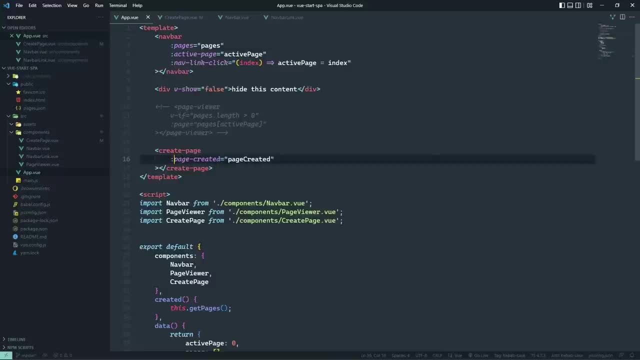 So this would be a lot easier to read and understand what exactly is going on if we were using the actual syntax for setting up an event handler. 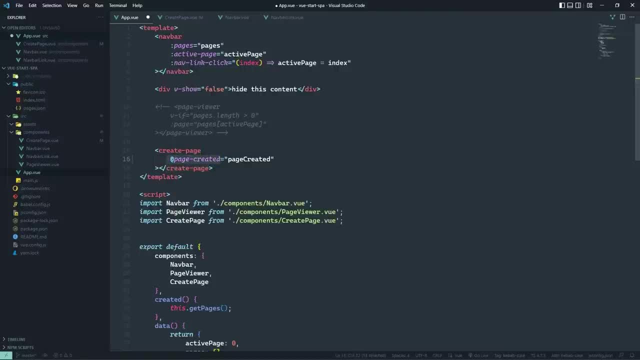 So now we have a page created event that we are handling with a function called page created. 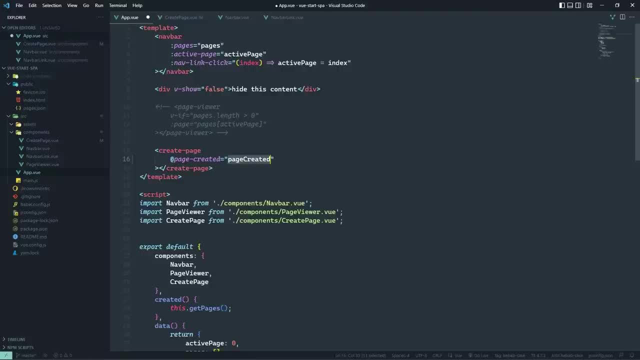 We don't have to dive into the code within our component in order to figure that out. Because it's very clear as what we are doing with just this line in our component. 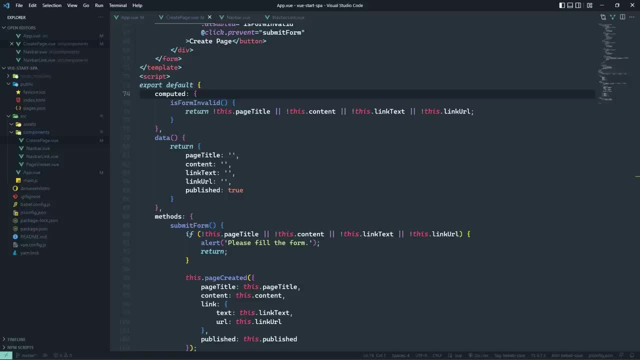 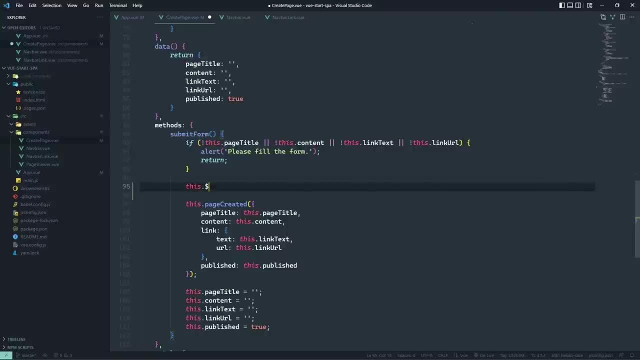 So now we just need to make this work with a custom event. And it's very easy to do, because all we need to do is emit that event. We have a special property called $emit. 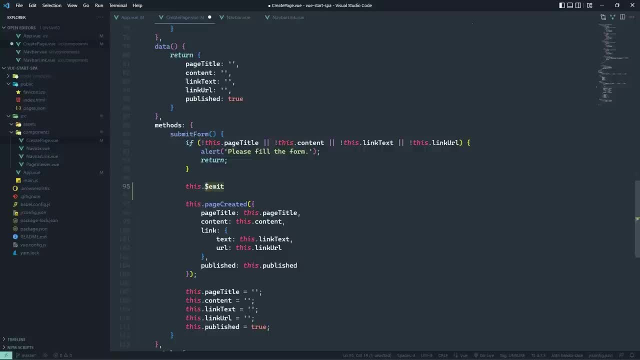 Now the dollar sign is there just to say that this is a public property. So this is something that is legal and actually encouraged for us to use inside of our components. 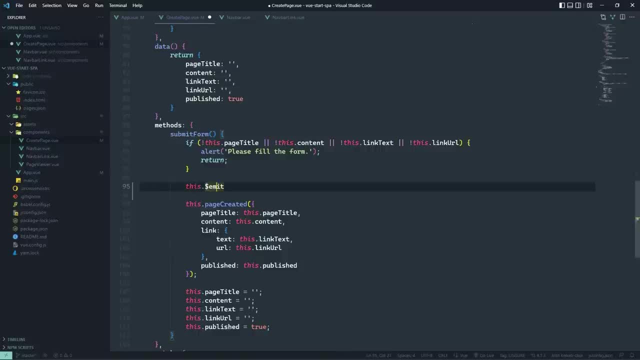 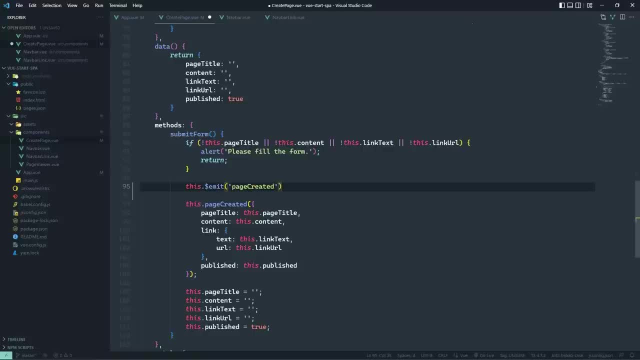 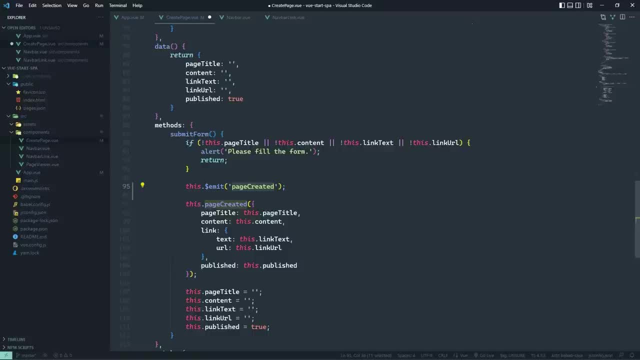 Now, there's something to notice here. I'm using camel case for the name whenever we emit this event. 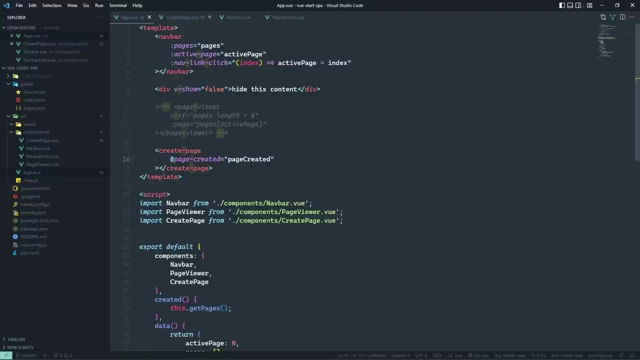 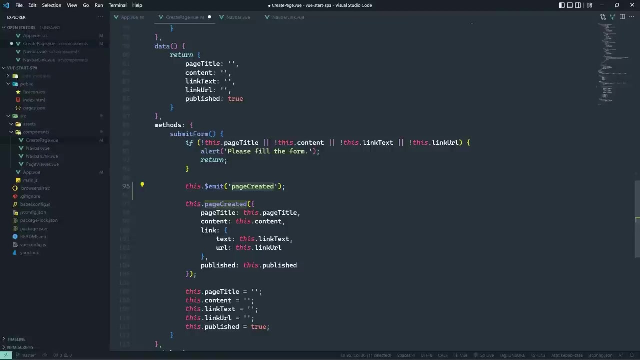 Whenever I set up the listener, I use a dash in between the page and created. So I'm following the same rules that we have for props, except that this is of course for events. So if all we needed to do is emit the page created event, then we're done. 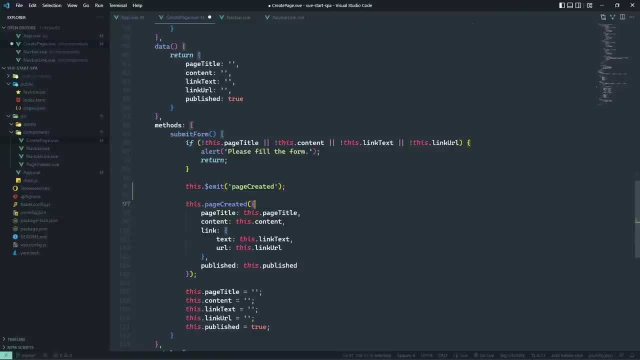 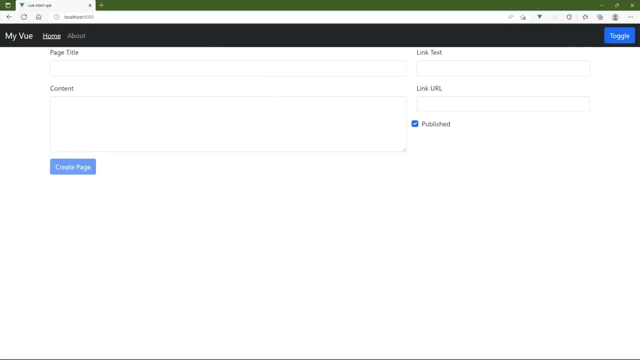 But that's not it. We also need to supply the information involved with that event. So for the second argument, we're going to pass in the object that is created when this page is created. So let's save this. Let's go to the browser and let's test this out. 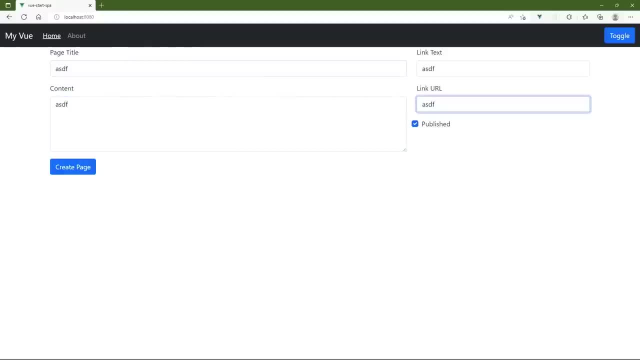 Everything else should work just as it did before. So all we need is some data inside of these fields so that we can click on create page. And there it is. 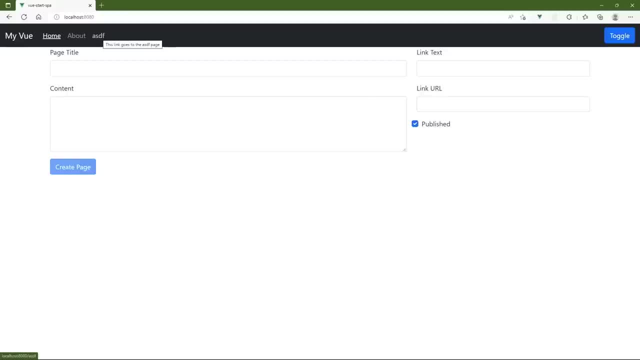 There's the page that we just created. And because we see this here, that means that the page created event occurred and the app component handled that event just fine. 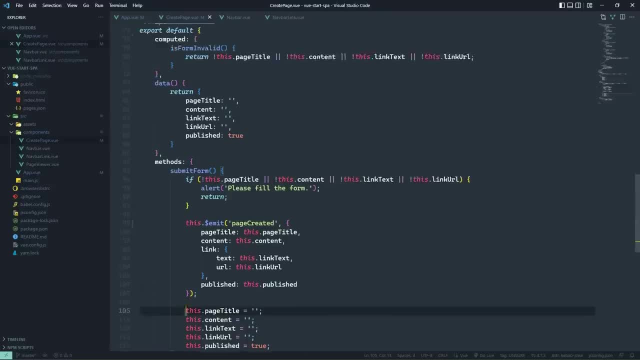 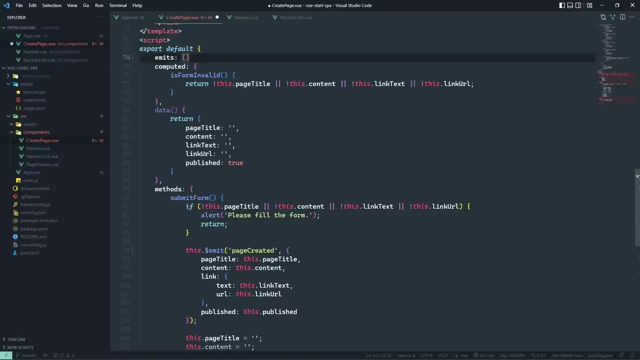 Now, I said that we don't have to declare our events inside of our components, but we can if we want to. And there are benefits to doing so. So first of all, the easiest way to declare an event is to use the. Emits option, and this is a lot like the props to where we can supply an array that contains the names of the events that we emit from this component. 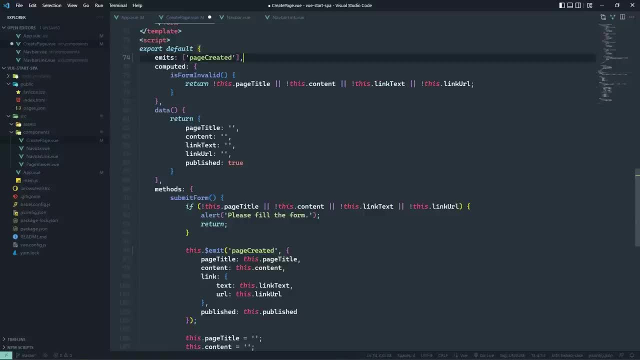 So page created, and that would be the easiest thing that we can do. 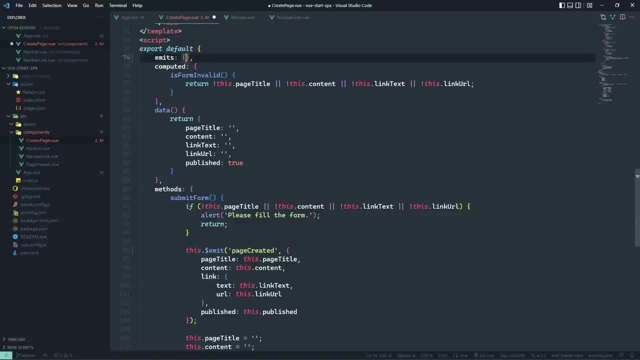 We can also set up the emits property as an object so that we can perform validation for our events. 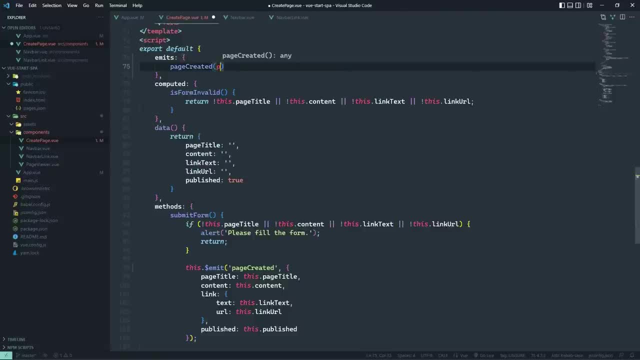 So, for example, the page created event needs to. Support. The page object that was created. 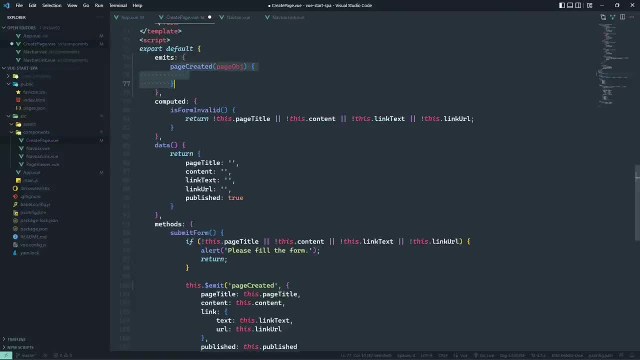 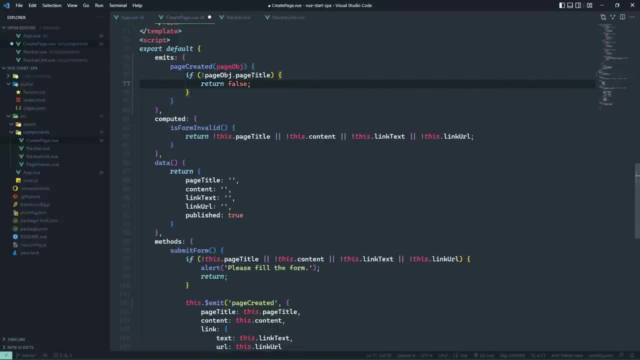 So inside of this method, we can write the code that will validate the payload that we are sending through the page created event. So, for example, if we check if the page title is not there, then we would want to return false because the validation of that object failed. It should have a page title. And if we. 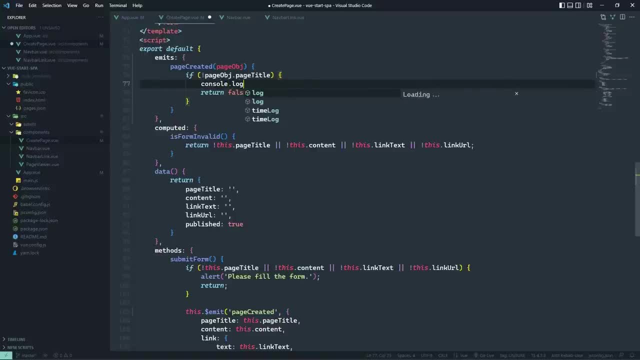 Needed to supply any information, we could do that by just writing something out to the console, or we can look at the console in the browser. 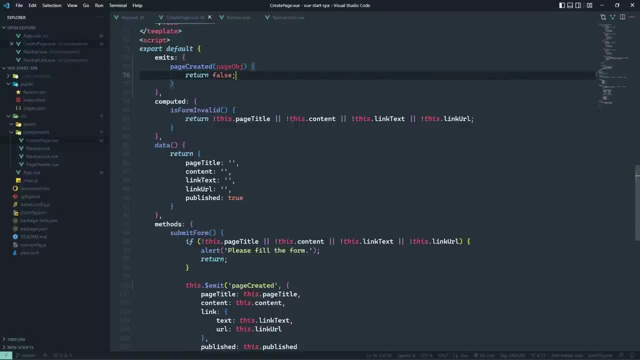 So let's just return false. Let's say that regardless of what we pass for the page created event, it's not going to pass validation. 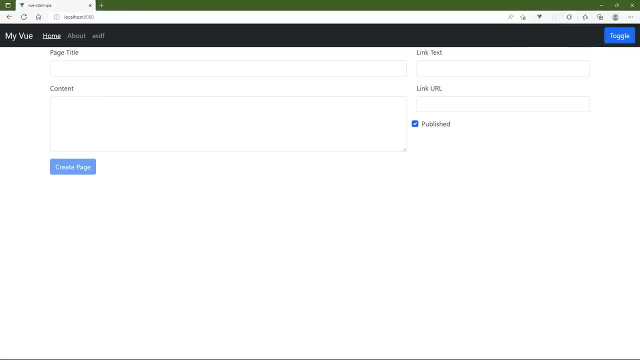 Now, this isn't going to prevent our code from executing. As you'll see, let's refresh so that we start out with a clean nav bar. 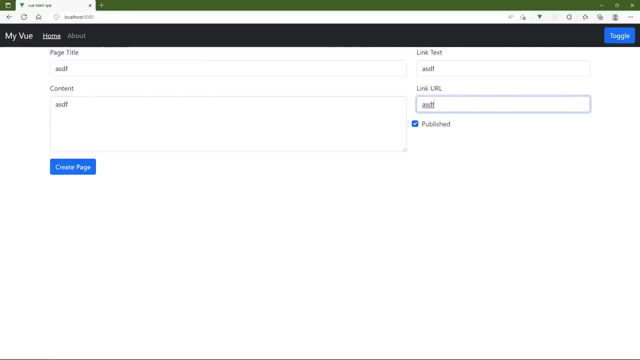 Let's add a new item. Let's pull up the developer tools so that we can. View the console. We'll click on create page. 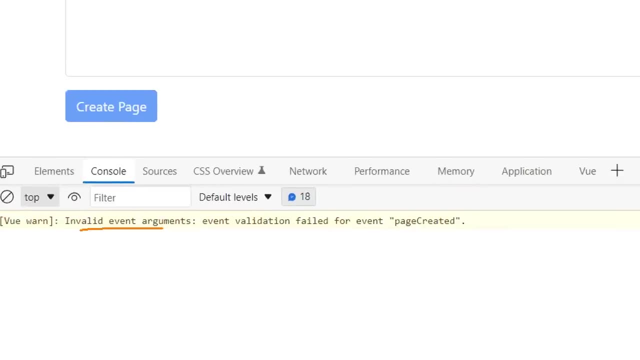 Now, we'll see this warning in the console invalid event arguments and that the validation failed because we returned false in our validation code for the page created event. 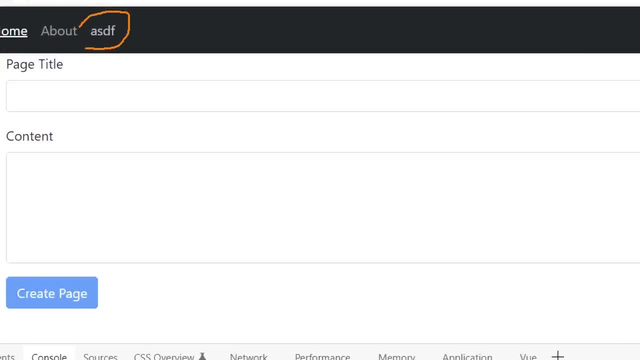 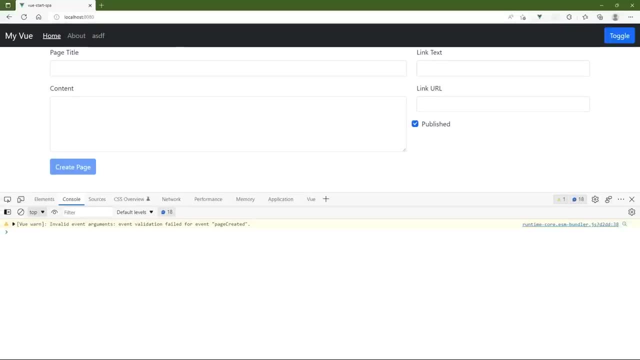 However, look at the nav bar. There is the object that we just created, so it's not going to prevent our code from working, but it does give us the ability to validate those objects that we include. 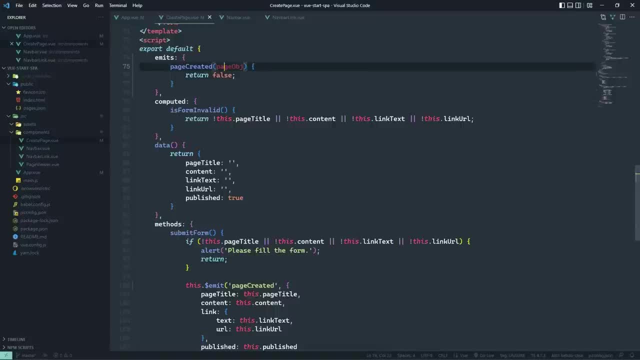 With an event. So let's do that very quickly. 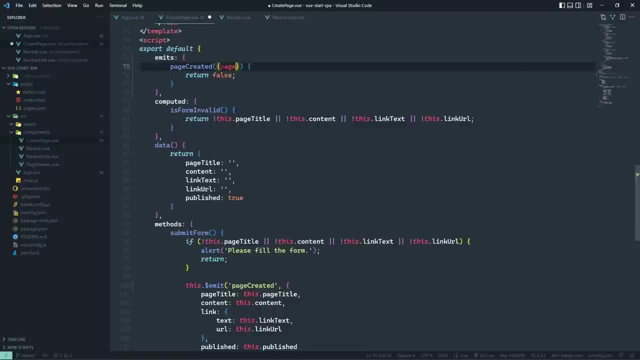 Let's break this page object into the different pieces so that we have the page title. We have the content and then we have the link. And we also have published, don't we? So we have four pieces of information. 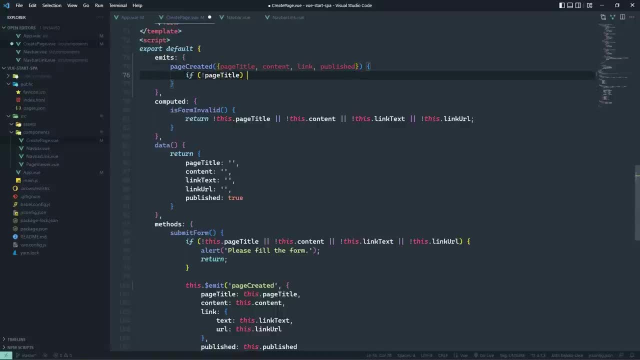 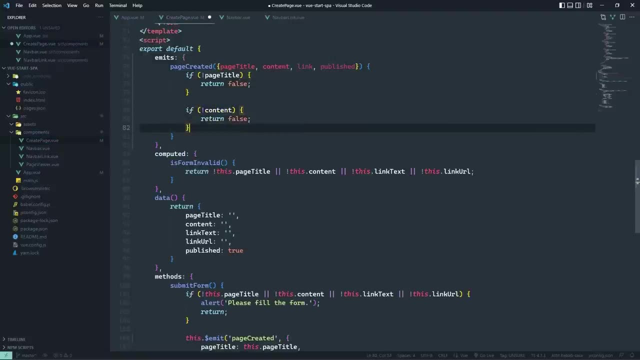 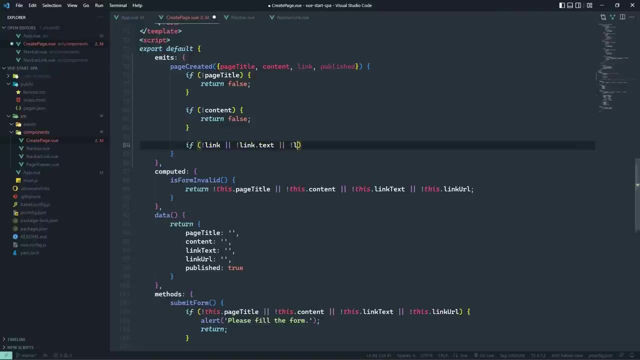 So now we can check if we don't have a page title, then we will return false. If we don't have content, then we will return false. Then we can check the link, if not link. Or if not link and what was it text or not link and URL, then, of course, we will return false. And then we can check the type of our published. So if type of published is not Boolean, let's not do that. Let's just leave published alone. So if everything else passes, then we will just simply return true. And there we go. 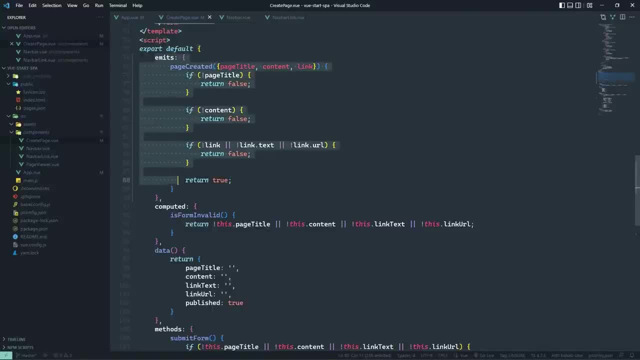 Once again, this is 100 percent optional. You don't have to declare. 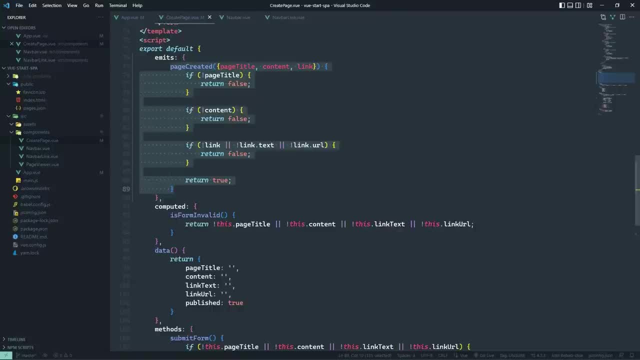 Your events, you don't have to validate them, but the ability to do so is there. And it can definitely make it easier as you develop your applications and as you are debugging them. 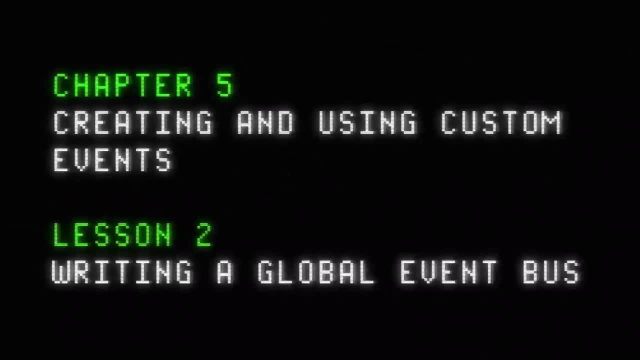 The ability to create custom events is a fantastic feature, and it's one that you will use in the majority of your applications. But there are some limitations and probably 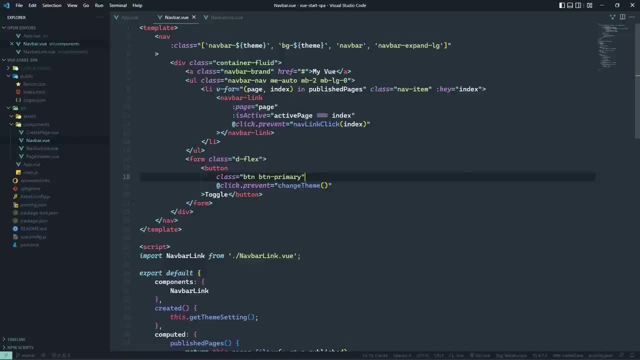 the most cumbersome is that component emitted events do not bubble. 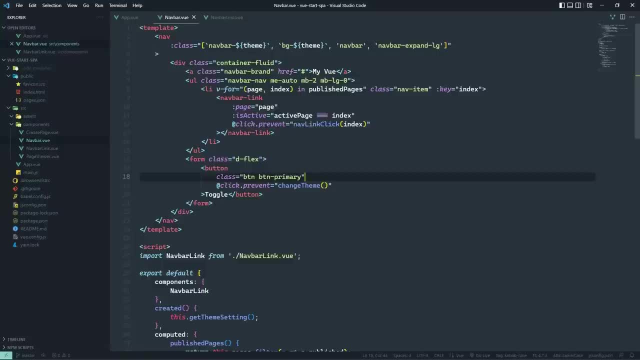 But what do I mean by that? Well, let's just think about normal HTML and JavaScript. Let's forget about view for a minute and let's say that we click on a button. Well, that is going to generate the click event and the target of that event will be that button element. But the event doesn't stop there, at least by default. It's going to bubble up to its parent, which is the form element. Then from there, it's going to bubble up to its parent, which is the div element. That will then bubble up to. 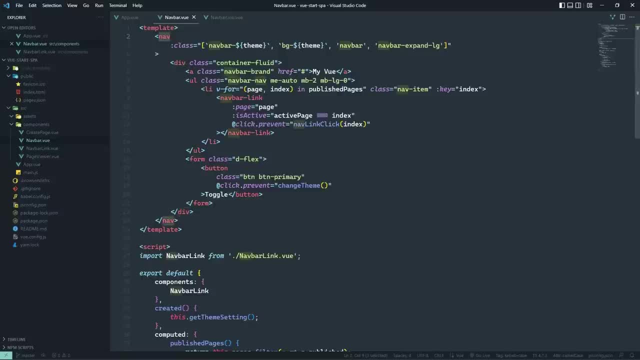 And it will keep bubbling up till it reaches the top of the element hierarchy. And the fact that events bubble gives us 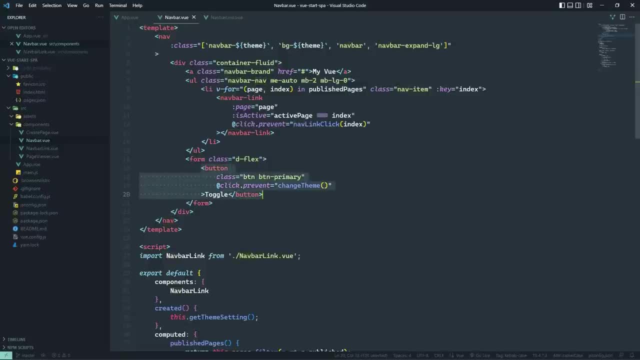 the ability to trigger an event on an element. And then we can listen for that event higher up in the hierarchy. 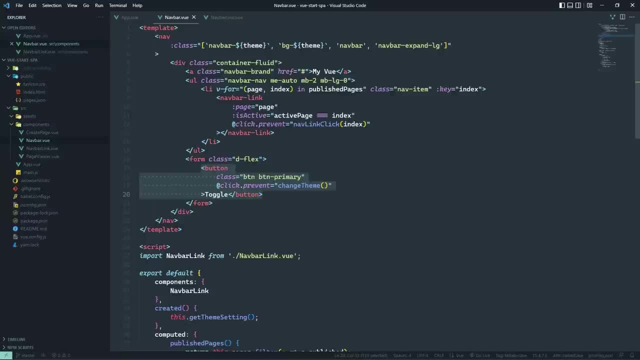 So now let's think about a view component. Whenever you emit an event from inside of a component, that event can only 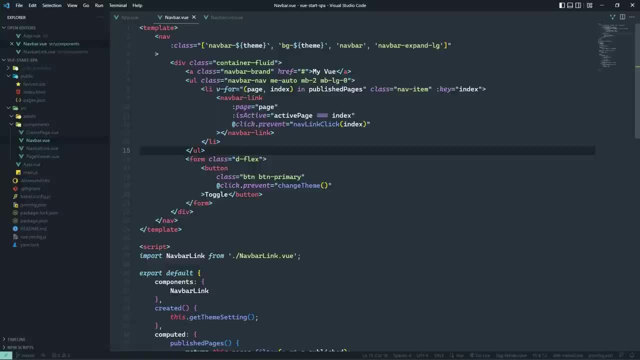 be listened for inside of the direct parent. It does not bubble up the component hierarchy. 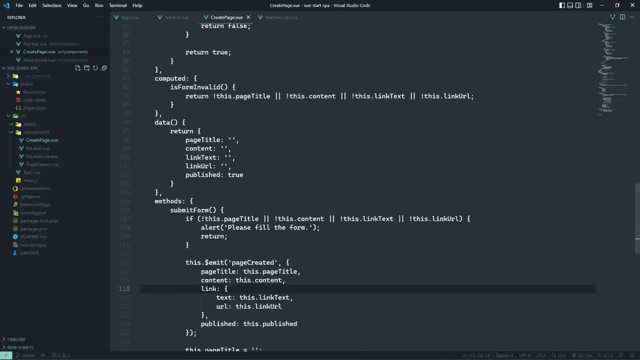 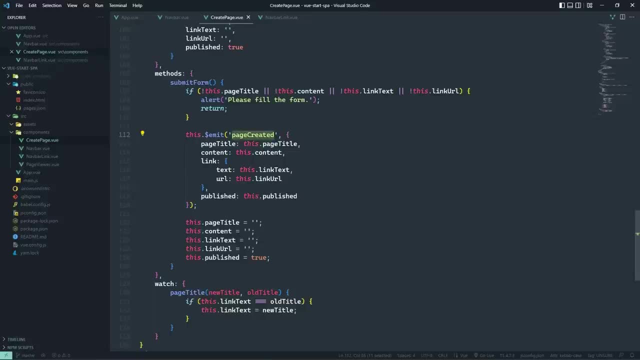 So, for example, we set up a custom event inside of the create page component where we emitted the page created event. 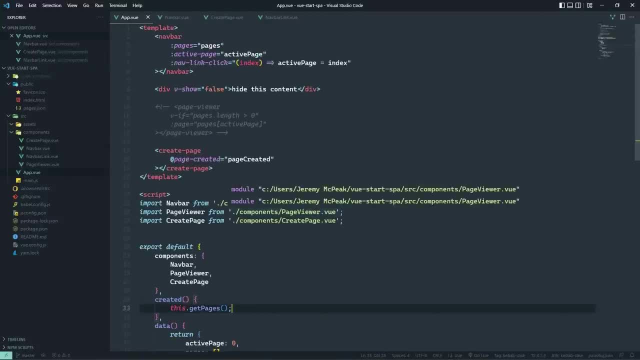 We listened for that event inside of app. Now, of course, app is the top of the hierarchy. But if there was anything higher than app, that event would not bubble up. 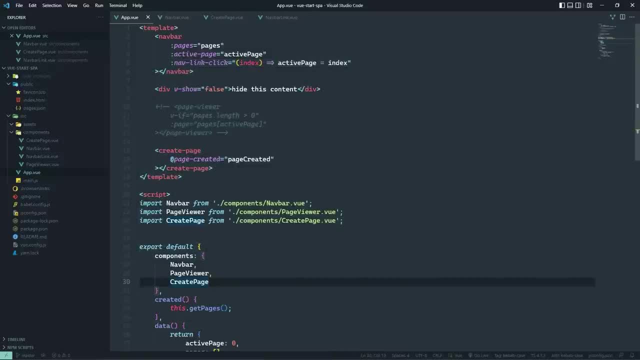 It stops here inside of the app component. And that can be very cumbersome because there are times that we need to listen 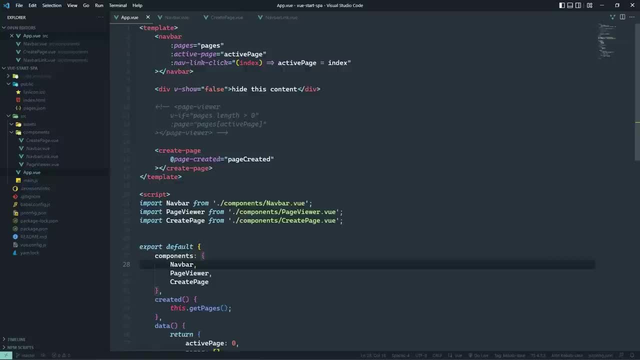 for an event that occurs deep within the component hierarchy. And there are ways that we can get around that. 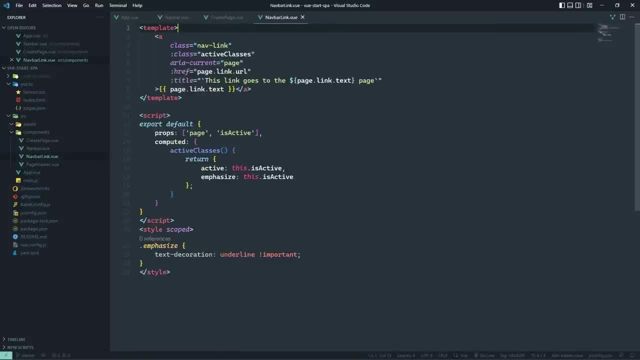 For example, I'm going to refactor our navbar link here so that inside of the navbar link, we have the li element. 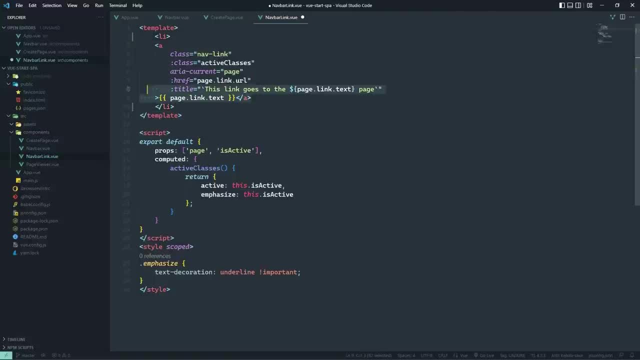 So we're going to generate that here inside of navbar link instead of inside of navbar. I think that it makes more sense in that case. 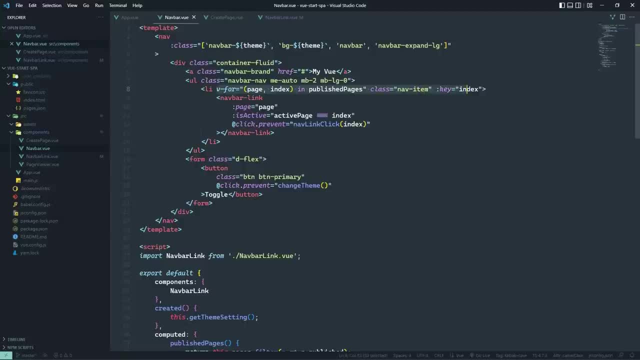 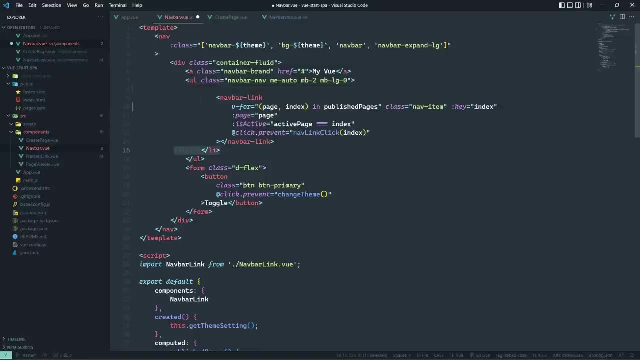 That means that we need to take the for loop and all of the other stuff and place that on navbar link, we can get rid of this li element. 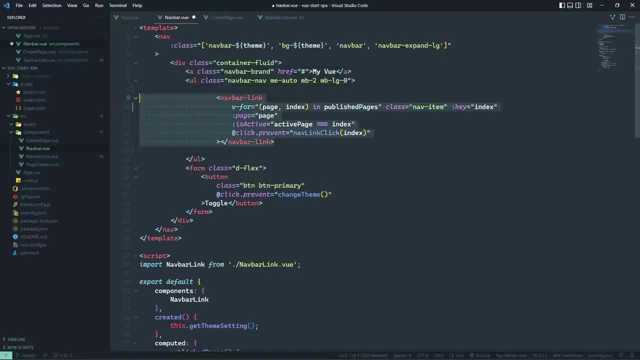 And for the most part, that's going to work just fine. 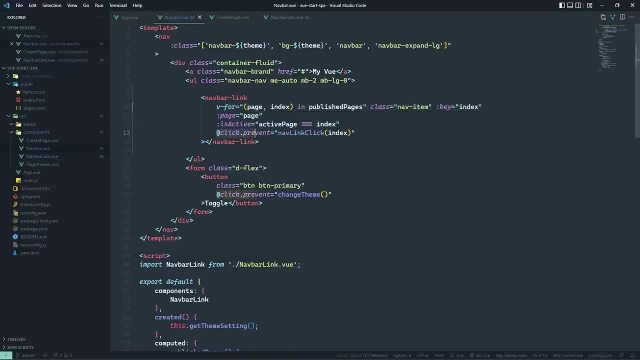 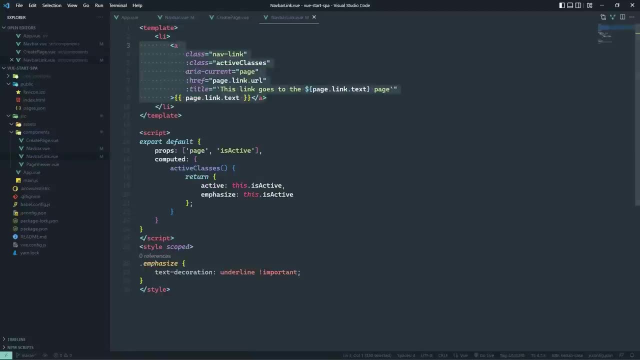 However, now I'm going to say that it really doesn't make sense to listen for any kind of events here on the navbar link. Instead, we would want to emit an event from inside of navbar link so that whenever we click on the link, we will set up the event listener to emit an event which we can call simply activated. 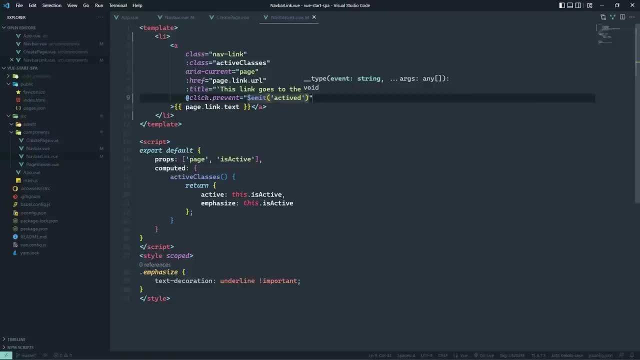 But in this particular case, the only component that needs to know that this link is activated is actually our app component, because that is where we actually do something. 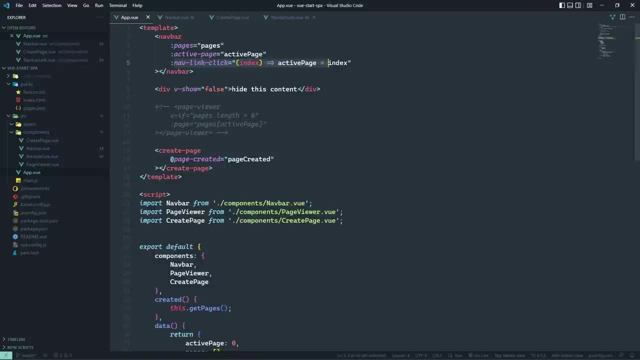 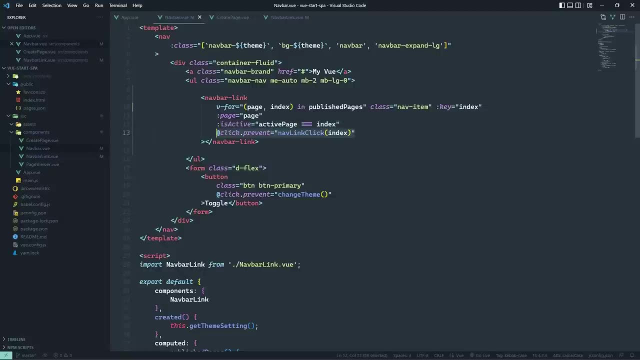 So in order for the app component to know that the activated event occurred, we would have to chain events so that inside of the navbar, we would listen for that activated event, but then we would emit something else. It could be called activated or it could be called something else. And then we'd have to pass on that 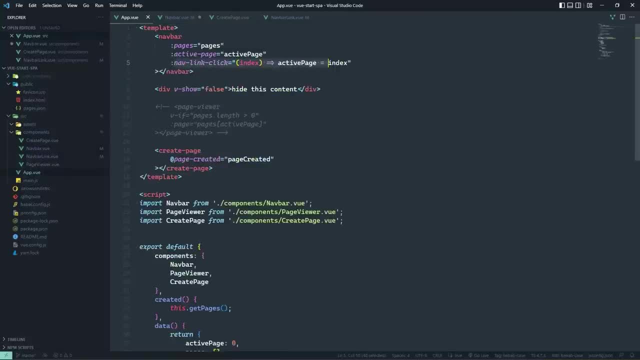 information so that then we could listen for it inside of app. 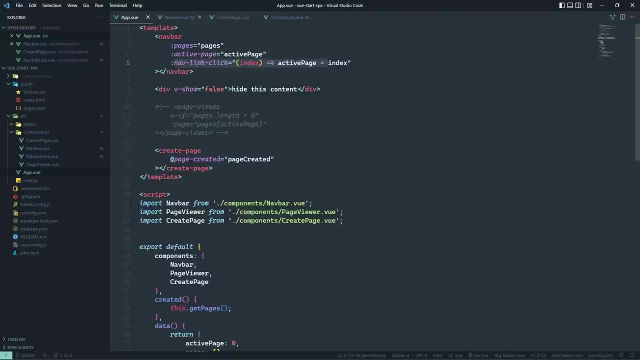 It works, but it's very tedious and it makes our code much more complex. It also makes it much more difficult to understand at a glance. Because we have to follow the chain of events. 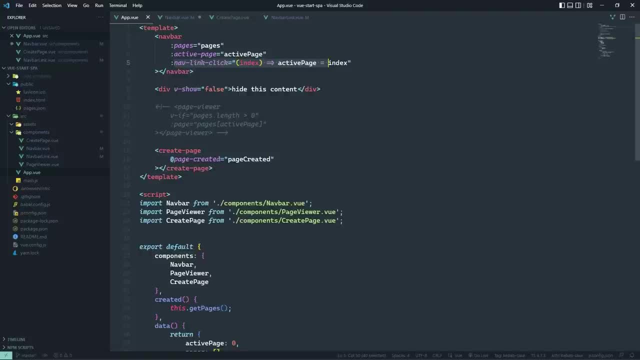 So in prior versions of Vue, what we would do is create what's called a global event bus. It allows us to essentially emit events globally so that we can emit them from any component and listen for those events inside of any other component, regardless of the relationship between those components. The problem now is that with Vue 3, we don't really have that ability. 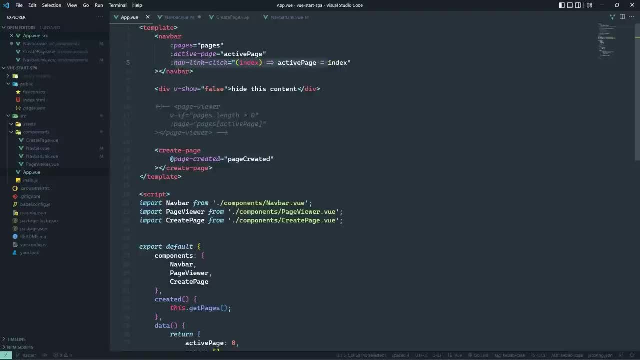 We have to write a lot of extra code in order to make our own global event bus. 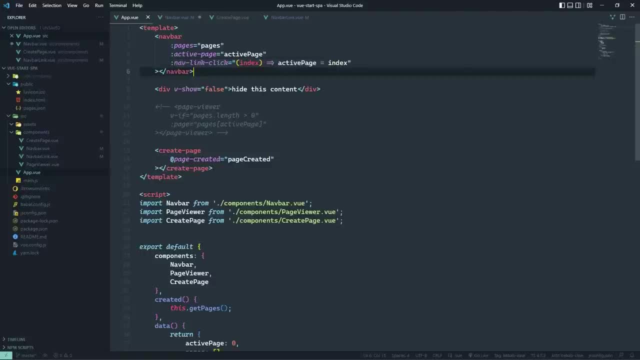 And it's frustrating to me, at least, because this was a pattern that was very commonly used in Vue version two. 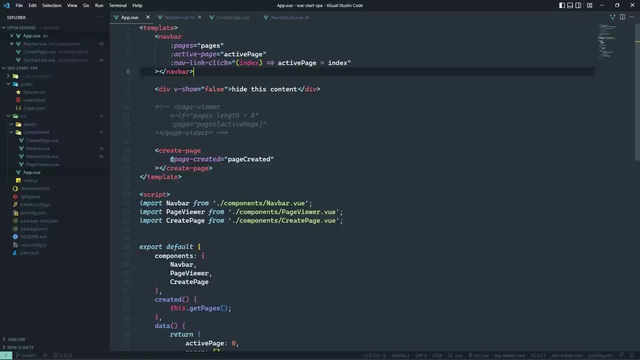 And I would have liked to have seen something like this built in. But with just a little bit of extra code, we can write our own global event bus. 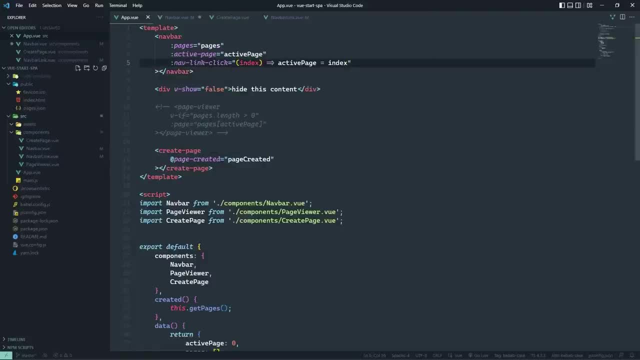 So here's what we are going to do inside of the source folder. We are going to create a new folder. I'm going to call it utils. 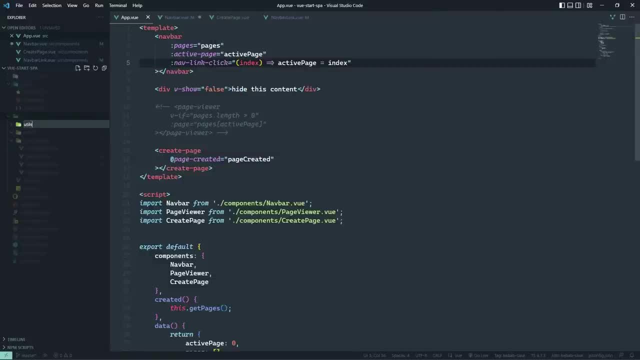 The idea being that this is going to contain some utilities that we can use within our application. 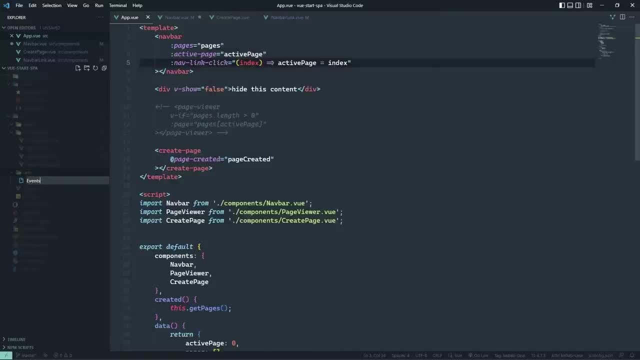 And one of those utilities is going to be called events. So we'll just call it events.js. 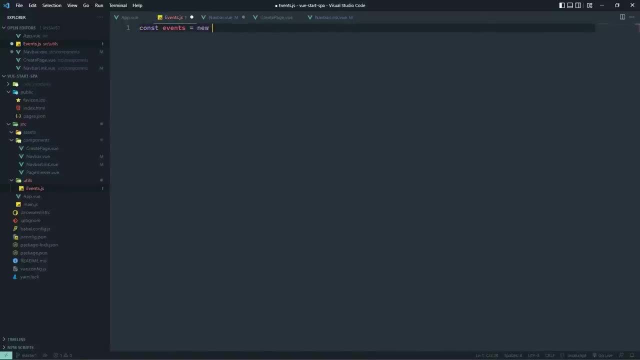 And we are going to create an object. Actually, we're going to create a map that we will use to keep track of all of our events. 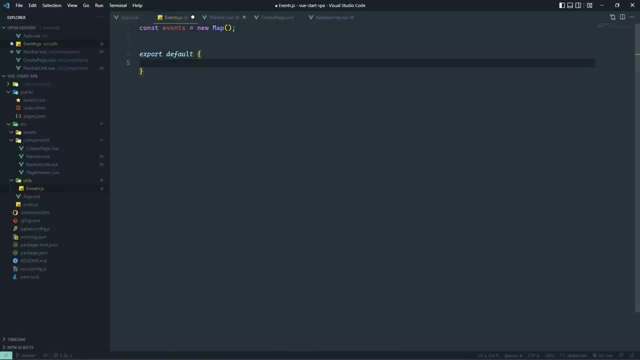 And then we are going to export an object that will have methods that allow us to set up events as well as emit them. 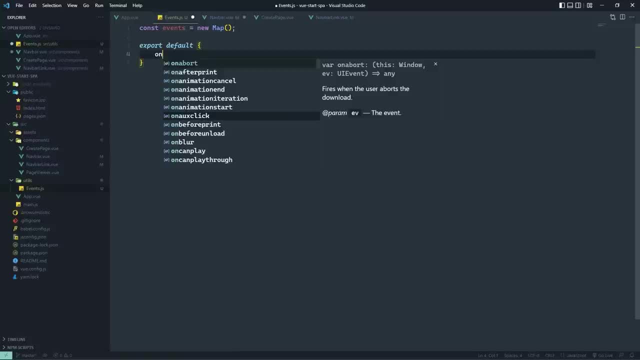 So let's start with the method that will allow us to listen for events. I'm going to call it on very similar to the idea from jQuery to where we could use the on method and then we could specify the event name and then supply the function, although in this case, let's just call this dollar on because that follows the convention that we would find inside of our Vue components. So here we want to check to see if we don't have an event with the given name. And the map object gives us this has method so that we can check if we have a key with the given event name. And if we don't, then we will create one and we'll give it a value of an empty array so that then we have an array. 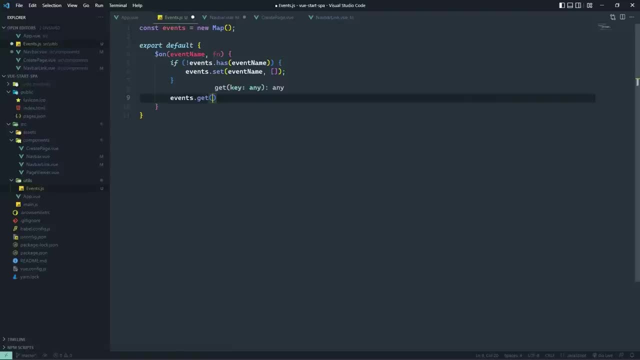 And that's how we are going to keep track of all of the functions that are set up for a given event. 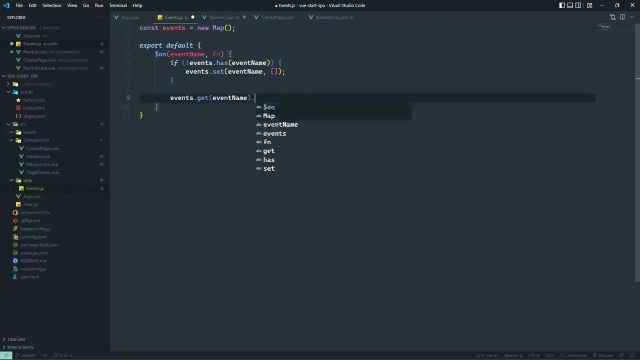 So we will get the array for the given event. And then we would push in the function that we wanted to listen for. 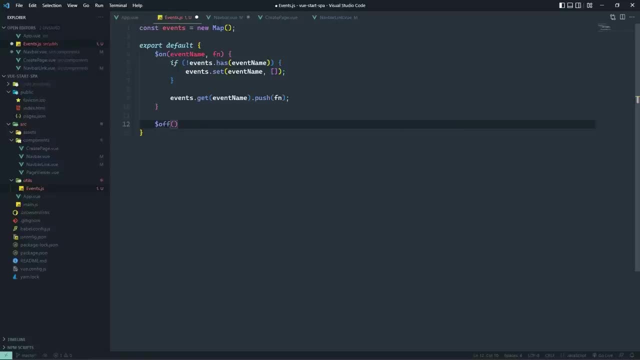 We could do something similar to remove an event, but this takes a little bit of extra code, so I'm not going to actually implement this. 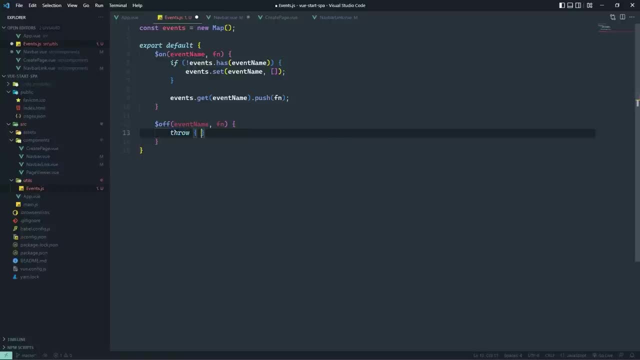 We will have this method so that if we do end up needing it, then we can implement it later. 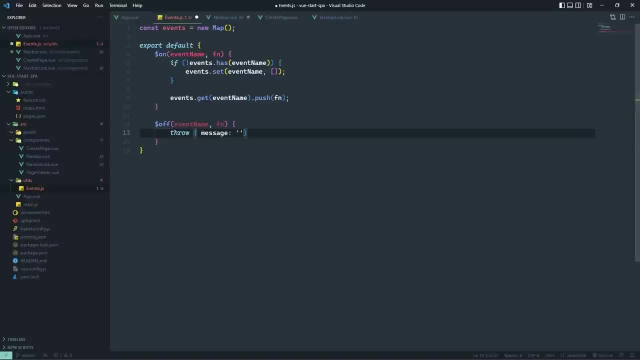 So for now, I'm just going to throw an object that has a message that says not implemented and that's going to be fine. 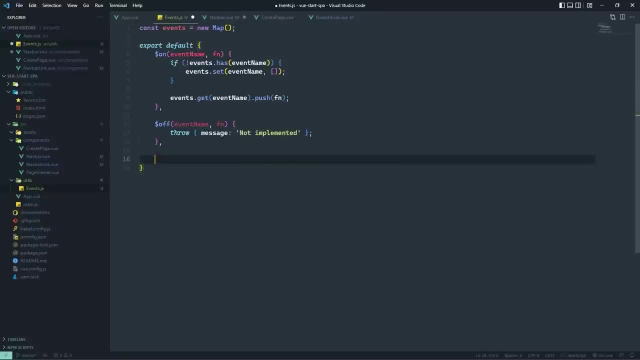 And then we need a method to emit our event to trigger it, if you will. I'm just going to use the same terminology that's used inside of you, and that is to emit an event. So we need the event name. We also need any provided data. And once again, we need to check if we have any events with the given event name. And if we do, then we want to execute all of the functions that have been set up for that event, which is very easy to do. 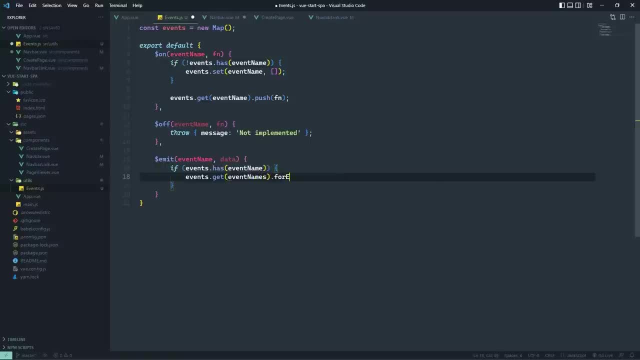 We once again want to get that array and we will simply use the for each method to where we will execute the function passing in the data. 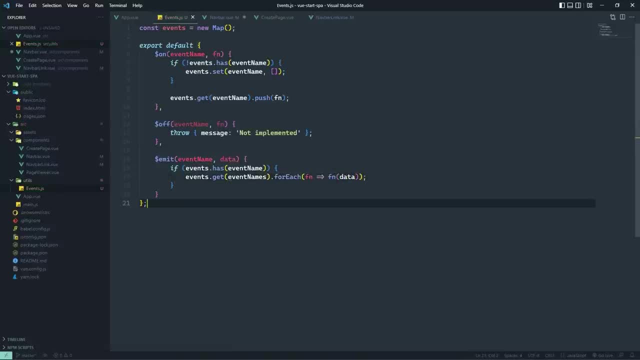 So then the question becomes, how do we add this object to our application? We want to make it very easy to use. So one thing we can do is just add it to all of the components where we want 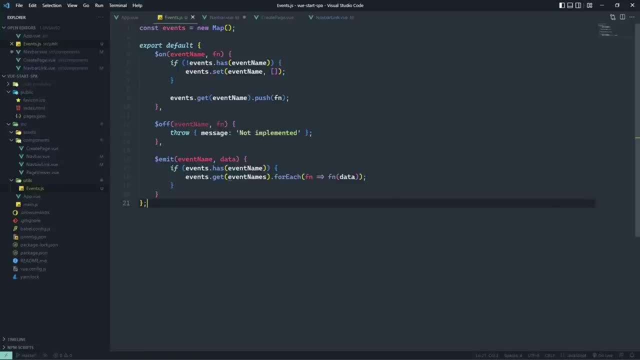 to use it and import it and all of that stuff. And no, that's a lot of work. 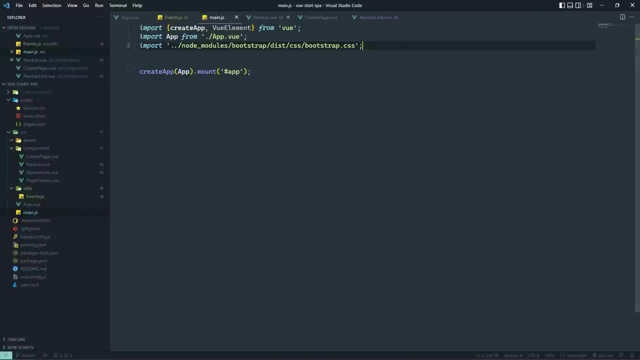 Instead, what we will do is make it part of our application so that we can use it from inside of our components wherever we want and we don't have to import it anywhere else except from inside of main.js. 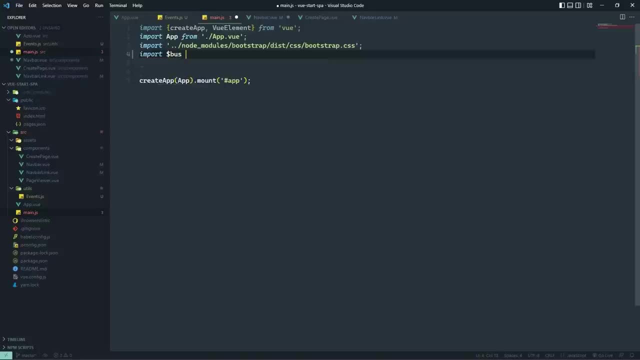 So let's import this object. I'm just going to call it dollar bus and that is from utils events. 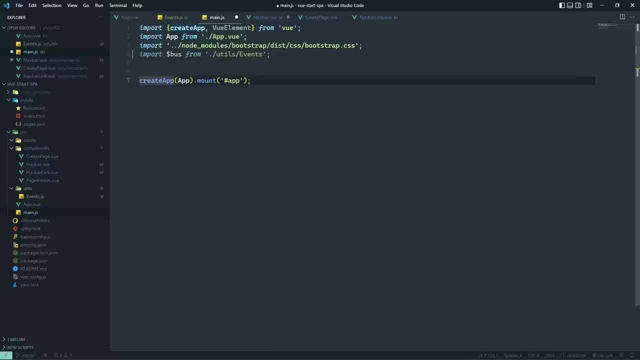 And we need to break up our line of code where we create the app and then we mount it kind of like what we did way back whenever we started this journey so that in between creating the app and then mounting it, we want to add to our configuration. There is a property called global properties, and this allows us to add properties to every component within our application. So we can call this dollar bus. 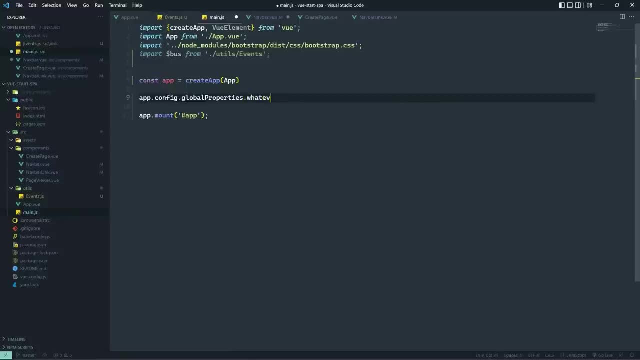 We can call it dollar event bus. We can call it whatever we want. 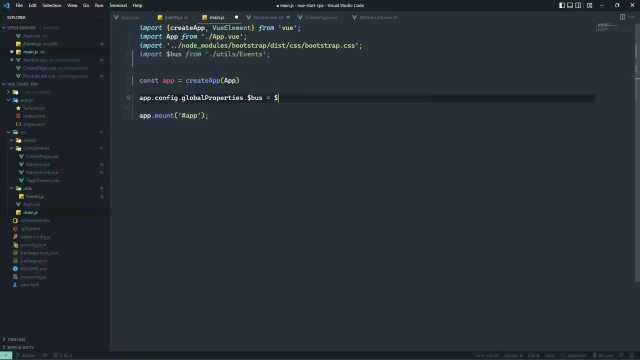 It doesn't matter, but I'm going to call it just simply dollar bus and we will assign it that value. 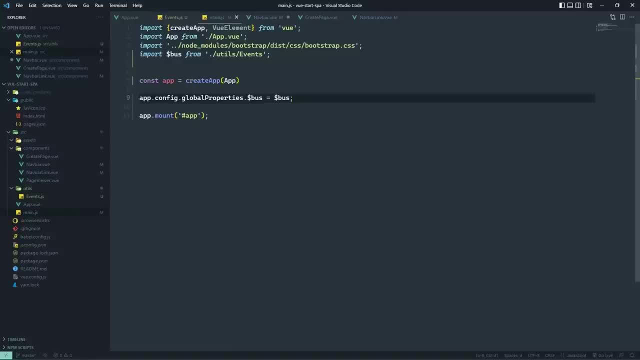 So now every one of our components is going to have this dollar bus property. So we can use our global event bus from anywhere. So that means inside of nav bar link, what we can do is use our bus. We will call the emit method and we need something a little bit more descriptive because now we are dealing with global events. 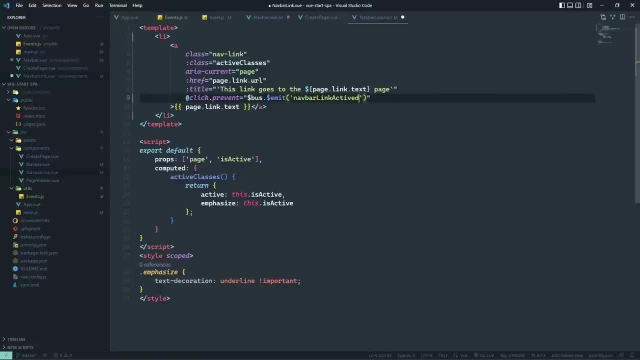 So let's call this nav bar link activated and it would be useful to provide the index, which we don't have, but that's easy enough to do. 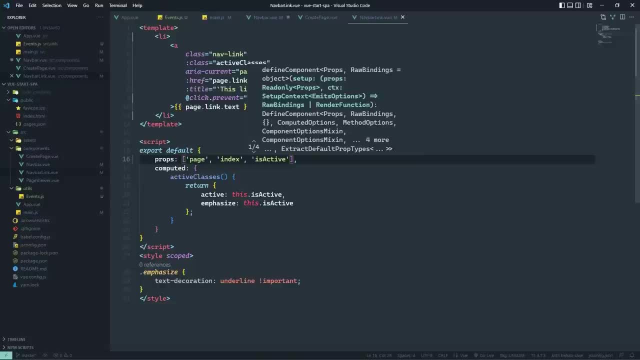 We can add index as a prop. And then inside of nav bar, we can add the index here. 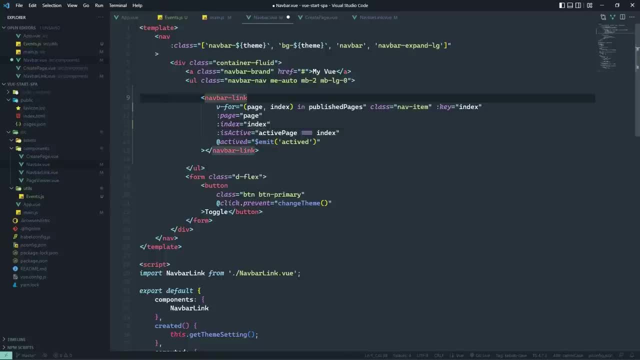 And I guess we should probably rename this from nav bar link to nav bar item, but we'll leave it like it is for now. 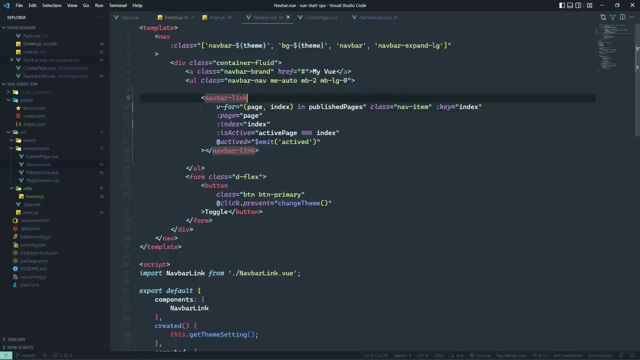 So now we just need to listen for that event and we can do that inside of app. But before we do, do we have any other code here? 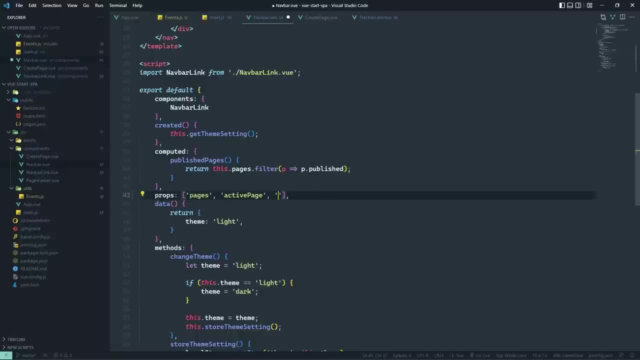 We had this nav link click prop. 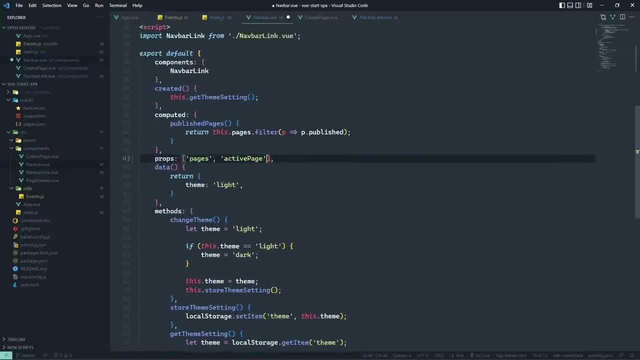 We can get rid of that, and I don't think we referenced that anywhere else. So we should be good to go. 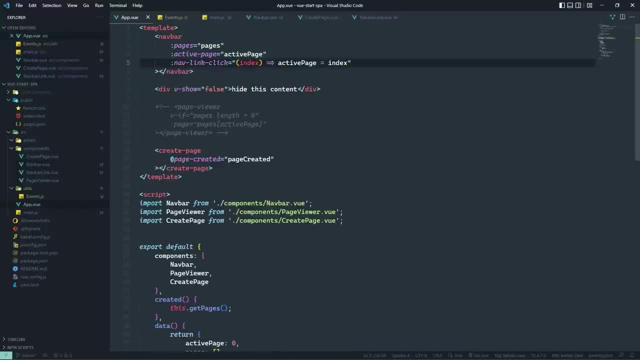 So that's inside of app. All we need to do is listen for that event. 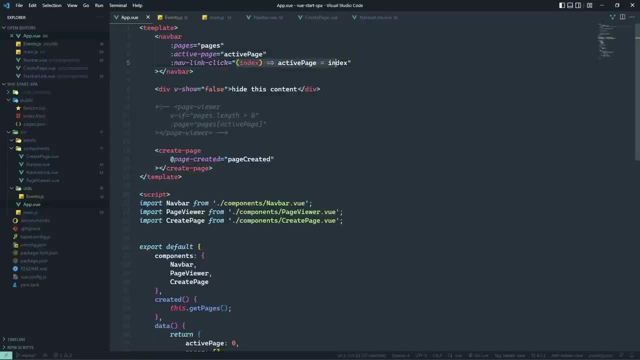 So that's what we would do is set our active page equal to the provided index. So let's cut that out. 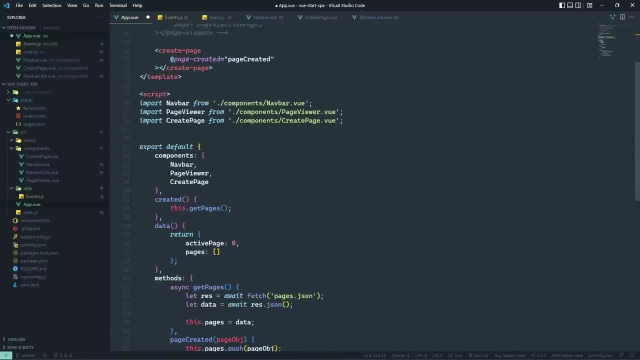 Let's get rid of this nav link click prop. And since we already have this created hook here, this would be a perfect place to listen for that global event. 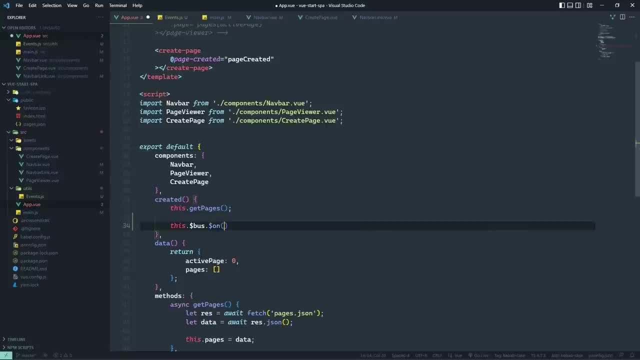 So we're going to use our bus object and we're going to listen. 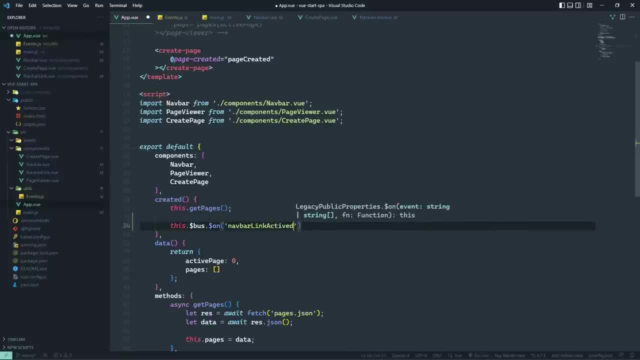 For the nav bar link activated, and this is going to give us the index so that then we can set the active page value equal to whatever the index is. 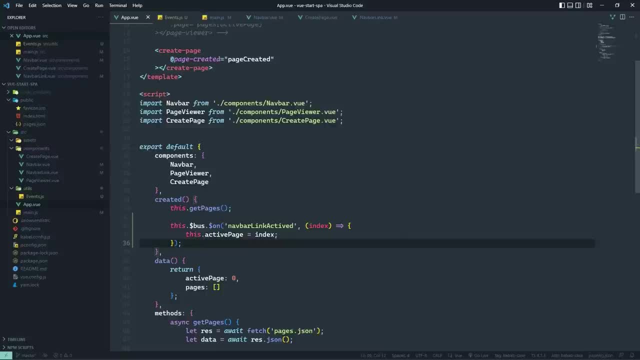 So this should still work as I should, because I haven't actually tested this with a map. I've always used just a typical object instead of a map. But to me, a map fits this purpose better than a normal object. So let's go to the browser. 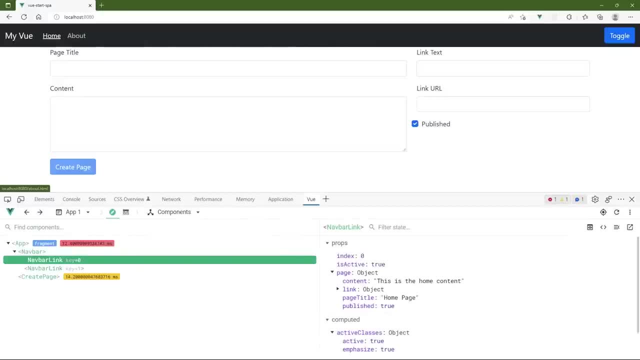 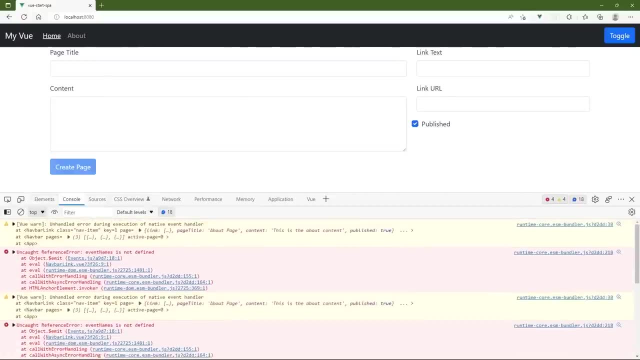 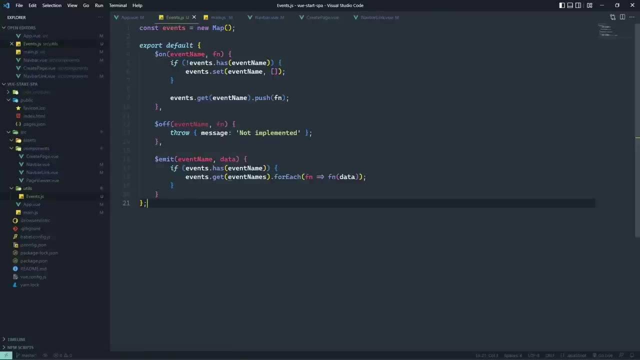 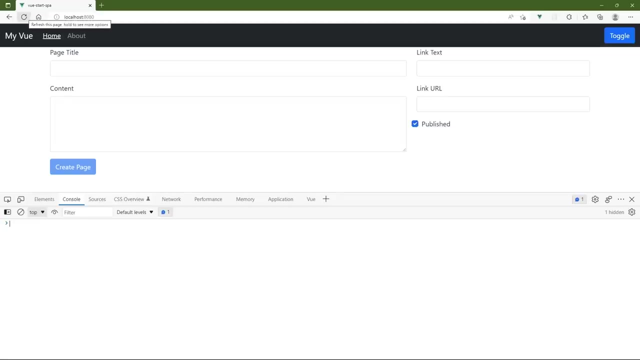 Let's refresh here and let's click on our link and nothing is happening. So let's take a look at the console. We have some errors here. So event names is not defined. And that's because I mistyped it somewhere inside of events. So that would be here. Line 18. So let's get rid of that s. Let's go back to the browser and let's try this again. Let's click on about. And it looks like it activated. If we click on home, we see the same thing. 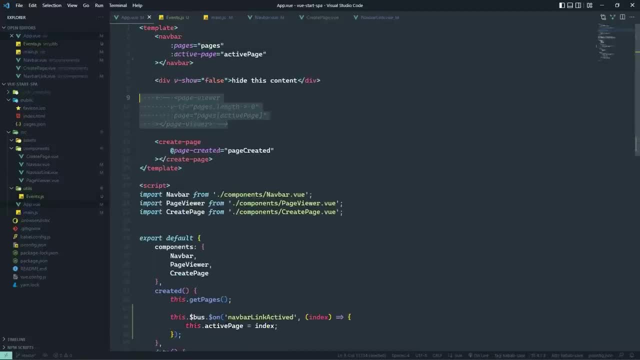 Let's go to the app component and let's uncomment out our page viewer just so that we can see if the page is going to change as well. So let's refresh. We have our content. 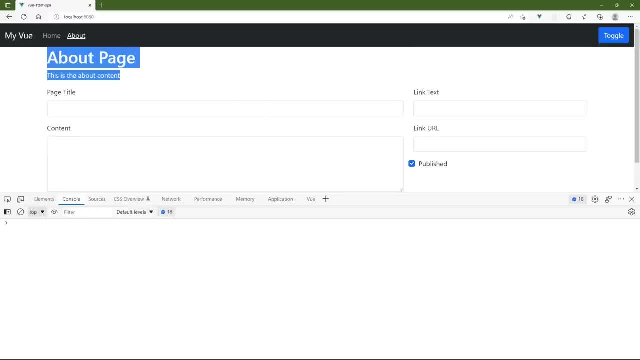 If we click on about, we can see that that's changed as well. So we are good to go. 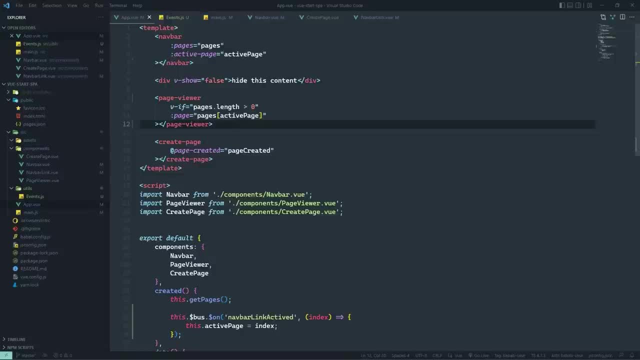 We now have a global event bus that we can use in our application. Now, a lot of times you might not need a global event bus, but if you do, that's how you can implement one. 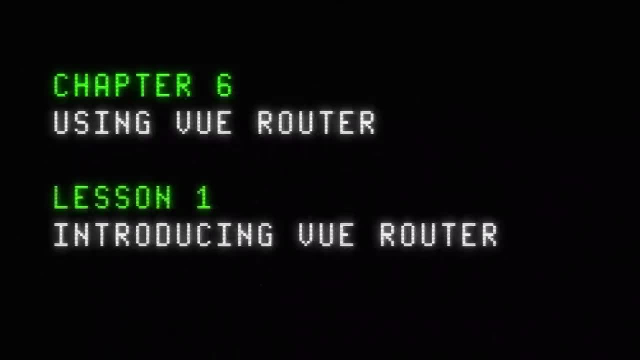 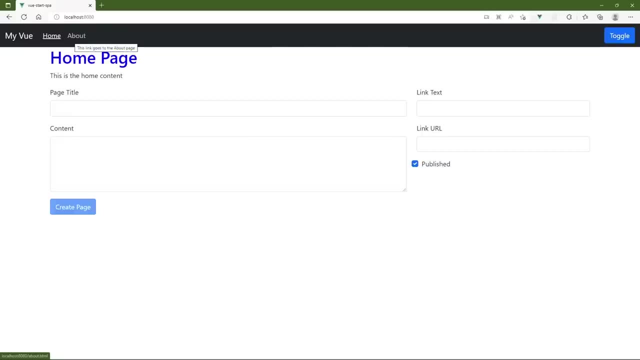 Our little application is technically a single page application. It is a single page that is loaded into the browser. And then we are able to navigate to other pieces within the application. Like, for example, for now, all we can navigate is between the home and about pages. But if you think about it, this isn't very scalable because the pages that we currently have are all of the same kind. 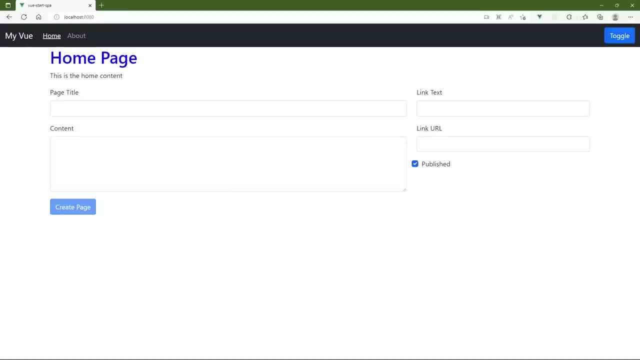 In fact, it's data driven. It's driven by the data for those pages. 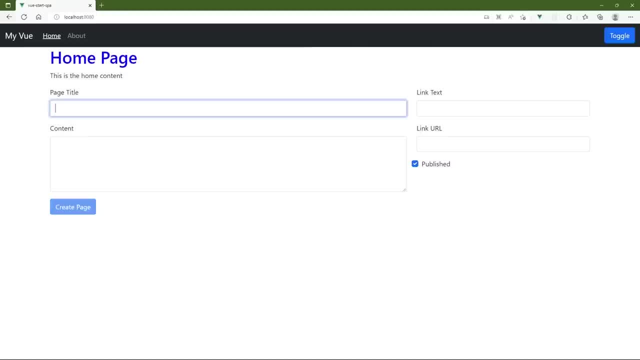 But we also have the page created component that has a form so that we can create more pages that would ideally be inside of another page that we would navigate to. And then if we had any other utilities such as being able to list all of the pages and edit them, all of those would be in other pages as well. 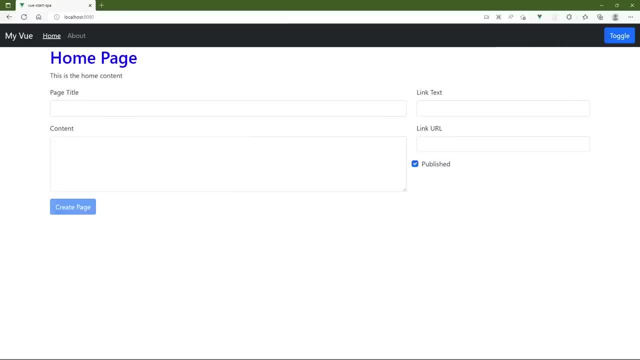 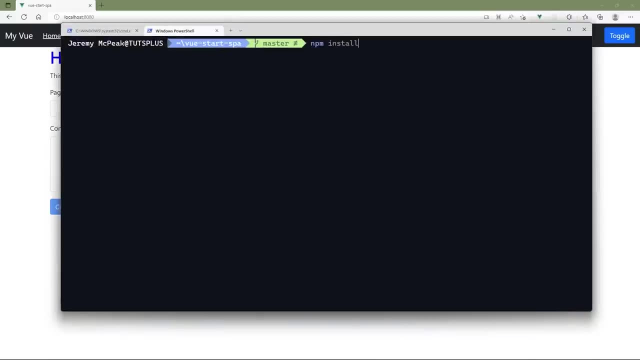 So if you plan to do any kind of navigation within your applications, it makes a lot of sense to just go ahead and get started with a router. Now, let's install the router and then we will talk about what it is. 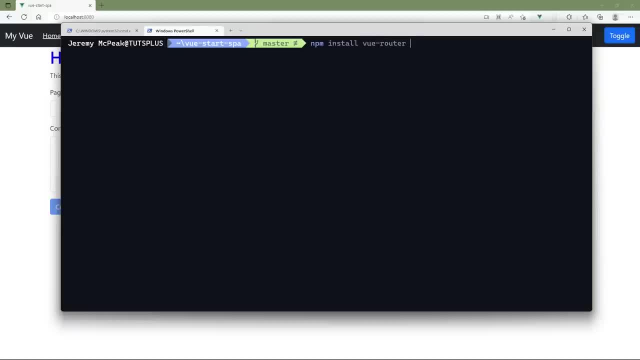 So for our Vue applications, we want to install the Vue router and we want to save that to our project. Now, a router in the sense of software 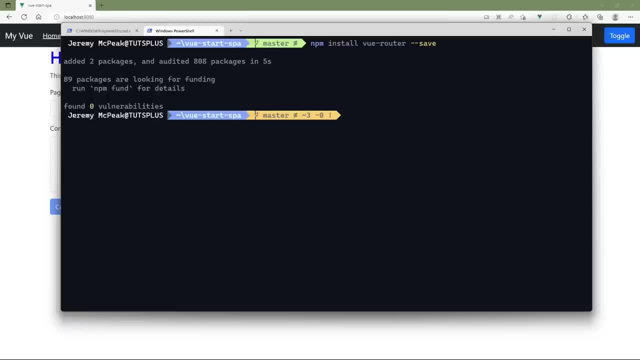 development takes user input and routes it to some piece of code that is going to handle that input. If you think of a server side application like 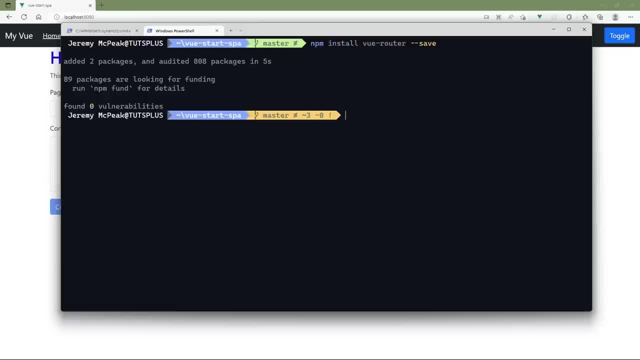 Laravel or ASP.NET, there is typically a routing engine that is looking for 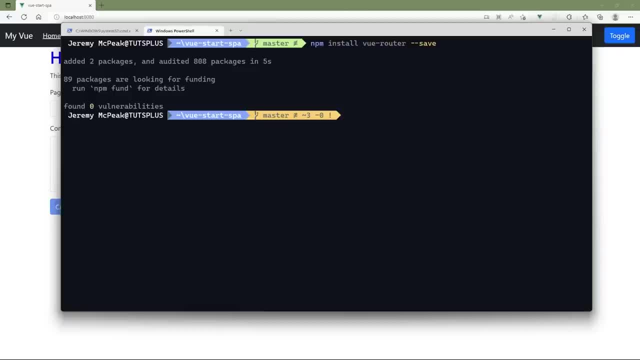 incoming requests and it will route those requests to different methods on a controller. Well, the same idea applies to our Vue application. 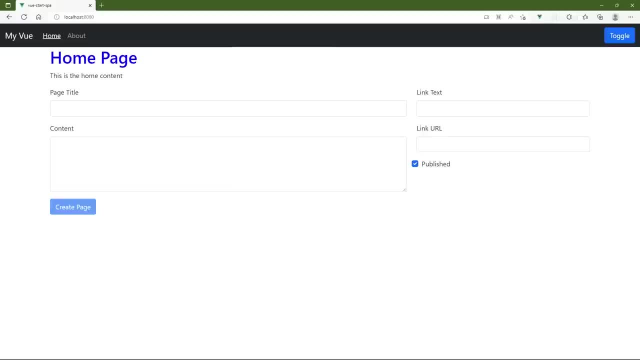 We have a router that is going to route URLs to a component so that it essentially treats an individual component as a different page within our application. 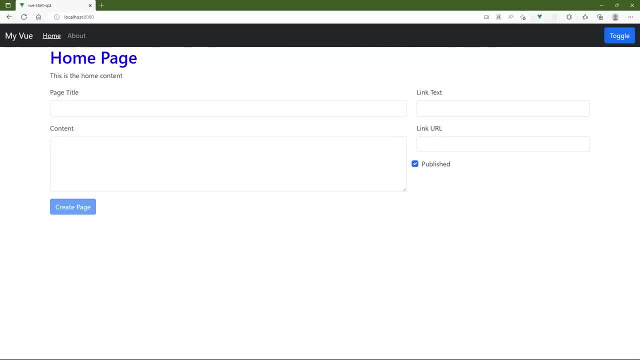 But the entire application is loaded within a single page. Now, the reason why you would want to start 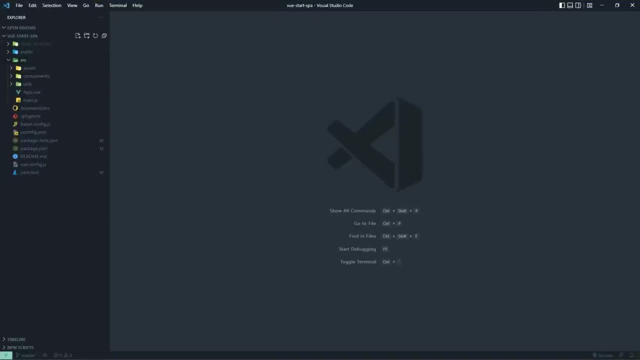 with a Vue router to begin with, if you have any kind of navigation, is because it changes the way that you need to develop your application. 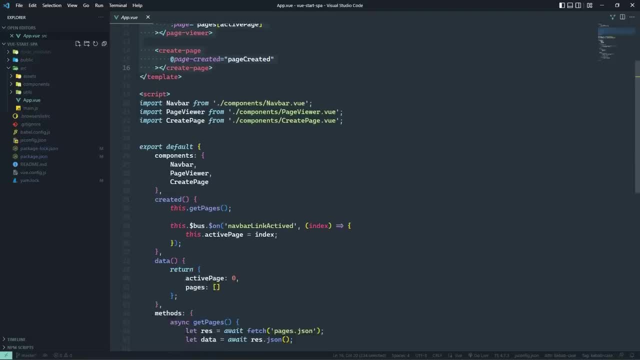 Like, for example, we have this app component, which is essentially the entry point of our application. 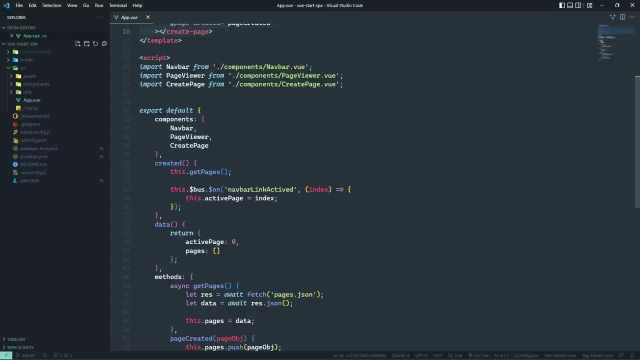 I know that the main JS file is, but this is where we load our data. This is where we pass data on to the other components. 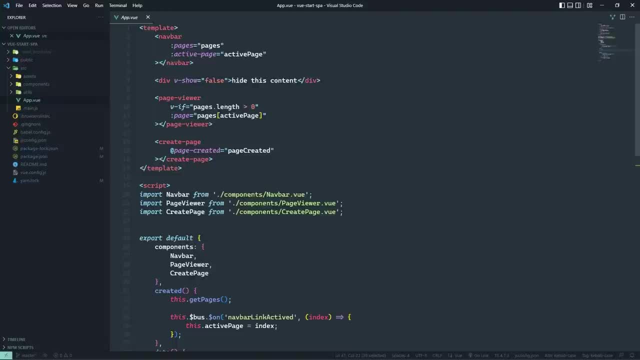 So this is the main piece of our application. But whenever we introduce the ability to navigate to other pages, well, the way that we interact with our data 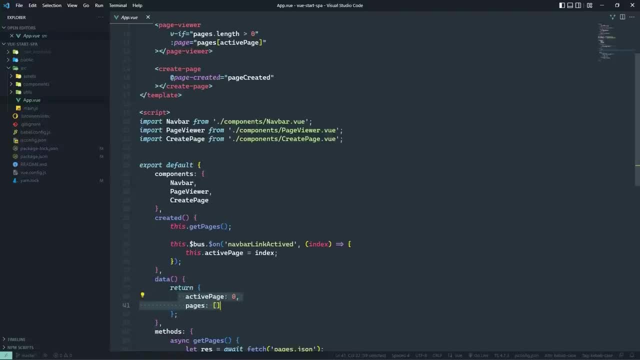 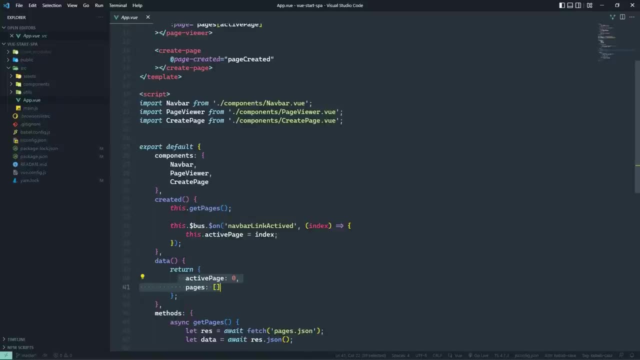 changes because it's not necessarily something that we can just load here inside of our app component. Instead, it's something that we almost have to do inside of each individual component that is going to be working with that data. And you'll see why that is. 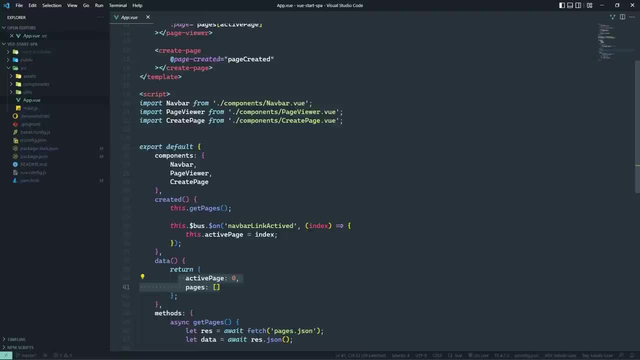 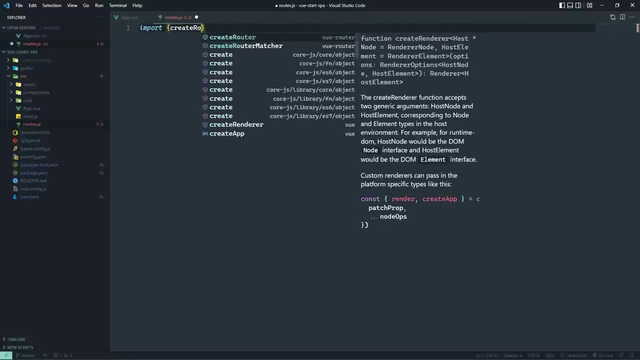 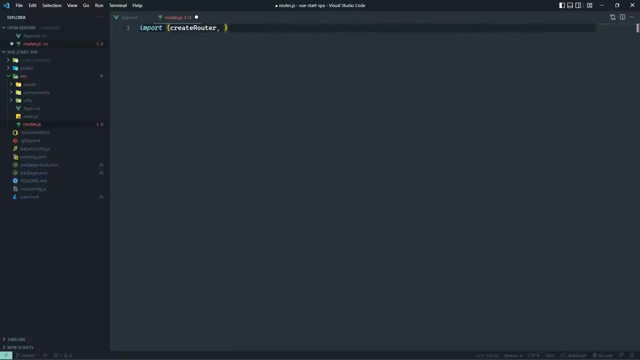 So the first thing we need to do is define the routes for our router. And we're going to do that inside of a separate file and we can just call this routes.js. And the first thing we need to do is import two functions. The first is going to be called create router. This is, of course, what we use to create the router. But whenever we create the router, we also have to tell it how to handle the URLs or at least how to handle the history. 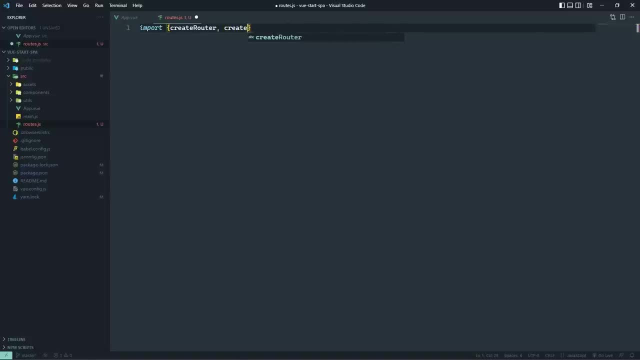 And since we don't have any backing server side application, what we are going to do is use the web hash history. So we need to also import this function called create web hash history. And we're going to use that whenever we create our router. So we want to import these from view router and then we will create our router. We will call the create router function and then we will pass in an object. The first property that we need to define is the history. How is the history going to be treated within this router? And this is where we use that create web hash history. 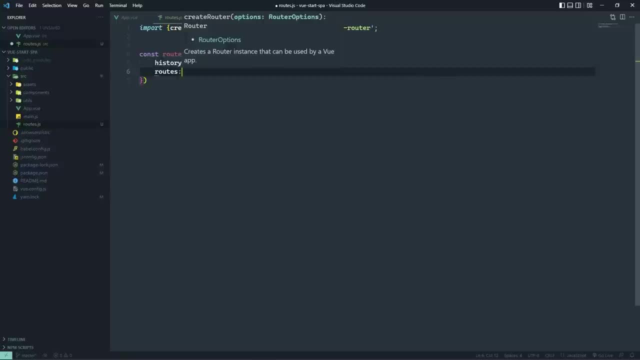 And then the second property are the routes that we are going to define for our application. This is an array of objects. And the most simple objects are going to have two things. It's going to have the URL path. This is essentially what we would see in the location bar. And this is how we determine what requests get routed to which components. So the home of our application would be just a slash. And then we would need to specify the component that is essentially going to handle that URL. 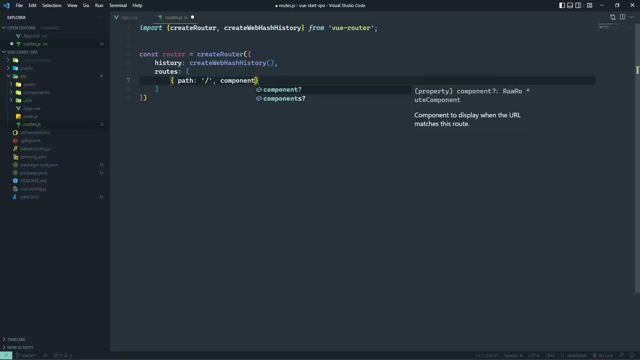 So in the sense of our application, whenever we navigate to the home, whatever component we specify is going to be displayed. Now, we have something already available that is responsible for displaying content, and that is our page viewer. 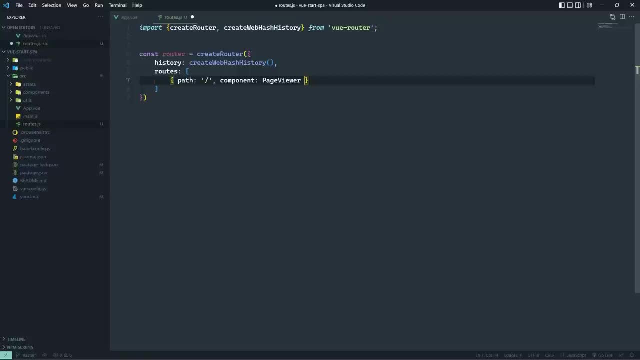 However, if you'll remember, the page viewer is very dependent upon the data that it receives, it needs to be able to display the individual pages. And we would pass that data through props. Well, now that we are going to use a router, we can't really use props. I mean, we can, but all the data that's going to be passed to the component is now going to be done through the URL as opposed to a parent component. 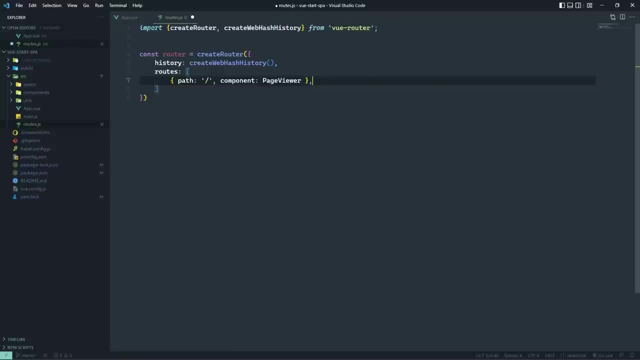 So we are essentially going to be breaking our application, and then we will fix it so that it will work with the router. 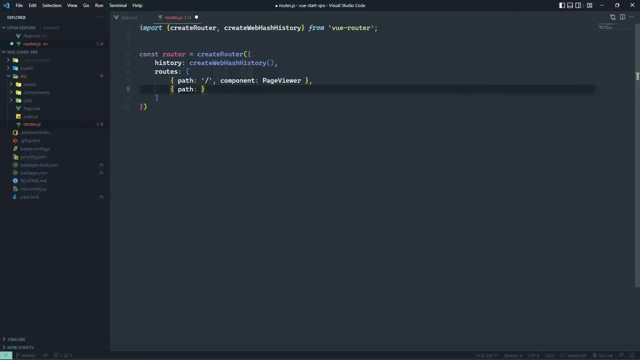 So we have our home route, which is going to be our page viewer. But then we also need a route for being able to create a page. 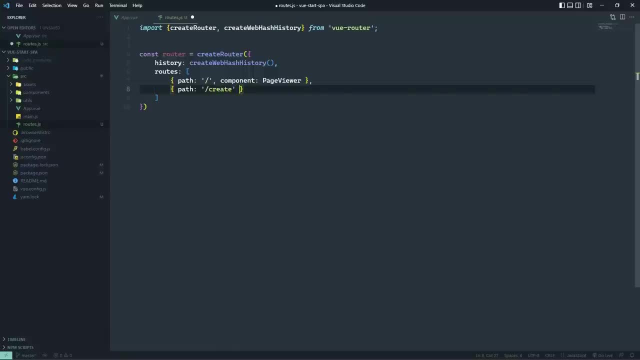 So let's define a route that has a URL of slash create. And then we want the create page component to be displayed whenever that route is handled. 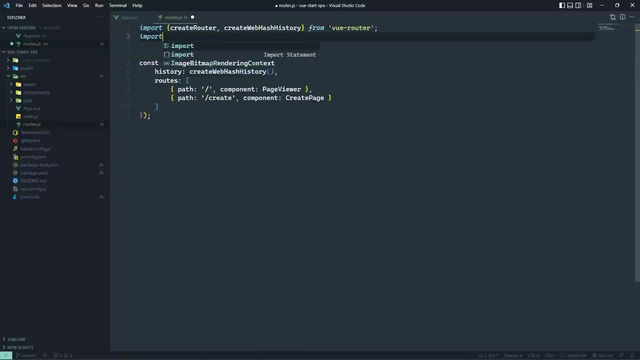 Now, of course, we need to import these components. So let's first of all, import the page viewer from our components folder page viewer. 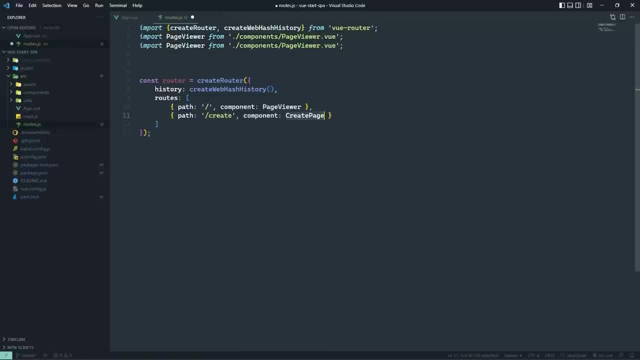 And we also need the create page component as well. And then after we create this router, we are simply going to export it so that we can then import that inside of our main file. Now, we still get to say that our app component is going to be the well, the app component. But then we will tell our application that we have this router that we want to use. Let's import that from routes. And then we want to call a method on our app simply called use. The use. 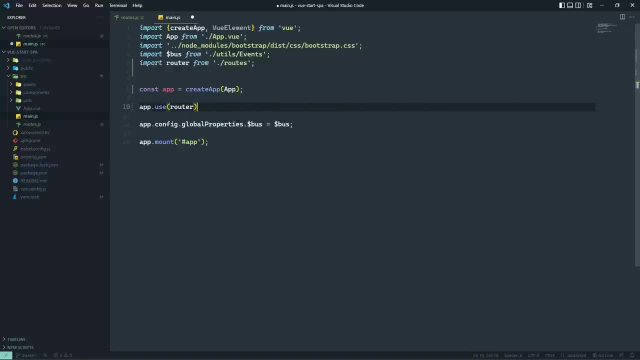 Method lets us pass a plug in and the router object that we just created is a plug in so that we tell our application to use the router. 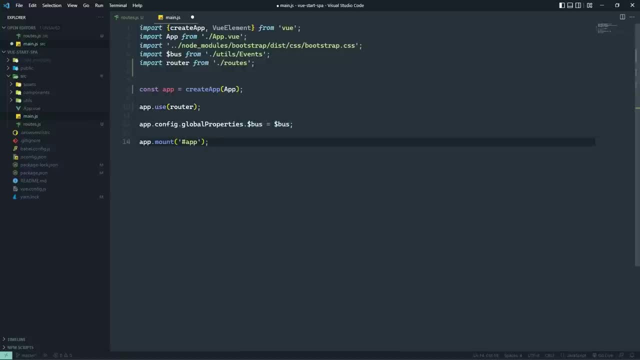 We still need to modify our global properties and then we mount our application. 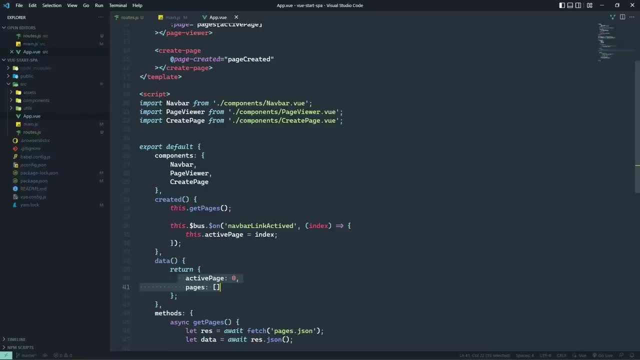 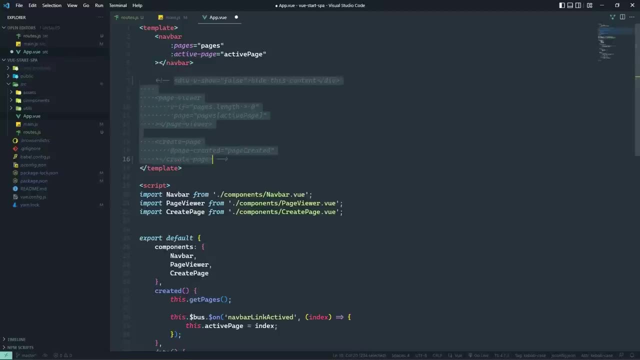 Now, the other change that we need to make is inside of our app component. We still want our nav bar here, but everything else we don't want because the router is going to be loading this information and we tell our application that we 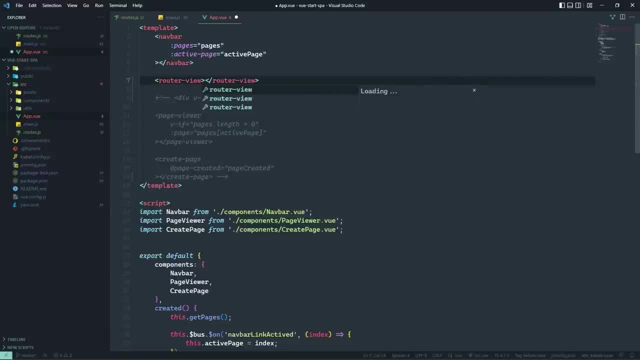 want to display that router information right here with this router view component. So the component that's going to be loaded by the router is going to appear here or if we wanted it above the nav bar, which doesn't make a whole lot of sense, we could do that as well. 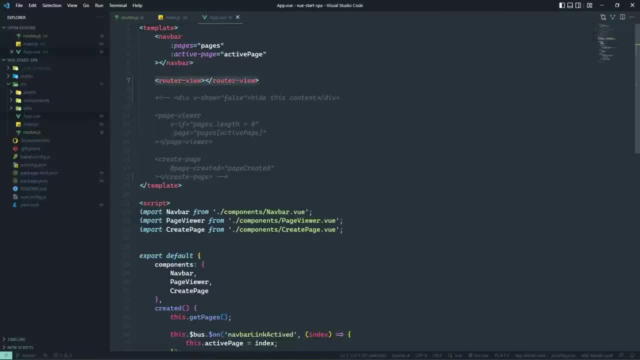 But the idea is that this is a placeholder so that whenever the view router navigates the user to a component, that component is going to be displayed right here. 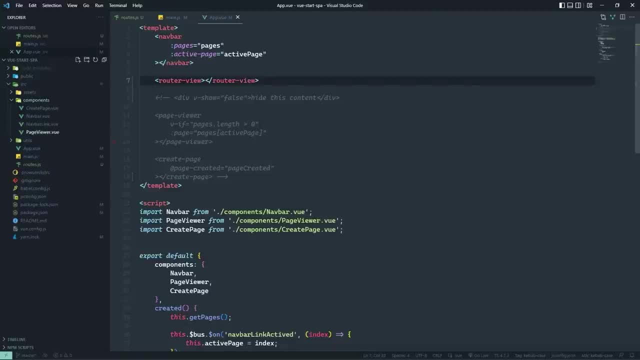 So our page viewer is not going to do anything right now. 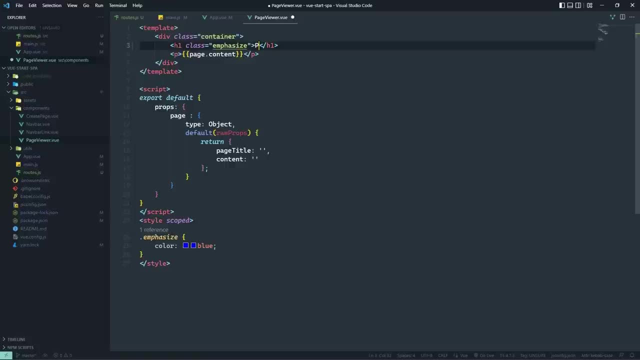 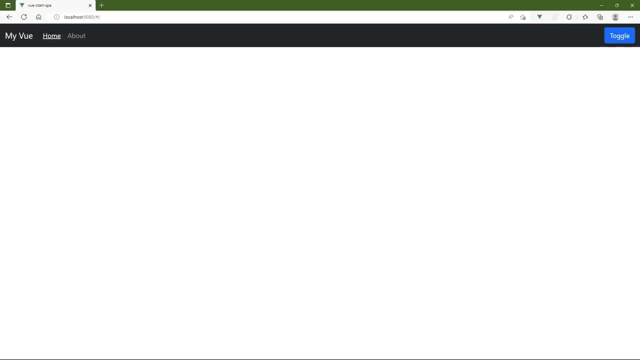 So let's change this so that we have some text that we can see. So we'll just have the page title and then we will have the content. And whenever we go to the browser, we should see that we have our nav bar and then we have the page title. So notice the URL. We have a hash. 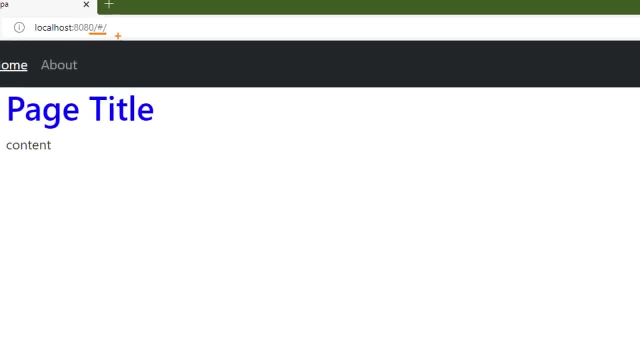 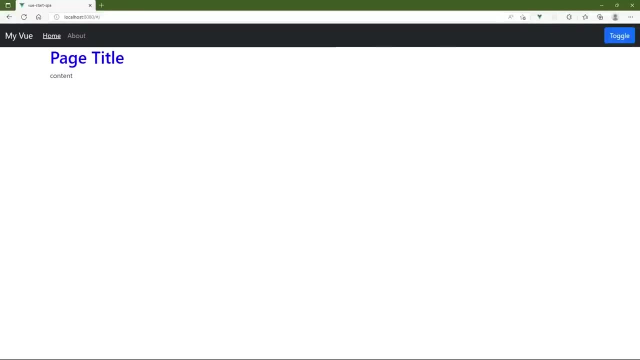 That's because whenever we created the router, we told it to use the hash history. So if we want to navigate to the create page, we will need to say 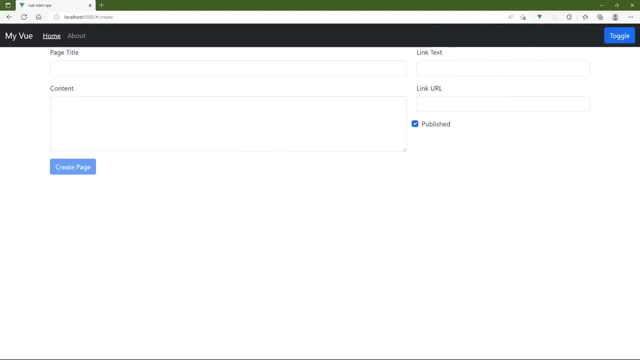 hash slash and then create and that will take us to the create page, which you can see now is our create page component. 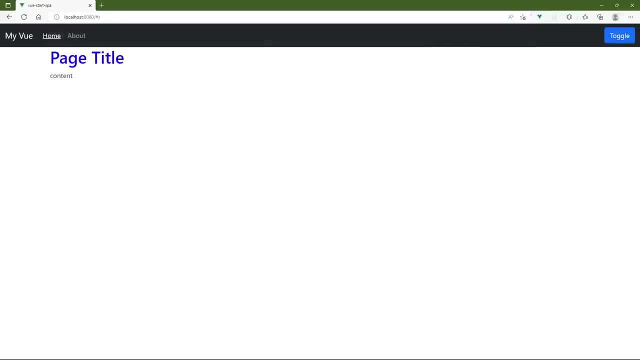 And so now the question becomes, how do we get our data? Now, of course, the nav bar is still displaying the links to those pages. And the reason is very simple, 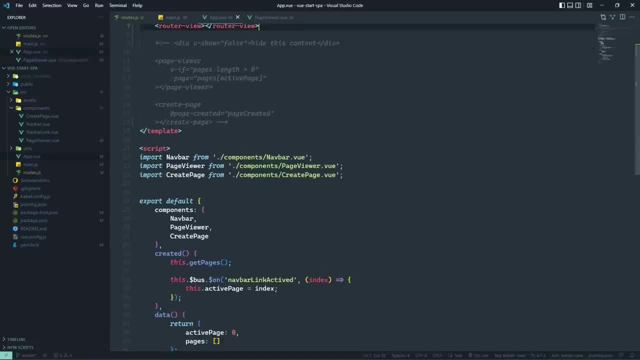 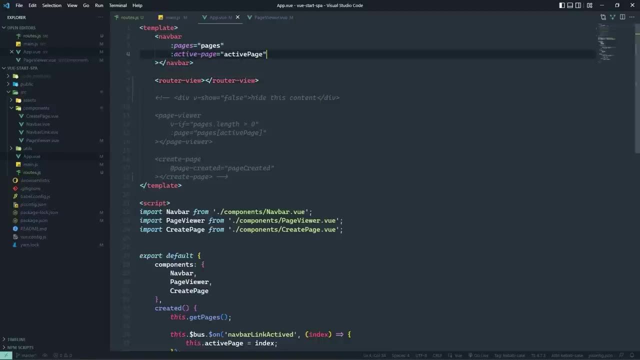 because we are still loading that data inside of the app component and we're passing those pages onto the nav bar, but we've now just effectively broken the functionality of this active page. 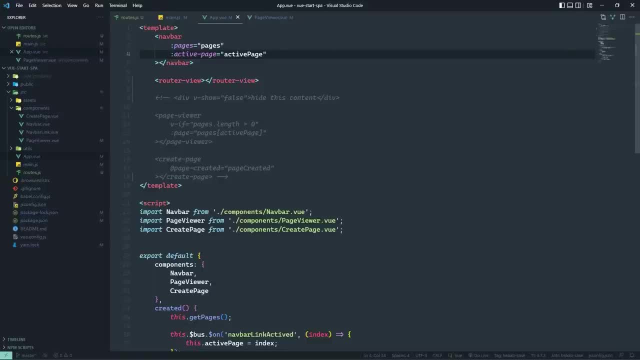 Data because that's what we used in order to display the given page. Now, of course, the active page was dependent upon knowing the index of the page that was currently displayed. 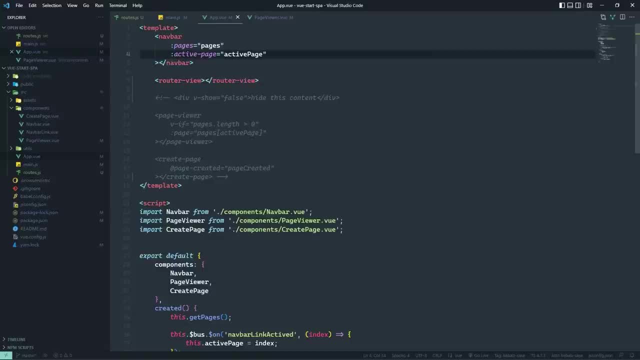 That information is now in the URL and we can get that information from route params, which we will look at in the next lesson. 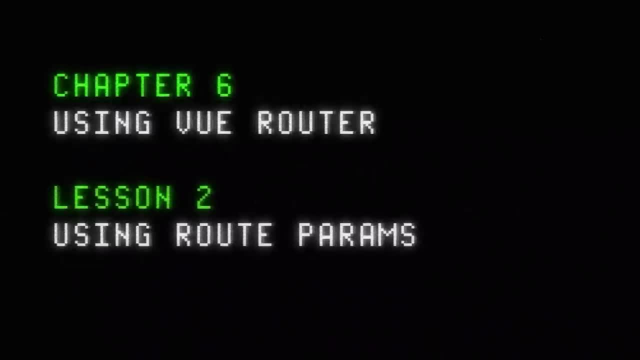 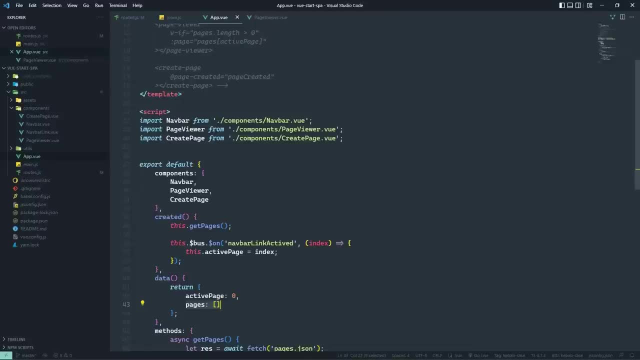 Before we just dive in and start refactoring our application, we first of all need to talk about how we need to refactor our application. And let's first of all, just briefly, recap of what we had. 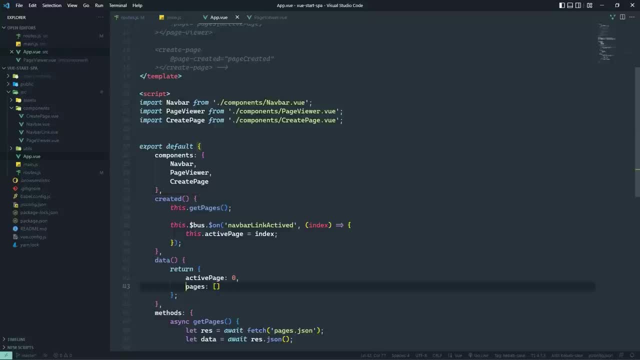 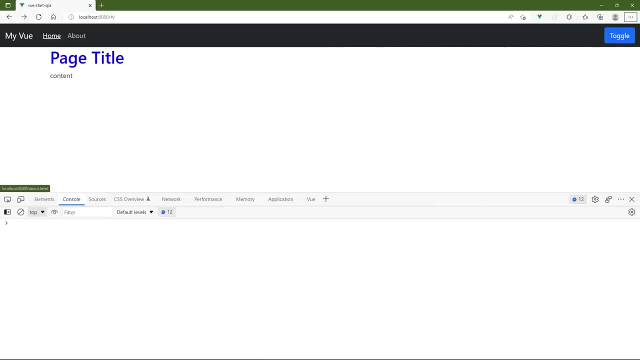 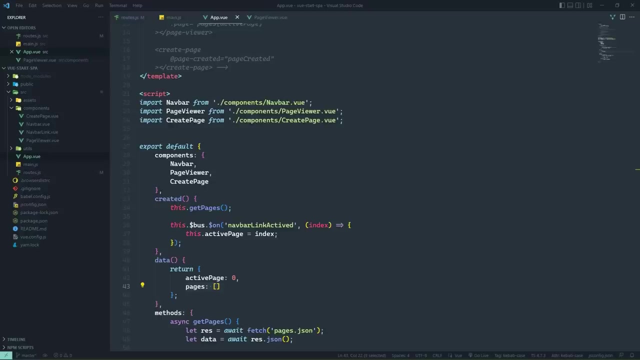 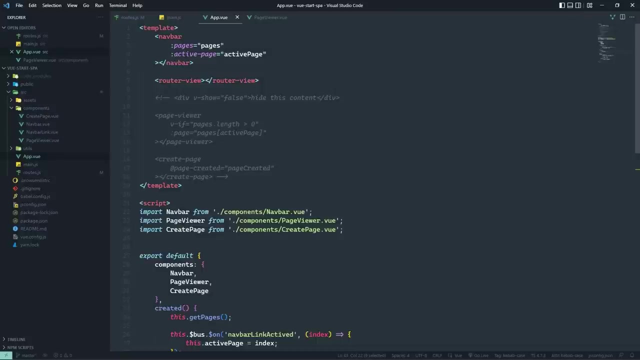 So we had an application that relied upon an array of page objects. And we used this array in order to build a menu. This menu had some links that whenever we clicked on the link, it didn't really navigate us to a different page, but it did load the content of the page object that was associated with the link that we clicked on. And all of that was handled through the app component. It kept track of whatever link we clicked on, and then it provided the page to the page viewer component so that then the content would be displayed. 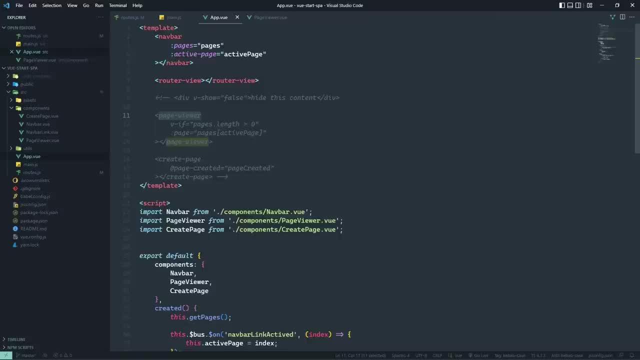 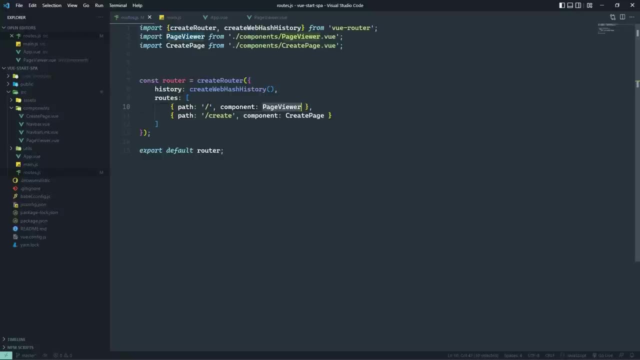 But in the previous lesson, we added the view router and that drastically changes the way that we are going to use our page viewer component because now page viewer is handling a route. 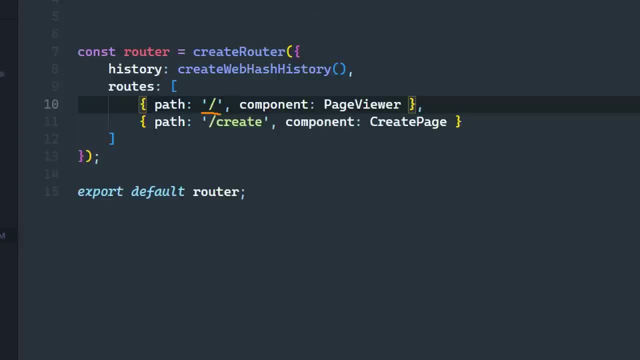 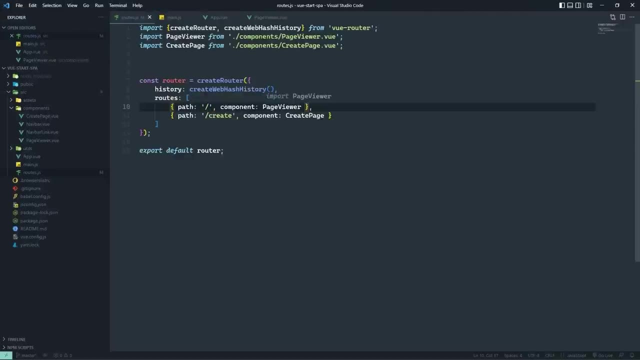 Right now, that route has a path of just a slash, which is the root of our application. And unlike before, we can't just pass the page to display as a prop. Instead, we need to start thinking in terms of just typical web applications. So if we forget about view for just a brief moment, let's imagine that we have 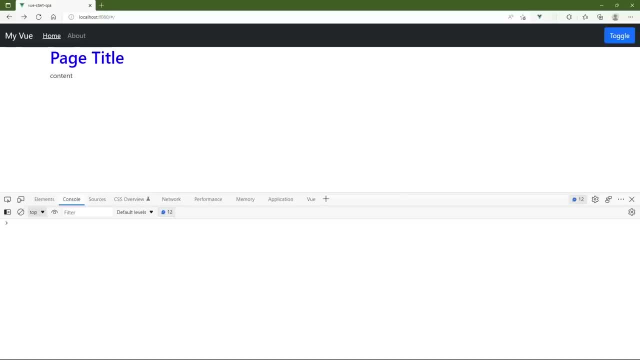 a blog website and we want to display an individual blog post. Well, the way that we would do that is to have some kind of unique identifier in the URL. 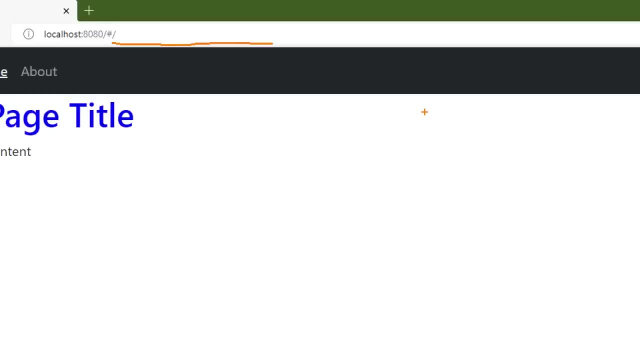 That way, the blog application could pick out that data from the URL. 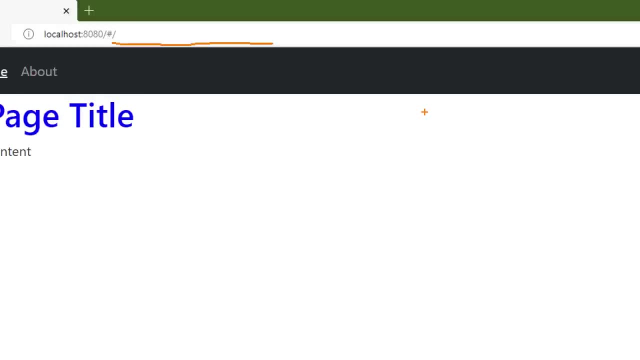 It could fetch the information from the database and then display that in the web page. 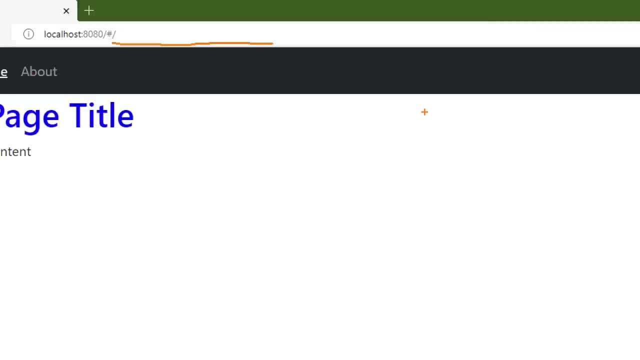 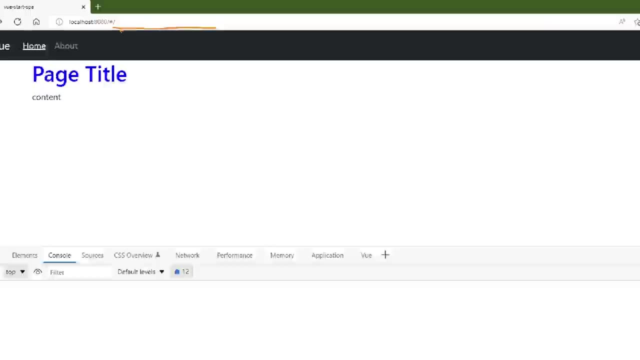 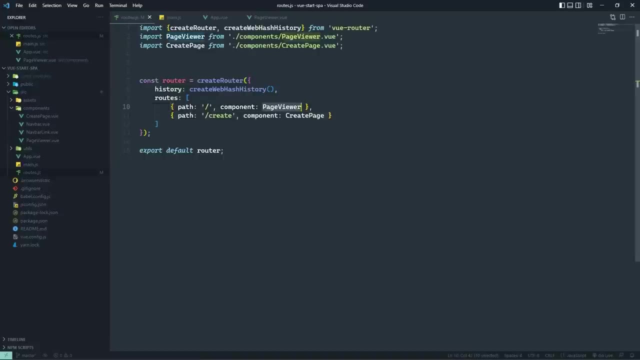 Well, that's basically what we need to do with our application. We need to provide the unique identifier for the page object that we want to display so that we can fetch that object and then display that inside of page viewer. So all of the data that page viewer is going to rely upon is going to come from the URL. 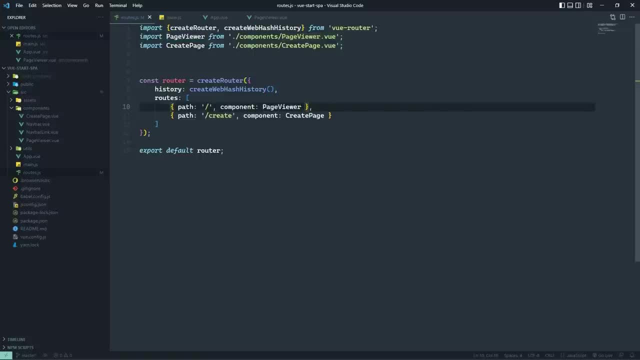 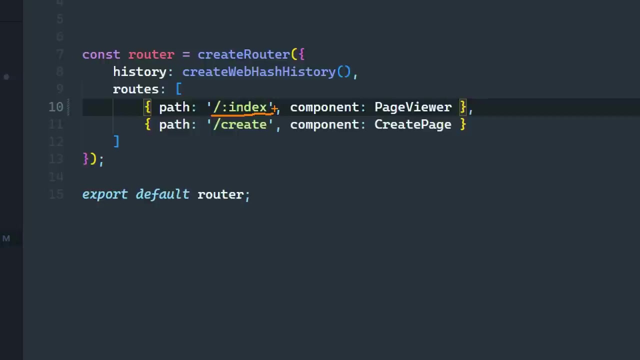 So we need to denote inside of our route that there is some unique identifier that we need to work with. And we do that with what's called a param. A param starts with a colon and then it's followed by some name. And in this case, I'm going to call it index because that is how we have been referring to individual page objects. So this route now has a path that expects an index, something that we can use to then go and fetch our data. And display that. 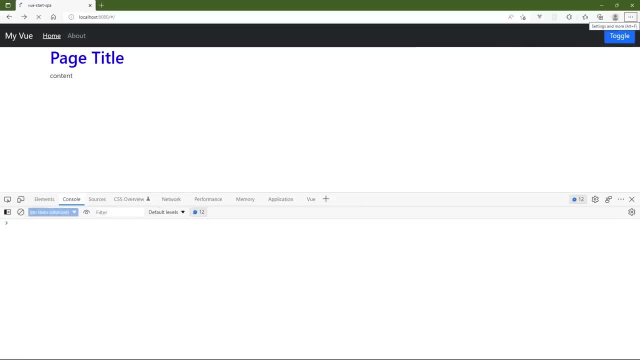 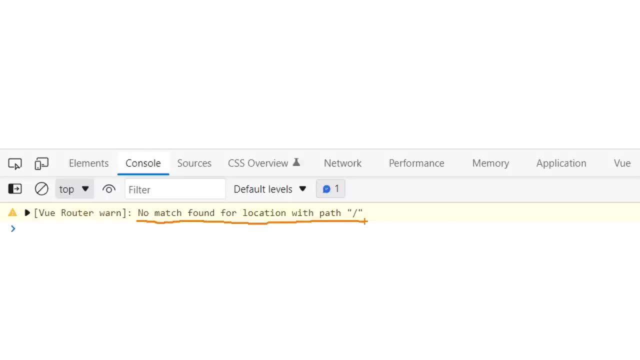 However, this is going to have a side effect that I'm not all that wild about, because now as you look into the console, it says that there is no match found for the location with a path of just a slash. 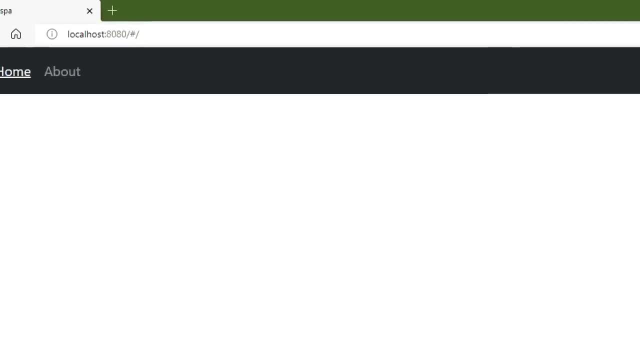 So I want this application to work like this. If we don't supply an index, then it's going to provide the default page. That could be index zero or that could be the lowest index of a page that is published. 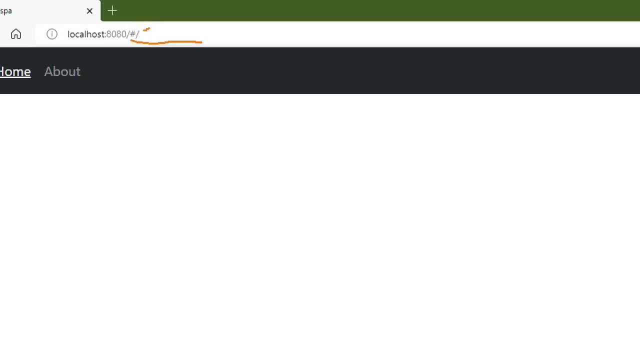 But if we do supply an index, like an index of one, then we would display the page with that index of one, at least as long as it is published. 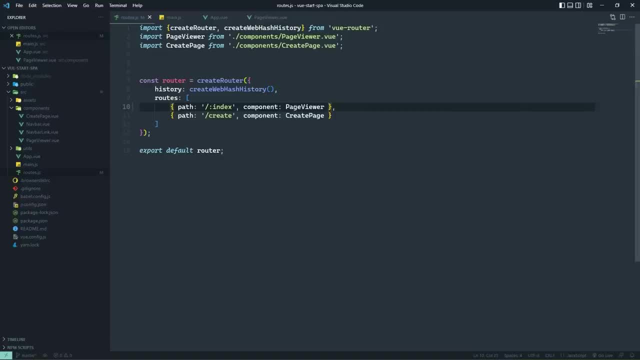 So this means that our index param needs to be optional. And we can do that very easily by just adding a question mark at the end of the param. 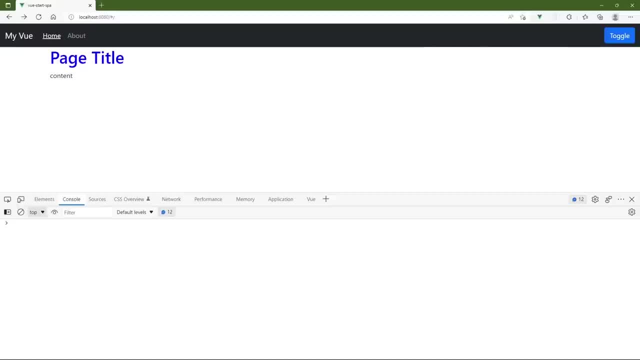 It is actually an empty page. We're going to see string whenever we go to retrieve that. 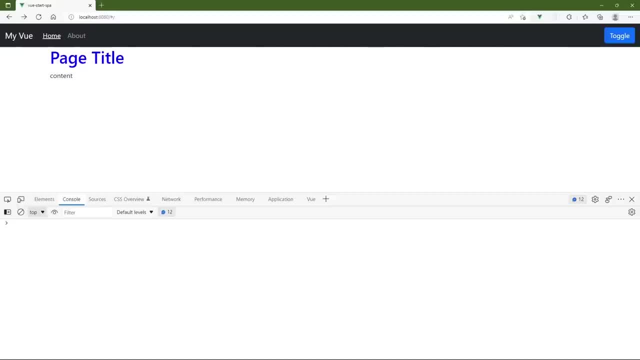 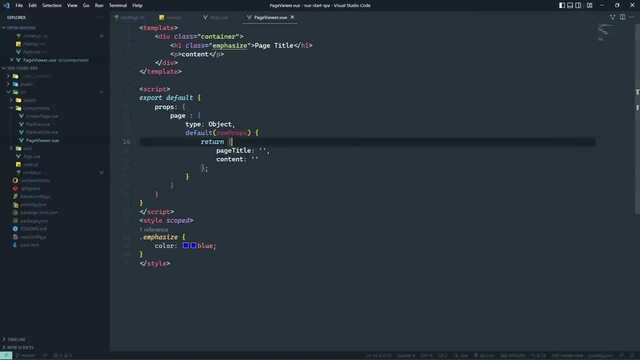 So now the question is, how do we retrieve that value of that index param? Well, let's go to our page viewer because this is now the component that is handling that route. We don't have the page prop anymore. 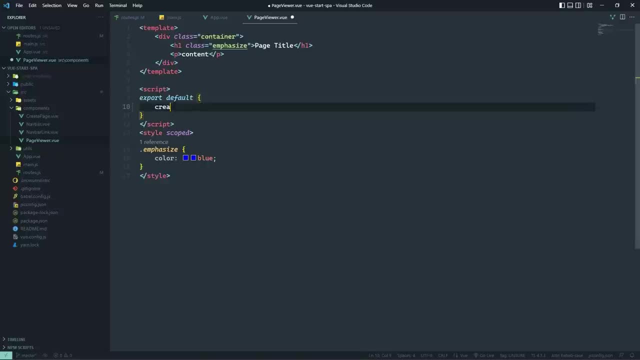 So let's go ahead and just get rid of our props altogether and let's add the created hook. 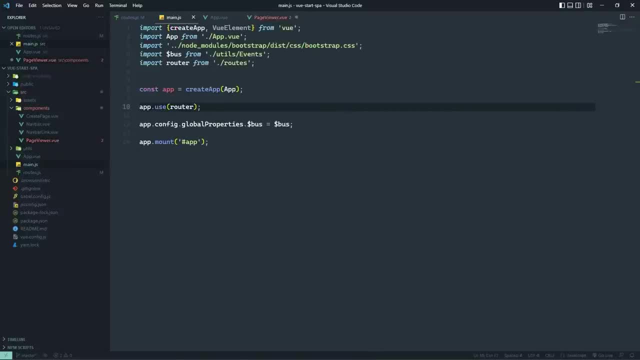 So in the previous session, whenever we created our router, we added it to our app with the use method. 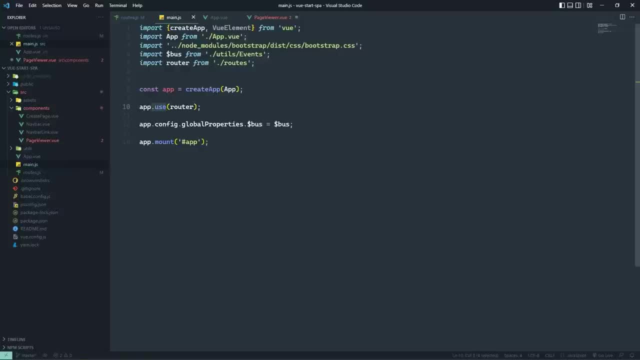 This was for including a plug in with our application. And whenever you do that, we get a special property that we have access to in all of our components called simply route. 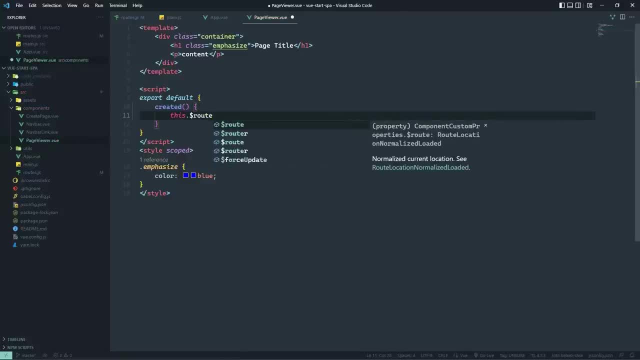 This refers to the route that is currently being handled by this page viewer component. 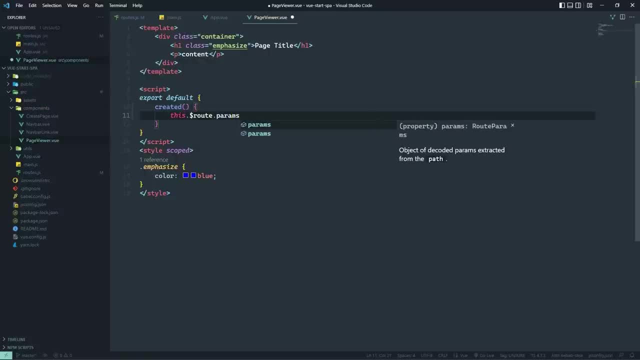 So this has a property called params, which is an object that contains all of the params that would be defined inside of our route path. So we only have one and that is index. 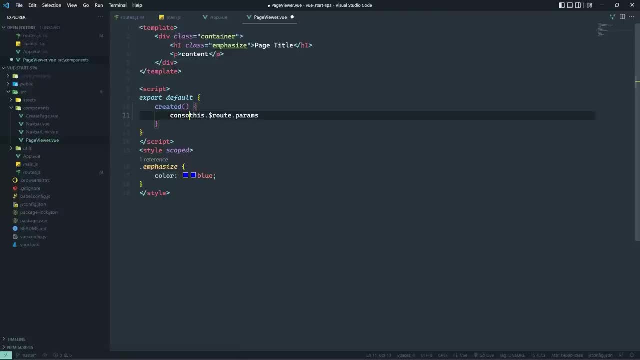 So we can actually write this out to the console so that we can see what that value is. 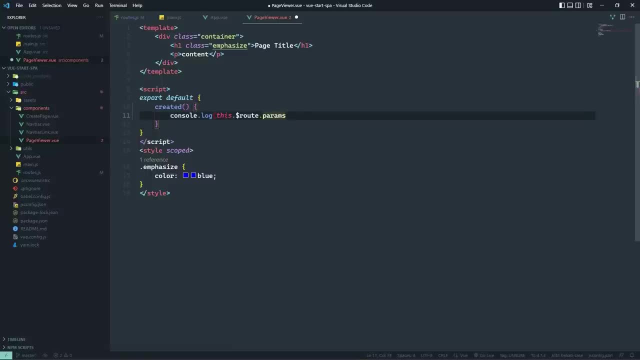 And if we just write out the params, then that's going to show us the object and everything inside of it. 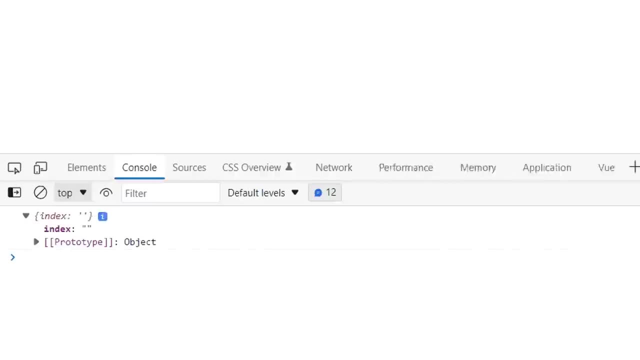 So whenever we go to the browser, we can see that we have an index, but it is an empty string. 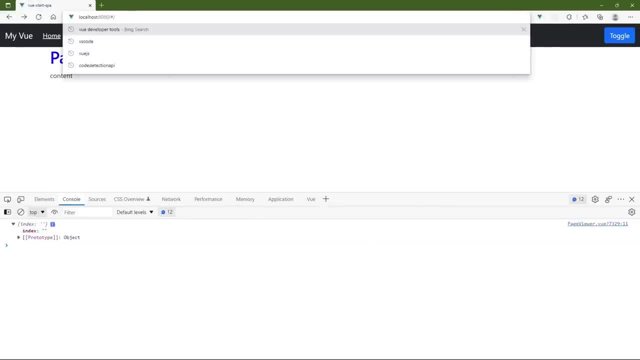 And of course, we could add some other value for the index. Let's add index one. And we can see that the value of index is 1. 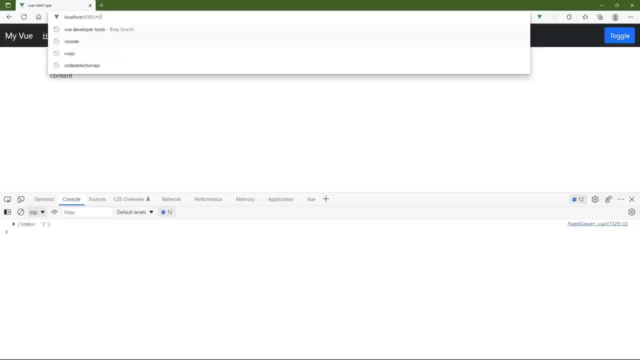 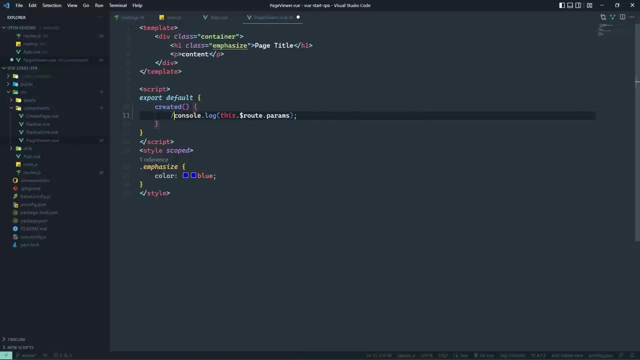 Now, there's a caveat with this, and that is it doesn't matter what we include as the index param, it can be a string of characters. And index will be that value. So there is some validation that we will need to do. So let's do this for the content. 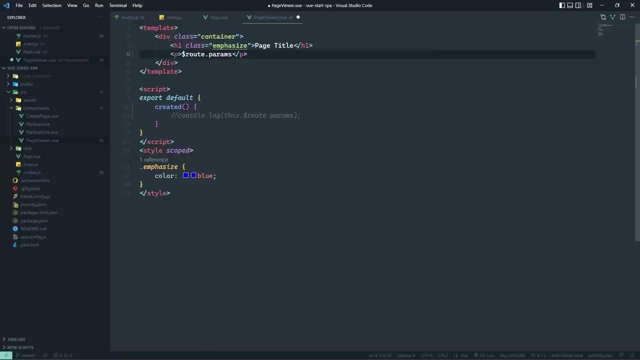 Let's take the index param, and let's just display that as the content. 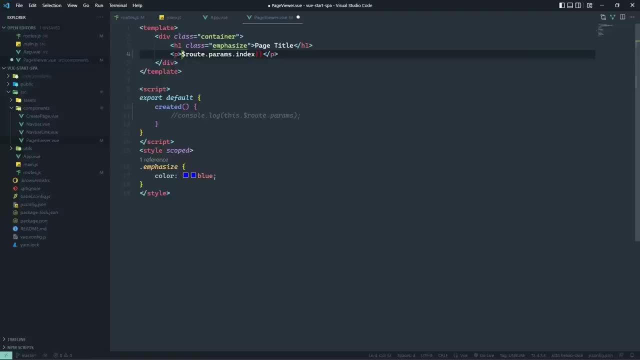 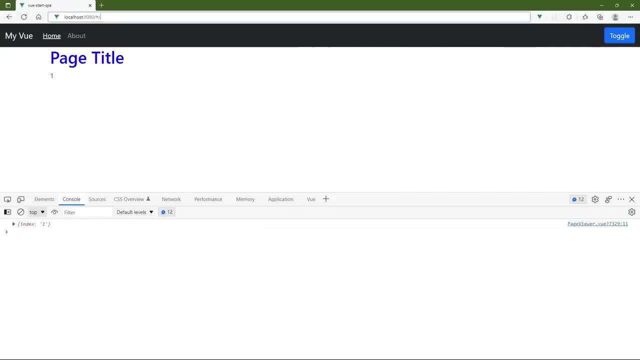 We, of course, need to use the correct syntax to output that value. But now that we know how this is going to work, we can then start to refactor our application. So that the page viewer can go out and fetch the appropriate page, 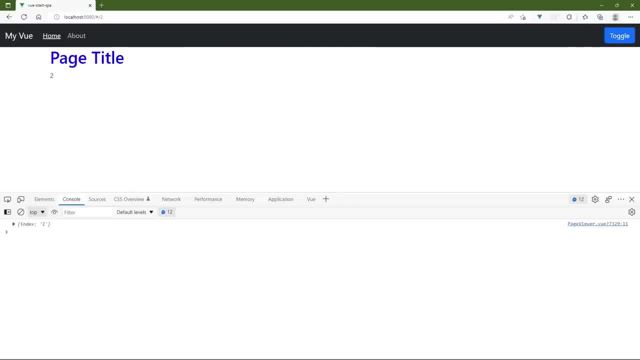 so that it can then display that content. And we will get started with that in the next lesson. 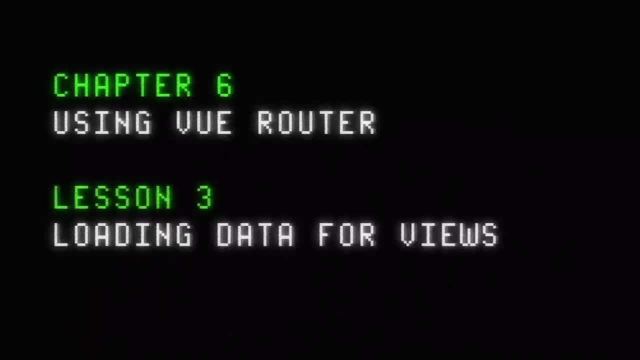 In the previous lesson, we discussed how we are going to get data into our page viewer component. 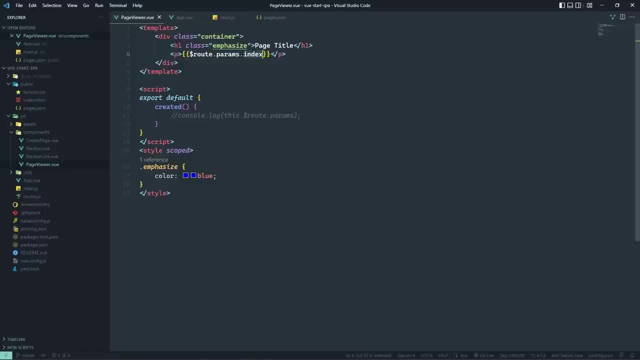 We are going to rely upon the URL, to give us the index of the page that we want to display. 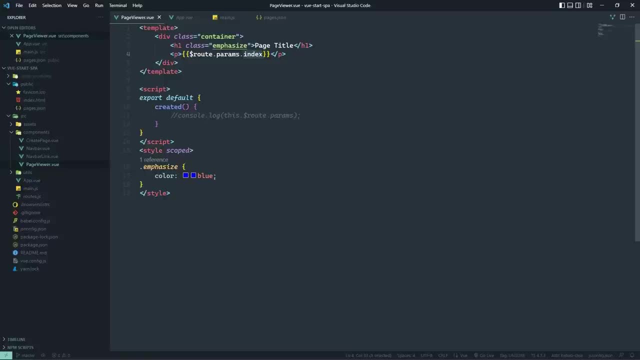 So that inside of the page viewer component, we will just fetch that page, and we can then display the content. 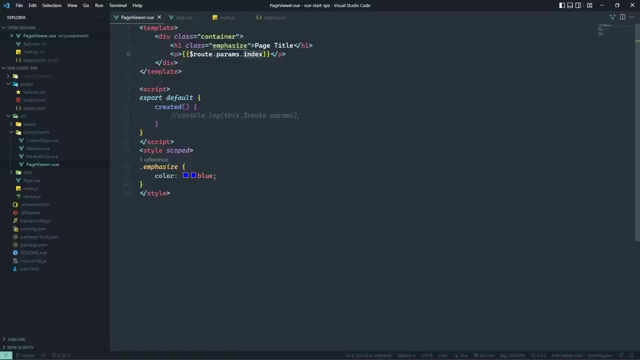 So the question then becomes, how do we go about doing this? Well, the typical pattern is to use a centralized data store. And ideally, we would use a data store that is reactive. Meaning that any time that there were changes made to our data, 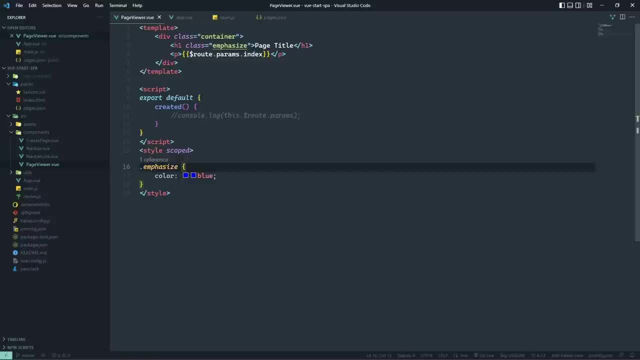 either by editing a particular page, or creating a new page. And adding it to the data store, then the application would automatically update to reflect those changes. 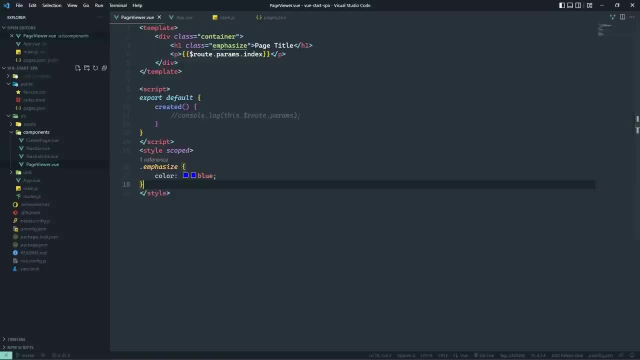 And there is a data store available that does exactly that, it's called ViewX. And we aren't quite ready for that. 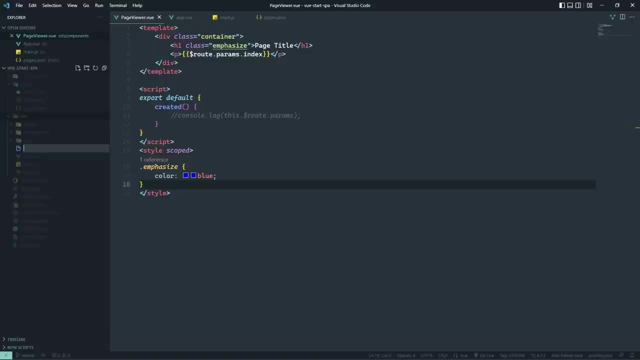 So instead, we are going to use a poor man's centralized storage. And that is basically, we're gonna write it ourselves, and it's going to be just simply an object that gives us access to our data. 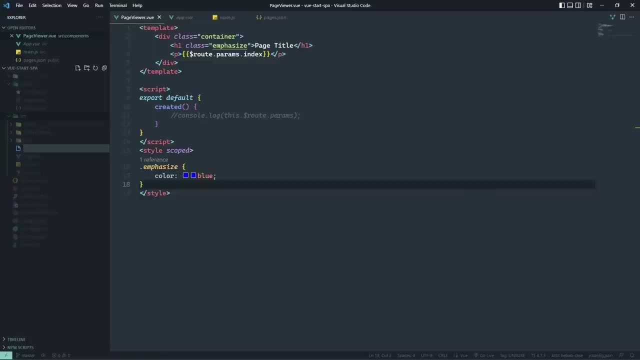 So, in this particular video, In this particular implementation, any time that we make changes to our data, we will then have to tell the application, hey, the data's changed. It's time to reload all of the data. 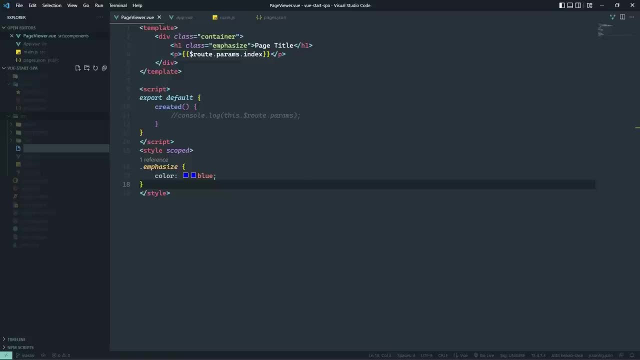 Thankfully, we have a global event bus that can help facilitate that. 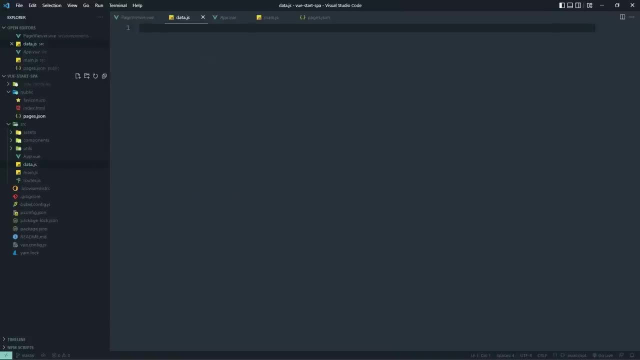 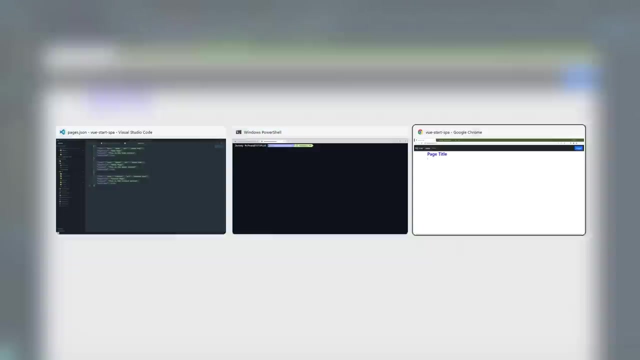 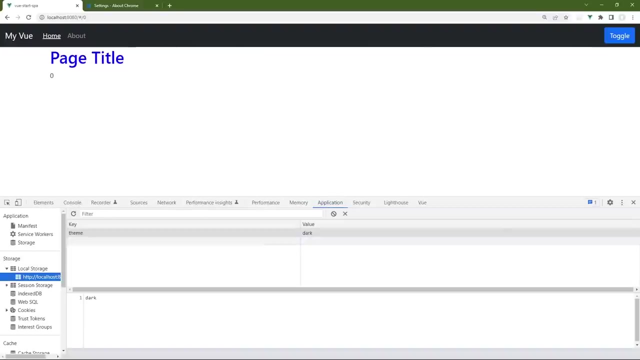 So the first thing I'm going to do is create a file just called data.js. This is going to signify our data store. And I guess really before we start doing this, I'm going to go to the content of our pages.json, and I want to go ahead and load that into the local storage in our browser. So I'm going to pull up the developer tools, go to the application tab. And for local storage for this application, I'm going to add a new item. Let's call this simply pages. 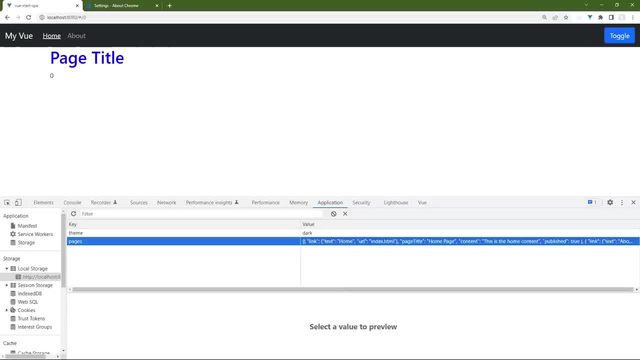 And then the value is going to be that JSON structure, so that then we can load that, parse it into an array, and then we will be good to go there. 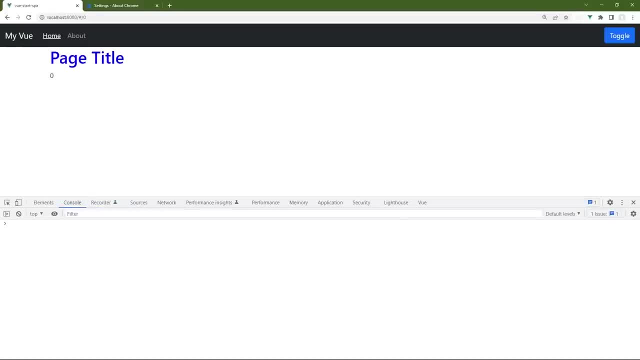 One thing I should point out is I am switching browsers. I have been using Microsoft Edge up until this point. And I ran into some issues with Edge not navigating in between our different components. Chrome did it just fine, no idea why. I spent a little bit of time troubleshooting, couldn't really find the issue. So I've switched to Chrome because Chrome was actually working when Edge wasn't. 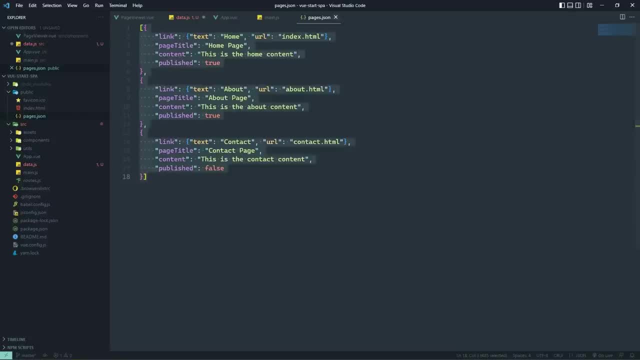 I'm sure that there's a Microsoft joke there, but I'm going to move on. 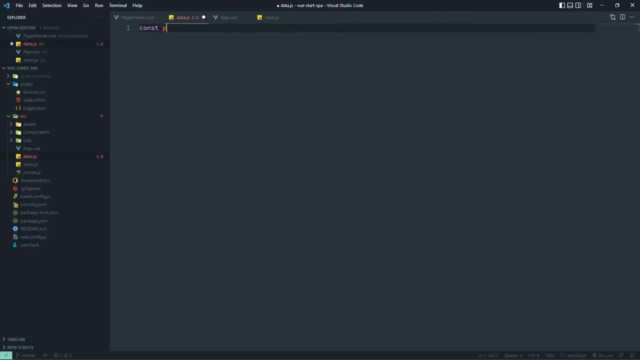 Okay, so for our data store, I want to store the key that we are going to use to access the local storage as a variable. So I'm just going to create this as a constant. That way, we don't have to worry about me mistyping a string, which is something that, well, I would definitely do. And then we're going to fetch the JSON from our local storage. So let's go ahead and do that with the get item method. 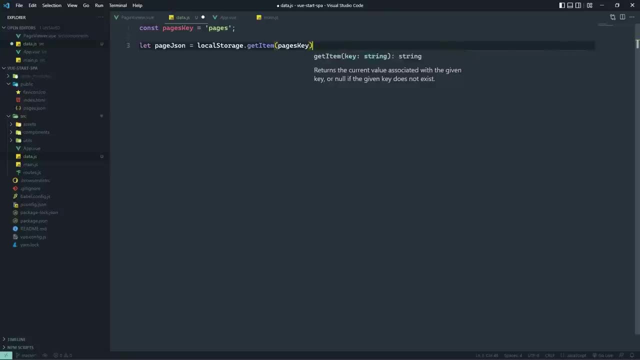 We will pass in the pages key that we just created. That will give us our JSON so that then we can parse that into our array. 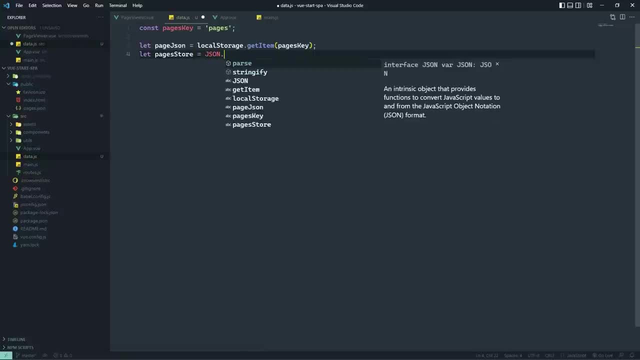 I'm going to call this simply pages store. And we will call the parse method on JSON, pass in our JSON structure, and we will be good to go to use that. 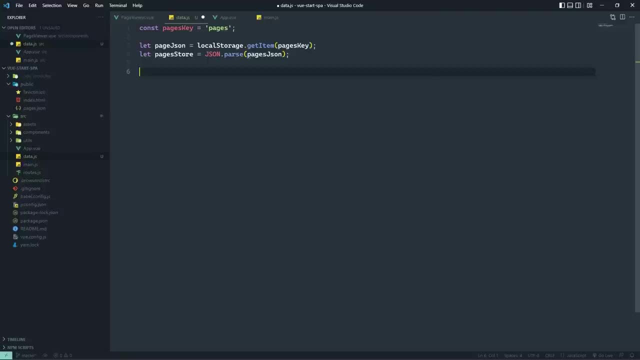 So I don't want to make this array directly available to whatever is going to be consuming this data store. So instead, I want to provide some methods that are going to wrap around it. 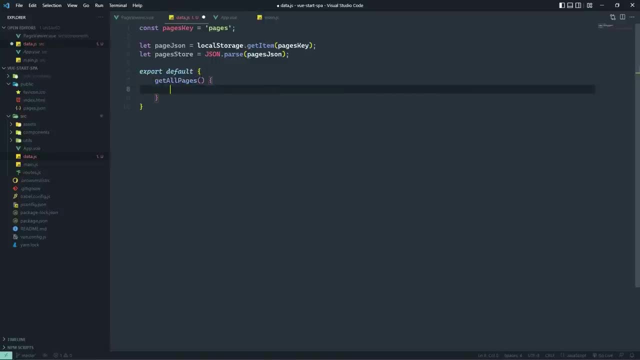 This first method, well, it's not really going to give us much of anything as far as protection is concerned because all this is going to do is return that array. So whatever we're gaining by trying to protect this, we've kind of lost just by returning this, but that's okay for now. 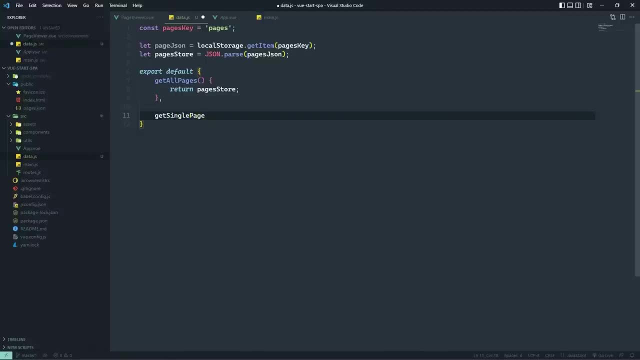 And then I want another method that we can use to retrieve a single page. All we need to do is provide the index, and we will return that page at the given index. Ideally, we would have some kind of validation to be sure that the index is valid and that we do have something at that index. But we're just going to keep things simple and go from there. 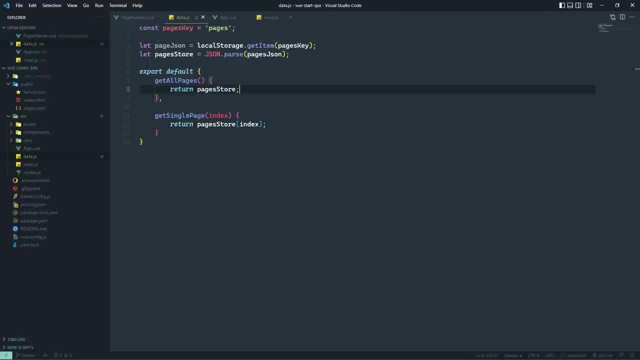 So this is our data store. We're going to make this available just like we did with our event bus. So we can import this. We can call it, let's call it $pages because that's essentially what it is. And that is inside of our data store. That is inside of our data file. So that we will make this available as a global property. We'll call it $pages again, and there we go. 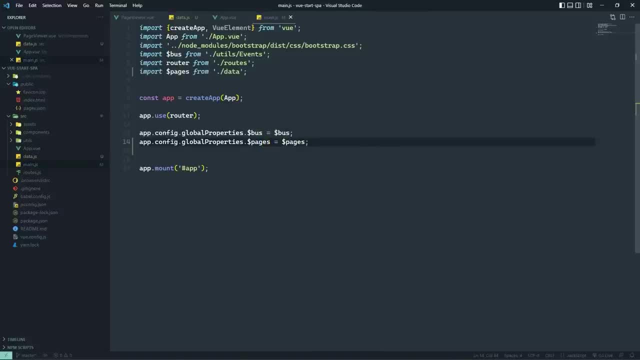 So this is going to give us access to our data store directly inside of our components. 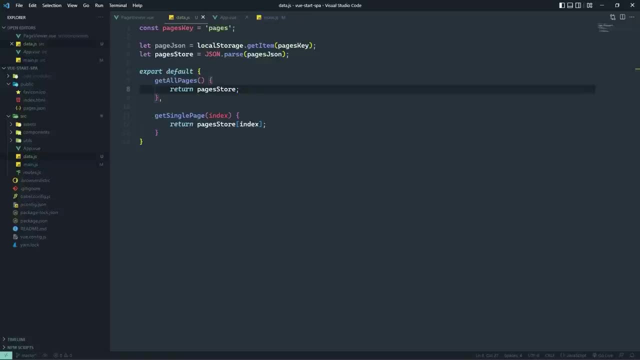 So now we can close all of these other files. Let's leave data up in case if I need to fix any issues there. 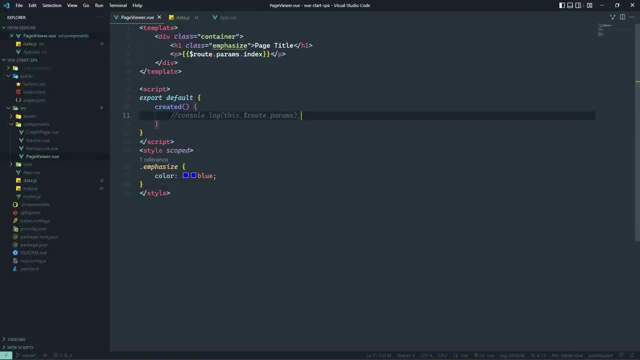 And let's go to page viewer because this is where we are going to be displaying that page. 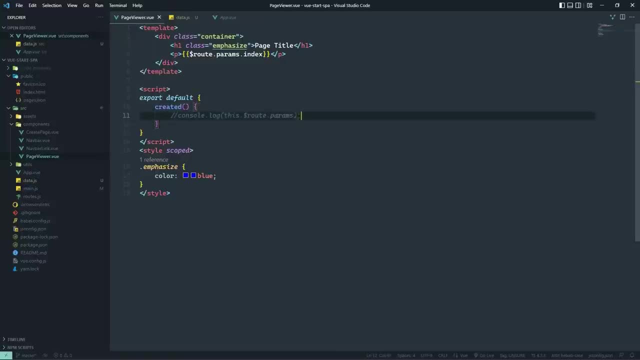 So inside of the created hook, sounds like a pretty good idea. Sounds like a pretty good place to fetch that page. 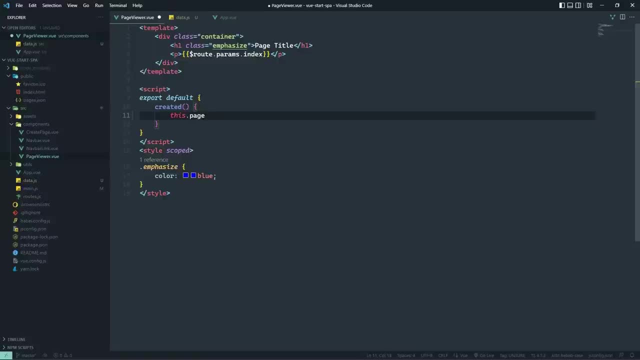 So let's say that we're going to have a data property inside of this component called page, and then we will use our pages object so that we could get a single page. 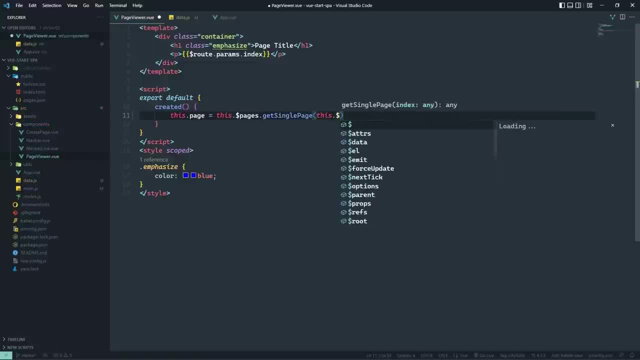 And then we want to get the page at the given index at the provided route. So we will access the route params, and we want that index value. So with just that change, although no. That's not just that change. We do need to define the page, and let's initialize this as null. 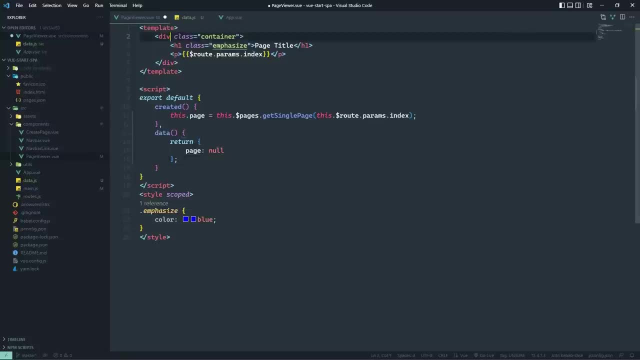 That way, whenever we display our component, we can use the VIF here to check to see if we have a page. And if so, then we want to go ahead and display that information. Otherwise, we would want to hide it so that we don't run into any errors there. 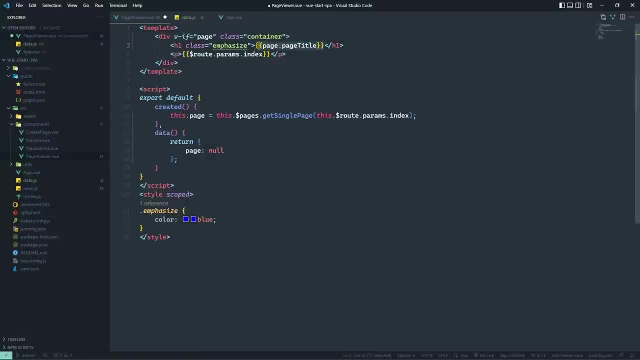 So we want to output the page title as well as the content. So let's do that. Add that back as our output. 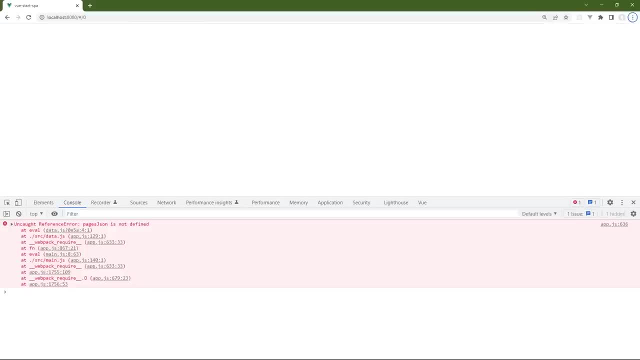 Let's go to the browser, and let's see this in action. We have an error, reference error, pages.json not defined. 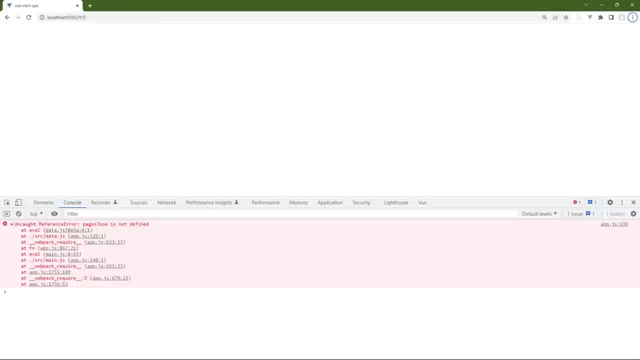 That is inside of data.js, and so pages.json. I'm glad I left that file open. 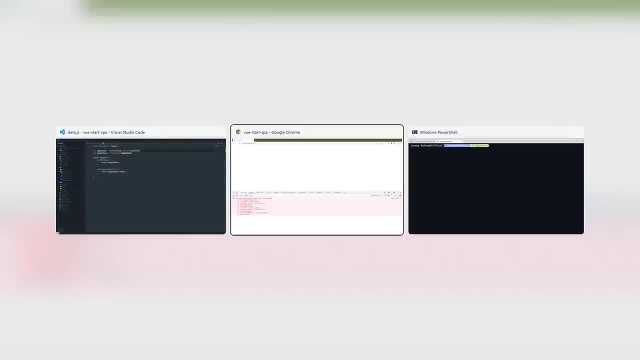 It's amazing what one missed keystroke is going to do. So let's go back, and there we have it. 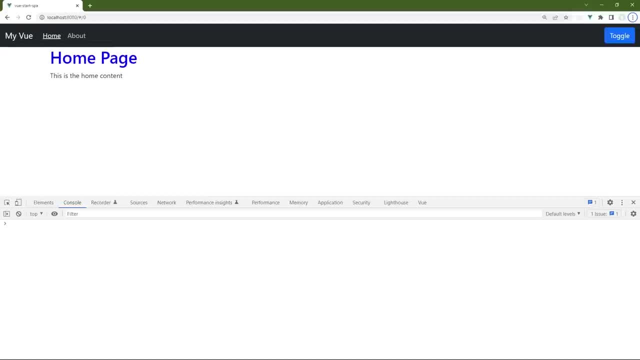 We can see the content for our home page. Now, if we click on About. 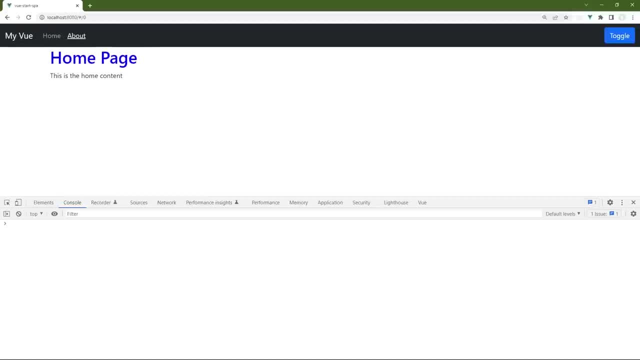 Nothing is going to happen, of course, because we have written nothing that is going to display the information because we haven't set up our application to actually navigate using the router. 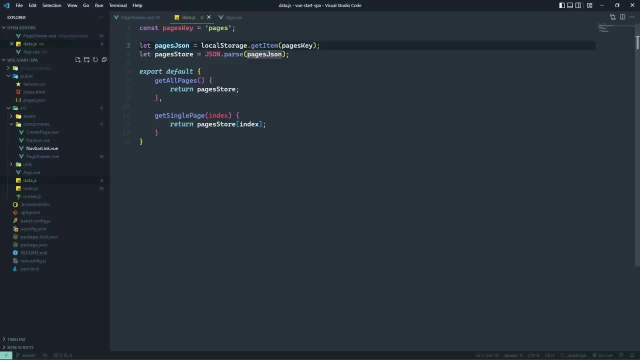 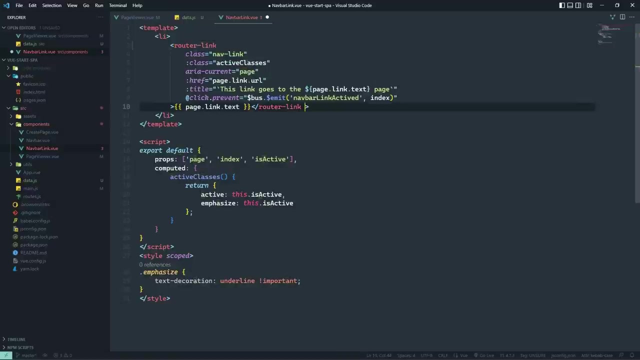 So we can do that by going to the navbar link. And instead of outputting this a element, instead what we want to use is called router link. It's a component that's automatically loaded for us, so that all we need to do is just use this router link. 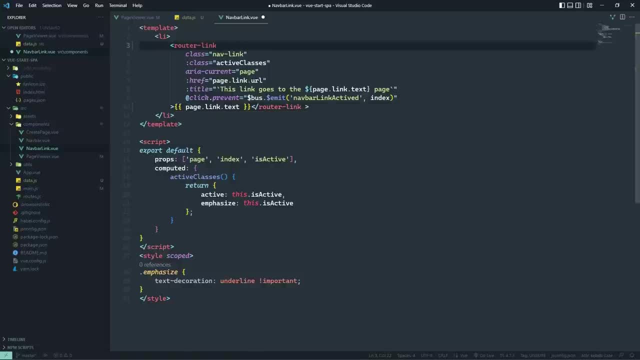 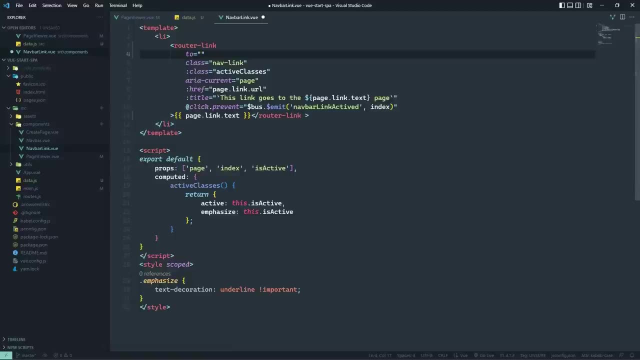 It doesn't have an href attribute. Instead, what it has is a to attribute. And then we specify the path that we would want to go to. So in this case, it would be a slash followed by whatever index. So we want to bind this then so that we can dynamically generate this using JavaScript. 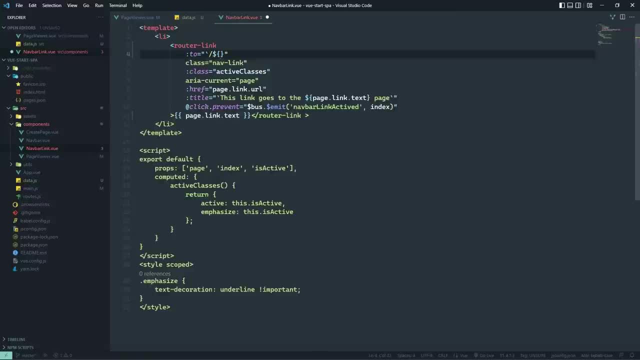 So our URL is going to include the route params index here. So it doesn't matter what component that we are in. The route is going to be the same as long as that component is displayed. 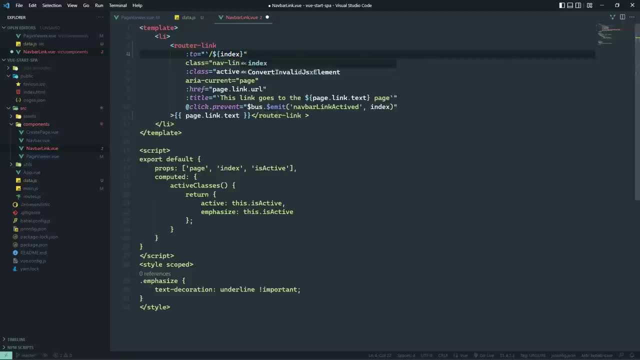 And then we want the index there. So that should give us our link. Let's see, we don't need the click event. This is, of course, going to break some things, but that's okay. And in fact, in this particular case, it's not because this, it was for telling the app component that this is the active page. So, we don't need that. Now, everything else should be okay. I don't see any other errors. 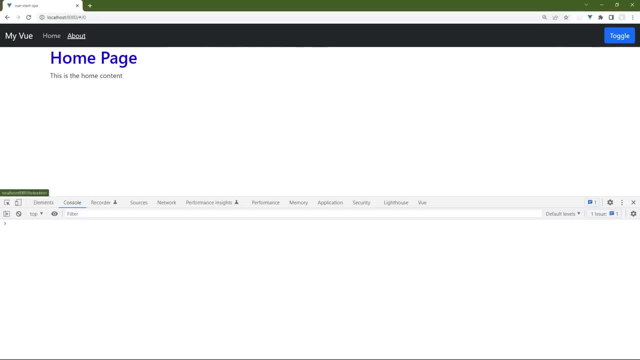 Now, as far as tracking the active page, it's going to be a little bit different now because, well, as you can see, that's not working. 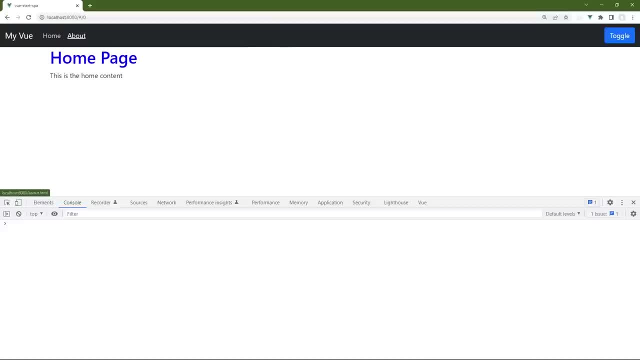 But you can also see that we aren't actually navigating to those different pages as well. 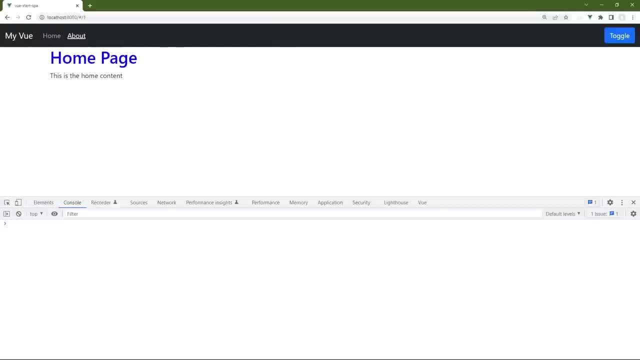 And the reason is very simple. It's because the page viewer component is already loaded. 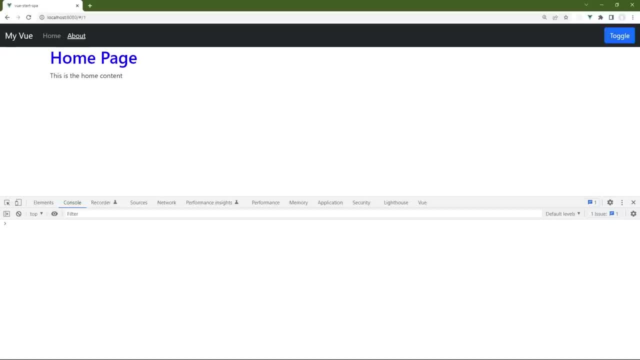 So here's the thing about navigating using the viewer. If you navigate to a different component, then everything's fine. You don't really need to do anything extra. 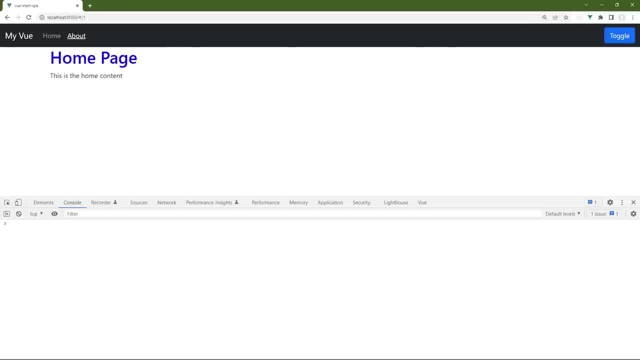 However, if you are navigating to a component that is currently loaded, well, then you have to tell your application, hey, the route parameters changed, so load new data into that component. 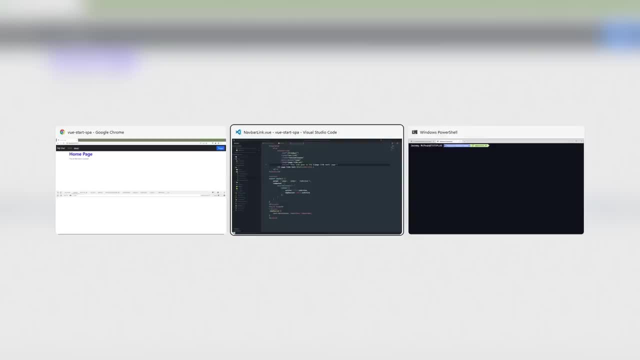 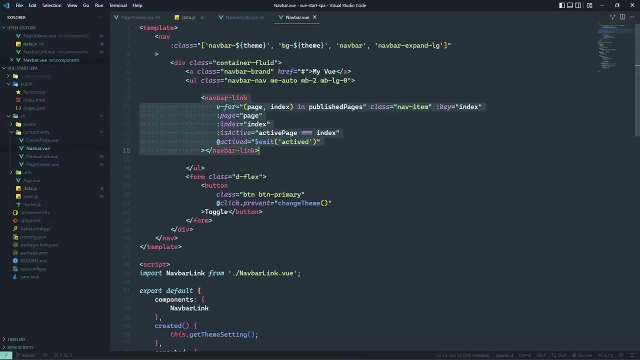 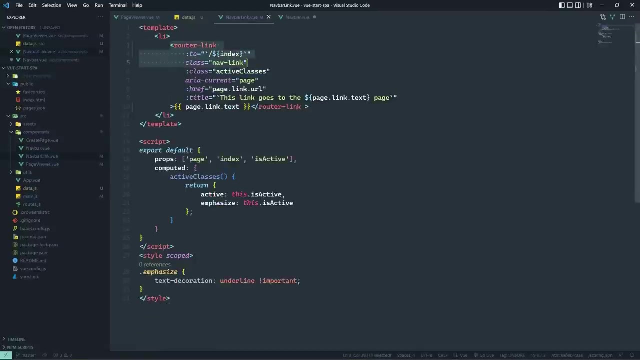 Now, we can first of all demonstrate this by adding a link to our create page. So let's do that inside of navbar because that's where we build the links based upon our pages. Now, we're going to add another link for the create. And I wanna make sure that we use all of the right CSS classes. So let's copy this router link and let's paste that into navbar. 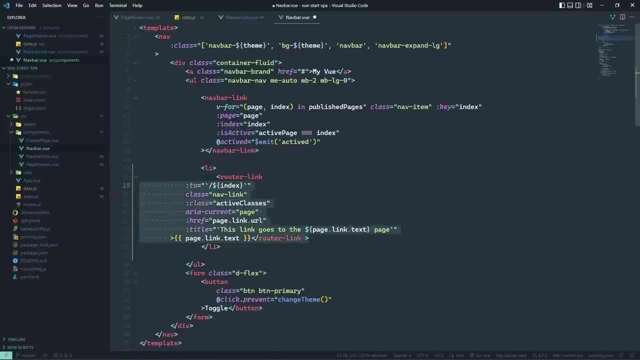 Cuz a lot of this is going to be the same because we still want to use a router link in this case. 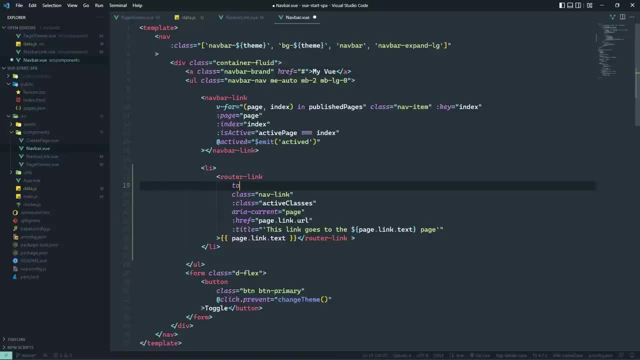 However, we can use just a straight up normal to prop here to where we want to go to slash create. 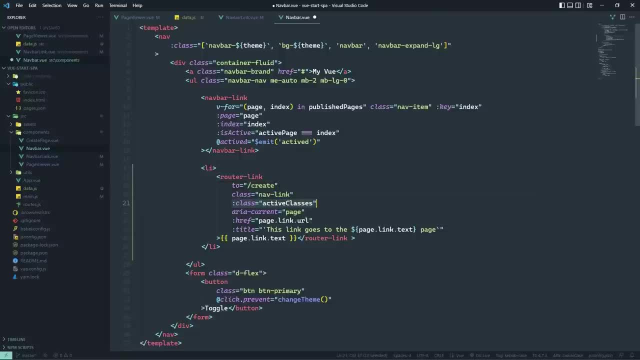 Now, let's get rid of the class binding for active classes because that doesn't mean anything here. 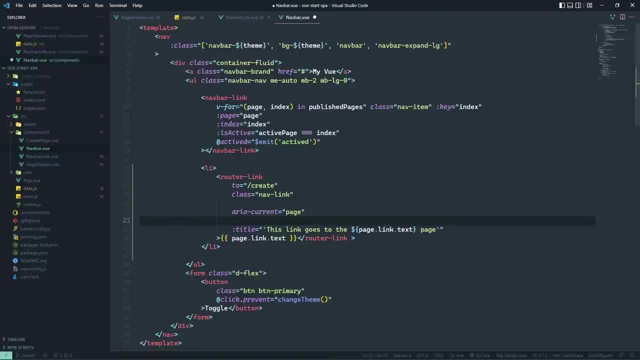 We don't need the href either and in fact, we should get rid of the href in the navbar link. 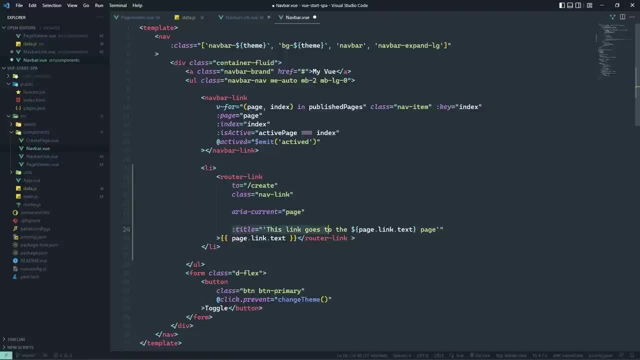 So let's do that. And then the title we don't need. 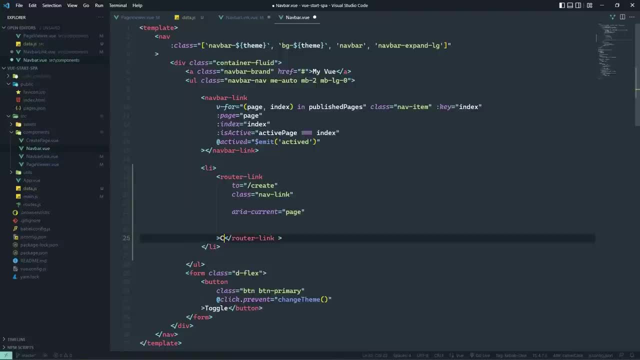 And as far as the text of this, let's just have it as create page. So with those changes done, let me make sure all of the files are saved. 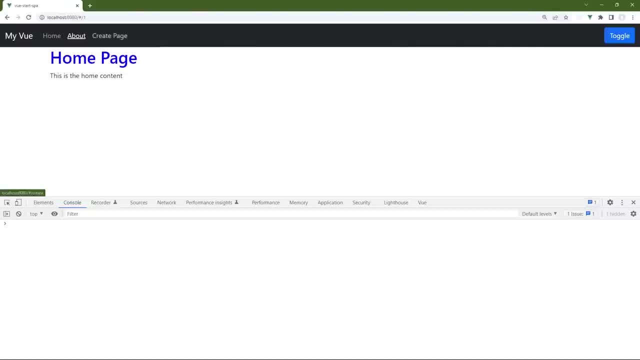 We can go back to the browser and now we see create page. 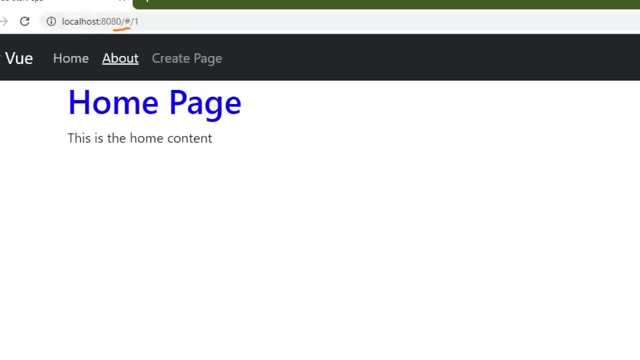 So we are currently at the page with an index of one, which is about. But notice that we are still displaying homepage. 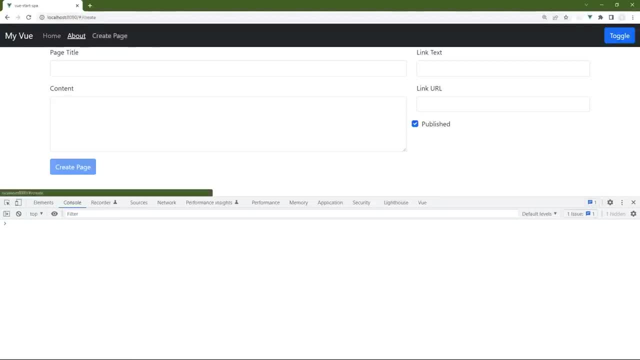 But if I click on create page, we see, well, it navigated. Whenever we click on about, we see about. If we click on home, we don't see that. If we click on page and then go back to home, then yes, the content changes. 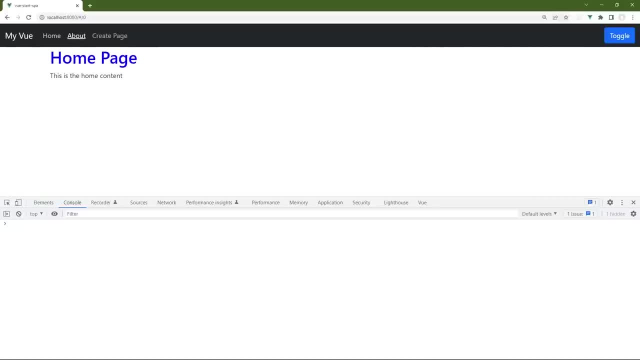 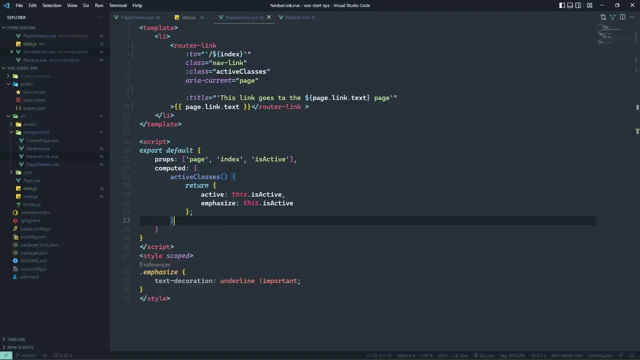 So in this case, we're going to add another page. So as long as you navigate to a different component, you don't really have to worry about anything. If you navigate to the same component, then we have to tell the application, hey, you need to update. And the way that we can do that is with a watcher. In fact, there's two different ways that we can do that, and we will look at how in the next lesson. 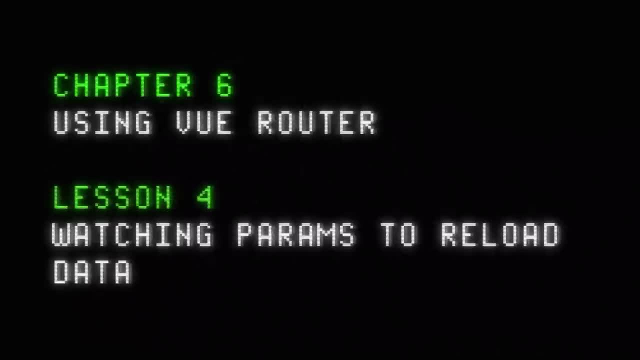 In the previous lesson, we set up the page viewer component to actually display the content of a page. 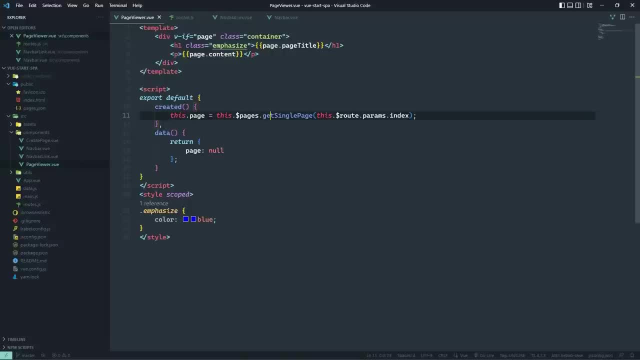 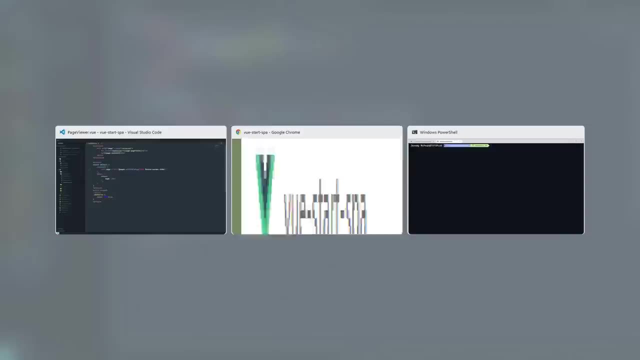 We created a makeshift centralized data store that gives us an easy ability to fetch the page based upon the index, and then we display that information. 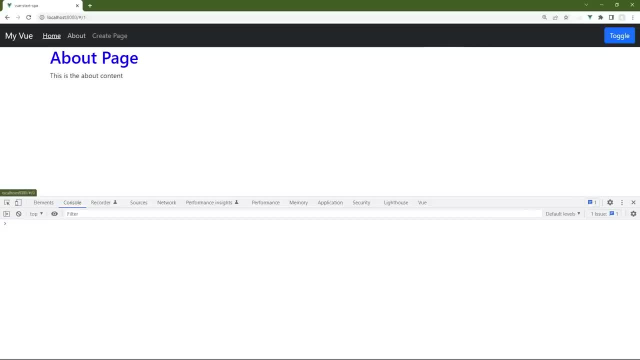 But there's a slight little problem. If we navigate to a page that uses a different component, then everything works fine. But if we navigate to a page that uses the same component, such as the home and about links, both of those use the page viewer component. 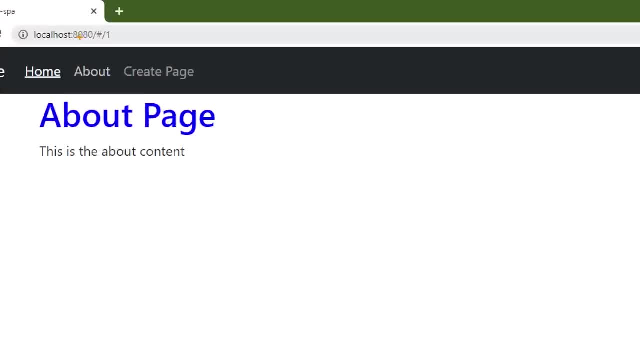 And notice that, even though I'm clicking on them and the values in the URL changes, 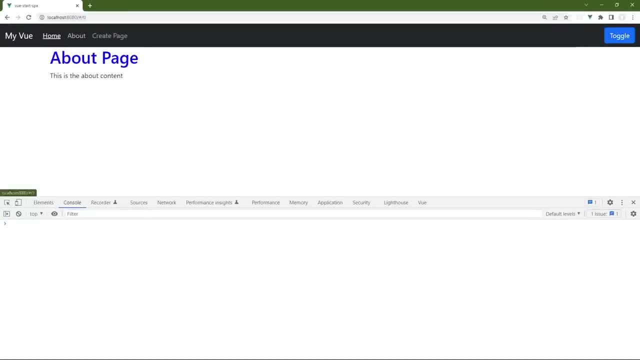 the content doesn't change. And the reason is very simple. 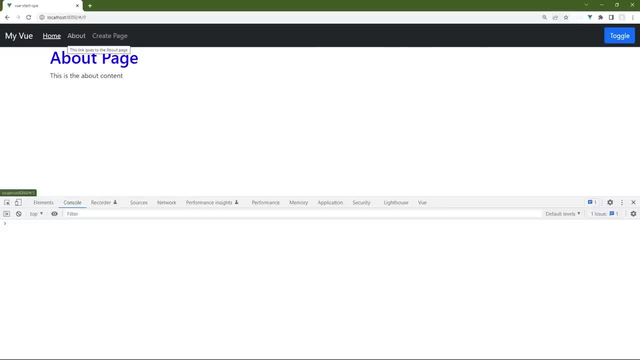 The page viewer component is already loaded into the application at this point, and it's loaded with whatever page content we first navigated to. So I went to the Create page, then I clicked on About, and 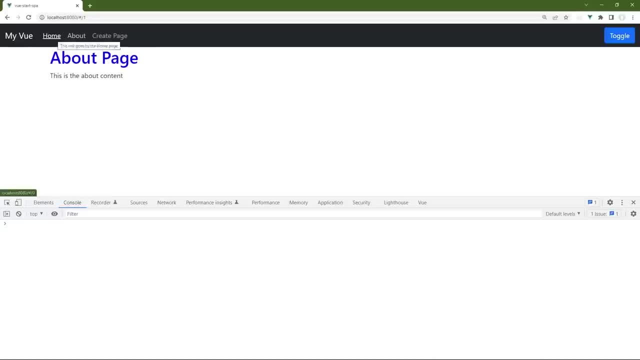 that's the content that we see. So even though the route params change, the content is still there. 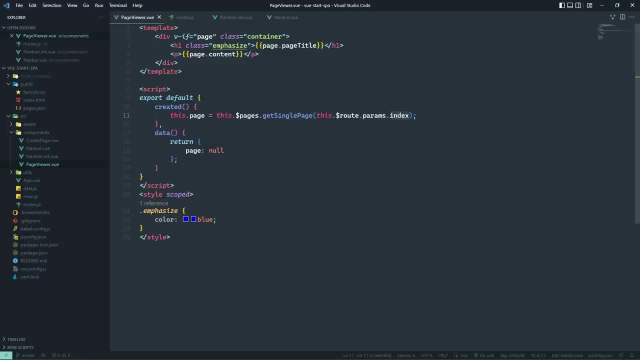 The page viewer component doesn't necessarily know that it changed and that it needs to update the page appropriately. So basically, what we need to do is use a watcher. We need to set up a watcher so that the page viewer component knows when 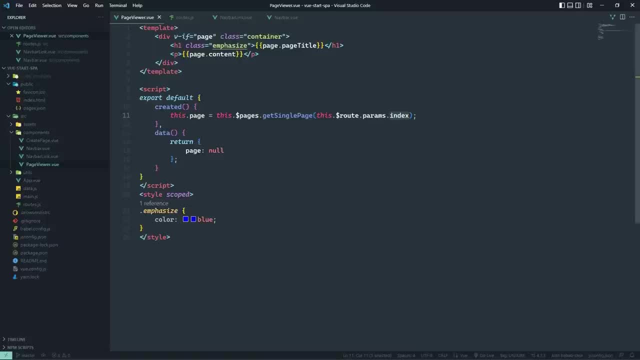 the params change, and then it will load the new page when that occurs. 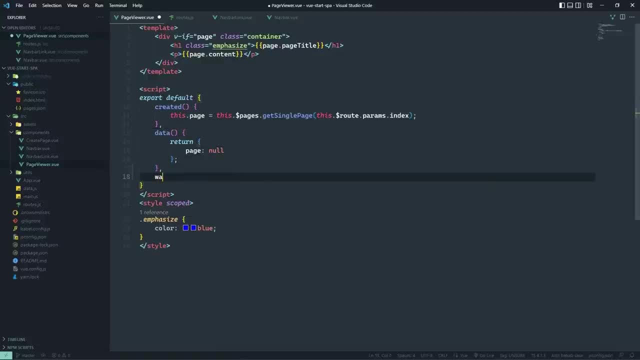 So great, we've written watchers before. So we will add the watch option. And then what do we use here for the watcher name because this would normally be some kind of simple identifier. 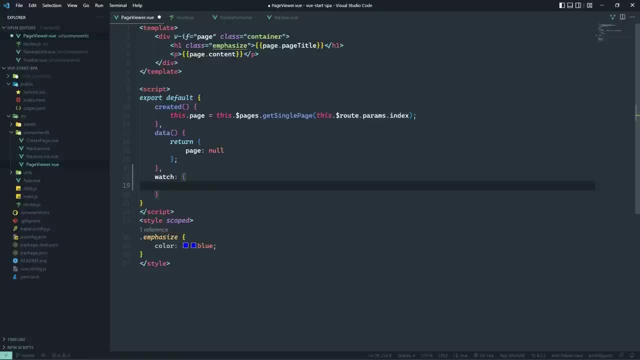 It would be a data property like page in this case, or it might be a prop name. 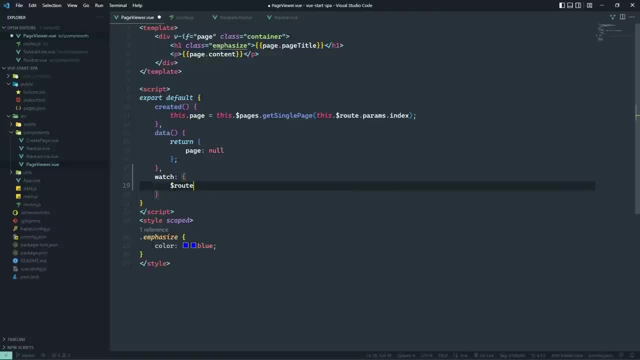 How do we do something that is reliant upon our routes.params.index? 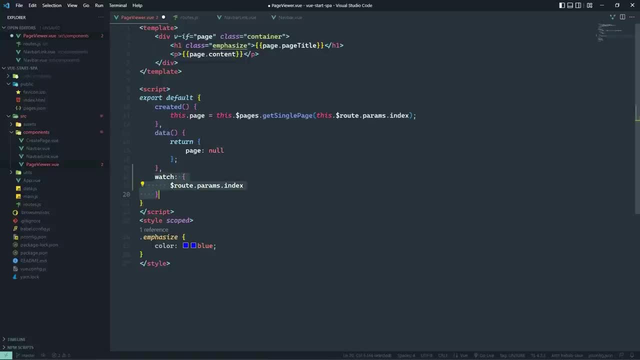 Well, we don't, at least we don't use the watch option. Instead, we can set up a watcher programmatically using the watch method. Actually, it's $watch. And the concept is somewhat the same. The first argument that we pass to the watch method is a function. And the return value is whatever it is that we want to watch. So in this particular case, that would be our route params. 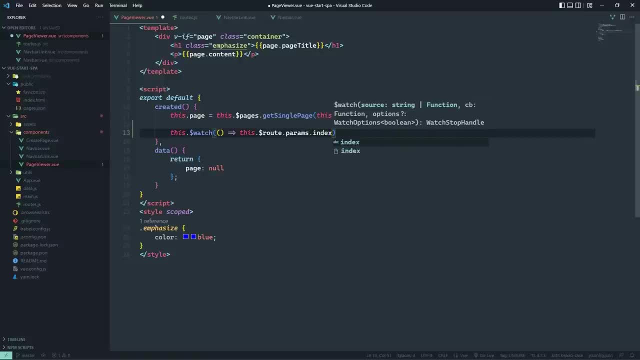 Or we could say that we just wanted to watch the index on our route params. But if this was a component that relied upon multiple params, it would make a whole lot of sense to just watch. 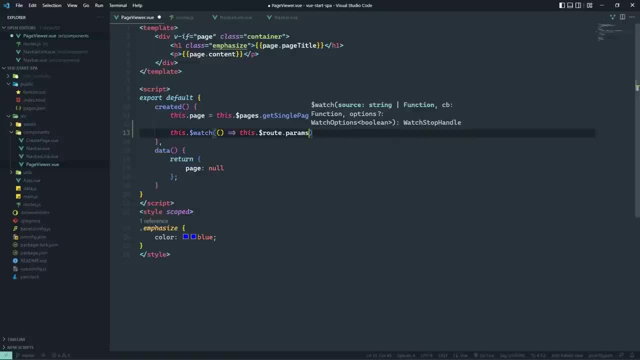 For the params itself, so that when that changed, then we could update the data. And that's the option that I'm going to go with here. 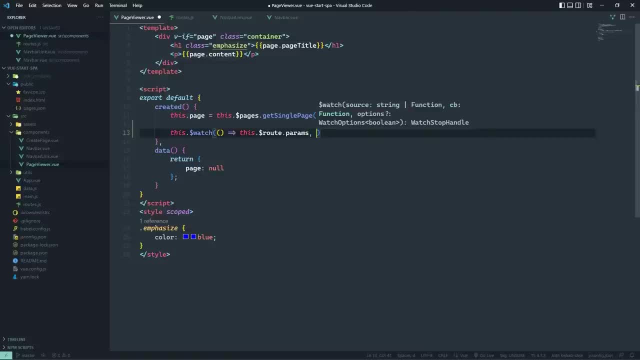 Okay, so that first argument is the function that returns whatever it is that we want to watch. The second argument is the function that is going to execute when the params change. And in this case, it starts to become very much like any other kind of watch 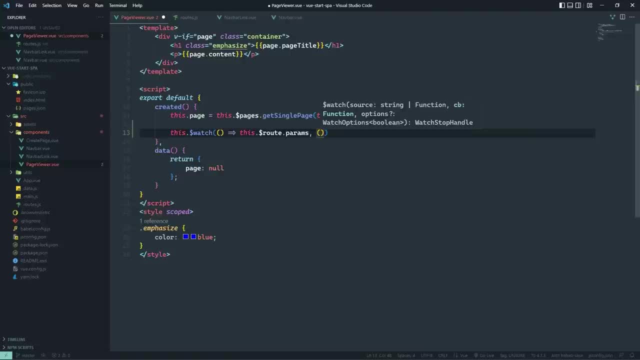 implementation, so that we have two parameters here. 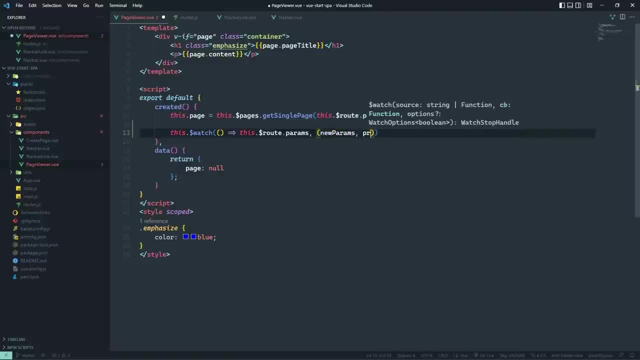 The first are the new params, the second are the previous params. And then inside of this function, we just do whatever it is that we needed to do. 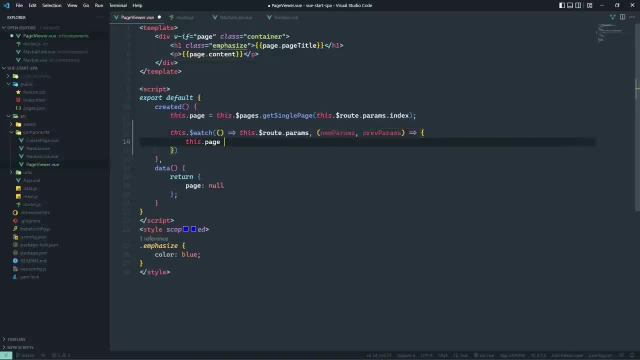 Which in our case, is to change the value of our page. So that once again, we use our pages data store to get the single page for 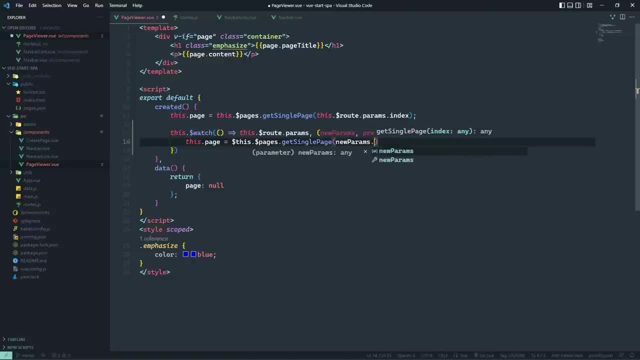 the index that is provided by the new params. 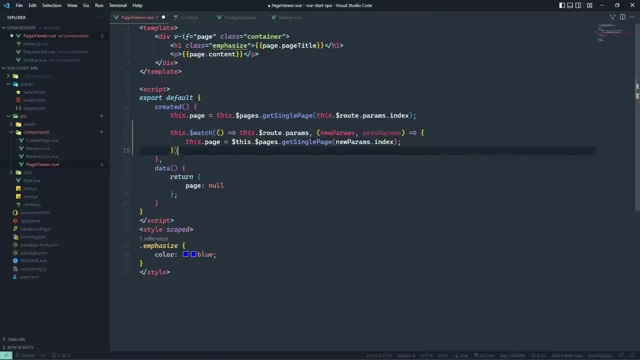 And so there we go. By saving this, we will be able to go to the browser. And we will see this work. 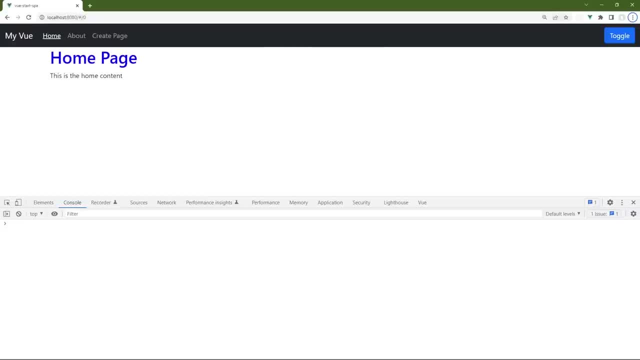 So we see that it switched to home page. 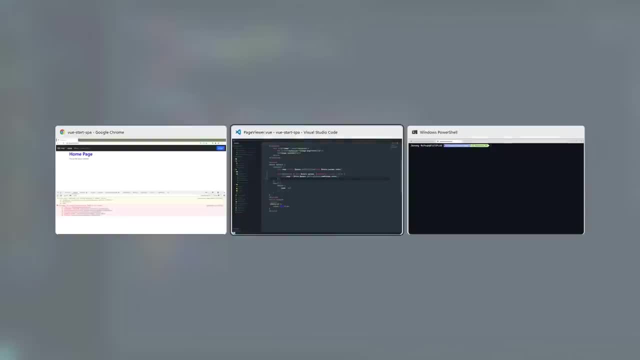 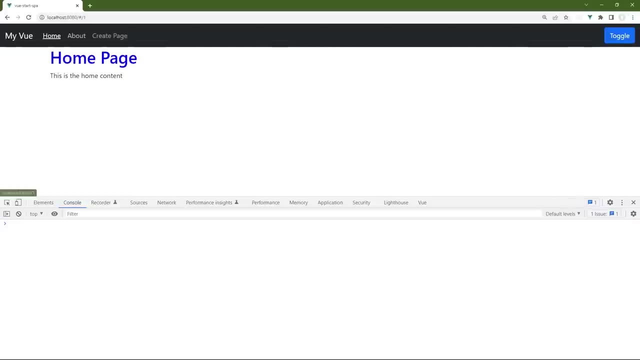 If we click on about, we get an error. That's because dollar sign this does not exist. Yeah, of course it doesn't. So let's go back. Let's clear out the console. And now let's click on about. Okay, let's refresh the page. And now let's click on about, which was already loaded because that's what the URL was. 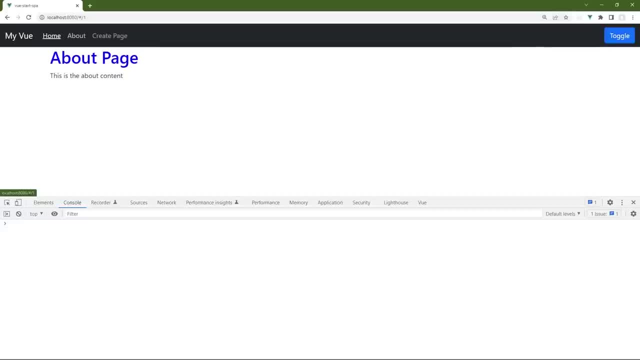 But if we click on home, we can see that the content changes. If we click on about, I mean, we can click back and forth all day long and that content is going to change. 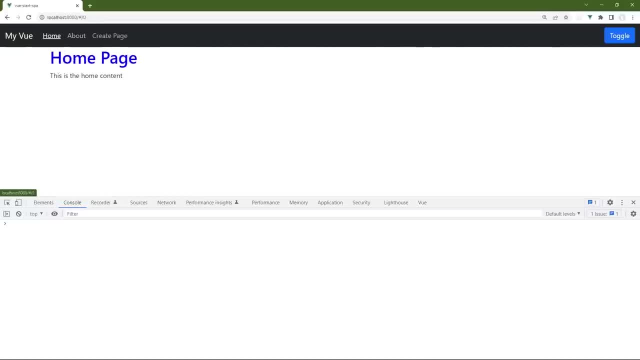 If we click on create page, that still behaves as it did before. So this is one way that we can go about setting up our components to 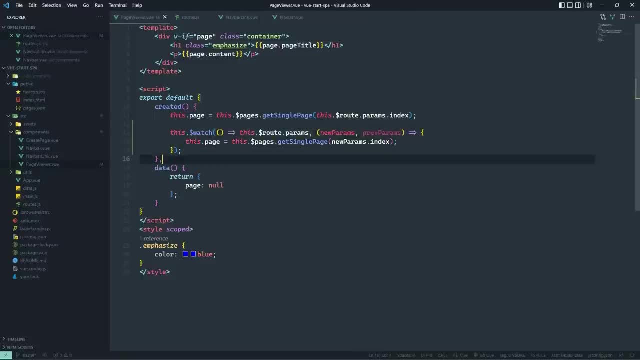 respond to when the params change. The second way is a little more straightforward and 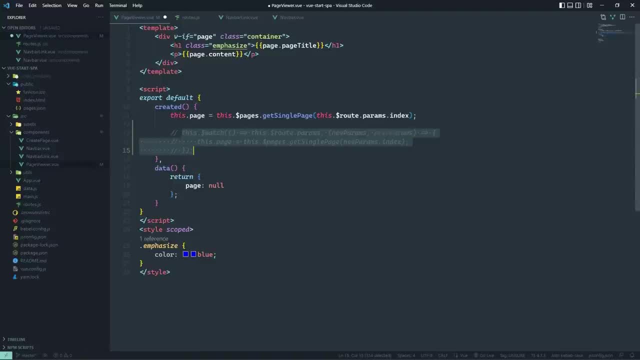 it's a lot more familiar. And that is, we can essentially tell our application that for this route, the route that's using the page viewer, we want the params to be passed as props. 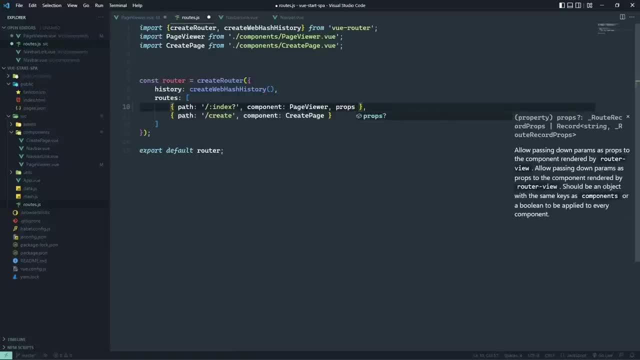 To do that, we pass in another option simply called props and we provide it the simple value of true. 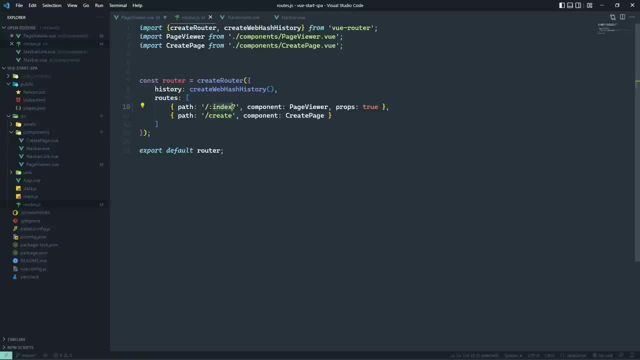 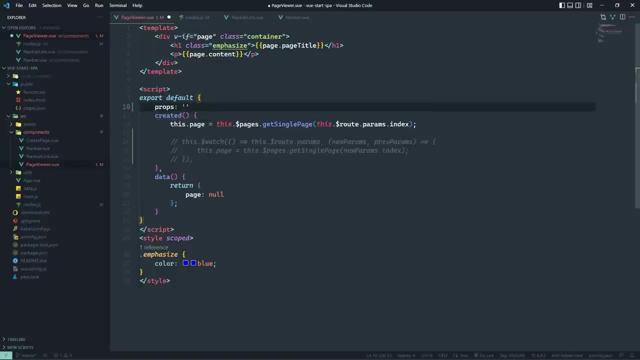 So now the value of index is going to be passed as a prop. Now this means that we need to define that prop. So let's go ahead and do that. 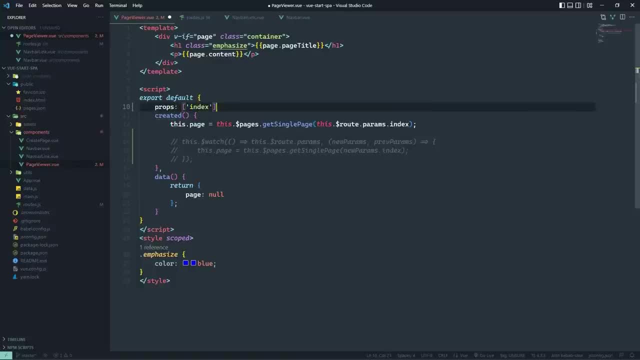 We don't need to do any kind of validation. We can just use the simple declaration and then we just need to go ahead and update our code appropriately, so that inside of the created hook, we just use simply this.index to refer to our index. 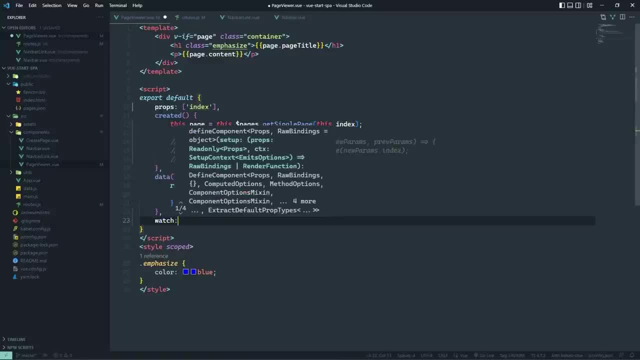 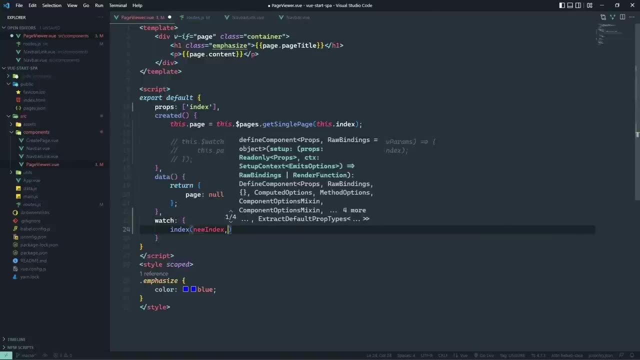 And now that we have a simple identifier, we can use the watch option. So that we can watch for index to change. We have the new index and the old index. So that's now we can simply set our page data property to the page with the given index. 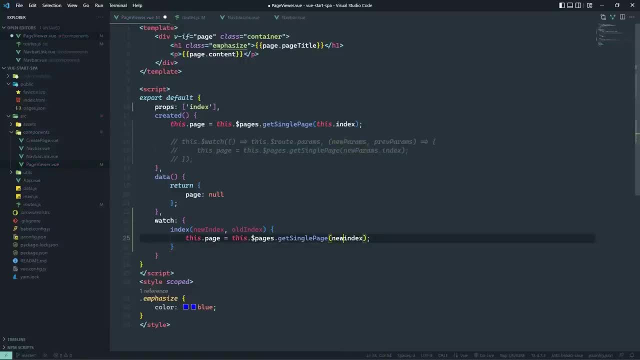 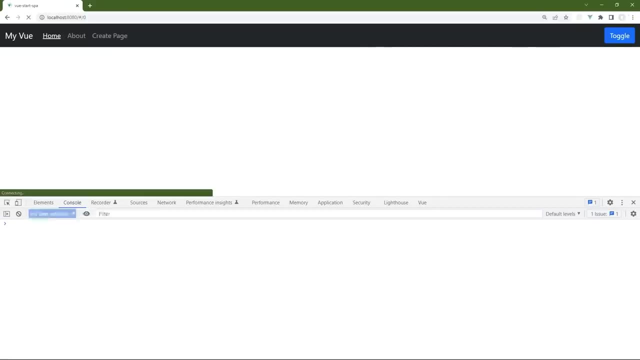 So let's just copy and paste and use the correct variable name. Same idea, but it's a bit more familiar. So let's go back to the browser, let's refresh the page. 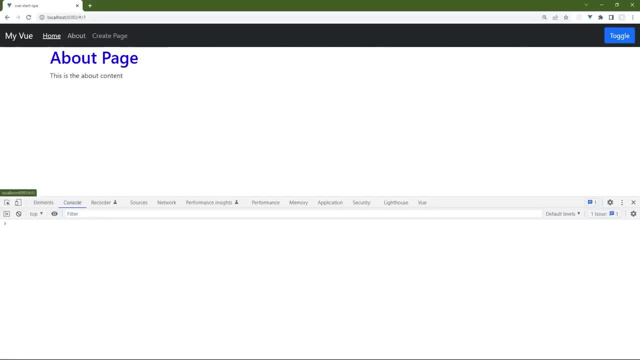 Home page is loaded, we navigate to about, we navigate to home, about. 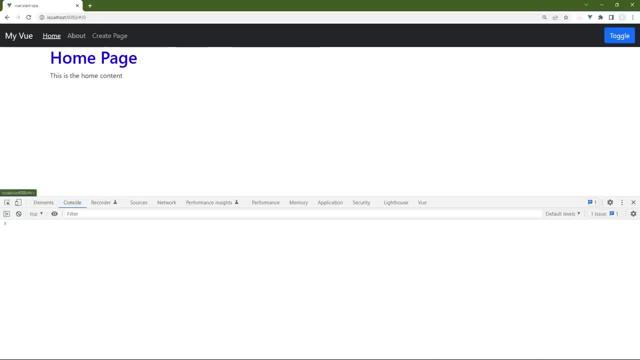 Once again, everything works as it should. Now there's no right or wrong way to go about this. 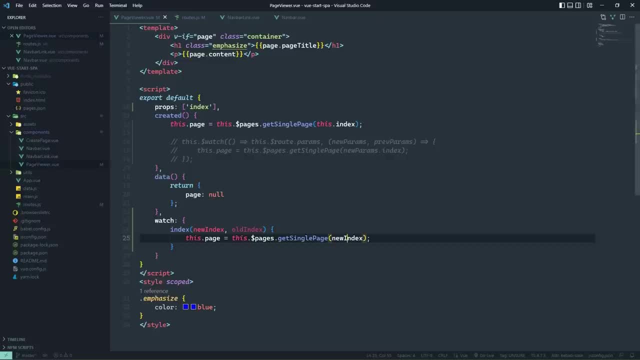 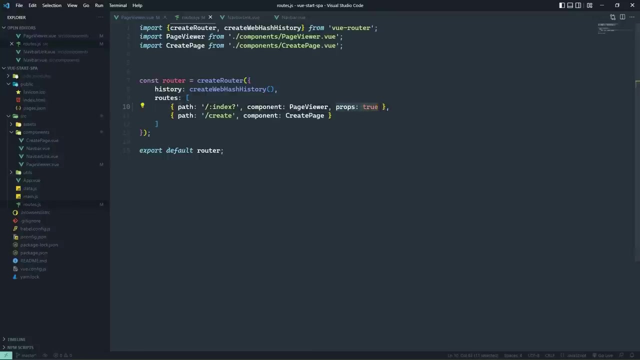 You can use whichever option that you want. If you want to define the watcher programmatically and use the route params, then feel free to do that. If you want to use the more traditional and more familiar approach of using props. You do need to tell the route to use props, props is true. That will pass the params as props, so that it gives you a little bit easier 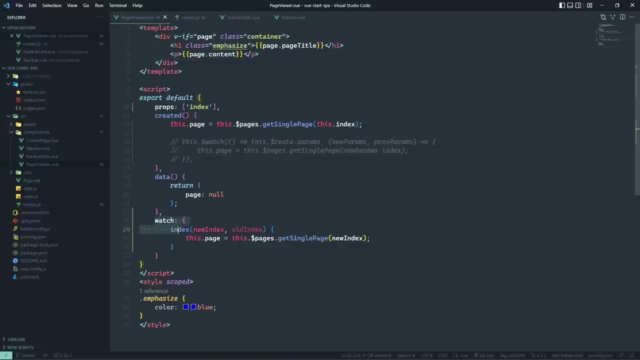 access to that data, and you can use the options to define your watchers. 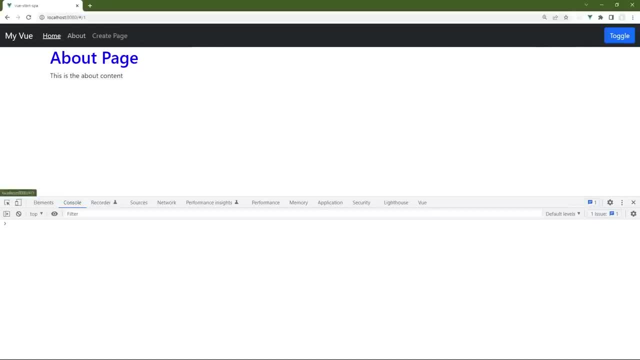 Well, in the next lesson, we need to go back to the browser and try to address the active link. Because now that we are using the view router, and we are loading this content differently, how we handle the active link is, of course, going to change. And we will look at that in the next lesson. 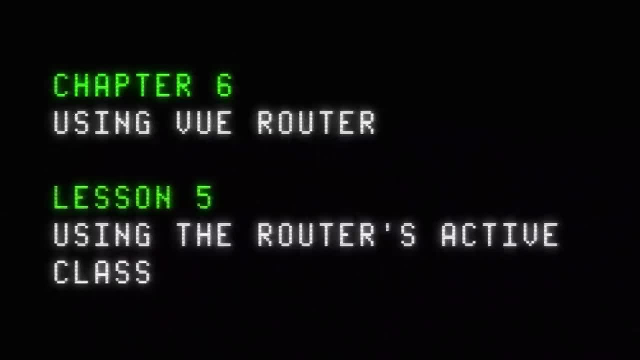 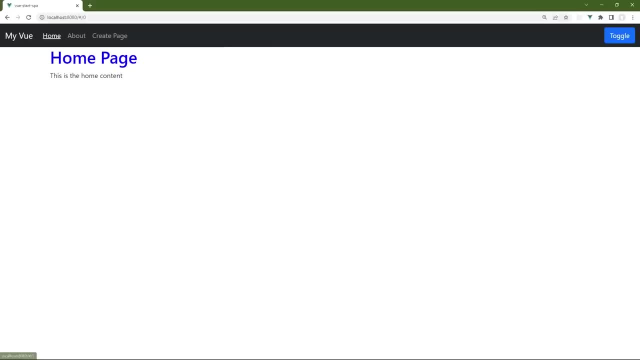 I think it goes without saying that if you want to provide navigation for your application, then you need to use view router, because that is, after all, what its purpose is. 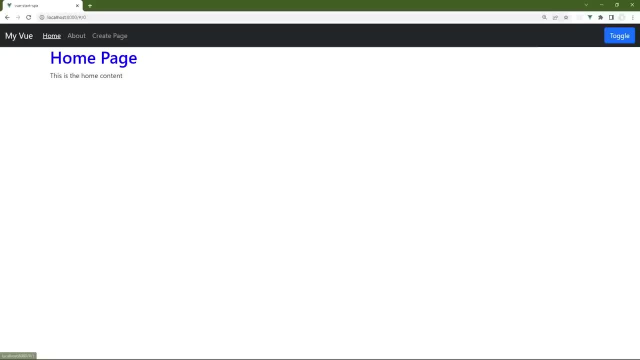 But one of its features is to keep track of the active link, which is something that's 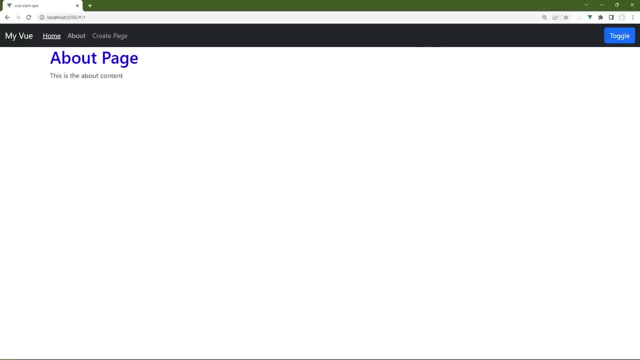 that we have done on our own. And I guess technically, we haven't kept track of the active link. We've kept track of the active page, and then applied the appropriate CSS 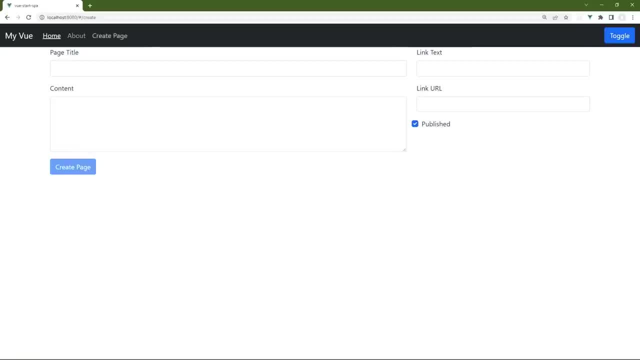 for the link associated with that page. Which meant that we had to plumb our application to track that particular value. Well, that's built in with view router. 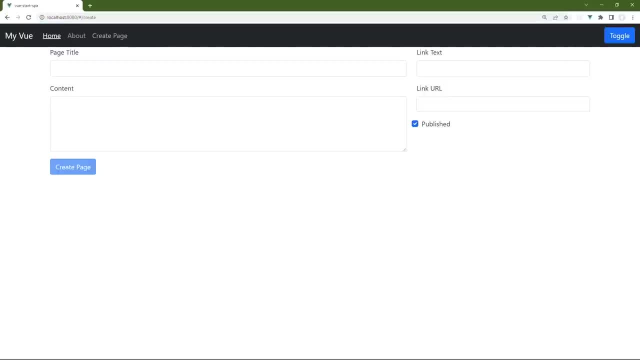 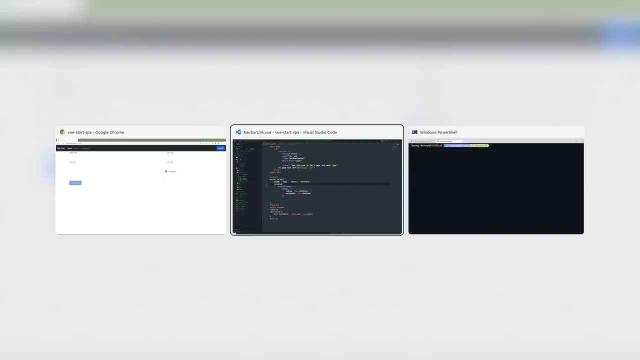 And in fact, it's based upon the URL. So instead of keeping track of something internal, it is looking at the URL and matching that to the paths that we have defined 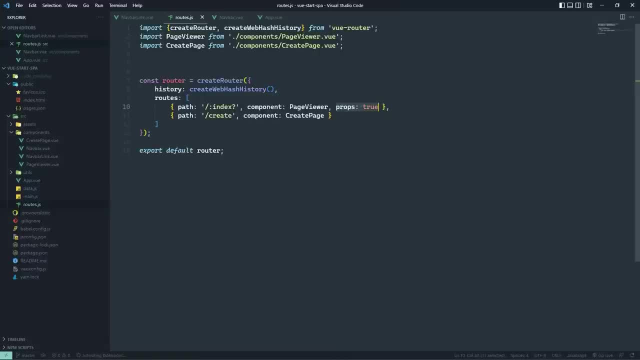 inside of our routes, and so then it knows what link is active. 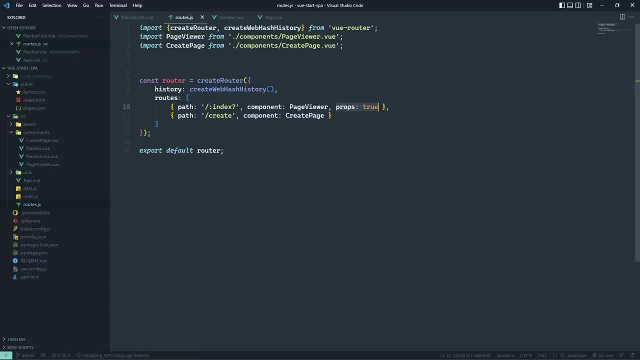 The only thing that we need to do is tell it what class that we want it to use when a link is active. 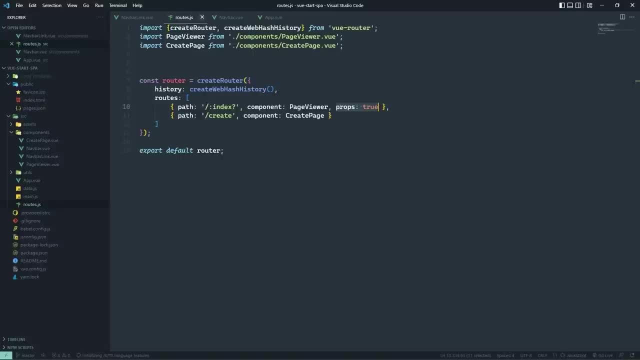 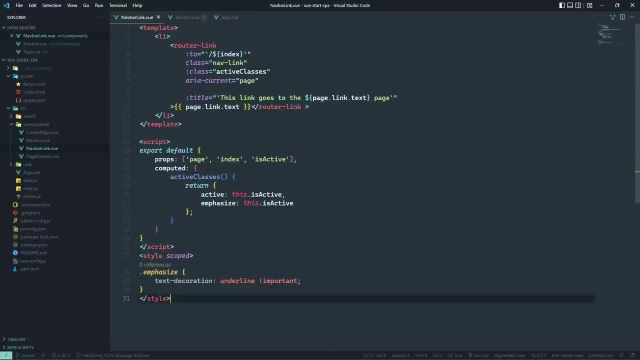 So let's go to our navbar link. And this is going to greatly simplify our navbar link, as well as navbar and app. So in navbar link, we're gonna have to go to our link, and we are using this active classes object. This was a computed object that allowed us to set both the active and emphasize classes. 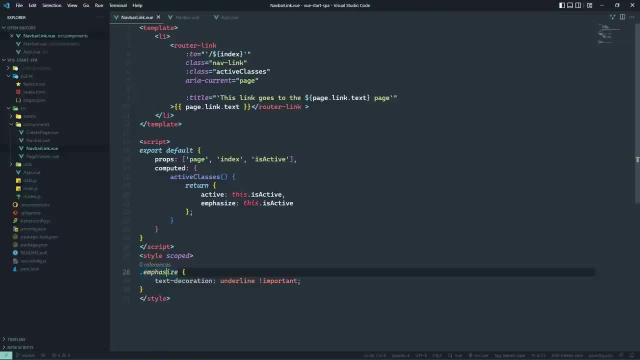 I want to get rid of the emphasize just because I don't really like how it looks. But we'll use it first, so that you can see that it is indeed working, and then we'll get rid of it. 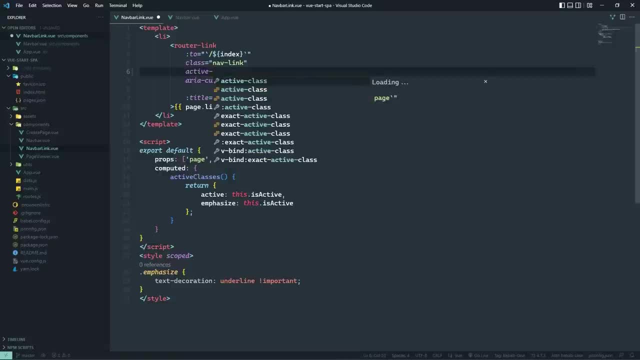 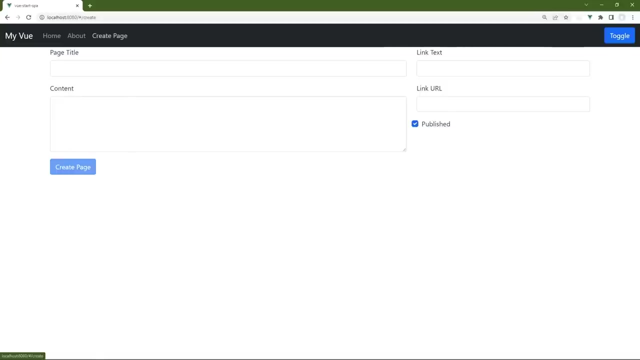 So all we have to do is add a prop called active class. And then we provide the CSS classes that we want. And then we're gonna click on the active link to apply to the active link. So in this particular case, that would be active, and then emphasize. So let's make that very simple change. Let's go to the browser, and we are on create, which we did not add that active class prop to, but we will here in a moment. 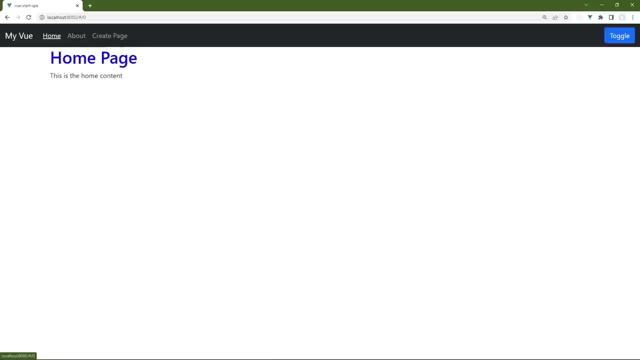 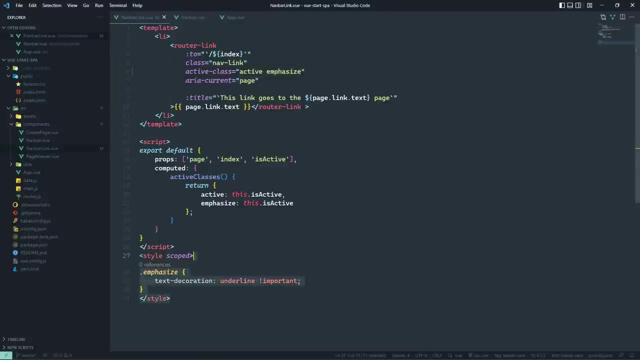 But if we click on about, we can see that the active classes are applied. If we click on home, the same is true. Now, to prove that this is based upon the URL, I'm not going to click on about. I'm going to change the URL, so that instead of the index 0, we're gonna use the index 1. I'm going to hit the Enter key, and voila, we can see that the active link changed. So I'm gonna get rid of that emphasize, which means that we can get rid of the style. 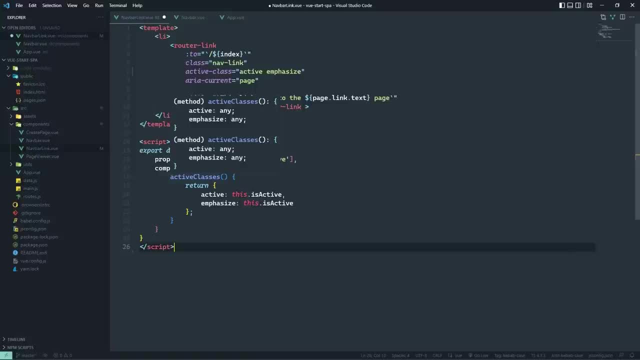 It also means that since the active class is being handled by the router, we don't need this computed object of active classes. 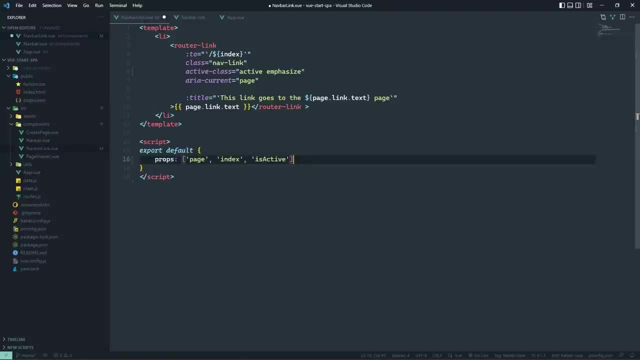 So we can get rid of that. Now, the active classes object used this index, 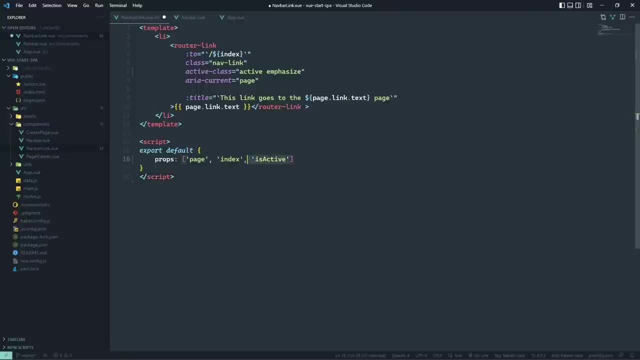 this is active prop, we don't need that either, so we can get rid of that. So that this component is only going to use the page and the index, and that's it. 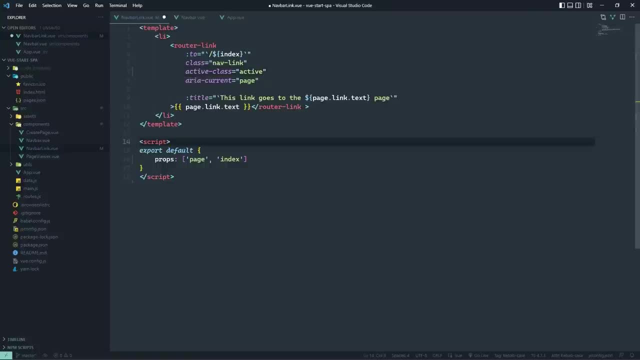 I think that's it, that's all that we need. So by just using the active class prop on the router link, we were able to greatly simplify this component, so that's one. 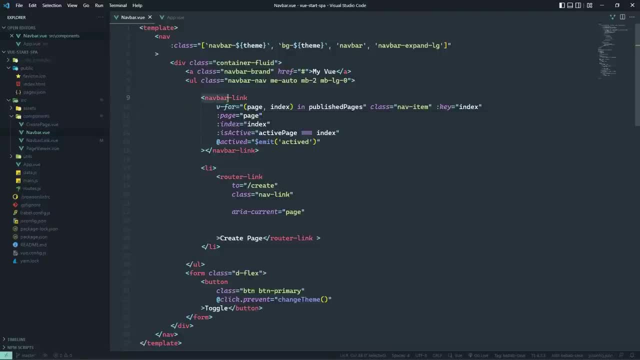 Let's close that, let's go to navbar. So our navbar link, this was generating the links for the pages. 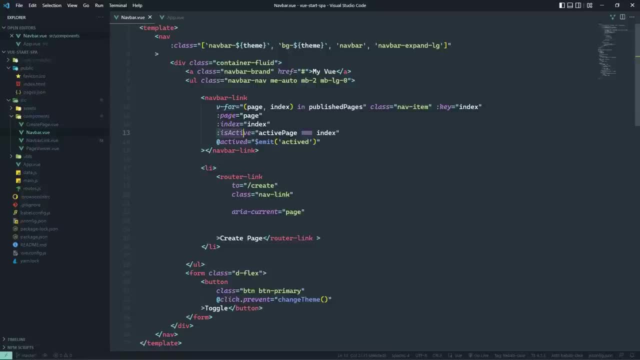 We need the page, we need the index, we don't need the isActiveProp, so we can get rid of that. 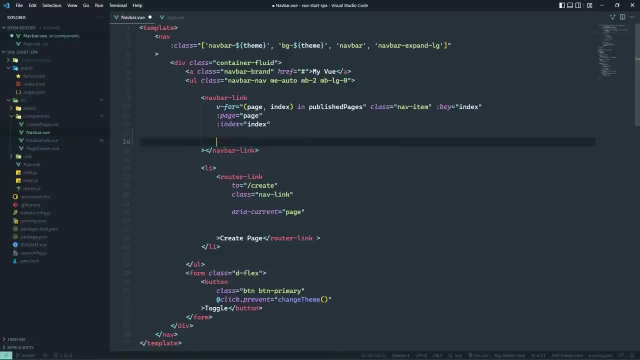 We don't need the activated event, so we can get rid of that. To the createPageLink, we do want to add that active class. 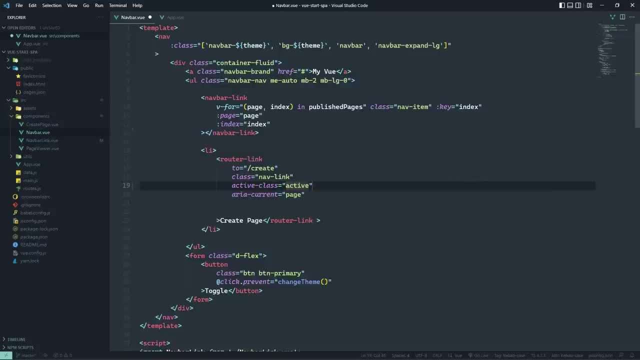 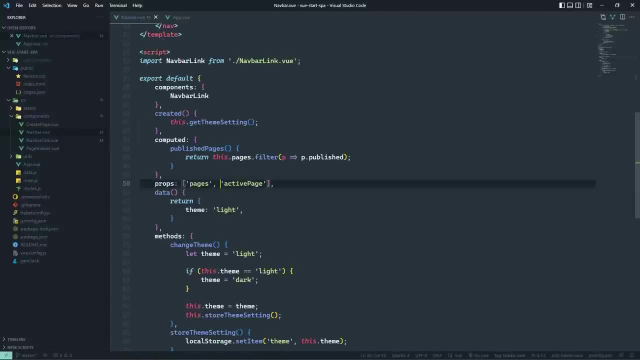 So we will set that to active, and everything else will be fine. So let's take a look at our props, because we did manage to clean this up so that we don't need active page anymore. 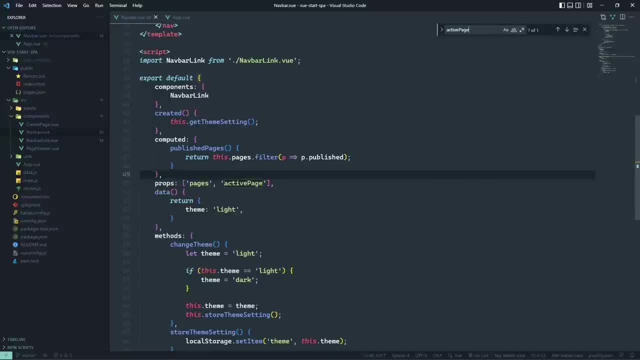 And in fact, let's search. Let's make sure that we aren't using that anywhere else. 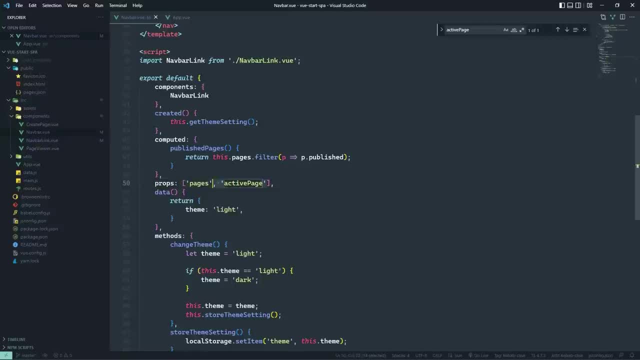 It looks like, no, we're not. So we can get rid of active page, so that this is only relying upon pages. 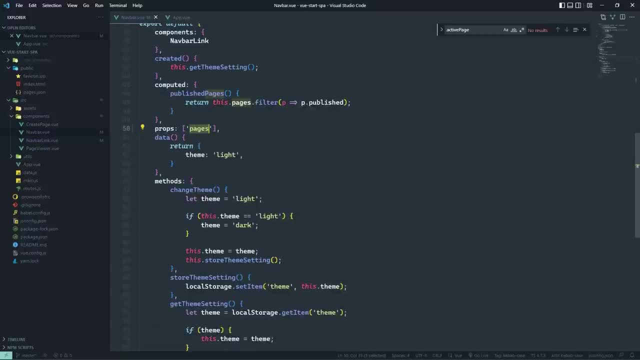 Which, that is something that we can change as well, but we'll get to that here in a moment. 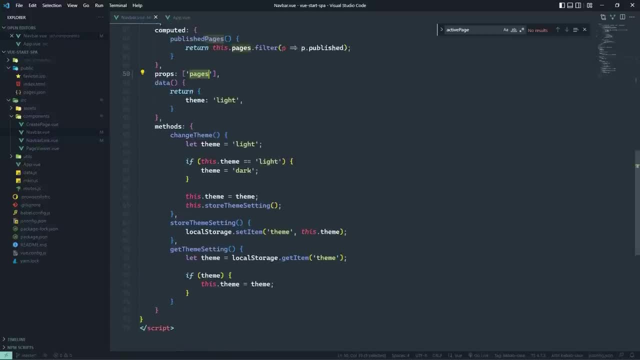 Let's make sure that there's nothing else. All of these are for the theme, so we are good there. 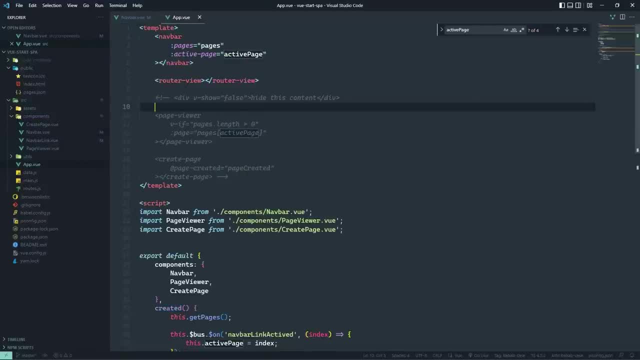 So now let's go to the app component, because this is where that active page was being passed in, so we don't need that either. Which means. 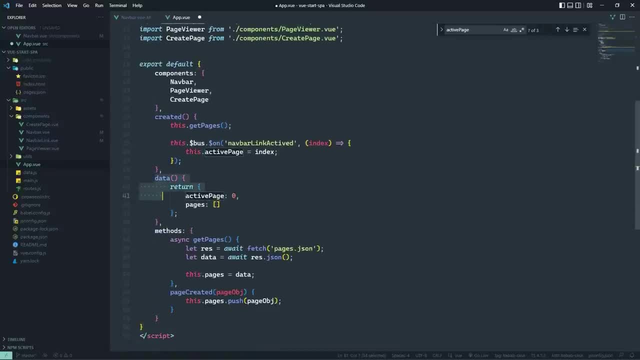 That we can get rid of our data. In fact, we can get rid of the created, well, at least for the most part, because we were listening for this global event of navbar link activated. That was primarily so that we could set the active page. We don't need that anymore, so we can get rid of that. 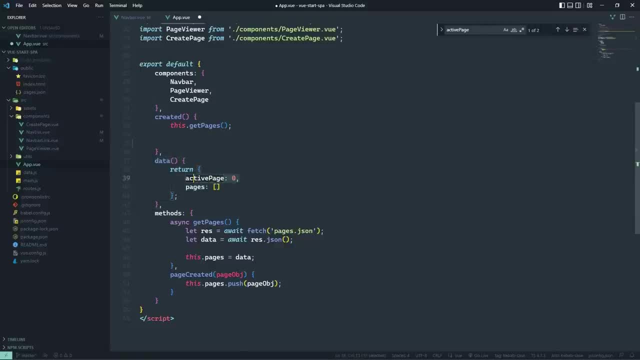 We can almost get rid of our data if it weren't for the pages array, which, well, let's go ahead and let's get rid of that. Let's also get rid of the created hook, because we aren't gonna need that. Let's get rid of the. 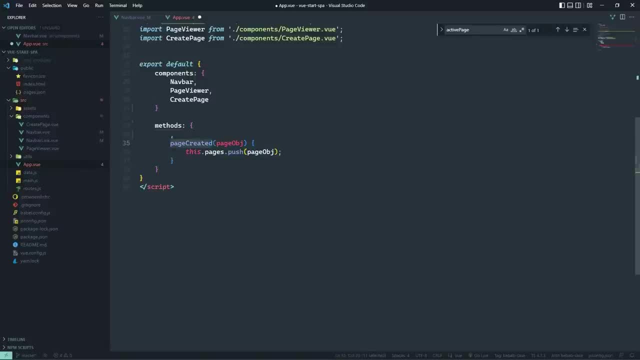 Get pages method. We'll keep this page created just for the time being. 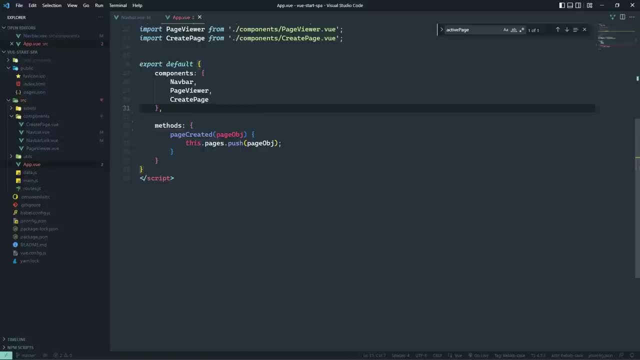 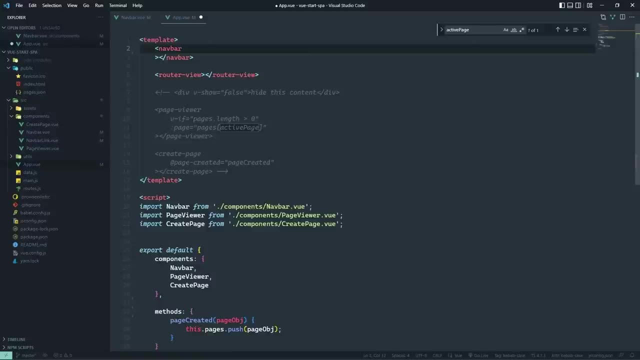 We will probably get rid of that at some point later. Now, the reason why I'm getting rid of the pages altogether inside of app is because now that we have our data centralized, the navbar can load 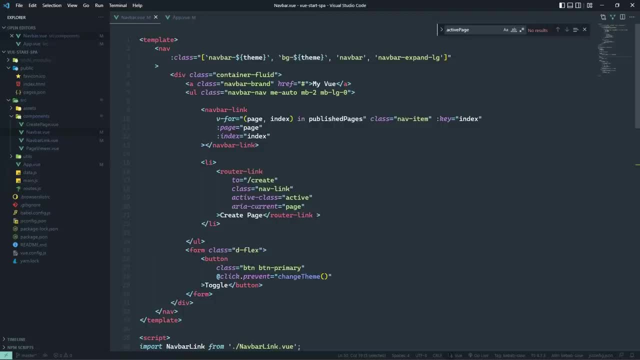 the pages itself. So let's go back to the navbar, and we are going to add pages to our data. 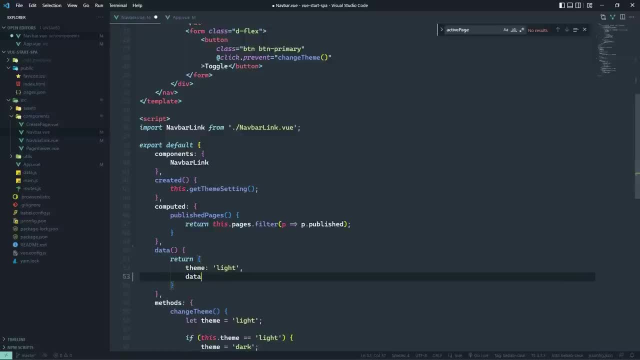 We don't need it as a prop anymore. We do want to initialize it as an empty array. 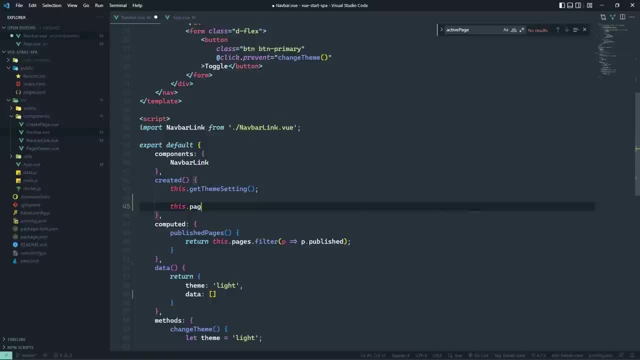 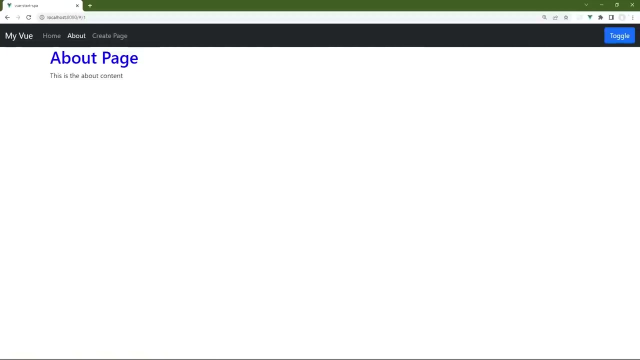 And then inside of the created hook, we will simply get our pages from our data store. So that is using the pages object. I believe the method was called getAllPages. We will find out if that is indeed the method or not. But that should be it. We can go to the browser. Let's do a hard refresh, make sure everything is loaded from scratch. The about page is currently active. We click on home, that works, about, create. 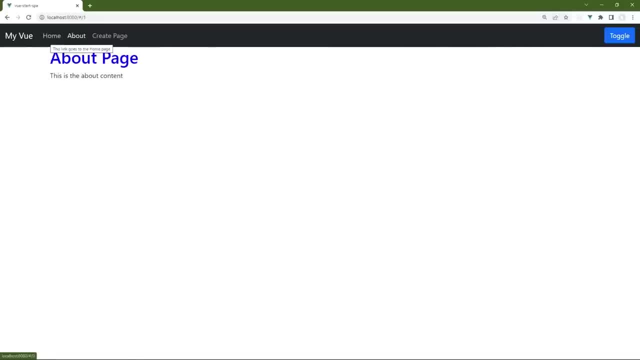 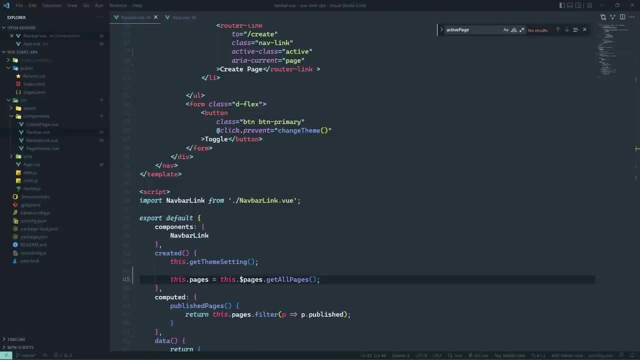 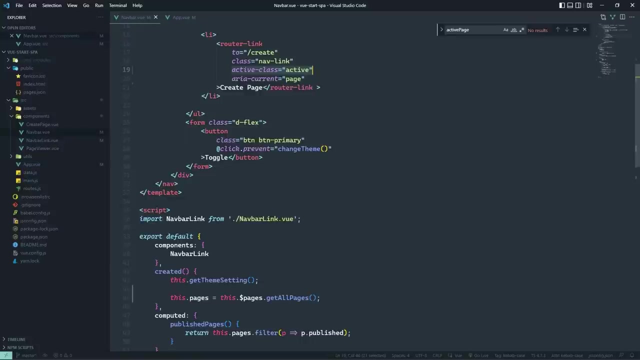 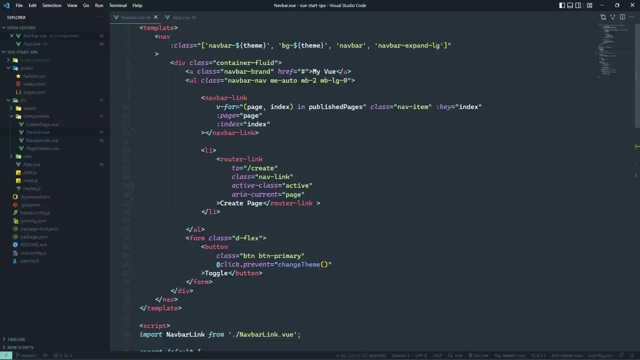 And we still have our navbar. So the pages are properly loaded, and the navbar is generated. So everything is working as it was. We were able to clean up three components by just using the active class. Which I don't know about you, but to me, that's huge. And then by changing the navbar so that it pulls in the pages, so that it can generate the appropriate links. So that we can clean up the pages. 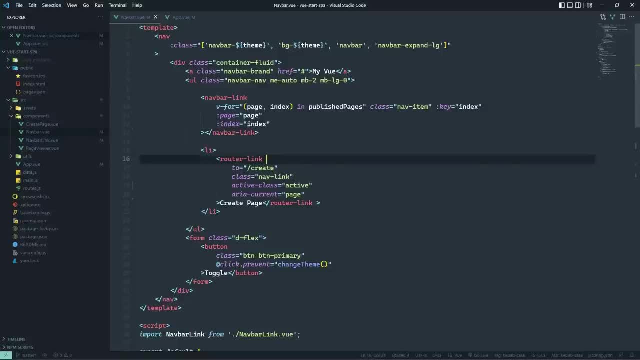 And then by cleaning up the app component, that was also a nice little side effect as well. 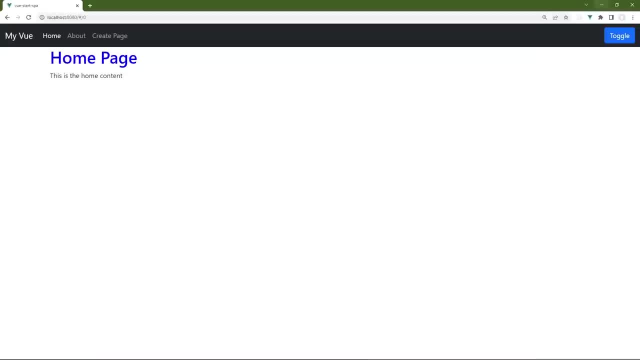 Well, in the next lesson, we are going to look at nested routes. So far, the routes that we have had are very simple. And simple is good, but in real world applications, we usually deal with more complexity. And nested routes give us the ability to handle that complexity. In this lesson, you are going to learn about nested routes, which are exactly what they sound like. They are routes that are nested. And nested routes are routes that are nested inside of other routes. 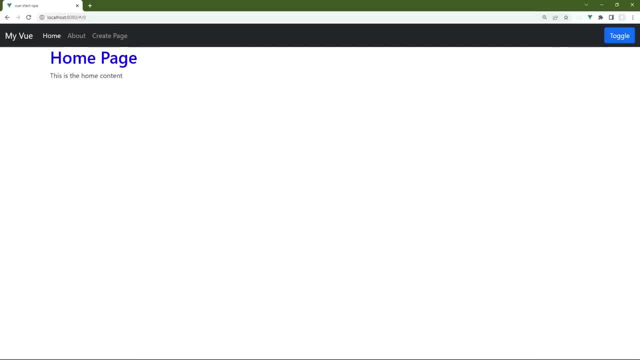 And you want to use nested routes when you want to build a UI that is structured in such a way that the components mirror the URL. 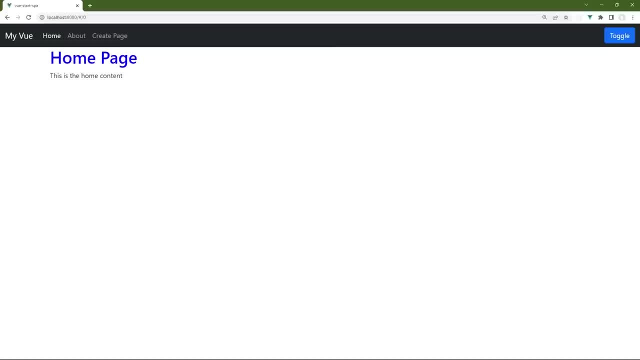 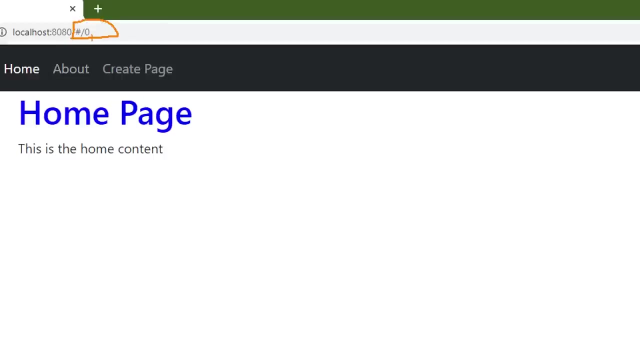 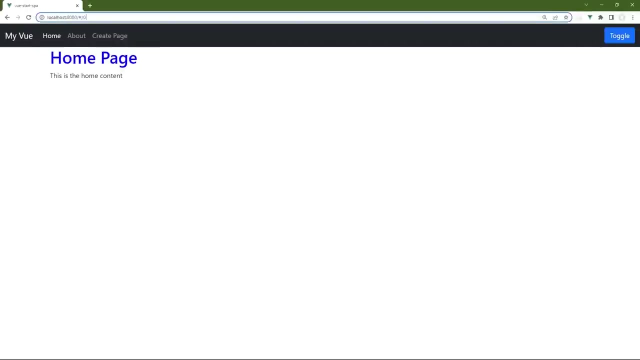 For example, let's just think in terms of typical web applications where we are working with an individual resource. In the case of our application, our resource are pages. We have a URL for displaying the content of individual pages. All we have to do is supply the index and we see the content. But let's say that we wanted a management section so that we can manage those pages. 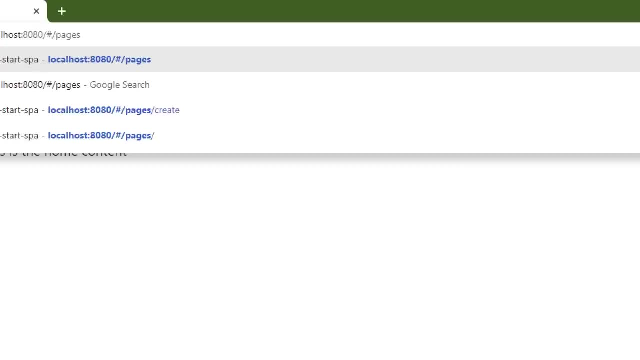 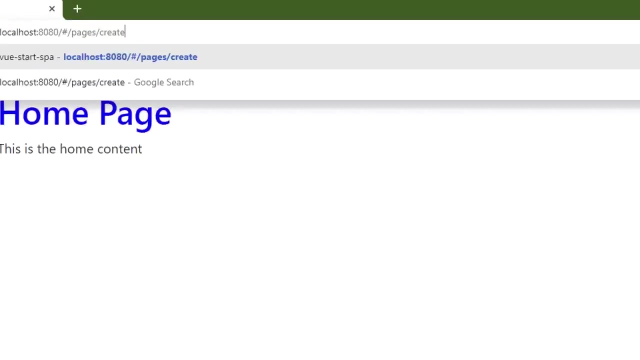 Well, within a typical web application, the URL would be slash pages. And then from there, we would have a structure representative of working with pages, so that if we wanted to create a page, then the URL would be pages slash create. 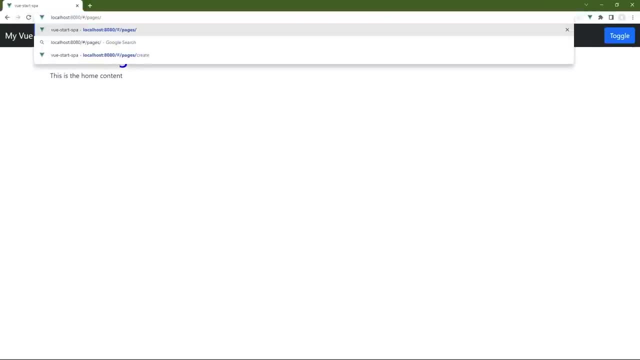 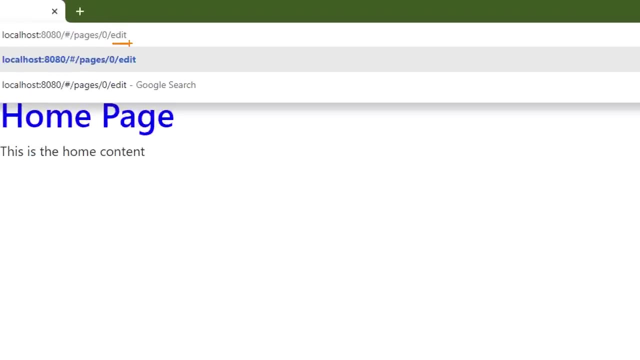 If we wanted to edit an image, we would have to create an image. If we wanted to delete an existing page, it would be pages slash the index number slash and then edit. And if we wanted to delete, it would essentially be the same thing, except that the last segment would be delete. 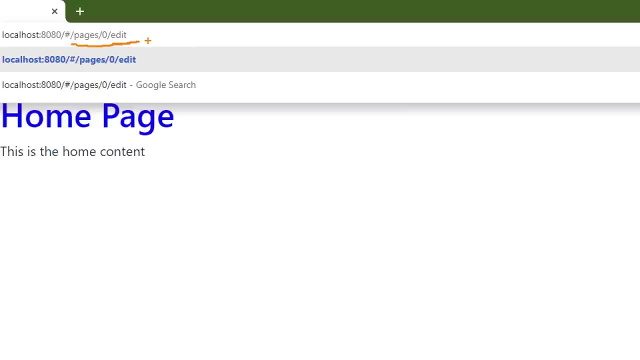 So this is a very structured URL. And we can translate these URLs into a series of routes that are nested inside of one another. 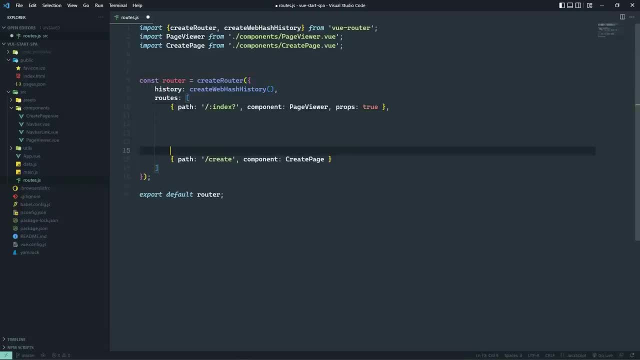 So if that's not clear, which I'm not sure it's even clear to me, the code makes it very clear. 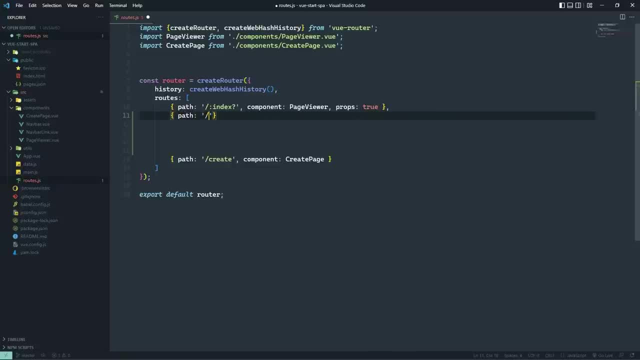 So what we are going to do is create a route with the path of slash pages. And this is going to be handled by a component that we will call just simply pages. 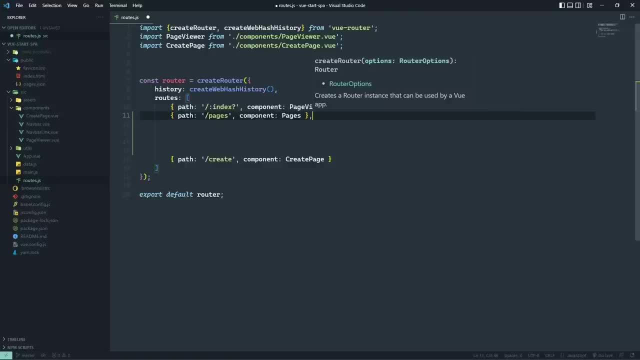 Now, if you look at other people's projects, you are probably going to see a folder called views. 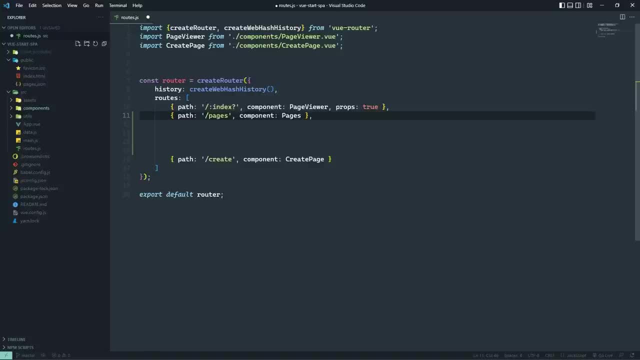 The views, or at least what are considered views, are the components that handle routes. 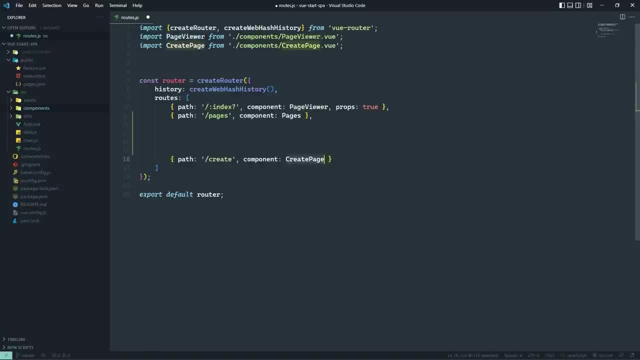 So in our case, we have the page viewer, we have the create page. Those are essentially views because they are handling routes. 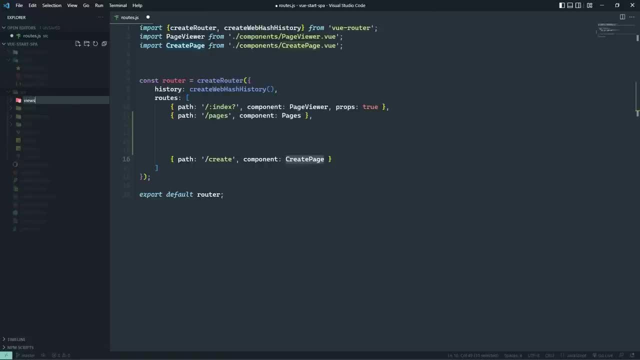 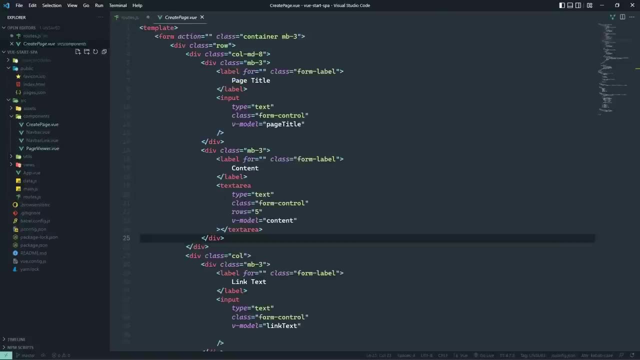 So I'm going to create a new folder called views. And I'm going to move those components into the views folder. Now, this is not necessary. This is just convention. But it's a good idea to follow convention. So I'm just going to drag and drop those. 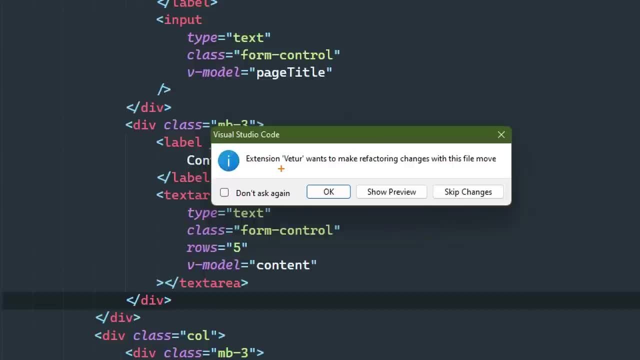 I do have a plug-in for Visual Studio Code called vTour, vTour? I don't know. I don't know how to pronounce that. 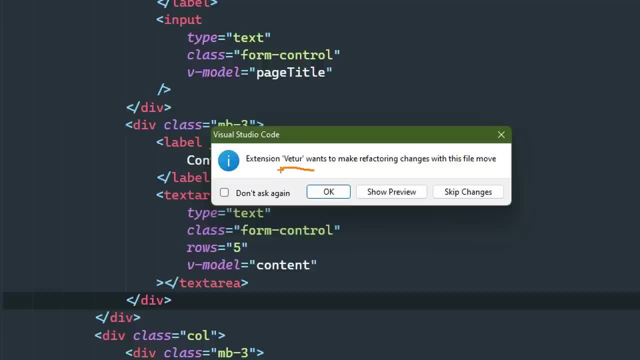 But this is a plugin. This is going to find where those files were referenced, and it's going to automatically update the paths. 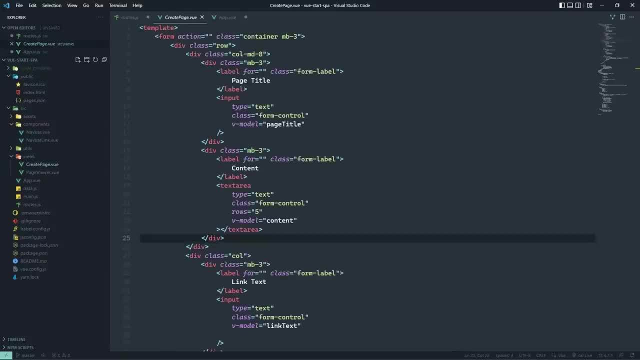 So whenever I click on OK, this is going to modify the routes file. 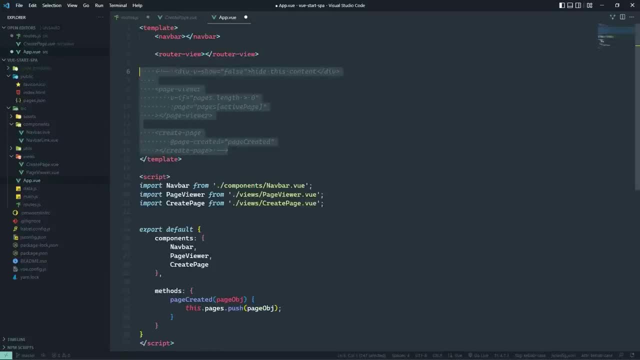 Why did it modify app? Because we still have those listed there. 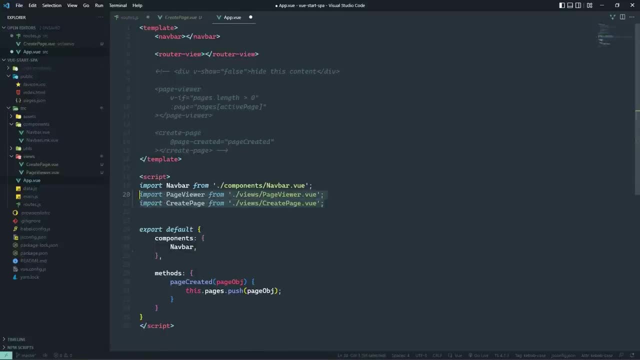 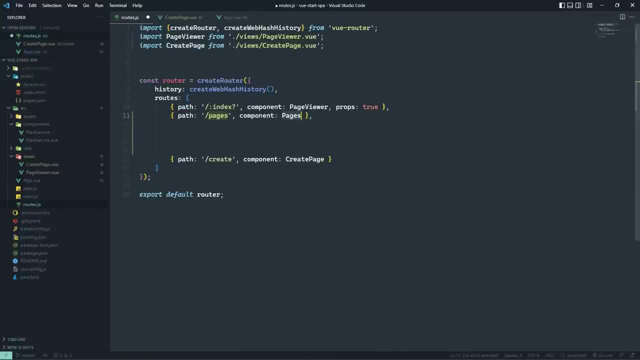 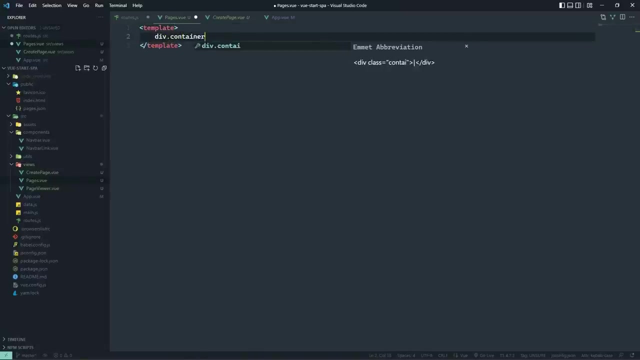 We don't need these inside of app, so we can delete those. Because now, all app is a container, basically, for the router view. Which is essentially what we are going to create, with this pages component that I have just talked about. So let's create a new file inside of the views folder. We'll call it pages.view. And the template is going to be very similar to our app component. In that, we'll have a div with a class of container. And then we're going to have a heading. 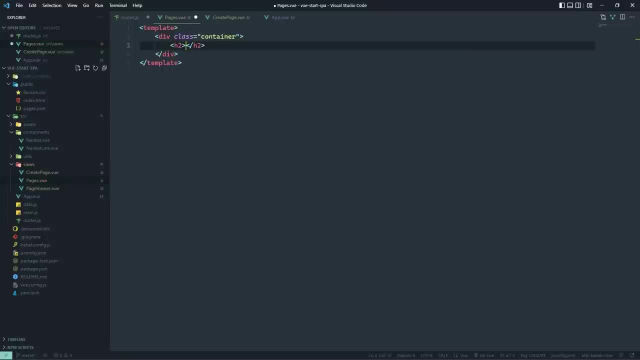 Because this is going to serve as a container for all of the nested routes. So I want this to say, hey, if you all have a computer, let's say page management, so that all of the child routes that we are going to visit are going to have this H2 element in them, so that we can see this is part of the page management. And then we will have our router view. So this pages component that we just wrote, this is going to be loaded inside of app.view. So it's going to be loaded right here, but it has its own router view. 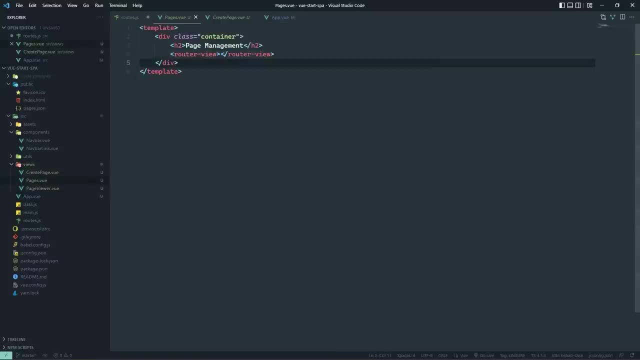 So all of the child routes are going to be rendered here. It's part of why this is called nested routes. You'll see the other reason why it's called nested routes, well, right here. 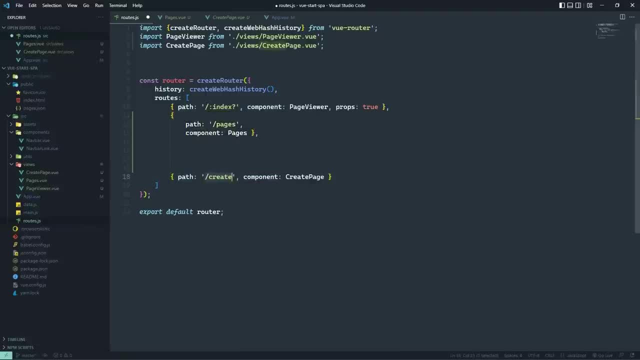 So I want to make the create route a child of our pages route. And we do that by just adding another property to this route object. It's simply called children. It's an array of other route objects. So we can just cut and paste. The path does not need the beginning slash for child route, but that is going to work. 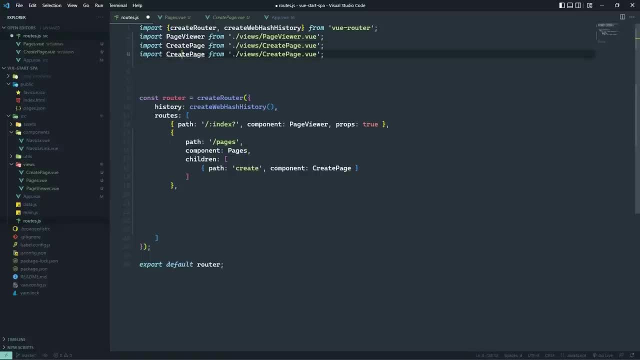 We do need to import this pages component though. So let's go ahead and let's import that. 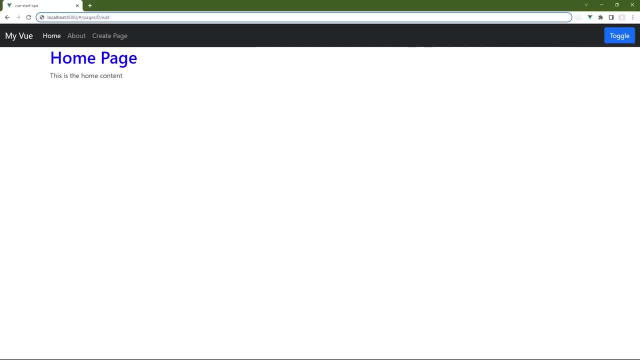 And whenever we go to the browser, let's let this refresh. Let's go to just slash pages, and we see page management. 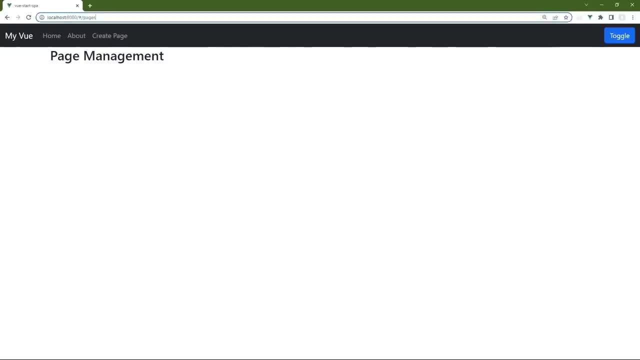 That is the pages component that we just created. If we go to pages slash pages, and 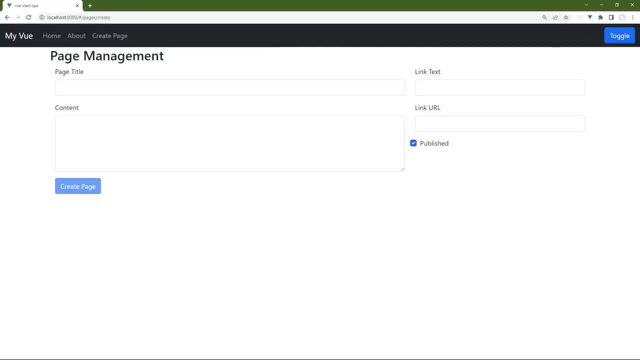 we go to create, we still see page management because that is the parent route that is essentially handling the pages part of the URL. But then we also see the form for creating a page. 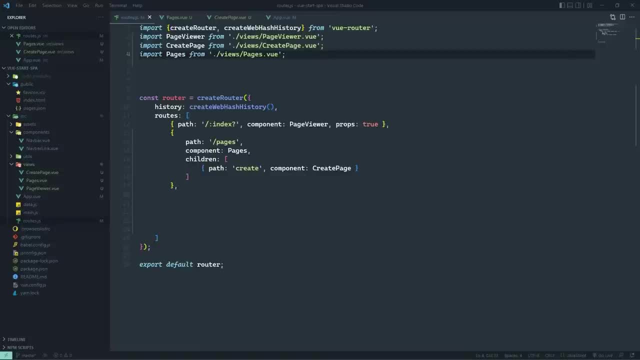 That is handled by the create part of the URL. But let's also say that if we go to just slash pages, I want to see something here. 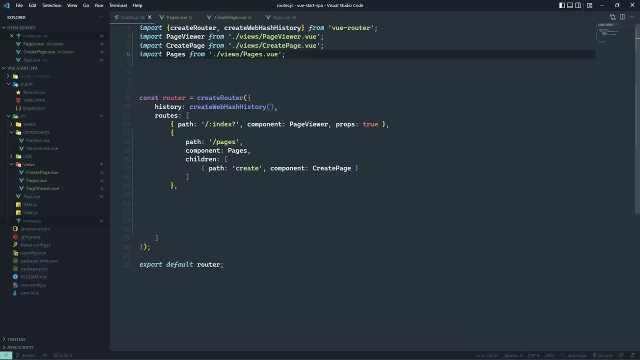 It makes sense to list all of our pages. We aren't going to actually list those just yet. 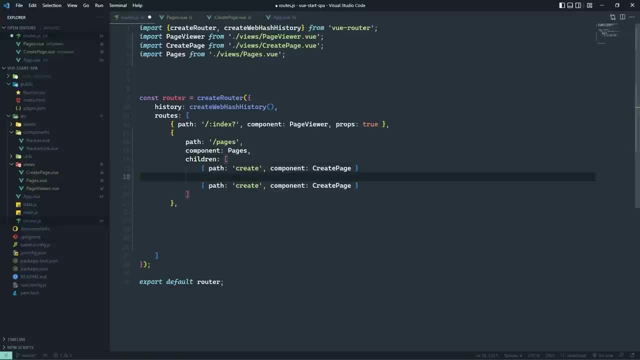 But let's go ahead and let's create the component that we can use to eventually list that. 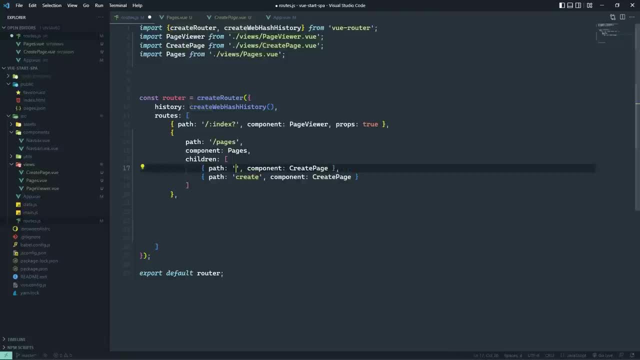 So to do this, our path is going to be just an empty string. So this will essentially be the default of the pages route. Let's call this component pages list. 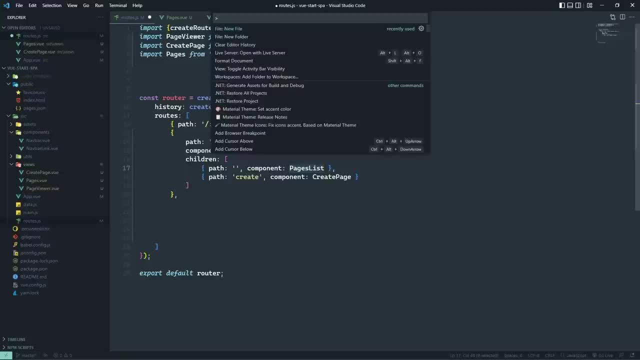 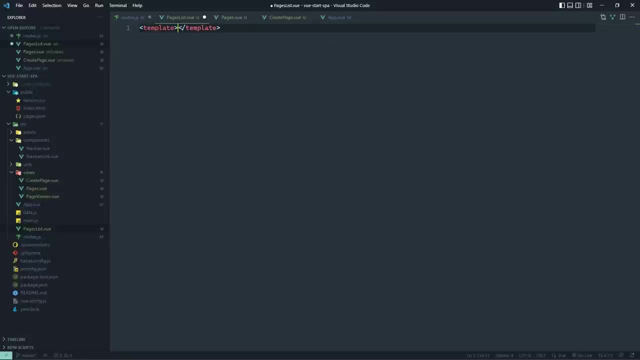 And of course, we need to create that file. And as far as its template is concerned, let's just have some content, something that we can use. We're going to use something to say that this is the list. So let's have a p element. This is the pages list. Let's move this into the views folder. And then we want to import this as well inside of routes. So we will have our pages list. 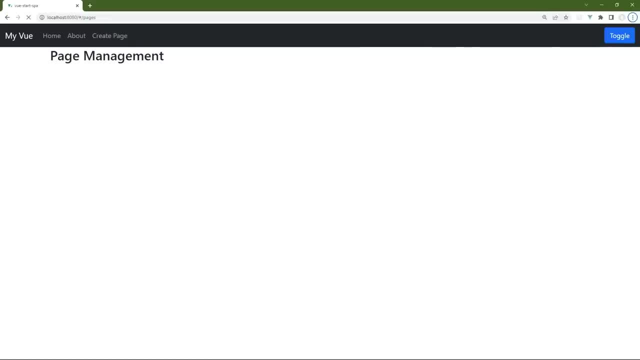 So that now whenever we go to the browser, we will see the text for this is the pages list that's going to be the default for going to pages. 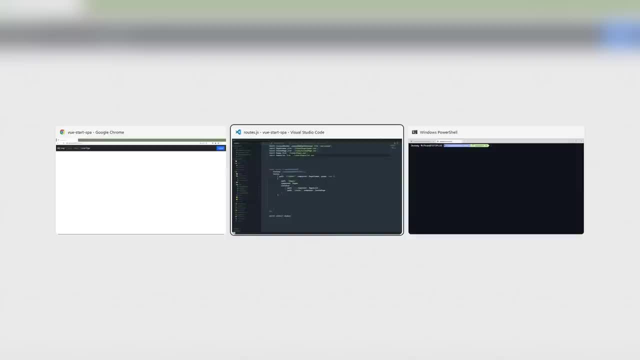 Whenever we click on create page, which, we need to update that link, don't we? 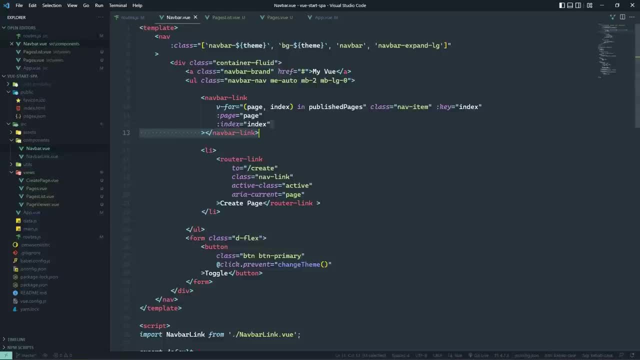 That is inside of navbar. So instead of going to just create, we need to go to pages create. 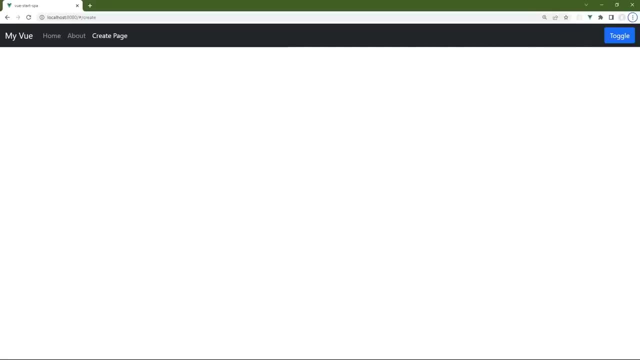 And I guess ideally, we should turn this into a menu so that we have all of the options available. So whenever we go to pages create, we see the page management. 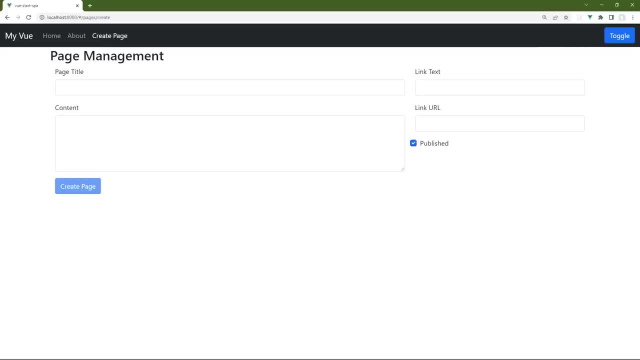 We have the form. We don't see the default text of displaying the list. But that's because we aren't at just pages. We are at pages create. 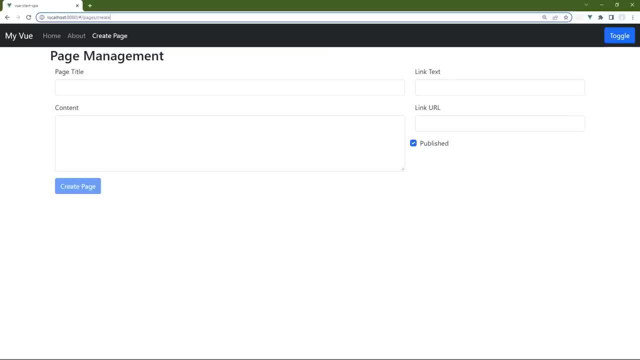 So in the next lesson, we can start to build our other components to handle those nested routes, and we will do so using the composition API. 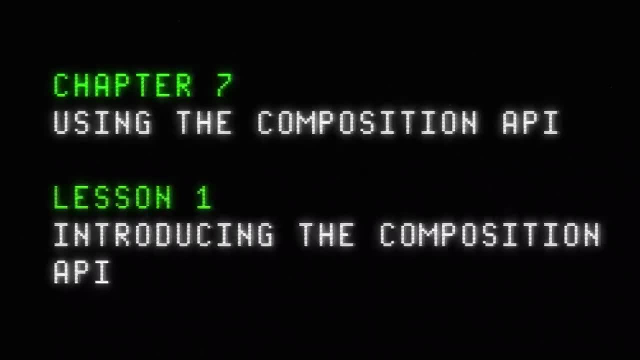 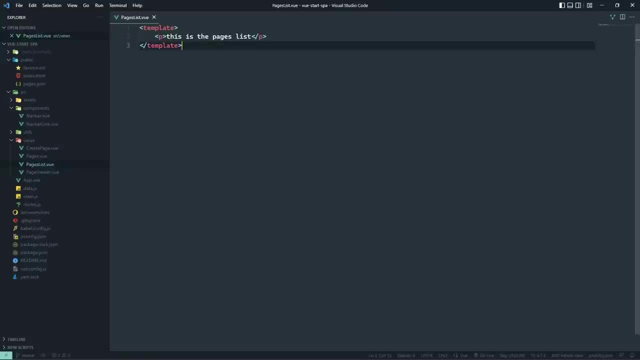 The composition API was introduced as a plugin for view two. And starting with view three, it is baked into the framework. And we have the composition API because of react function components. 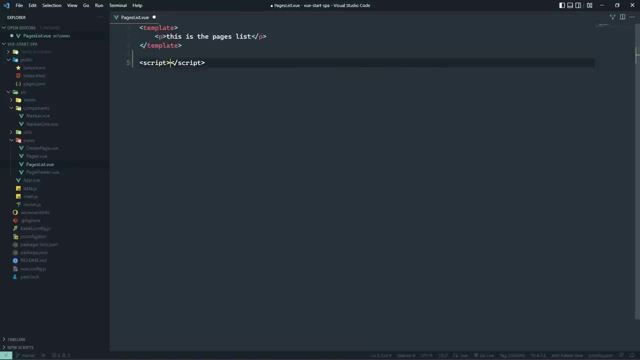 In fact, if you look at the documentation for the composition API, it's very clear. It says, this was inspired by react. And I feel like I need to give you just a little bit of background on react components because it gives you an idea of why the composition API exists and why you would want to use it. 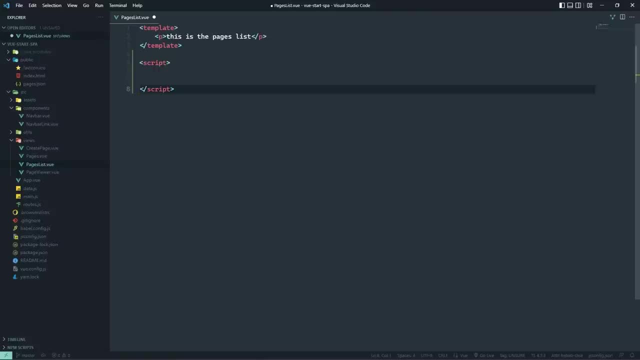 So in react, you can create a component in two ways. You could write a class or you can write a function. Although originally, the only way that you could go about it was with a class. And it would, of course, have all of the functionality that you would need within a component. It would have. 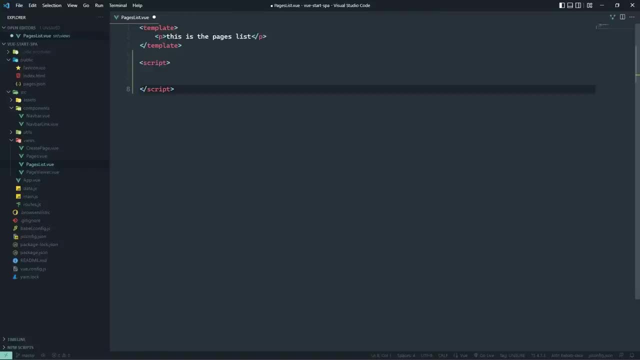 You could have states, you could have methods, and it could be very complex. But then they created function components. And originally, function components were just very simple. You essentially fed them data, and then they would output that data. They might manipulate it, but the manipulation was only for the output. There was no state, there was nothing, they were just very, very simple. Well, people liked using the function components. So they wanted to essentially do the same things that a class could do. 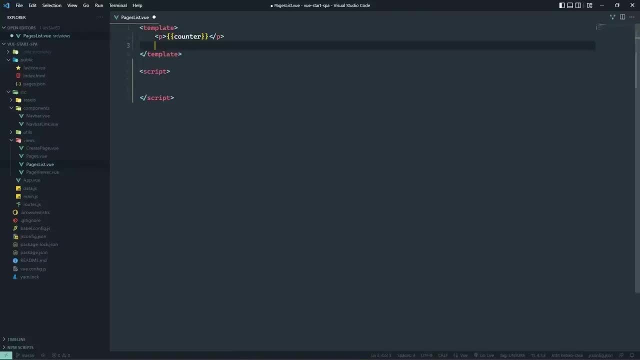 So in order to facilitate that functionality, they created what they call hooks. They are just basically functions that you import, and you would use the hooks that you needed within that component. So if you needed state, then you would import a function to use that state. If you needed some other functionality that was provided inside of a class, there was a hook for that. 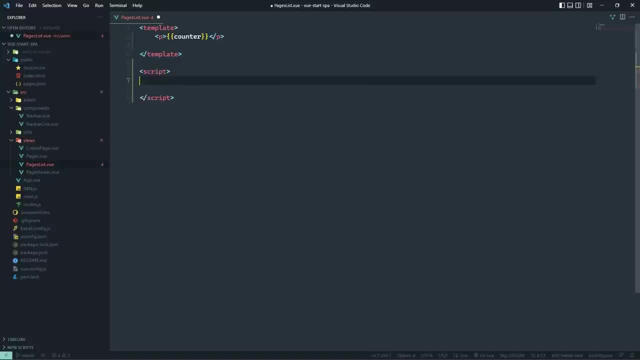 So you just imported that function and used it, and then there you go. So the composition API in view, was based upon that idea, except that they did a much better job of it. 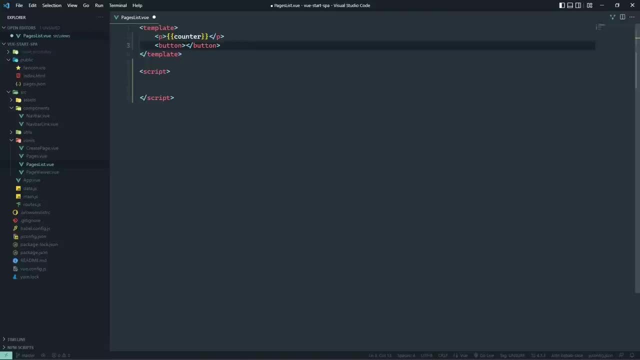 Not only are they easier to write, at least in my opinion, but they also perform better. 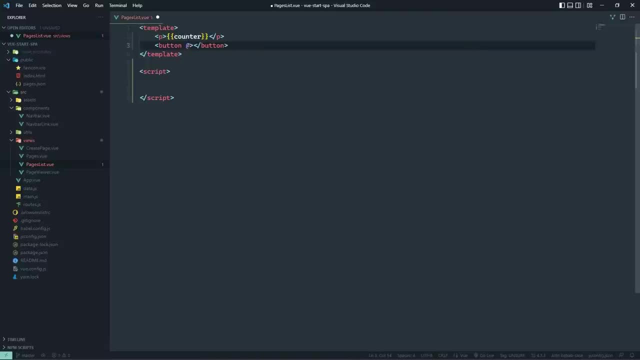 Because there are some performance issues with function components in React. And View's composition API is also much easier to understand and follow than React's functional components. 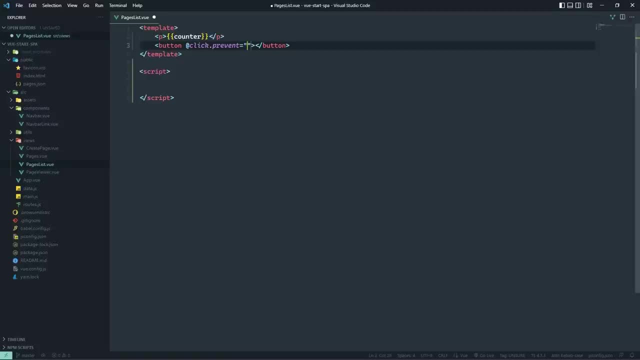 There are just some things that you have to think differently in order to use those features. 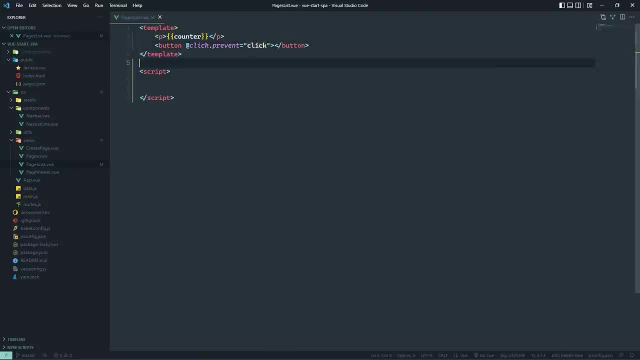 And with View's composition API, you pretty much don't. So what we're going to do is look at the differences between the options API, which is what we've been using thus far, where we export a default object. 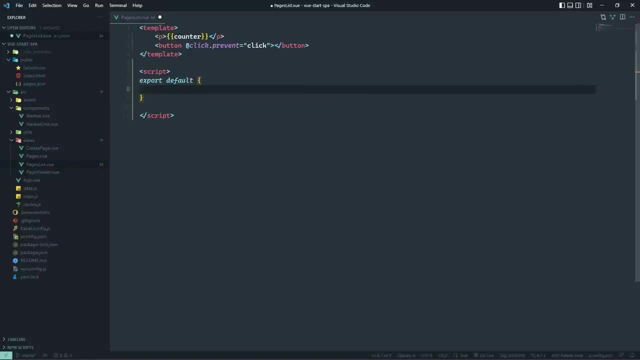 And then we will do the same component, but with the composition API. So this is, of course, the pages list component, but we're gonna use it for 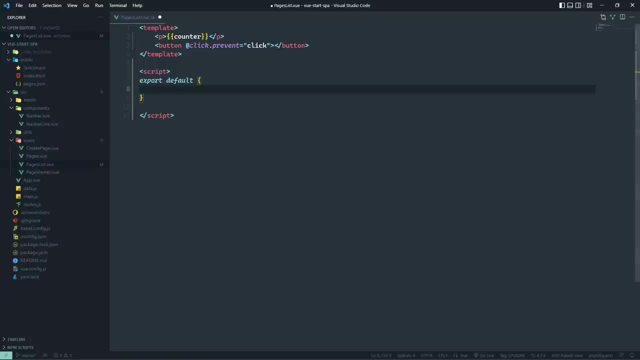 this example, and then we are going to actually, well, list our pages. So this is just gonna help you out, but we're gonna have a simple counter. We'll click on a button that we'll call the click method, and it will update the counter. 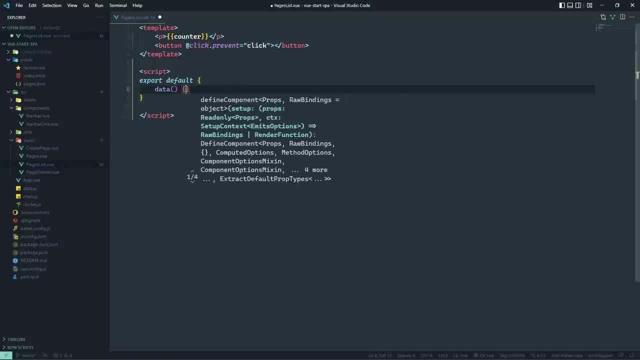 So for the options API, we would need the data, which we have to define as a function, which returns an object that then has the data that we want to work with. 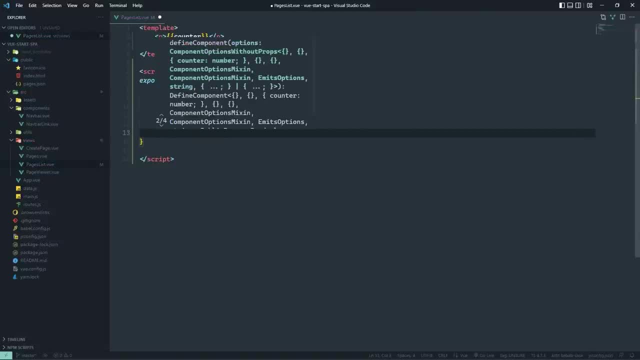 So counter, we will initialize as 0. But then we have that click method. Now, we could simplify this to where right here we just increment counter, and that's fine. 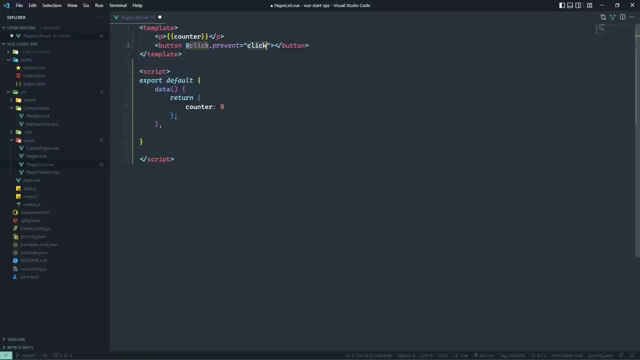 I want to do this to where we say that we have this click, and we would need to define that as a method. But to do that, we have to, first of all, have the methods option. Then we would define click, and then we can update our counter whenever we click on it. 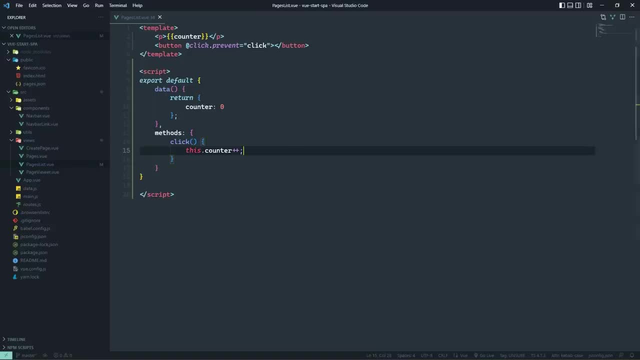 So whenever we go to the browser, we are going to see, well, let's add some text for the button so that we can actually click on it. 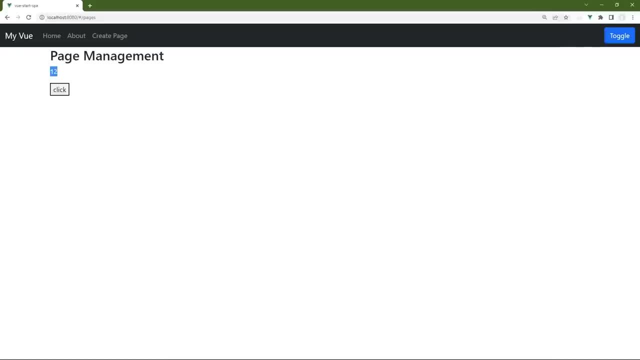 And whenever we click, we see that the value changes. There's nothing out of the ordinary here, but there is a lot of boilerplate, right? 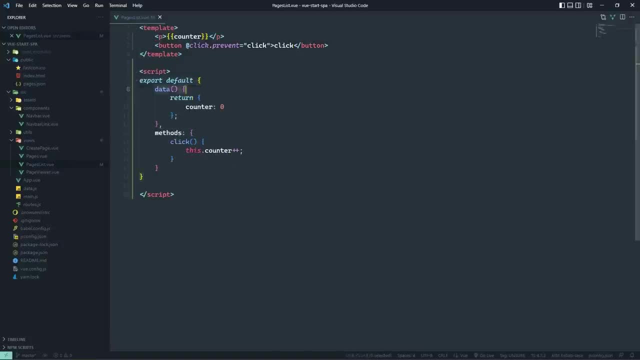 There's a lot of boilerplate involved. We have to export an object. We have to define the data method that returns an object. We have to use the methods option if we have any methods. 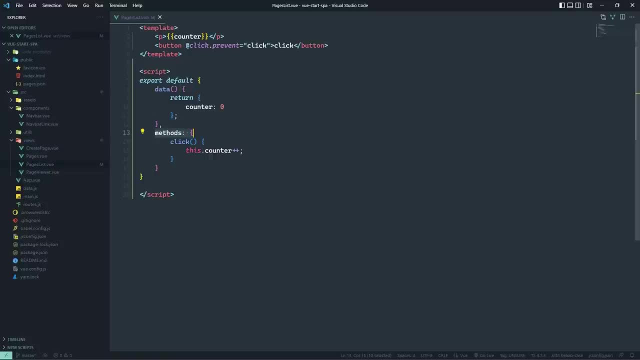 The same is true for computed values and watchers. And by organizing our code into these different little sections, the overall functionality and flow and logic is kind of disjointed. Because our data is up here, our methods are down here. 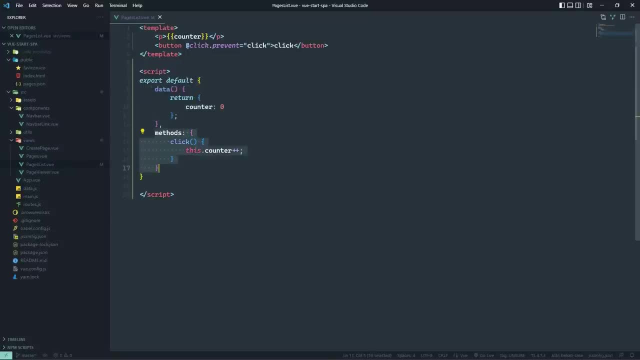 And it's not that bad with this particular component, because it's very simple. But in a very large component, you're jumping all over the place in order to change the data. Okay, I need to go to the method now and change this. 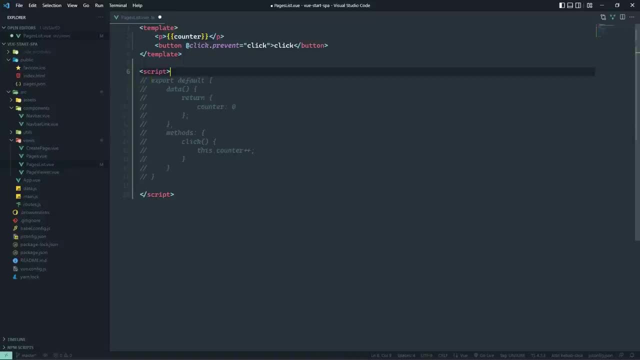 Okay, now I need to go to the computed. It could be a lot better. 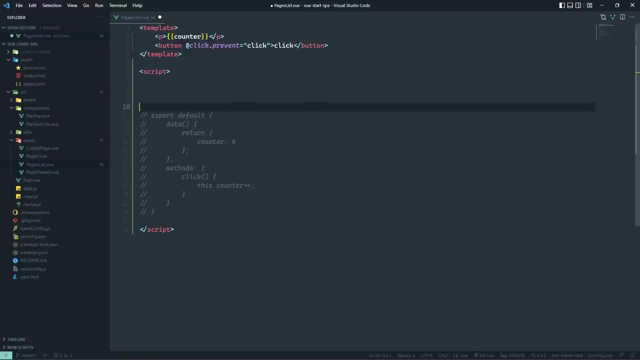 And that's what the Composition API aims to achieve, to give us the ability to organize our code logically. So to use the Composition API, we need to add the setup attribute to our script element. And the reason is, 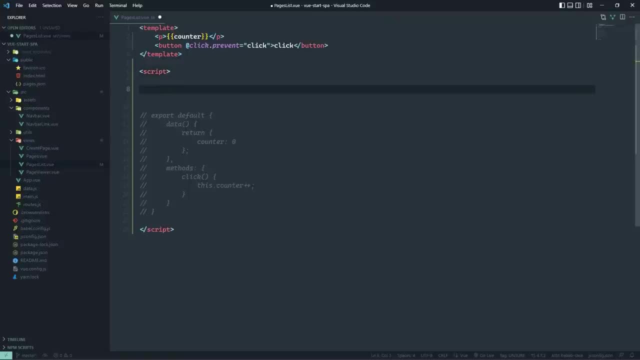 and the reason why is because in the version two, we would have to define a function called setup, which was used for setting up the code for our component. 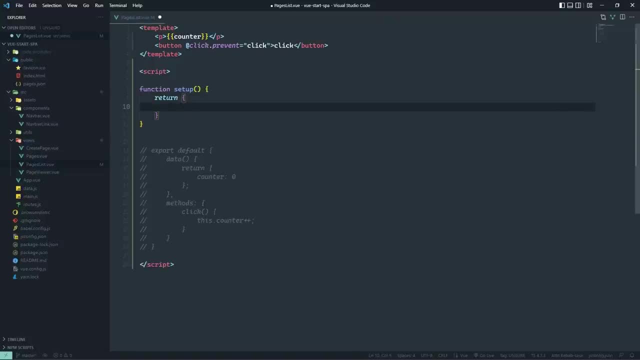 And this would also need to return an object that contains the things that we would need to use inside of our template. 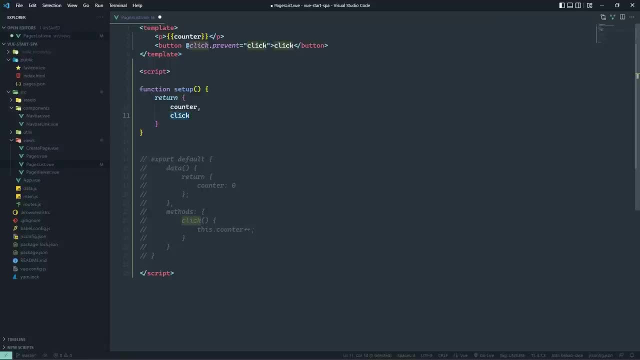 So if we wanted to use counter and click, we would have to return those in an object. Wasn't that difficult, but it was more boilerplate that we had. 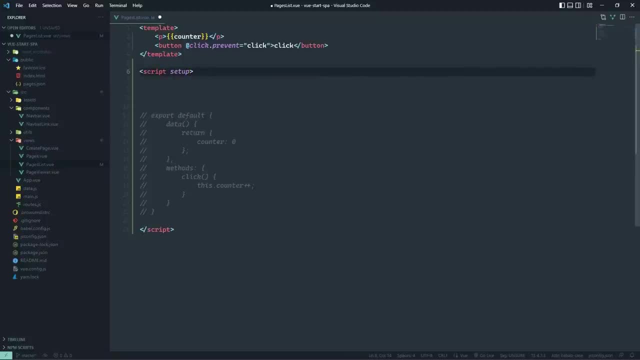 But now we just have to use the setup attribute on the script. And then we're good to go. 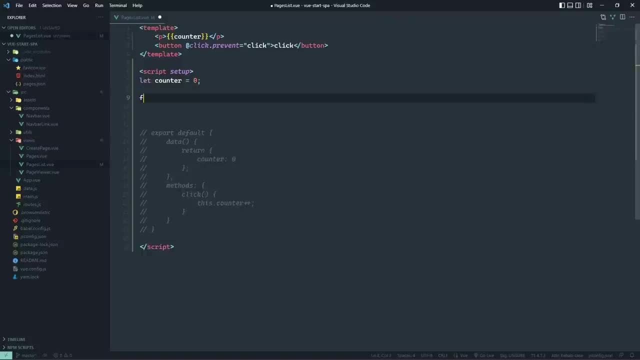 So let's start by creating a counter variable. And then we will just define a function called click, to where we will increment the counter. 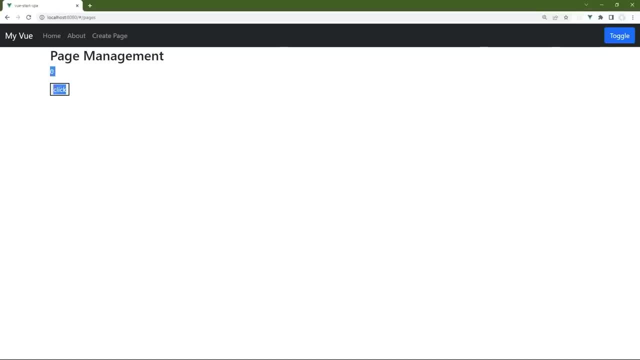 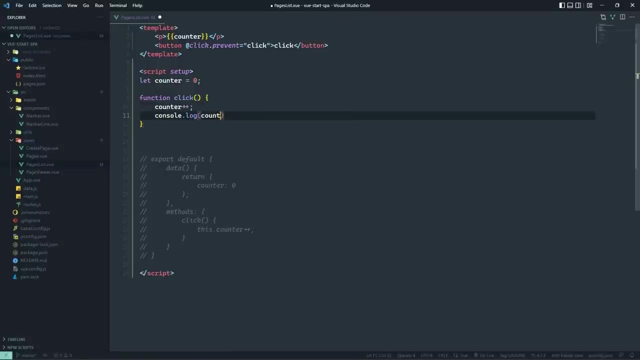 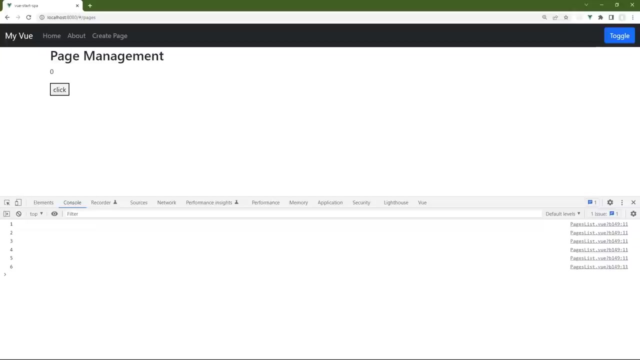 And whenever we view this in the browser, it's going to look like it's going to work. We see the value of zero, we have our button. But whenever we click, nothing happens. Well, behind the scenes, the value of counter is changing. In fact, we could write the counter and, and then we could change our value. we could write that out to the console, and we could see that being updated. But it's not going to be updated within the browser because we are using just a simple variable. It's not reactive. 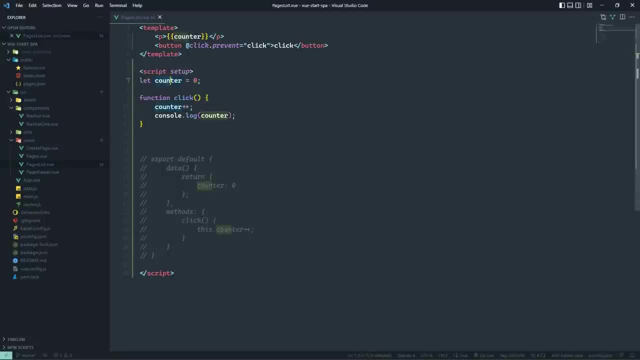 So behind the scenes, Vue doesn't really know that this value is changing. It's not going to update the component in the browser. So instead, what we need to do is tell Vue that this value is reactive. And we can do that in one of two ways. We are going to use a hook. So we have two that we can use. One is called ref, the other is called reactive. You can use one or the other, but there are some things that you need to be aware of. First, we'll talk about ref. 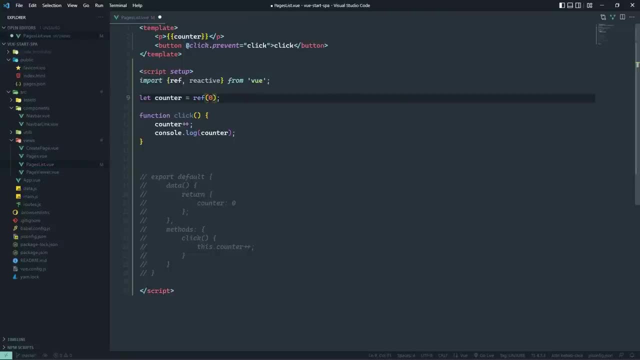 Ref allows us to create a reactive value. That value can be a primitive value like a number or a string or a Boolean value. Or it can be an object or an array or anything. But we're going to use just a simple numeric value. Now, whenever you do this, we have initialized our reactive variable, counter, with a value of zero. We can also do this because behind the scenes, what we actually end up with is an object that has a value property, and it's going to be initialized with zero. 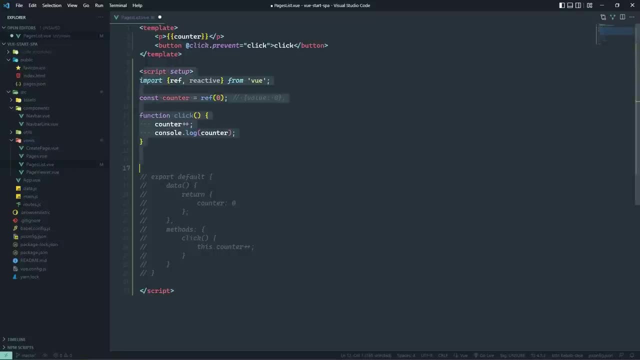 So this means that inside of our code or inside of our script, we have to use the value property any time that we need to update that value. So in the click function, we would use counter.value, and we would increment that. 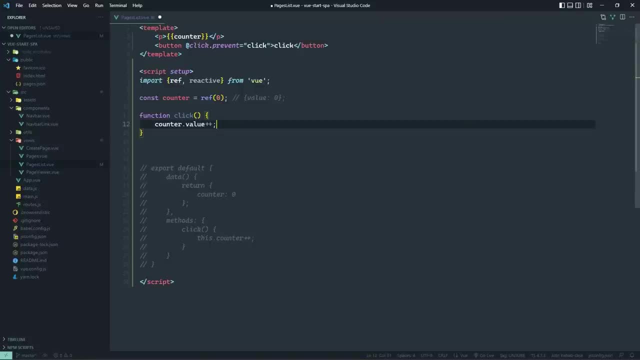 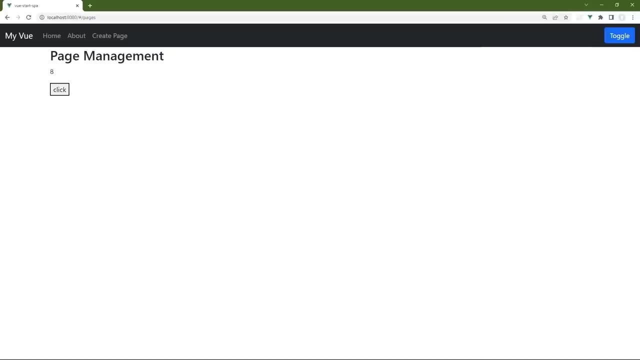 But inside of our template, we don't have to use that value. It's automatically implied. So with that simple change, we can go back to the browser, and whenever we click, we can see that it does indeed increment. So that's one way. 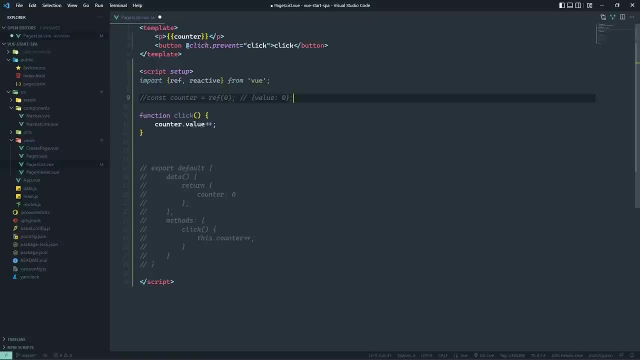 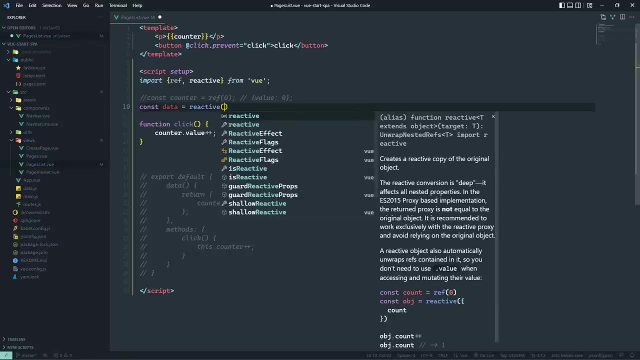 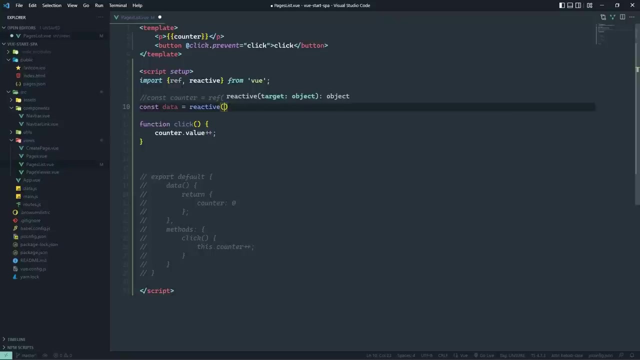 The other way is to use the reactive hook. I'm gonna create another variable, and I'm gonna call it data. And the reason is because whenever you use the reactive hook, you use reactive. This is not for primitive values. So you can't use a numeric value, a string, Boolean, anything that's primitive. It is for anything that is based off of object. So it can be an object, an array, even a function. Anything that is considered an object, you can use reactive for. 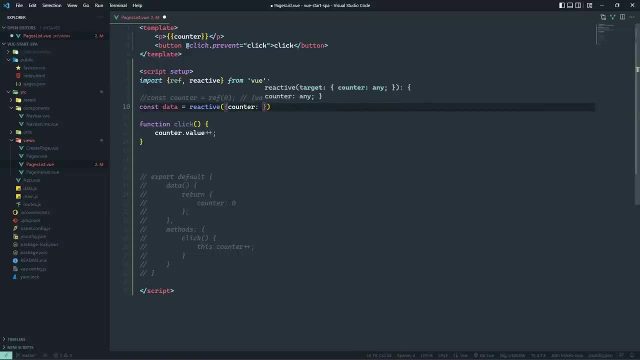 So this is very similar to the concept of data, at least in my opinion. So in my code, what I would use is just simply the name data. So that I could define the properties that I would need for my data, which in this case is going to be counter. This changes our code though, so that inside of click, we would need to use our data counter and then increment that. And then inside of our template, we would need to prepend counter with data. But other than that, everything else is going to work just fine. And of course, we could simplify this just like with the options that we have, and we could use the options API. 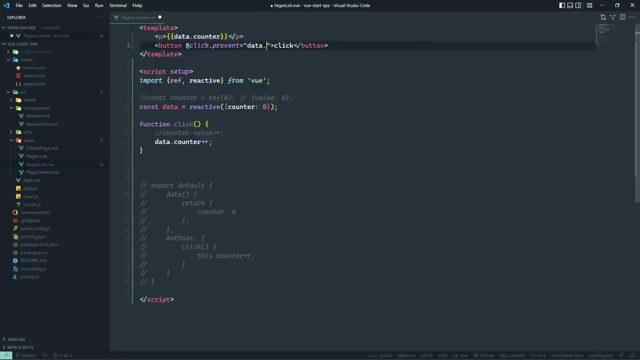 So that instead of defining this click function, we could say data counter, and we could increment, and we would see the same functionality. And the same is true for using ref if we wanted to go that route as well. So this is the primary difference between the options API and the composition API. 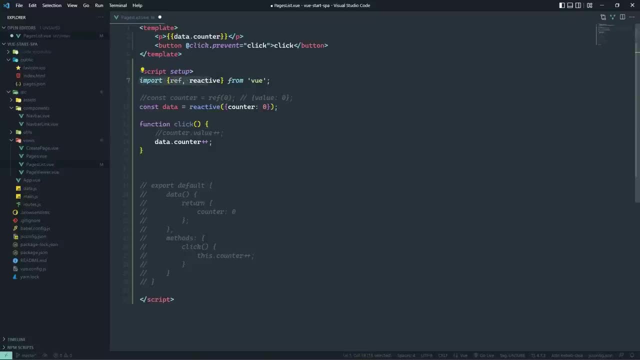 There is a little bit of boiler plate because we do have to import the functions that we need to use. 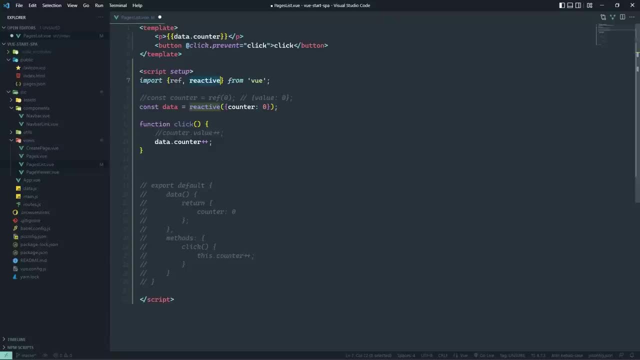 Of course, we will talk about the other functions such as setting up a watcher, setting up computed values, even using a life cycle event. 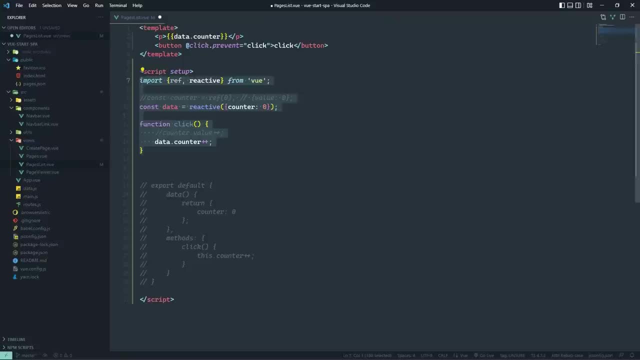 But it makes our code much more logical, makes it easier to read and understand what's going on behind the scenes. And it can be much more concise as well. 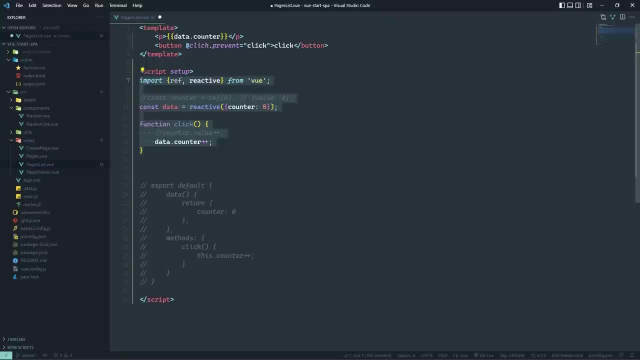 So in the next lesson, we will start to implement the pages list. 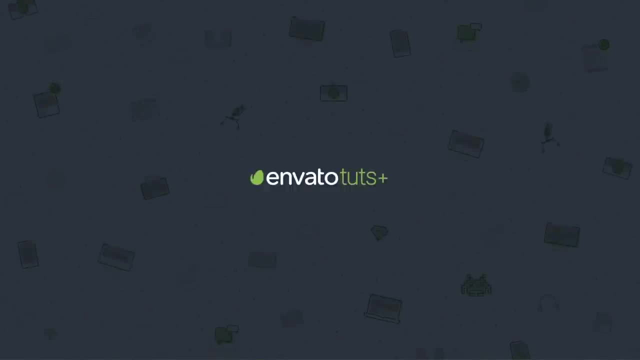 In the previous lesson, I introduced you to the composition API, which is a very useful tool. 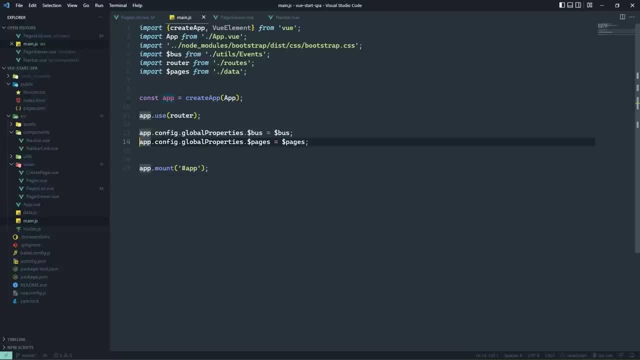 It's a different way of writing components. It takes a more functional approach as opposed to the object-oriented approach of the options API. 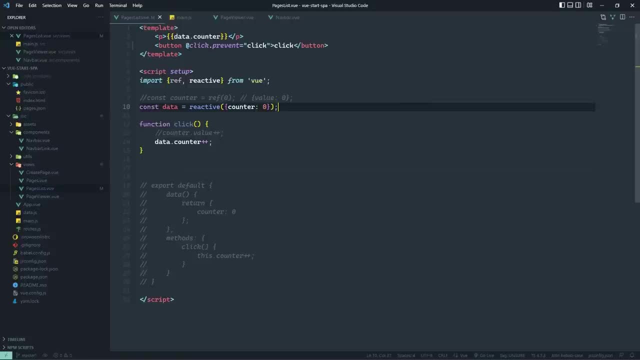 Now we have the pages list component, and we want to display our list of pages so that one, we can see that list, and two, so that we can navigate to a dedicated edit page for each one of those pages. 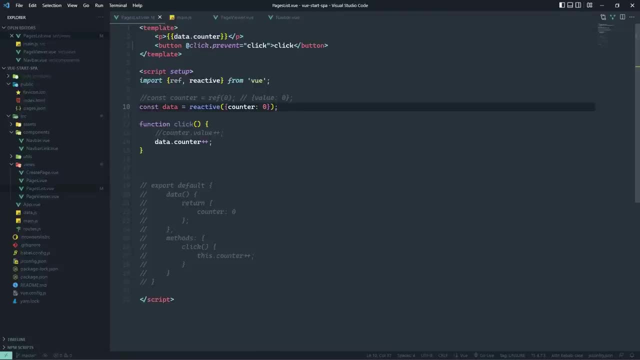 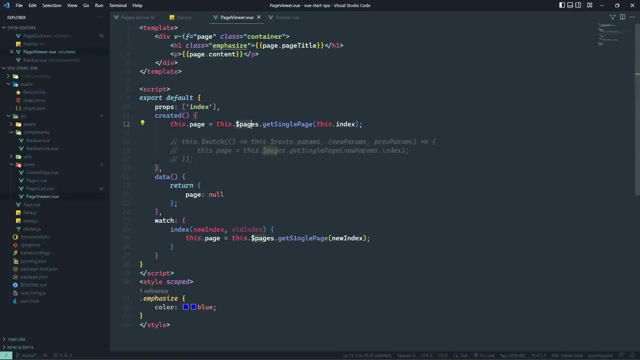 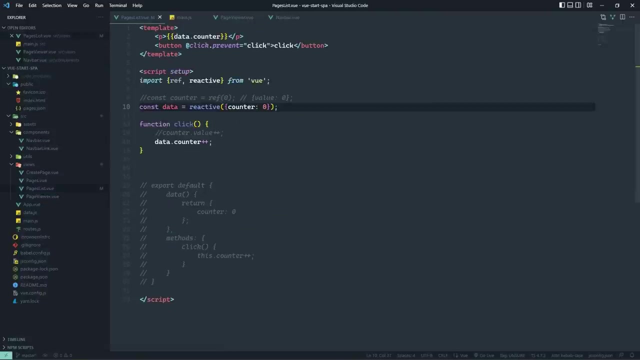 So we need our list of pages here, and the question becomes how do we get that data? Because currently, our pages are provided as a global, global property, it is available to the components using the options API. We use this dot and then dollar sign pages. We did that in both the page viewer and the nav bar. But inside of our pages list, which uses the composition API, we don't have access to this, or at least this doesn't refer to this component. 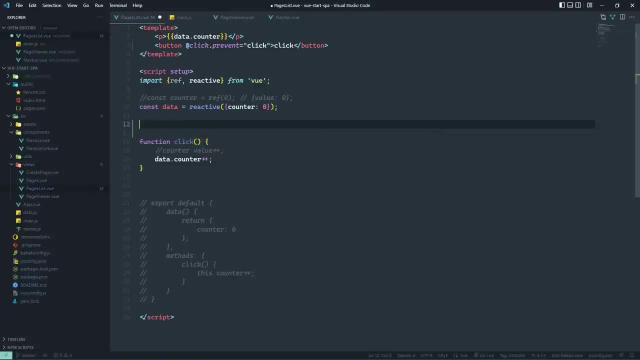 So we can't access pages in that way. 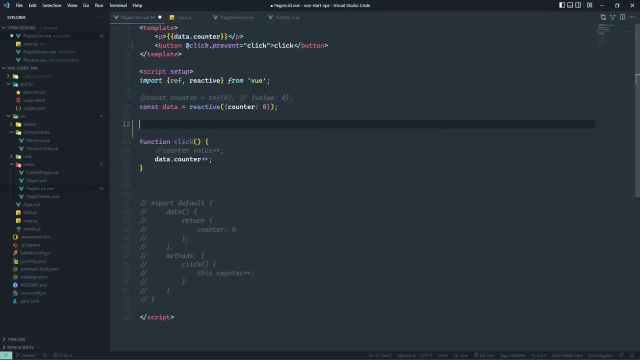 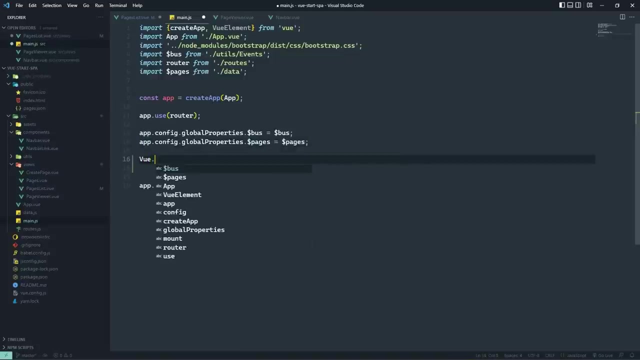 Now we can import some functions. And we can get to our global properties, but it's not very straightforward. And in fact, using global properties really isn't the best way of providing information to components that are deeper in the application. Because this is really just an escape hatch. This was to provide the same kind of functionality that was available in Vue 2. In Vue 2, we were able to add global properties by just adding them to Vue's prototype. 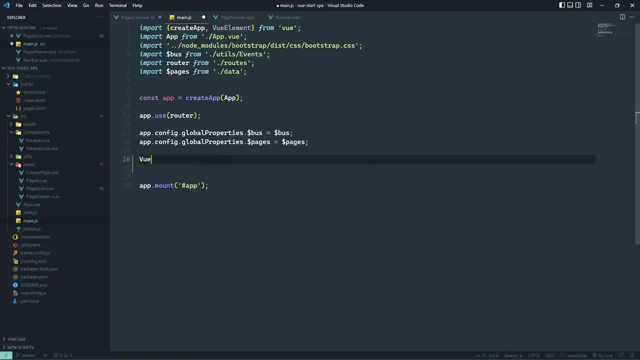 But with Vue 3, that was taken away and the global properties were then provided to replicate that functionality. 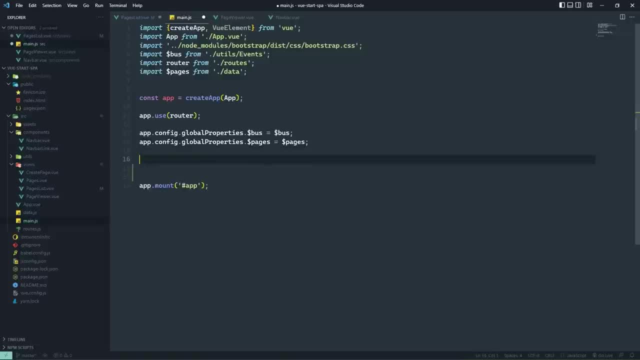 But there's a better option. We can provide information that we can then inject into child components. Now, let me first of all say, the primary way that we get data from a parent to a direct child is through props. There is no better solution there. 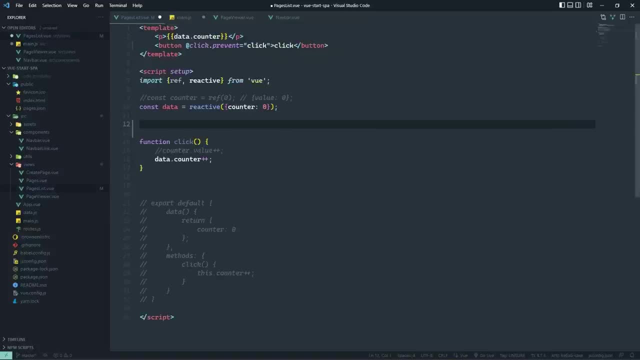 Unfortunately for us, pages list really isn't a child. 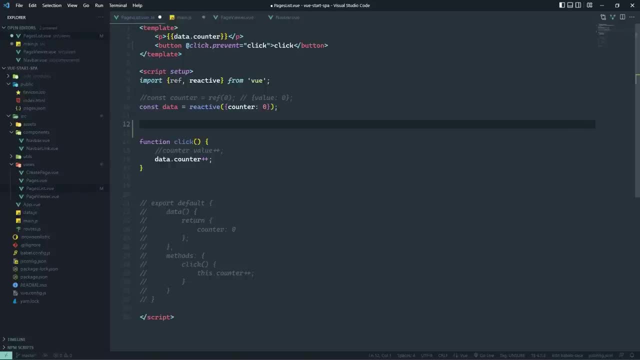 It is a view that we can use. There is a view that is going to be displayed by navigating through the router. 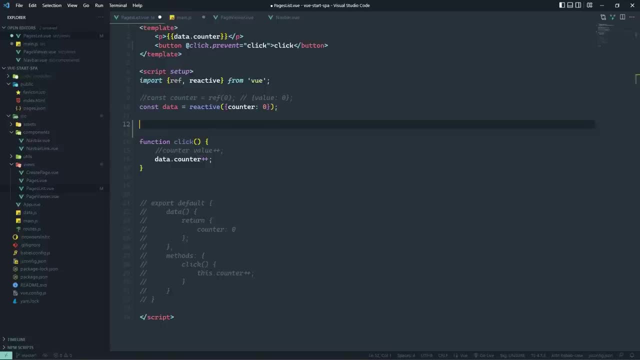 So we can't really pass props here, but instead, we can provide our pages object. So I'm going to comment out this line because we don't really need that site after we do this. 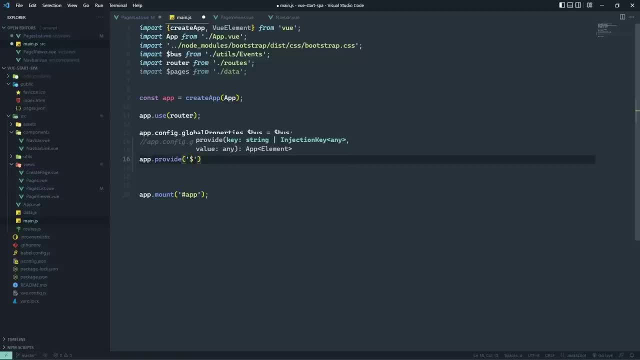 We will use our app object, we will call provide and this accepts two arguments. The first is the key that we need to refer to our pages, which I'm just going to continue using dollar sign pages. 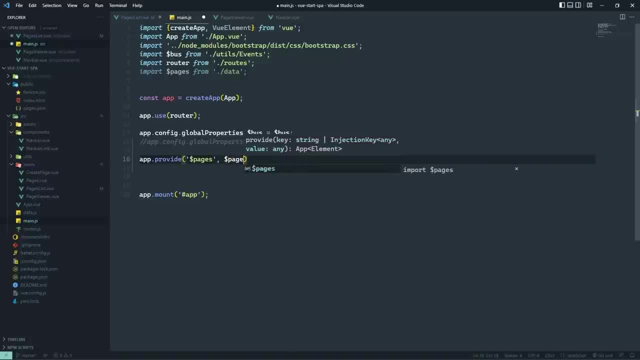 Yes. And then, yes. the value associated with that key, which is dollar sign pages. 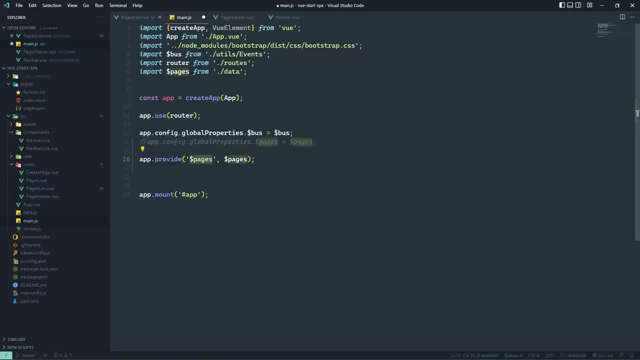 And this is essentially going to provide our pages to the app component and all of its children. 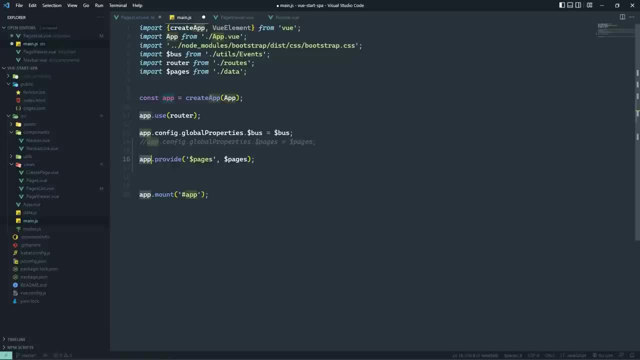 So for all intents and purposes, this is providing a globally accessible object that we can access from any component. 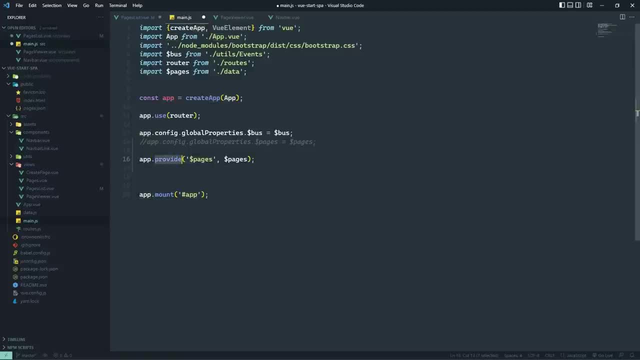 But we can provide anything from any component, and it will be available to all of its children. 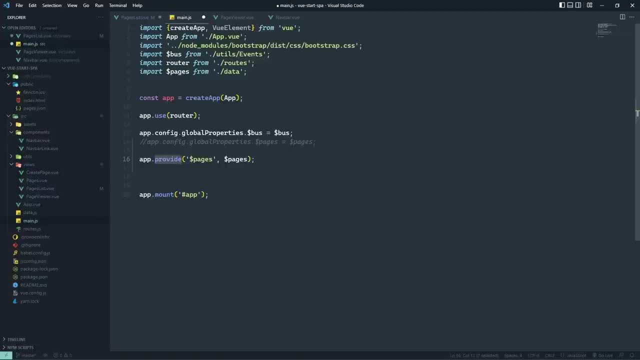 It can be a direct child, or it can be one that is farther down the hierarchy. 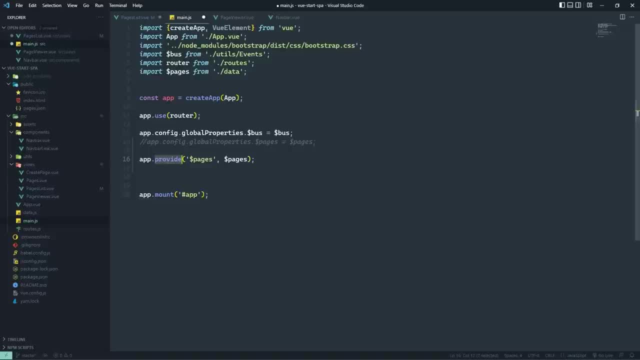 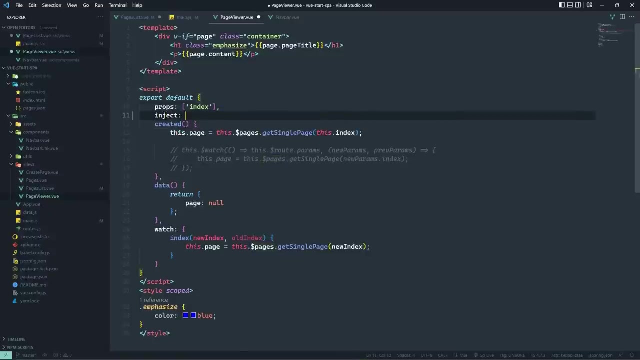 So this isn't an automatic thing. What we have to do is go into the components that need access to this, and we need to inject our pages. So the first one is inside of our page viewer. We will use an option called inject, and then we simply provide the keys that we want to inject here. That's going to be dollar sign pages. The rest of our code, it is going to work just fine because this becomes a property on this inside of the component. 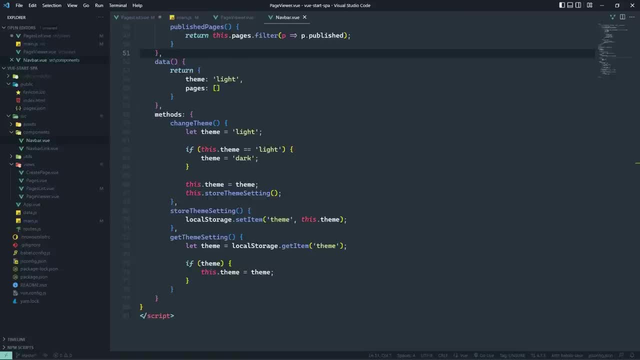 We will do the same thing inside of navbar, and then we can do a sanity check and make sure that everything is working as it should. 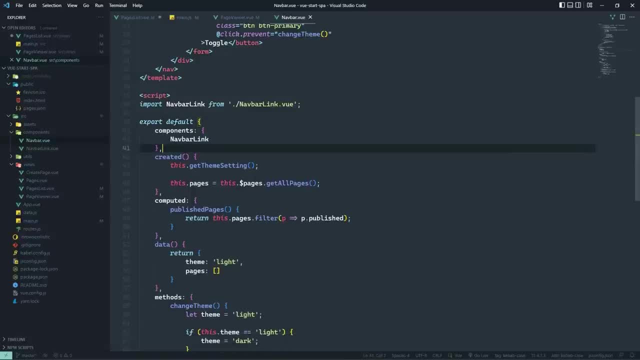 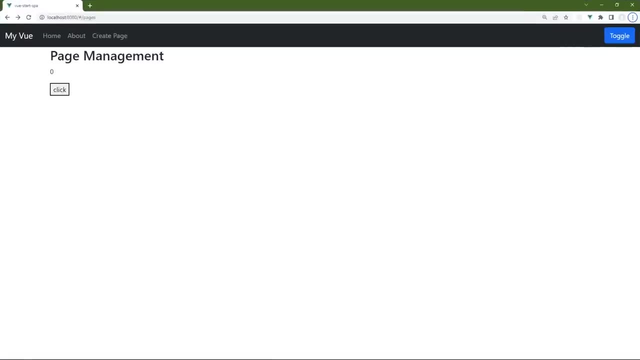 So let's add that inject. I'm gonna do it higher up in the object definition, because to me that's kind of important. And whenever we view this in the browser, everything should still work. 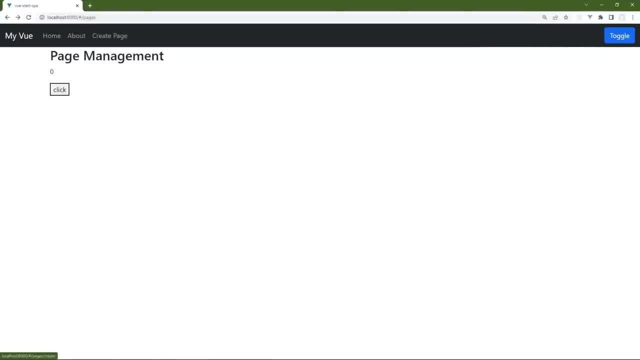 Let's do a refresh, and our navbar, and then we're going to go back, and we're gonna go to our page viewer. 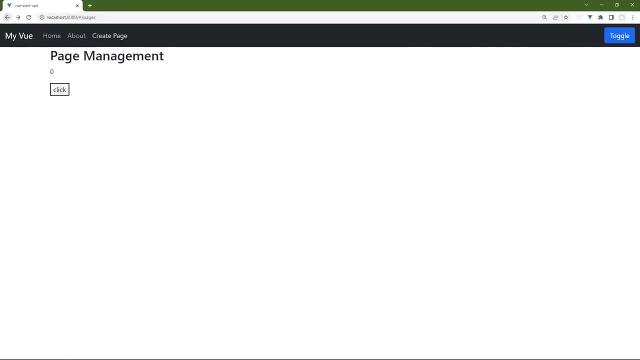 So now we can see that our page is displayed. We can go to about home and create page, everything works there. Let's get back to our pages view. 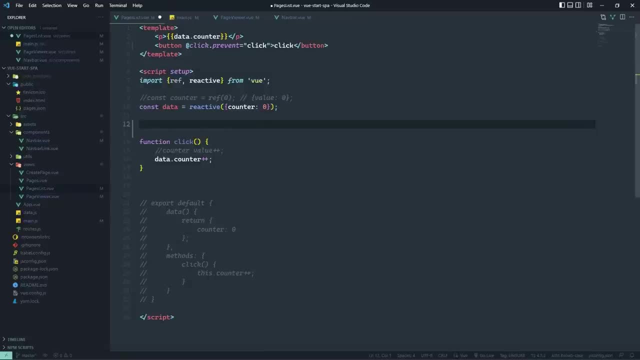 So now we want to be able to get this dollar sign pages, and we do that by first of all, importing the inject function. And then we will get access to our pages by calling inject, and then passing in the key that we want to access, in this case, dollar sign pages. 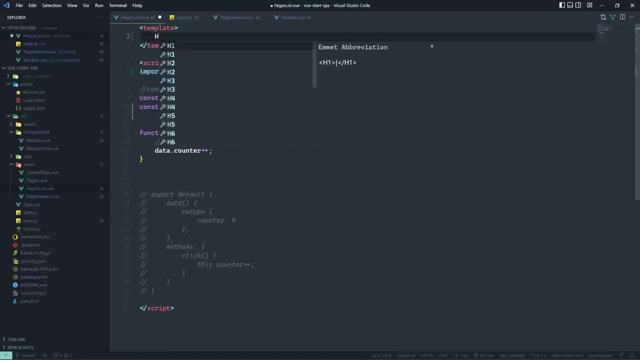 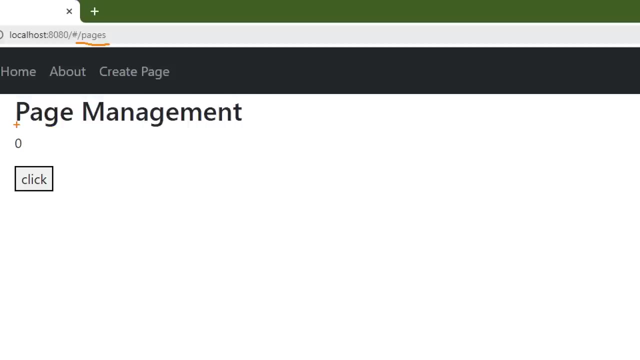 And that's to generate our list. So let's have a subtitle here, because all of our pages inside of the pages child routes are going to have this page management. So I want a subtitle. 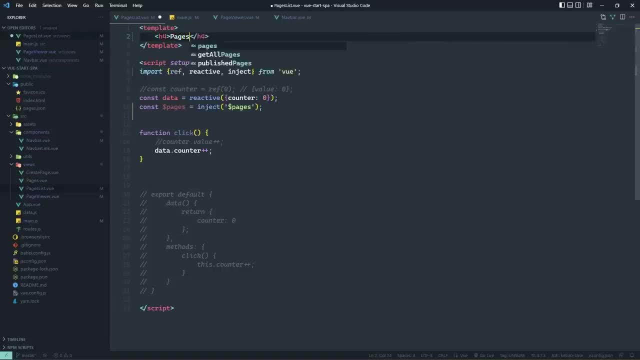 Let's use an h4, and let's set the text to just simply pages. Then we will have a table, and let's use the table class. We'll also want this to be striped, and let's also use the table hover class. And let's define the head of this table. Let's just have three columns. We'll have one for the title, one for the link text, and then one to signify whether or not the page is published. We don't necessarily want to display the content here, because if it's a lot of content, well, that could be a lot to display. 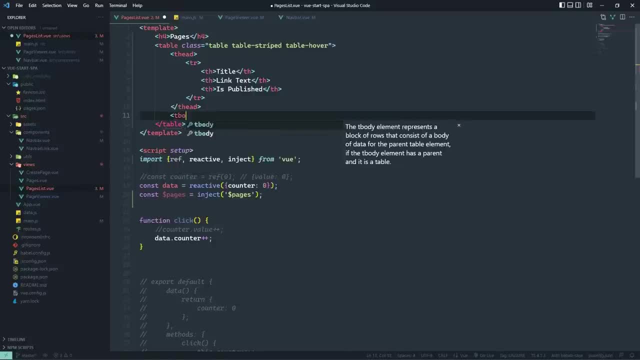 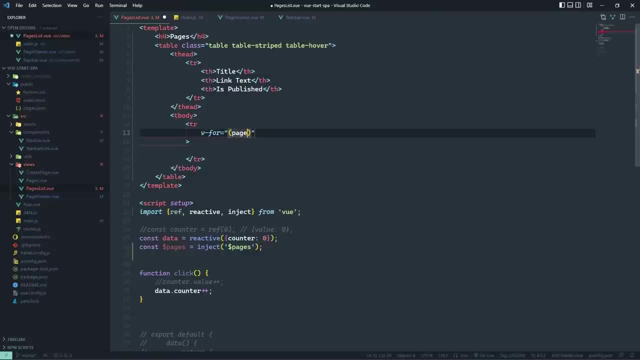 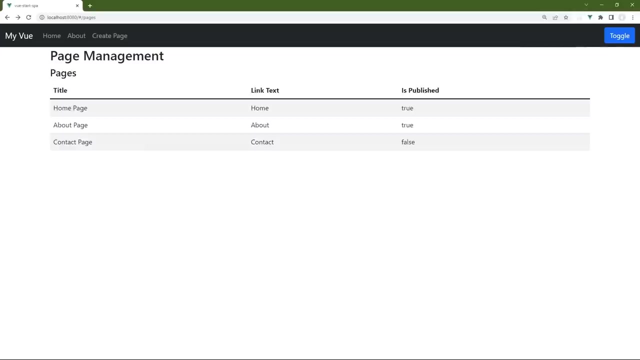 So then we need to generate our body. We'll use tbody first, and then we want to generate a table row. We'll use the v4 directive, and we want to work with the page and the index that is given to us from our pages.getAllPages. We, of course, need to set up the key, so let's use the index for that. And then we just want to display the column information, such as the page title, the link text, and then whether or not the page is published. So with that, we should be able to go to the browser. And we should see our list, but I want to change this isPublished. 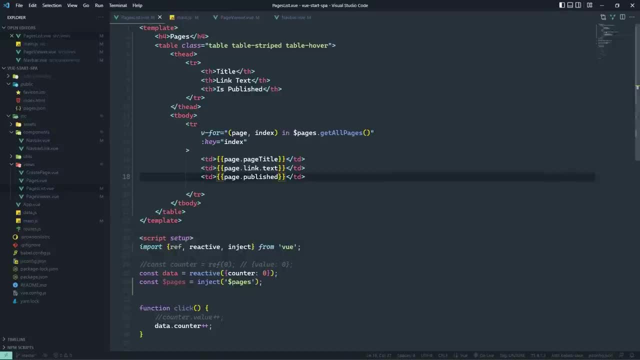 I don't want to use true or false, I want yes or no. So we can easily change that with a ternary expression. 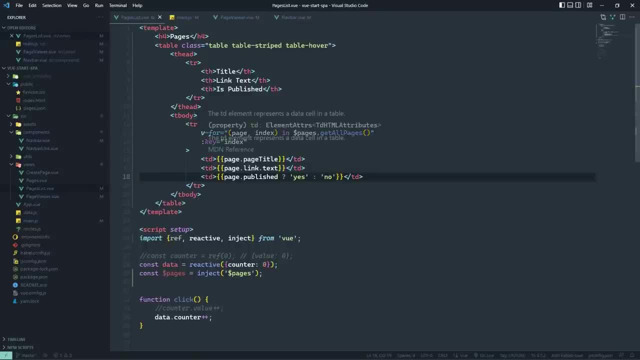 And I want to be able to navigate to the view that enables us to edit each one of these pages, which that's something that we will do in the next lesson. 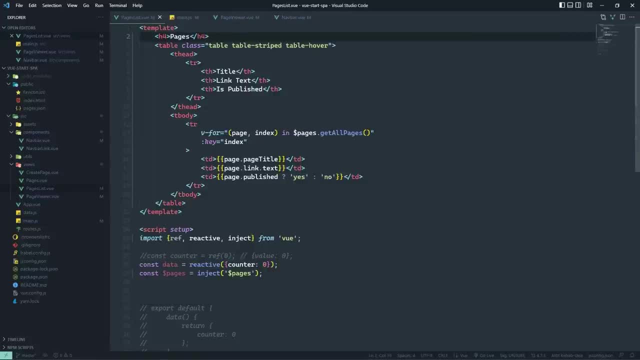 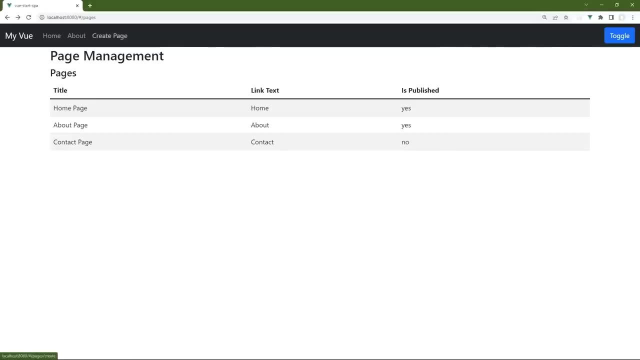 But to prepare for that, I do want to add a Create button. Because I want to take out this Create page link, and I want to add a page link, because to me, it doesn't make a whole lot of sense to have that there. Instead, it makes more sense to have our pages link, so that we can see the page list. 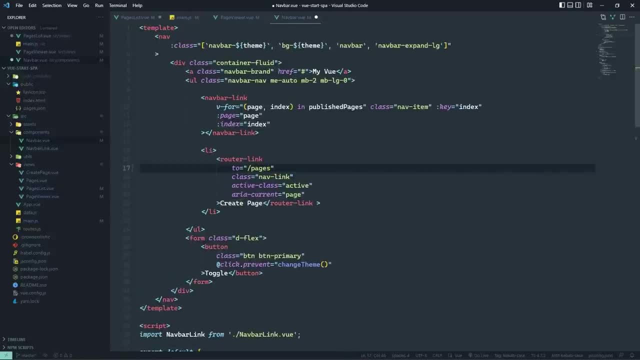 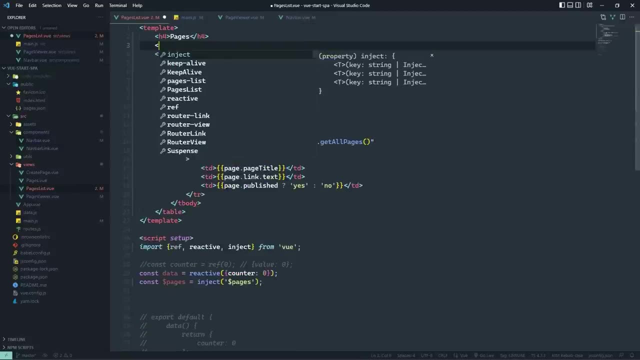 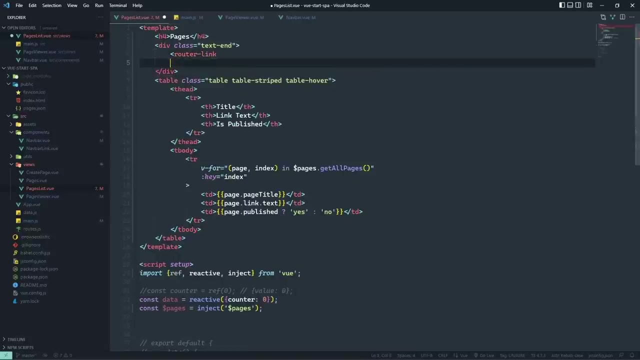 So let's change that link so that it's going to just slash pages. We'll change the text so that it's pages. And then we will add that button inside of the pages list view. We can just use a div. Let's align the text to the end. And then we will use a link to get us to the page list. And then we will get us to the Create, so we will use our router link component. We don't have to dynamically build this URL, so the path will be just simply slash pages slash create. 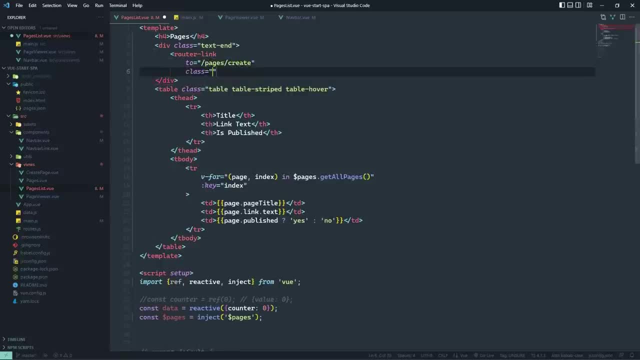 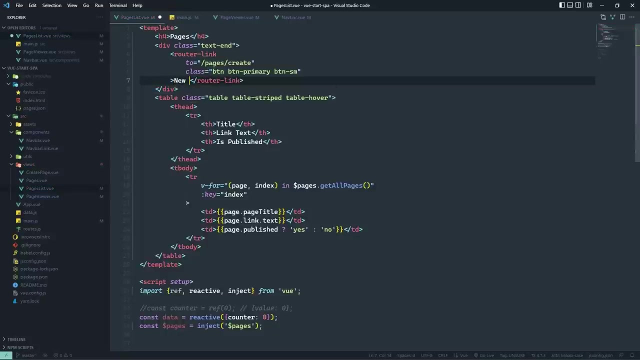 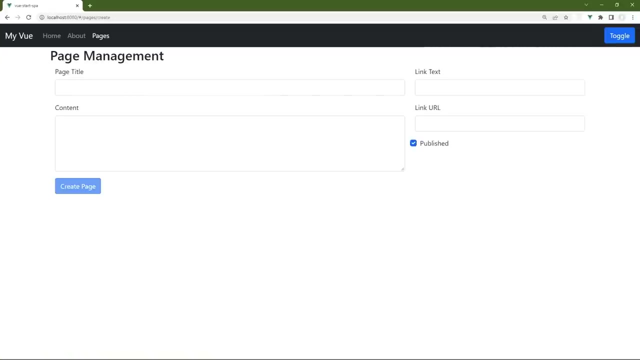 But let's make this look like a button. So we will use some of Bootstrap's classes to make it look like a button. We'll have the button and then the button primary. Let's also use the button small class so that it's not too big. And then we'll have the text of new page. And now there's our new page, we should be able to click this that takes us to the create page that works just fine. 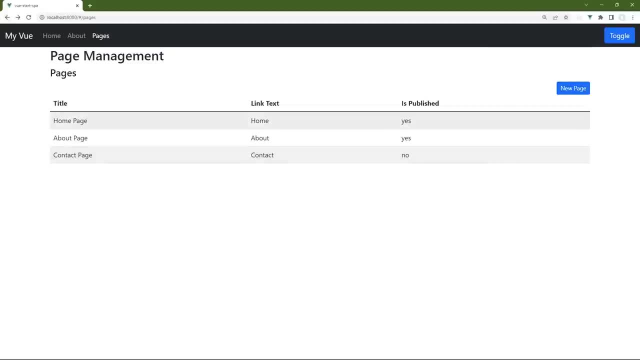 We have our list of pages and now we just need to be able to create our edit view for each one of those pages and we'll get started with that in the next lesson. 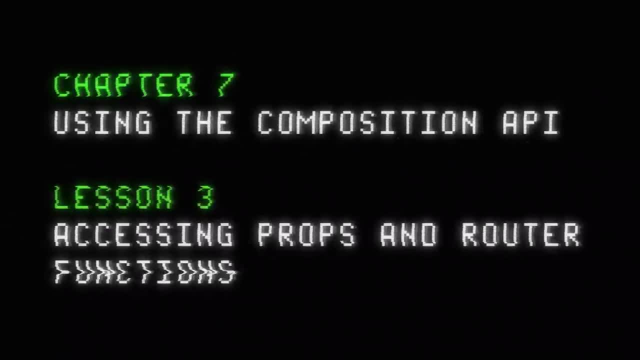 Now that we have our list of pages, I want to be able to navigate to the edit view for any one of those pages. 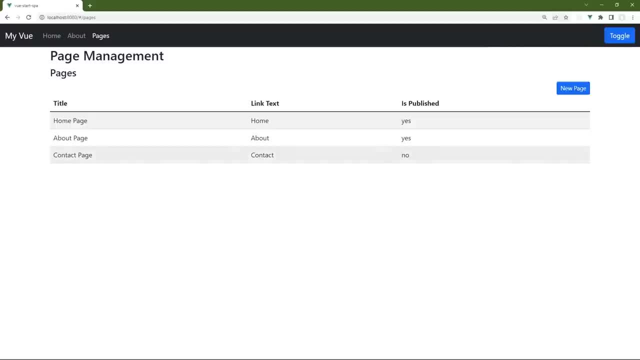 And of course the most straightforward thing that we can do is use the router link component. 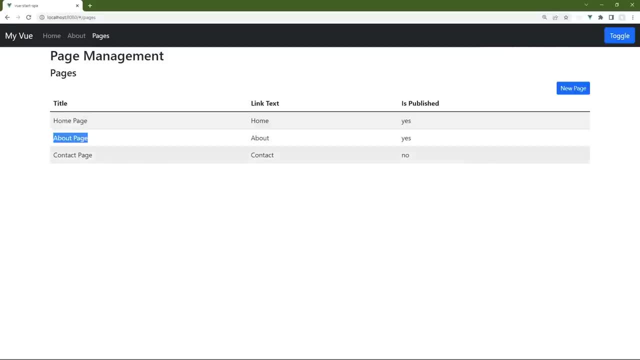 turn the titles into links that the user can then click on, and then there they go. But I want to make this so that the entire row is clickable. If they click anywhere, that's going to navigate them to whatever page is associated with that row. 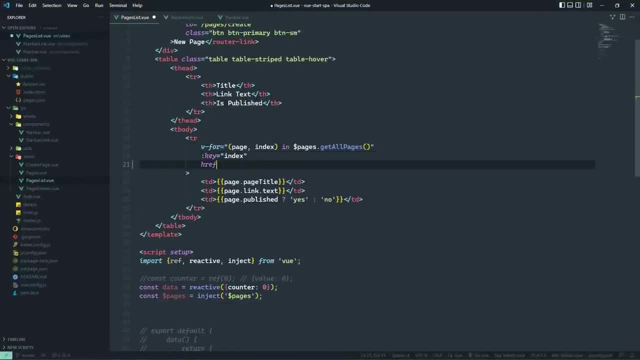 Now, of course, the tr element doesn't have an href attribute. 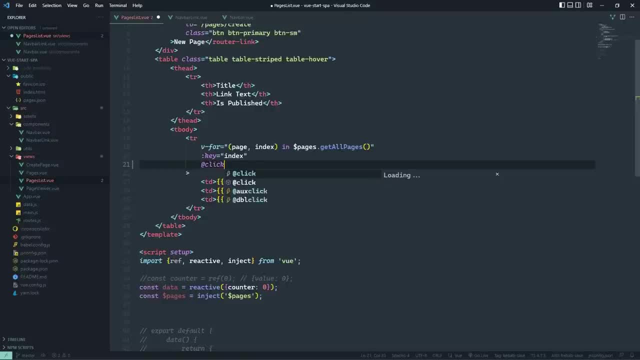 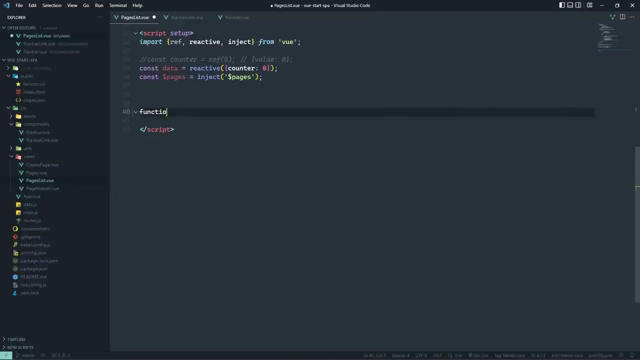 It doesn't behave like a link. So we are going to have to write the code to do that, which means that we need to handle the click event. And we can say that we're going to write a function called goToPage, where we pass in the index of the page that we want to go to. So we can go ahead and we can start writing that function. But we're going to hit a brick wall here pretty soon because, well, 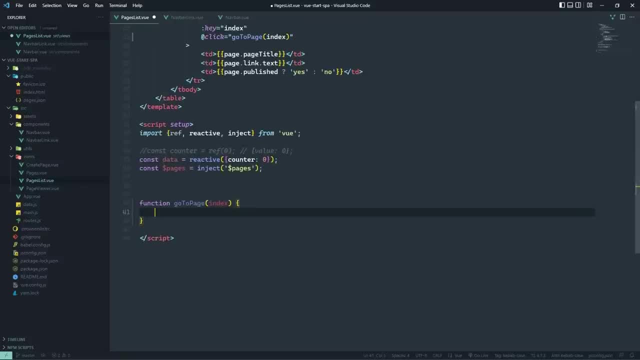 how do we navigate using JavaScript? And the answer is very simple, we just use the router. 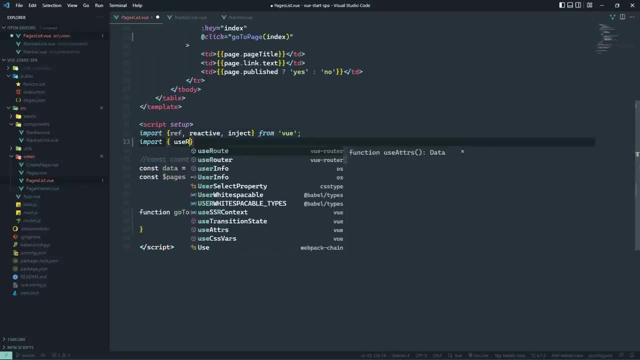 So to get access to the router, we need to import a function called useRouter from viewRouter. Now, we haven't specifically accessed the router, but we do have a function called useRouter. 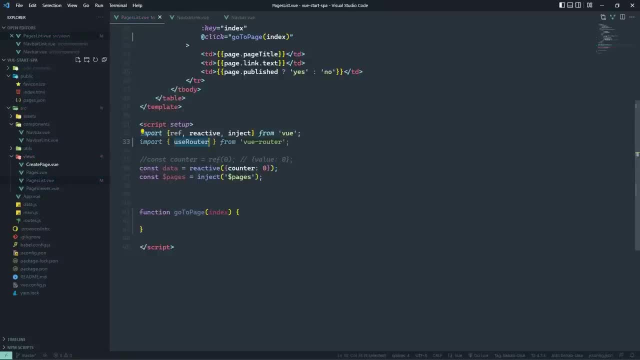 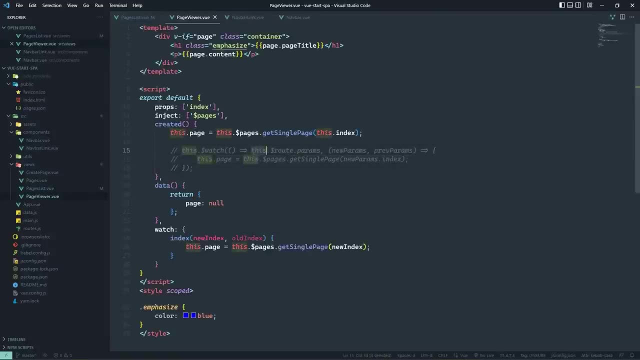 Before using the options API, we did access the route so that we could get to the params, and I believe that was inside of pageViewer. Yes, it is. So we use that $route property in order to get to the params. 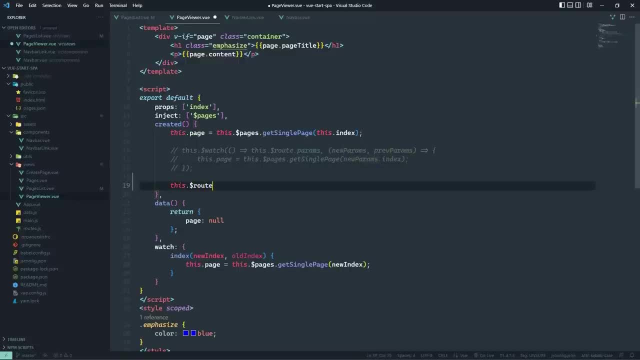 Well, we could do the same thing to get to the router if we needed access to that. 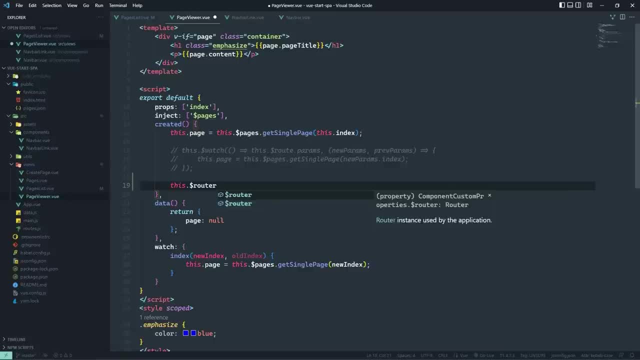 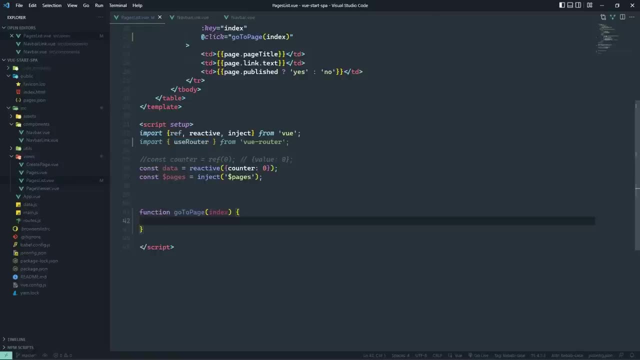 And once you have access to the router, then the API is all the same. So we want to navigate to a different page that is going to be the EditViewer. So we need, first of all, the router. We're gonna call the useRouter to get access to the router. And then we're gonna call a method simply called push. We are pushing in the path of where we want to navigate to. And in this case, it is going to be the pages, and then the index of the page, and then edit. Very simple and straightforward. 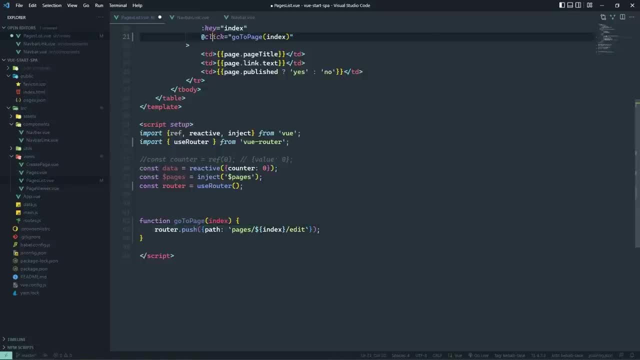 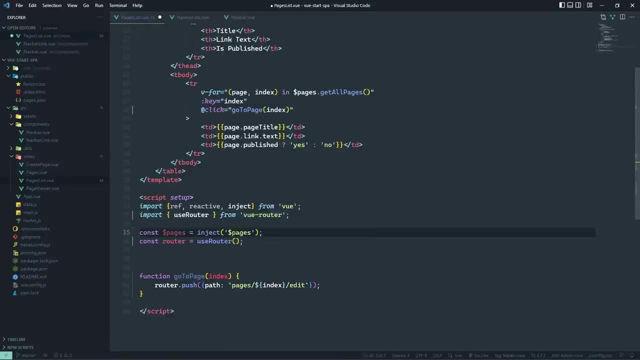 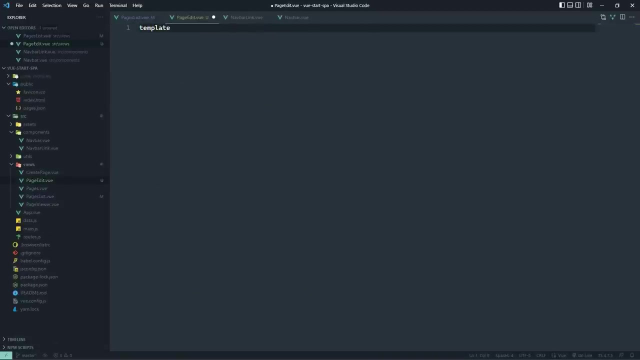 And then by clicking on the tr element, it's going to say, well, it's going to navigate us using the router to that particular view. Now, of course, we don't have that view, so let's go ahead and let's define that. We'll call it editPage, or no, let's do this. Everything begins with pages, or page. So let's say pageEdit.view. Let's have our template for right now. We'll just have some text that says editPage. And then, of course, we need to add a route to this view. 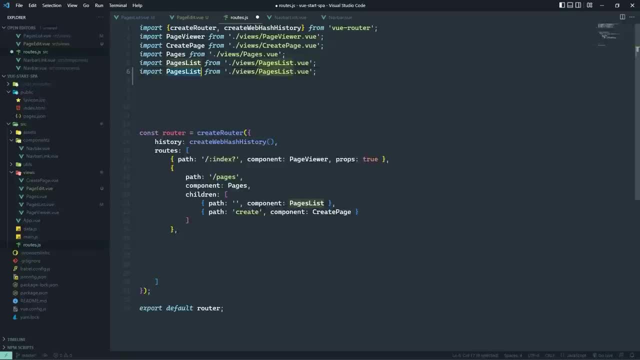 So let's open up Router. We need to import this component, so let's do that. And then we want to add this as a child to our pages. So we're gonna add another entry to the children. And the path is going to be that simple path of the index program followed by edit. And then our component is going to be the pageEdit component. So with that in place, we should be able to click on any one of these, which, I think, signify that we can click there. So let's change that. 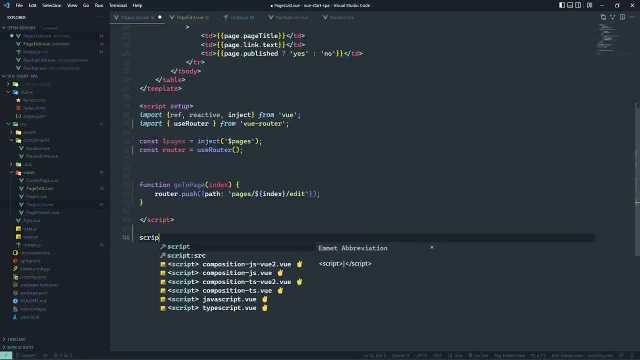 Let's go to our pages list and let's add some style. We can make this scoped to this component, cuz really we wouldn't need it anywhere else. 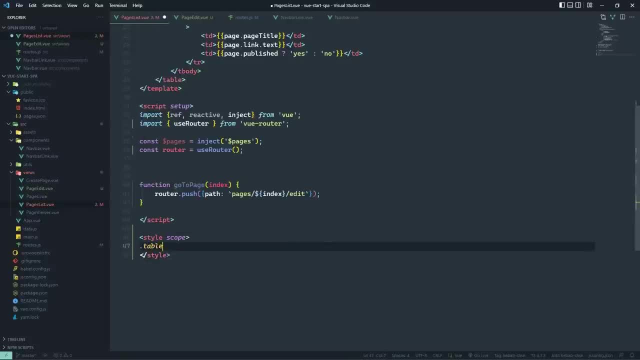 And we want to add some styling to the table that has the table hover. We want to do this on the tr element whenever we hover over it, and we are just going to change the cursor to the pointer. 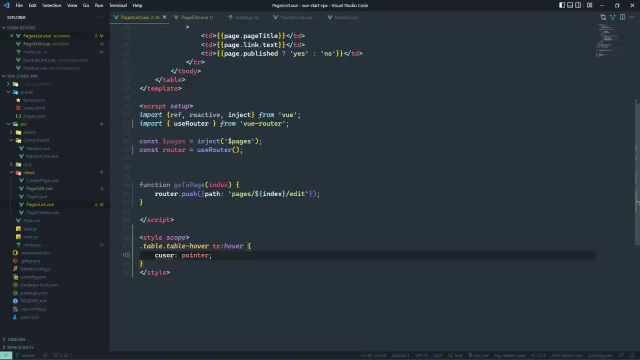 Typically signifies that this is something that you can click on. So that's going to work there. 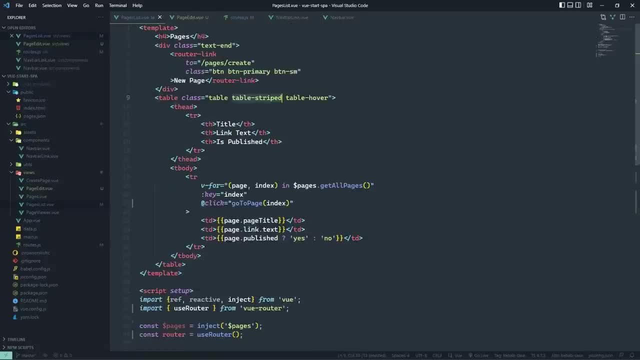 Let's also get rid of the striped, because since we have hover, we don't necessarily need striped. 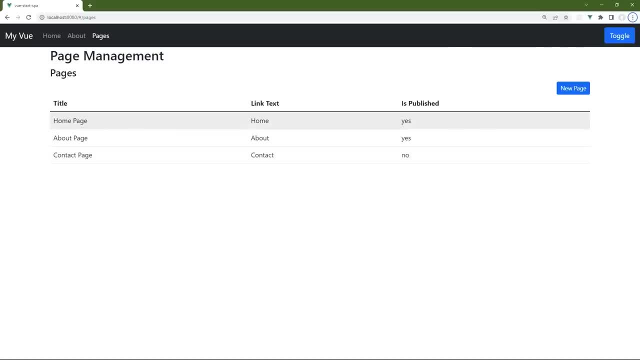 Because the striped is there to make it easier for the user to see what data is on which row. 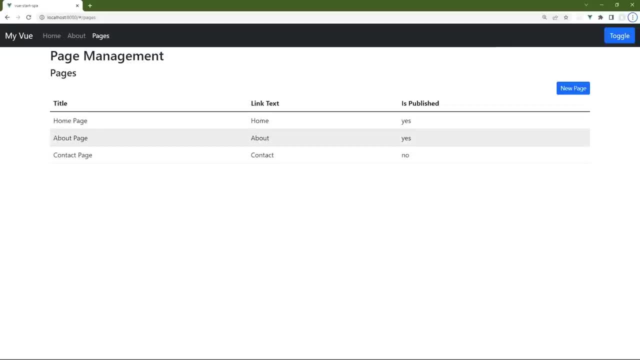 But whenever you have the hover, we don't need that at all. So whenever we click on this about page, we should be taken to the edit page. 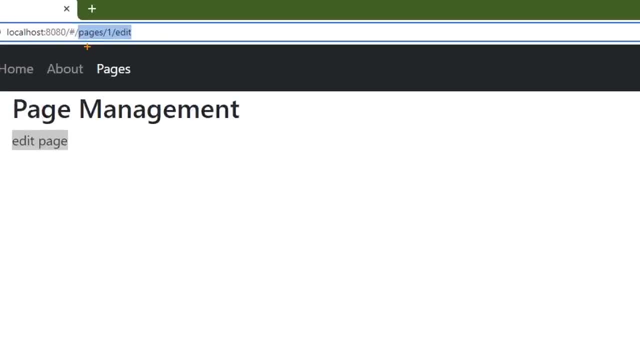 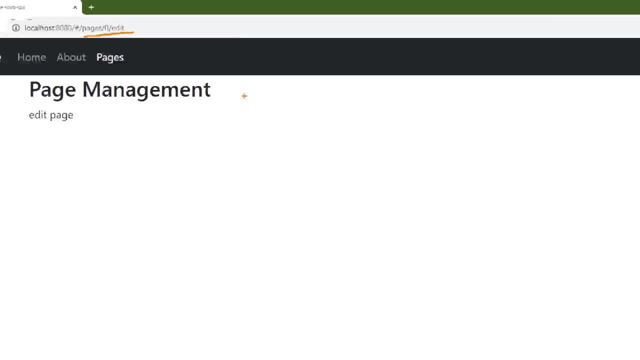 The URL is what it should be. It is pages slash one slash. Edit, if we click on home page, that should be pages slash zero slash edit. 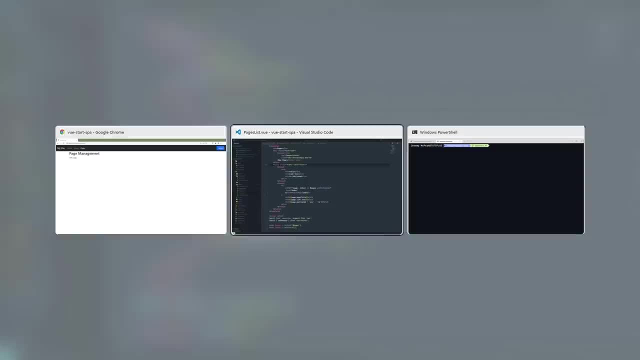 So yes, this is indeed working. So that's great. 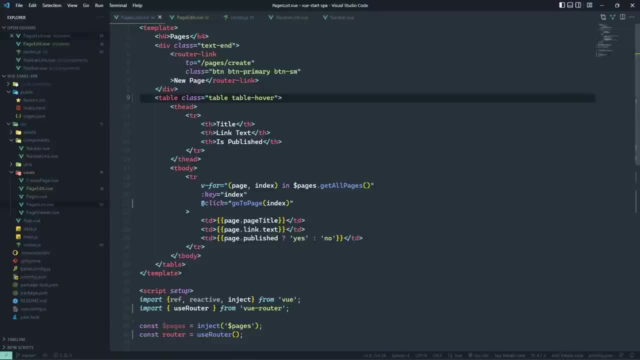 Now we need to be able to get the param information from inside of our page edit. 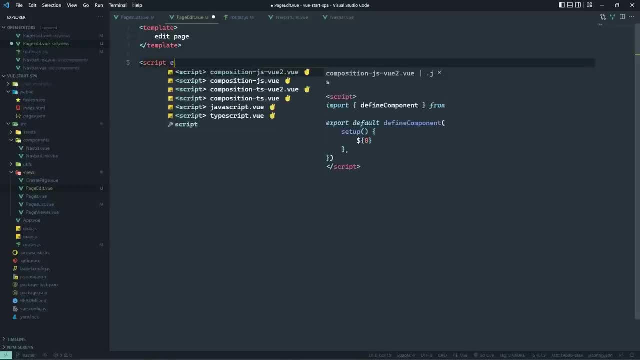 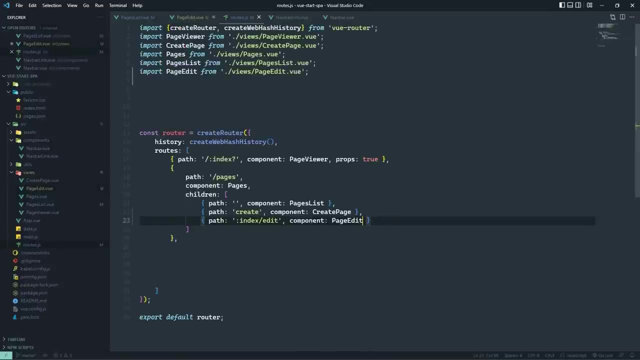 So let's start adding our script for that. We'll use the setup attribute. And we know that we can get this data in one of two ways. We can get it from the params from the route. Or we can define that the params will be passed as props. Let's look at both. So let's add the props equal to true for that particular path. Let's go back to page edit. 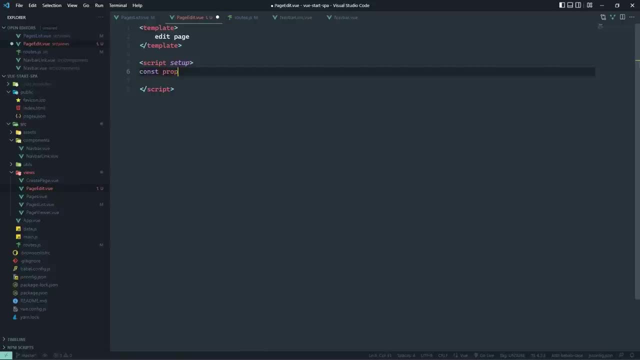 And the first thing that we will look at is getting our props. So there is a built-in function that we can use without having to import anything. And it is called define props. And it works a lot like the props option in the options menu. But if we go back to the options API, we can pass an array that contains the strings of the props that we need. So in this case, that would be index. And then from there, we can use our props as an object to get our index. So by saving this, let's go back to the browser. Let's refresh, and that says edit zero. 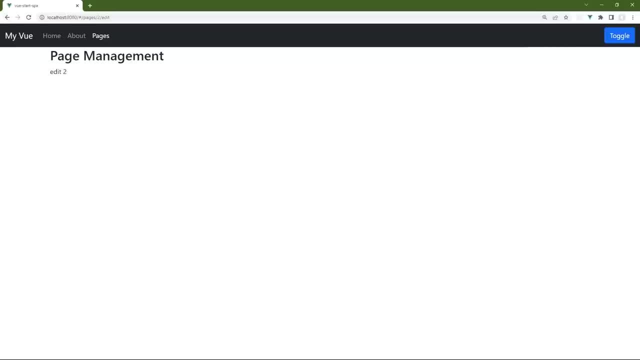 If we go to the about page, edit one, and of course contact is edit two. So that all works. 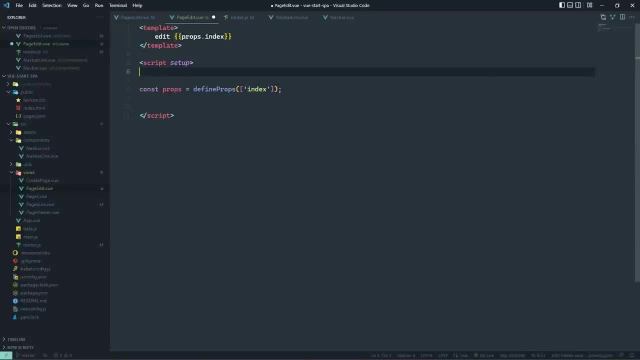 But let's look at how we can do the same thing. Okay. if we don't want to use the params as props. 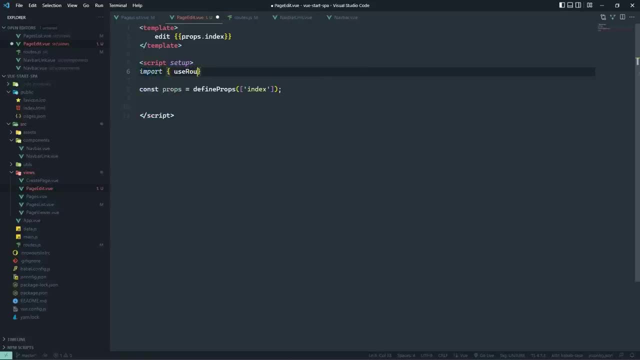 The first thing we need to do is import the useRoute function, which is from viewRouter. And then we want to get the routes, which is essentially the dollar sign route property that we would use inside of the options API. 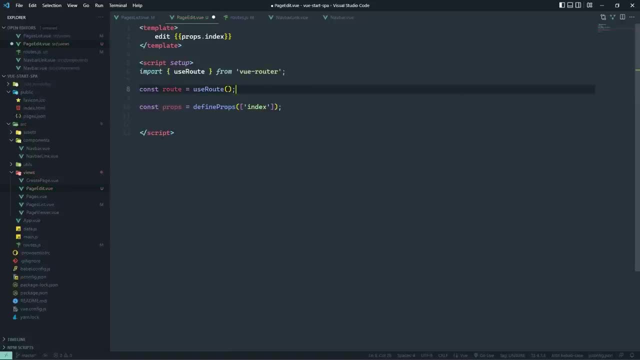 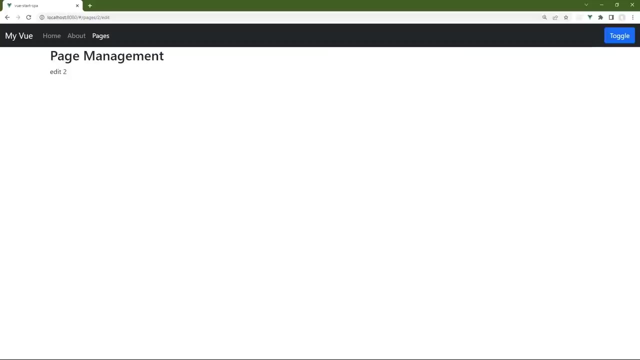 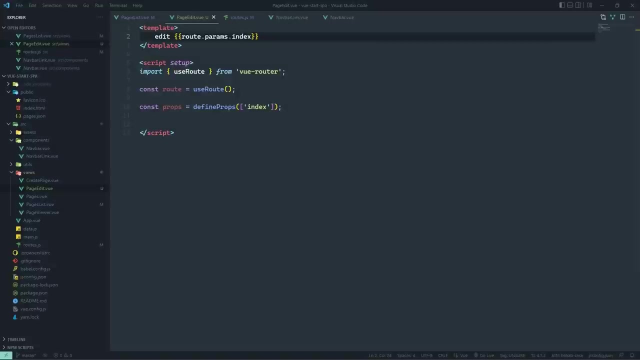 And we get that by calling that useRoute function, so that then from there, we can use the route to get to the params and then get to the index, which whenever we view this in the browser, let's just do a refresh. We see once again, edit two for the contact page. If we click on the homepage, edit zero, click on about, edit one. So the composition API doesn't hinder us really in any way. 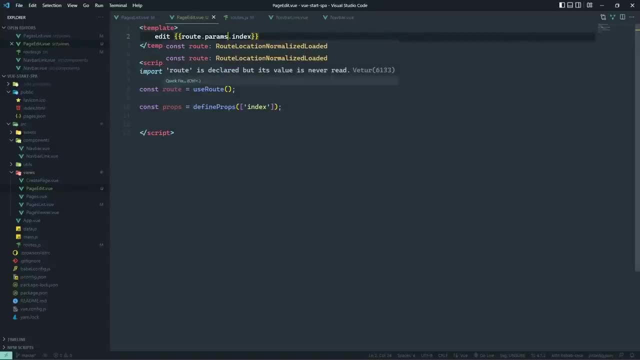 We might have to write a couple of lines of extra code in this case to get the route so that we can get to the params, but that's arguably negligible. 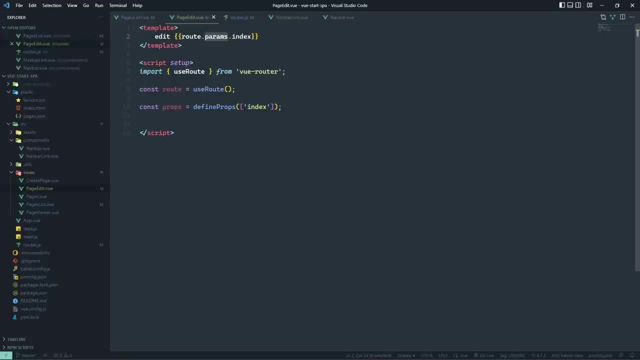 And so in the next lesson, we will implement, we will implement the edit view. 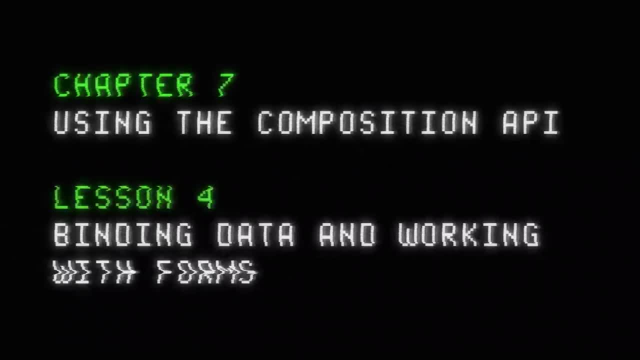 We are finally to the point to where we can actually start working with our data. And we will begin in this lesson by implementing the edit view. Now we have a lot to do, so I'm just going to jump right in. 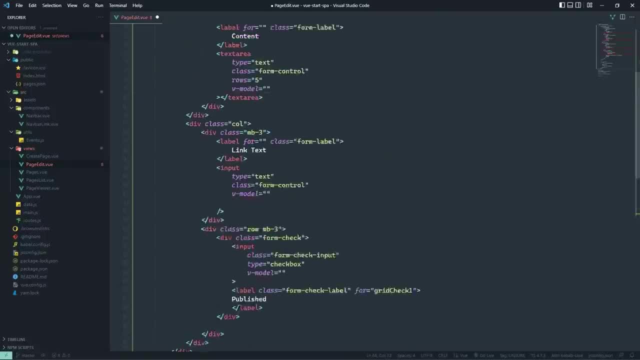 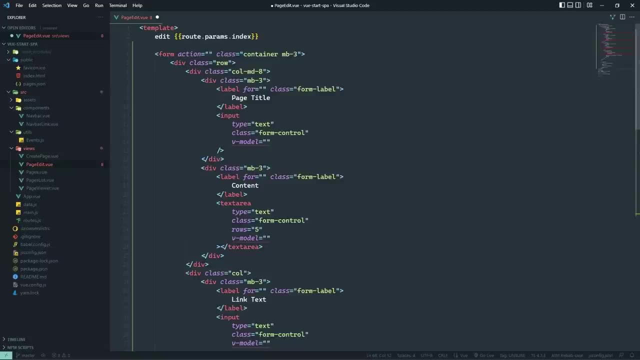 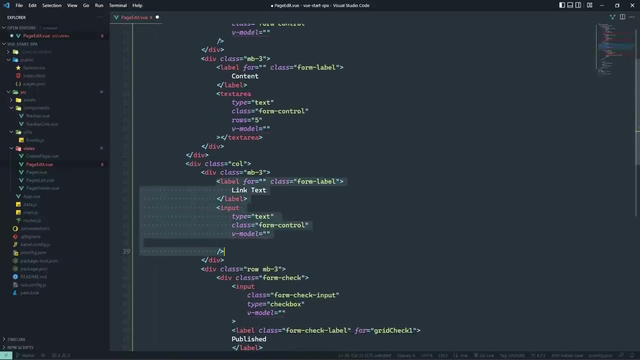 And the first thing I will do is paste in the markup for the edit form. Now this is almost identical to the form in the create page view, which is also something we need to fully implement, but there are two differences. The first is that there's not a link. There's no URL field because, well, we don't need that now that we're using view router. And there's also a cancel button. 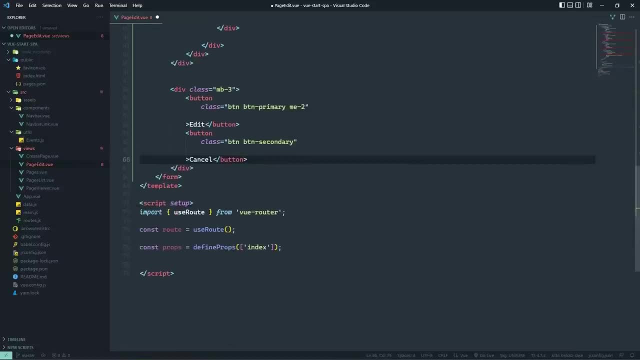 So those are the two changes. And let's just start with our JavaScript. Now, as far as our index is concerned, 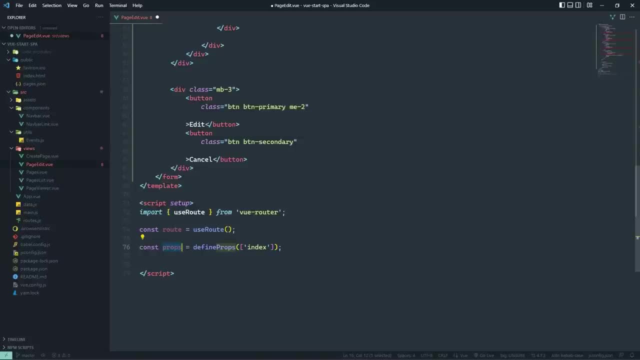 I think it's easier to just get that from our props because we are set up to do so, and we can destructure our props so that we just have direct access to index, which can't beat that. 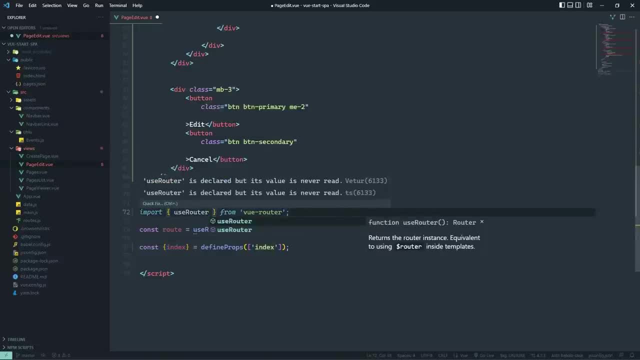 Now we will need the router. So I'm going to change this import statement. 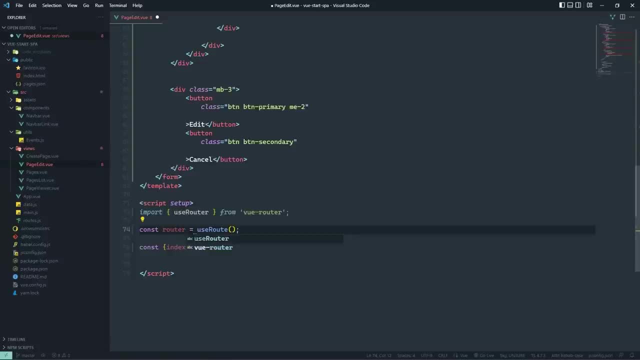 So that we import the use router and we'll go ahead and get our router. But we also need the inject method from view because we need to be able to pull in our pages data store. So let's go ahead and let's do that. We'll just call it pages. And the key that we want is dollar sign pages. And then that is going to give us the ability to just get the page object that we want to work with. So we will use the page object. So we will use the page object that we want to work with. We will use pages. 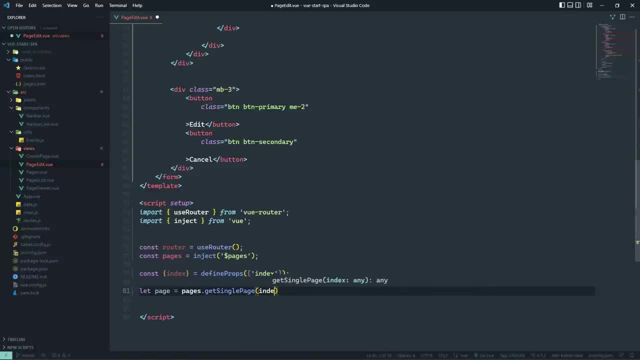 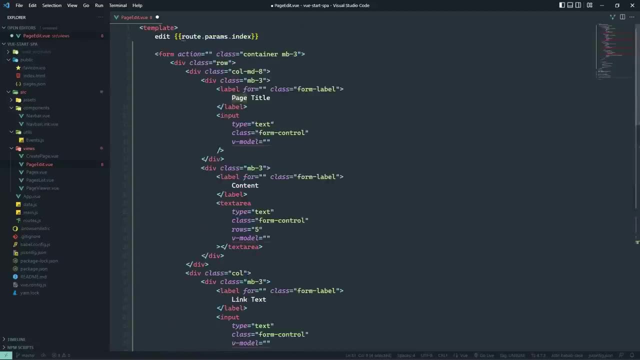 I think it was called get single page and we will pass in the index. So this page object that we get is what we can use to tie into the individual fields within our form. 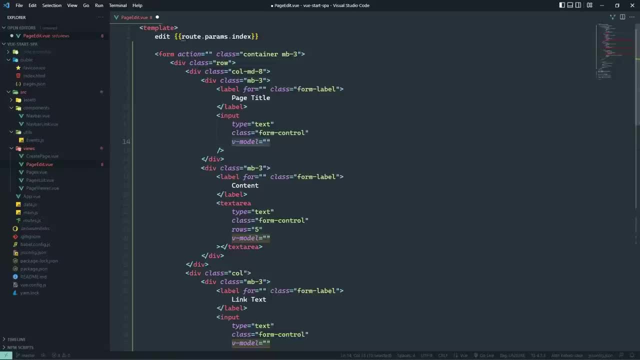 You know, we have V model and in the past we've just set that to an individual value within our component, but we don't have to do that. 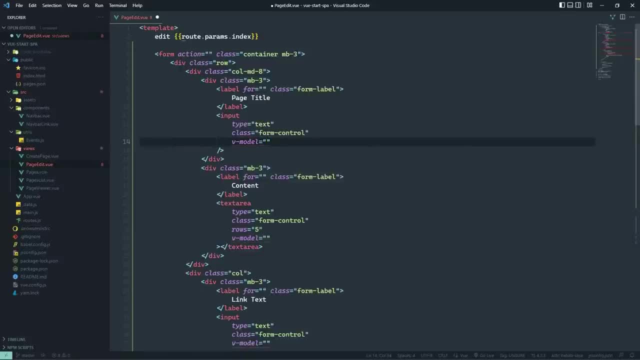 We can also set up the V model so that it is bound to a property on the page object. 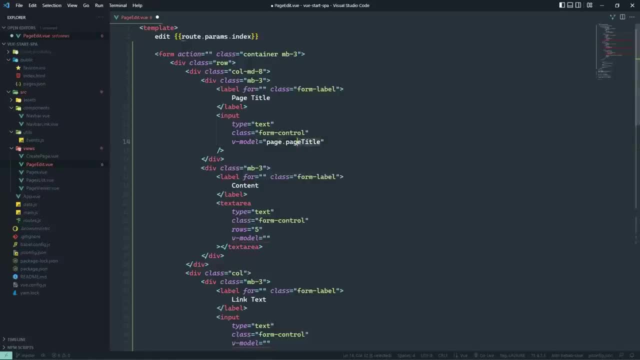 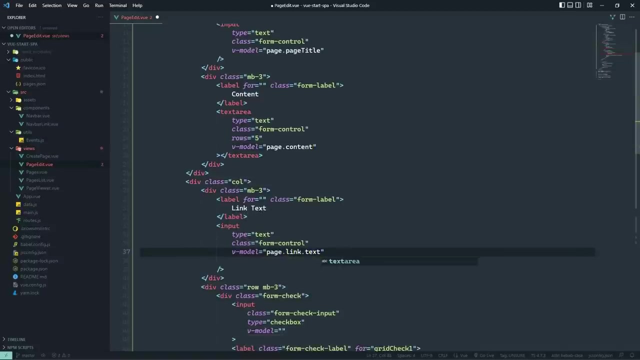 So the page title property will be the V model for the page title field. And then the content property will be the V model for the content. The same will be for the link text, except that that is link dot text. And then finally the published, and this is going to make our lives so much easier because we get the functionality of V model, but then we don't have to make any changes to the page object because that was automatic. It was automatically done by V model. So we're all good there. 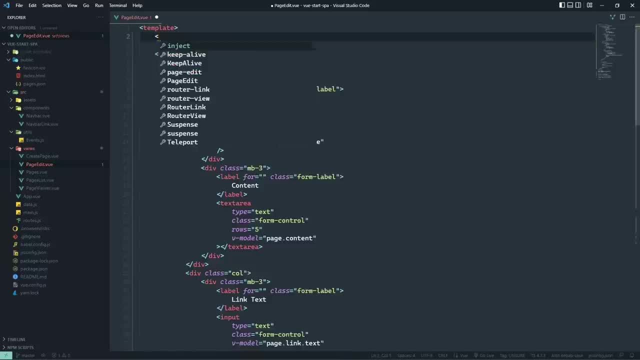 Now there's one thing I wanted to do and that is change the title. I believe we used an H4 in the pages list. So we'll do the same thing here. 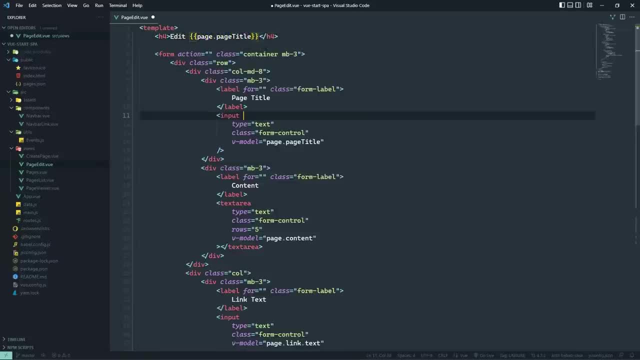 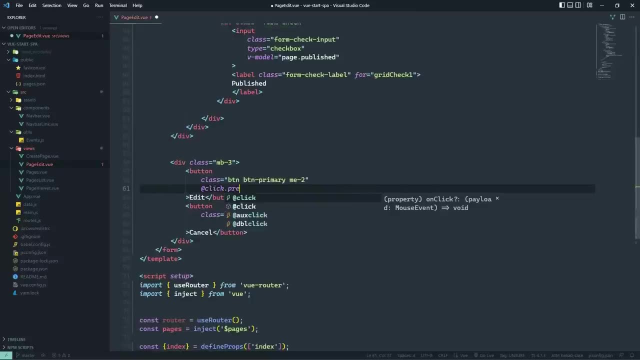 We'll just say edit and then we will use the page title so that when it comes time to actually save this for the edit button, let's listen for the click events. We will of course prevent the default action and we'll just call this submit. 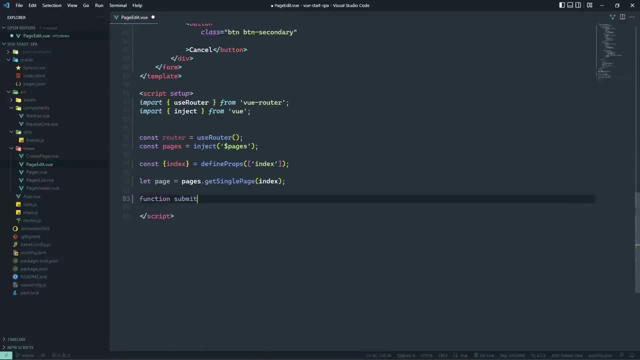 And then inside of submit, we will do, this. 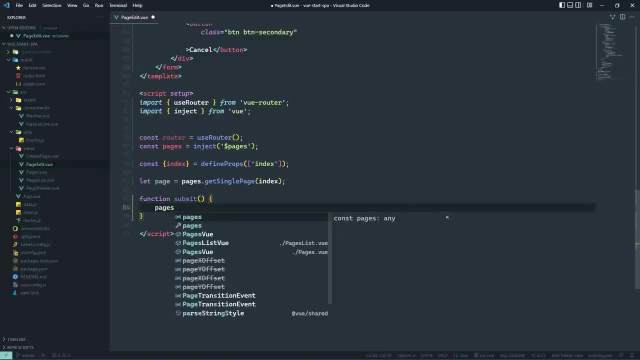 It's going to start off fairly simple in that we will use our pages. Now we don't have this method yet, but let's just say that we'll have a method called edit page to where we can supply the index and then the page object that we want to save. And that'll be it at least for now. 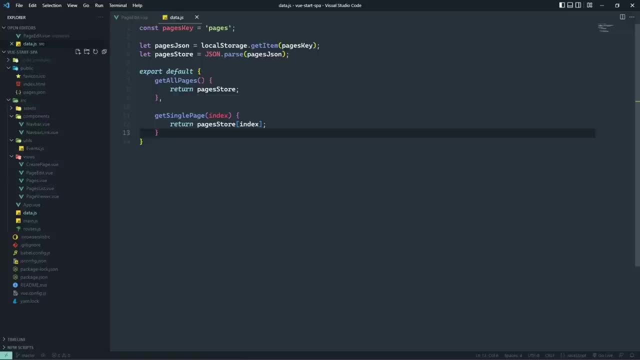 So that means that inside of our data, we need to implement that function. So let's do that. 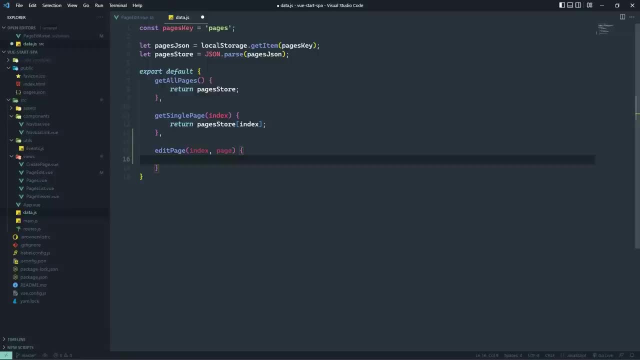 We need the index and the page, and we need to do two things here. The first is to update the pages store array so that at the given index, we now have that page object, but then we also want to store this in local storage so that it persists between refreshes. 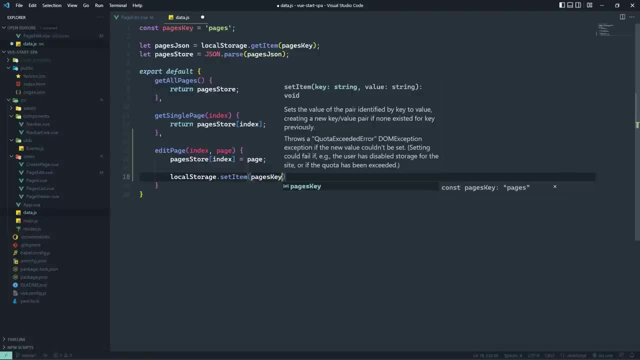 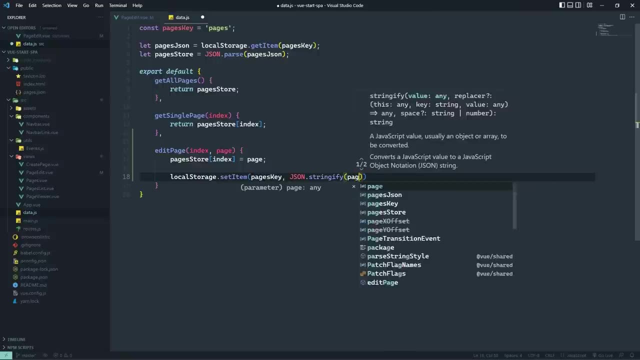 So we'll call set item. We want to use that pages key as the key, and then we'll use the serialized pages store as the value. So that should work. 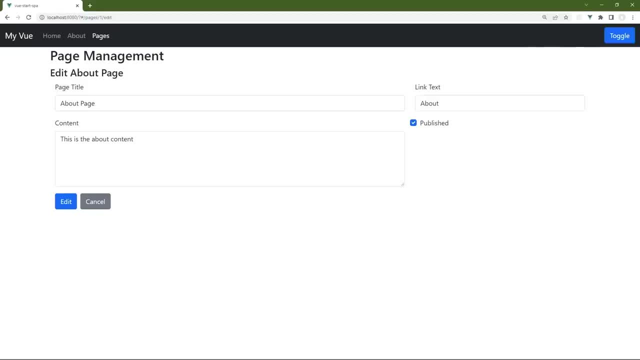 And with that done, we should at least have the basic functionality so that's let's go to the browser. 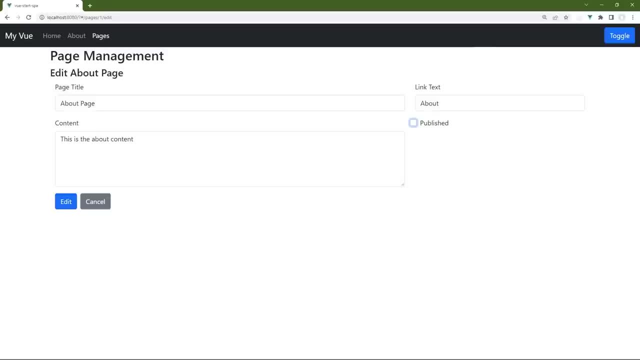 Let's uncheck published here for the edit page. Let's also pull up the console so that if we get any errors that we can see that and let's click on the edit button. 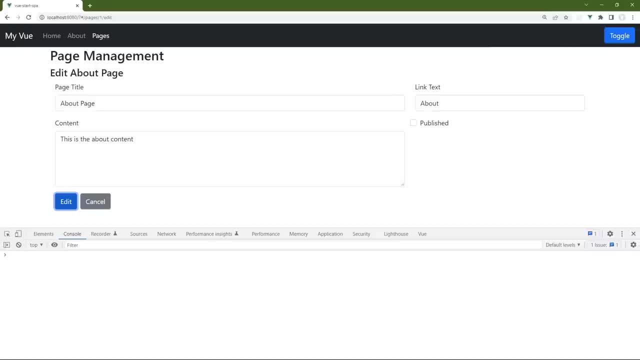 Now it looks like nothing happened, but really that's what we want because we don't have any interactivity or any reactivity, I should say. 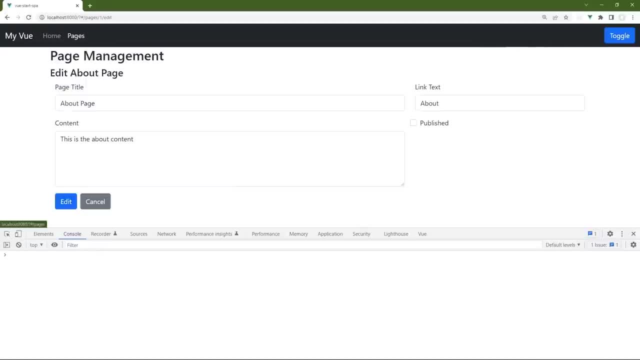 So let's refresh the page and the about link should be gone. It is. So. 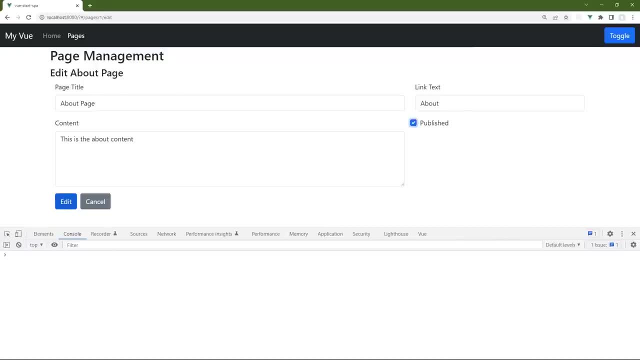 It's working at least as far as editing and saving this information. So let's make it published again. 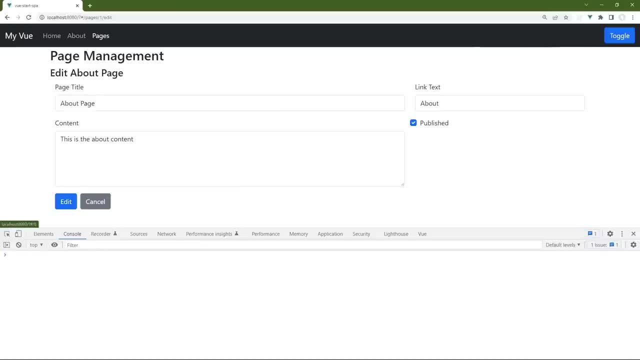 Let's refresh so that we can at least see the about link there. So we have the basic functionality, but now I want to make it so that whenever we save a page, 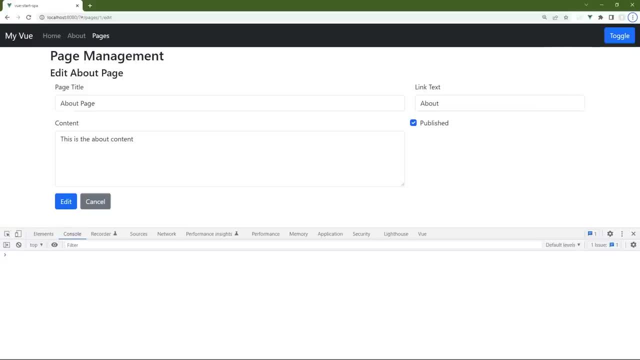 it's going to reload everything that relies upon those pages. And I think really the only thing is our nav bar because it needs to reload the published pages here in order to generate those links. 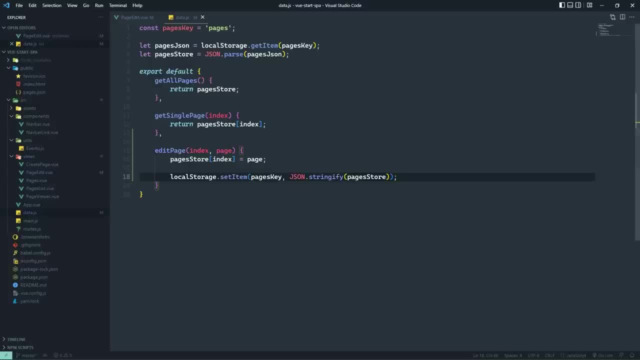 So the way that we can do that is by using our global event bus. I mean, we have that, so we might as well use it. 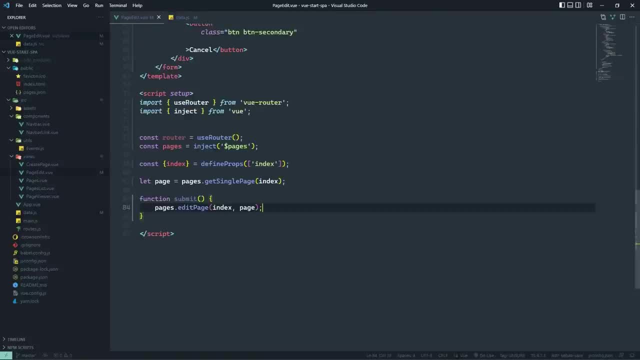 So that's whenever we submit the form, what we could do is use our bus and we would use the emit method to where we could say a page updated. 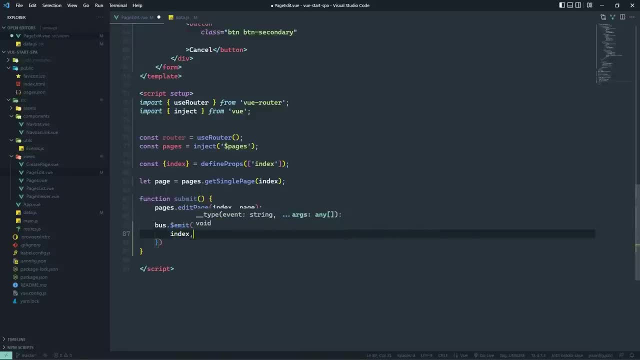 And then we could also supply some information about the page that was updated. 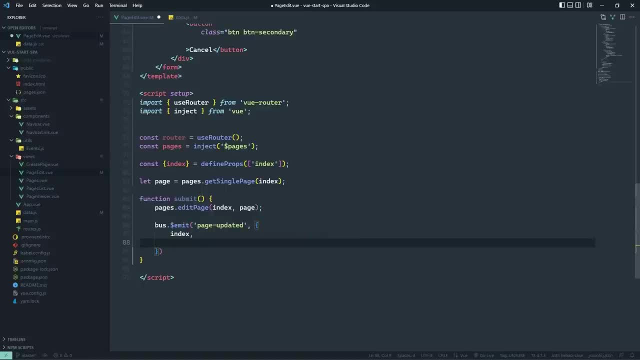 Now, not everything would need this information. Like for example, the nav bar wouldn't really care what page was updated. 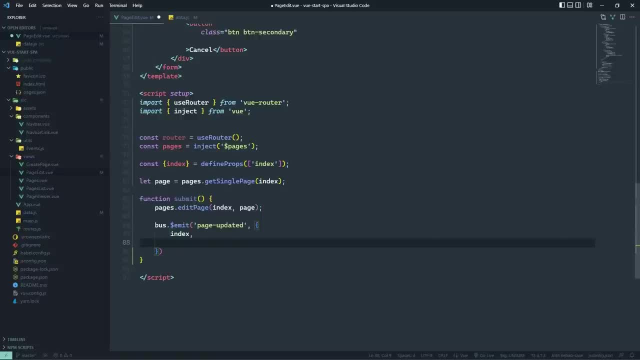 It just needs to know when the page was updated so that it can reload the pages. 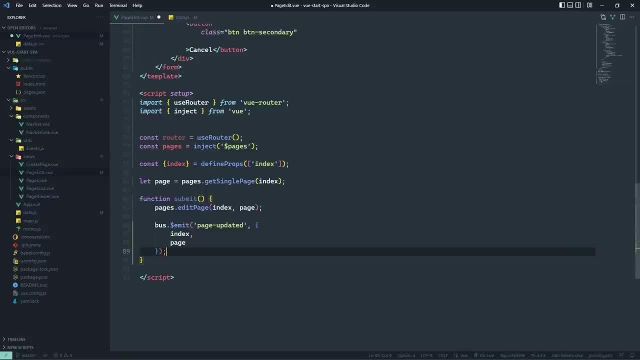 But this way for anything that needs this information, we can supply that because it's easy enough to do. 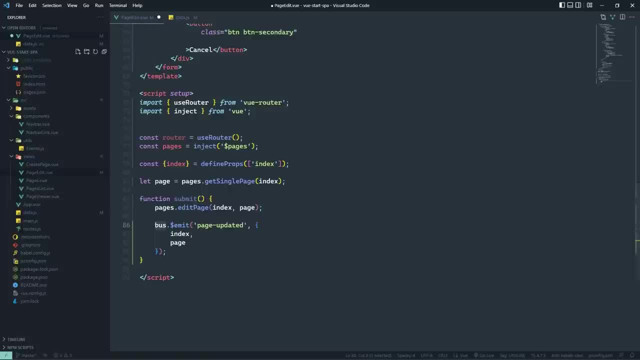 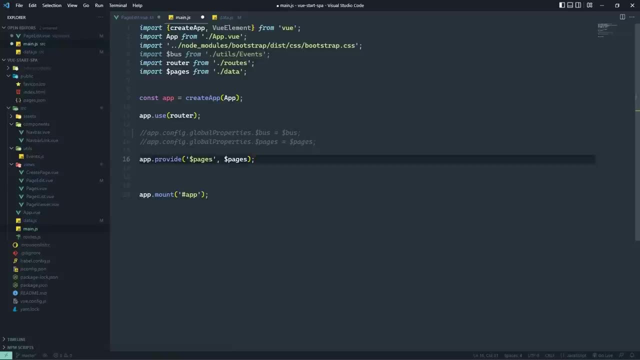 Now, of course we need that bus and currently it is set up as a global property. So we will essentially do the same thing that we did for the pages. 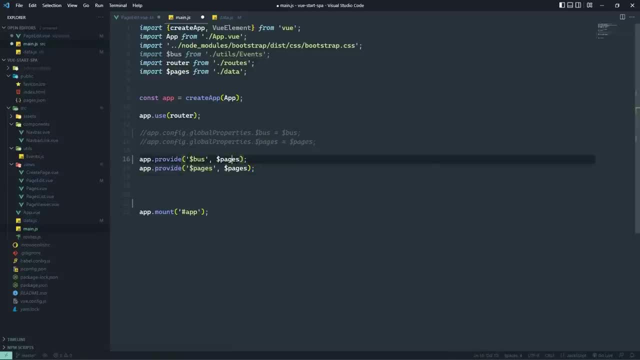 So that's, we'll just have dollar sign buses for the key and then dollar sign buses for that value. 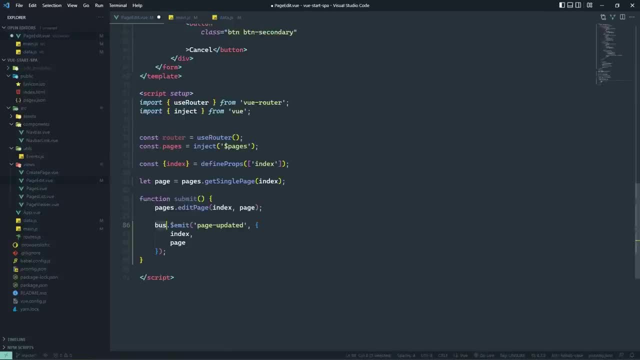 So that inside of page edits, we can inject that just like we did the pages. So let's do that. We'll just call it bus because we already have the code. That's going to do that. 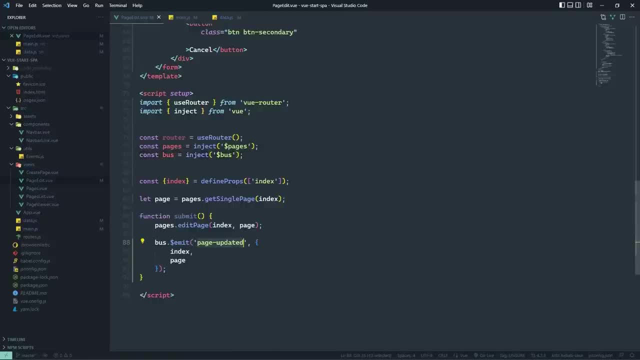 And then we need to listen for this event inside of nav bar. 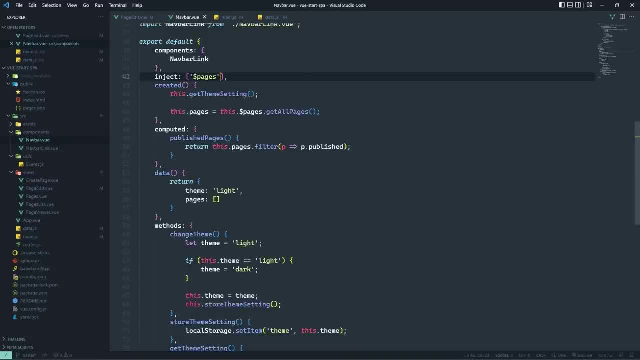 So let's open up nav bar and we want to inject dollar bus as well. 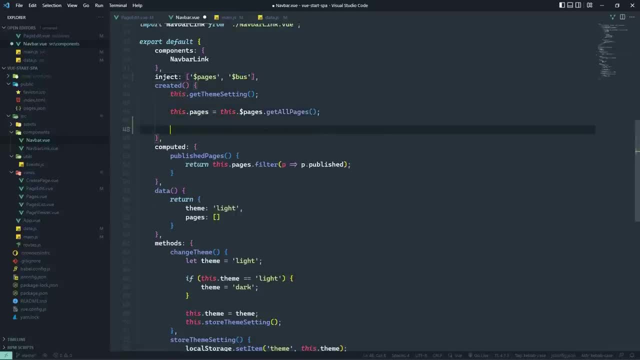 And then we went to set up the event listener for that page updated. 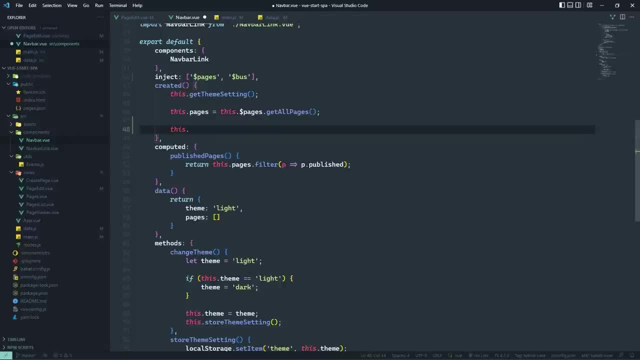 So we can do that right here inside of the creative. Created hook to where we would use our bus. And we will call the on method. We want to listen for page updated and for the function that's going to execute, all we need to do is update our pages. 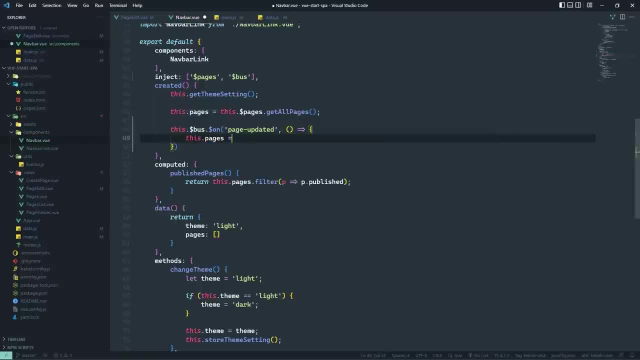 This is the pages data property inside of this component with the new pages. So that should work, right? 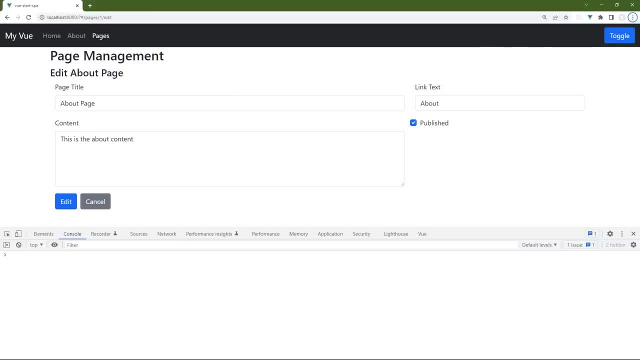 Well, it's not, and we'll talk about why here in a moment, but let's, first of all, prove that it doesn't work. So I'm going, to unpublish this, I'm going to click on edit. 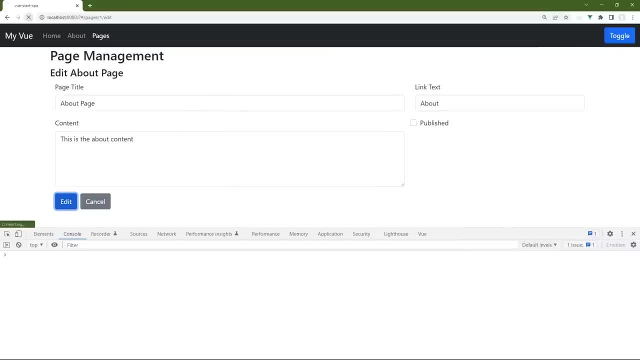 We don't get any errors and it doesn't look like anything works, but whenever we refresh the page about is gone in the nav bar. 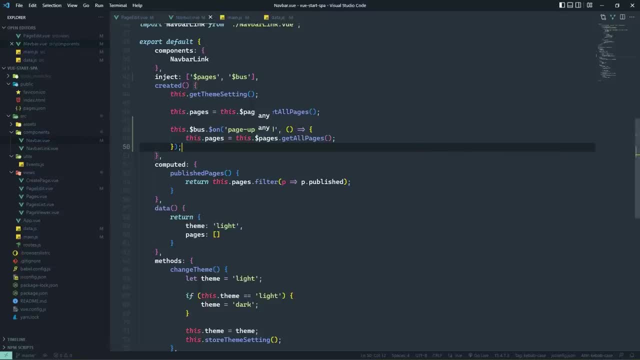 So let's talk about why the nav bar didn't automatically update. And it's really very simple. And it's because of this right here. Uh, 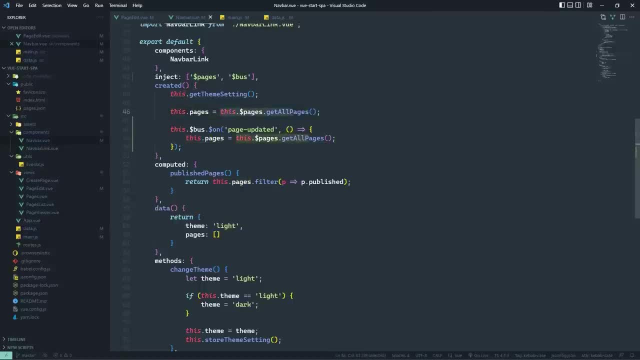 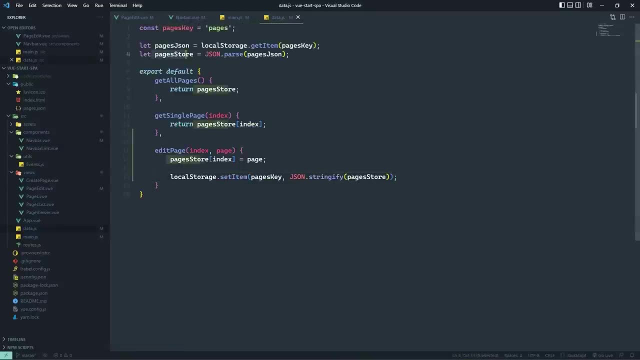 whenever we set pages originally, we did so by calling, get all pages. This is returning that array. That is, 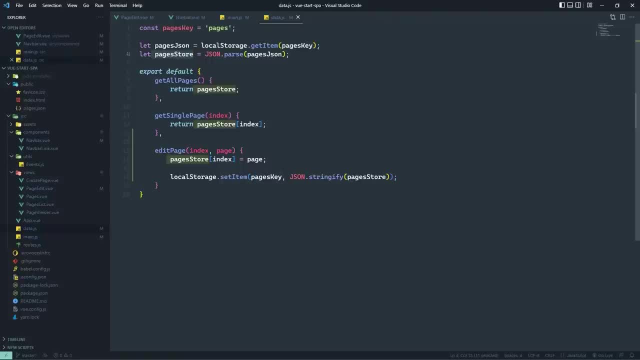 inside of our data. So this array object never changes the data inside of it may change, 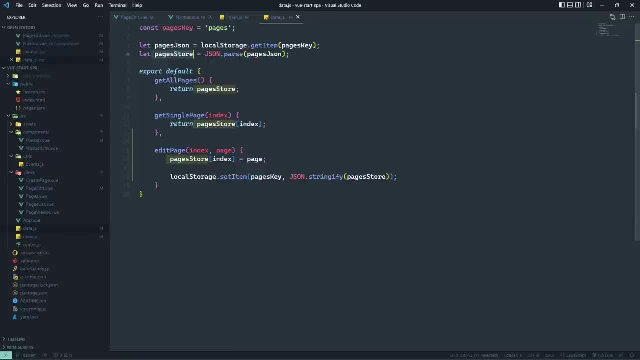 but the array object itself never changes. 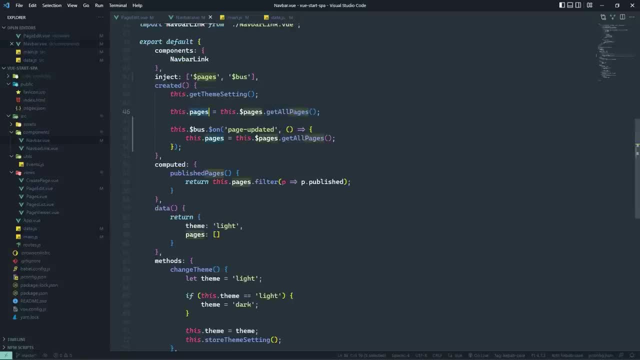 So inside of nav bar, whenever we set the pages data property to get all pages, 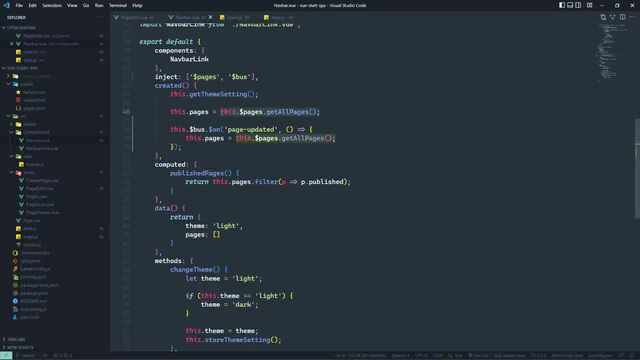 it's watching that array object. And even though we update the contents of one of the objects inside of that array, 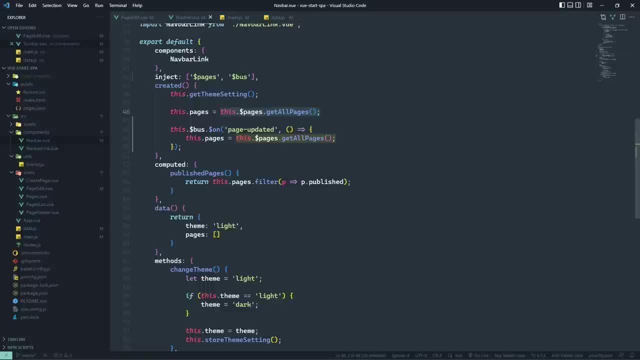 it's not watching the individual objects. It's just watching. That array. 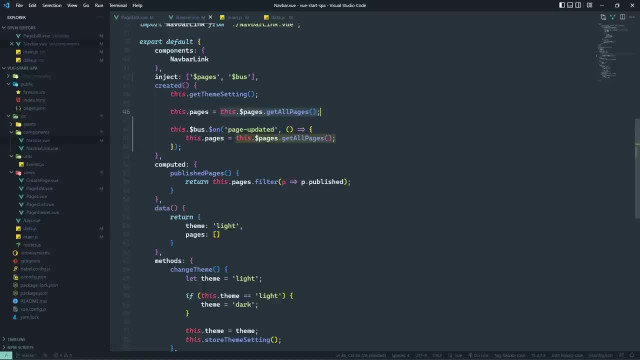 Now, if we added an item to the array, then yes, it would recognize that this array changed, 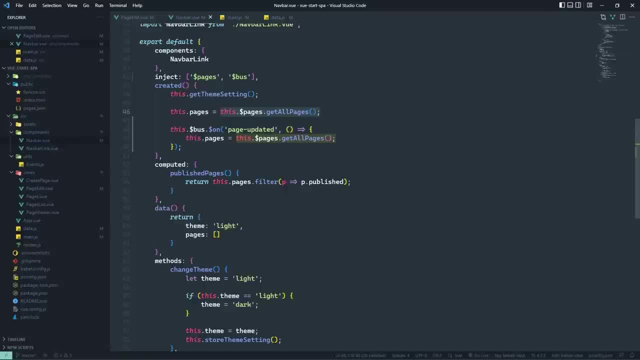 but it's not watching the individual objects inside of the array. 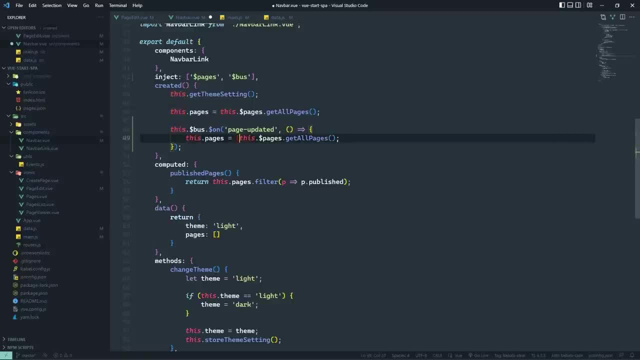 So what we can do then is this. We can assign a new array to the pages data property inside of nav bar, 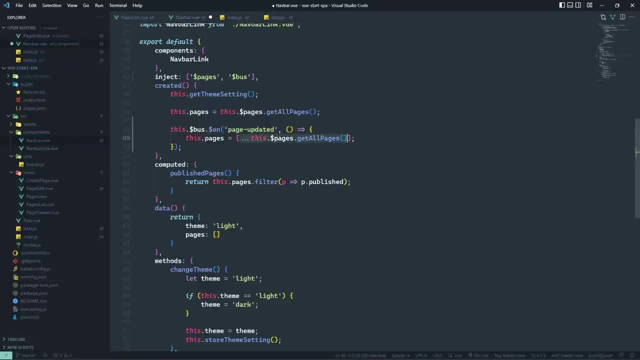 and then we can fill it by spreading out the array that we get from get all pages. So we are creating a new, a new array object. 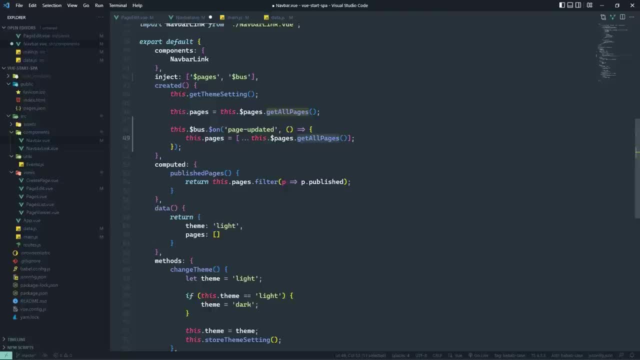 We are populating it with the elements from get all pages. And so every time page updated occurs, then it's going to be a new array. 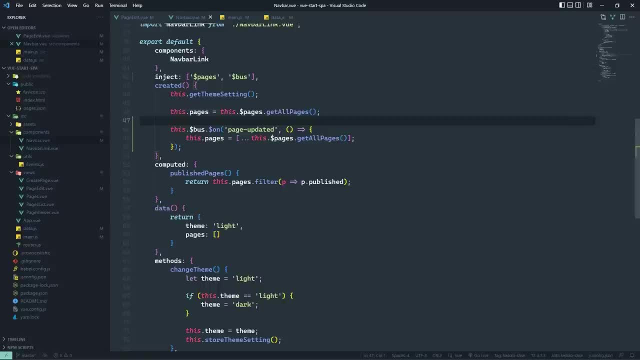 And that's going to tell the nav bar component that, Hey, the pages array changed. 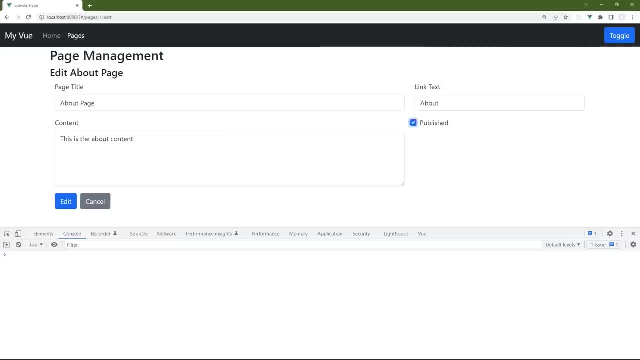 So with that change, we should be able to click on publish. Now click on edit and we see about appear. And if we, unpublish it, click on edit that goes away. 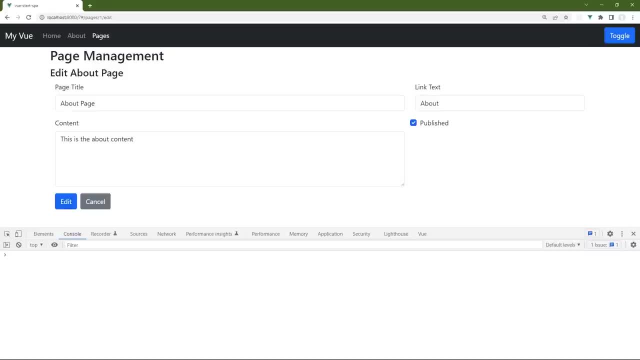 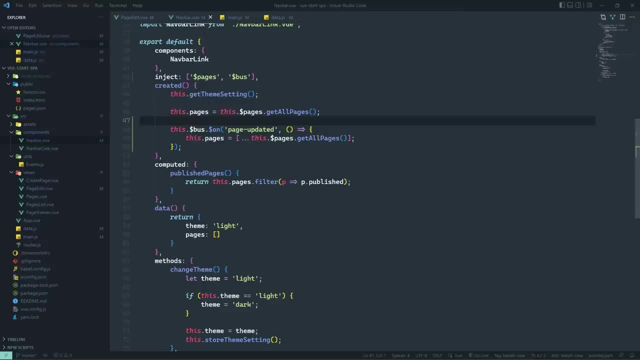 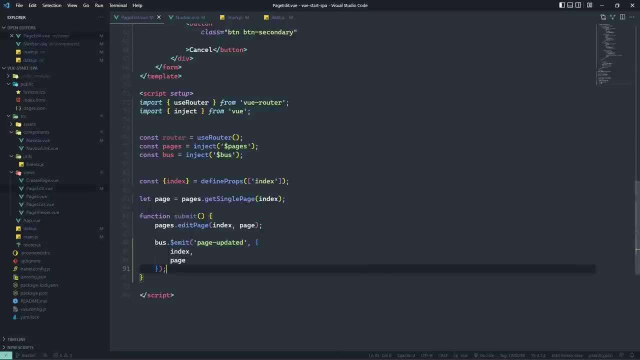 So now the only other thing that I want to do is navigate back to the pages list whenever we click on edit or whenever we click on cancel, because we need that functionality so that whenever we edit a page, of course the page will be edited, but we need to navigate back to our pages list and we already have our router. So let's do this. 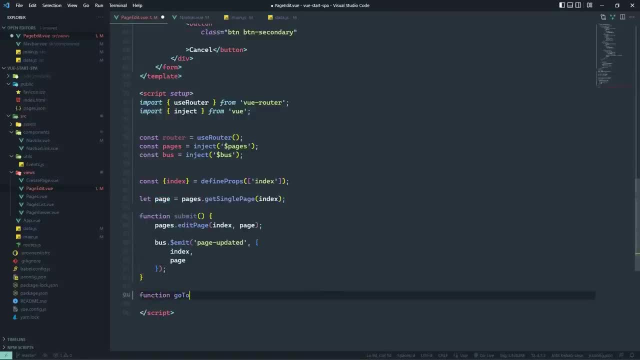 Let's write a function called go to pages list. 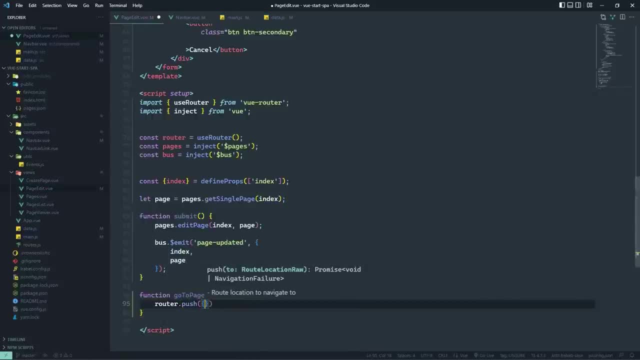 We will use this function to create a new page. We will use our router. We will push in the path to the pages view, and then we can call go to pages list inside of submit. So that after the page is updated, after the event is emitted, then we will go back to the pages list. 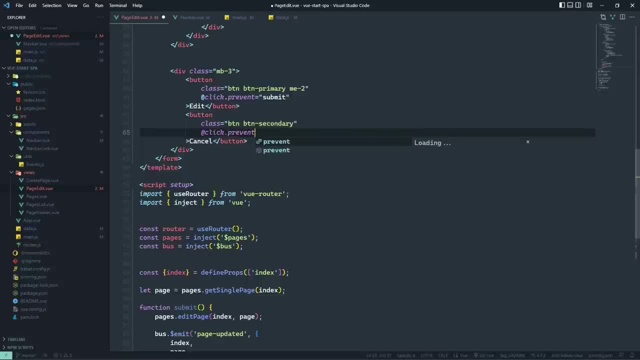 And then for the cancel button, we can handle the click event using that to go to pages function. 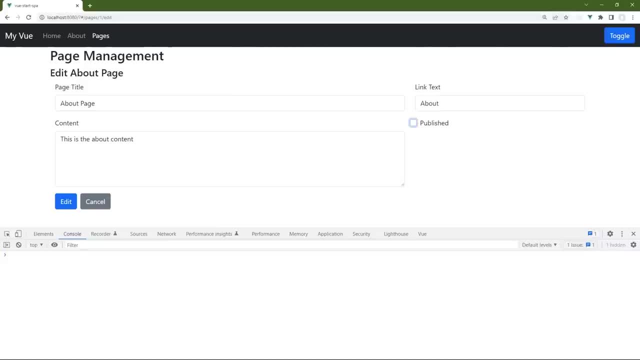 So now let's test this out again. Let's unpublish about, we click on edit. We go back to the pages list, 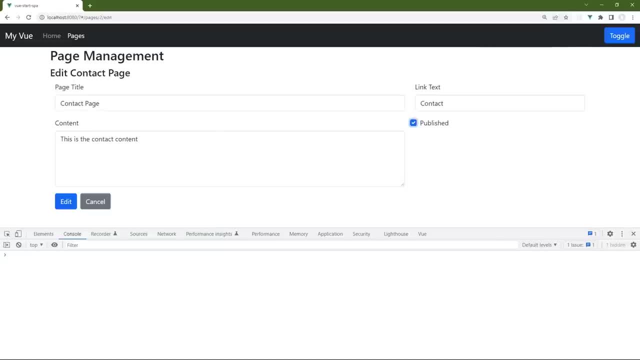 but I want to add contact. So let's go to contact let's publish and let's edit. But of course, all we've been checking is published. 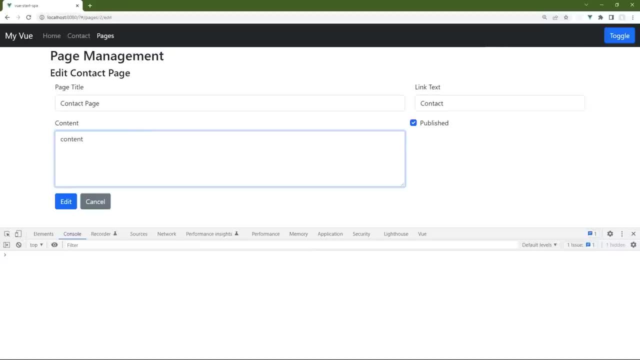 So let's change the content of the contact page. 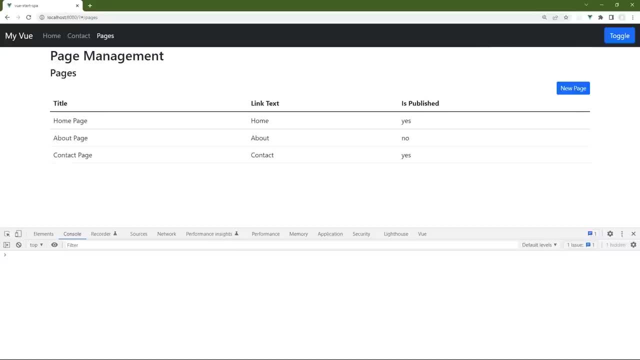 We'll say contact content goes here. Let's save it. 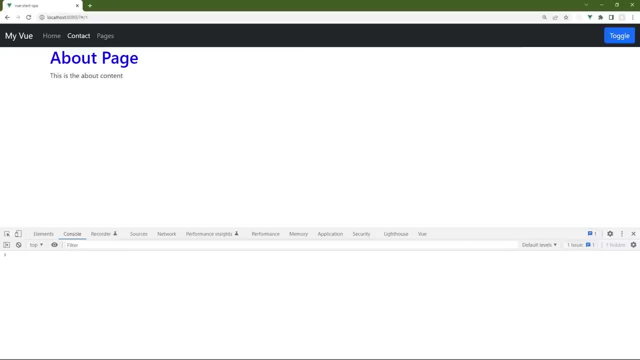 Let's navigate to contact and well, yes, there is a bug because we are relying upon indexes as opposed to actual IDs. So that is actually correct. At least as far as the code is written, we need to go to index two because that is the actual index. 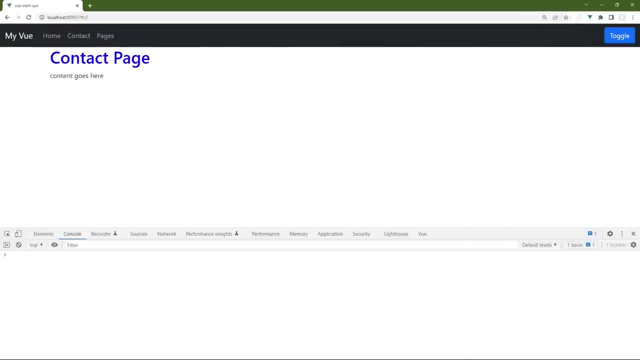 So here we can go to contact. We see that content goes here. 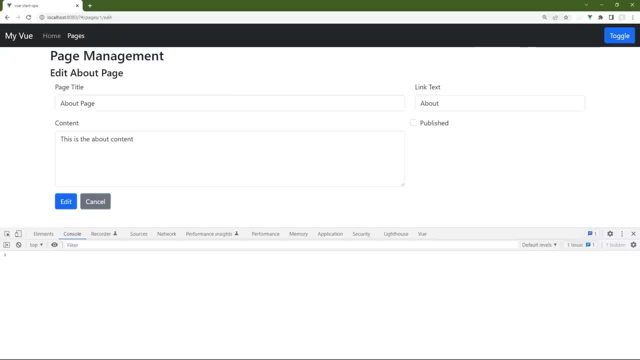 Let's unpublish contact. Let's go to about let's publish that. 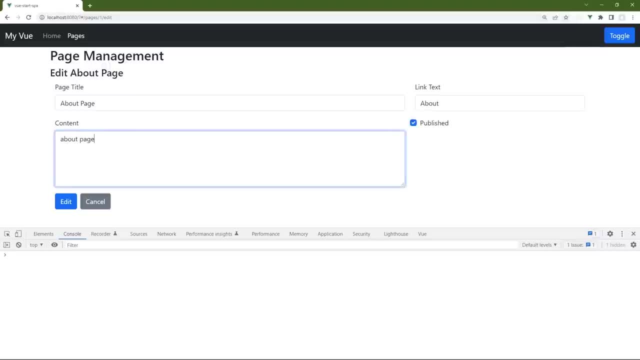 Let's change the content of about let's just say about page. And so now whenever we go to about our edits are 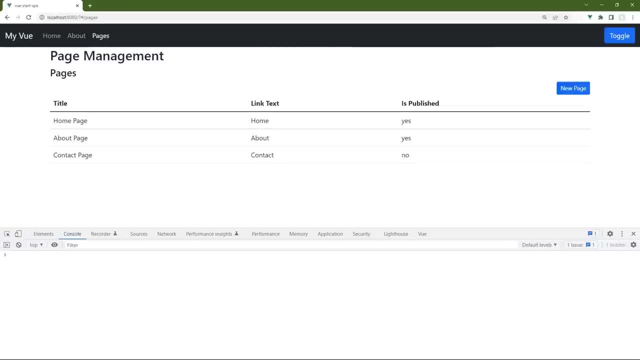 indeed updated. So we now have the functionality for editing. 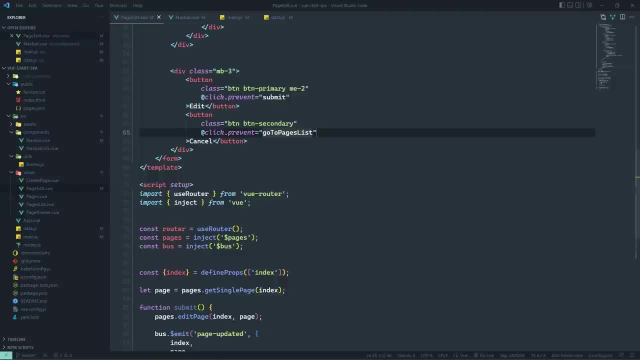 Pages in the next lesson, let's implement the code for creating a new page. 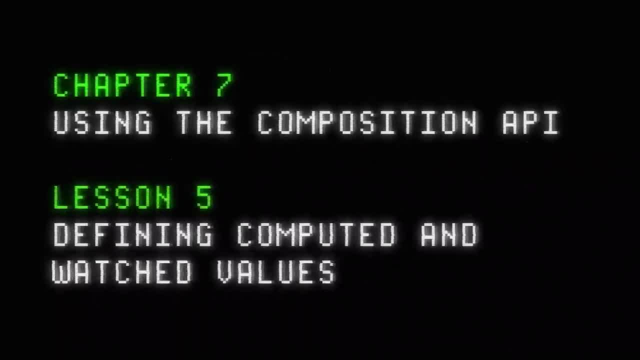 We need to revisit the create page view because we haven't done so since we started using the view router and we centralized our data store. 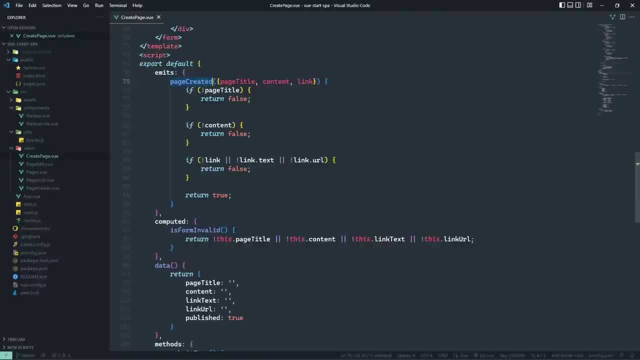 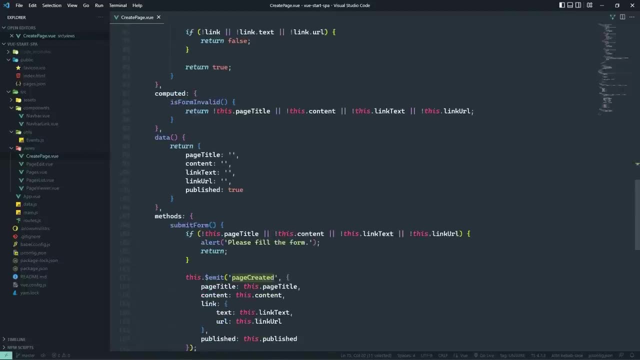 So I want to transition this from the options API into the composition API, because this is going to give you the opportunity to see how we can define computed values as well as watchers. 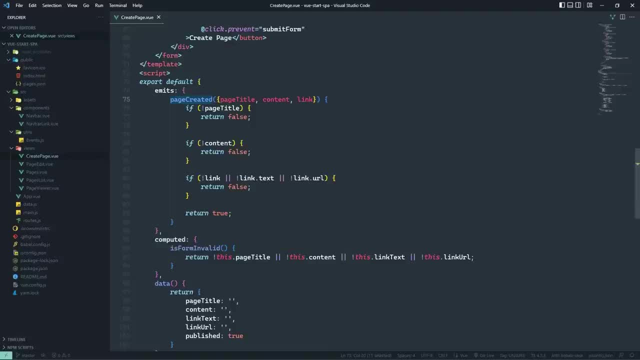 But we also, we need to discuss what is and isn't going to transfer over. 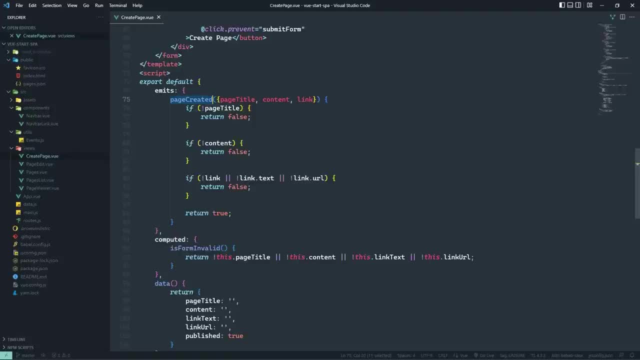 Because like the page created event is not. If you'll remember, 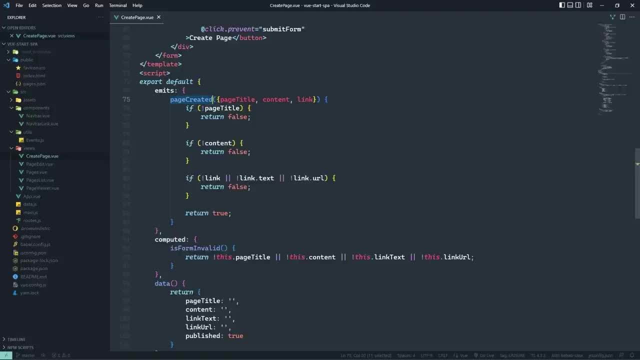 the create page view was a direct child to the app component. And we used the page created event to tell the app component that, hey, this page is created so that you can add it to the pages array. But now the create page view is rendered thanks to the router. And we will need to use our page. 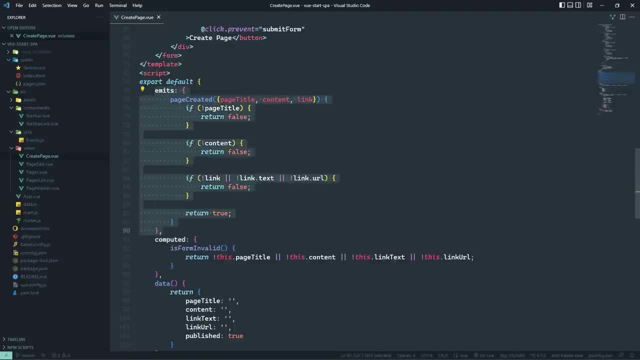 Our global event bus to tell the rest of the application that a page was created. 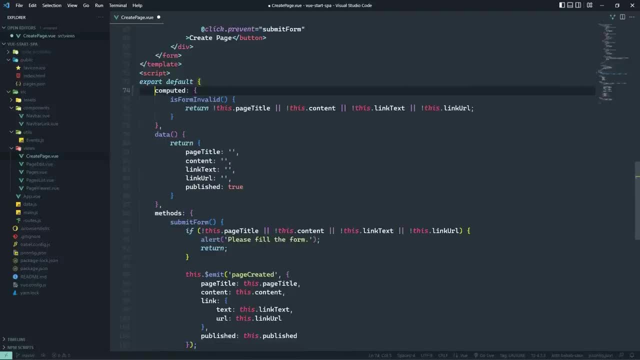 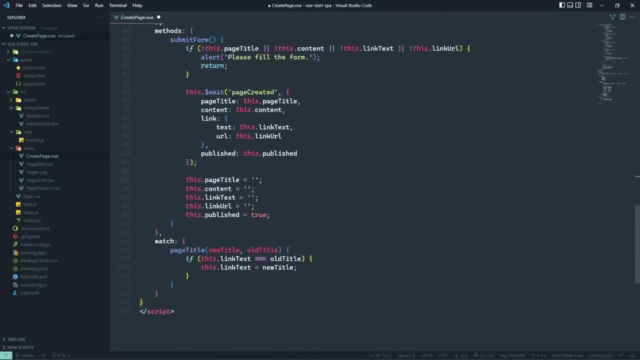 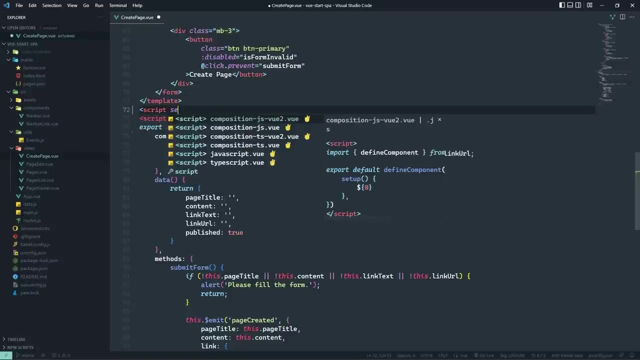 So we don't need this emits anymore. We will still need our event bus, but we will get to that. So as far as everything else, computed data, our methods and our watchers, everything else should transfer over just fine with a few modifications. So let's go ahead and define our scripts for our setup. 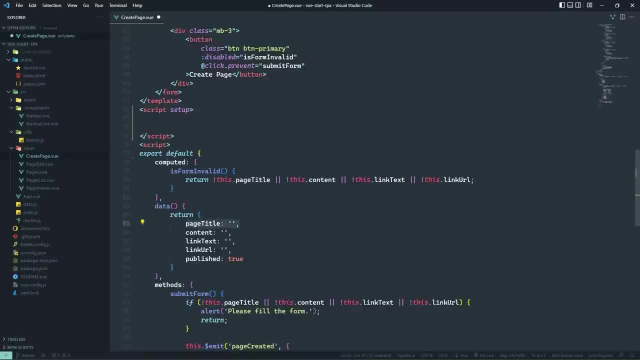 And we will start with our data. Now we have two options. We can create individual, 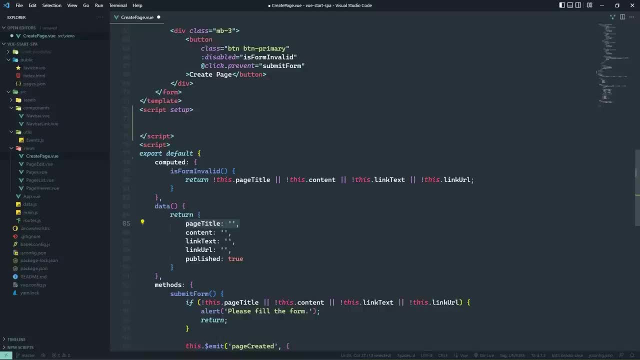 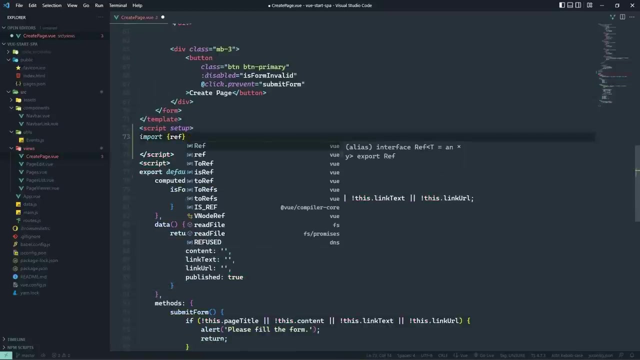 individual variables and use the ref function to make them reactive. Or we can use the reactive function and then make this entire object reactive. Now it's a little tedious, but I'm going to opt for the ref approach. Because I would prefer to just work with simple variables as opposed to having to use an object to get to the property that I wanted to work with. So we're going to import ref from view. 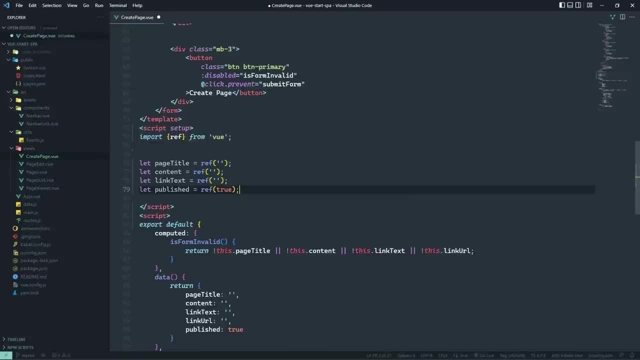 Then we will define those variables. Now by taking this approach, it means that we don't have to make any modifications to our templates. 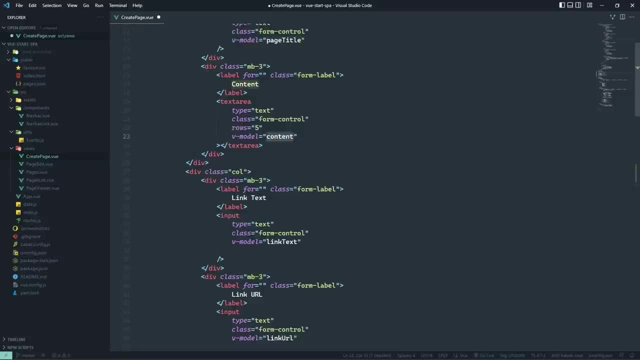 Because the V models for all of these fields are just simple values. So we're good to go there. 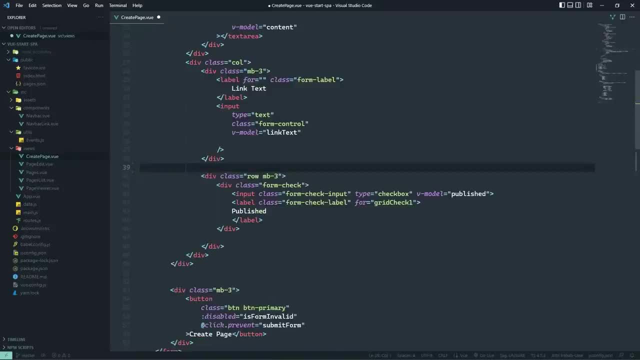 Although let's get rid of our link URL because we don't need that anymore. So now that we have our data, 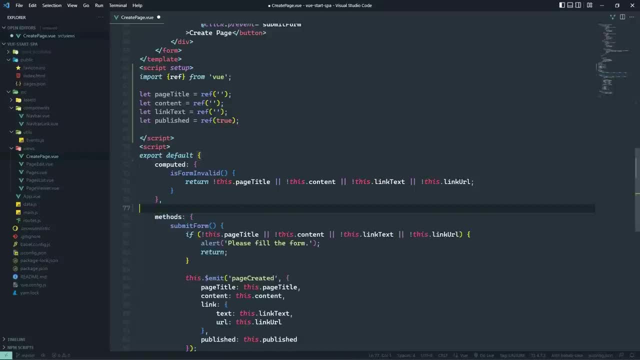 let's just get rid of that data option so that we can keep track of what we have and haven't implemented. 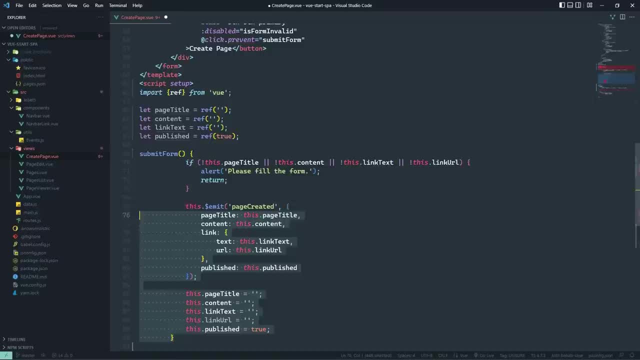 Let's paste that into our new script element. And of course, we will need to make some changes here. The first is that we no longer are using this. We have just simple variables so we can get rid of this dot on just about everything. But in this case, we need to get rid of link URL. We can also get rid of these lines that reset the form. 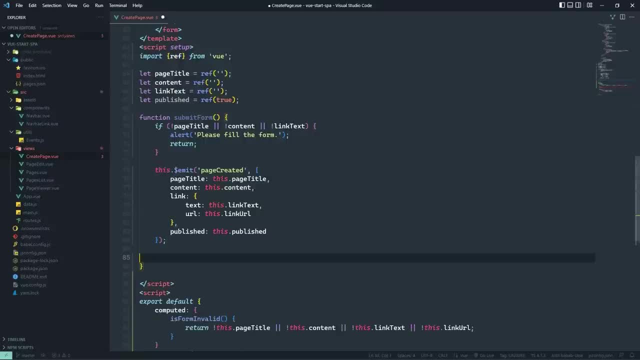 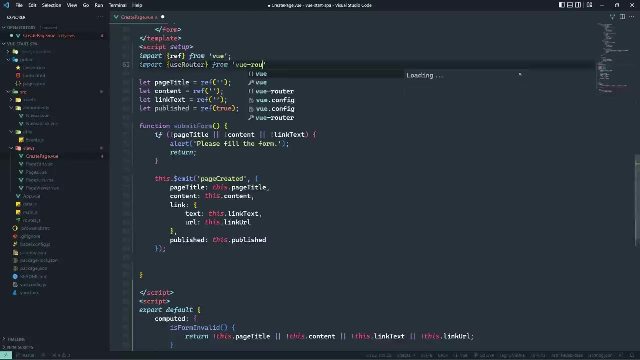 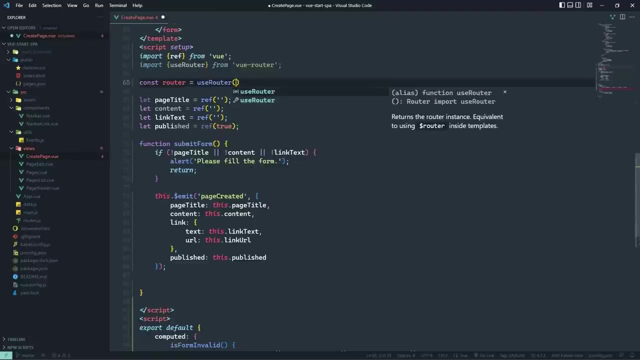 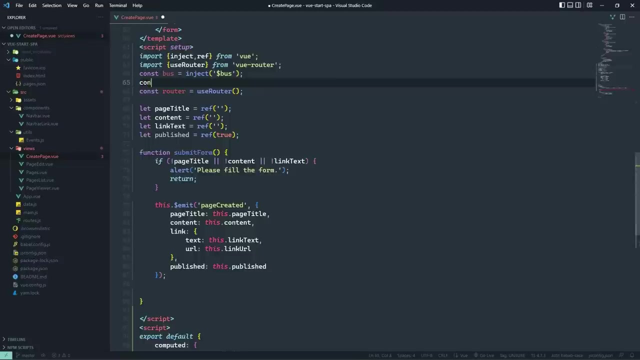 Because I want to follow the same behavior that we did from the edit. Form so that whenever we create a page, we just take the user to the pages list. So we will also need to import the use router function. So that we can get the router and we can navigate. So let's go ahead and do that so that I don't forget to do that later. And we will also need our event bus so we can inject that. And since we're doing that, we might as well go ahead and do our pages as well, cuz we will need to interact with our data store. And so when it comes to emitting this page created events, we will need to use our bus here. 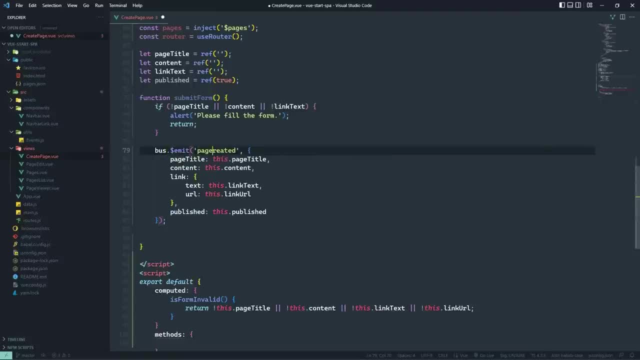 And I'm gonna change the name of this event because for our edit view, I used a hyphen to separate the two words. 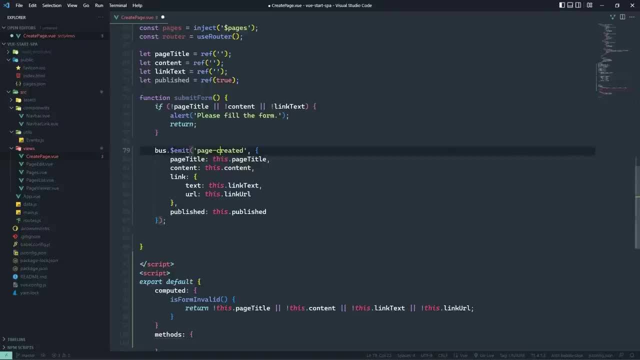 Since this is our own event bus, we don't have anything to translate between the different naming styles between using dashes and then a camel case. So, we're gonna go ahead and do that. 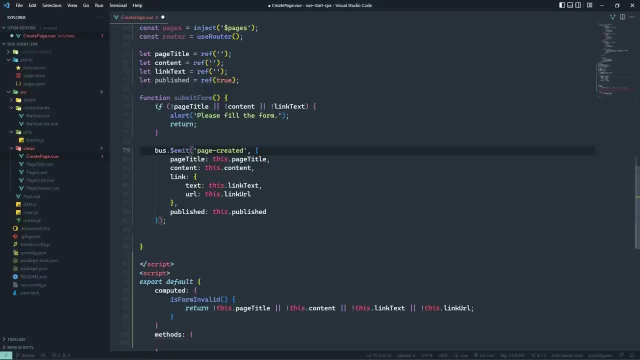 So instead of going back and changing what we did for the edit form, I'm just going to make this one follow suit. So we'll call the event page created. 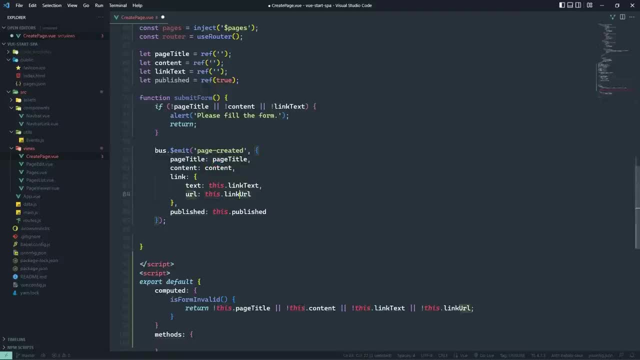 We don't need this in front of all of these values. 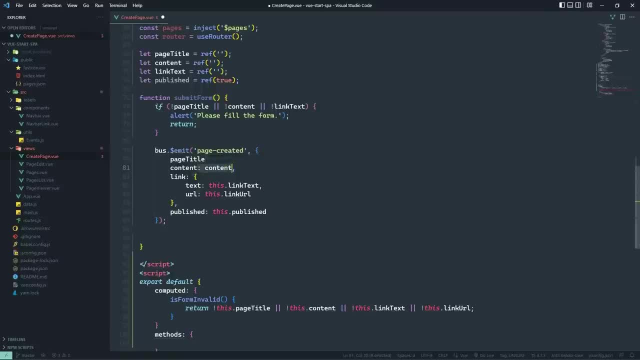 In fact, we can just simplify this by using the names of the variables. Although for the texts, we will still need link text, but 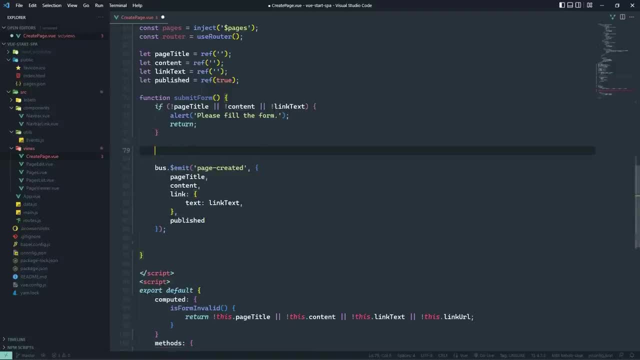 everything else should carry over fine. And then before we emit this, we will need to add this page to the list. So we'll add this page to our data store. So we'll call the method addPage, we will pass in a page object. So let's do this, we will create a page object. We'll just call it newPage, set it to that object so that then we can pass newPage to addPage. 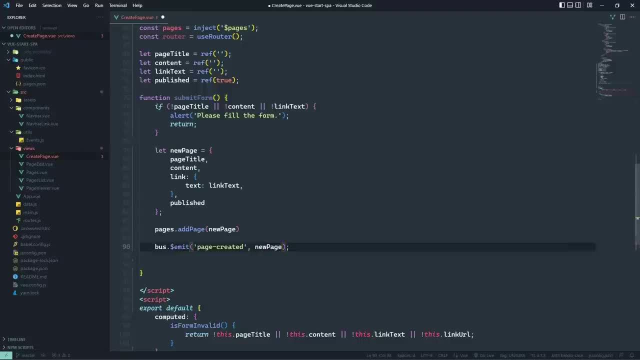 And then we will do the same thing for the page created event. And after that, we will use our router to navigate to slash page object. 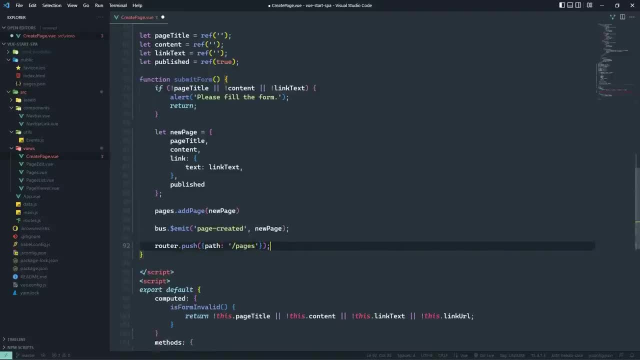 And so that should be that for the submit form function. 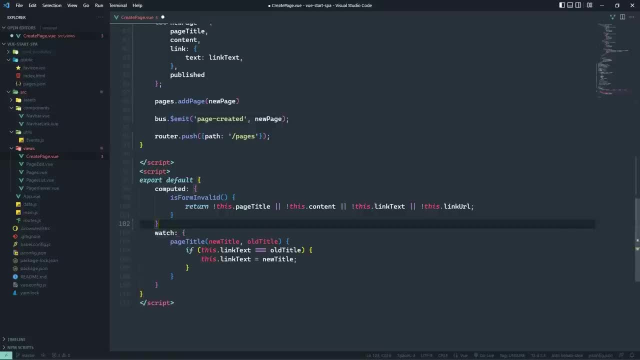 So let's get rid of our methods. Now our computed and our watcher, all we have to do is import 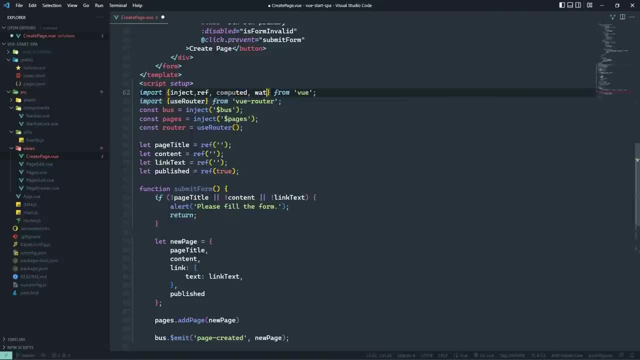 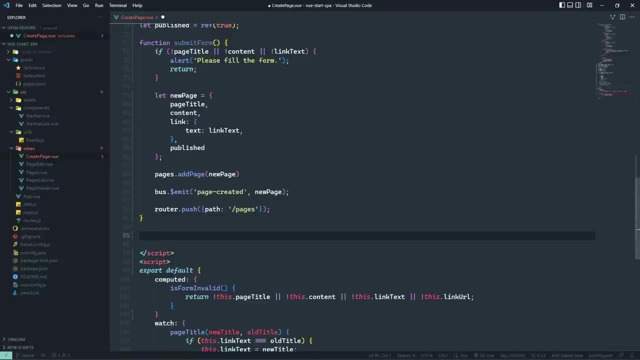 a function called computed and another one for watch. And setting up a computed value using the composition API is almost exact. 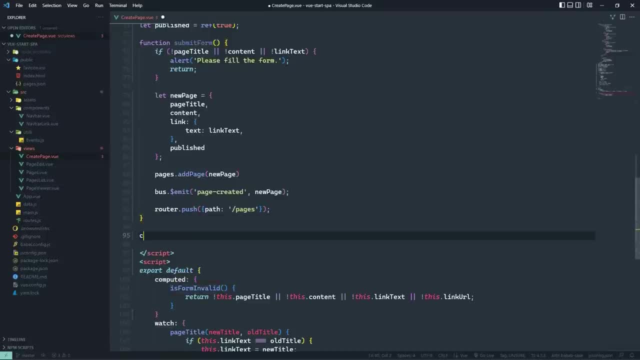 Well, it's not almost exactly. What we want to do is create a variable with the same name as the property. 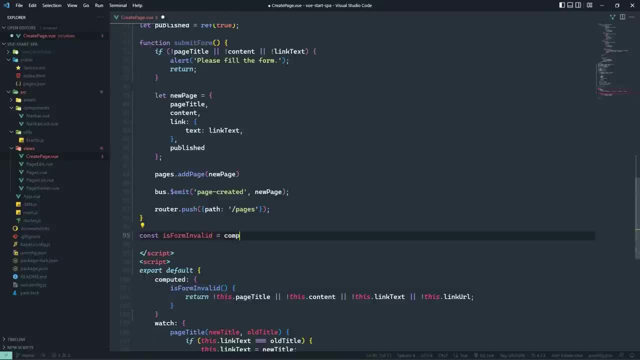 That we used in the options API. And then we will call the computed function. This accepts a callback function that is going to do whatever it is that we need to compute, which in this case was just checking the values of our form. So we will essentially do the same thing. 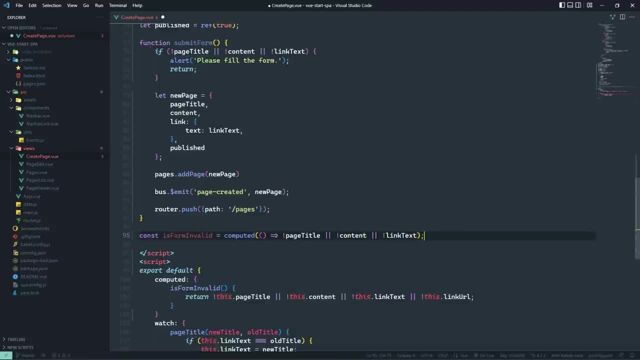 Let's get rid of this because we don't need this, and that should be that. 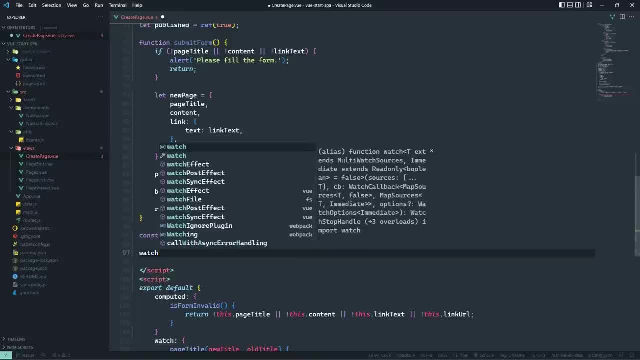 Setting up a watcher is also very simple. We call the watch function, we pass in the value that we want to have, and we pass in the value that we want to watch, which in this case was simply page title. 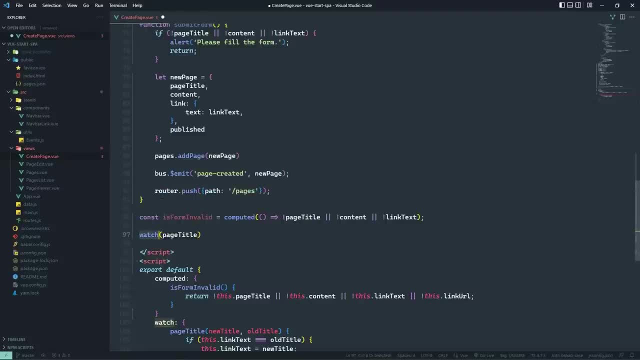 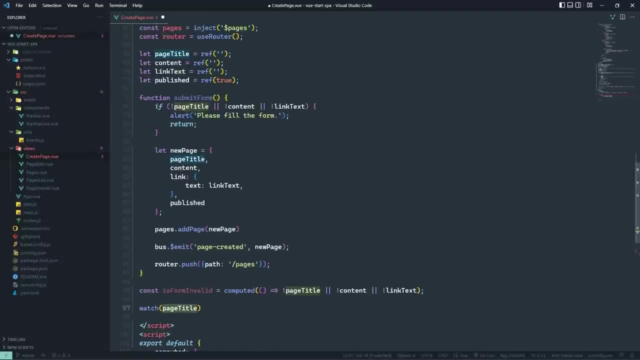 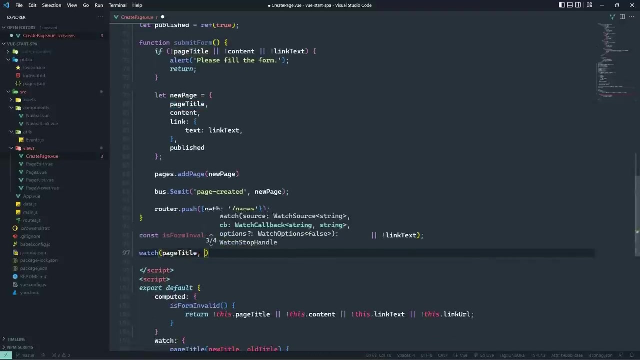 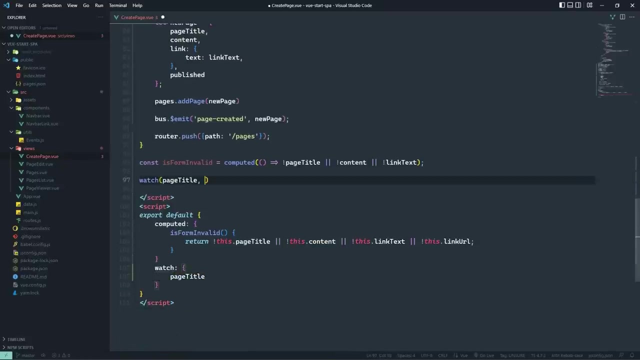 Now, there is some rules about setting up a watcher. And that whatever it is that we are watching has to be reactive. So that means the value has to be created by calling ref or reactive. So keep that in mind. But then we also pass in the callback function that will execute when that value changes, which we can essentially just cut out the code from the watcher, from the option. So we can see that we have a callback function, which we can actually use in our functions API. 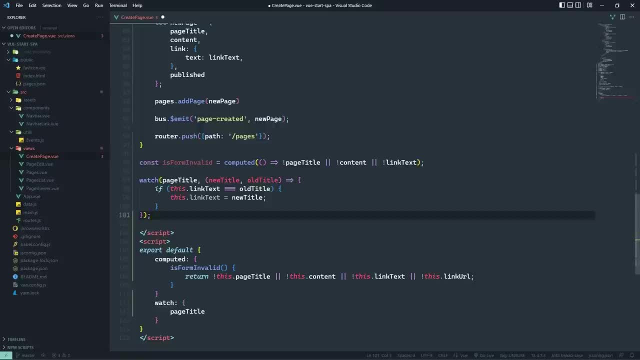 We do need to use the correct syntax here using our arrow function. And of course, we want to get rid of the usage of this. But other than that, it's the same function. And with those two things implemented, we can get rid of the old script element altogether. So that should be good. 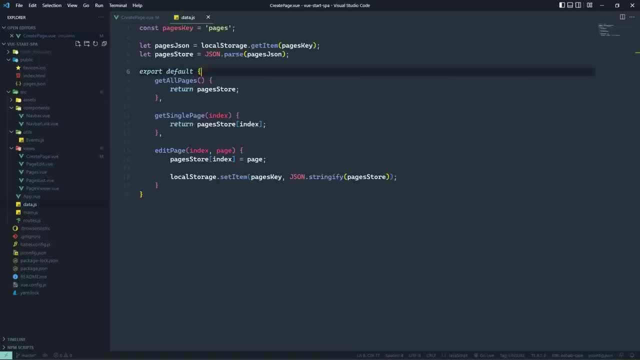 Let's go to our pages and not our pages. We need to go to our data and we need to add that add page. It sure is. 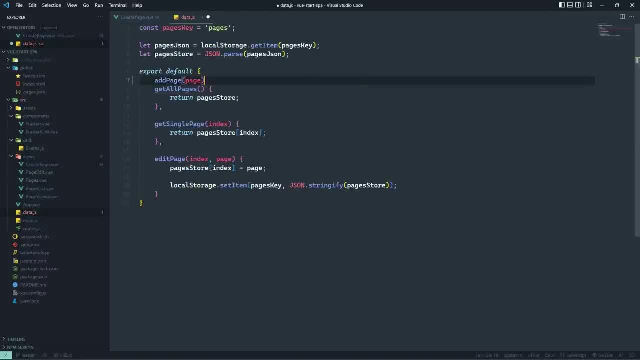 So let's add, add page. And all we need to do is push this into our pages store. 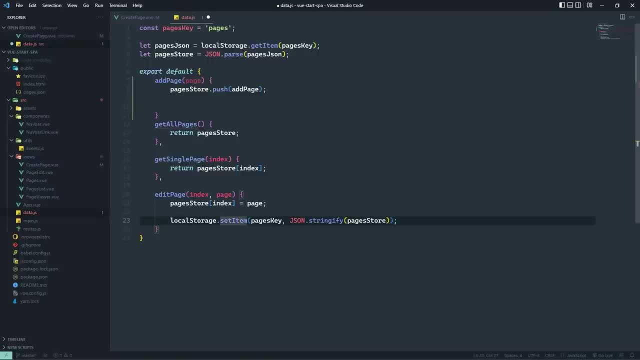 And then we need to save that. So we will save it back into local storage. And that should be that. 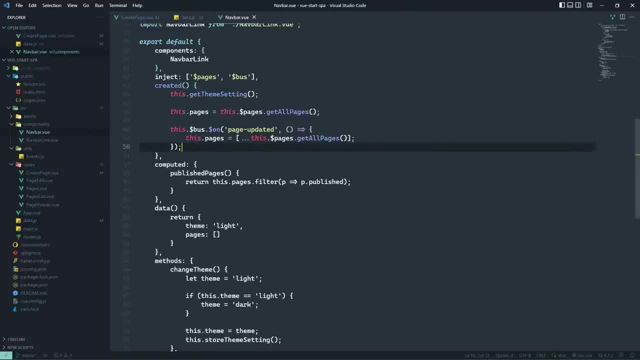 And then we need to go to our navbar because after we add the page, we need to be able to listen for that page created event so that we can redraw the navbar. So I'm just going to copy and paste, change the name of the event. And that should be fine. 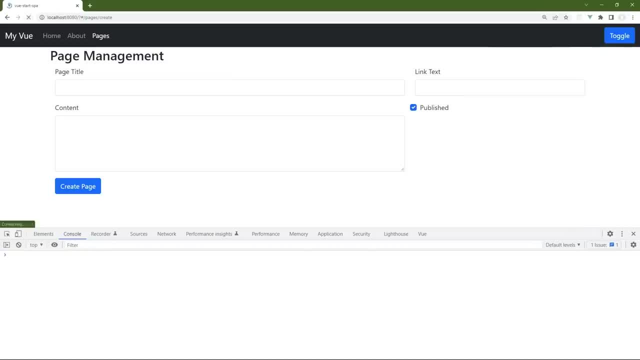 So let's go to the browser and let's refresh. Let's see if we get any errors or warnings. Everything looks good. 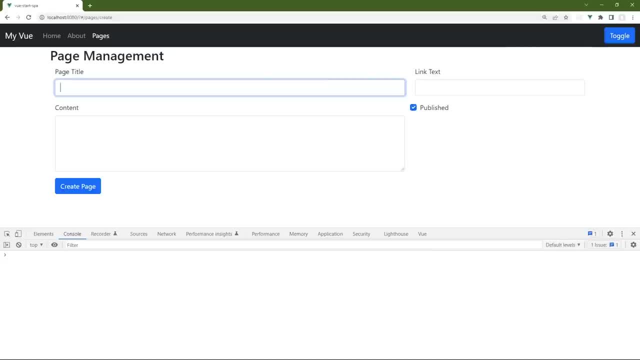 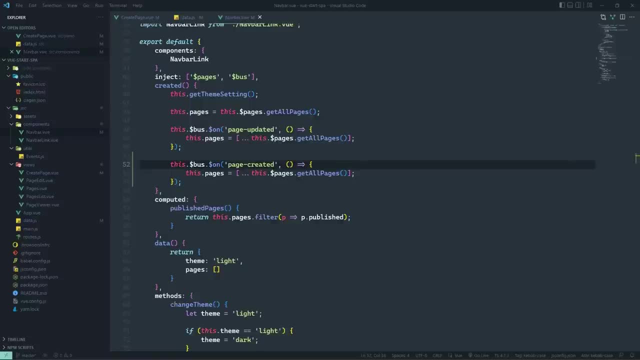 So for the page title, let's just start typing. We'll have new page. Now our link text was not updating automatically. And I know why. 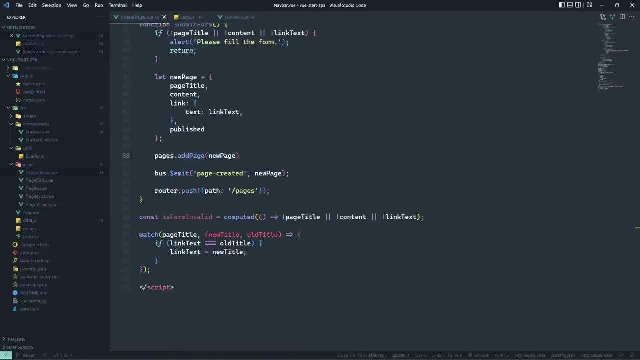 That's because we didn't use the value property. 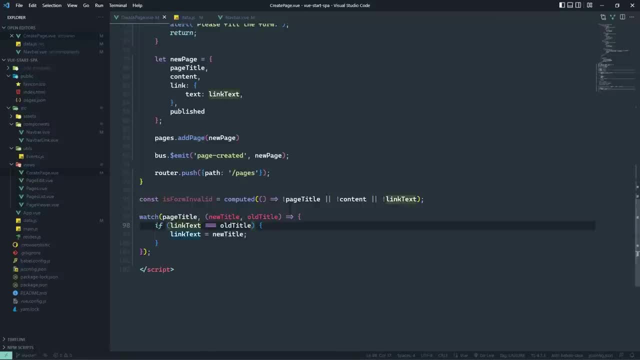 Whenever we set the value for link text. So we want to check if link text dot value is equal to the old title. 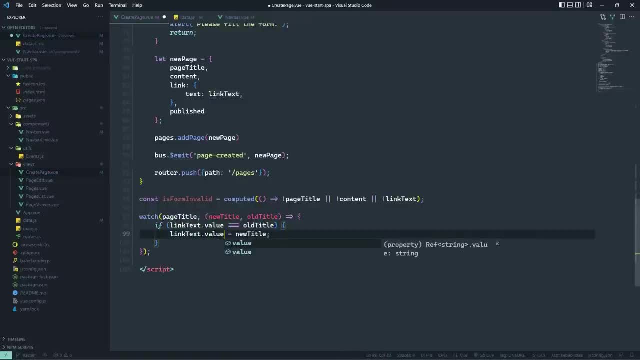 In which case, we want to set link text dot value equal to the new title. 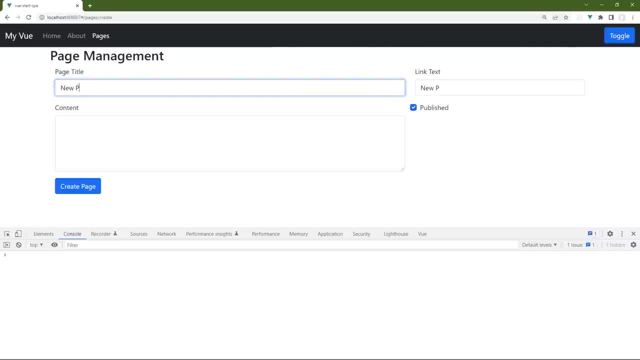 So let's go back to the browser. Let's try this out. New page. There we go. We have that functionality. Let's change the link text. 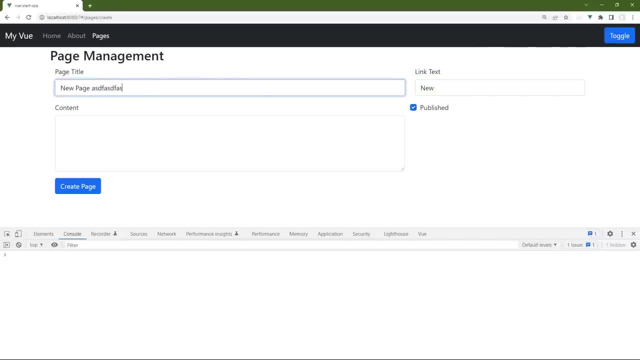 And then let's change the title again. We can see that it's behaving the same way that it did before. So that's always a good thing. 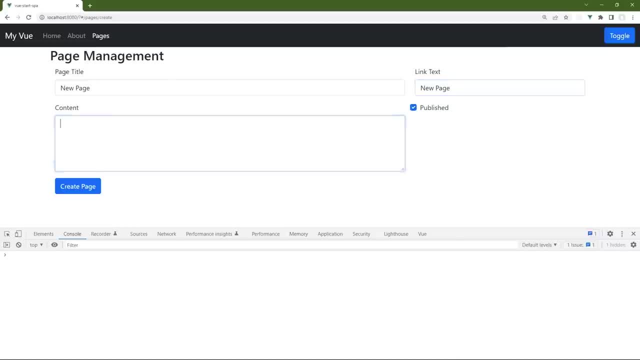 But let's have the page title and the link text as the same. As far as the contents, we don't care. We just need some content. Let's make this published. 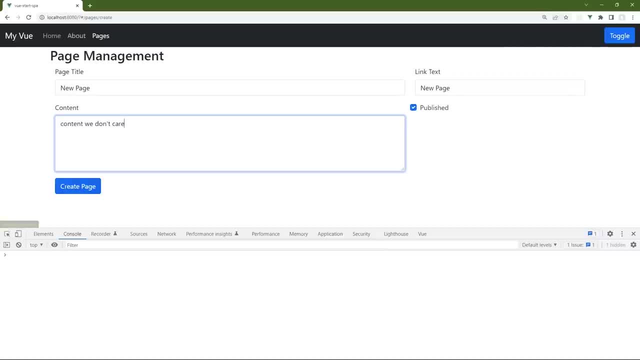 So whenever we click on this button, it should add the link to the nav bar. It should navigate us to the pages list. 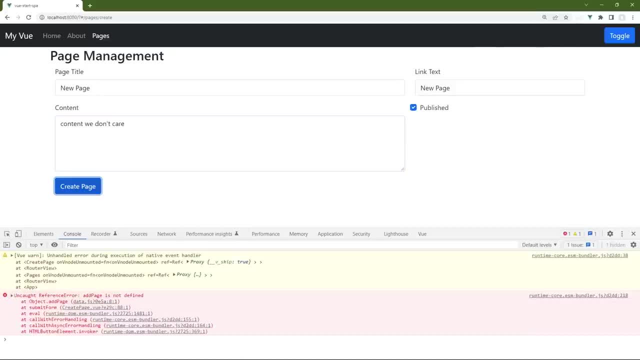 And no, we get an error. Add page is not defined. 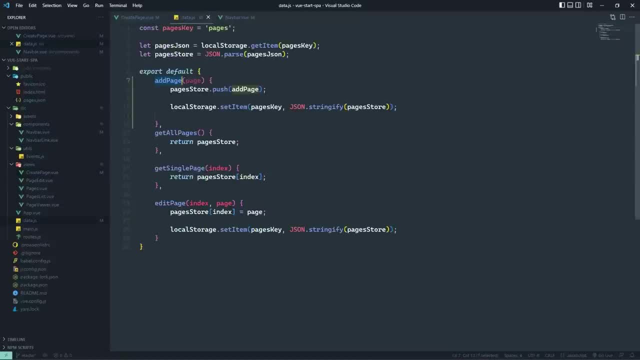 Now I know we wrote that. Add page is right there. Oh, there we go. Yeah, we need to do that. We need to do that. We need to push page there. Let's go back to the browser. 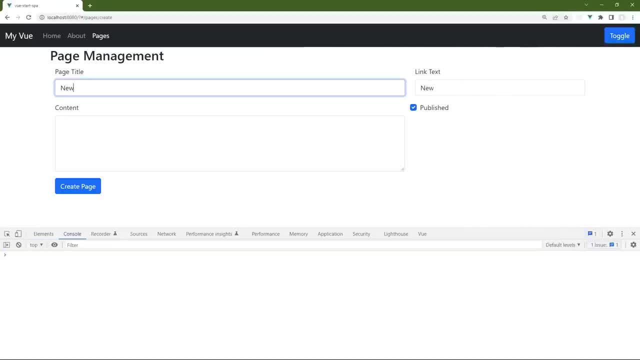 Let's do a hard refresh. And let's try this again with new page. The content doesn't matter. 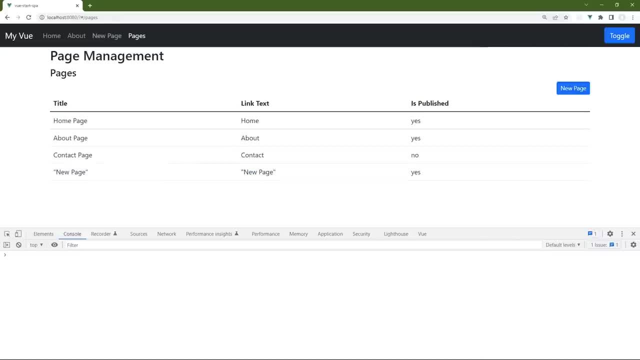 And let's click on Create Page. And there we can see that new page was added to the menu. 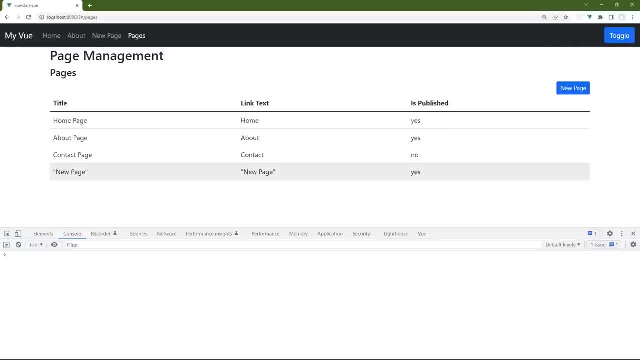 The title and the link text are strings. And now that I think about it, I think I know why. 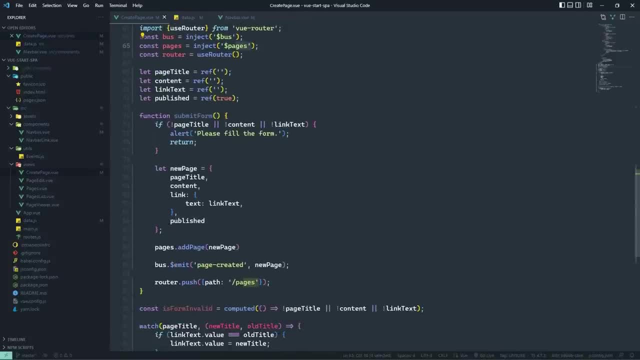 Let's go back to our create page. Cuz whenever we create this new page, we're using page, title, content, link, text, and publish. 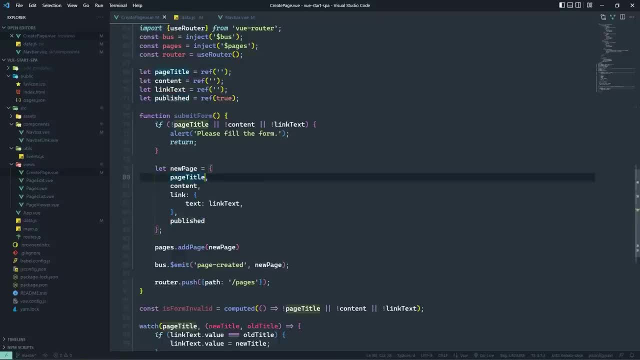 These are refs. We need to add the value. So this needs to be pageTitle.value. And we will do the same thing for all of the other values. 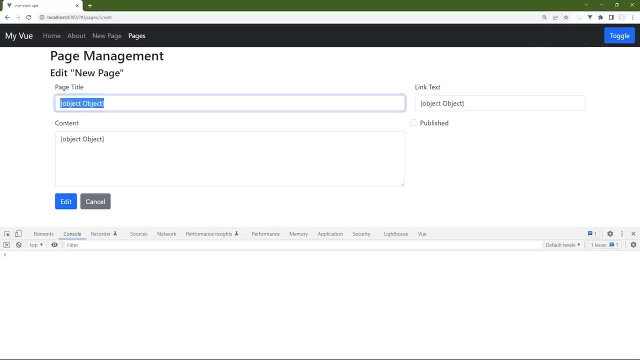 It's always the little details that end up biting you. So let's try this again. 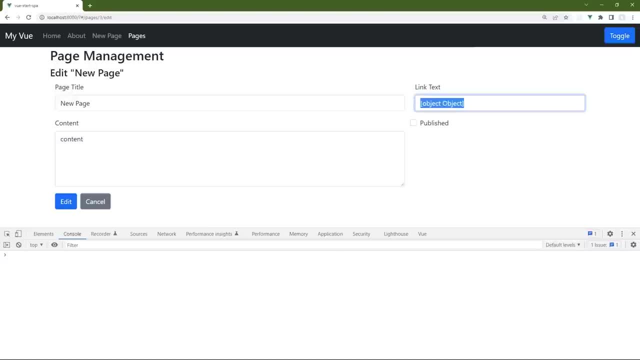 Let's change this to new page, the content, the new page link text. Let's do that. Let's do something completely different, and let's edit. 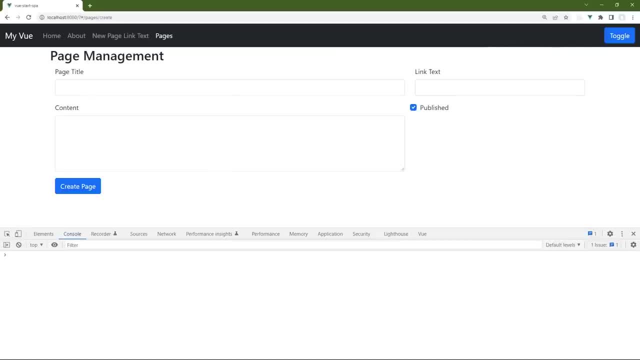 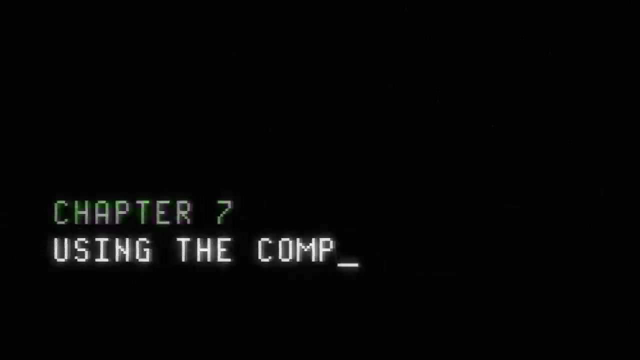 Okay, there we go. That looks like it should, but let's make sure that everything's okay. We'll say new page, content, create page, and there we go. So now we have the ability to create pages. We have the ability to edit them. We can navigate to those pages, and deleting them should be very simple. And we will add that functionality in the next lesson. We need to provide our users with the ability to edit pages. 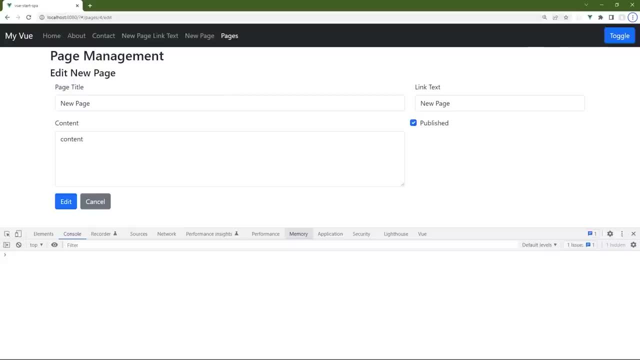 And we have a couple of different options when it comes to implementing this. 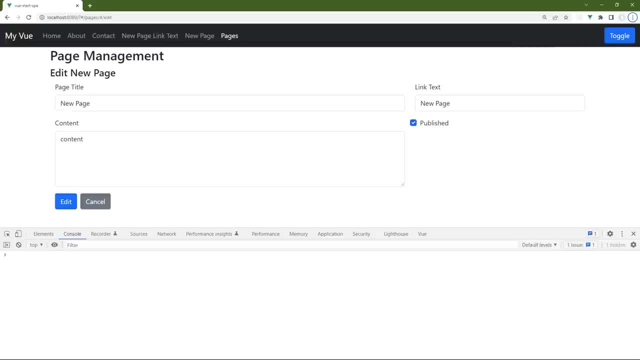 So we could add a delete button to the edit view, which kind of makes sense. Because that would force the user to have to click on the page in order to then click on the delete button, kind of like a two-stage confirmation. Are you really, really sure you want to do this? 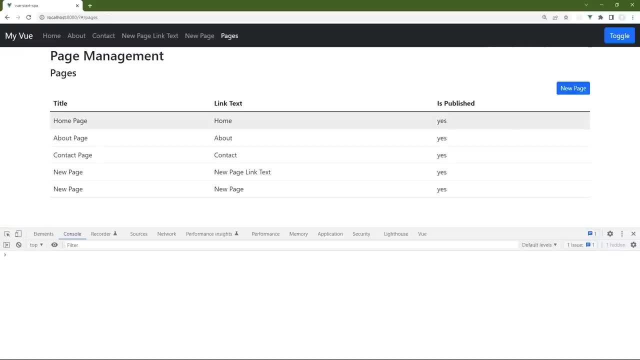 Another option would be to add a delete button to the pages list, over on the right-hand side. And then we could add a delete button to the pages list, you know, over on the right-hand side. And then we could add a delete button to the pages list, you know, over on the right-hand side. And then we could add a delete button to the pages list, you know, over on the right-hand side. So that they could just easily delete that. 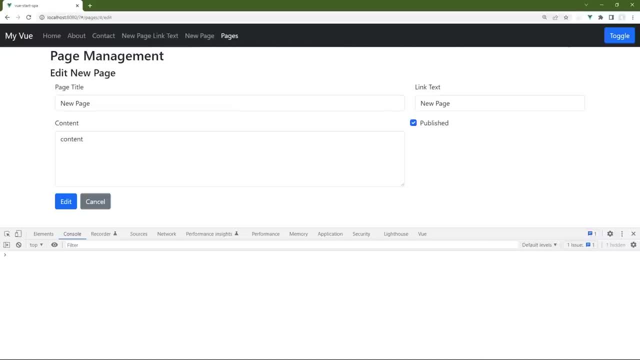 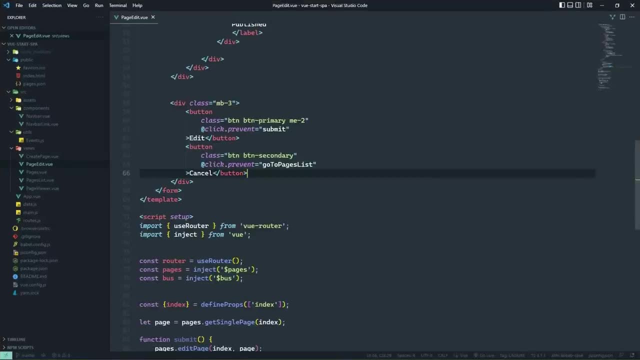 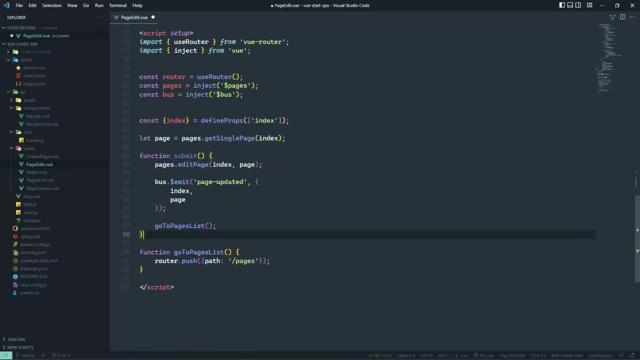 We could go either way. I'm going to lean towards implementing the delete on the edit page. So let's add another button. And ideally, it would be completely separate from the edit and cancel. But we're just going to keep things simple and put it right next to each other. As far as the coloring is concerned, I'm going to use the danger class. The text will just be delete. And then for the function, let's call it delete page. And let's go ahead and implement that function, which should be relatively simple. 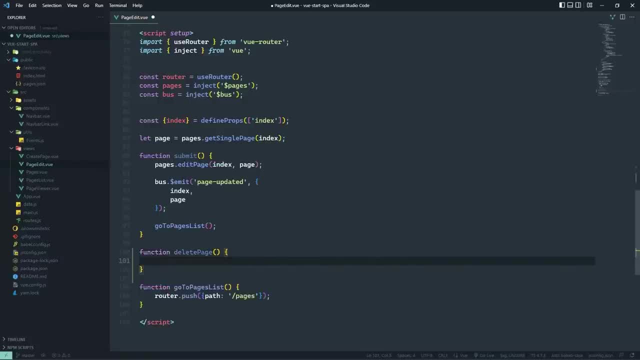 Because we have all of the information that we need. We just need to interact with our pages. And we could say that we have a method called remove page. We would pass in the index, and that would take care of that. But of course, we need to tell the rest of the application that a page was deleted. So we can emit another email. We could call it page deleted. And the only information that we really need to supply would be the index. I mean, I guess we could supply the page as well, but I think index is going to be fine. 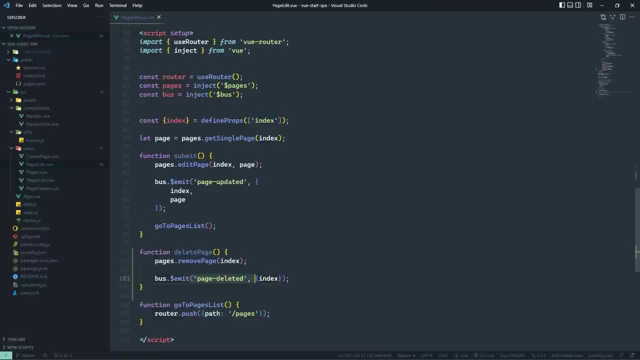 And really, the only thing listening for this is going to be the nav bar. So really, it doesn't need to know. But again, having that information available could be useful later on. 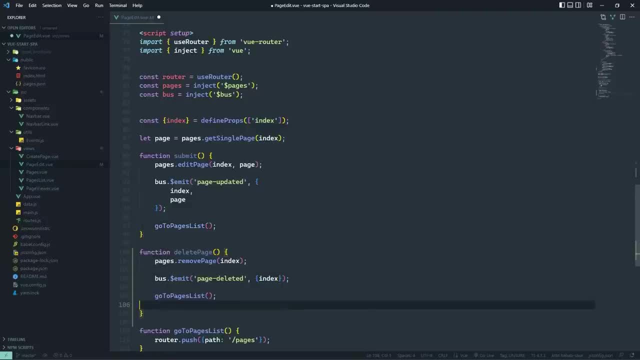 Now, of course, after we delete a page, we want to go to the pages list. So. We'll make that the last thing that we do inside of delete page. 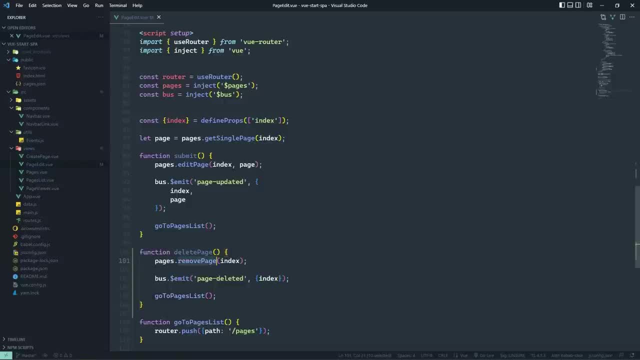 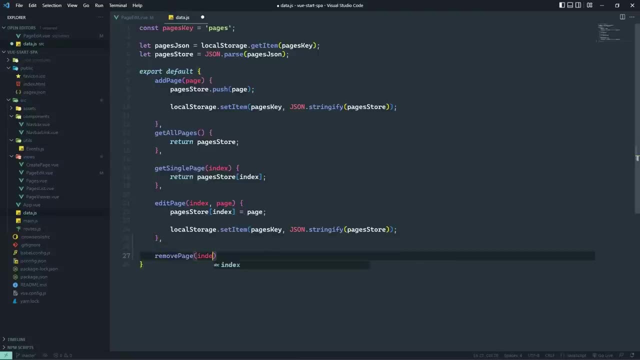 So we need to implement this remove page method. So let's go to our data store and let's add this remove page. We want the index. 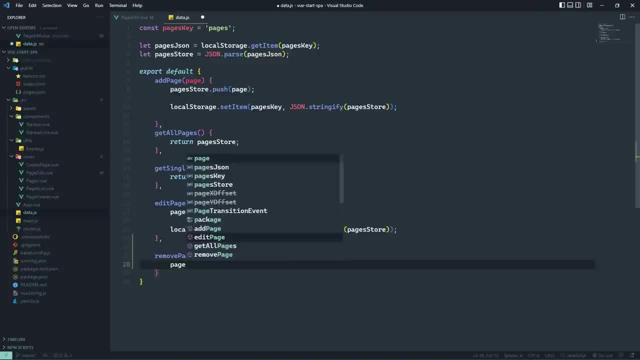 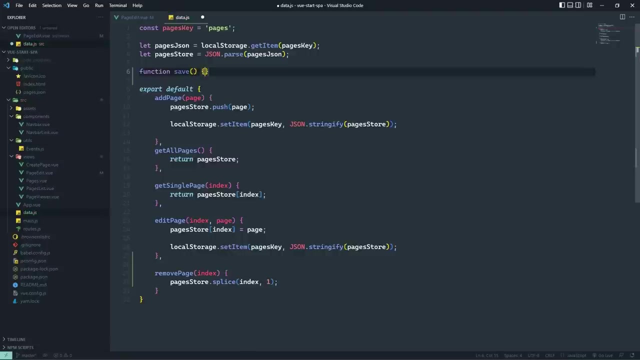 And all we really need to do is splice out that item at the given index. And then we want to save that. Now, since we have saved data two other times, let's just do this. Let's write a function called save to where we will save our data. That will make things a whole lot simpler and really easier to read. Then whenever we edit a page, we will save. And whenever we remove a page, we will save. And then, of course, we need to listen for that page deleted event inside of our nav bar. So let's go there. 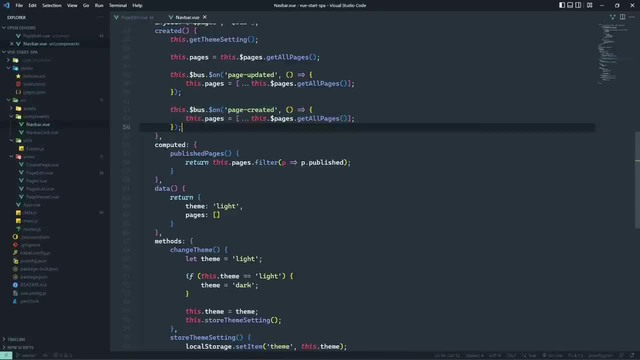 Let's set up another event listener. I guess if we really wanted to spend a lot more time on this, we could do that. 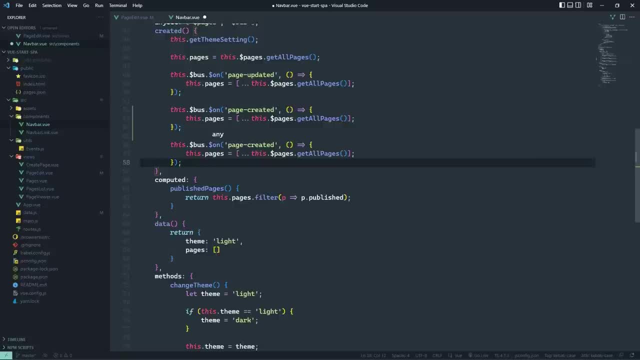 If we really wanted to spend a lot more time on our global event bus, we would add the ability to pass in an array of all of the events that we would want to listen to. 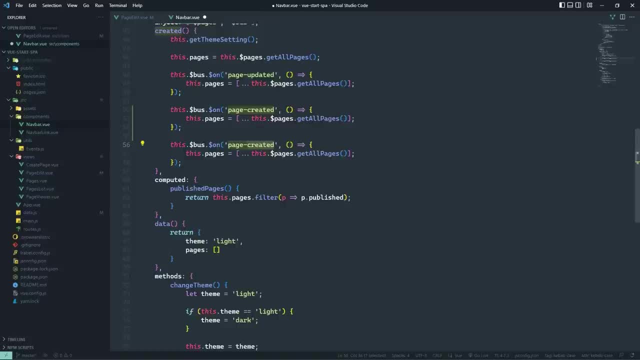 Because in this particular case, it really doesn't matter what happens. If we do anything to our pages, we want to update our list of pages that are displayed in the nav bar. 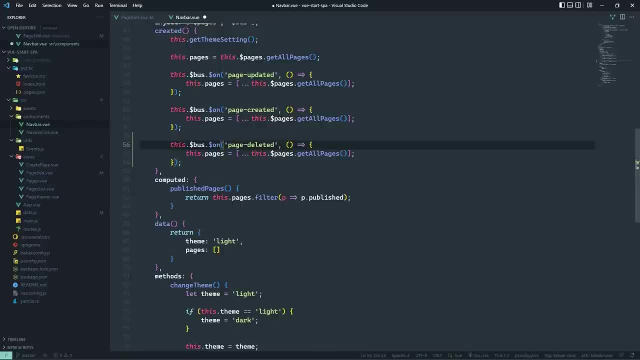 So it would save some time if we could pass an array of strings for the event's names, but this is going to be fine. 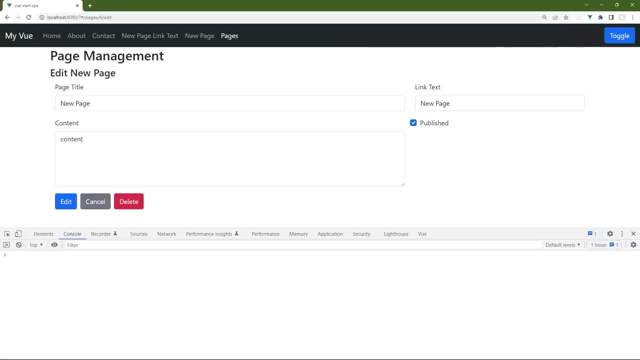 So with that in place, we should be able to delete a page. 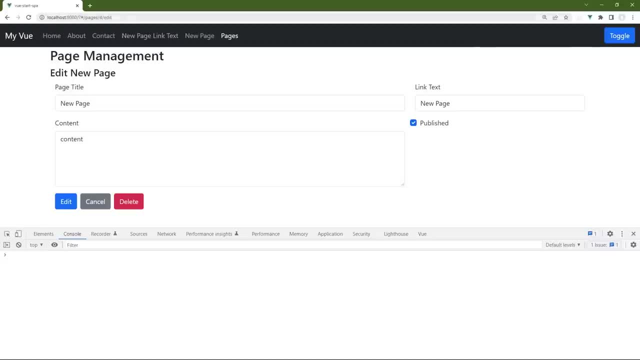 So here we have the one with the index of four. This is what, the new page. So if we delete this, there goes that page. Let's try to delete the other new page. That's gone as well. 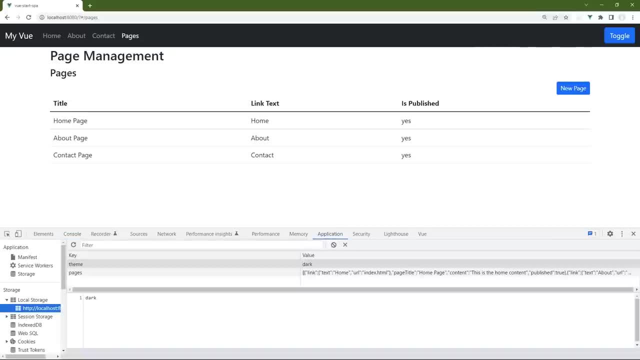 Let's make sure that we are actually saving that data. So let's go to the application, the pages. 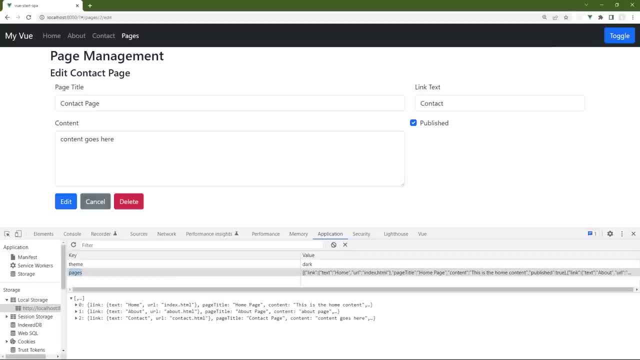 Yep, we only have three items there. So if we decide, okay, we don't want people to contact us, and 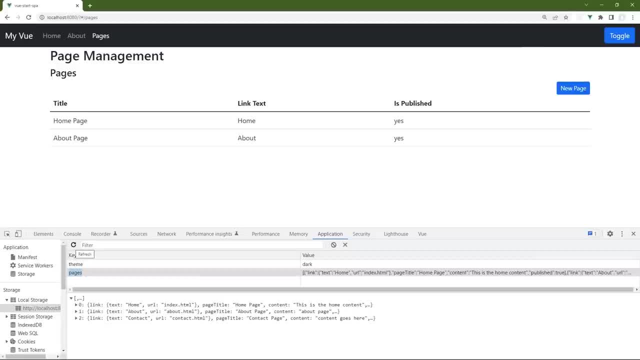 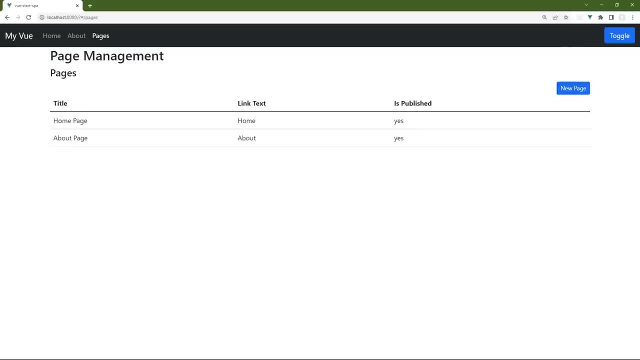 then that has gone as well, we can refresh the application tab, and sure enough. So we now have the ability to delete, edit, and create pages.